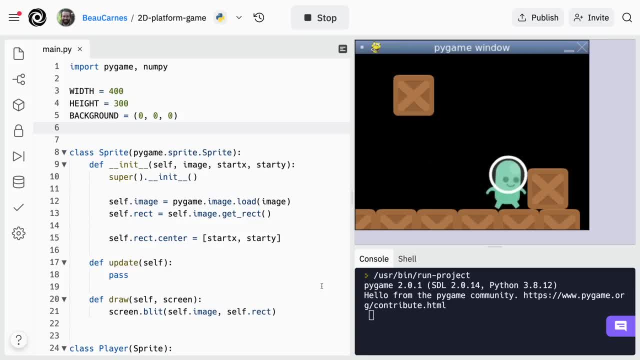 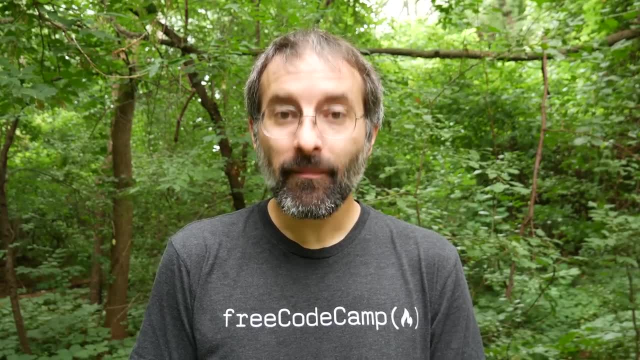 analysis and machine learning, But it can also adapt to create games and work with embedded devices. We're going to jump right into it so you can start coding your first Python program as soon as possible. To get started quickly, we'll use Replit. 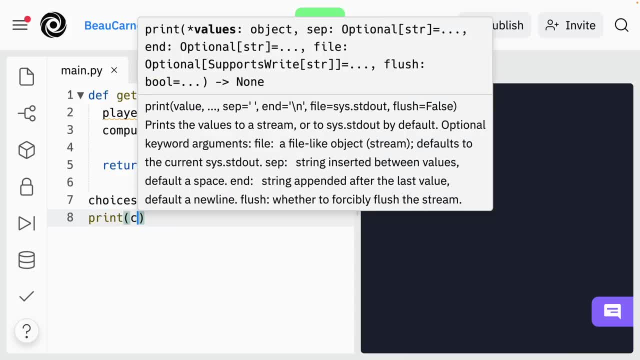 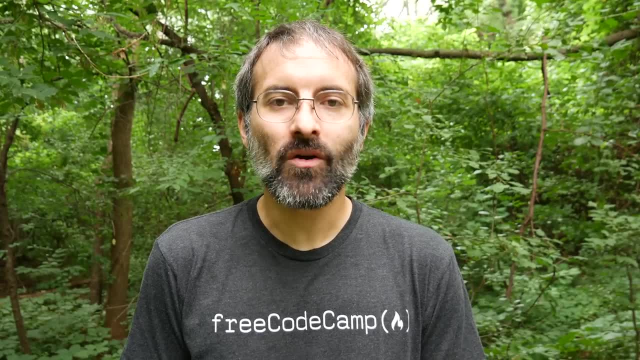 which is an online IDE that allows users to code and run programs in a variety of different languages, all in a web browser, And later I'll show you how to get Python set up on your local operating system. After the first project, I'll go into more detail about each. 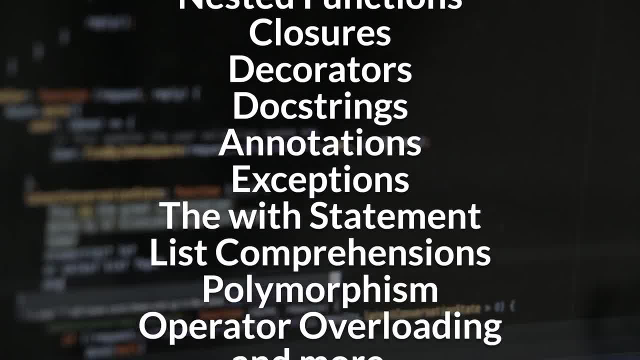 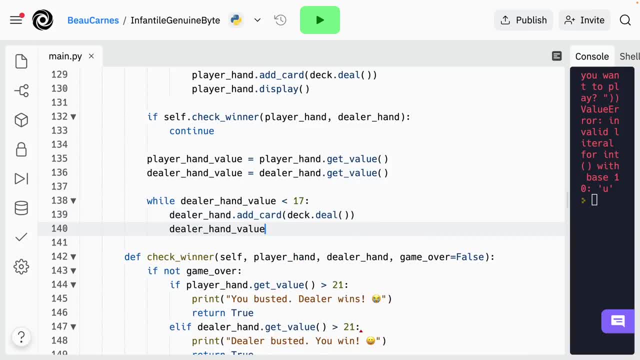 of the main features of Python. This section is comprehensive and detailed, And in the final section you will use what you've been learning to code a blackjack game, with me guiding you every step of the way Throughout the course. there will be a little repetition. 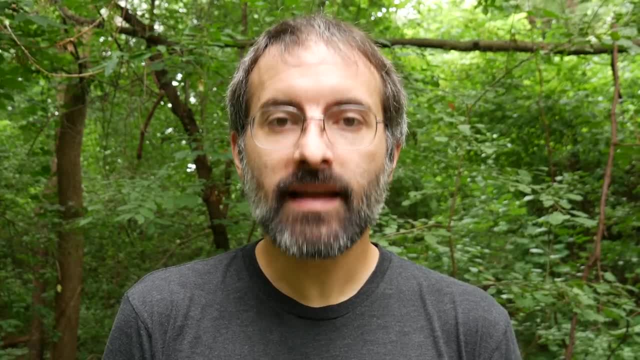 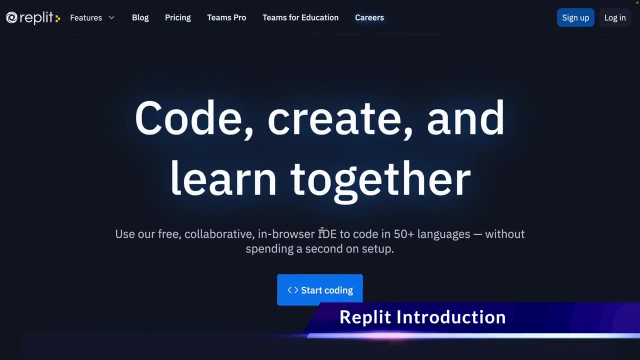 of some of the key Python programming concepts to make sure you have a deep understanding of the language. So let's get started. We're going to start by creating a simple rock paper scissors game And we'll start by going to replitcom. Replit provided a grant that made 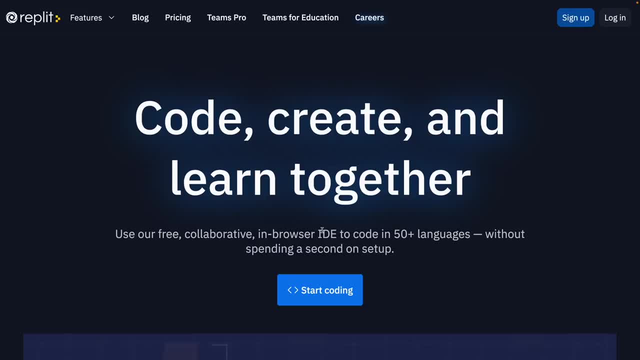 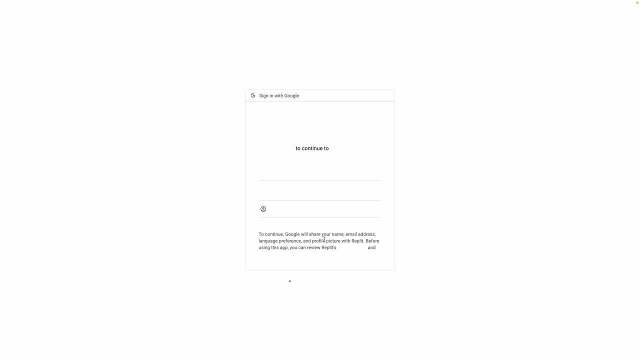 this course possible, And Replit is going to make it super easy to get up and running really quickly, So you can either sign up or log in and create an account. I'm just going to use my Google account. Okay, now that you're logged into replit, you can either 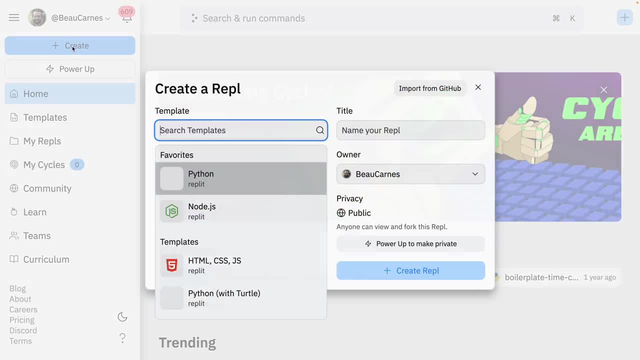 just click the Create button or this plus button over here to create a new replit, And I'll make sure to create a Python replit. But you can see, you can also select all sorts of different programming languages. Oh, these are just the ones that start with the word. 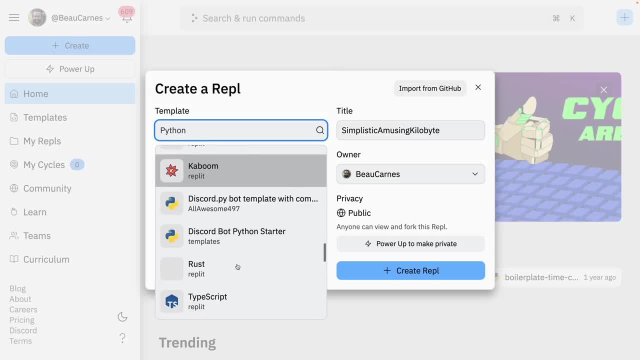 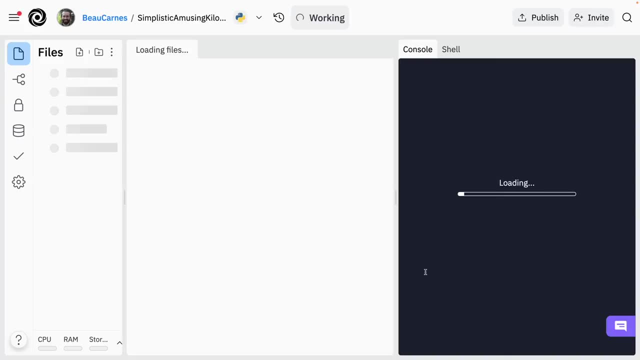 Python. But so there's there's tons of different programming languages you can select, But in this case we are just going to use Python And then I'll click create, And now I'm going to click Create REPL. Okay, so let me just kind of show off, replit a little bit This. 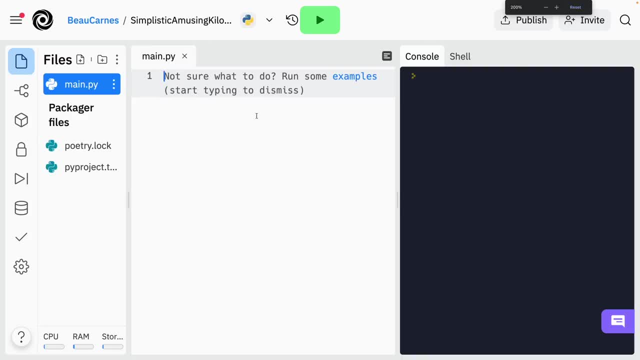 is where we're going to create our Python code. zoom in just a little bit. So we're going to write the code right here And then we can see some output over on the right side, And then you can create different files over on the left side here, And then there's some. 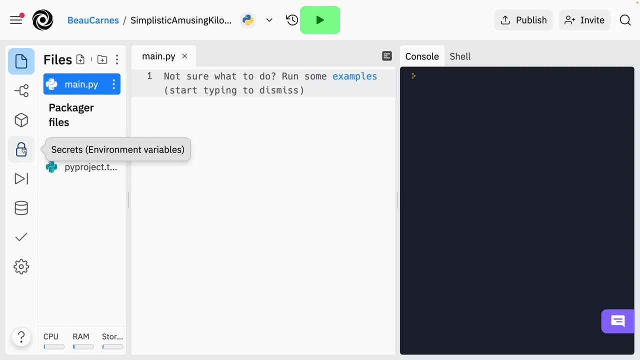 other things, like you can connect to version control And if you have environment variables. we're not even going to be discussing those in this course. There's a debugger, you can connect to a database and just some other things. But we're mainly going to just be using this main dot pi program to write our program And we're 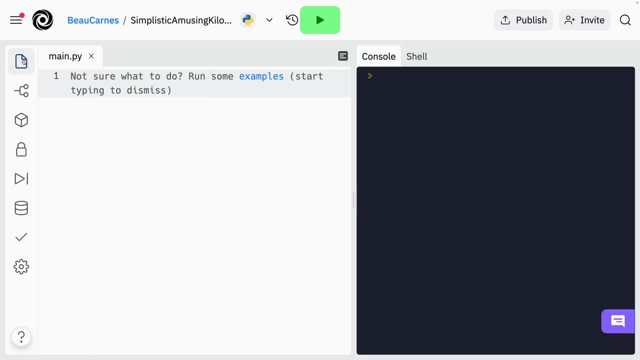 going to see the results in the console, So I'm just going to close this files window. So it's a little bigger here. I'm going to start off by showing you how to create a variable with Python. So this is a rock paper scissors game And there's going to be a players a 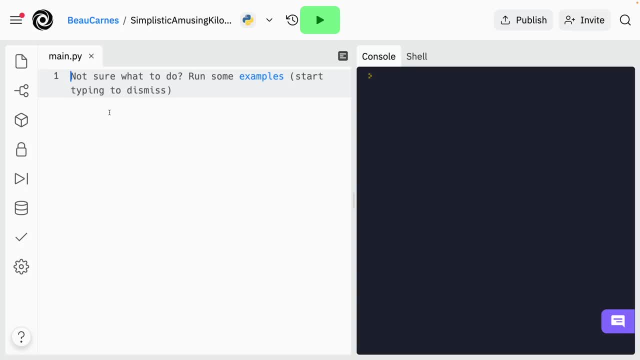 player is going to have a choice and a computer is going to have a choice. So I'm going to create a variable called player choice And I'm going to set that equal to rock. So let's look at a few components about this. This is the variable name: player choice. 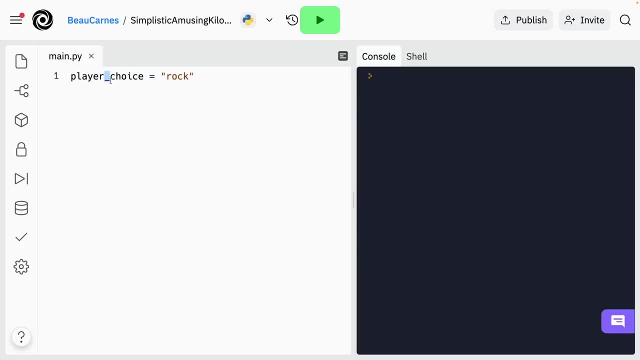 And you can see if you we use an underscore. that's just kind of the convention for Python to use an underscore if you're going to have a space in the variable name and we're going to assign it. that's what this equal sign. 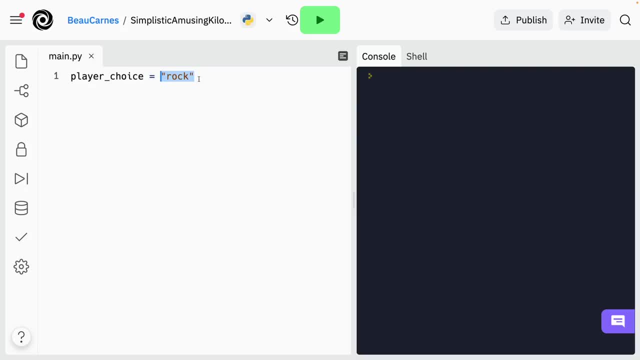 The assign operator and we're going to assign it to a string. a string is just a word or a collection of characters, like rock, and we're going to put quotation marks around it. Now, we could have also used a single quotes instead of double quotes. As long as you use. 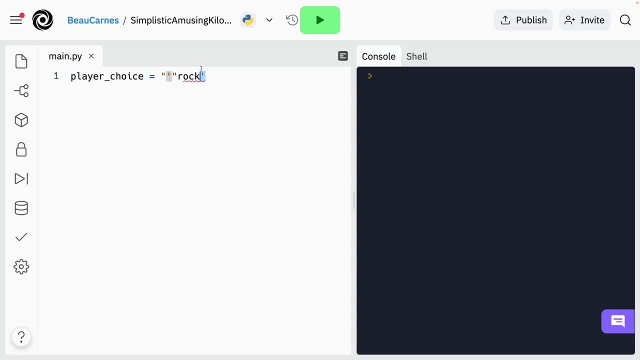 the same quote on each side. that's what's important. So we've now created a variable called player choice and assign it to rock, And now we can reference this variable later And whenever we reference the variable called player choice it's going to the code is going to automatically replace that player choice with rock. So this: 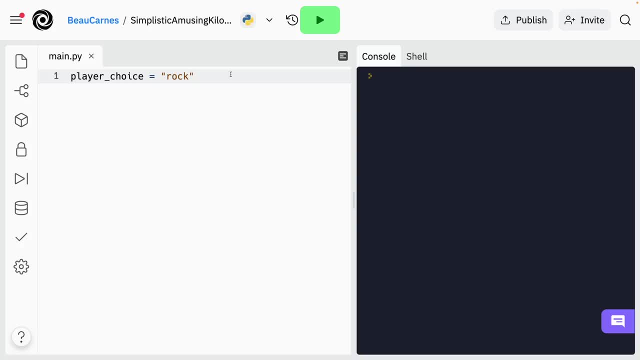 is going to be a very interactive project. I hope you're following along. I hope you have already got replete, loaded up like this. Now, throughout this project, I'm going to tell you what the next thing to do is, And I want you to try doing it yourself before. 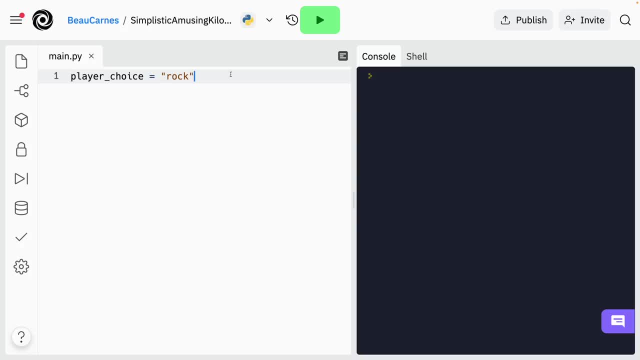 you watch what I'm going to do, So periodically, you'll want to pause the video And I'm going to go back to the video based on what I say. you and try to implement what I say before you come back to the video and watch me implement it and see if you've implemented the same. 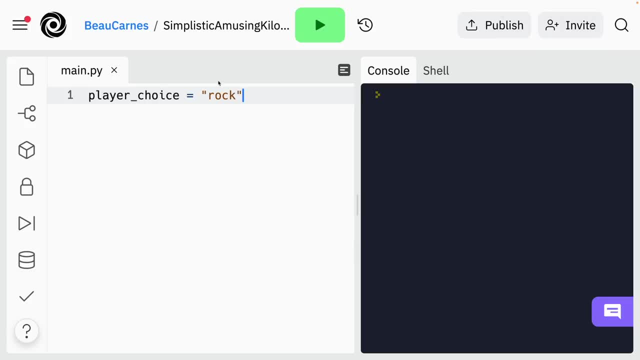 way. So I'm just going to zoom in one more time, And this is the first thing I want you to do: See if you can make another variable on the next line. So you're going to press return or enter to go to the next line And this variable should be called computer choice. 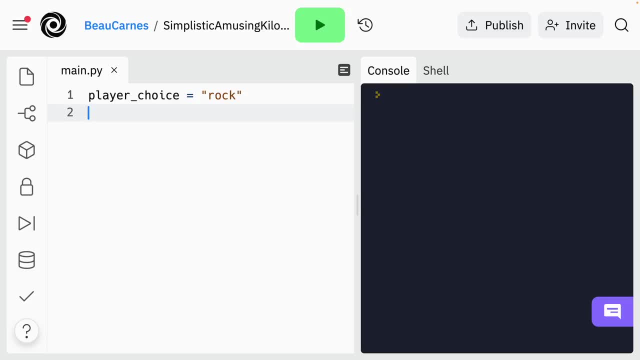 And you should set it to equal paper. Okay, so you can pause the video and see if you can make a variable called computer choice and set it to equal paper. So here it's pretty simple. here it's going to start simple. 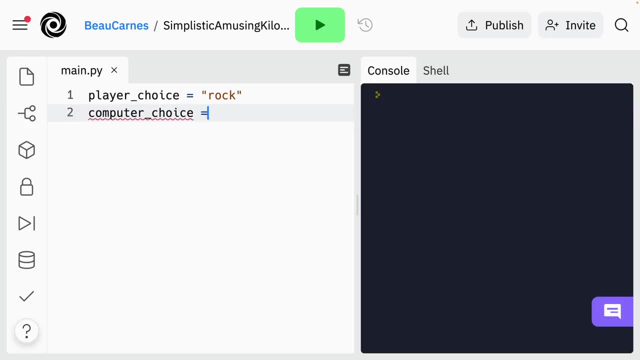 but it's going to get harder as we go. So computer choice equals paper, Okay. so, like I said, starting simple, but it's going to get more complex as we go along. If you've done that, you've now written your first line of Python code in this course. Okay now. 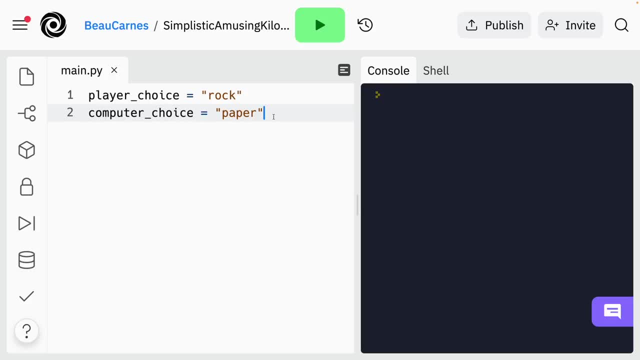 I'm going to talk about functions Now. a function is a set of code which only runs when it is called, So I'm going to show you how to put this code into a function. Now, one thing about Python is that indentation 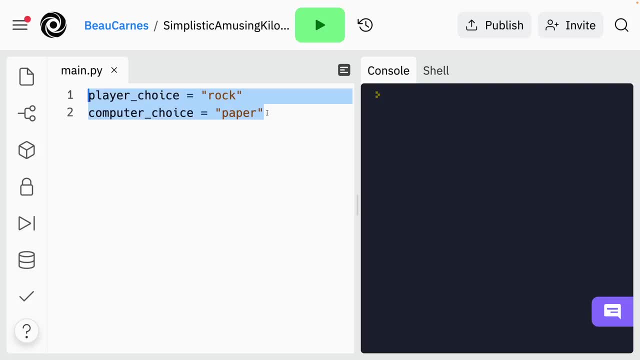 is very important. So after we create a, we define the name of a function. any line of code that's indented, the same amount is considered within that function. So I'm going to create a new line of code at the top And I'm going to call that function. I'm going to call it. 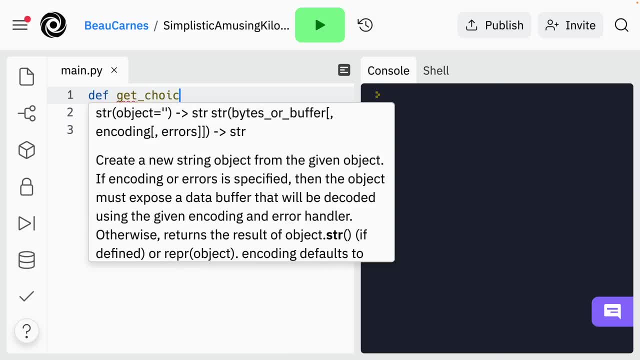 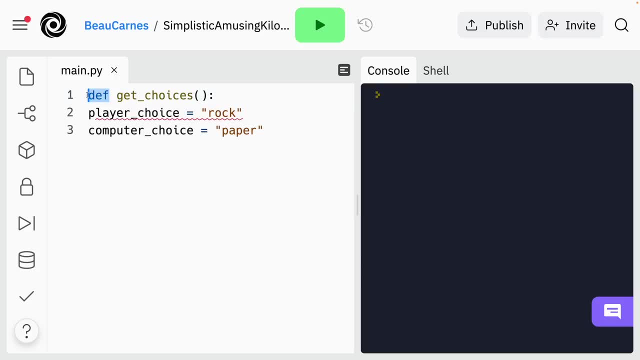 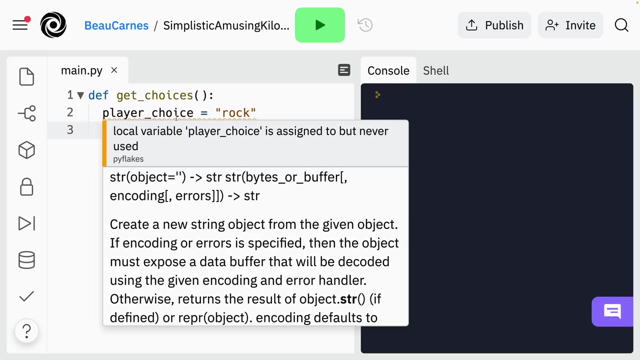 call it get choices. Okay, so we define the function with D, F and get choices, And I'm going to select all these, these two lines of code at the same time and just press the tab key And that's going to indent all these, the same amount, And you can see, sometimes 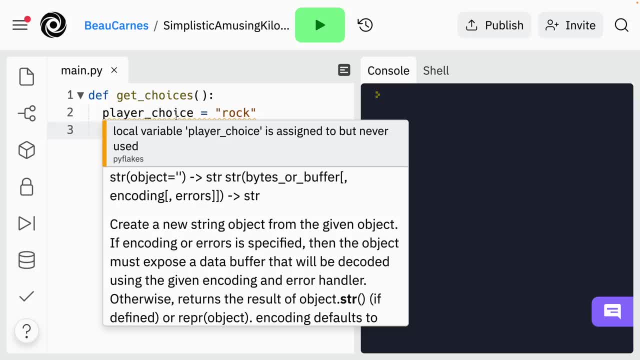 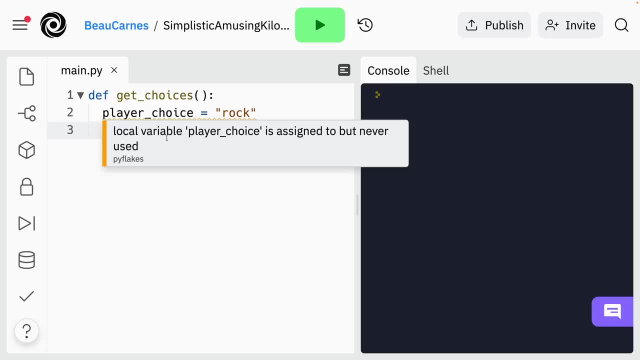 there'll be squiggly lines And if you hover over some of the squiggly lines it will tell you something. in this case it just says the local variable called player choice is assigned to but never used. That's not necessarily bad, It's just just telling us that usually 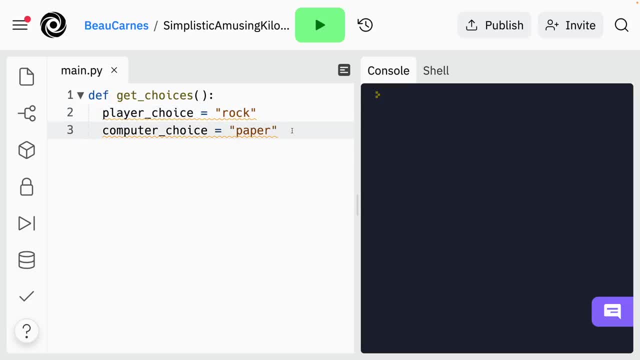 if you create a variable you're going to want to use it later. Well, we are going to use it later. we just haven't gotten to it yet. So sometimes the squiggly lines will indicate there's some sort of error in the code. Usually, I think, it's the color red. 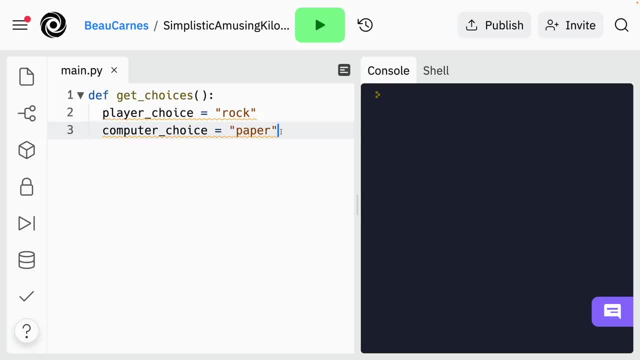 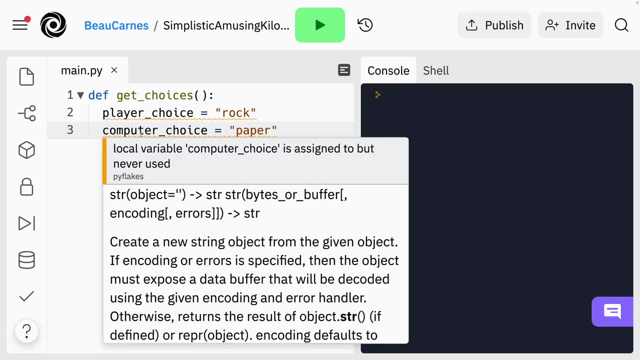 will indicate an error, But if it's a different color, it just may mean that there's something. maybe not quite right, But it's not really that big of a deal. So if you have a variable that's assigned to but never use, that's not going to stop your program, But it's just saying that it's not. 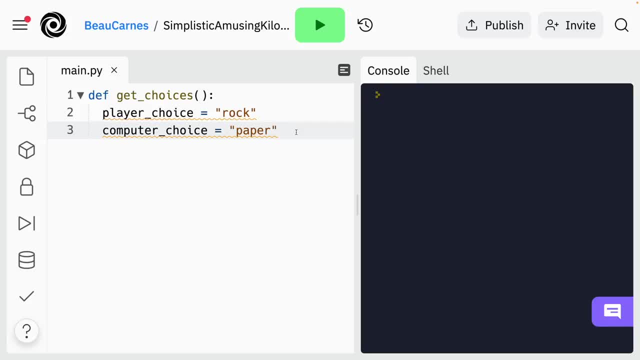 this variable isn't really being used for anything yet, But we will change that, this function. I'm going to show you how to call a function later, But we're creating a function called get choices that assigns these two variables And it's also I'm going to put. 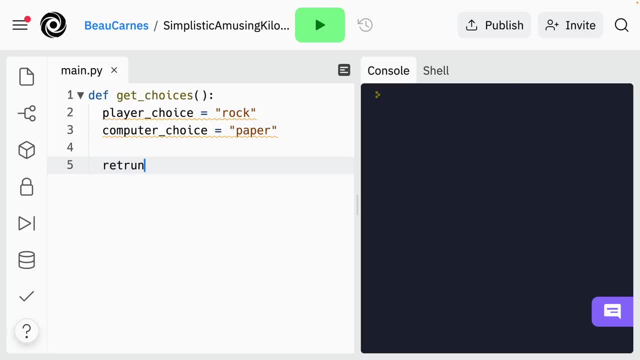 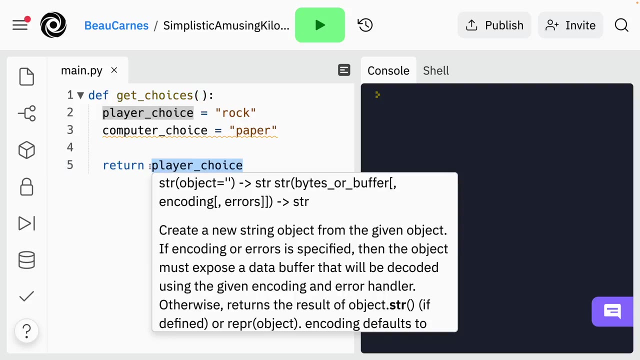 another line at the very end here And it's a return statement And I'm going to return player choice. This will indicate what's returned when this function is called. So later we'll call this function get choices, and it will return something. 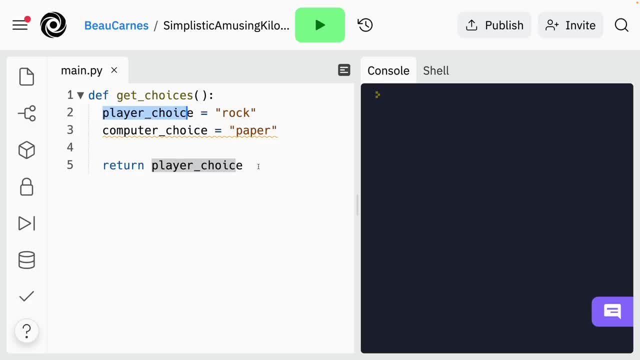 it will return the player choice, which is right here. we'll turn in this case rock. that we can use somewhere else in our code And I did just happen to put an extra line here. That's just, that's optional. I put a blank line here just to kind of make things. 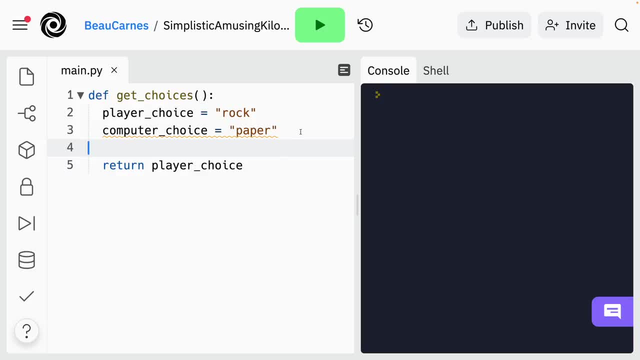 easy organize the code a little bit So different sometimes, I'll just put an extra line between different sections of code And it just makes it easier to identify the different sections when you're looking at the code. For the computer those extra lines don't mean anything. The 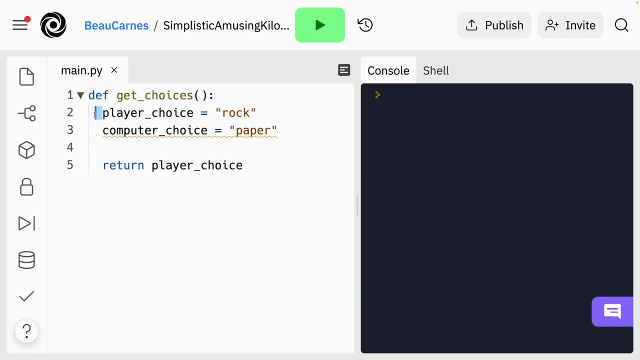 indentation, though, definitely does mean something. So, as long as every line of code is indented, the same amount as the previous line of code, and it's all within the same function. Okay, so this is what I want you to do: See if you can change the return statement. So, instead of 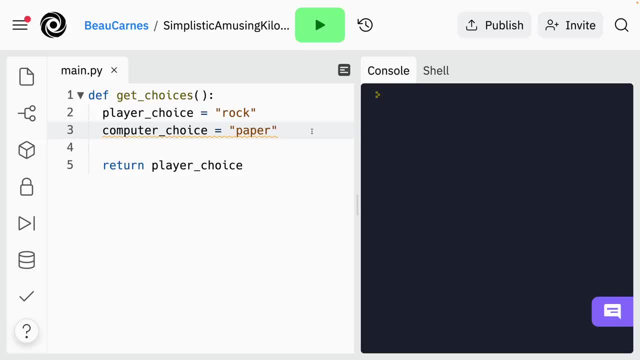 returning player choice. it's returning the computer choice. So that's pretty simple. It's now returning the computer choice here. Now I'm going to create another function down here. This is just going to be an example function, just so I can demonstrate something to you, And then we'll. 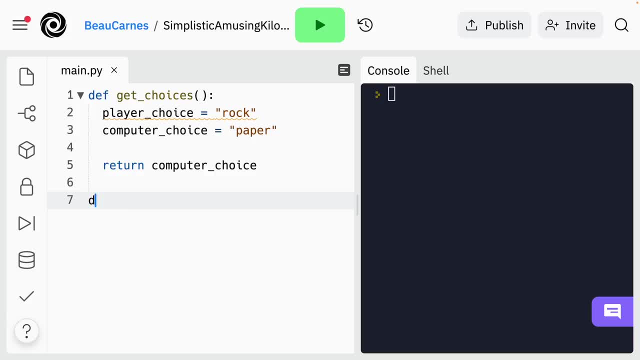 delete it. it's not gonna be part of our rock paper scissors game, But I'm going to create a new function called greeting, And then I am going to add what it's going to do. Oh yeah, put the semi colon. you also know a. 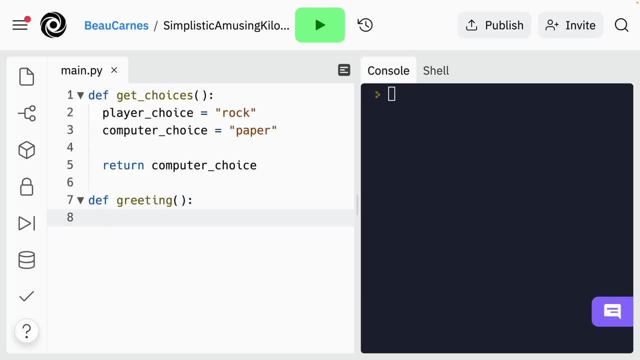 colon. So a function always has to have a colon at the end of how we define it. So I'm going to return a string and it's just gonna say hi, And one thing you'll notice is that there's no, you don't have to put any anything at the end of each line. some programming languages, such as 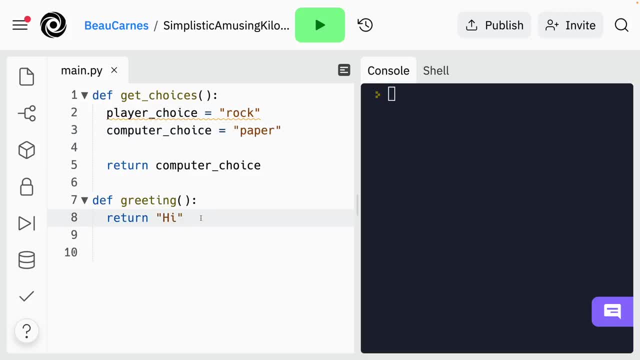 JavaScript you're gonna put a semi colon at the line, at the end of the line. But in Python it doesn't matter, You don't put anything at the end of each line. So now I'm going to call the function, to call the. 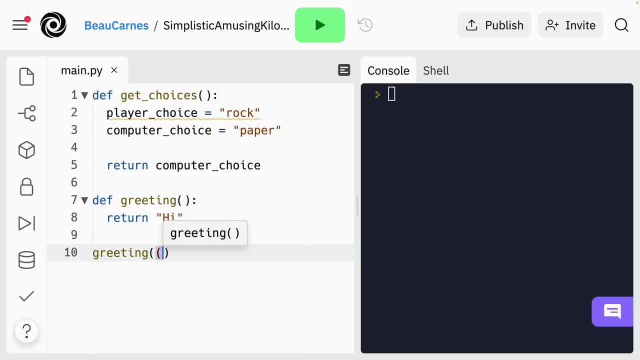 function. I just typed the name and I put the parentheses at the end, So it's going to say so: greeting is now going to call. it's going to call this function and that's going to return the string high Now. it's not going to do anything with the string because our program doesn't do. 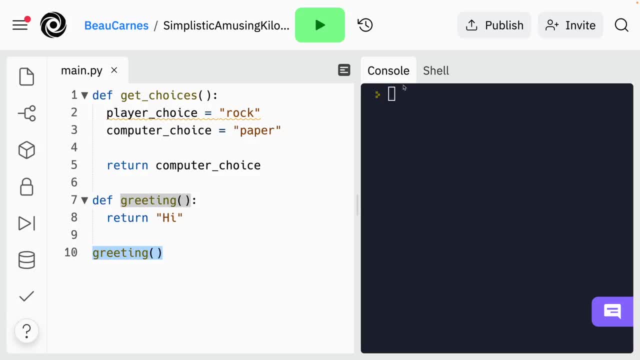 anything with the string that's been returned. It's not going to go into the console or anything, But let's add additional code So we will make this string high. go on to the console. First, let me create a variable that takes what? 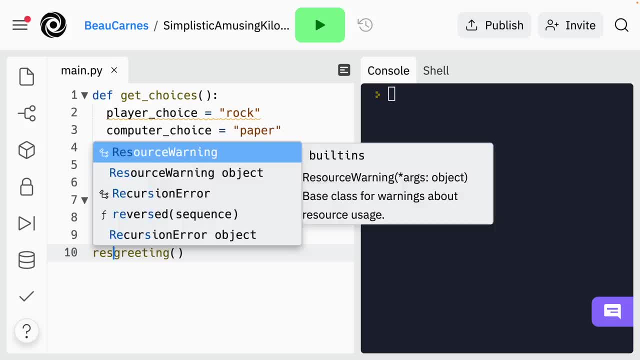 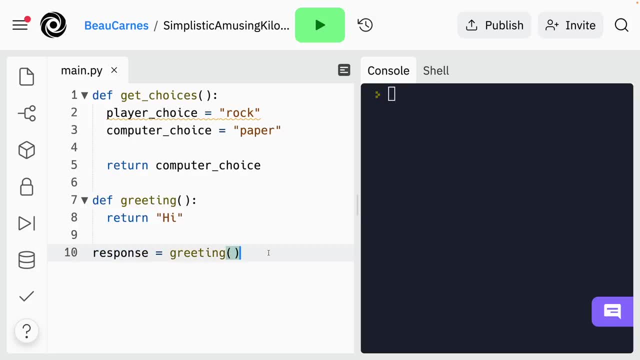 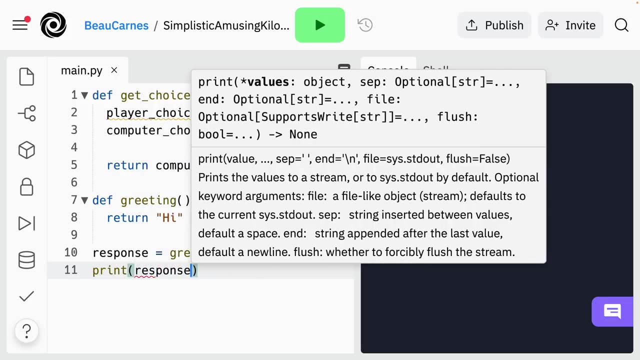 this greeting function returns. So I'm going to type in: response equals greeting. So now we've set the what greeting is being returned to this variable called response, And now I can use the print function And I can print the response And this will print it to the console. So now I can we. 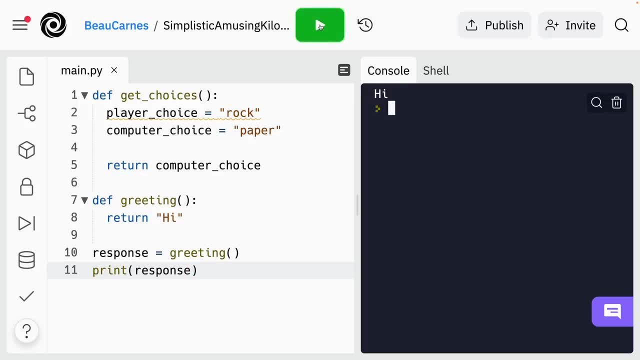 have this green button here. this runs the program. I'll click this green button here And now we can see it's high. So this response is getting this high from here And then we're printing it right there. Okay, I'm actually. 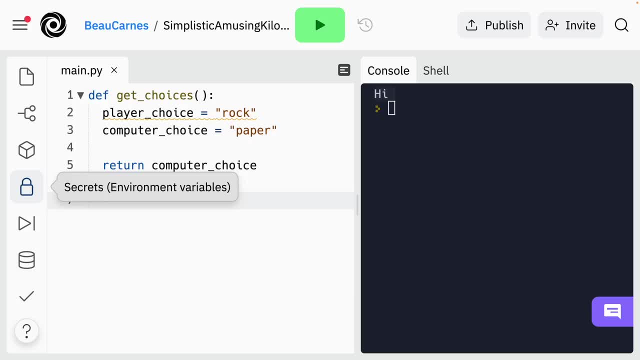 going to delete all of this, And what I want you to try to do now is to call the get choices function and store the response in a variable called choices and then print the value of choices to the console, So you can pause and try that really quick, And then I'm going to show you. 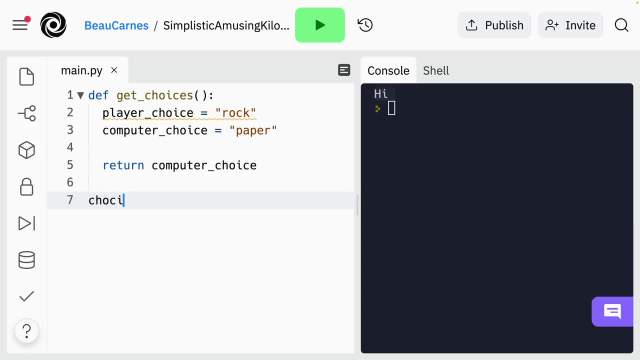 how okay? so remember the variables called choices, And we're going to set that equal to the get choices variable now in the get choices function. Now, instead of typing out get choices, you can see that this code editor is actually giving us suggestions on what we want to put in here. So 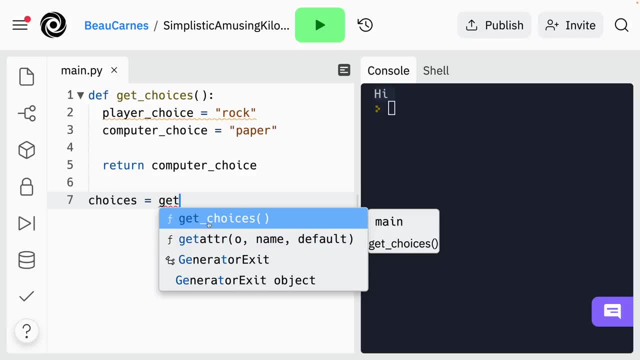 I just typed in get and you can see it's now saying get choices, right here. So I can actually, instead of typing out the whole thing, I can either click there or I can just press the Tab key and it's going to fill in the rest of that function name. So that's just something little that makes. 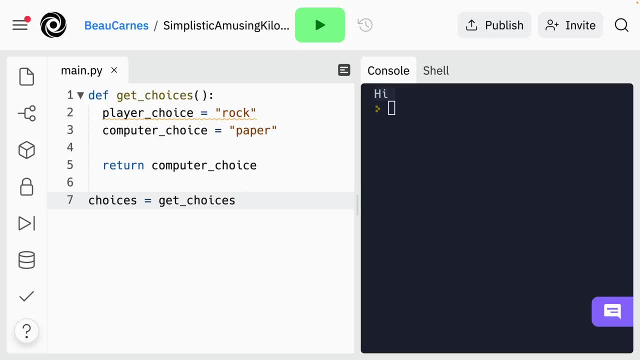 it easier to write a program. you don't have to type out every single thing. So if you've already created a function or a variable, then the, the code editor, then replica will suggest what you may want to fill in when you're typing, And most other code editors do something similar. It's: 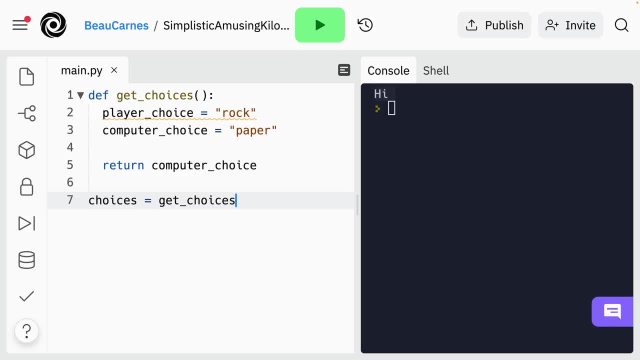 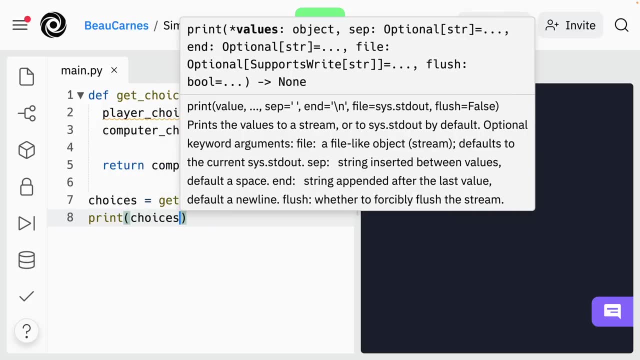 called code completion, So I'm going to be so. I still have to add parentheses at the end, And now I'm going to print The choices. Okay, so I'm going to just click this play button to make sure it does what we're. 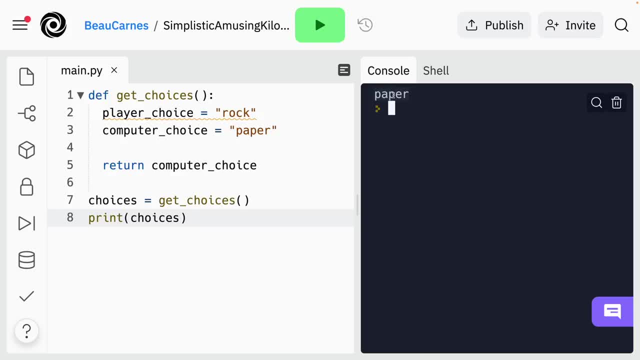 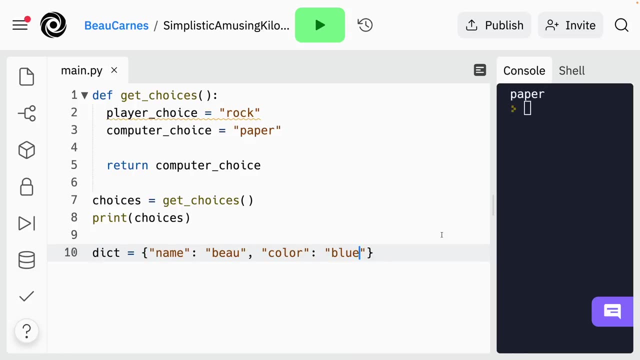 trying to do. Yep, it clicked paper. Great. Now let's talk about dictionaries. dictionaries in Python are used to store data values in key value pairs, So let me just show you an example. Okay, so a dictionary is going to have these curly braces at the beginning and end, And then here: 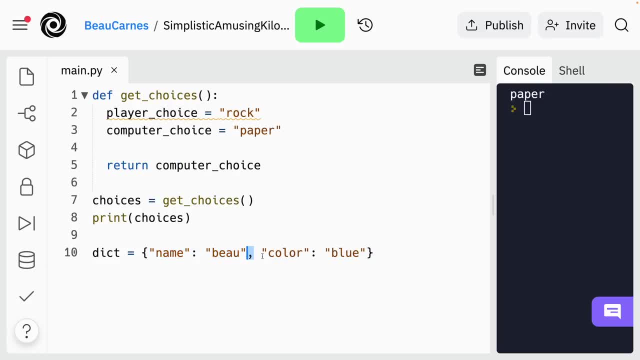 here's a key value pair, there's one, it's separated by a comma. And then here's another key value pair. So we're setting name, we're setting that to equal bow and we're saying the color to equal blue. So here's the key, Here's the value, Here's the key, Here's the. 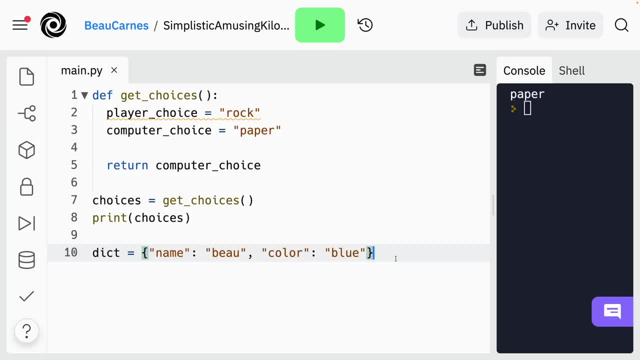 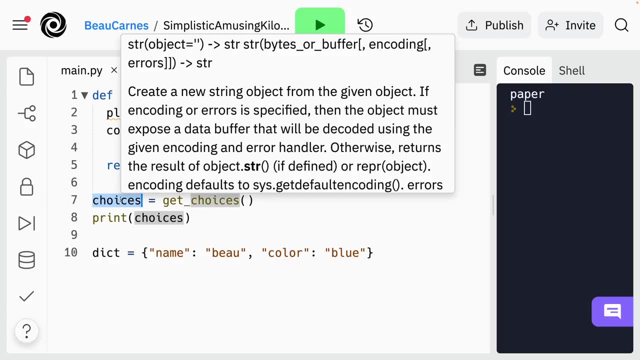 value And the key or the value in a dictionary can be a variable like the color. we could set that. we already created this variable here. I'm just going to copy that word choices And we can put choices And you can see. now it's not surrounded by the quotation marks. 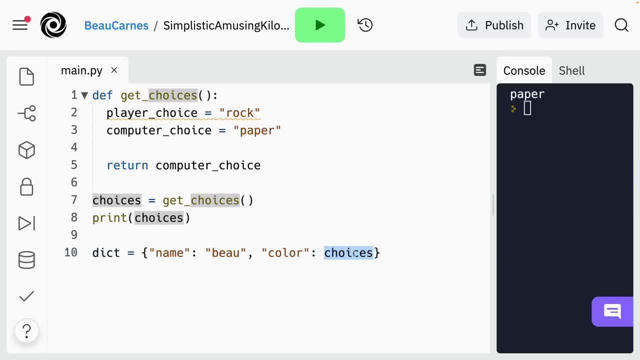 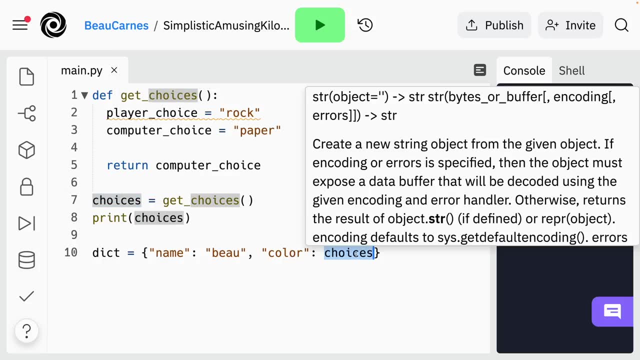 So if you saw, surrounded by quotation marks, it's a string, But if we don't surround it by quotation marks, it's getting the. the variable here, choices. So this would be set to paper because that's what choice is going to: is going to equal. So we're about to delete this. 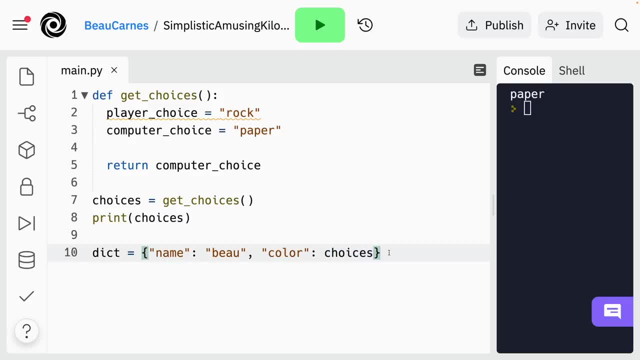 line, because that was just an example. But now, before the return statement in this function, we're going to add a new line, we're going to create a variable named choices And we're going to make it equal to a dictionary. the first key should be: player with a value of 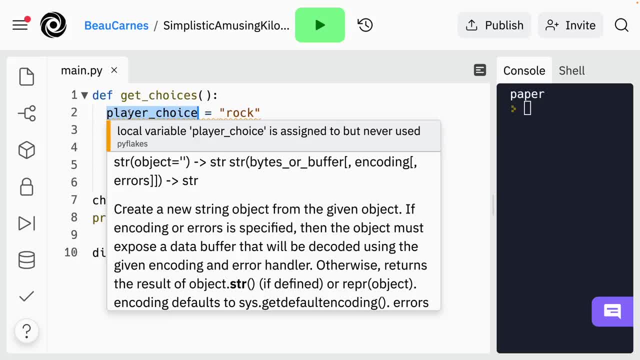 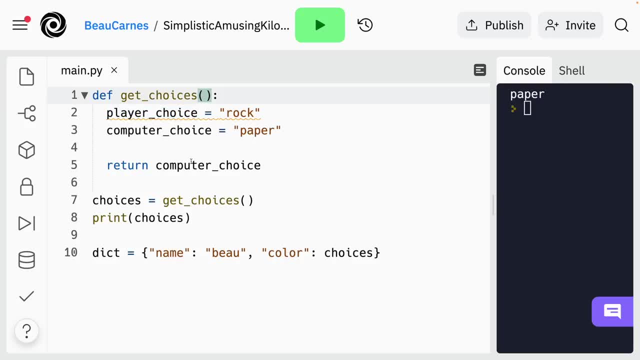 the player choice. they actually this variable. here the second key should be computer with a value of computer choice. And then we're going to update the return statement to return the choices dictionary. Now I'm not going to keep telling you, to pause and try it yourself. 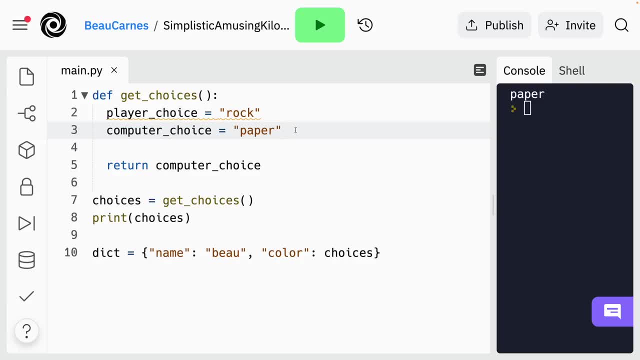 So just the rest of this time, whenever I say what we're going to do, you'll know that after I get done explaining it, you're going to be able to see that, the return statement. you can pause it and try it yourself, But that's what we're going to do now. So I'm 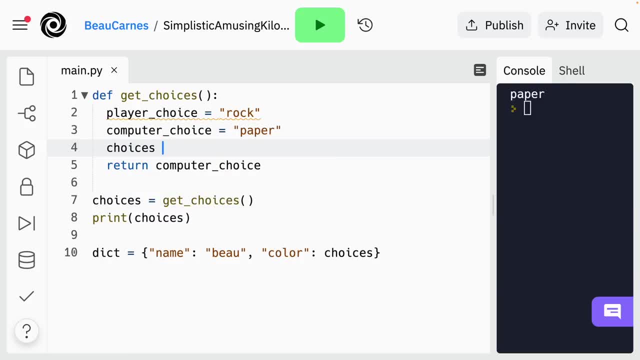 going to create choices And it's going to be a dictionary, And then it's going to have a player. That's the key And the value is going to be player choice, And I was just able to press tab to fill that in. And then we're going to have computer and it's going 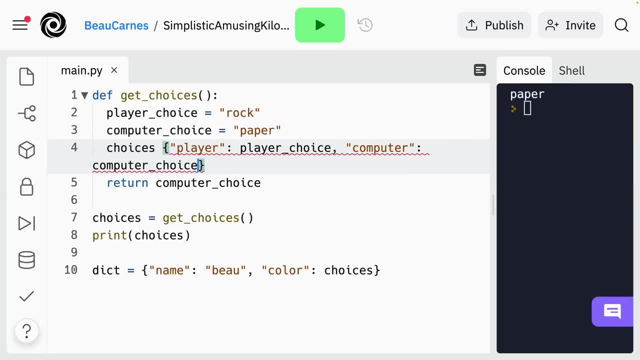 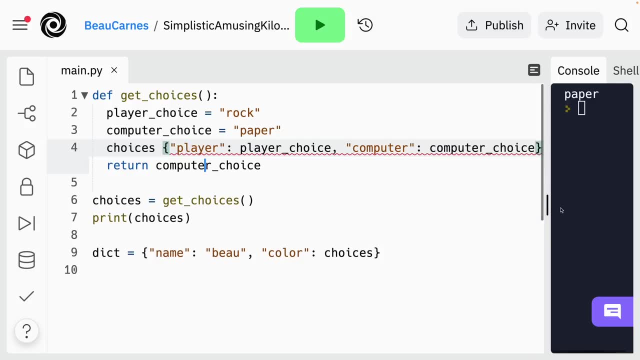 to be computer choice. Okay, and you can see, sometimes if it goes to the next line, there just won't be a line number right here. But I can move this over for now And then I am going to. Oh, I forgot to put. 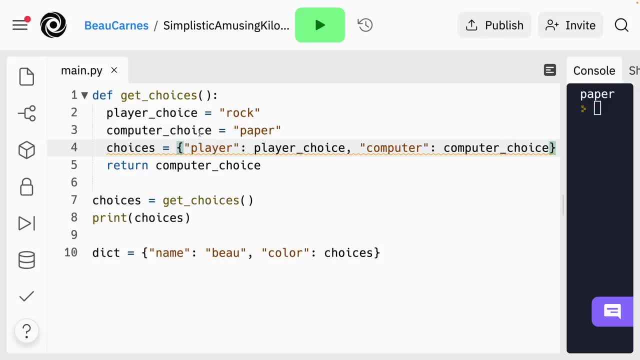 the equal sign. That's what that red squiggly line means. So, because the red means there is a problem, the program is not going to run correctly Now. the orange just means that we haven't used choices yet, which we will right now, because we're going to return choices. 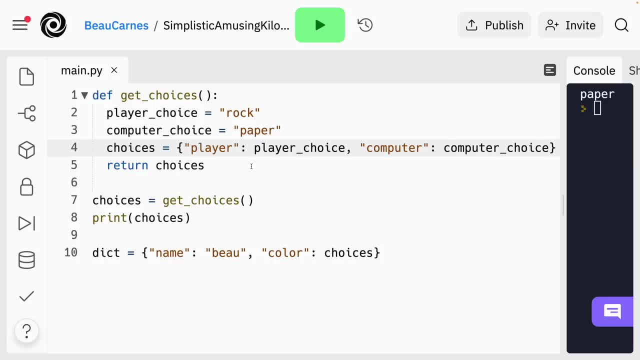 Okay, so now we don't have any squiggly lines because we're using every variable that we created And we're returning choices here. So you may have noticed that player choice it does not actually get set to the players actual choice. So let's fix that. the input: 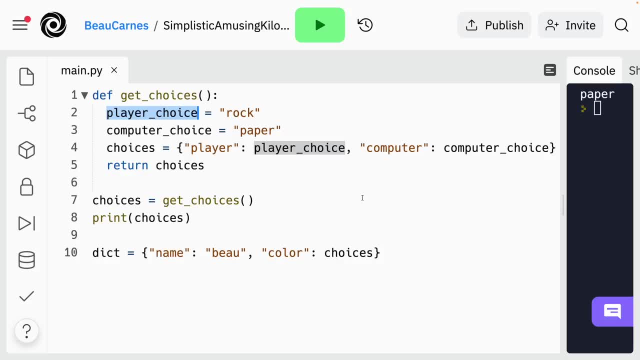 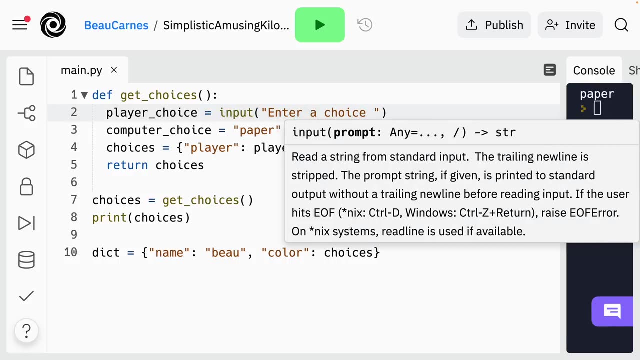 function gets input from a user and we'll use it to get the players choice. So, instead of having players choice equal rock, we're going to make players choice input. Enter a choice Rock paper scissors. Okay, so this is how you get input from a user: we use the input function And this is going to 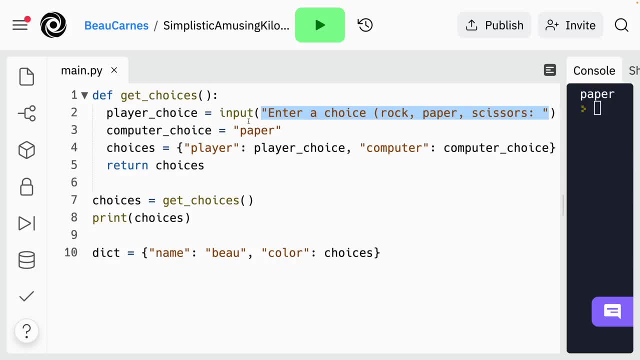 be something that's going to be printed. we'll print to the console here And whatever the result of this input will be that the the player that the user entered will get stored to this variable, which we then can use later in our program. So let's just try that out. I'll click. 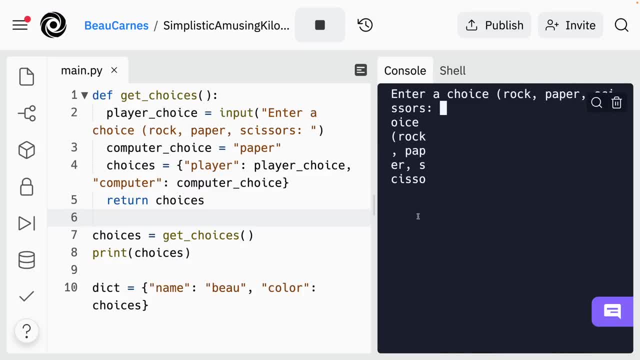 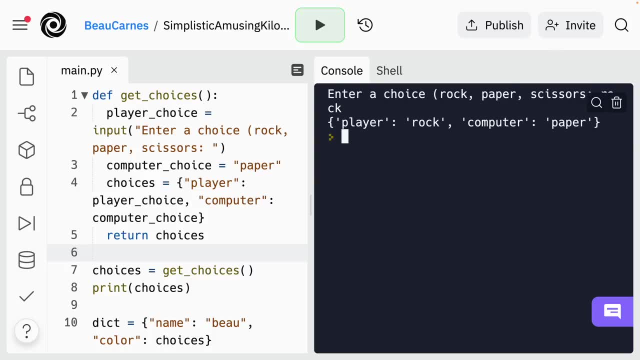 Run and enter it. Let me just stop and run it again. Okay, enter a choice: rock paper scissors. I'll just put rock And now you can see the players choice. we're still printing that and it's going to print as rock. 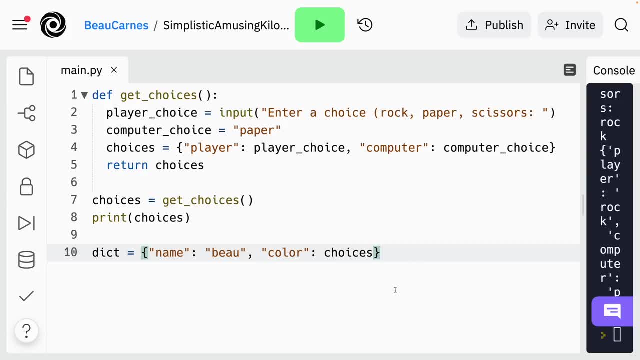 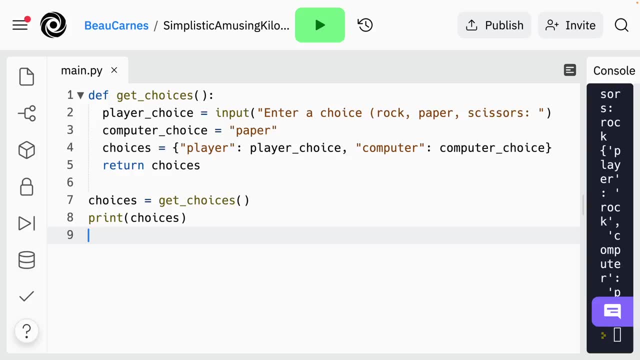 Great. Now let's just clean up this code a little bit. We still have this here. we don't need that dictionary. that's not going to be part of our final code, And now we'll make it so the computer can actually make a choice. So we're going to learn about importing libraries, creating lists. 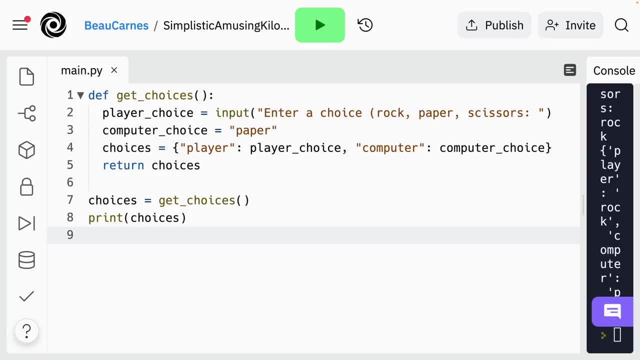 and calling methods. Python libraries are a set of useful functions So you don't have to write code from scratch. When you import a library to your program, you get access to more features without writing additional code. With basic Python it's challenging to get your program. 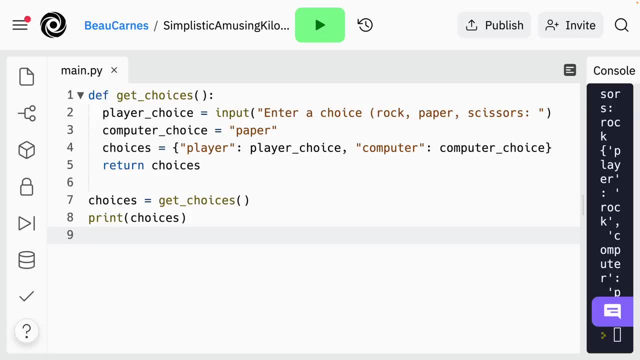 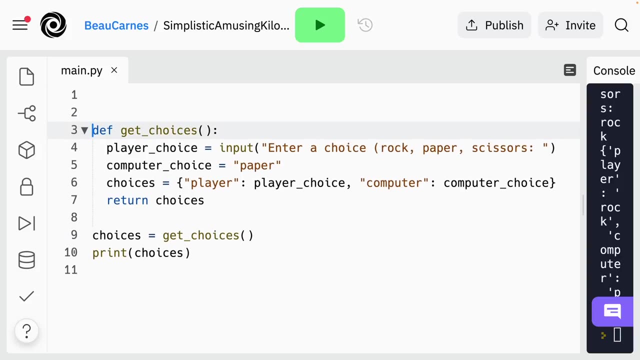 to do something randomly, But it's easy to choose something randomly using the random library. So let me show you how we can import the random library. import statements are used to import libraries and they're usually put at the top of a program, So I'm going to press Enter a few times. 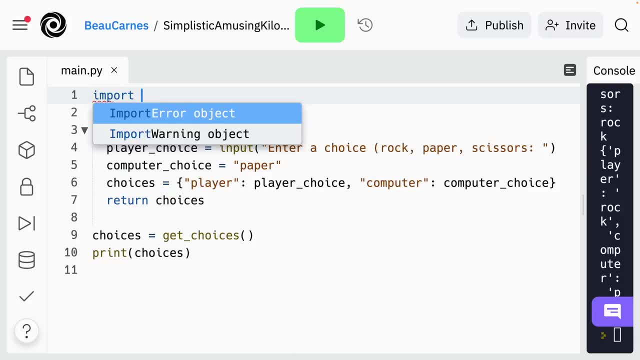 here to add some lines at the top And I'm going to do import random. So now we are going. we we've imported the random library, So we're going to use that random library soon. But now let's learn about lists. A list in Python is used to store multiple items in a 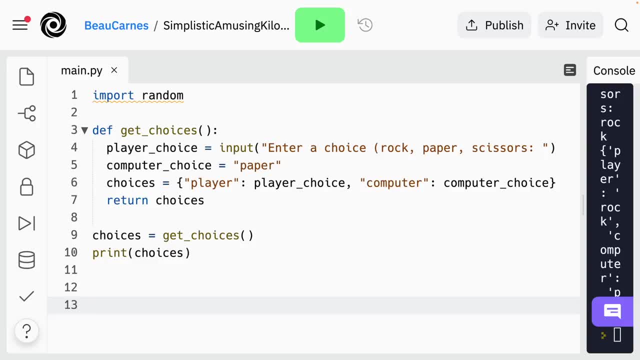 single variable. lists are surrounded by brackets and each item is separated by a comma. So here's an example: I could create a food, a variable called food, and set it to this list. it's going to have three items: pizza, carrots and eggs. So this is a list of strings. 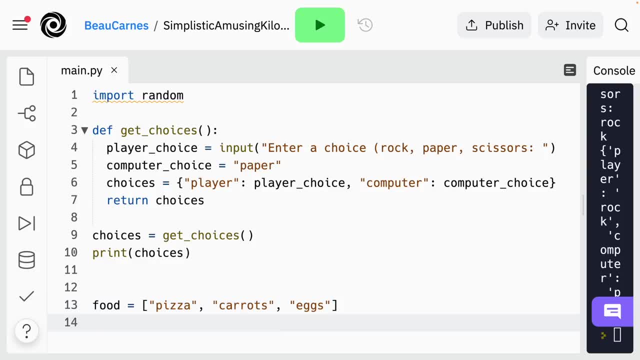 And then you can also get a random item from the list Using we're going to use- now we've imported random, we can get a random item by using that, that random library. So I'm going to put: dinner equals random dot choice And then I'm going to pass in the list here. So, using their random 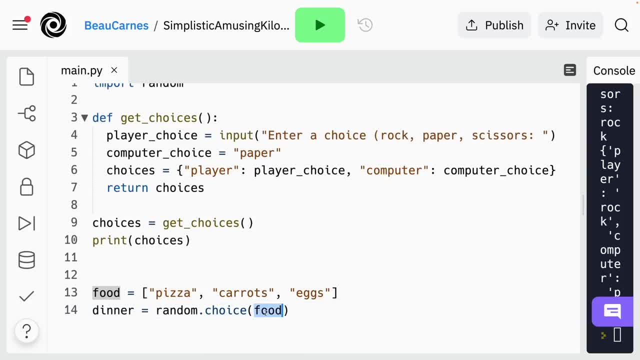 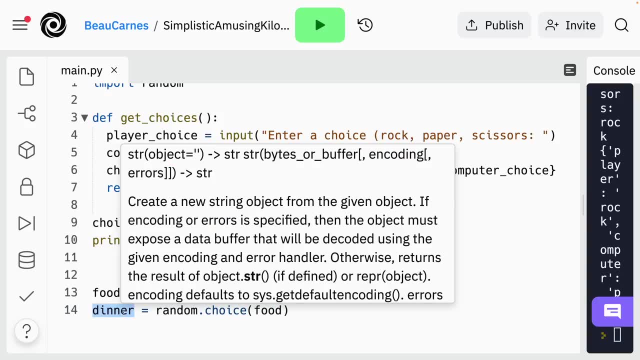 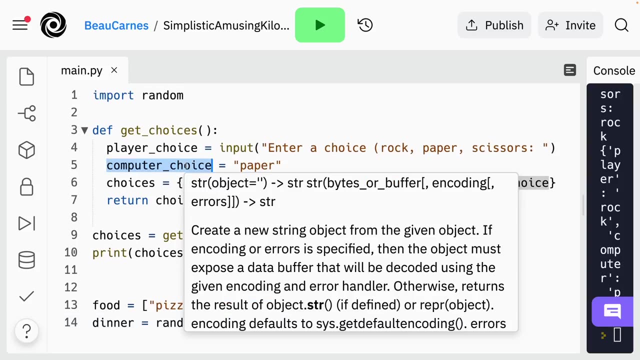 library we can call choice And then we can pass in a list and it's going to choose a random item from that list and and set it to equal this dinner variable. So right now the computer choice always equals paper, but we want it to be a random choice between rock. 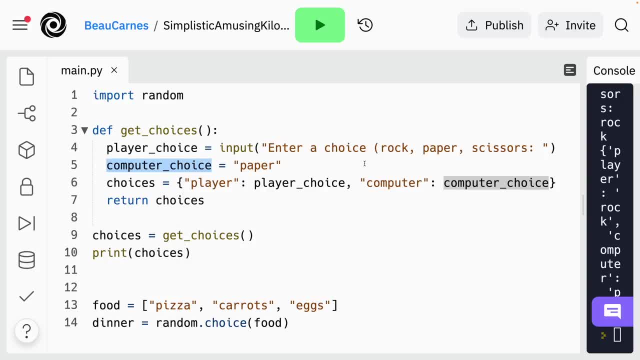 scissors and paper. So before the computer choice variables created, we'll create a new variable called options and assign it to a list of the possible options: rock, paper, scissors. then we'll set the computer choice variable to be a random choice of one of. 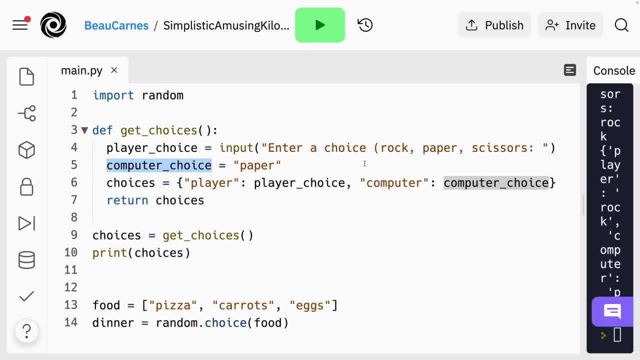 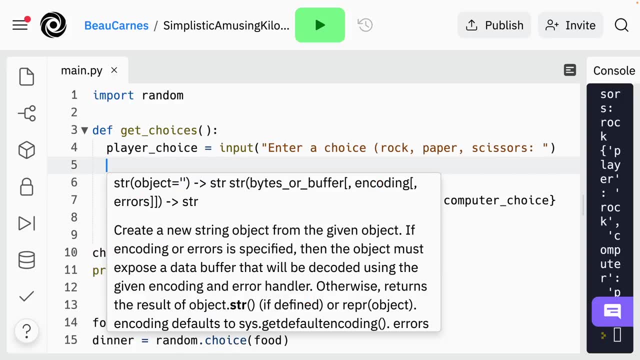 the items in the options list. Okay, I hope you already tried this now, But let me show you how that's going to work. We'll create options And we'll set it equal to this list of rock paper scissors, And you can see the code editor will often pop up these boxes with more information. 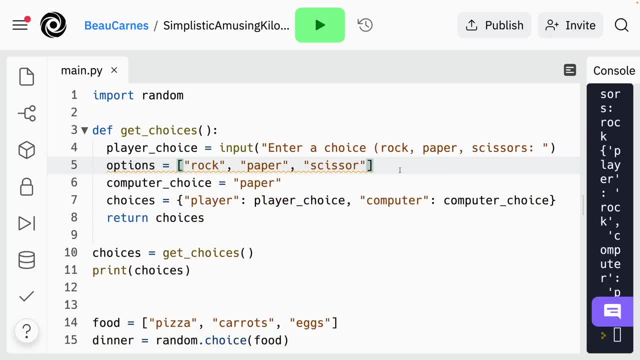 about what you're looking at. So we're going to call this list of options rock paper scissors what we're doing to give us some some help with what we're trying to do here. So we're going to set this computer choice to be random dot choice- Food, not food. I was looking at food down there. 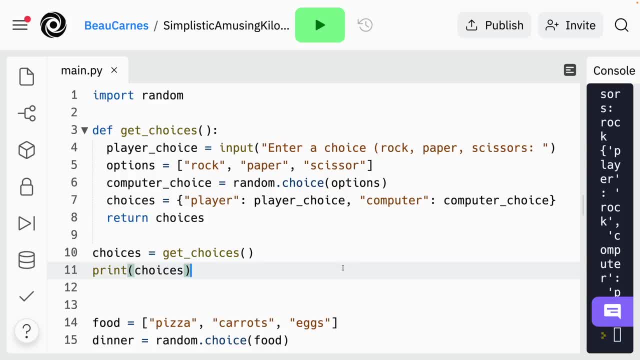 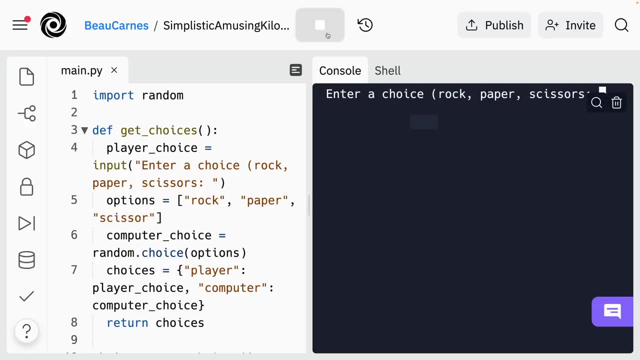 there's gonna be options. There we go And let's just try running this program and seeing what happens. So I'm going to put rock And then we see the computer chose scissor. it should be scissors. That's why we're testing it out. I guess I spelled that wrong. Okay, so scissors with an S. So now. 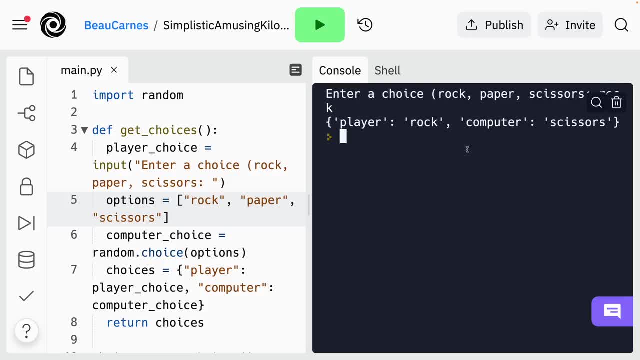 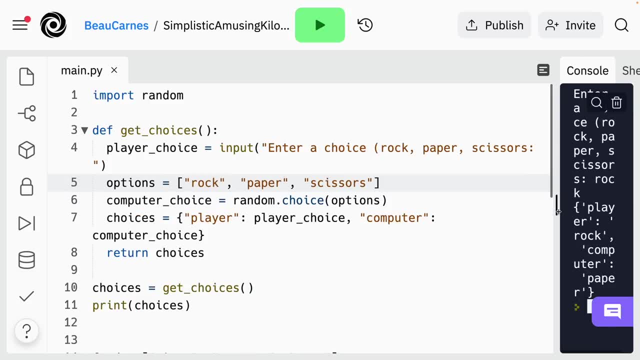 let me try running it again And you can see it shows scissors. but if we run enough time, it should. now it's choosing paper, because choosing it at random, Okay, that's working, Okay. so now let's just delete all this crap. 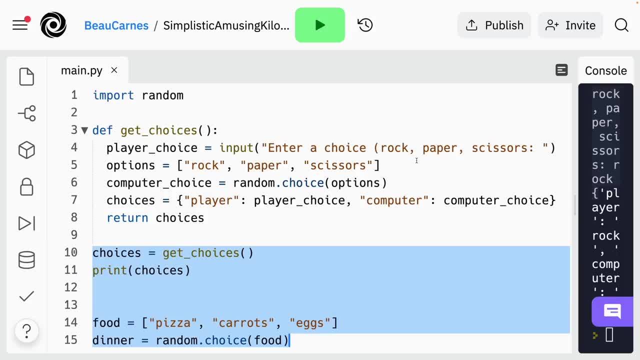 Code after the get choices function. we don't need to test that get choices function anymore. And now let's create a new function called check when. So you shouldn't know enough how to? you should know enough about how to create a function. So def: check When. so this is just an empty. 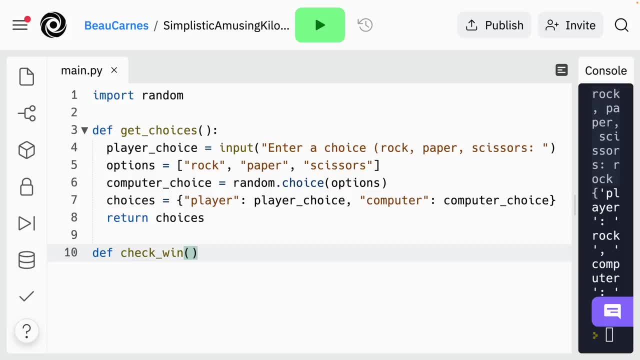 function with nothing inside it. yet. But before we add with the colon, so before we add any code inside the function, we're going to create some arguments. Function can read, functions can receive data. when they're called, the data are called arguments. So when creating a function, 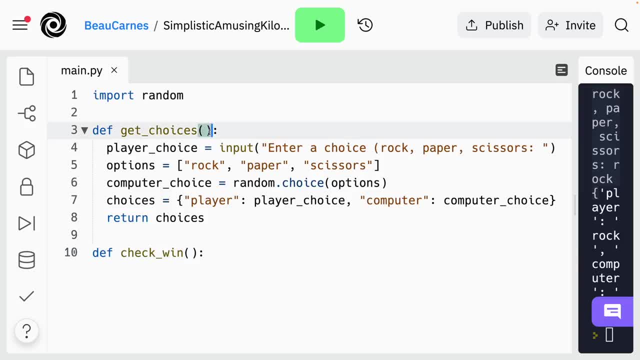 you can specify arguments inside the parentheses. So we've been using this empty parentheses. but I can put in tooth, I can put in things within these parentheses. When this function is called, we're going to give it two pieces of data. we're going to pass two pieces of data into the function. 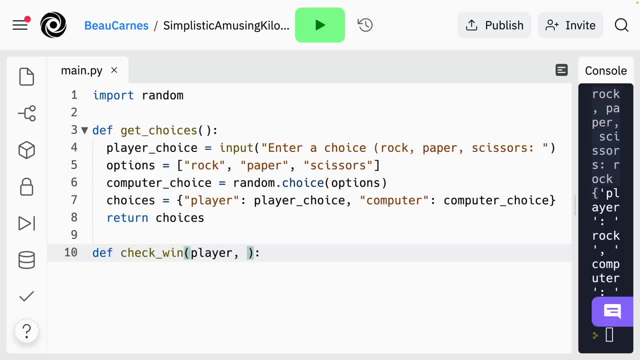 The first piece of data is going to be player. the second piece of data is going to be computer, So the you can basically call these anything you want. These are just very. we're creating new variables, But when we call these functions we'll pass in two pieces of information that 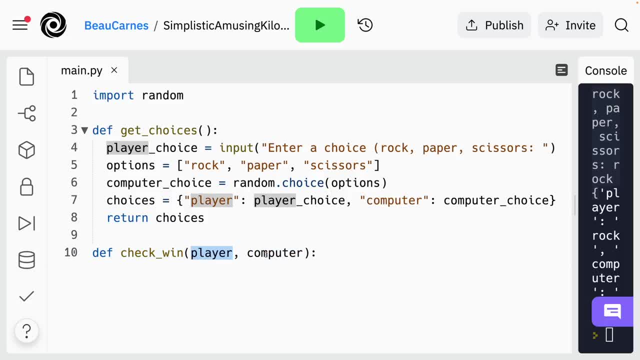 will then be assigned to the variable names player and computer that we can use inside the function. So for now let's finish up with two. for a complete function, the function has to have some code within the function. So let's just add return statement, that's just. 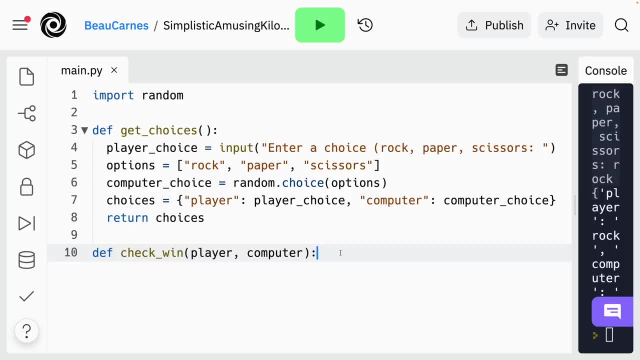 going to return a list containing the elements player and computer. So this check when function shouldn't actually return this. this is just to kind of get get it quickly created. it should actually return different things depending on the player and computer. arguments And if statement. 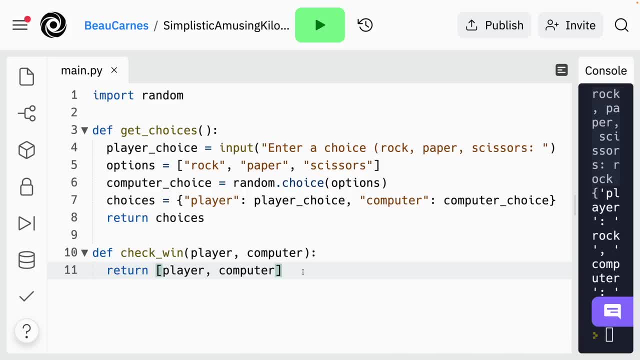 will allow a program to do different things depending on certain conditions. So in this statement we'll first check a condition And if the condition is true, then all the lines of code under the if statement that are indented the same amount will execute. 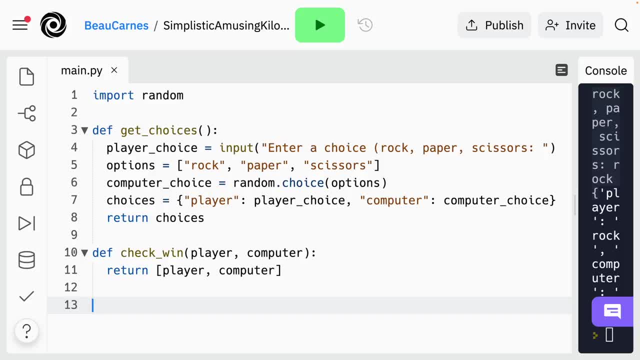 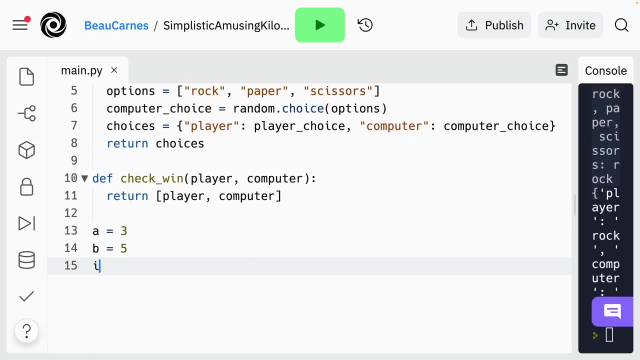 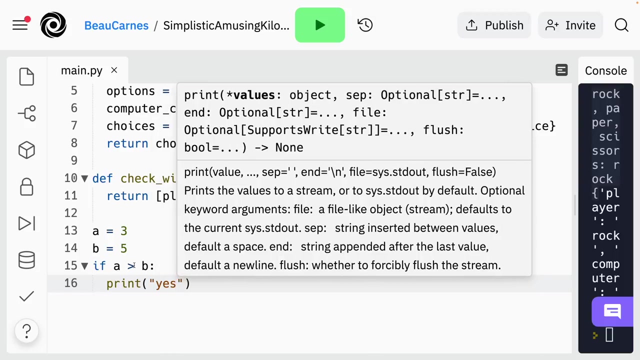 So as a quick example, I can say: A equals three, B equals five, And then we can create an if statement here. if a is greater than B, then we will do something like print Yes, or we can do if a is less than B, or we can do if we want to check if A and B are equal. 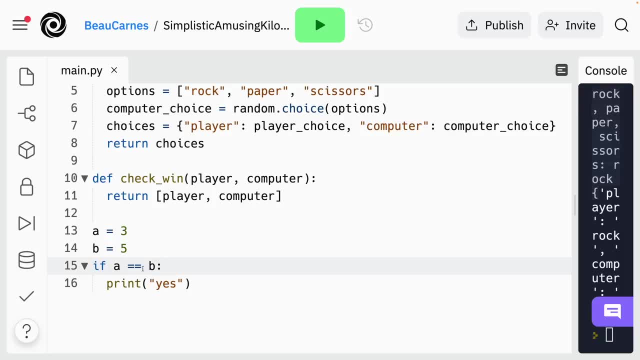 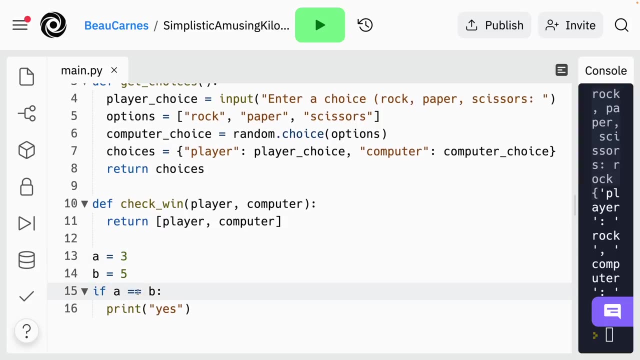 we can do equally will put two equal signs. Now this is very important. you never want to use one equal sign because a single equal sign is the assignment operator. That's how you assign what variables are equal to. So if you use a single equal sign, or like then if I put if a single, 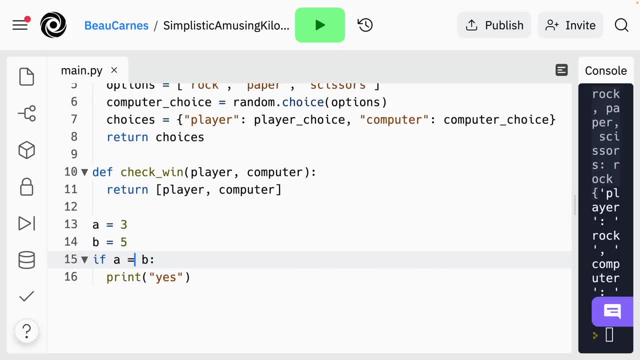 equal sign B. without a double equal sign, then the assignment operator is going to put the easy sign that is going to set a to equal B, which is not what we want. the double equal sign is going to check if a and B are the same value. basically, it checks if two values, values are equal. Now 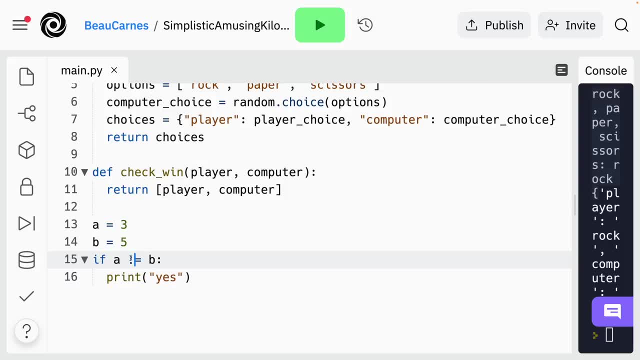 you can also do a not equal. So if you use the exclamation point, that's not equal, or you can use less than or equal to, or you can do more than or equal to. So I'm just going to delete all this for now. So now we're going to update this return statement. Before the return statement: 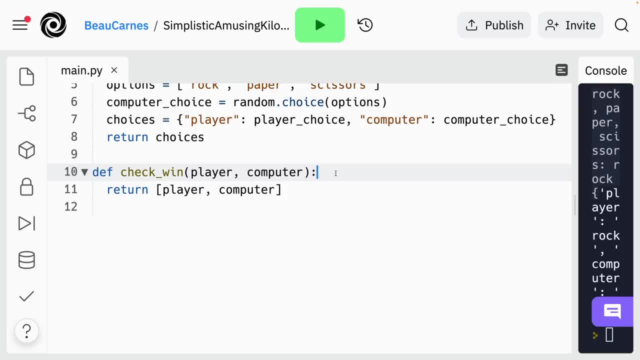 we want to. we're going to check if player, if player- equals computer and if so, if true, we'll return the string. it's a tie. So let's do that If player equals computer, and this is something that maybe you figured out yourself before you, before you're watching this. 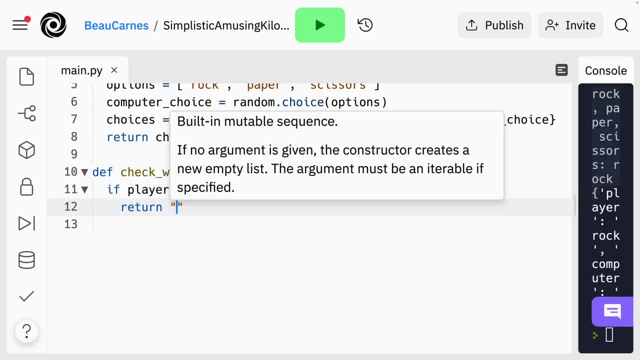 and we'll return a string and the string is going to be: it's a tie, Okay, so now it's only going to return. so a function does not have to return something And for this function it's only going to return something. If this is true, if player equals. 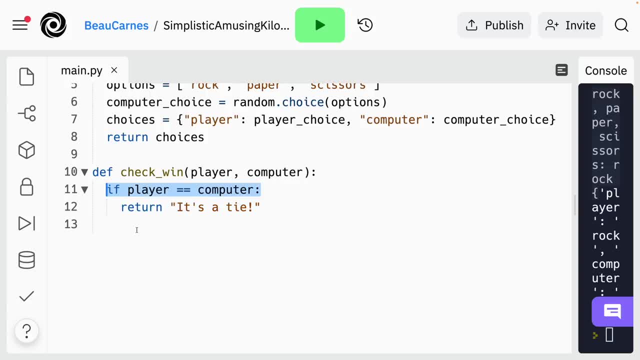 computer. if not, it won't return anything. And it's just to make make you notice this. see, this line is indented within the if statement, which is indented within this function. And just really quick thing to note. 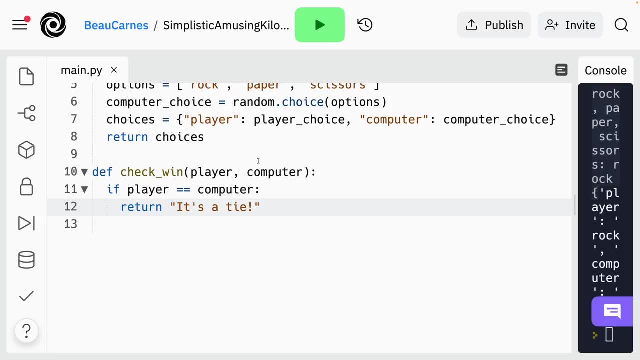 for a return statement. parentheses are optional, So I could also add parentheses like that, but you don't need them, But for now I'm just going to get rid of them. So currently, when there's a tie, the program now returns. 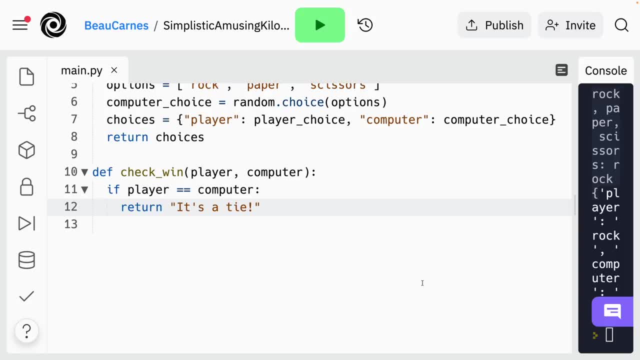 it's a tie. but how does the player know that's true? Now let's have the program print which options that the program now returns are by default, which are the ways back to the back end. they're the ways back to the back end. But now let's make sure that this is a tie, Because now 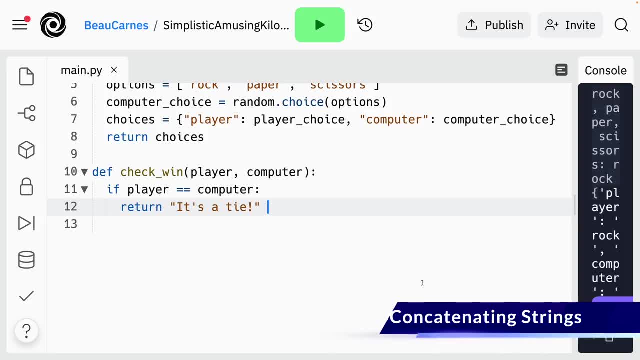 the program is now showing it's a tie. But how does the player know that's true? Now let's have the program print which options that the program has to return. Let's go back over here. And that the player and the computer chose: You can concatenate strings with the plus operator. That 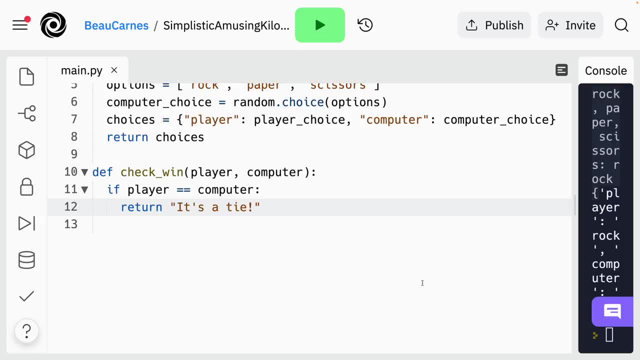 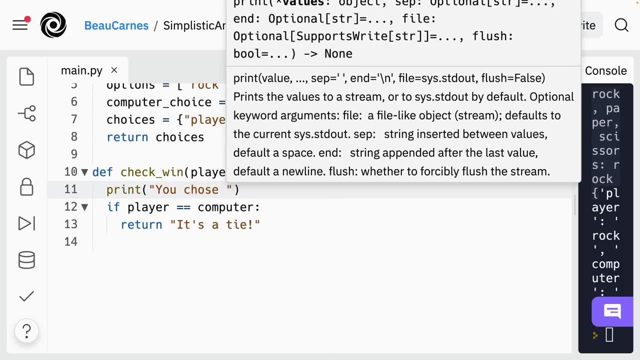 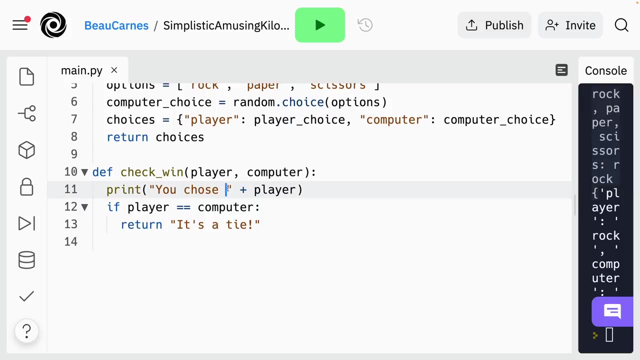 just means you can combine strings with other strings or strings with variables. So let me show you how you can print which options were chosen. So I'm going to print you chose and then I'll put player so you chose, and then we have to add a space here because it's going to print a. 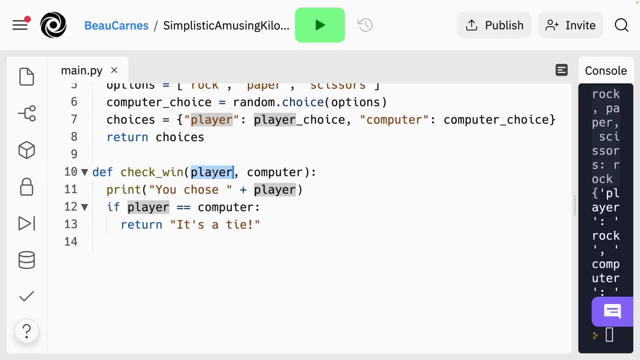 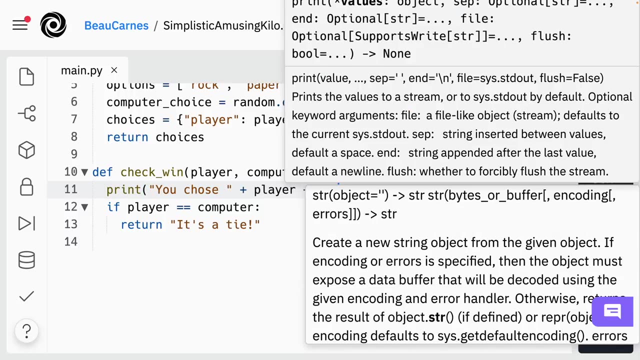 space and then it will choose. it will print this. So if the player chose rock, we'll say you chose rock, And then we can concat. So we concatenate these together. but we can add another plus sign and put another string here And it's going to say: computer chose us, like being covered up here by 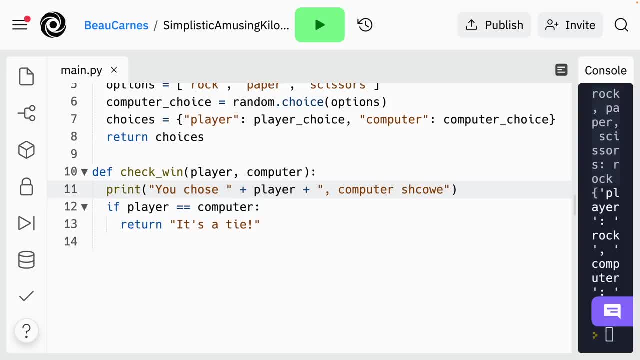 everything Computer chose. Now I'm just about to type it in, but see if you can figure out what to add at the end here to put in what the computer chose. So computer chose computer or the value of this variable here. So a lot of times when with programming there's a bunch of ways to do the same thing, 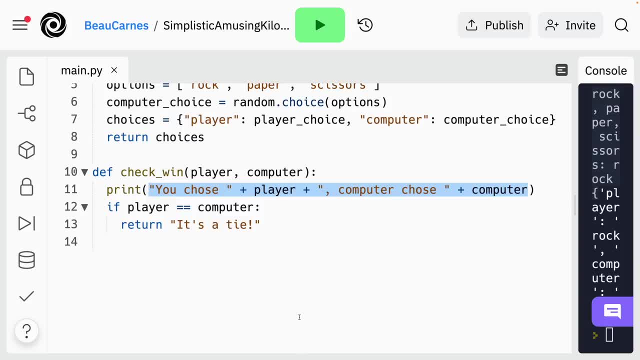 So this is one way to combine strings and variables together. There's another way that's a little simpler, called an F string. So an F string will allow you to make strings with and with variables and other Python code. So to do that, you just put a variable or you just put F. 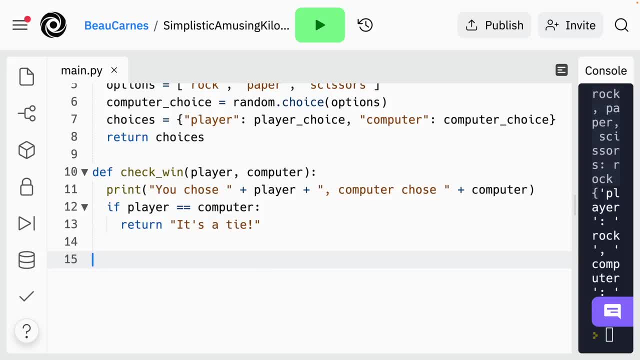 at the beginning of a string. So let me just give you an example. So we do, age equals 25, we're going to create a variable And then I'm going to make an F string. we'll make a string, And then we're going to create a variable, And then I'm going to make an F string. 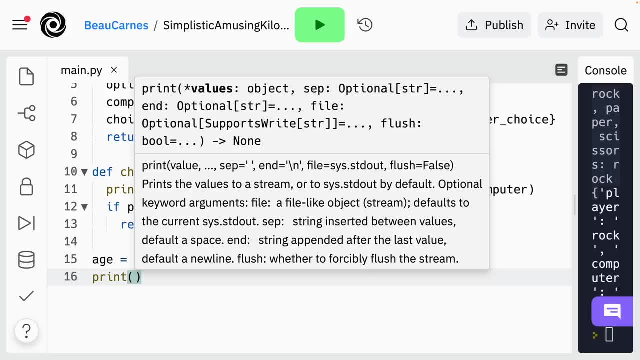 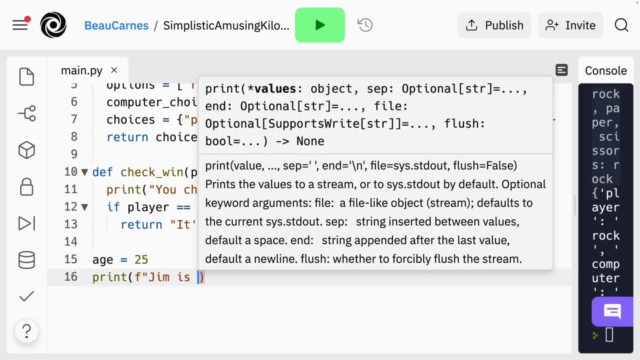 get a print statement And I'm going to put a string in here, But instead of starting with a quotation mark, it's gonna start with an F, And then I'm going to put Jim is, and then, whenever you want to put a variable or any kind of Python code, we're going to put some curly braces. 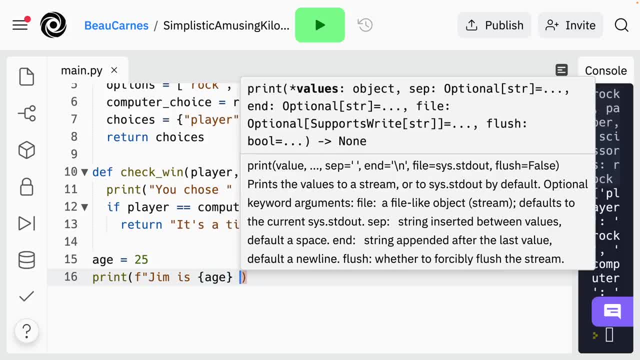 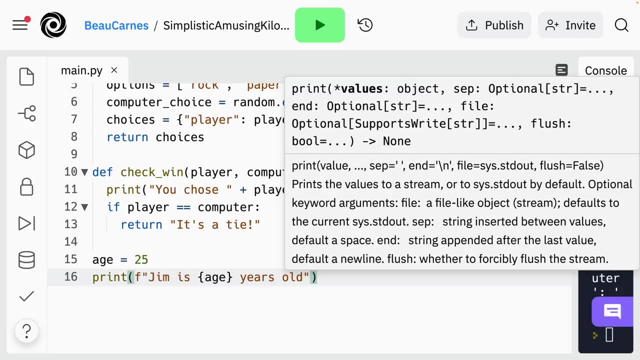 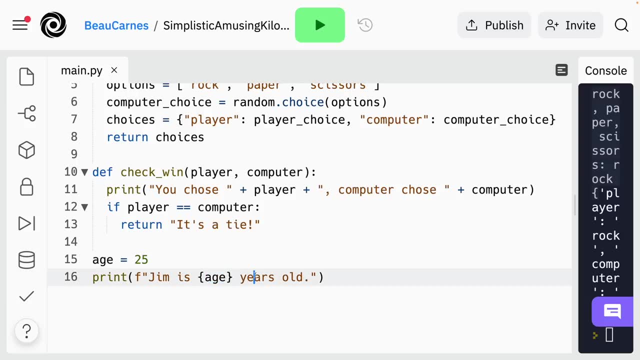 And I'm just going to put the variable within the curly braces- So years old, and I'll put the end of the string, or let me put a period here. Okay, so Jim is age, which is gonna be 25 years old. So the F string is just a slightly simpler way to combine the 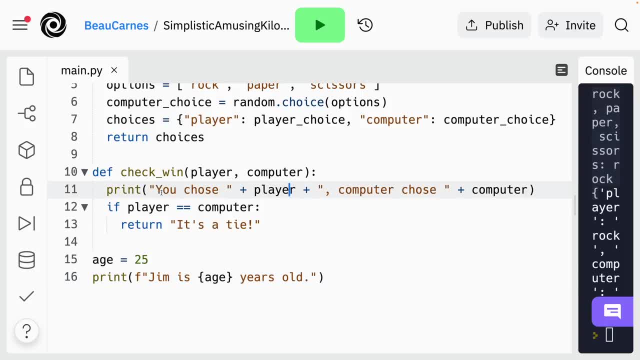 strings and the variables. So what I want you to do: see if you can figure out how to update this line right here. So it uses an F string and it uses these curly braces instead of all these pluses up there. So, yeah, we're gonna put F and they can delete a lot of these things here And 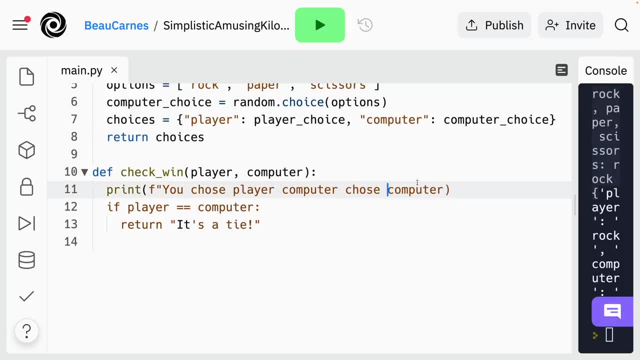 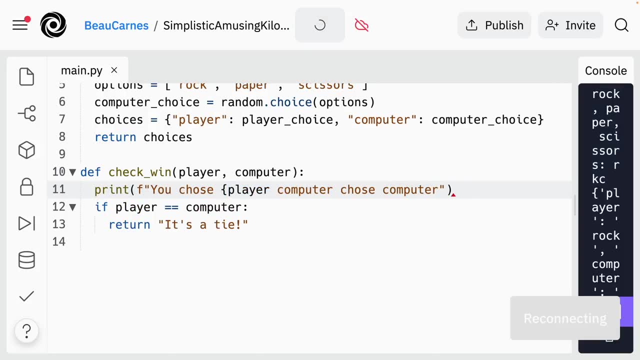 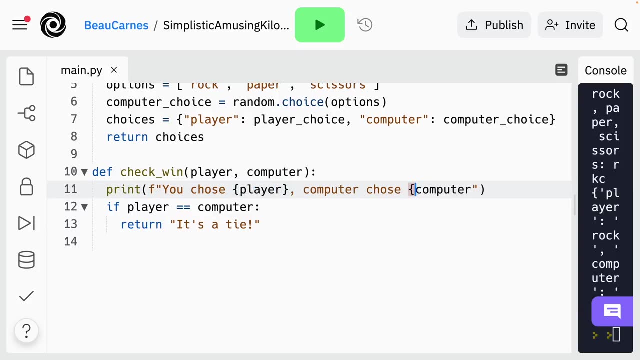 then I'm going to put some curly braces. you chose player, There we go, Okay. you chose there was a camera here. you chose player. computer chose computer- Okay. so now we've been able to put in the variable within this string with the F string. 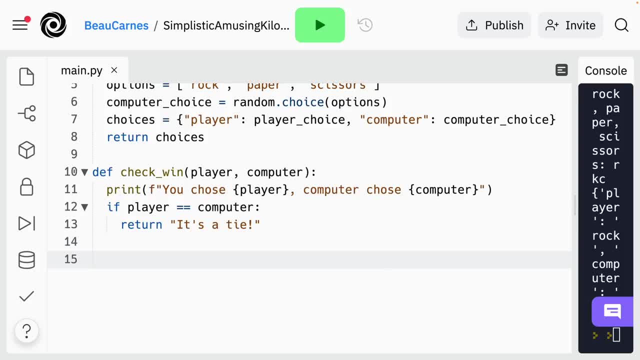 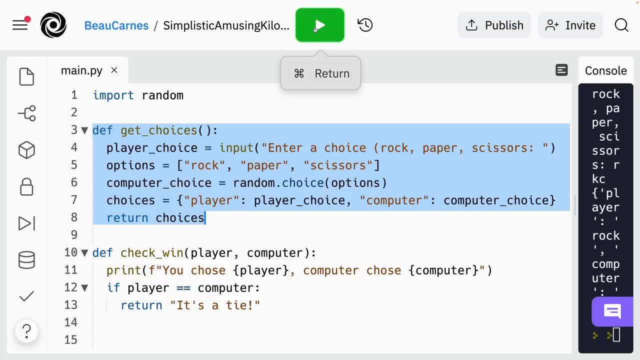 So we're going to test this out. So in a code the code in this function never gets run. So when we press the Run button it's not going to run any of the code within the function unless the function is called within the program. So we're not going to test out this function. all right now. 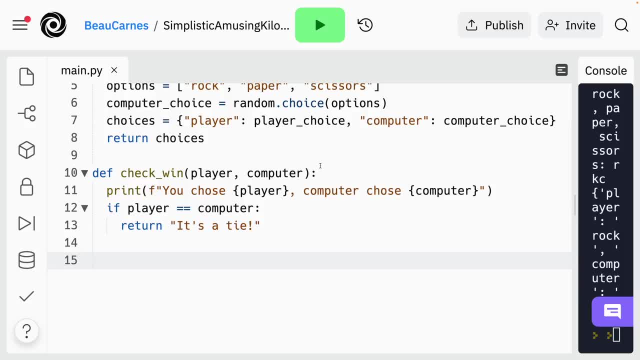 what I want you to do is see if you can add a line to call the check when function and just call it with rock and paper. So we're going to just do check when rock or x- we we have to pass in strings here- rock. 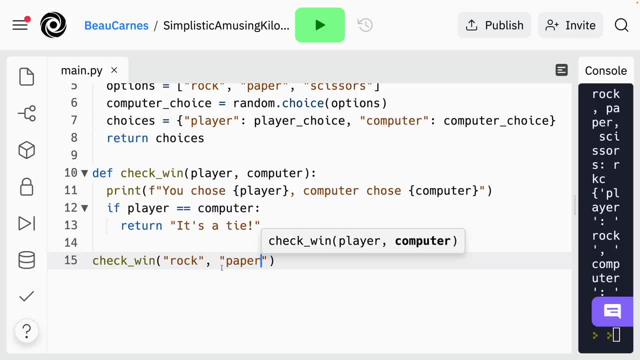 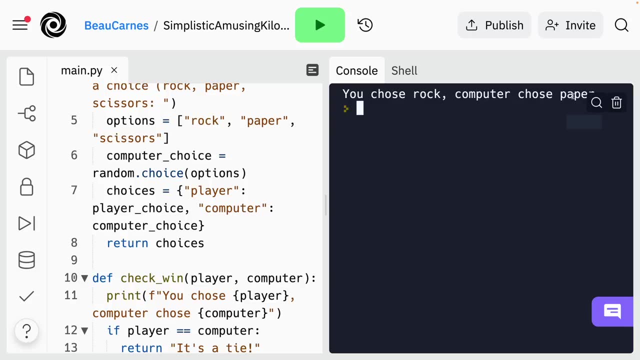 paper. So this is going to. it's going to call this function with rock in terms instead of player and paper instead of computer. So let me try to try running this program. You chose rock, computer chose paper, And just don't worry about that, I'm just going to call it rock And I'm going to 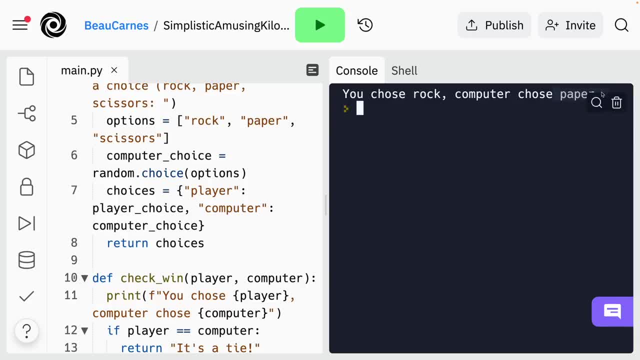 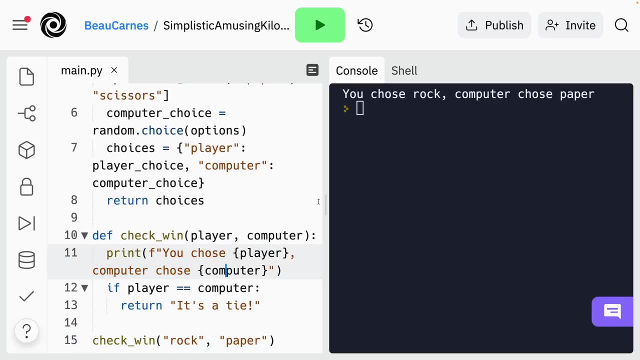 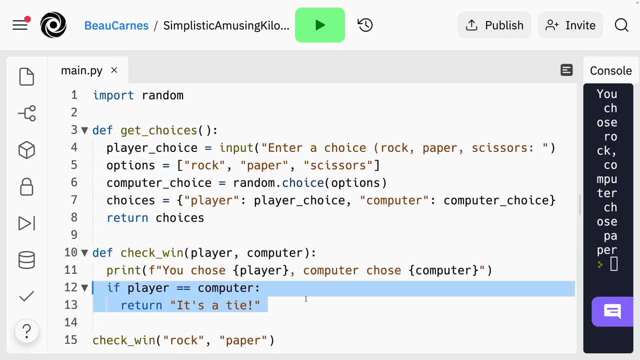 go out these little icons here. sometimes they just block what's in there, but it's still behind that little search icon, So it's to see it's doing. you chose rock computer, chose paper. Now let's get back to checking the winner. So far, this function is only going to check if there's a tie. 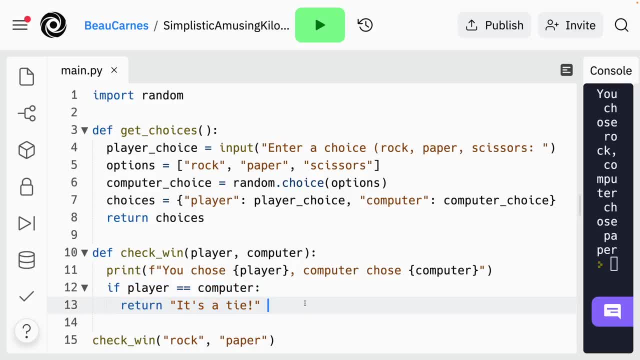 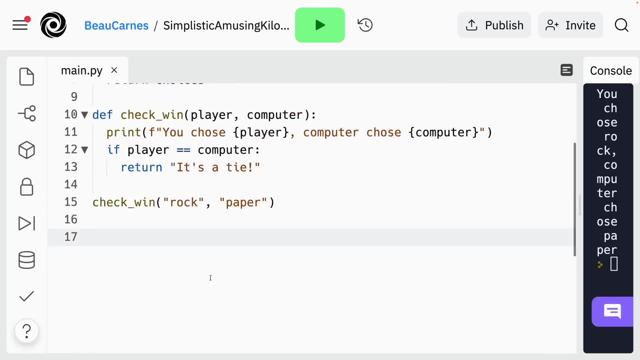 Now we'll start adding code to check different wing conditions. So let's learn about else and elif statements. Okay, so down here, I'm just going to give you, I'm just going to paste it in here, And I'm going to paste it in here, And I'm going to paste it in here And I'm going. 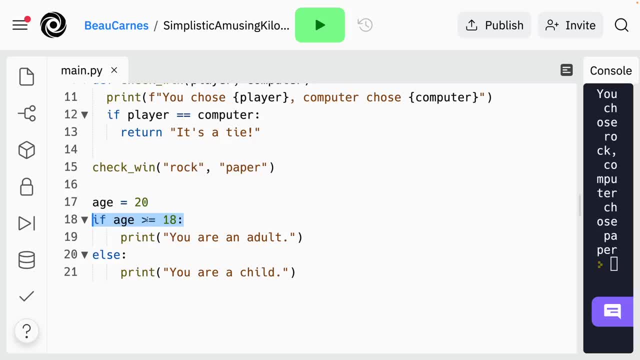 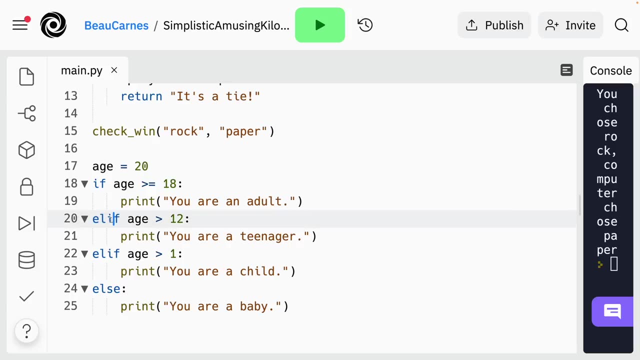 to paste an example. So So here's the if statement: if age is greater than or equal to 18, it's going to print this else. So anytime this is not true, then it's going to print your child. Okay, now here I've combined it with something else. that elif statement, ls just stands for else. 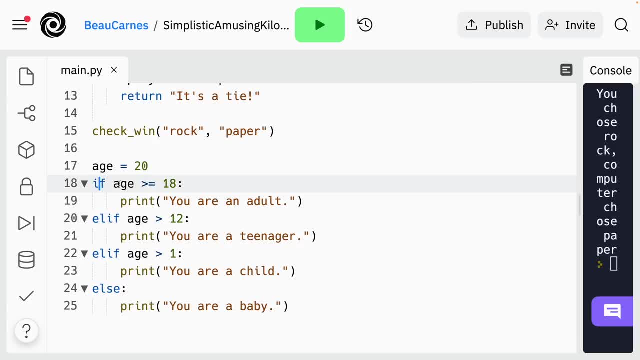 if it combines else, and if so you have to put a condition. So if age is greater than or equal to 18, print your an adult. else, if now we're going to check if age is more than greater than 12, you are a teenager. else, if age is greater than one, print you are a child, Or else, if none of 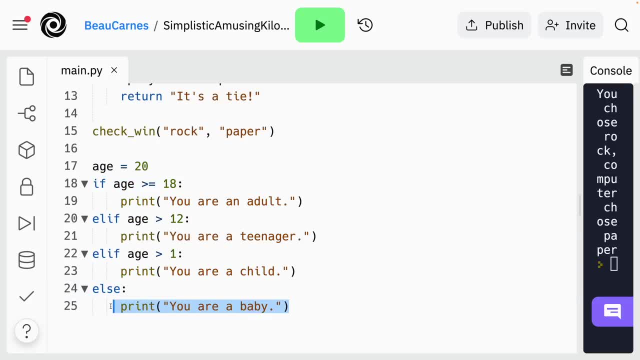 these other things are true. we'll just print: you are a baby, So it's only going to do one of these. it's going to get to the foot. once it gets to the first one, that's true- then it's not going to check. 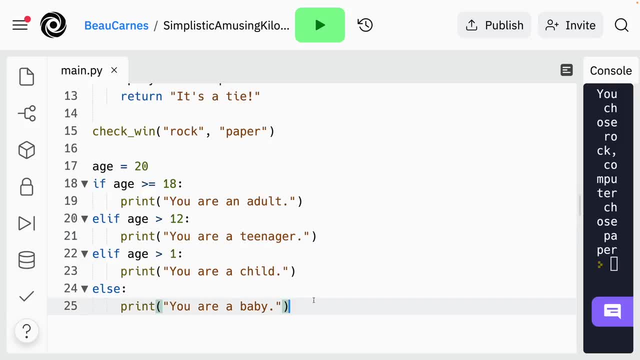 the rest, it's just going to kind of go to the next line of code after all these statements. So it's just going to choose one And then it's just going to go to the next line of code after all, and then once it gets the first one, that's true, then it's been done with this whole section of. 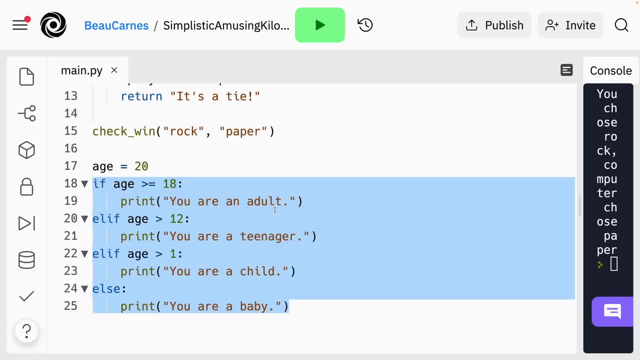 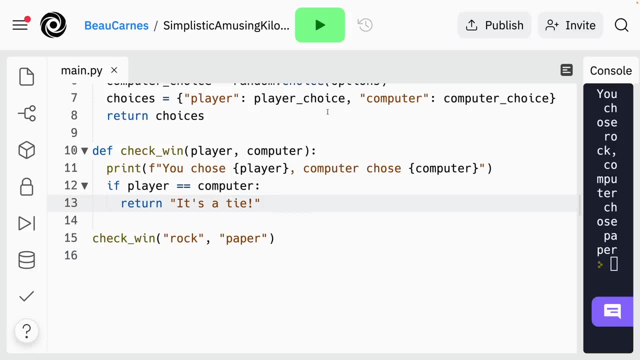 code. You can also check for two conditions at once. Let me give you an example. I'm just going to delete all this code And I'm going to create an lf statement here. lf else if, and we're going to check if player is equal to rock, And I'm just going to type in the word and, and computer is. 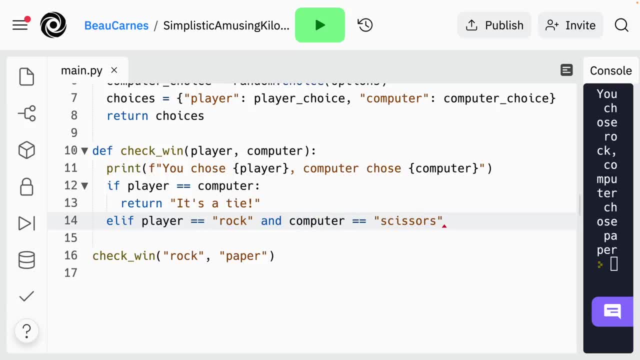 equal to rock, And I'm just going to type in the word and and computer is equal to rock, And I'm just going to type in the word and, and computer is equal to scissors. So now I'm checking if both these conditions have to be true. So this condition and this condition have to be true before the 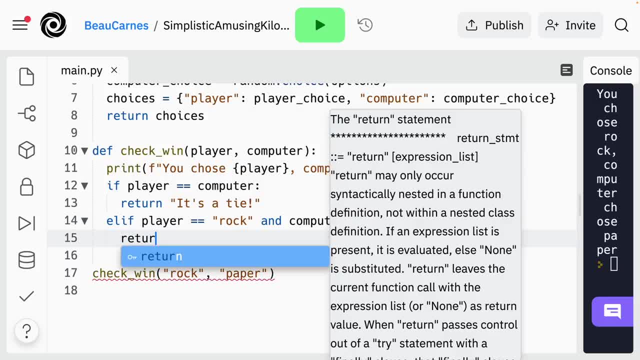 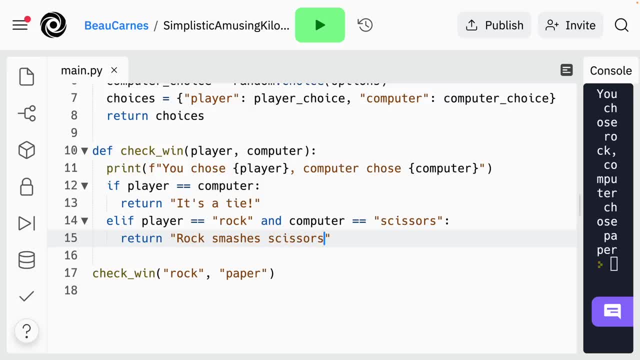 following statement will happen, which we're going to just put return: Rock smashes, scissors, You, you win. Okay, now the next thing we're gonna do- let's see if you can figure out how to do this- we're going to add another lf statement, And this time we'll check If players 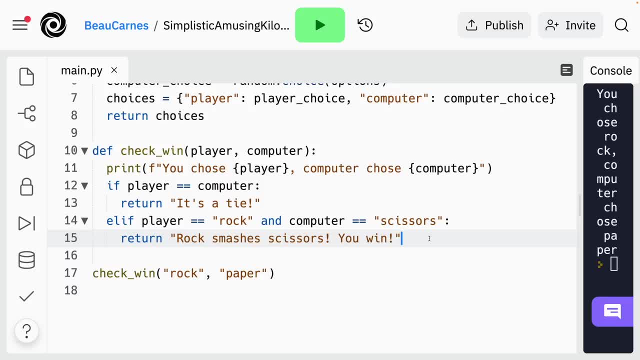 equal to rock and computer is equal to paper. And if so, we'll return paper covers rock you lose. So we're gonna make this kind of easier by just copying this code And then I'm just going to paste in this And then I'll just change this so players equal the rock and computer is equal to paper. instead of scissors. You know it's not an easy thing. I'm going to copy this down, So let's type in the word and I'm just going to paste it into this class And then I'll just change this. So players equal to rock and computer is equal to paper instead of scissors. 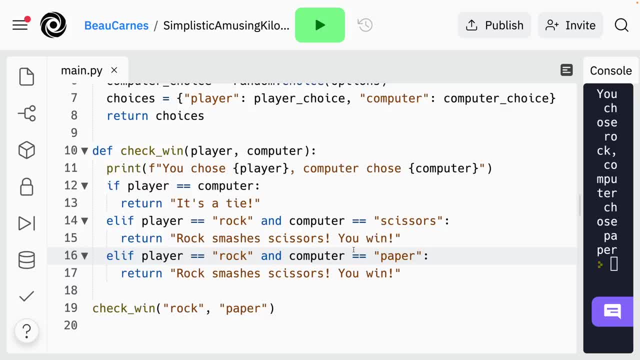 paper and it's gonna say: paper covers rock, you lose, And we won't even have an exclamation point anymore, because it's not exciting to lose. Okay, and you can kind of see there's a few. we could add a few more lf statements to cover all the different situations, But instead we're going. 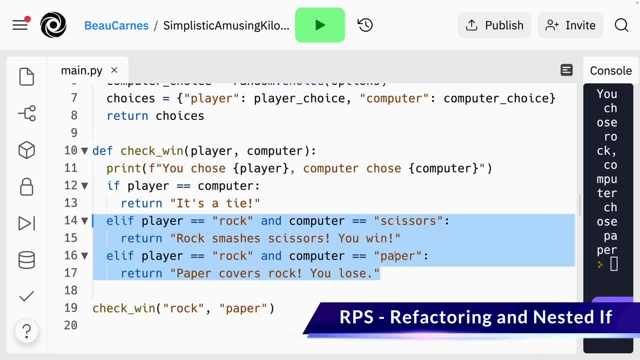 to talk about refactoring. refactoring is the process of restructuring code while keeping the original functionality When created. a pro, when creating a program, it's common to refactor code to make it simpler or more understandable. So we are actually going to refactor this code that I've 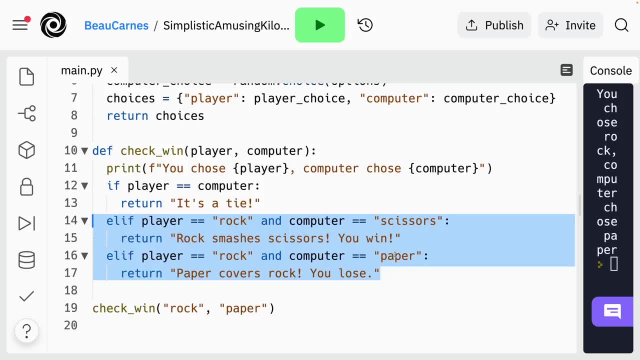 highlighted now And we are going to instead use a nested if statement. a nested if statement, a nested if statement, will make the code more understandable at a quick glance So you can put an if statement inside another if else or lf statement. So you'll notice here the first. 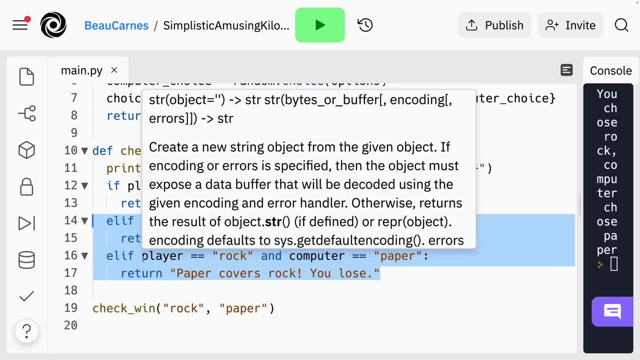 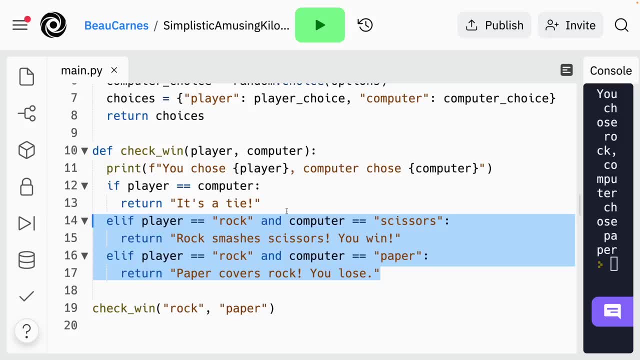 lf statement is if player equals rock and the second lf statement is if player equals rock. So see if you can figure out how to refactor this to not have to use the and anymore. we're just going to use one if statement and one lf statement, and then an if statement on. 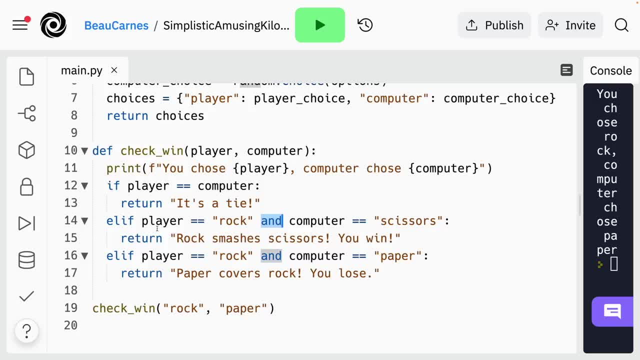 under that lf statement. If that doesn't make sense, you can just see what I do right now. So I'm going to just move this down a little bit. I'm going to actually copy and paste some of this, these items, but we're going to start with lf: player equals rock. we're not going to have this. 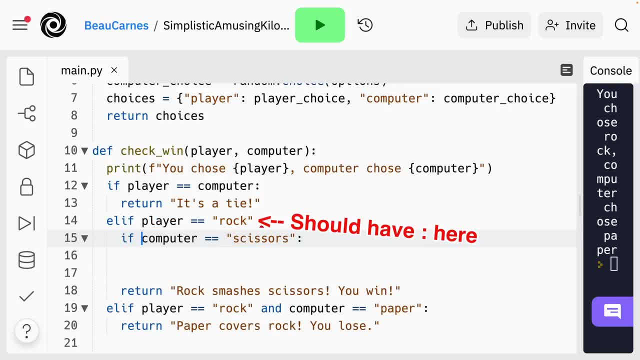 I'm going to put this on a new line and say: if computer equals scissors, So first we're going to check if player equals rock And then, if so, we're then going to check- it's going to be a nested if statement- if computer equals scissors. and if computer equals scissors, then we're going to use 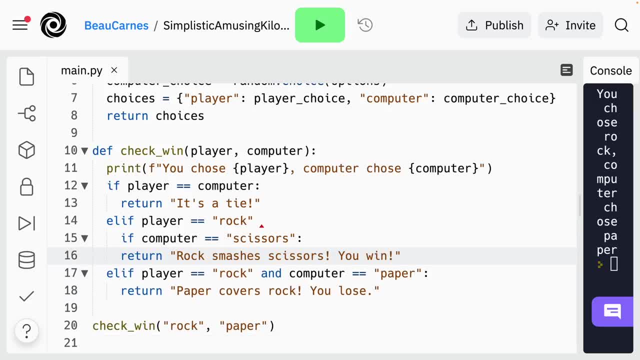 this, this return statement here, So I have to make sure it's indented correctly. it's going to read: so this will we have. we have player. if player equals rock, then if computer equals scissors will return. Oh, this needs to be indented one more time to be inside that if statement. And 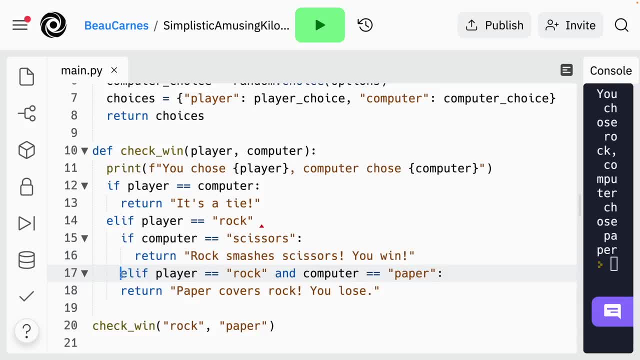 now we don't even need this lf statement. This can just be an else statement else. Because if the computer equals scissors, there's only one other option. because we already know: if player equals rock and computer equals rock, we'll have already returned. it's a tie. And, by the way, 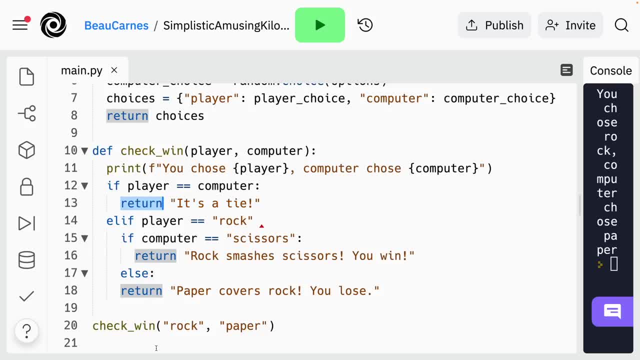 once you return something, the rest of the code in a function does not run. So for returning it's a tie. nothing else after that is going to run. So we know that computer can't equal the rock at this point. So it's either going to be scissors or paper. So don't, we don't even have to check. 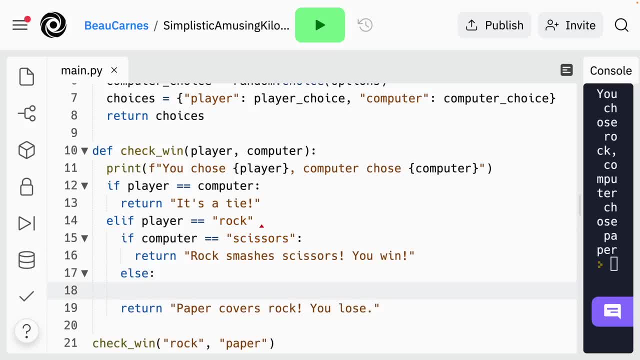 if computer equals paper. So we don't even have to check if computer equals paper, because at this point computer has equals paper, And then we'll just return this this line. Let's see, There we go. Return paper covers rock, you lose. So now we just basically have to add two. 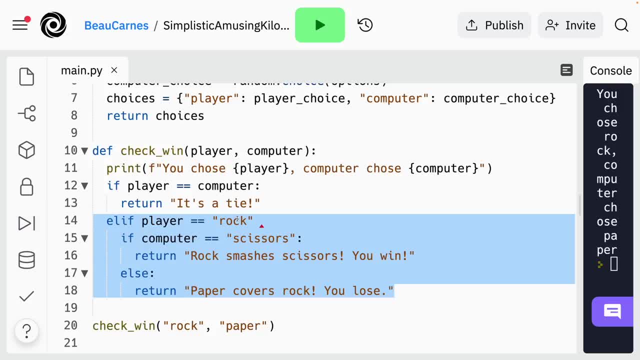 more sections similar to this. So this one is: if player equals rock, then we have to have another section if player equals paper, and then if player equals scissors, and then we just have to have. the stuff inside is going to be pretty similar, just corresponding to the different relationships between rock, paper, scissors. So 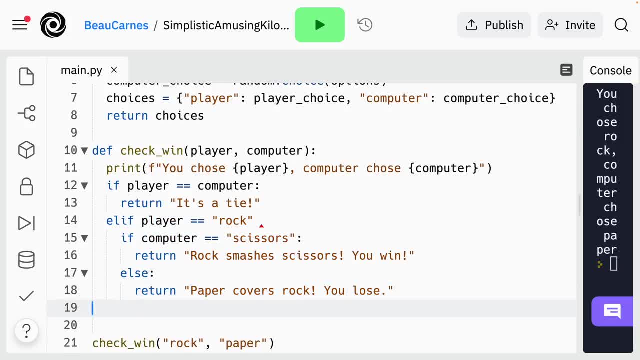 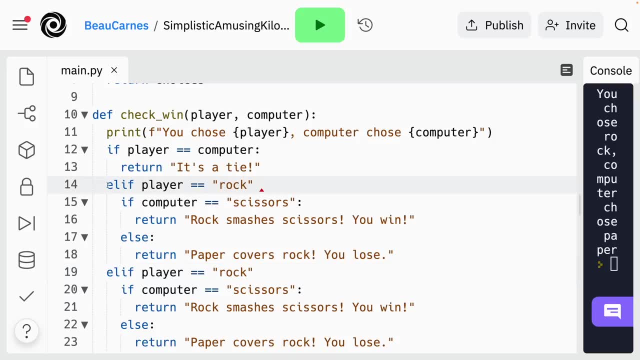 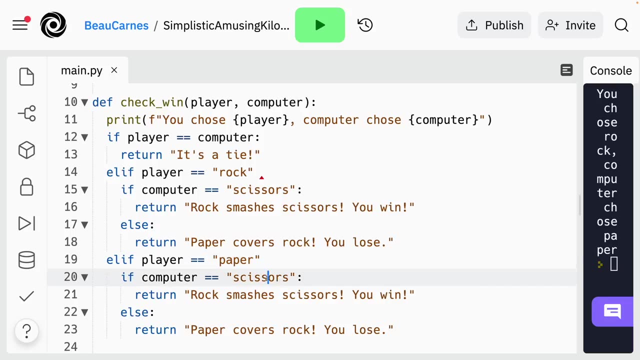 I'm just going to copy that And then I will paste it here. And then one thing important you to make sure this LF statement lines up with this LF statement And this is now going to be paper. And then we are going to check if computer equals rock and a computer equals rock, then we will. 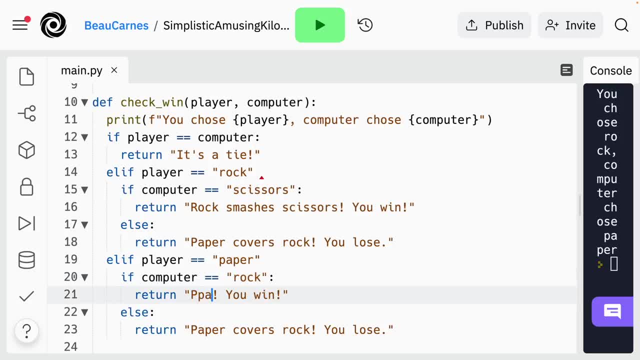 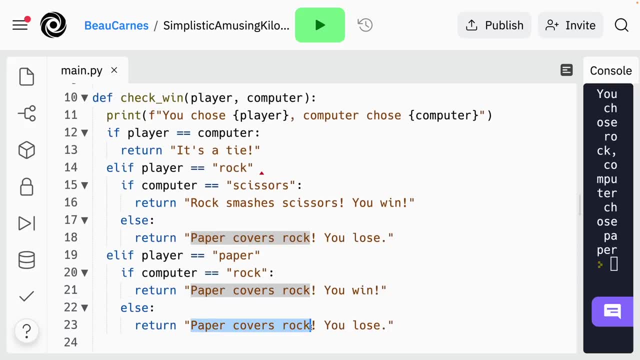 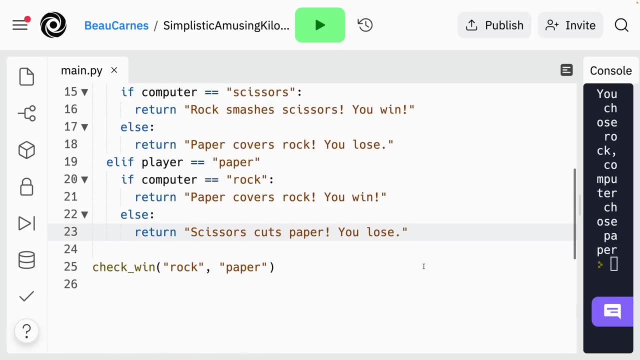 say that paper covers rock, You win. or we'll say: scissors cuts paper, you lose. And then the final one, which at this point I'm sure you can figure out on your own: we're gonna add one more. 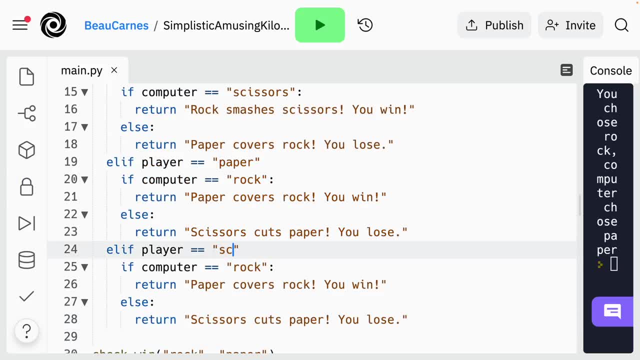 section, And it's if player equals scissors. And then first we're going to check if, if, if, if, if computer equals paper, If so we will do: scissors cuts paper. what is it making sure we're just? 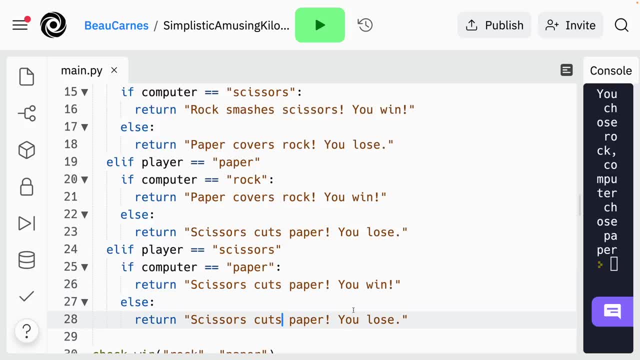 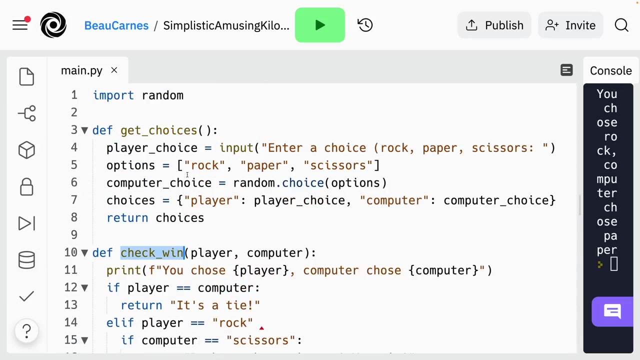 making it so every time the first one is you win and second one is you lose. but you could do it the other way around, And then we will do rock, smashes, scissors- you lose. Okay, we're almost finished with this whole program. So both the get choices function and the check when function. 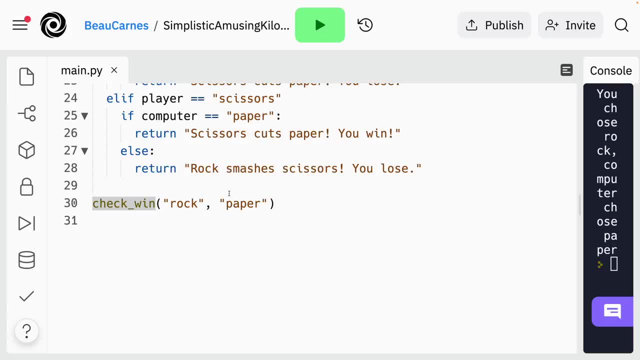 they're both complete. Now let code to call the functions and play the game. So first let's remove this, this check, when now we'll create a variable called choices and make it equal to the result of golf, calling the get choices function, And we just have to make. 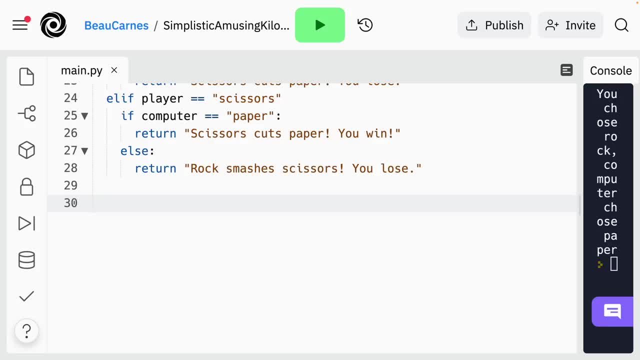 sure it's not indented, It's on the first. the first column, I guess right here not ended at all. So we'll do choices equals get choices. And one thing about this is it's going to return a dictionary. So if we look at the get choices, so it's returning choices. 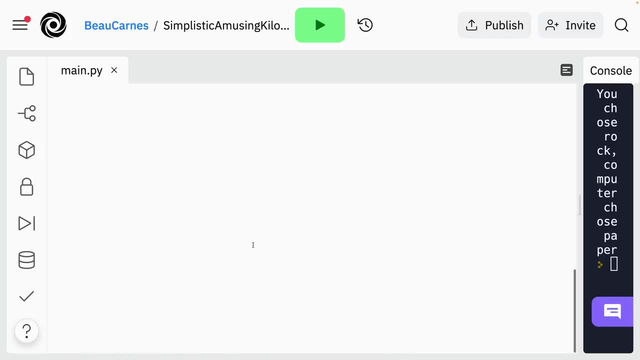 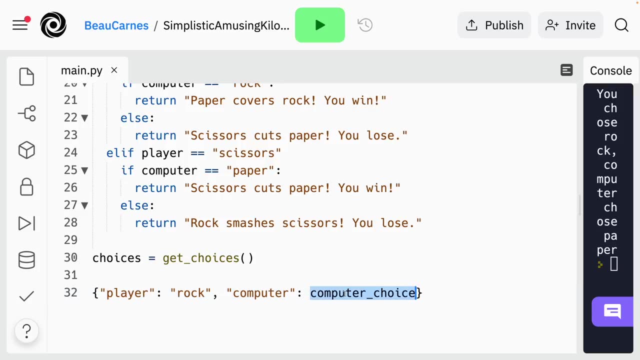 and it's going to be a dictionary like this. Now let me just copy this. I'm going to show you something down here. I'm going to just paste it down here And we'll just make an example of what it could look like. it could look like rock. 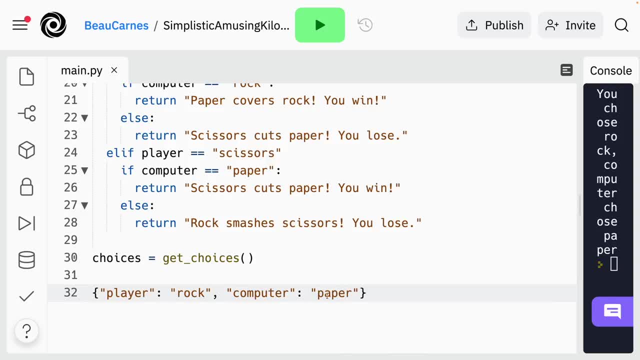 and paper. I always use rock and paper as examples, because scissors is a little harder for me to spell, So that's a little easier. So, so let's. one thing we haven't talked about is how to how to access a specific element within a dictionary. So this is a dictionary, So let's. 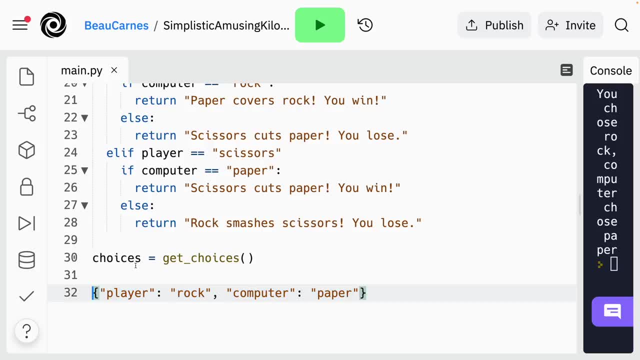 say, if I call this, we'll just call it choices, even because we're going to delete that, And so we're only going to have this choices. But choices equals this. And let's say: I just want to get the choice of the player. Let me show you how I would do that. I'll just do p choice for. 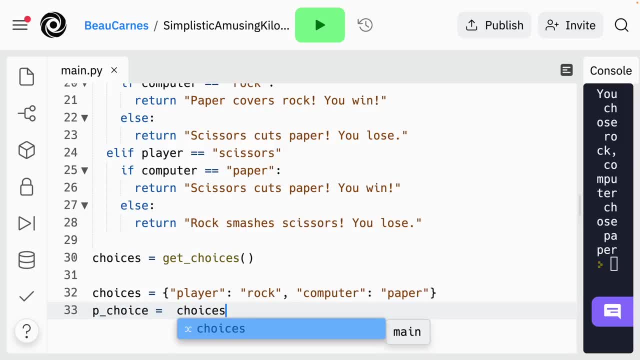 player choice And I'm going to put equal choices And to get just the value of the player. I'm going to put brackets, So the brackets look like that, And then I have to put the, the key that I want the value of. So the key would be player. 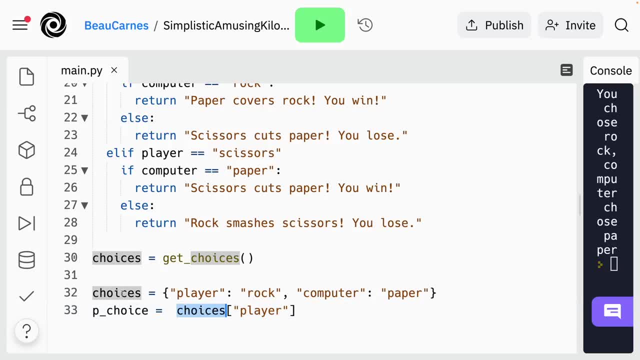 So if I put the name of the dictionary, which is this, and then I put some brackets, we're going to use brackets to identify what is the key that we want the value of. So here's the key of the with the value of rock And here's a key with a value of paper. So this is how we can. 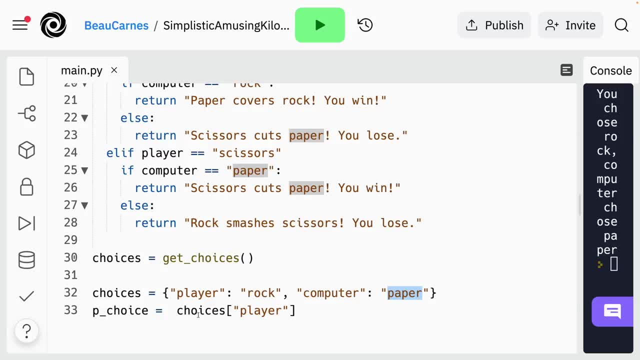 get the player choice And I'm sure you can see how you get the computer choices if, instead of if, we take this computer word and put it right here: Computer. Okay, I'm going to call this value of rock And I'm going to put the value of rock And I'm going to 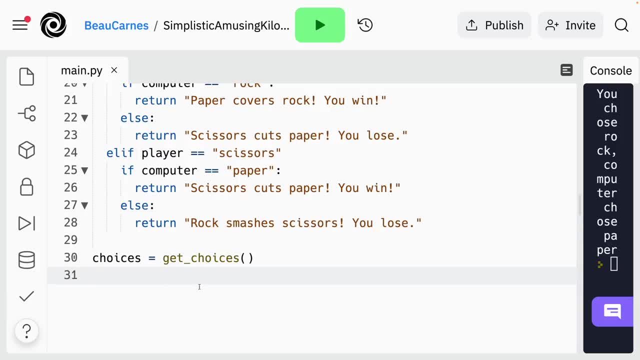 I'm just going to get rid of all this here, And we're gonna. we have to get choices here And now listen carefully to what we're going to do next. we are going to create a variable called result and make it equal to the result of calling the check win function. And when we call the check win, 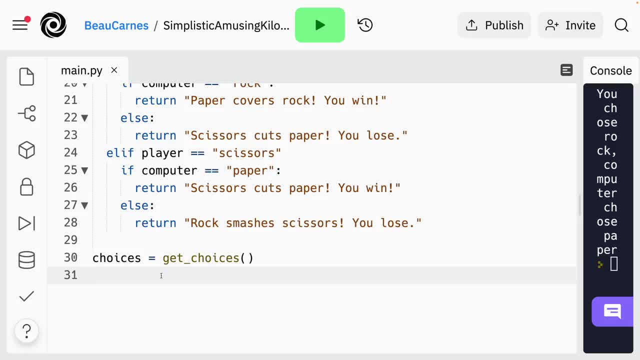 function. we're going to pass in the value of the player key and the computer key of the choices dictionary. So let's do that. So then you'll see what I mean Result is going to be. we're going to call, check when, And then we are going to pass in. we're going to pass in with choices- player and choices. 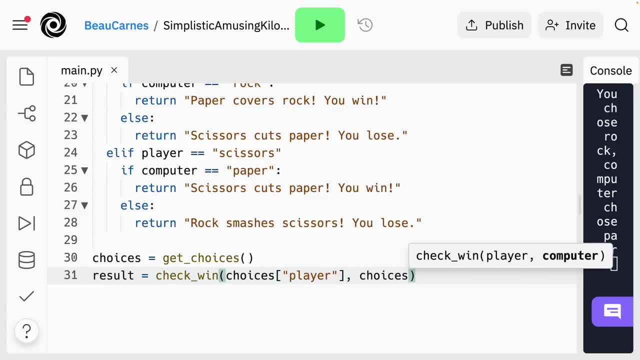 Computer. So because, remember, we had- I showed the example- that dictionary. so we're getting the player key, the value of the player key and the value of the computer key. So now we know who wins. Well, we've now this result. variable is going to be. one of these strings have been returned: either it's a. 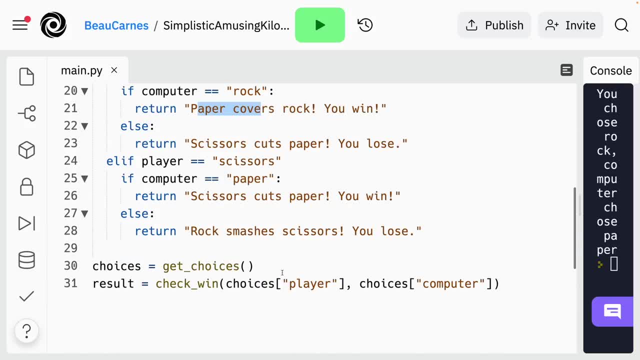 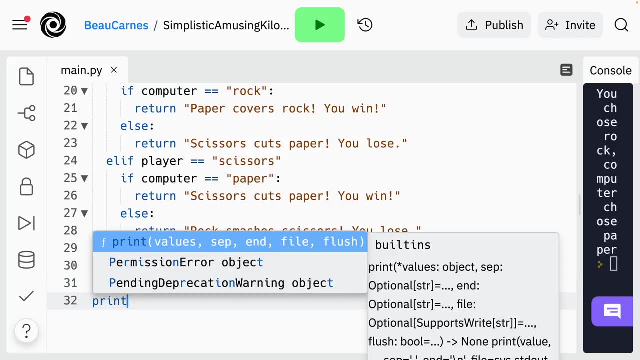 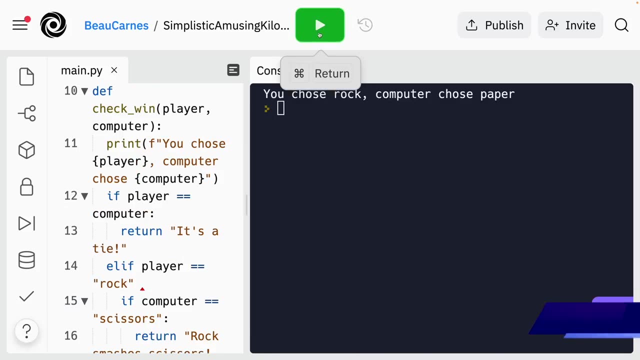 tie rocks, faces, scissors, paper covered rocks and so on. So now we just have to print the result. We're going to print the result. Okay, we can try out this game. I'm going to just click the Run button. Okay, this is why it's. 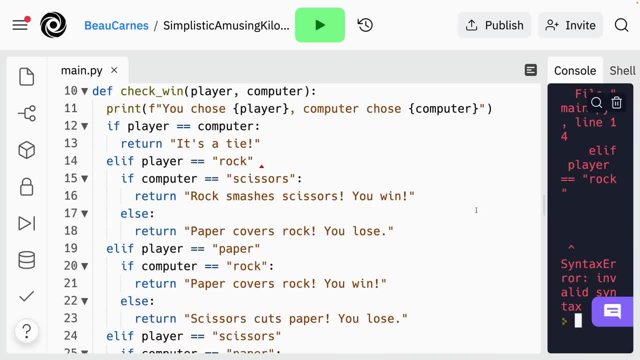 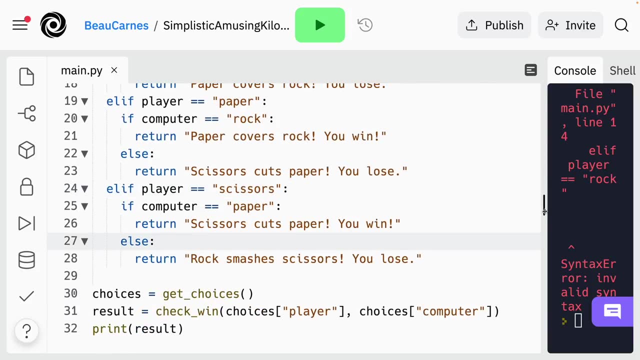 sometimes better to test a little earlier. I just forgot the semi colon on some of these. So semi colon And see, I see there's a red arrow. I should have seen that. semi colon and semi colon. Okay, now let's try it. I'm gonna play the program. 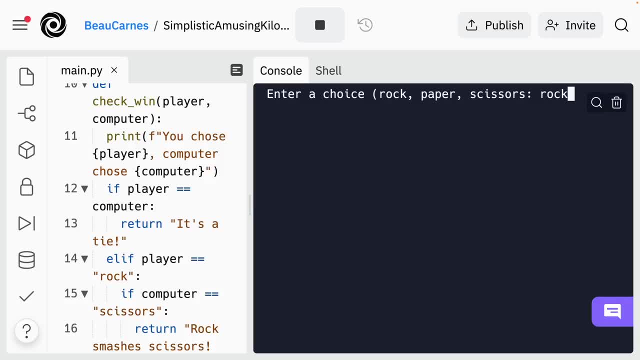 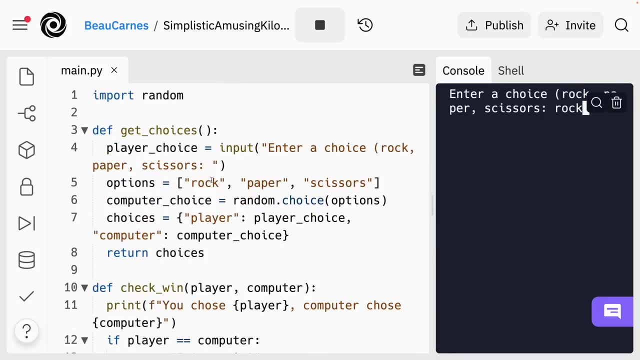 Intra choice. I'm going to do rock And I just noticed something else I want to change. So intro choice, Yes, such that there's a parentheses here. there's no parentheses at the end. So, again, I'm just going to change that really quick. So enter a choice And we're going to put it in. 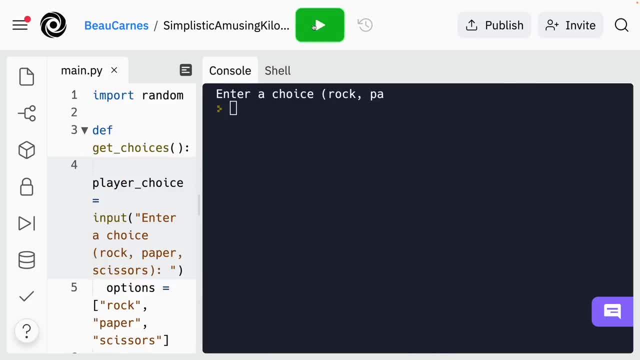 parentheses here and test again. So rock- Okay, you chose rock. computer chose rock. It's a tie. Okay, I'm gonna play it again. Paper, You chose paper, computer chose scissors. scissors cuts. paper- you lose- Okay, we just created a Python game, So hopefully this gives you a better. 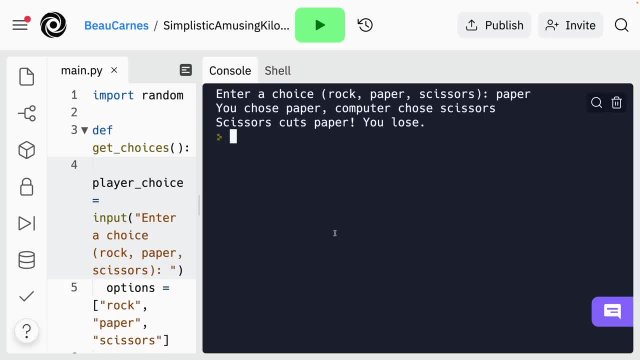 understanding of what it's like to program in Python And you. you now know about some of the basic concepts of Python. Now there's a lot more to learn in Python And we're going to be covering a lot more in this course. I just wanted to start with a game and a full program, So just right off. 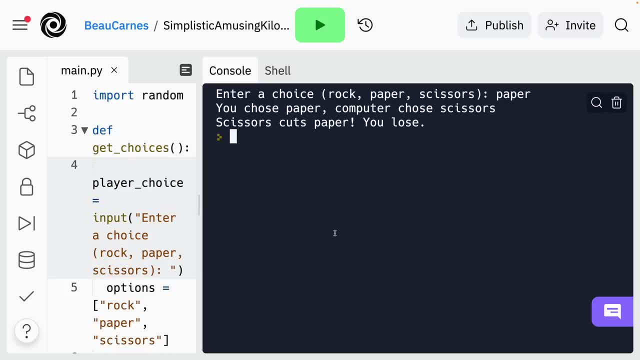 the bat you could code a program. So in the next section I'm going to show you how to code a program. So in the next section I'm going to show you how to code a program. So in the next section I'm going. 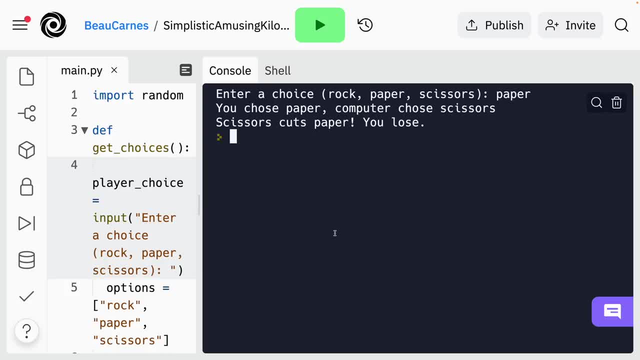 to start going over in detail all the most common features of Python, And we're going to cover some of the features that we've already used in this game, plus a lot of additional features, additional common features that were not used in this game, And then, in the final section of the course, we're 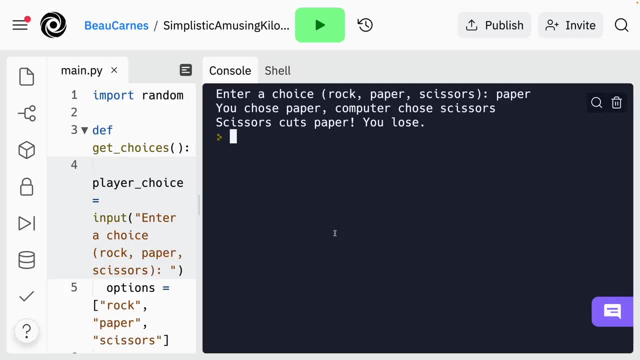 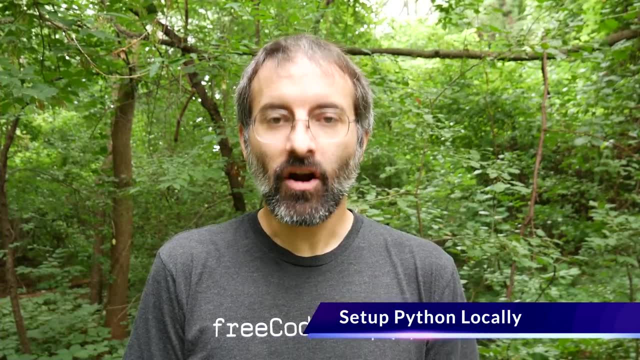 going to code a more complex game, a blackjack game. So let's get started with the next section. One of the quickest and easiest ways to code a game is by using David's actions, So I just want to. ways to get started with Python is by using repletcom, But you may also want to get Python. 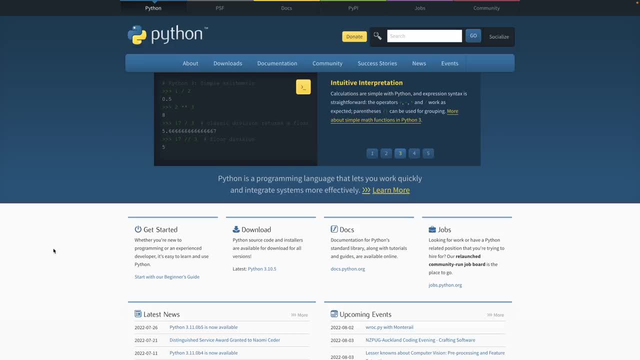 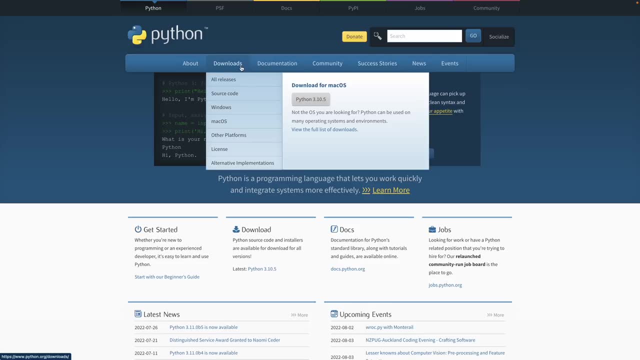 running on your local computer. So if you want to do that, you can start by going out over to pythonorg And these go to the downloads menu And then you're going to just click what you want to download for it for. so it's going to default to be for you the operating system you're on. But 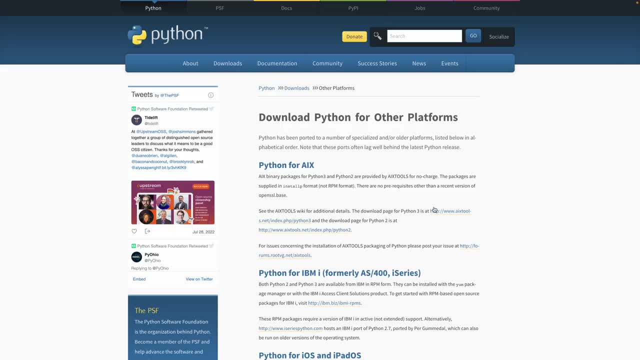 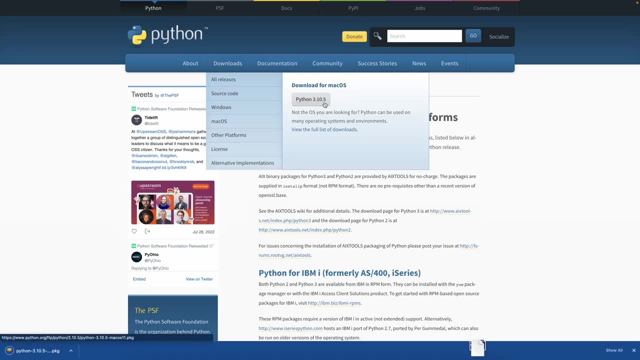 you can also go to other platforms and make sure you can then just find the platform that you want to download on And there's going to be instructions on here that's going to tell you how to go about getting installed on your specific computer. So there's a few different ways to run a Python. 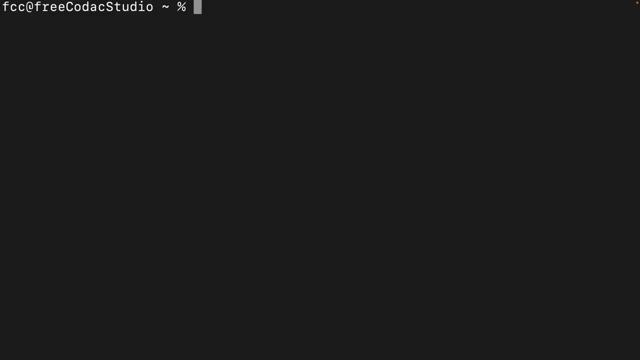 programs, And one of the ways is with an interactive prompt. So after you get installed, if you open up your terminal and type in Python- or sometimes it's going to be Python three, depending on how you got installed- you're going to see this interactive prompt And then you can. 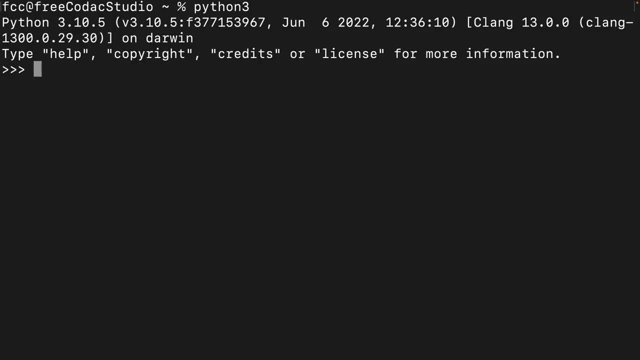 just this is called a Python rest, And then you can just this is called a Python rest, And then you can just type in the variable name, name, and it's going to show you, show me- the value of the variable And you can type in most different. 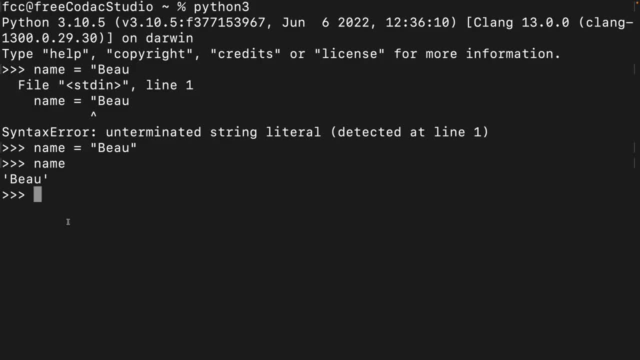 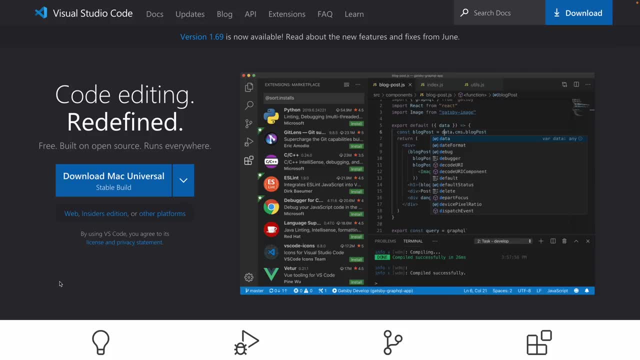 Python commands right into this interactive prompt here, And then I can just quit it when I'm ready to quit. It's also common to run Python using Visual Studio code. So if you just search for Visual Studio code you can get to the download page And then you can just download it for your. 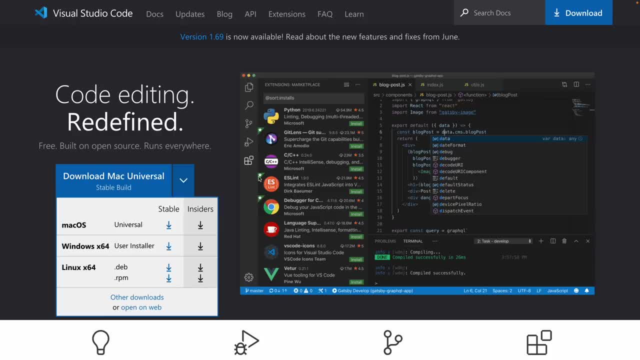 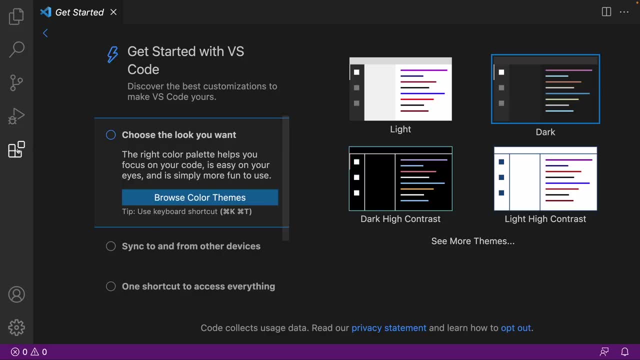 system And there's also you can download for different systems. And then, once you open up Visual Studio code to get Python working, you're going to want to install the Python extension. So I'm going to click over here to extensions And you can search for Python, or it may just be listed. 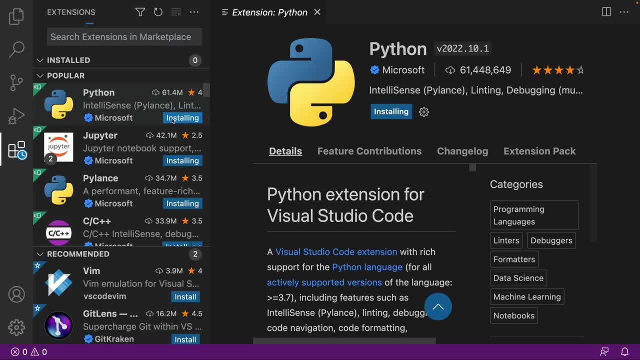 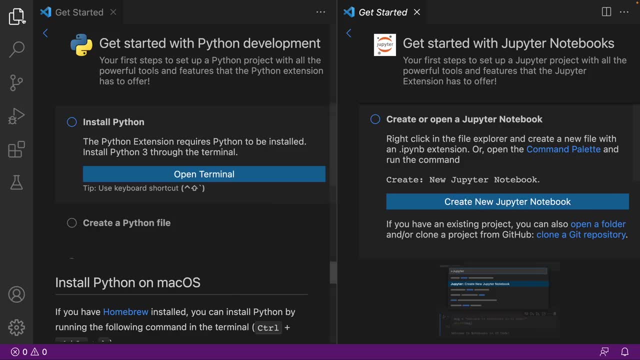 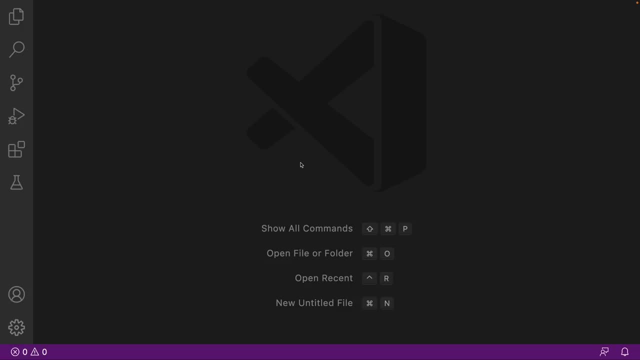 here under popular extensions And I'm just going to click Install And this is going to make it easier to work with Python on Visual Studio code. So now I can just kind of close some of this stuff here And I'm going to create a new file And I can just call the and I can just type a name. 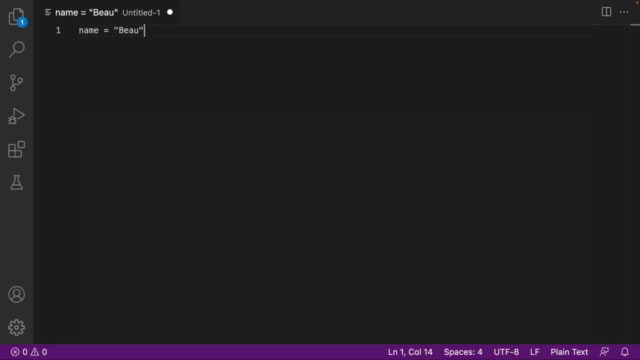 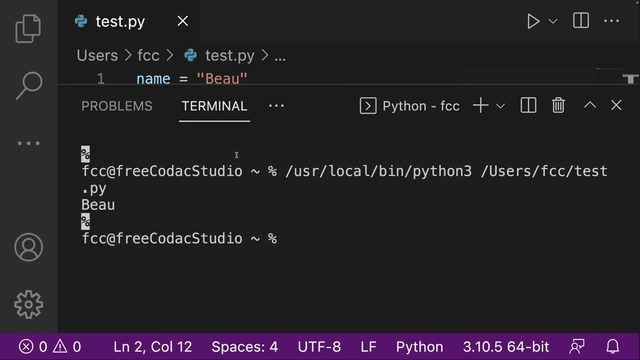 Equals bow print name. And then, if I save this as test dot pi, it's going to now it's going to add the colors that correspond to Python And then I'm just going to click this play button here And it's going to play, it's going to open up a terminal window here And it's going to run the program And 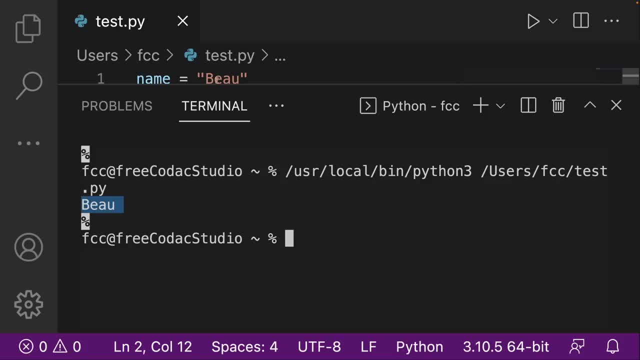 it's going to print bow And then I'm just going to click this play button here And it's going to go. That's what my program did. If I zoom out a little bit, you'll be able to see the difference. 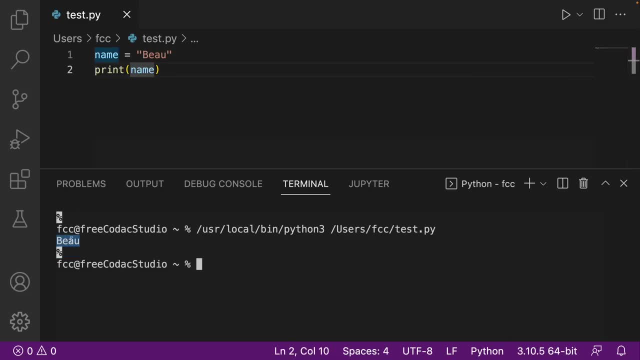 So we just print the name and it runs the program just like that, And then you can see on the terminal how they the command that was used to run that. So we could use the same command on any terminal And instead of typing this whole thing for the location of Python three. I can just do. 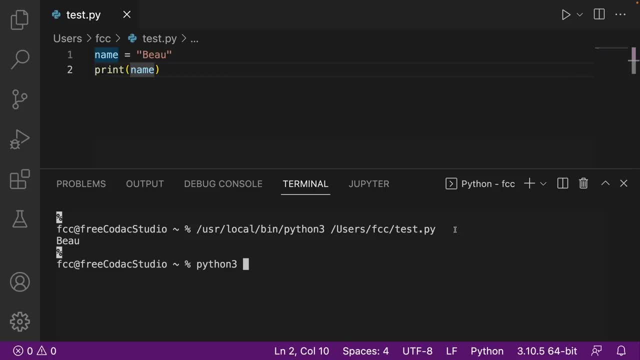 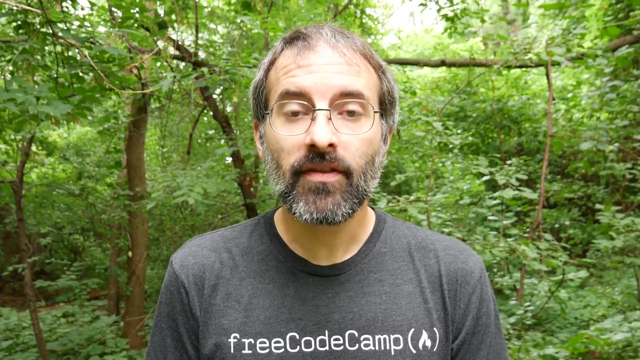 Python three And then you- this is where that file is located, So just copy that And I can paste it in here And it's going to run that program. In this section we'll learn about the core features of Python. I'll go into more detail about some of the things we learned in the first. 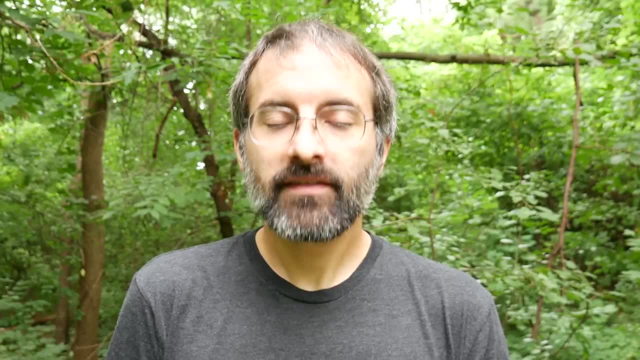 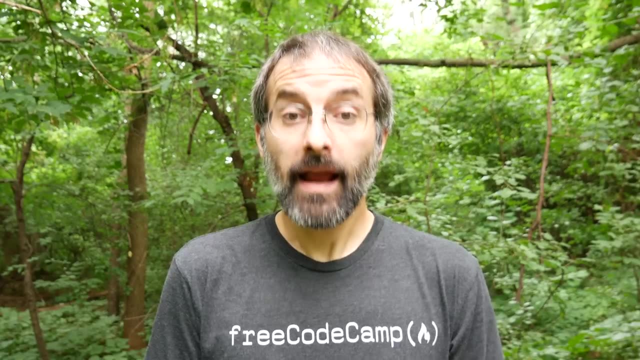 project And I'll be covering a lot more concepts. This section was heavily inspired by the Python handbook by Flavio copes And you can check that out. on free code, camp news And, like the first part of the course, I'll be writing Python in replit, So once you get logged into replit. 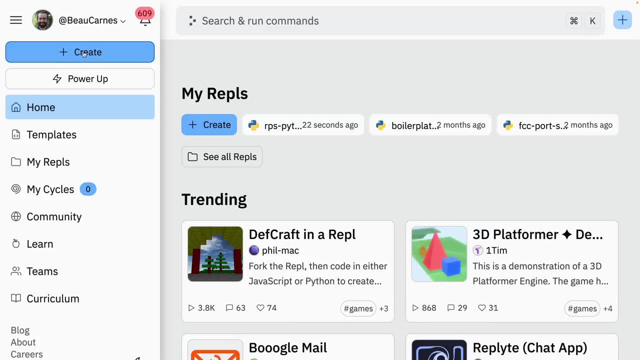 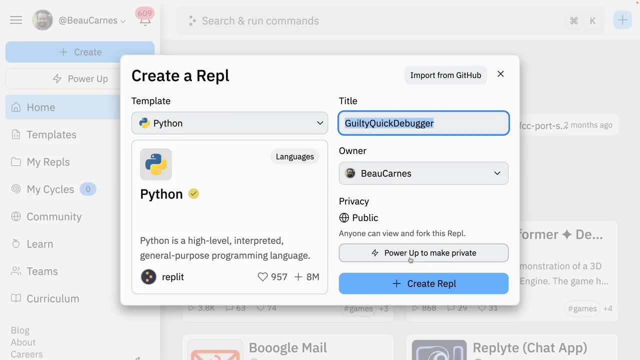 just like I already showed you before, you can hit the plus button here or the Create button to create a new replit, And then you can search for the programming language, Or you can just click it down here: Python. we'll just create a Python repl And then we can. 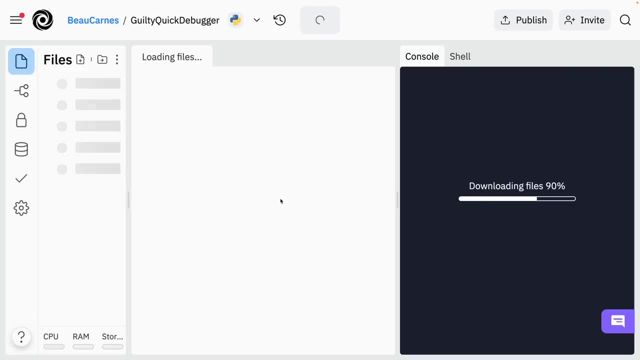 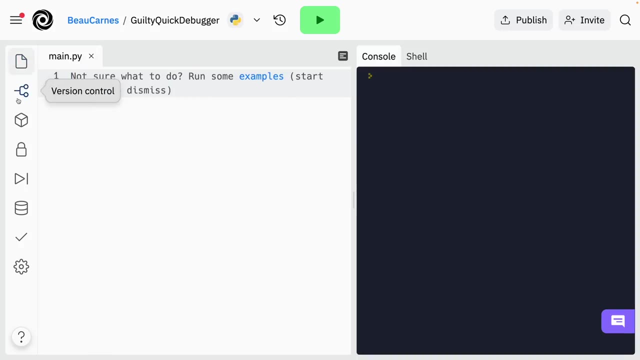 instantly start creating writing Python code in replit. So, like I showed before, we got our different files here. we're just going to start by using one file here And this we're going to code and this is where it's going to appear if we run the code. So I'm going to close off the list of 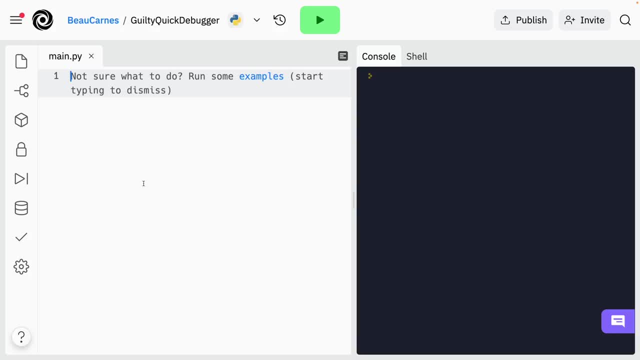 files here And let's just start at the beginning again. So you've gotten used to coding in Python through creating a rock paper scissors game, But now we're going to kind of do a deep dive into all the basic commands of Python. So there's going to be some review, but we're going to be going into more. 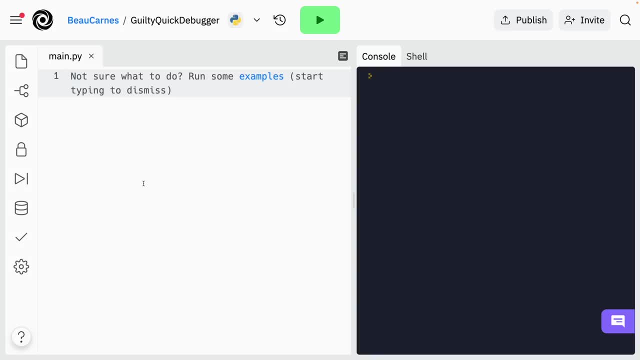 detail about each of the elements, And the first thing we're going to talk about is variables. So we can create a new Python variable by assigning a value to a label using the equal sign or the assignment operator. So let me give you an example, just like I was showing you. 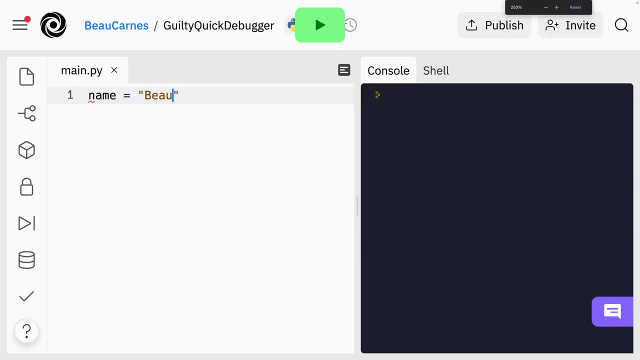 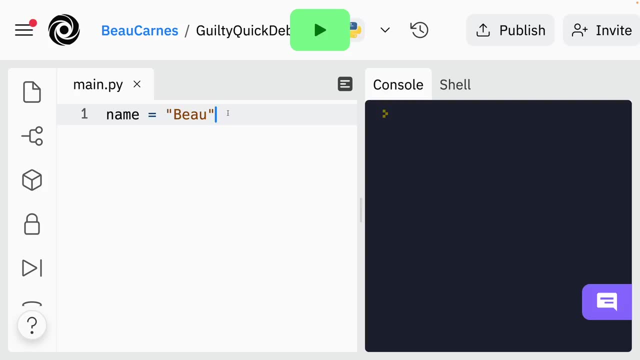 before. just name equals bow. So let me just zoom in a little bit more here. And so now our variable name is name and we've assigned it the value of bow, And then we can also create. we can create a variable with a number, So I could do: age equals 39. So a variable name can be composed of characters. 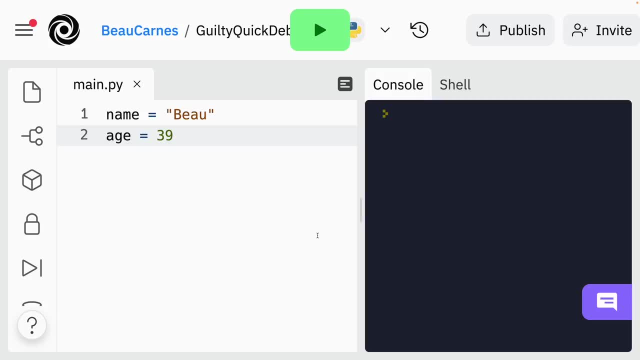 numbers and an underscore character, but it cannot start with the number, So it could be anything like name one, it could be all capital letters, it could be. it could have an underscore, it can start with an underscore, like I said, like that, And you can see that these are all. it's putting these red. 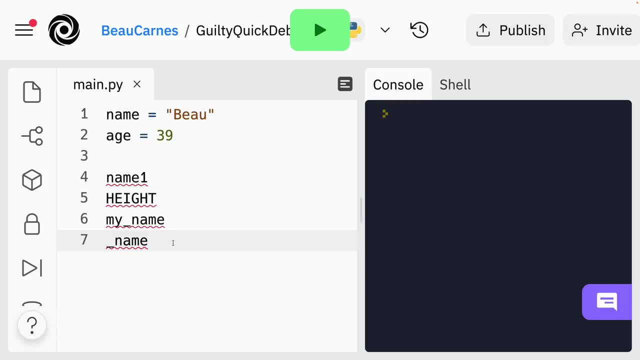 squiggly lines because it's showing that that's not actual Python code. if you're going to create a variable, you should be assigning it to a value or you should be using a variable that already exists. But I'm just showing you some. 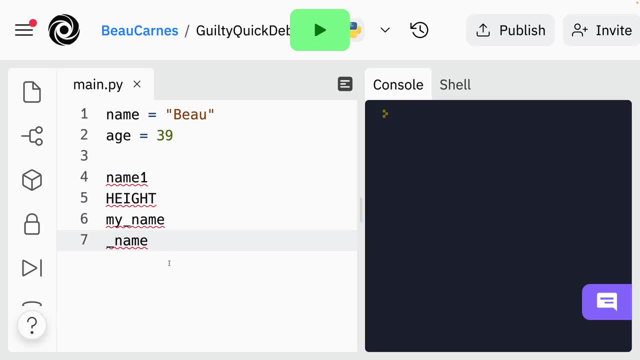 different examples of different variables Now. So here's an example of an invalid variable name. if you just start with a number, like that, that can't be a variable, because you can't start with a number And I couldn't put something like test exclamation point. you can't use exclamation. 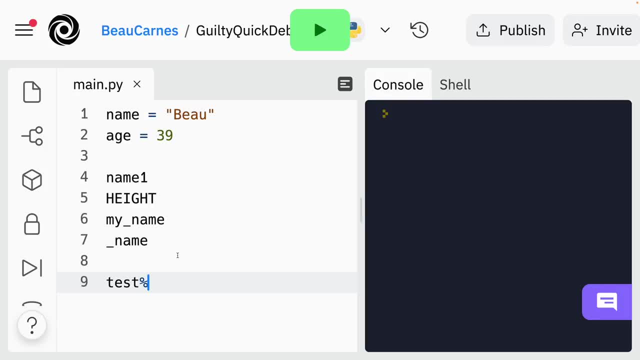 points. you can't use percent signs And other than that, anything is valid unless it's a Python keyword. So there's some keywords. a keyword is something that's used to to write Python, like for if, while import. these are all words that have very specific meanings within Python, so you cannot use. 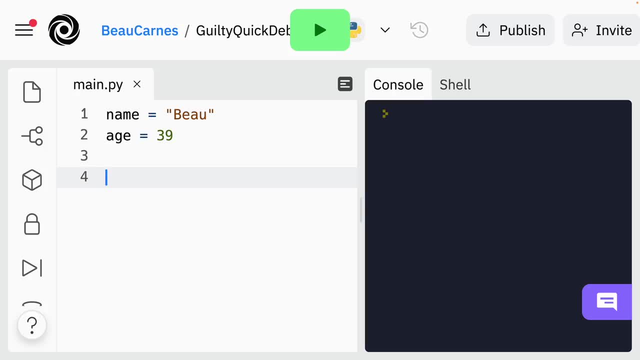 them for a variable name. Now there's no need to memorize them, as the Python editor here will alert you if you use one of those as a variable. So that was just like if I say if equals hi, and then you can see it's going to show you right here with these squiggly lines that we've done. 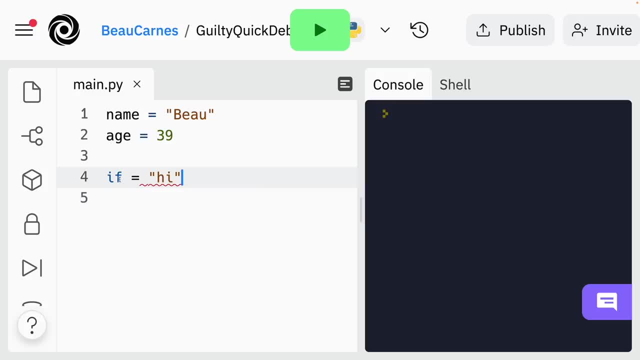 something wrong, invalid syntax because- and then also you can see that it turns blue. this word turns blue because it's a keyword. you can't use it as a variable name. So, like I said, it's an alert you, if you, if you use a keyword as a variable, and you'll start to gradually 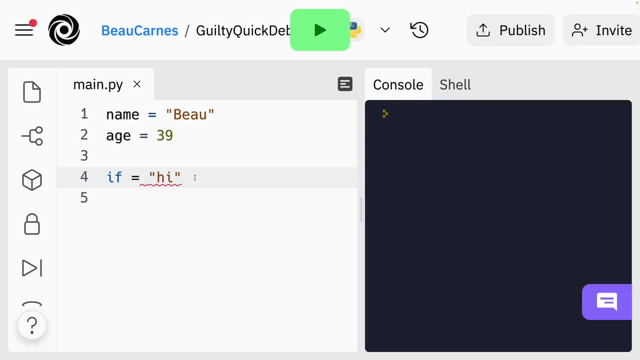 recognize them as part of the Python programming language syntax. Now let's talking about talk about expressions and statements in Python. So an expression is any sort of code that returns a value, Like friends, if you do one plus one, or if you just do a string like bow, this is going to. 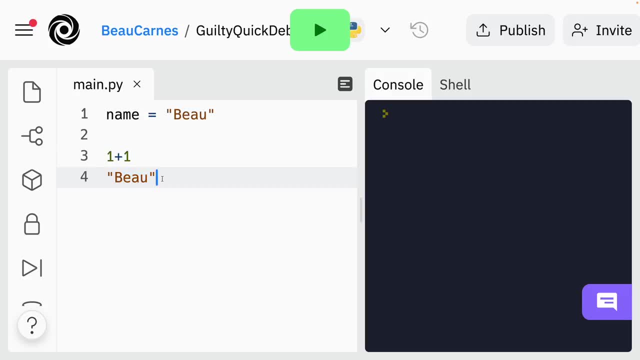 like this is going to return to this is going to return the string bow. So a statement, on the other hand, is an operation on a value. So, for example, these are: this is a statement here, because we have an operation where a sign. 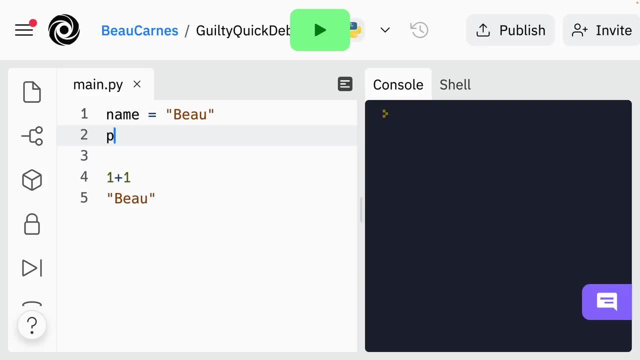 this to the variable, And then another statement would be like this: print name. So that's going to be a statement, because it's doing something to the value. Now, a program is formed by a series of statements And each statement is put on its own line, like we have these two lines here. But 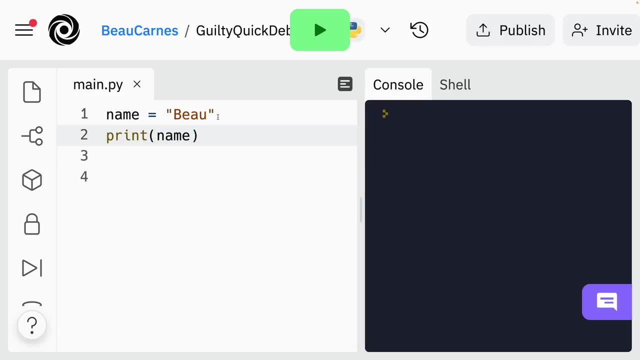 you can use a semi colon to have more than one statement on a single line. So I could put a semi colon here And then if I run the program it's still going to print the name, And let's just do that. We already learned how to run a program in replica, which is just a click. this: 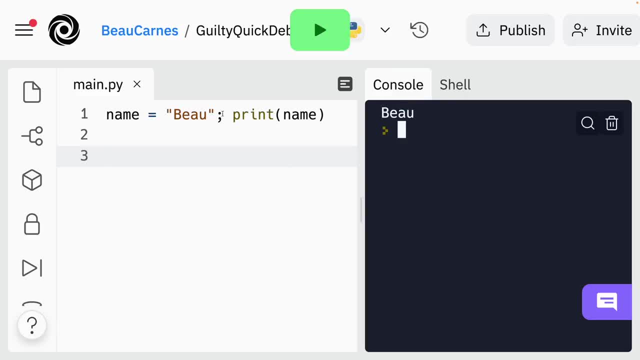 button right here. But we can see it's going to print bow And if I put these on two different lines it's going to do the same thing. If I run the program, it's going to still do the same thing here. Now let's talk about comments. This is something we haven't talked about in this course. 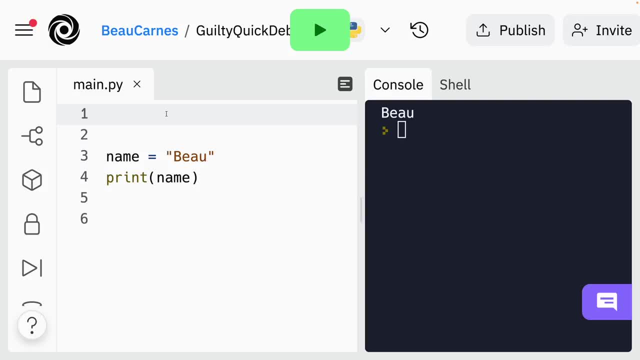 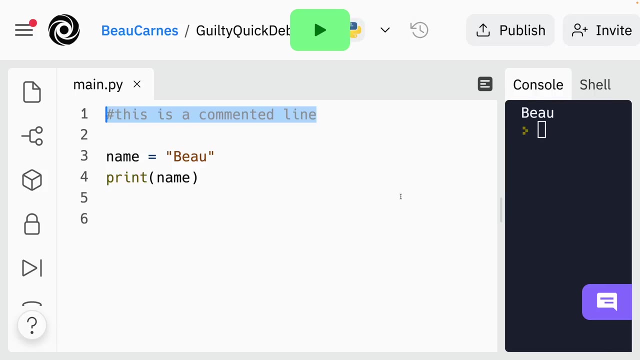 yet. So in the Python program everything after a hash mark is ignored. So let's talk about the comments. So if I put a hash mark, I can say this is a commented line, And when we run the program this line is going to be completely ignored. And then we can also put in inline comment. If I just 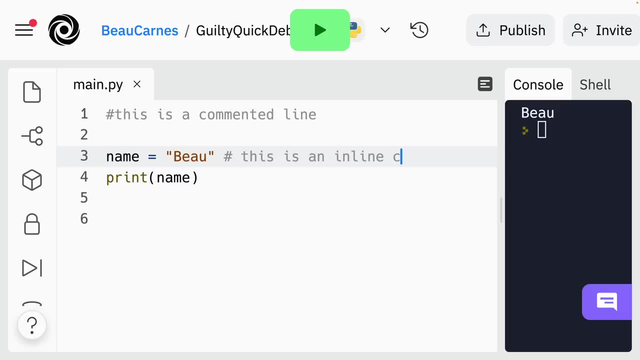 put the hash mark here. this is an inline comment, And the cool thing about most code editors, including replete, is it's going to put comments. it's going to make them gray. So you know that this isn't really part of the program. This is just some sort of 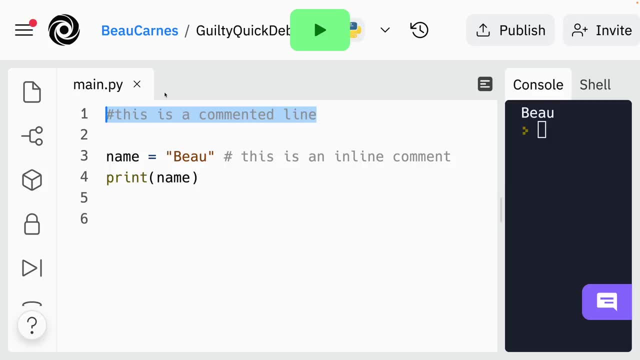 special note that the programmer wants to put as part of the program. So I want to emphasize again how important indentation is, So it's very meaningful in Python So you can't randomly indent things like you can't just press tab here to indent here and how this is kind of lined up. 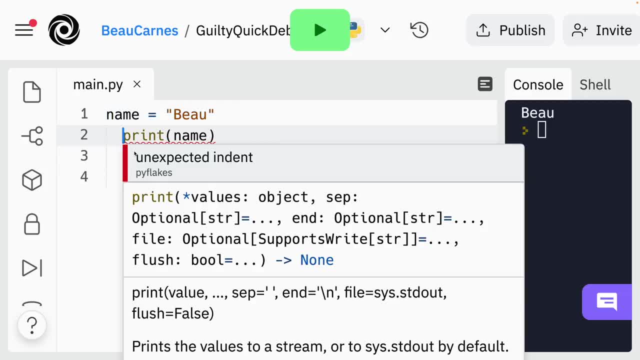 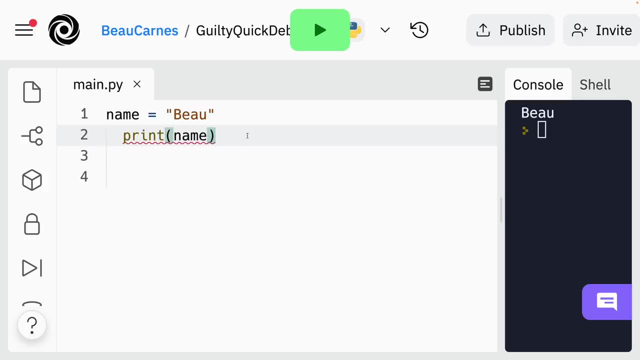 here. this line up here you can see this red squiggly line says unexpected expected indent. So some other languages do not have meaningful whitespace and indentation doesn't matter. But in Python indentation matters. So in this case we try to run this. 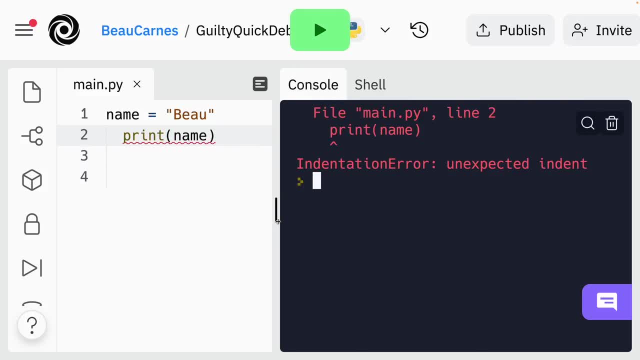 program. we can run this and you'll see an error right here showing up in red. here It says indentation error, unexpected indent, because indentation has a special meaning, So I can just unindent that here. Everything indented belongs to a block like a control statement or a. 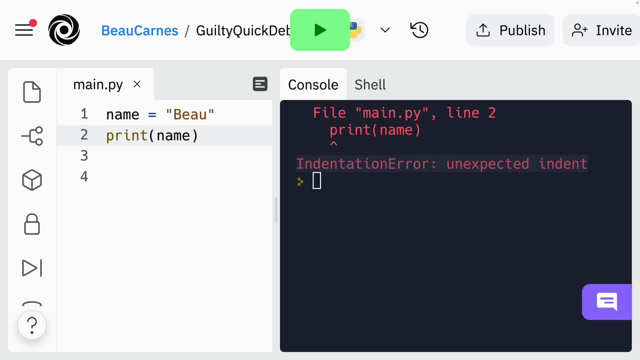 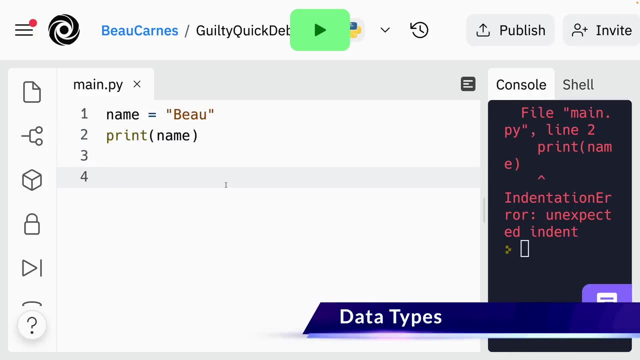 conditional block or a function or a class body, And that's what we're going to do here. So we're going to take a little bit of our code here And we'll be talking more about those different blocks later. Now let's talk about data types. Python has several built in types, So for 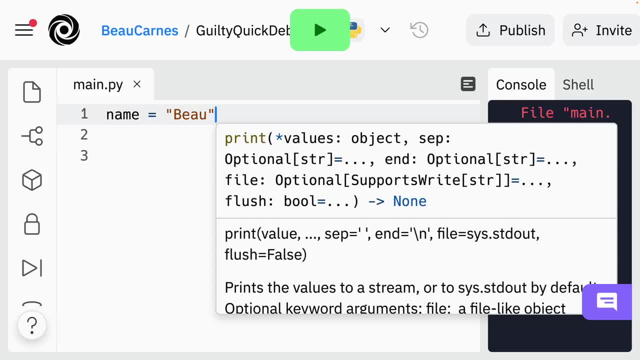 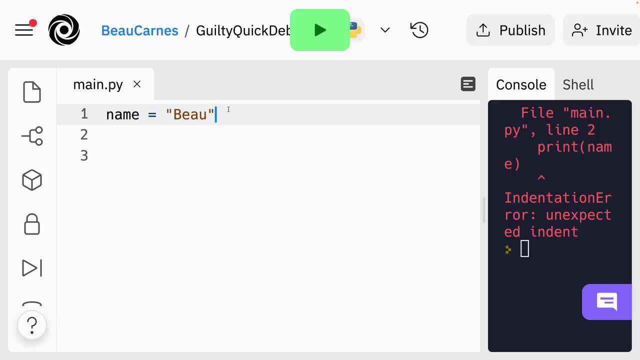 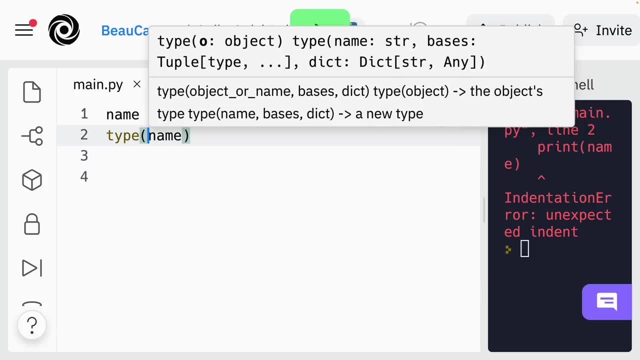 instance, this is a string, So anything surrounded by quotation marks is a string. that's one data type And you can check the type of a variable by using the type function. So I could say type and then I'll put name And to make sure to be able to. 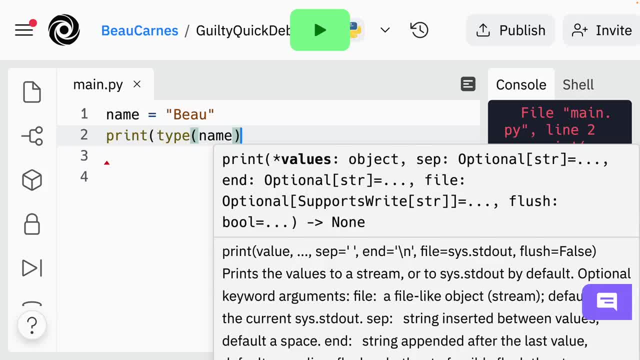 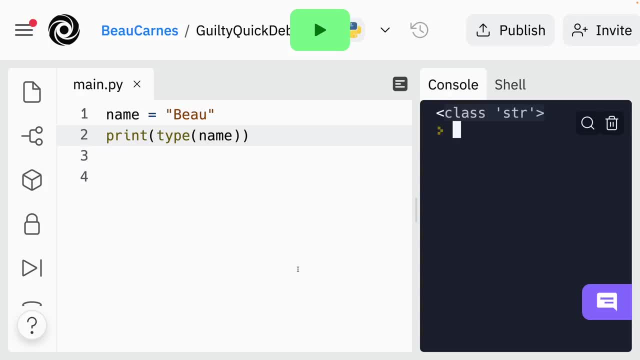 see in the console. I'm going to print what the type is here And if I press, if I run the program, we'll see that the type is the class of str, which stands for string, And then we can test to see if. 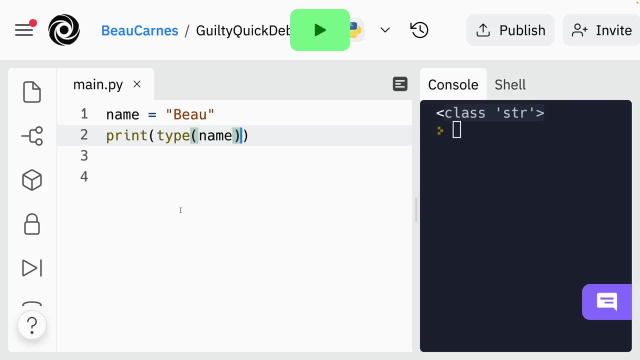 something is a string by comparing it to str. So I could do equals equals str And then if I run that it's going to say true, because the type of name does equal a string, And then we can also use is instance. So I'm going to, So if we, instead of doing type, we do is instance, and then we have 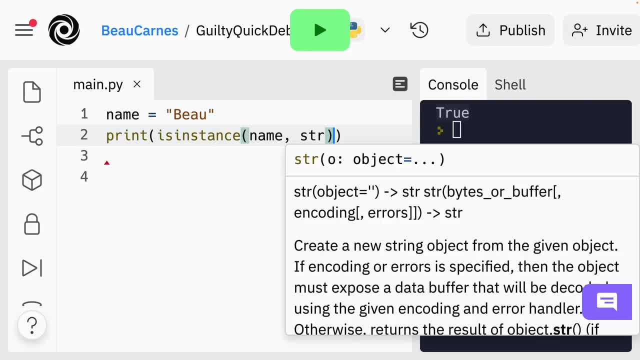 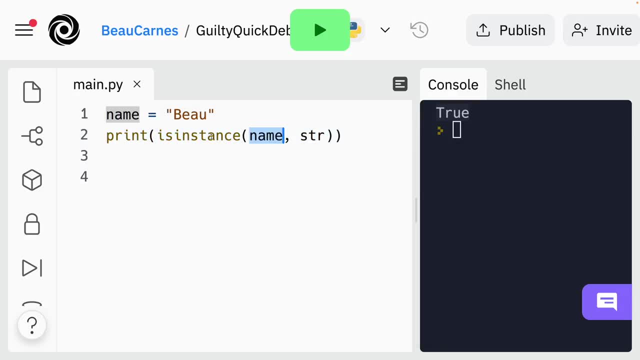 to pass it to things. So the first thing we're going to pass it, so we have is instance. we're passing up the name, that's this variable And str. we're trying to see if name is an instance of a string And if I run that it should say true. 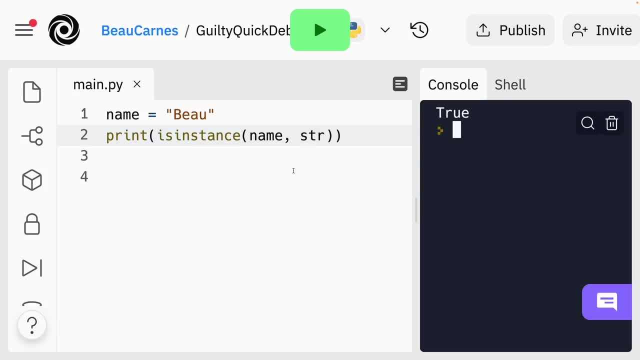 again. So we've been testing against the str class, the string class, but it works the same for other data types. So there are some data types around numbers, So an integer number, integer numbers are represented using the int class or the int class And floating port point numbers or fractions are a. 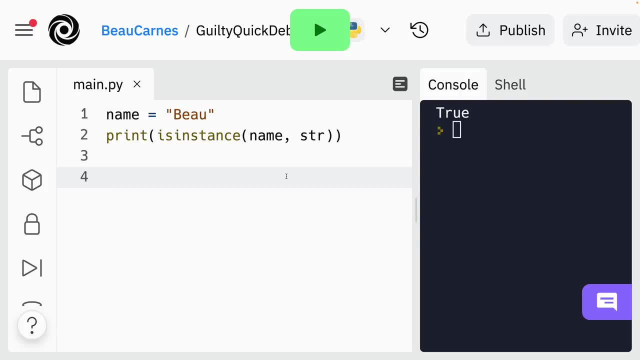 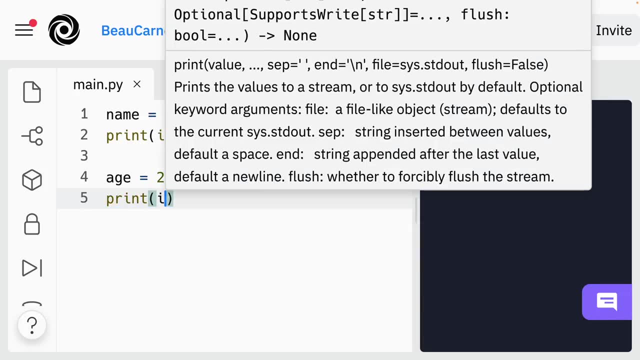 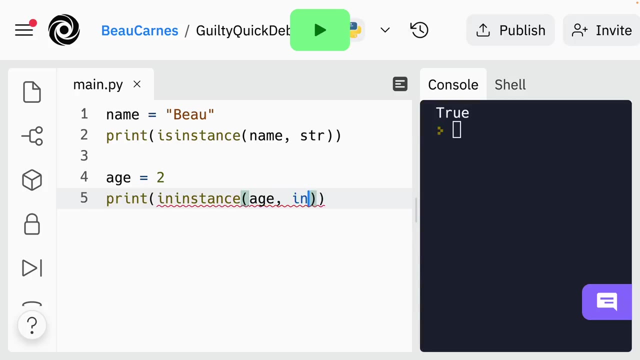 type of are the type of float. So I can say age equals two And then we can just check is instance And I can pass in the age and then I can pass in an int. So if I run that we're going to see that I've done something. 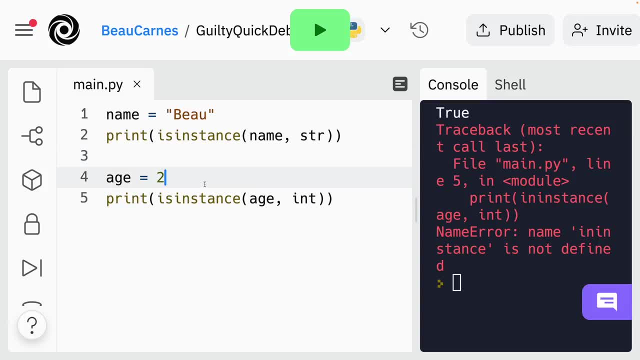 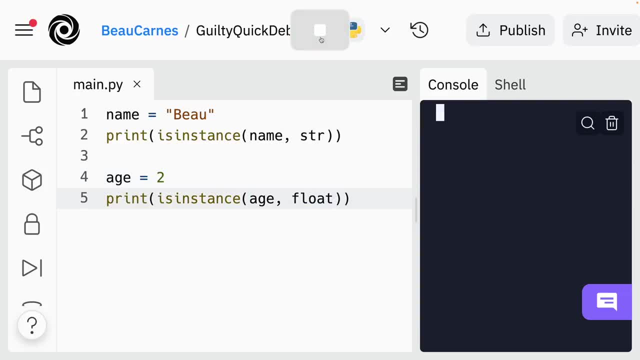 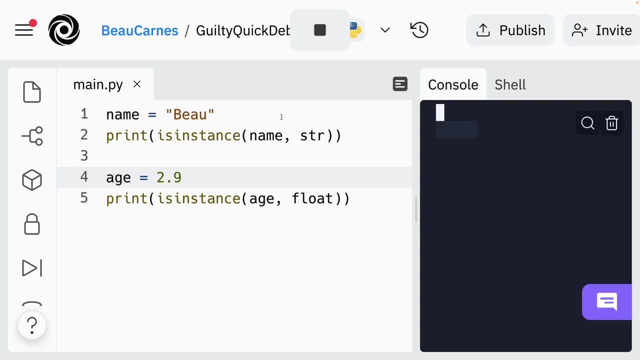 if I did 2.9, then it should show that it is a float because it has a decimal. So Python automatically detects the type from the value type. So it automatically knows this is a string. it automatically knows this is a float. But you can also create a variable of a specific 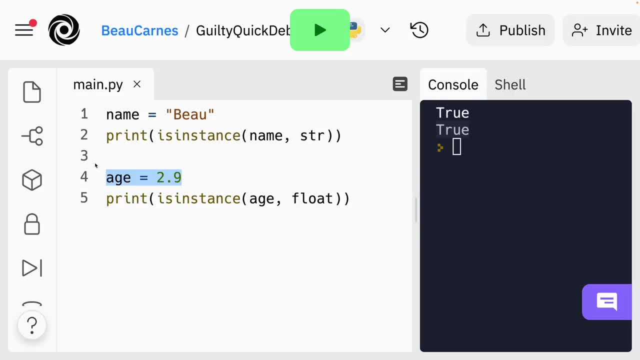 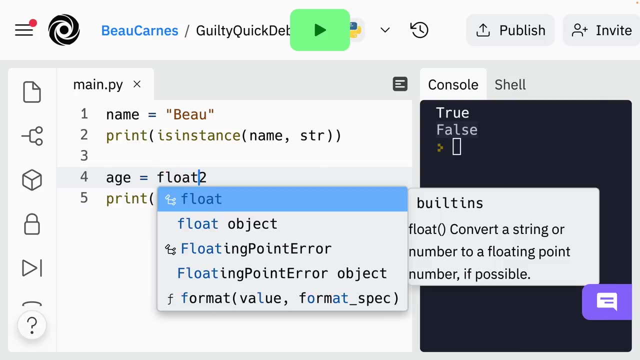 type by using the class constructor, passing a value literal or a variable name, Like, for instance: we have this and we check to see if this is a float and it's saying false. but I can make it a float by typing and float and just putting the value into the float here. So we're going to 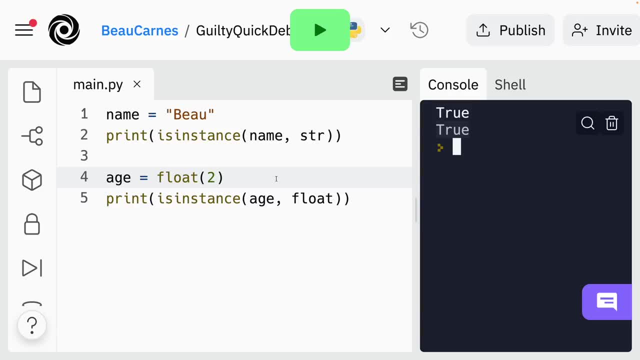 make it a float. So now it's true. true, And you can do the same thing with strings or integers or other data. And you can do the same thing with strings or integers or other data, And you can also convert from one data type to another by using the class constructor. So that's basically. 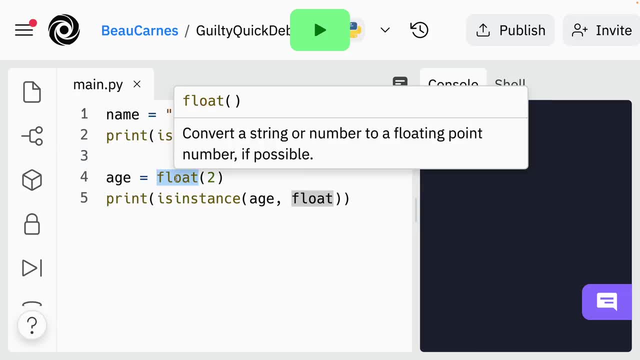 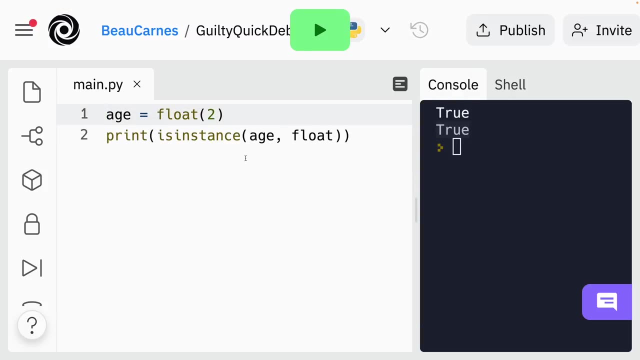 what we did. we just converted this from an integer to a float. But I can also do something else. I can convert something from a string to an integer. So, for instance, I'm going to: we'll just get rid of this one completely here And we'll just use this one. So a string is anything in. 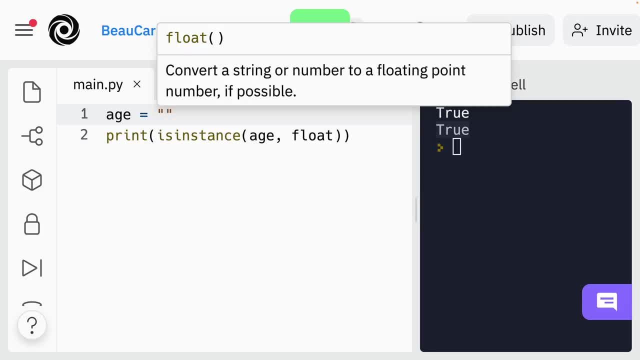 quotation marks. So if I do, I'm going to do a string. I'm going to do a string. I'm going to do a string is anything in quotation marks. So if I do 20,, age 20,, and I test if this is a, an int. 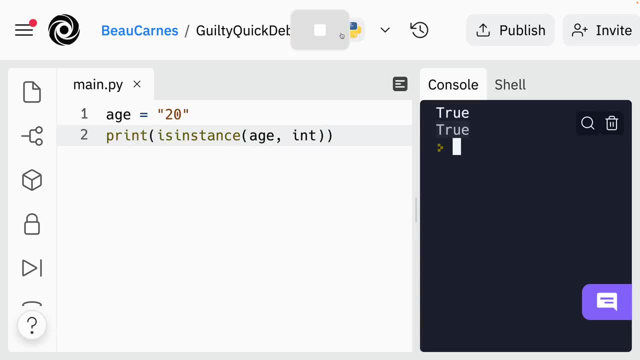 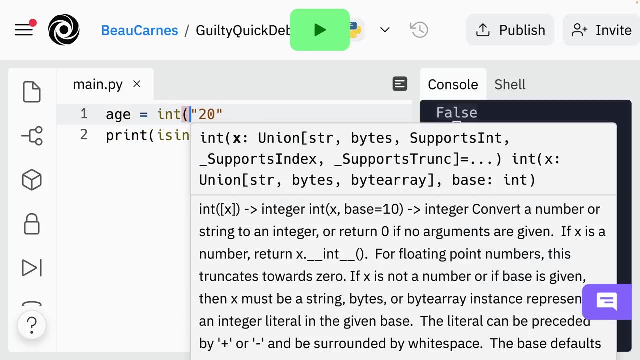 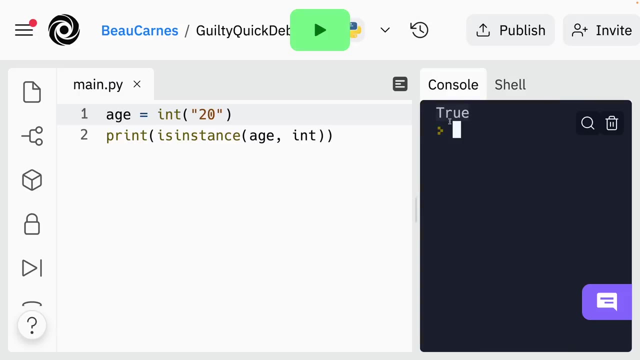 it's going to say false. it's not n, so I'm printing whether it's an instance of an int. but I can convert this string into an integer by just doing integer And this will run the program And it says true. Another thing about this is you don't just have to pass in the actual 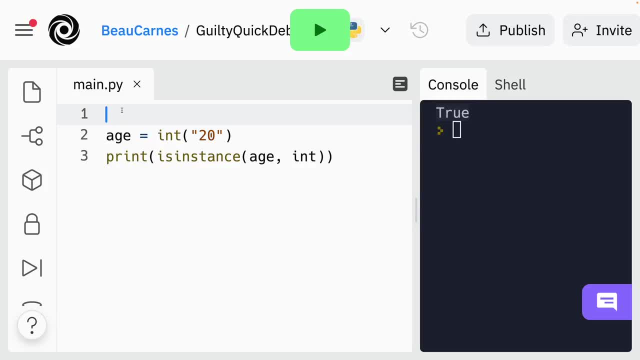 data or the actual string. I can pass in a variable, So I can say number equals. and now I'm going to make it an X. it says number but it's actually a string. but I can pass in the number here And then it's going to set that age And it's going to be true. So we create the string. 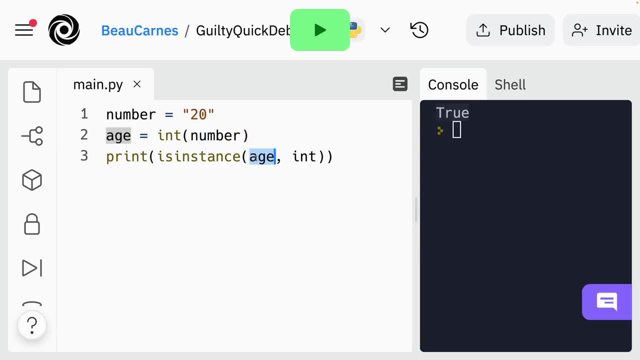 we convert the string to an integer And we tested that that age is an integer. So when we do something like this, this is called casting. we are, it's, basically trying to extract an integer from this string. Of course, the conversion might not always work, depending on the value that's. 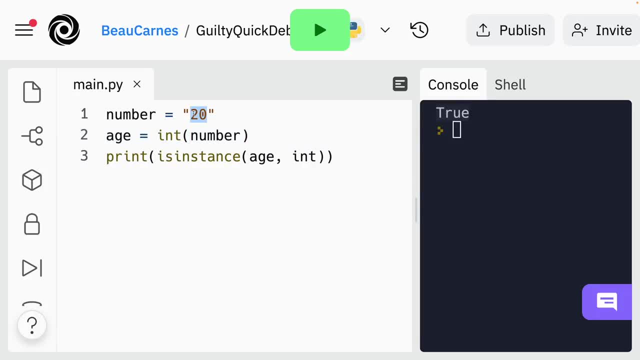 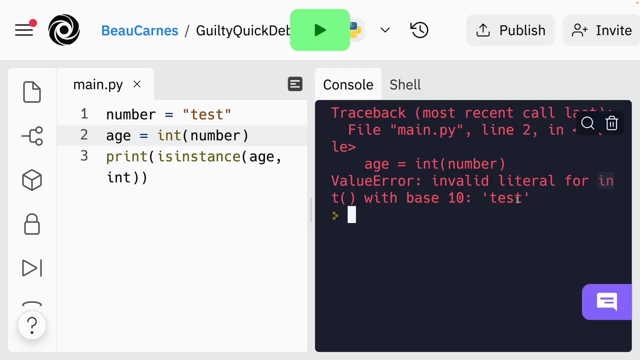 passed. So for instance, if we write test here in the string instead of the 20, we make an error. So let me just run this and see. now we have an error. says invalid literal for for int. I am t with base 10 tests. so we can't convert the word, we can't convert the string test to an. 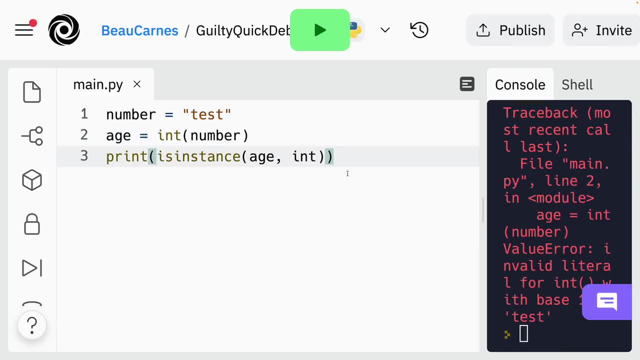 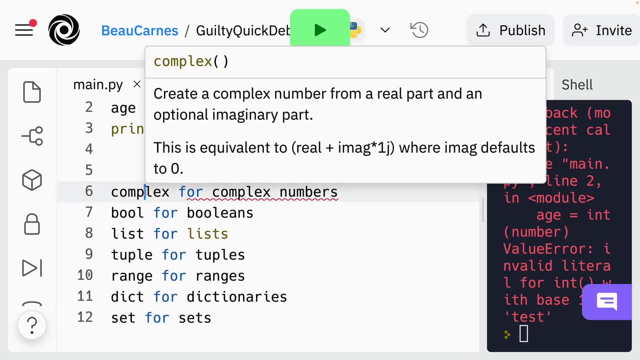 integer. So Python does its best to do the conversion, but it doesn't always work. There are a few other types So he only see here are some other common types of types. So there's the type of complex or complex numbers: bool for Boolean, list for lists, tuple for tuples. 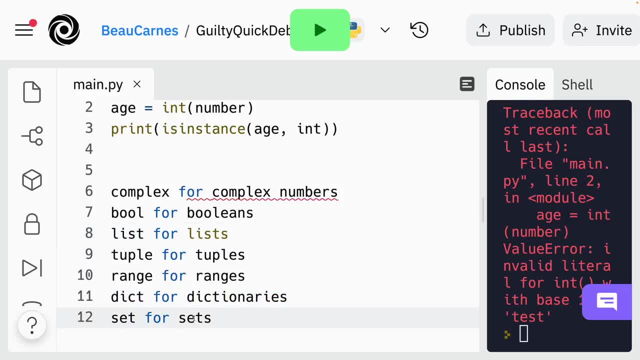 range for ranges, dict is our dictionaries, and set as a type for sets, And we'll explore all of these soon. what we'll go into more detail about, about all these different types of types- Well, now let's talk about operators. we've already seen one operator. that's this one. That's the. 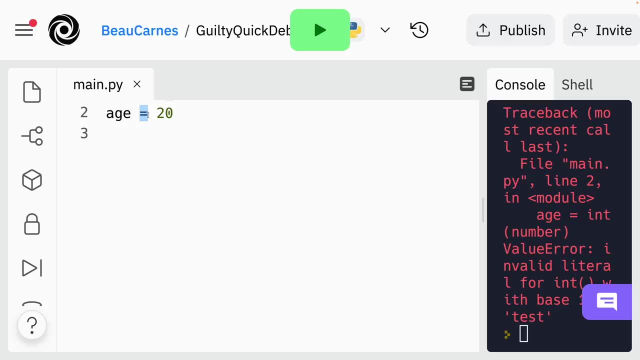 assignment operator, But there's also arithmetic operators, comparison operators, logical operators, bitwise operators and plus some interesting ones like Is and in, So we're going to be going over a lot of those right now. So we talked about the assignment operator, which is used to assign. 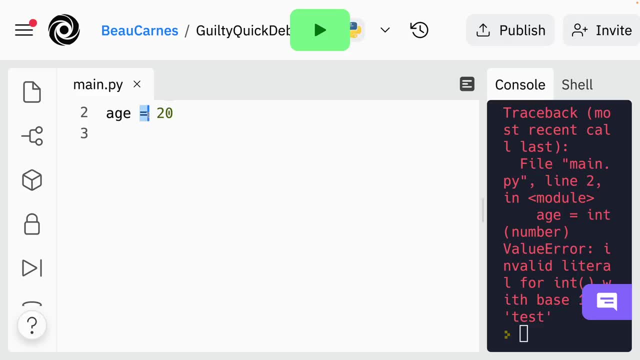 a value to a variable or to a variable. And then we're going to talk about the assignment operator: assign a variable value to another variable. Now let's talk about arithmetic operators. It's just what you use to do math, mathematics. So here are the different arithmetic operators. So we have. 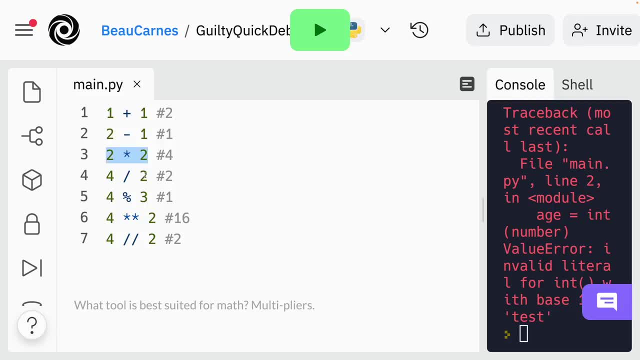 plus one plus one equals two. then minus multiplication division, we have remainder. so four divided by three equals one, but there's a remainder of one. we have x. one is four to the power of two is 16.. And floor division. So floor division does a division problem, and then just. 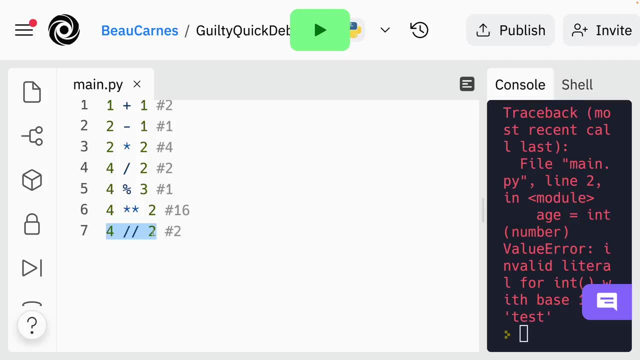 basically rounds down. So floor division does the division and rounds down to the nearest whole number. So actually this would be better seen if we do four, five divided by 25, floor division divided by two is going to be two, normally be 2.5. But floor division is rounding down to the nearest. 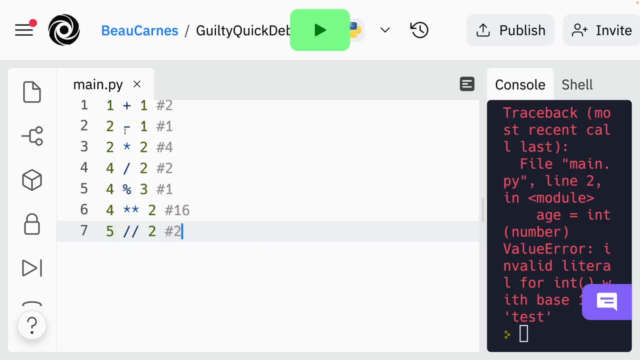 integer the nearest whole number And then also note that that the minus can also be a make something, a negative number. So I could do four plus negative, or I mean one plus negative one, and then that's just going to equal zero. And then the plus operator can also be used to concatenate string values. That's something we 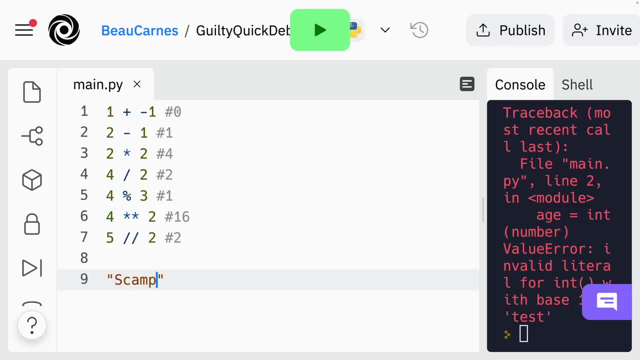 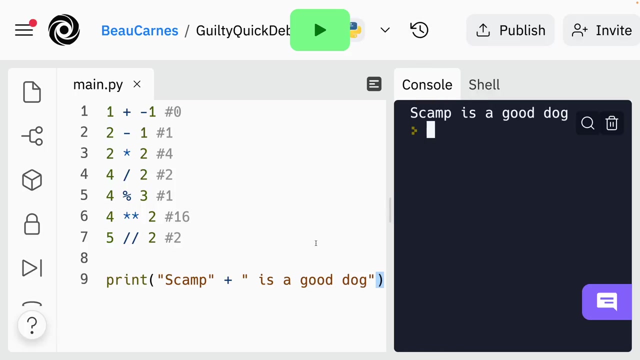 talked about earlier. But I could say scamp and then put a plus is a good dog And then like, if I print this out, I put the the parentheses around it, I can, and then we'll see the whole string here. skip, scamp is a good dog, That was the name of my 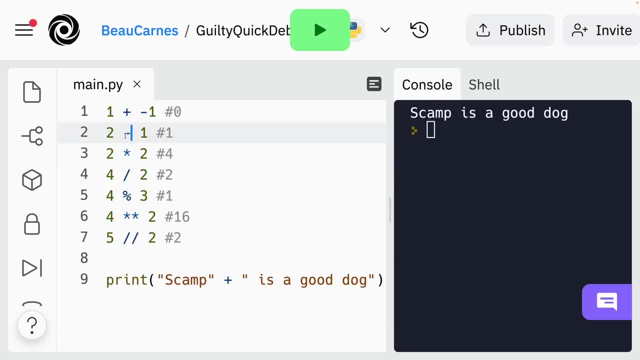 first dog when I was a kid. So we can also combine these arithmetic operators with the assignment operator. Well, let me show you what I mean. So let me just get rid of this Here And I'm gonna do age equals eight and age plus equals eight, And they'll do print age. So 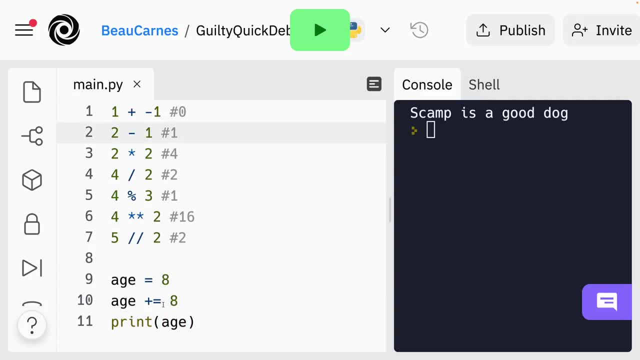 we've. so all these different operators can be assigned with, can be combined with the assignment operator, And now it's going to add eight to the age. So if I run this it's 16.. So this actually just means age equals age plus eight. So this age plus equals eight is the same. 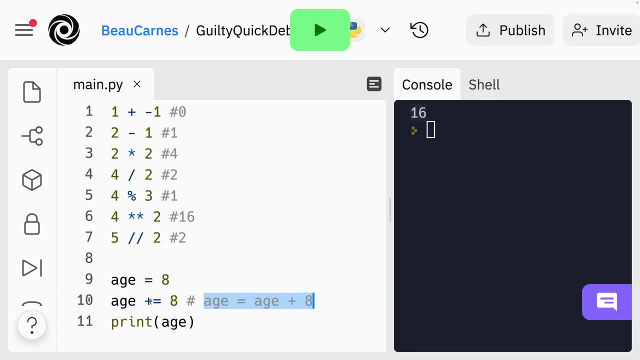 as saying age equals age plus eight. So it's just going to add this number to the current age and set it equal to the age, And you can do that with any of these, Like I could do times, And that would be: age equals age, times eight and 64, and so on with any of these. 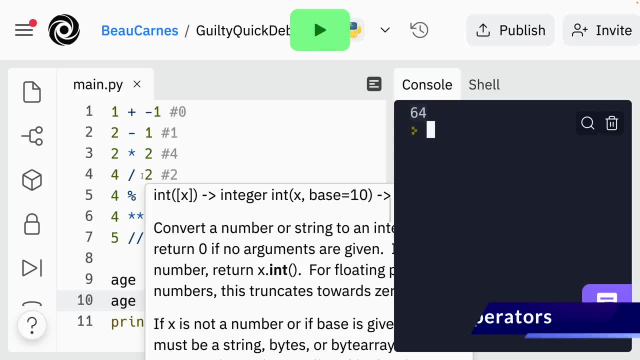 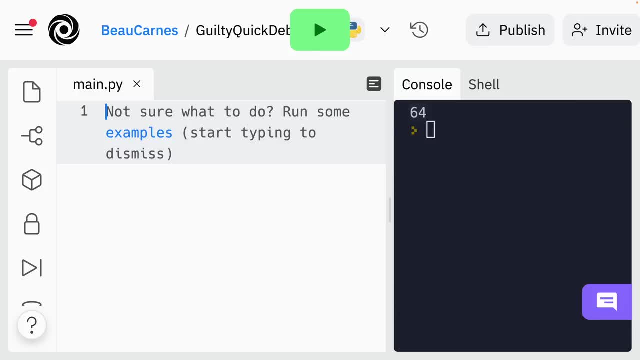 arithmetic operators. Okay, now let's talk about comparison operators. Now we talked a little bit about them before, But let's see some examples again. So this is to compare. if two things are equal And then we have not equal, we're comparing them to see if they're not equal or count. this is: 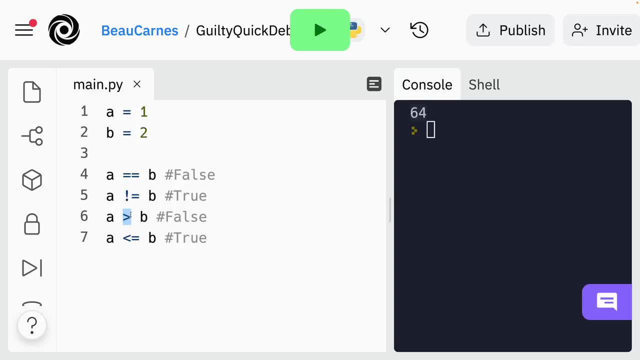 if a is greater than B or more than B, And then there's: this is less than or equal to B. Now let me just tell you a trick of how I keep that, keep track of which one is greater than and which one is less than. if you see this, less than one, if you kind of tilt your head a little bit, 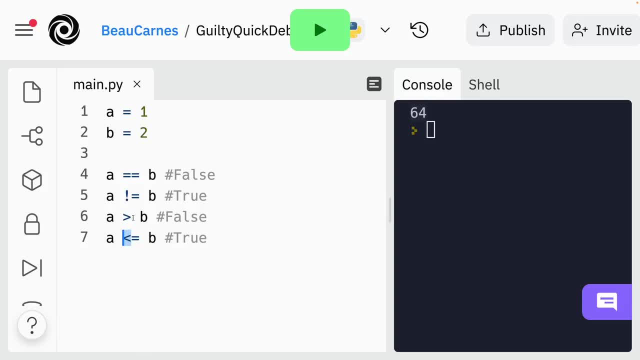 it kind of looks like an L, see like L, and this one doesn't look like as much of an L. So this less than operator kind of in some ways looks like a capital L that's kind of just squished. 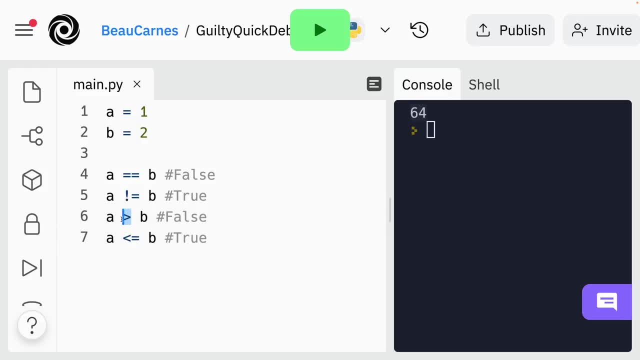 over, And that's how I keep track of which one is less than, which one is greater than, And so these are all going to give either a false value or a true values. Speaking of true and false, True and false are examples of Boolean, the Boolean data type, the Boolean data type just means true. 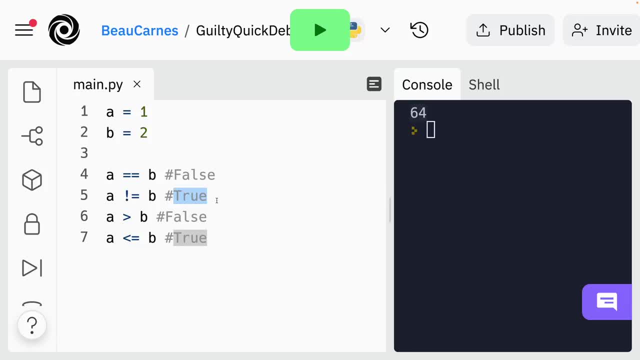 false or true. So a Boolean is either true or false. And if you're using Boolean data type, so a Boolean is either going to be true or false. there's only two options And there are a few Boolean operators. So let me show you what the Boolean, the Boolean operators, are: either not. 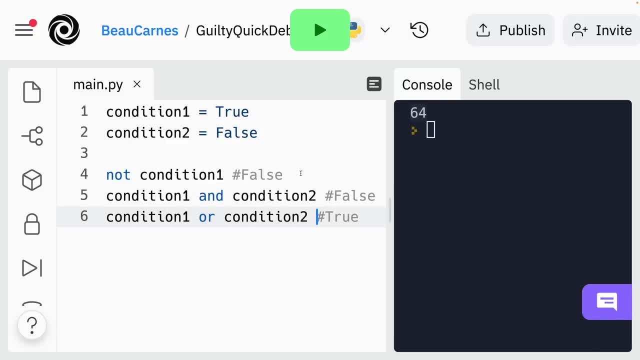 and or or So. when working with true or false attributes, those work like logical and or and not. So when you're using not, it means it's not true. you're checking, you're checking, you're checking to see something is not true and means they both have to be true And or means. 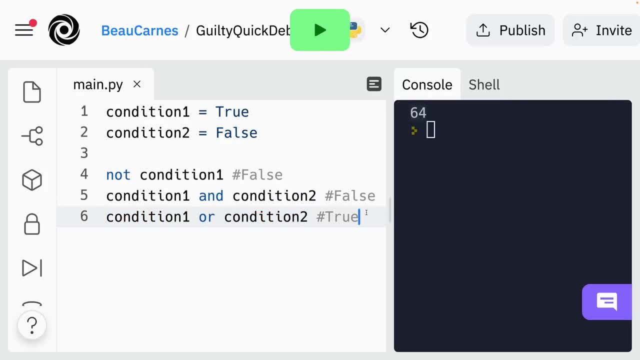 either this one has to be true, or this one has to be true in order for the full thing to be evaluated as true. And let me show you something about. or now, or using an expression: returns the value of the first operate operand. that is not a false value or a falsie value. Otherwise, 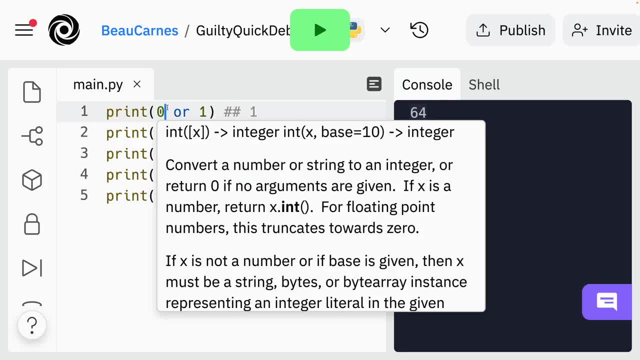 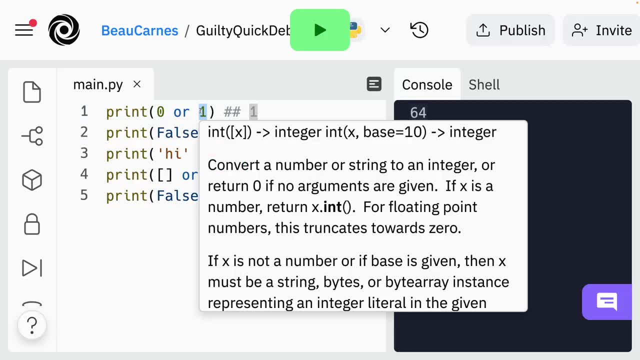 it returns the last operand. So it's going to return the first operand. that is not a falsie value, But since this is a false value, it's returning the second operand. Since this is a false value, returns the second one, since this is. 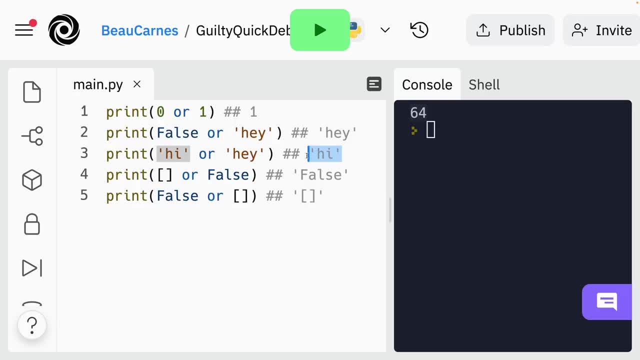 not a false value. it can return the first one, And this is considered a falsie value. if it's just an empty brackets, that's false. So it's going to return the second value, which just happens to be false, And since this is a false value, it's going to return the second option. 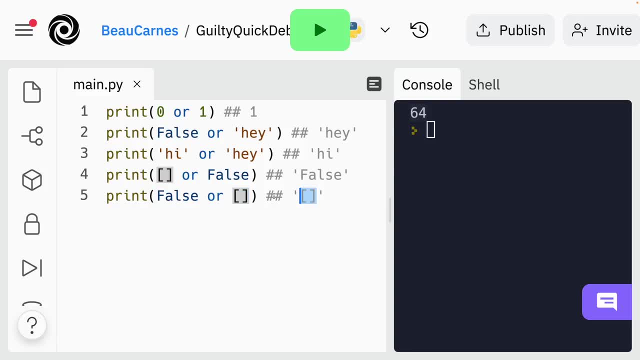 Which also happens to equal to false. So one way to think about it for the word or is so the pipe. this is how the Python docs describe it. If x is false, then y else x, So this would be like x. 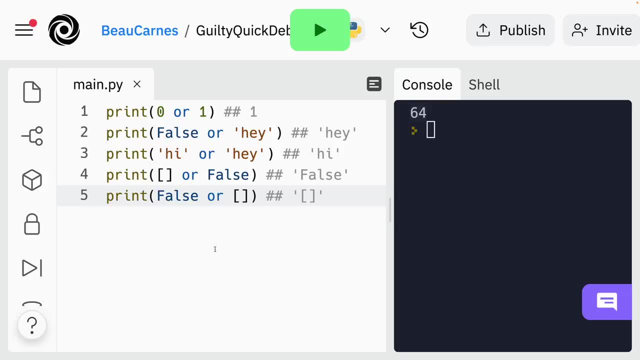 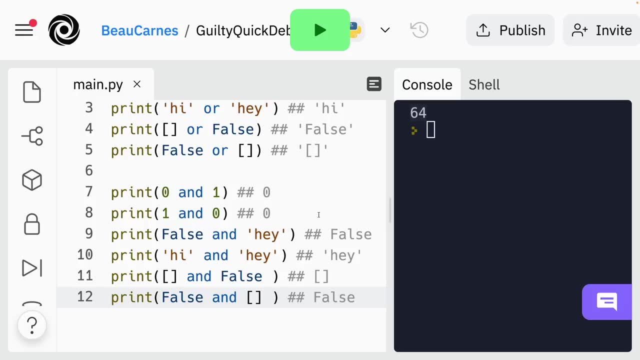 this would be y. if else is false, then y else x. And then for an down here. let's look at some examples for: and: and only evaluates the second argument if the first one is true. So if the first argument is falsy, such as false, zero and empty string, empty. 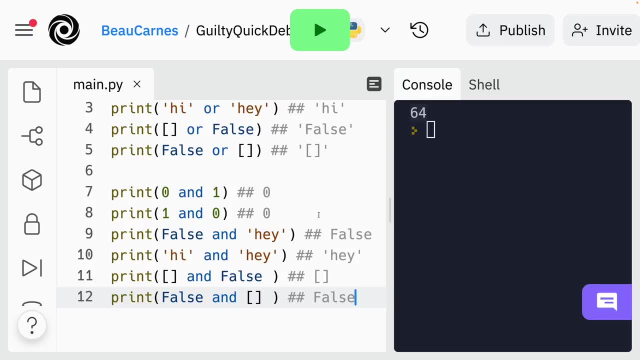 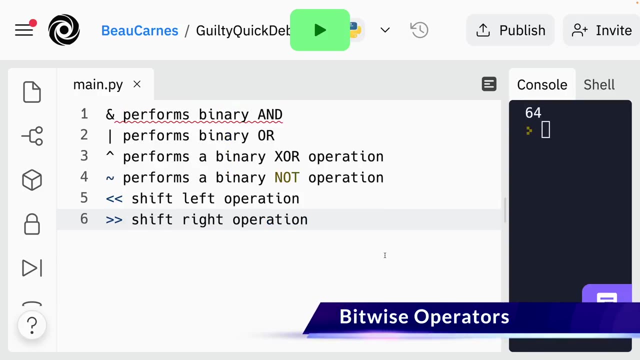 brackets, it returns that argument, Otherwise it evaluates the second argument. So the way- that way the Python docs describe it- is: if x is false, than x, else y. Okay, let's quickly discuss bitwise operators. They're very rarely used, only in very specific situations, But it's worth knowing what. 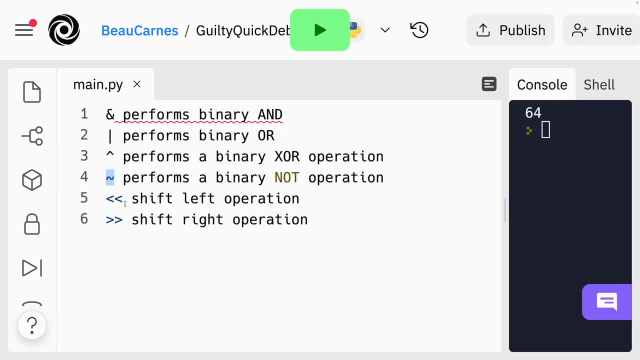 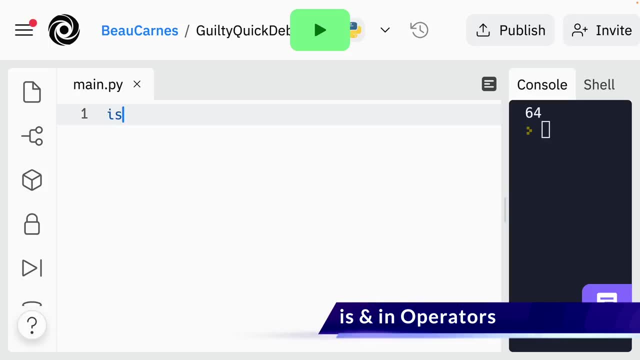 these bitwise operators are just in case you're in the very rare situation that you need to use them. And then two other types of operators are, is, and in now is is called the identity operator. It's used to compare two objects and returns true if both are the same objects. 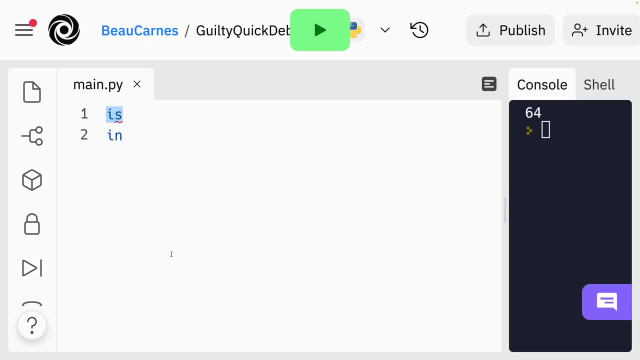 both are the same object And I'll be talking more about that later in the section on objects. And then n is called the membership operator. This is used to tell if a value is contained in a list or another sequence, And we'll be talking more about the in operator when we're discussing lists. and 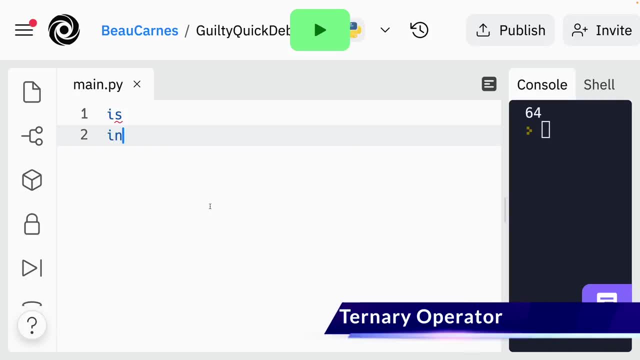 other sequences later in this course. And the final thing I want to talk to you about is the ternary operator. Now, the ternary operator in Python allows you to quickly define a conditional, So he will be like kind of the slow way to do it without a ternary operator. So let's say you have 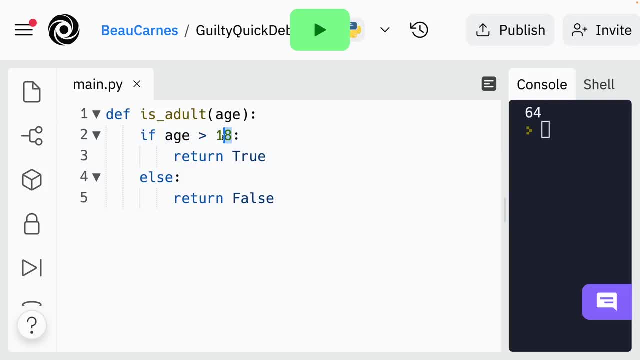 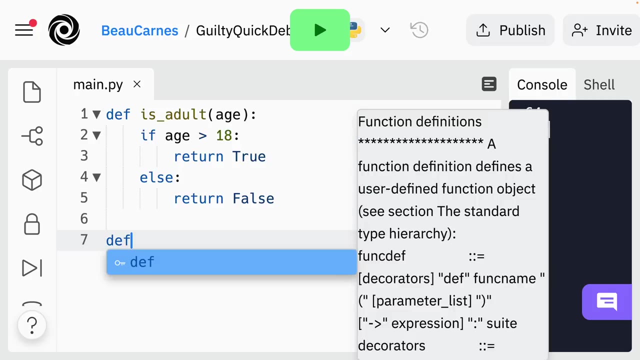 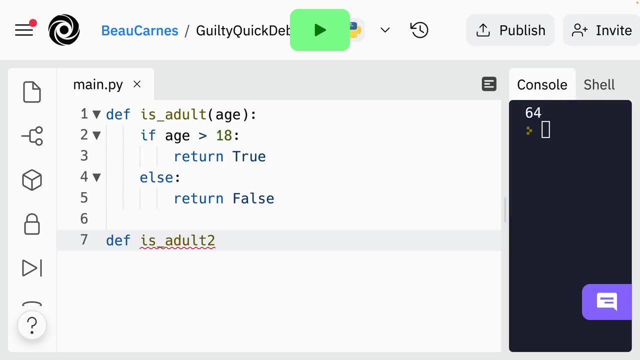 a function that in this function is comparing age with 18. And it's going to return true or false, depending on the result. So instead of writing like this, we can implement it with a ternary operator. So let's do: def is adult. I'll call it is adult two, because it's the second way of doing it, And this: 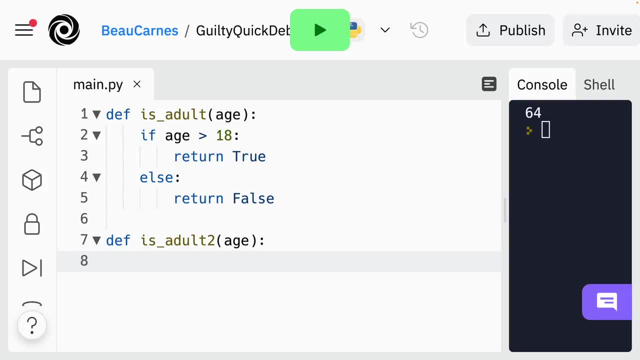 time we're going to use the ternary operator. it's just going to be return true if age is greater than 18.. Else, false. So you can see, first we define the result. if the condition is true, then we evaluate the. 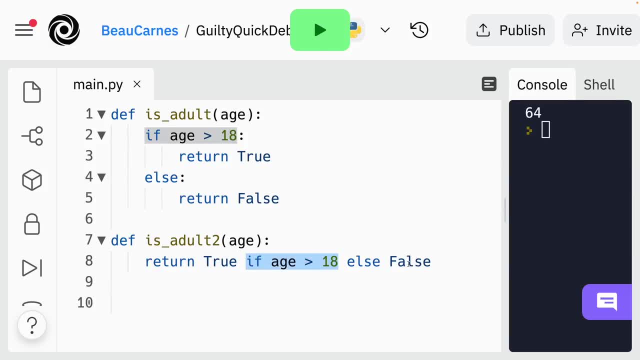 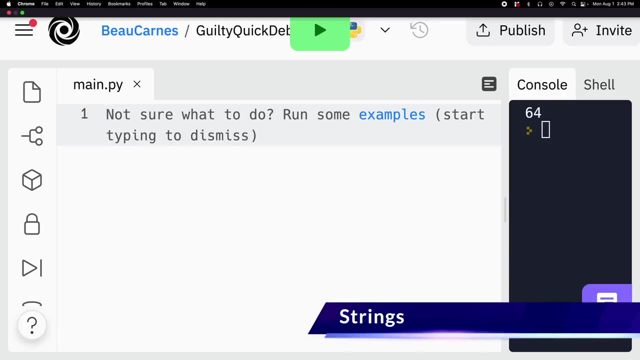 condition And then we define the result. if the condition is false, it's basically an if else statement, all on a single line. Okay, let's talk more about strings in Python. So a string of Python is a series of characters enclosed in quotes and double quotes, or it could be single quotes. 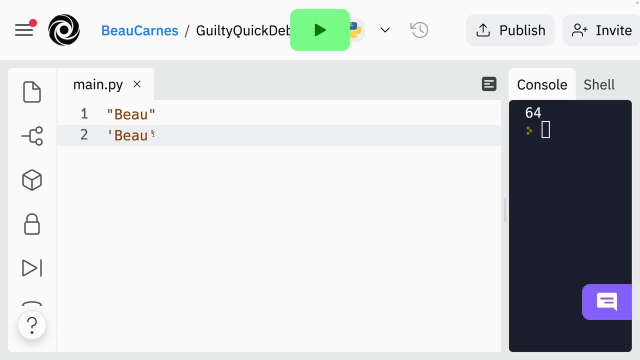 As long as the type of quote is the same on both sides. And we already talked about how you can assign a string to a variable, And we already talked about how you can concatenate two strings using the plus operator, like phrase equals bow, and then you can concatenate with the plus operator. 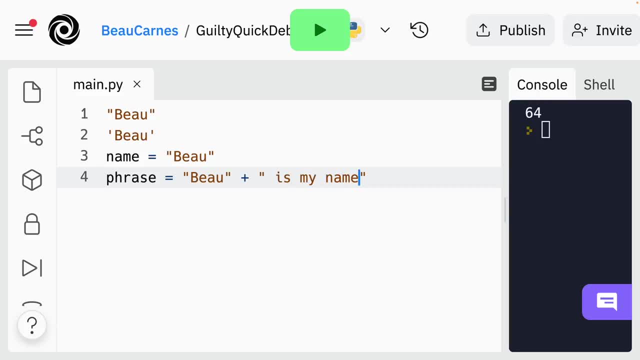 is my name, And then well, also, instead of putting a string here, you can put the variable. so I could put: name is my name and we already have the variable here to equal bow. So when you concatenate, you can concatenate the strings or the variables. you can also append to a string using the plus. 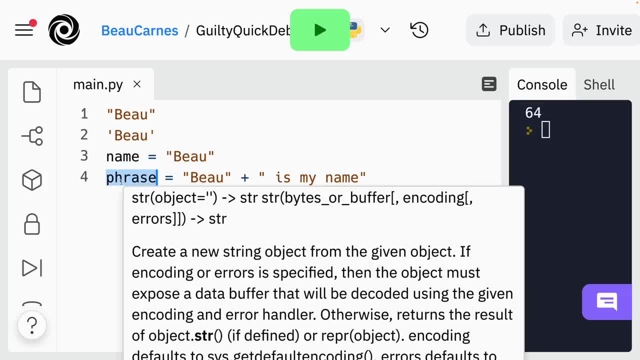 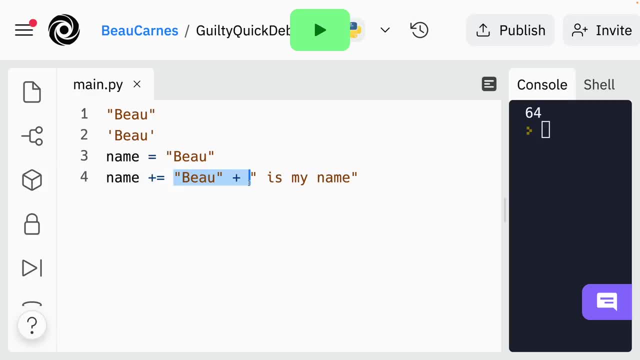 equal operator. So let's say I want to add to this name And so I'm going to say name plus equals. plus equals Is my name. So we're adding is my name to the end of this So I can say print name And then 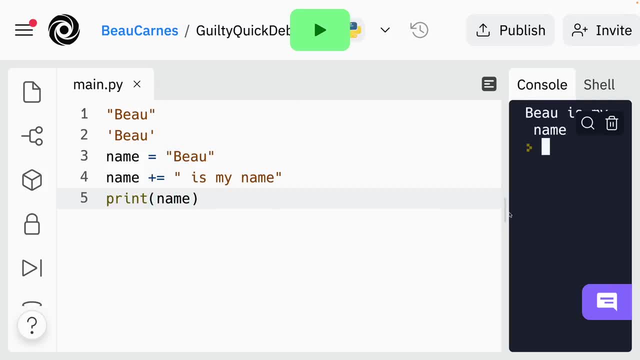 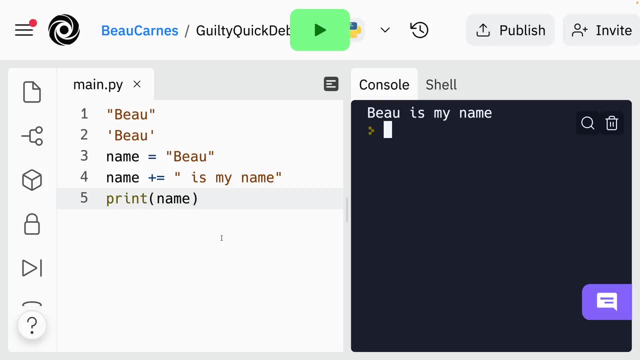 we can see what it looks like when you use the plus equal operator. So bow is my name. And then we already talked about how you can convert a number to a string using the STR class constructor, like if we have age, age, age. 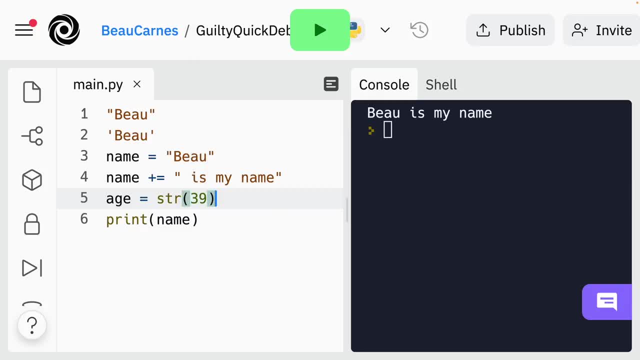 age we could make this a string. But we pass this integer, it converts to a string, and now it's going to be a string. Now here's something new: a string can be a multi. what can be multi line when defined with a special syntax? So if you enclose it, if you enclose the string in a set, 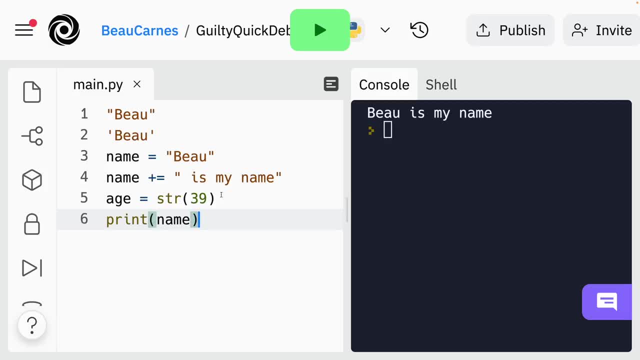 of three quotes. so let me show you an example. we'll get rid of all this And I'm going to print an entire string here. So we're going to make this a multi line string. I'm going to put three quotation marks And then it's going to start with three quotation marks and in with three. 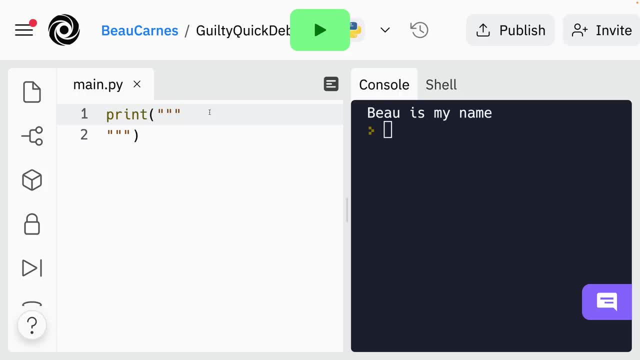 quotation marks and then I can make it multi line, So I can say bow is and then I can put some extra lines: 39 years old Now, if I print that and you can see it's going to print, print the different lines here. So we just made a multi line string And you can also, instead of using the, 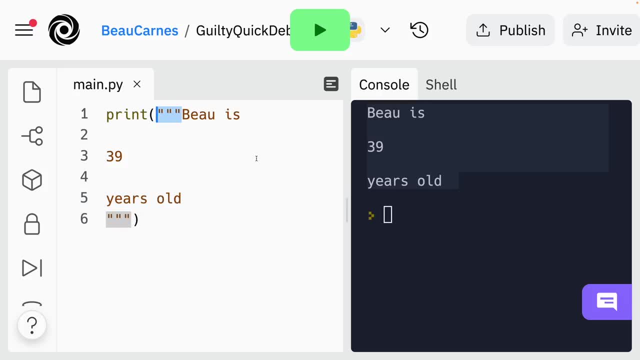 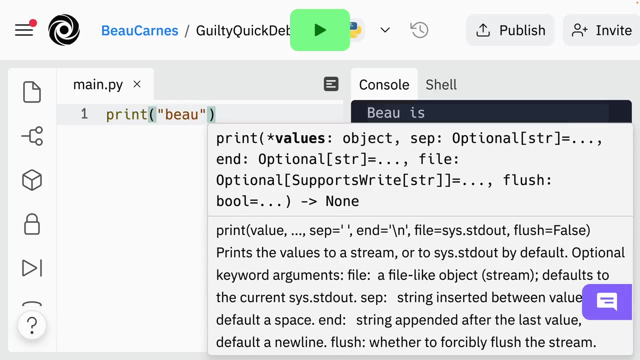 double quotes. you can put a single quote as long as they're the same at the at the beginning and ending. Now a string also has a set of built in methods. Let me show you an example. So if I have this string bow, but I'm going to put at the end of the string, I'm going to put dot upper. 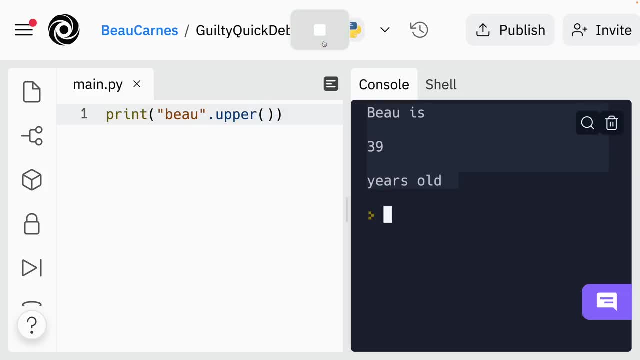 and I put parentheses at the end. So if I run this now, it's going to print it in all capital letters And the same thing you can use with lower. So if it, if I had a string that had a few capital letters, okay, now it's all lower Now. 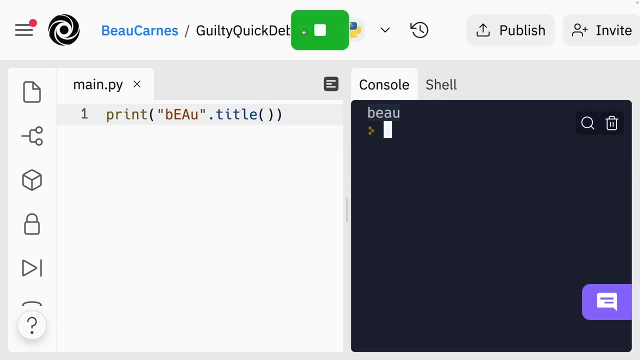 I can also type in a title And this is going to make each lot. so I can say bow person And I do this, So it's going to count, it's going to a title and then I'm going to put in a capital letter. 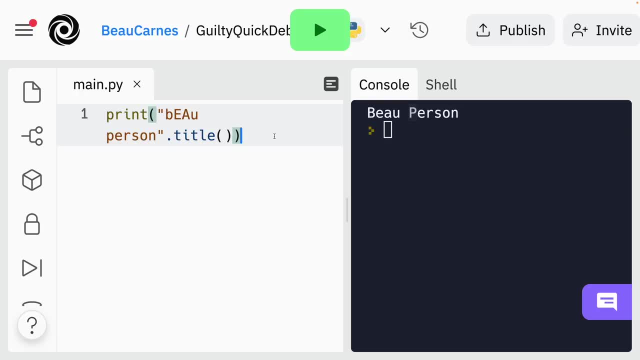 It's going to make the first letter of each string a capital letter. I can also check things like I can say is lower and it's going to check if it's all lowercase letters, false. But if I make it so it is all lowercase letters, it's going to say true. So here's just a list of a few common. 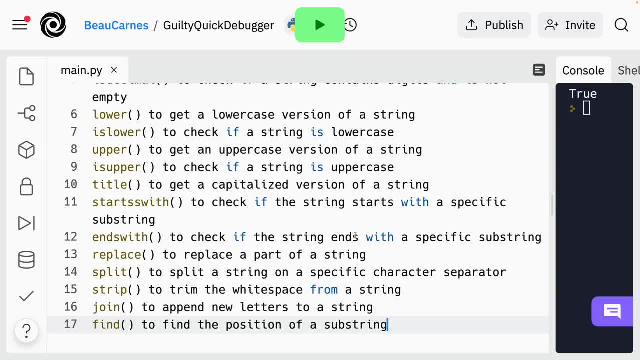 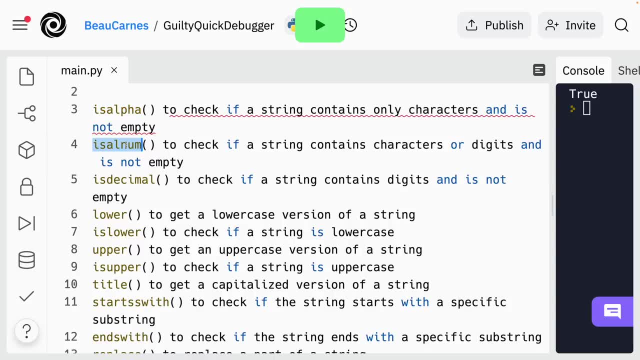 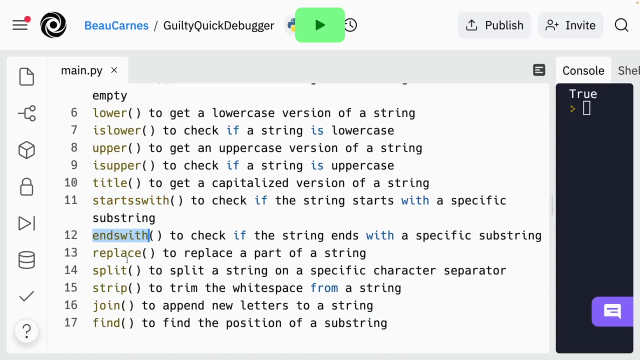 ones You can do is: a Is alpha to check if it contains only characters. Is l num to check if a string contains characters or digits And it's not empty. is decimal lower to make it lowercase. is lower upper is upper. title starts with the check. if it starts with a specific substring to check the int with, you can replace: 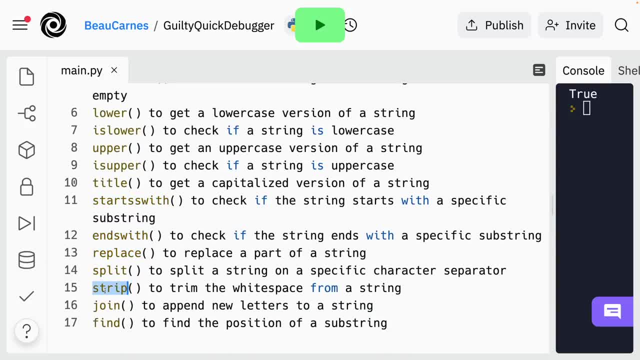 part of the string, split a string, you can strip the white space for a string, you can append New Letters to a string, you can find the position of a string, substring, spring string And there's a few more, But these are some of the most common things. you 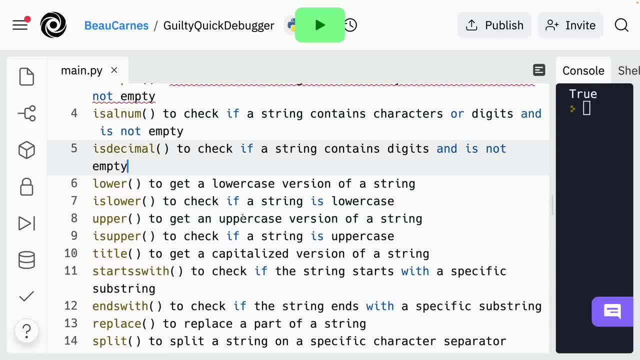 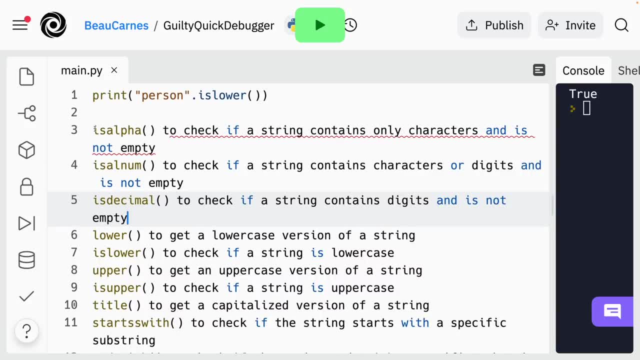 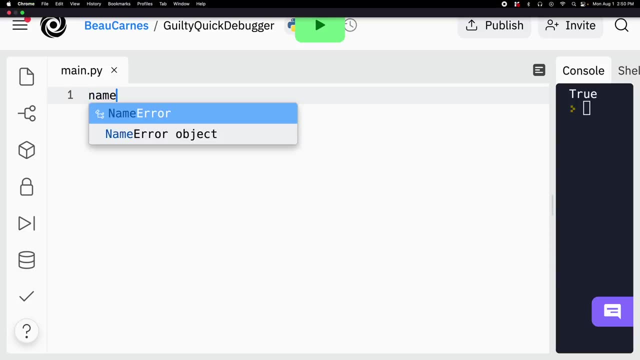 can do with a string. And then one thing to know about these is that they, they all return a new, modified string, that they don't actually alter the original string. So let me show you what I mean by that. So let's say, we have, we'll do, a name equals bow. again, let me zoom in a little bit And we're. 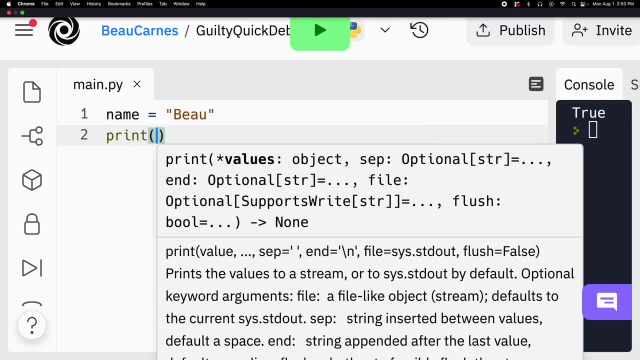 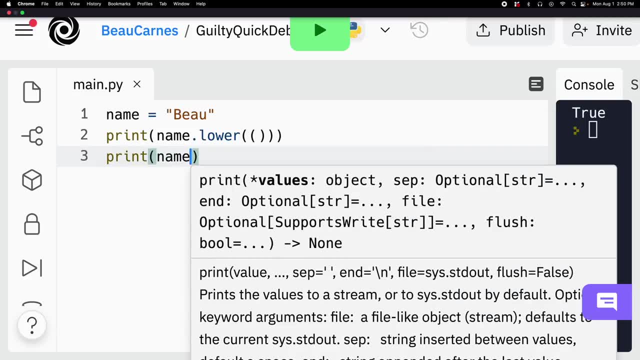 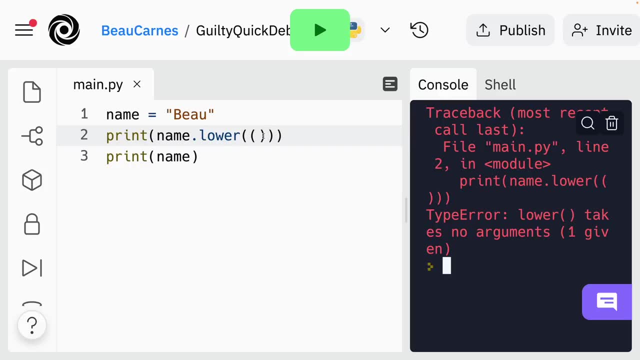 going to print name dot lower. Now I'm going to print name. So if I just run this and we first figure out what went wrong here, it looks like there's a few extra parentheses. Okay, let's run this And you can see that it's not going to change anything. So I'm going to print name dot lower. 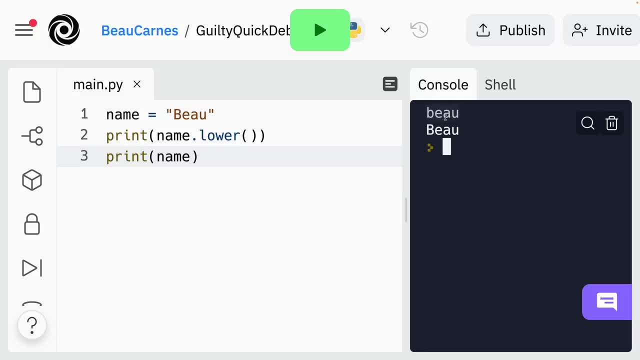 So if I just run this and we first figure out what went wrong here, it looks like there's a few extra parentheses. Okay, let's run this And you can see it's gonna make it all lowercase. But then when I print the name again, it's not still lowercase because this just returns a brand. 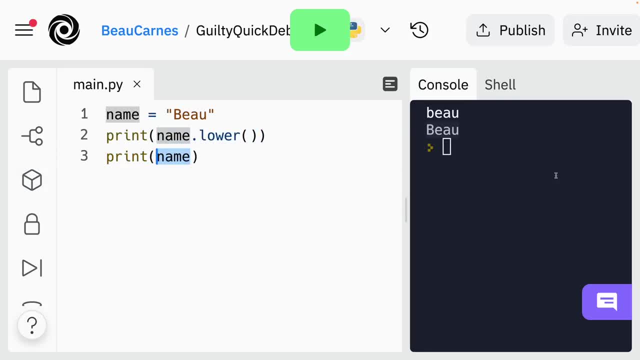 new modified string. it doesn't actually change anything in the original string, And then you can use some global functions with strings as well. So one function we haven't discussed yet is the le n function, which stands for a link. it can give the length of a string. 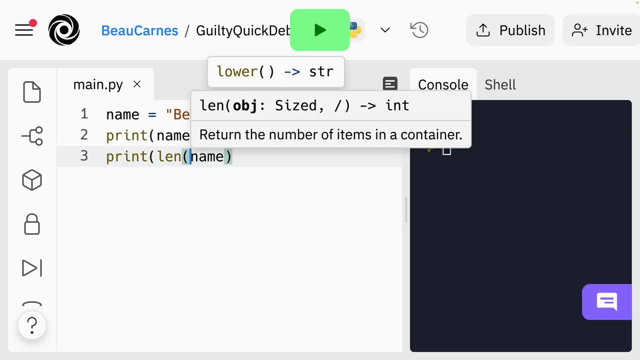 So I'm going to type an le n And then. so there's just some global functions that work with a lot of different types of data, And the length of this is four you can see, And then you can use the in operator. Now I briefly mentioned the in operator earlier, So let me show you one use. 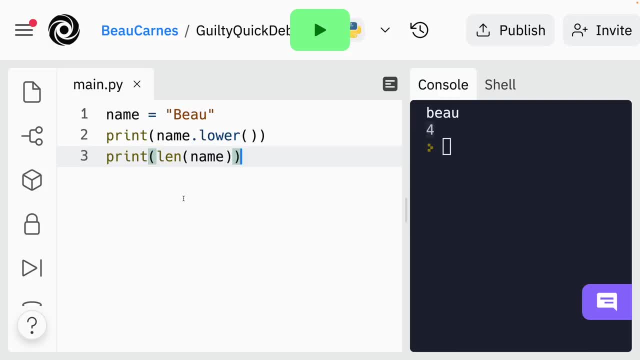 case. So we can use the in operator to check if a string contains a substring, Like, for instance, I can say a u in name. So let's check if name contains the letters a, u. Well, true, it does, But if it, if it does, if it, if it didn't, if I just add an extra string, it's going to say false. 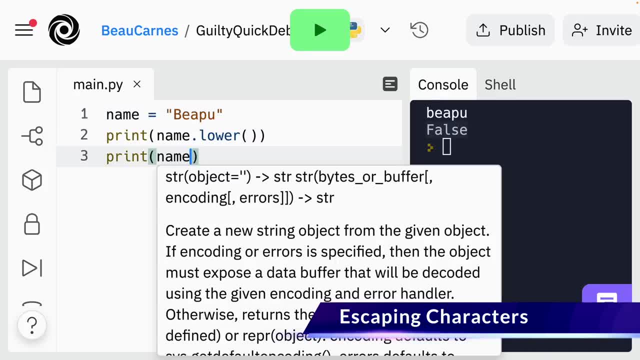 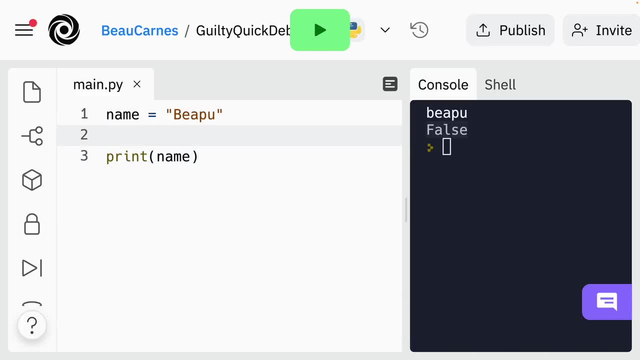 Okay. another thing with strings: Escaping is a way to add special characters into a string, For example, let's say we wanted to add a double quote within the string. how can I get a double quote into a string that's wrapped in double quotes If I put a double quote like that? 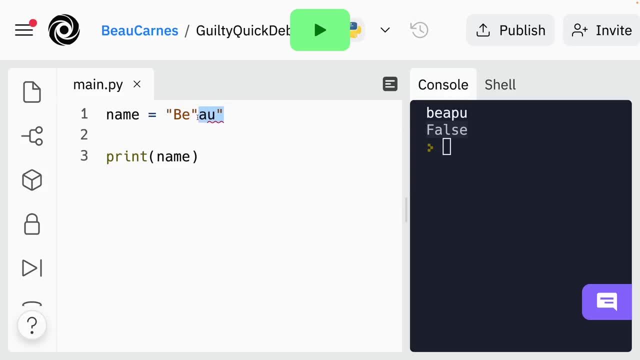 that's not going to work because this is going to be the string and then it's not going to the code editor. it's not going to know what to do with this last little bit here. So the way to go is to escape the double quote inside the string with the backslash character. So right before this. 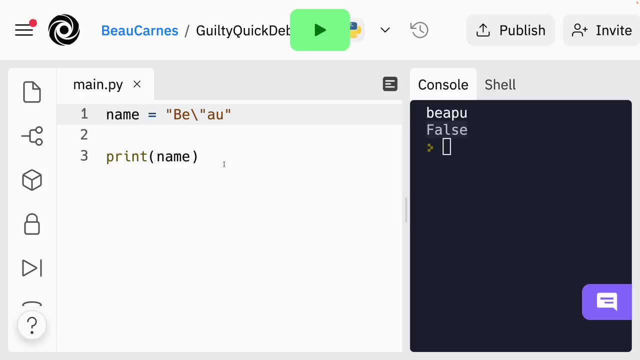 quote: I'm going to put the backslash character And then you can see it. now all is all the same color as a string And if I print it it's going to. it's not going to print the backslash character, So 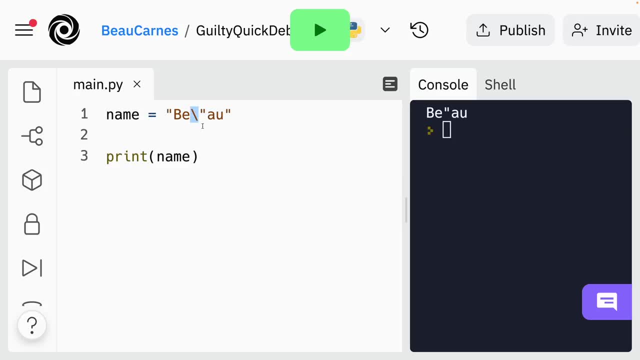 putting a backslash is how you escape a character, And that just means this: the the backslash character means that the next character is not going to mean what it normally means. It's going to actually just be the string of that character, And 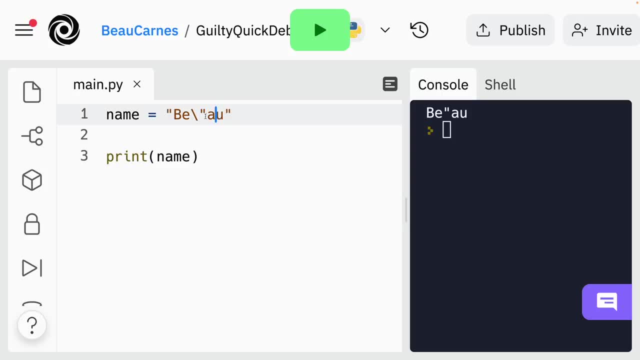 So you can do the same thing with. so with in this particular example, you may not need to do it, because you can always just put a single quote at the beginning and ending, And as long as you have a different type of quote at the beginning and ending, then you can put a double quote in the 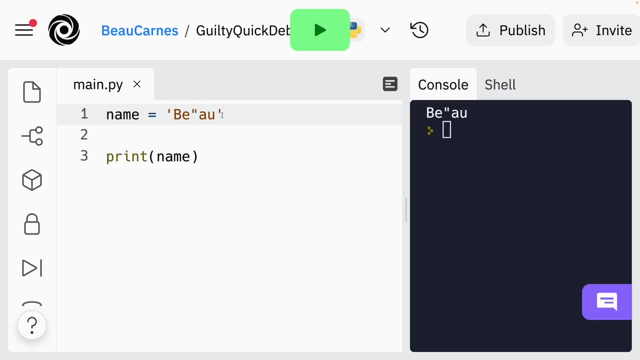 middle. But let's say you want a string that contains both a single quote and double quote within the string, then you will have to backslash, like if I just put a single quote there's going to mess it up, But if I put a backslash now it's going to have the single. 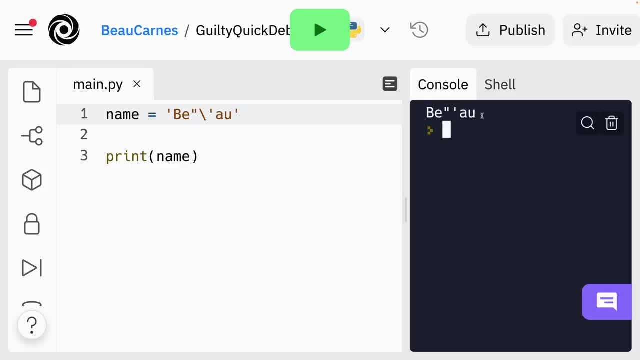 the double quote and the single quote right within the string, And you can also use the escape character for special formatting characters, Like, for instance: what if I want there to be a new line between the first two and the last two letters of the string, if I do slash in? 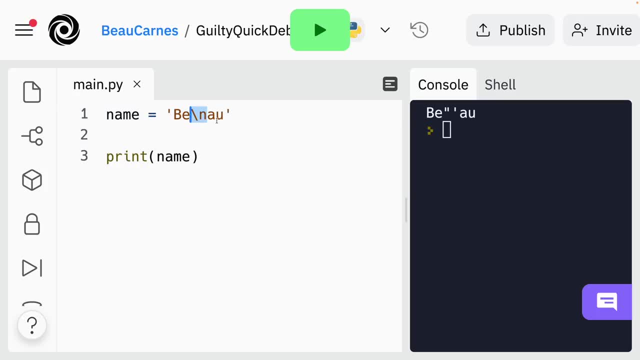 that is going to not actually just put a slash in. let's see what happens. when I put that this is means new line, you can see it says be new line a you And then another way, a reason why you may want to use an escape here, like: 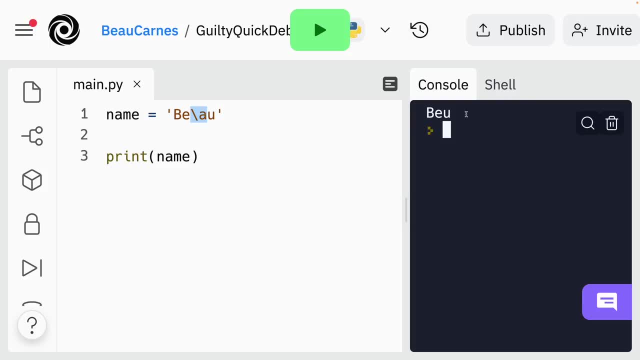 let's see what happens if I do this. this that's not looking how I want to look, because it's normally. normally when the code is running, if it sees this backslash, it thinks it's an escape character. So if you want to actually add a backslash to a string, you have to escape the. 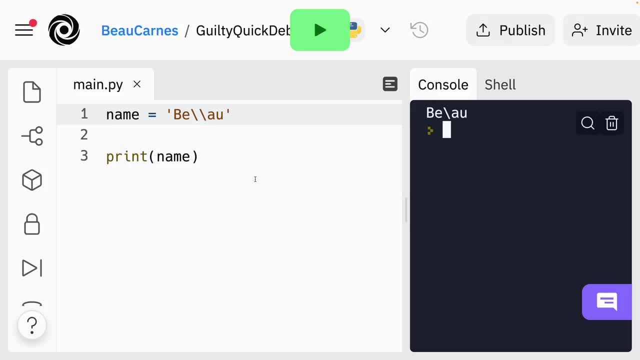 backslash. So if you want to actually add a backslash to a string, you have to escape the backslash. So now it's be backslash a you. Okay, we're done talking about escape characters. Now I'm going to tell you how you can get a specific character in a string. So, given a string, 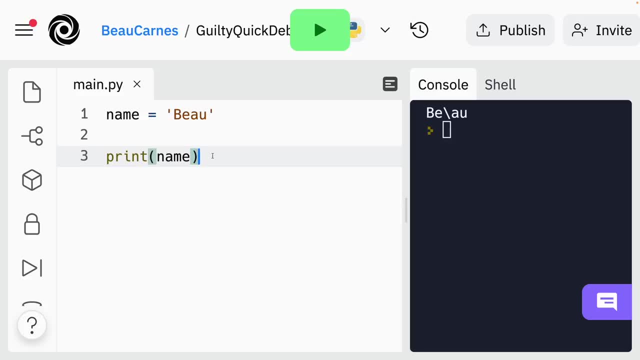 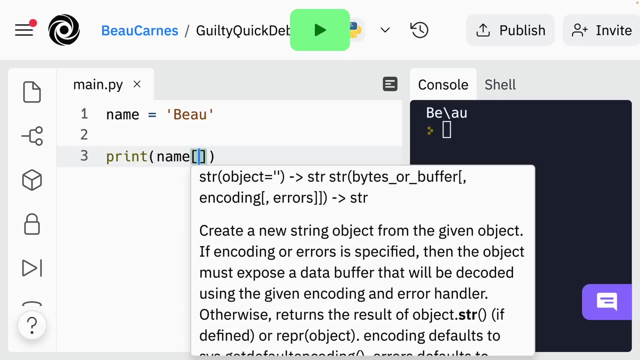 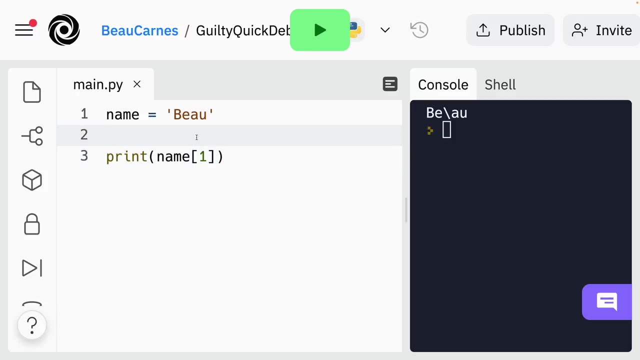 you can get its character using square brackets to get a specific item given its index starting from zero. So one thing to know about programming is that whenever you're counting for in, in most programming languages you start counting starting at zero. So this is going to get the 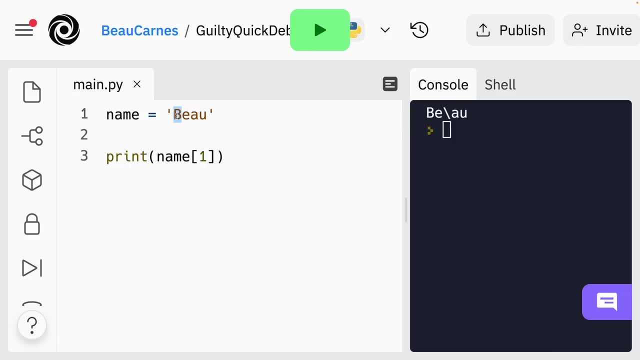 letter at index one. So this is index zero. the B, the E, is index one. index two, index three. So if I run that we can see we are getting the E. that's at index one. if I want to get the B, 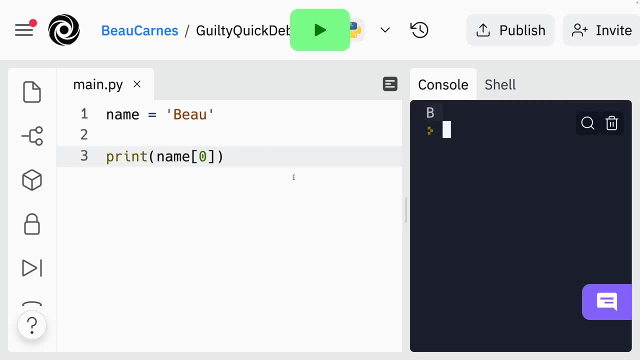 I just put a zero in the brackets and we get the B And then we can use a negative number to start counting at zero. So if I run that we can see we are getting the E. that's at index one, if I want. 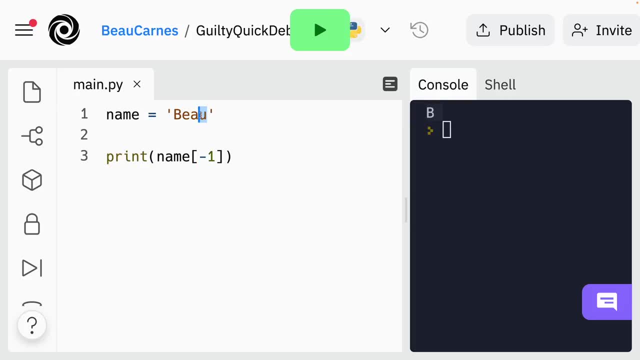 the end. So if I put negative one, it's gonna start here zero one and that's going to be a oh you, Okay, I guess when it's going backwards it's not going to start zero because there is no. 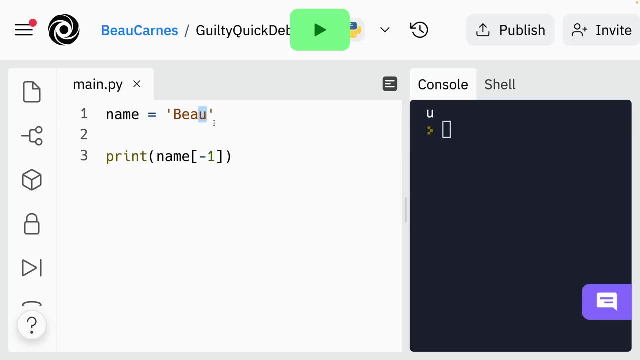 negative zero. That makes sense. So negative one is going to be the last character in the string. So negative one, negative two, negative three and so on. We can also use a range using what we call slicing. So if I put one colon two, this is going to be every character. 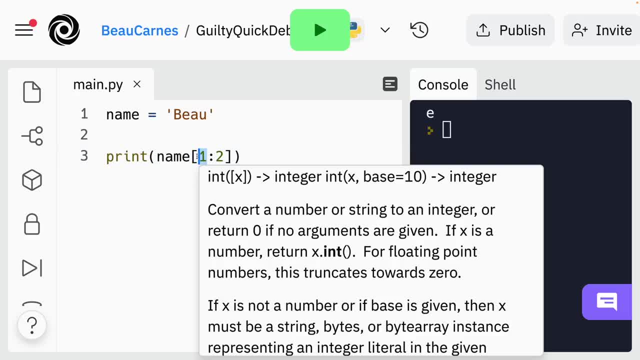 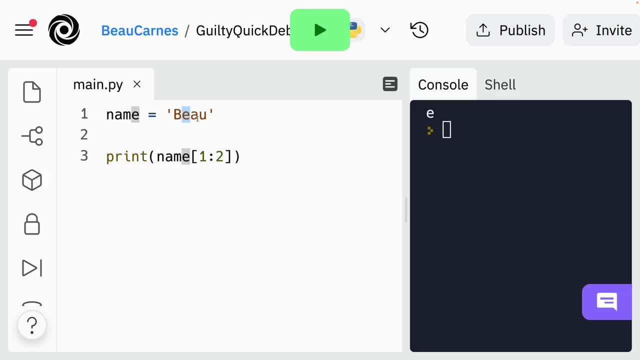 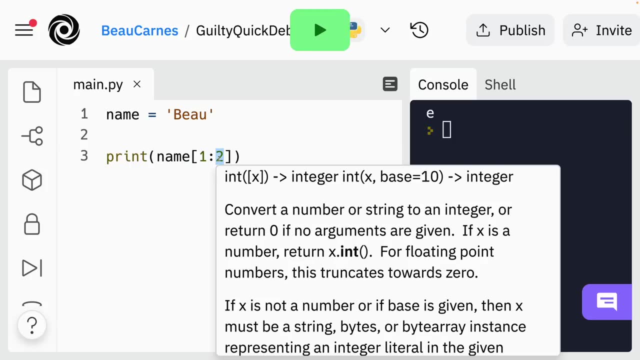 starting at index one and ending before index two. So it starts at index one, so it starts with that character and it ends before and next two, which is a. so that's actually only going to return an E, But if I put three here now we can return a U. And if I put bow, 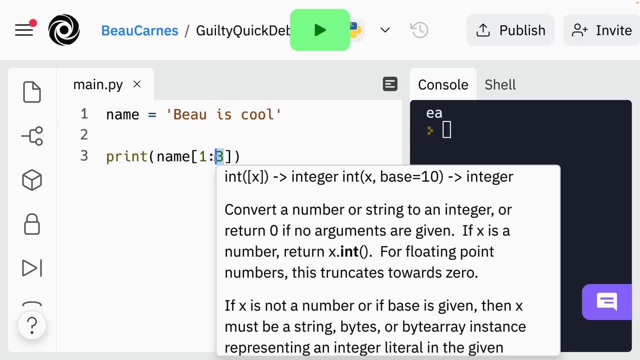 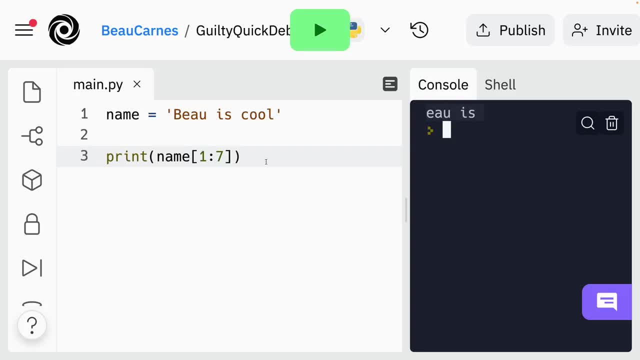 is cool. we can put one further down. I'm going to put seven and we can see it's correct. going to return part of this string And then you can also start. if you just put a blank before the colon, then it's going to return everything up to. it's going to start at the. 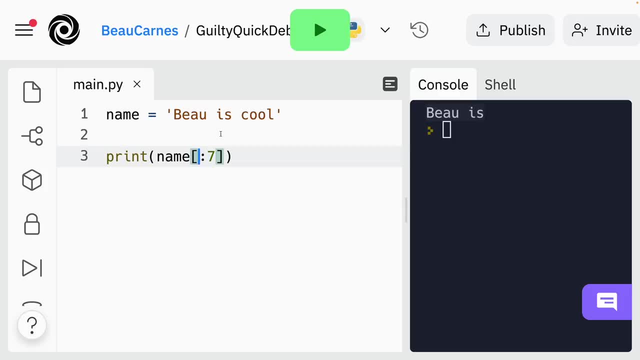 beginning and return everything up to character seven, And you can also do in the opposite direction. So if I put a blank after the colon, it's going to go to the end of the string. So it's gonna say: is cool. So let's talk about Boolean. Well, we already talked more about. 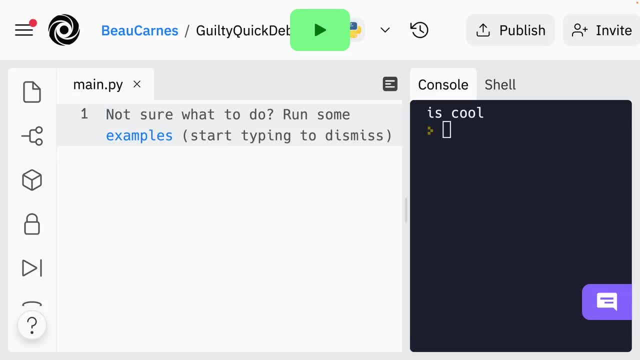 we already talked about Boolean, But we're going to talk a little bit more about Boolean, which is considered the bool type, And this can have two values, true or false. So I can say: done equals true. or you can do: done equals false. Now notice that it always has a capital. 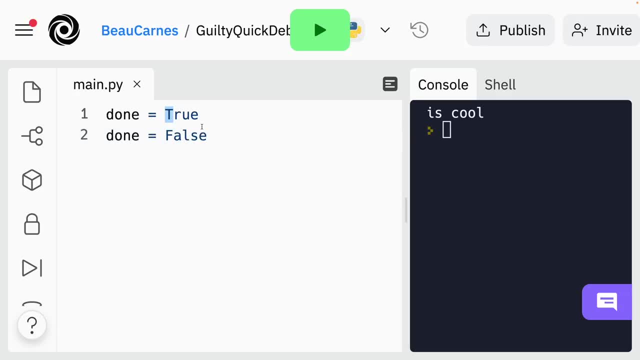 T or a capital F. So if you don't put a capital T or capital F, it won't be considered the true Boolean value. 007. Python And Booleans can be especially useful with the conditional code, with conditional control structures like if statements. Well, we already discussed if statements in the 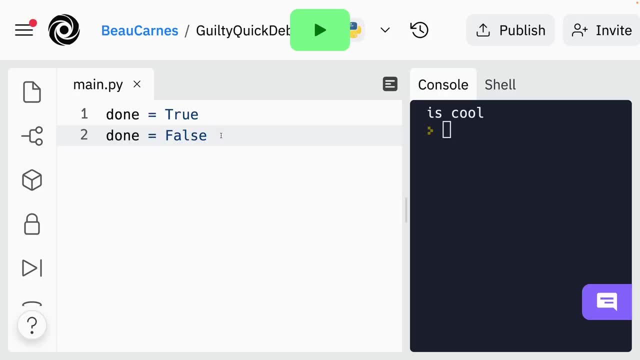 first part of the course and we'll be discussing them more in detail later, But let me just show you an example. So if done- and I'm going to erase this: done because we want to be true. So if done, and then we'll say print. 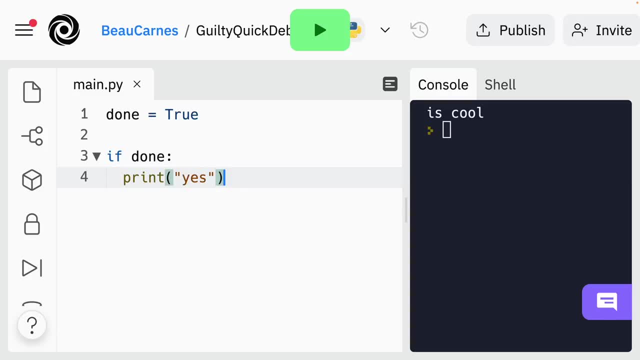 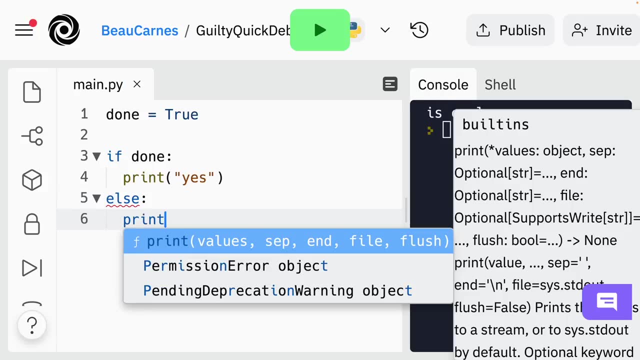 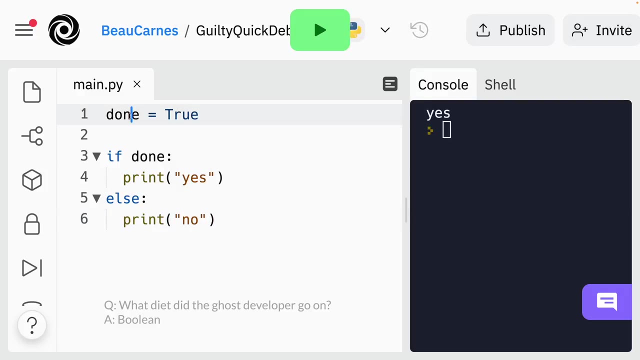 This else print No. Okay, so I can run that And it's gonna print Yes, because done equals true, But if done equals false, that's just gonna say no. So when evaluating a value for true or false, if the value is not a bool or Boolean, like if it's not true or false, we have some. 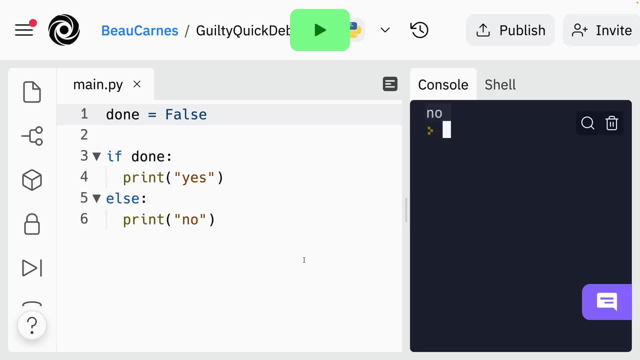 rules. depending on the type we're checking, The numbers are always true except for the number zero, Like if I put zero here it's going to evaluate to false, But if I put any other number here it's going to be true, even like negative one or anything like that. 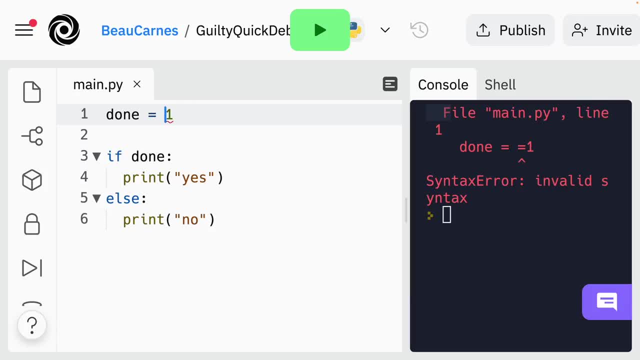 It's going to be true. Oh, I guess That I didn't put negative one, I put equals one. So if it's negative one, that's going to be true. So strings are always false. Oh, strings are false only when empty. 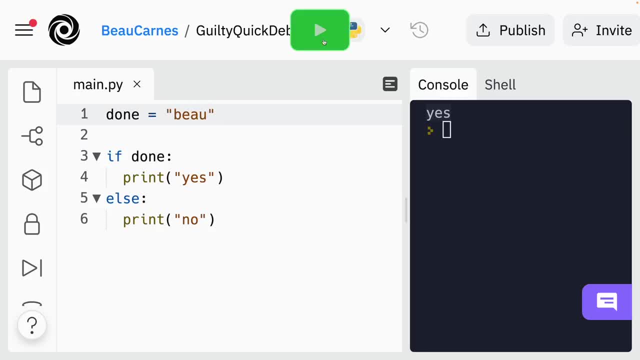 So if I say bow here, this is going to be true because it's not an empty string. But if I make an empty string then it's going to be false. list tuples and sets and dictionaries- which we'll talk about more later- are false only when empty. So it's gonna be if a list tuple 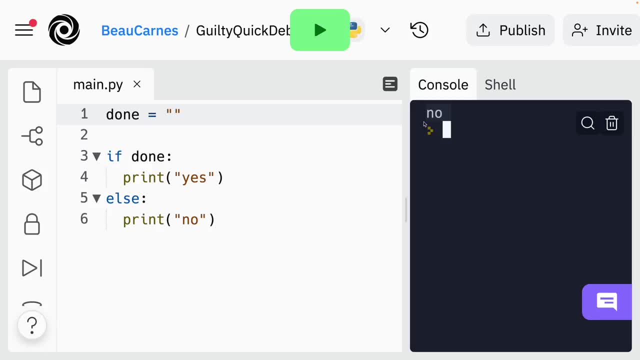 set or dictionary is is filled with something that is true. And then also you can check if a value is a Boolean. So if I say done equals true, I can do print type: we're gonna check the type. we're going to check if the type of done. 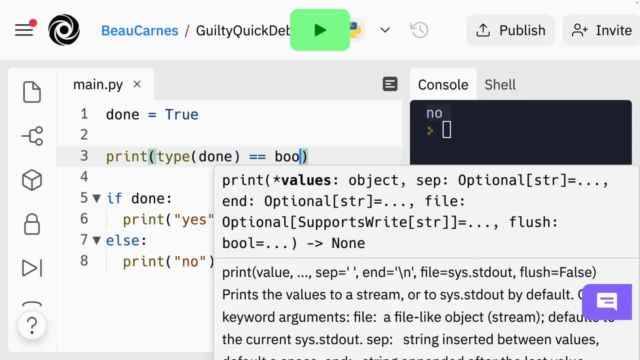 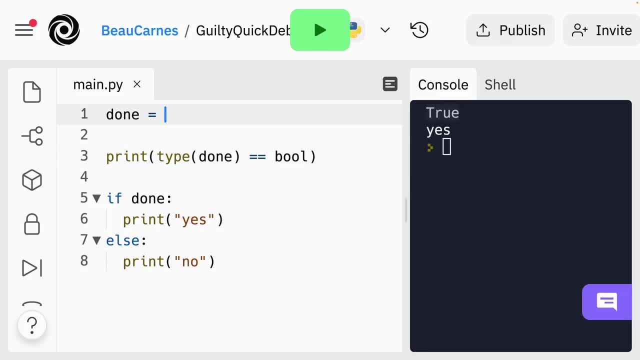 equals bool. So let's check it. Does that equal Boolean? True, it does. Now let's see. let's change this to a different type And it's going to say false. So it can still evaluate whether this is true or false. but the type is not a Boolean. the type is a string And 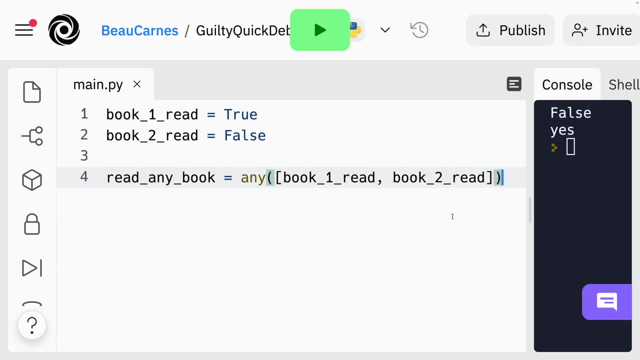 let me show you another example code. So the global, the any function. it's a global function. it's very useful. I'm working with Booleans. it returns true if any of the values of the interval, such as a list. if any of them are true, it's going to return true for all of them. So, for instance, 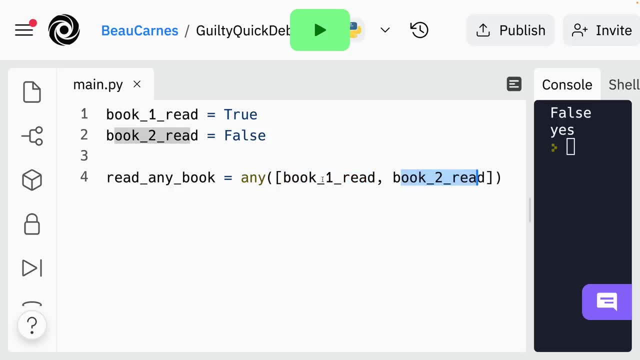 book one read that's true, but book two read that's false. But this is going to return true because it's checking if any of them are true and then it's going to set this to true. Now the all function is is similar but returns true. 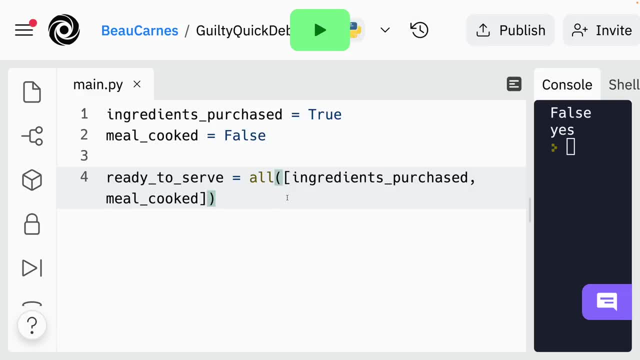 If all of the values are true. So we see, we have this value as true, we have this value as false, whereas any would have returned true. this is going to return false because only returns true if all of the values are true. Okay, now let's talk about more number. 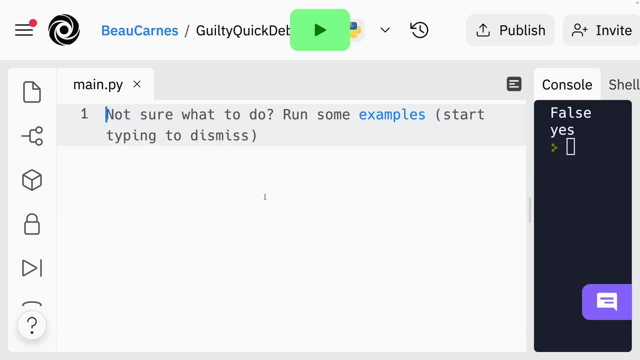 data ties. we already talked about int and integer whole number. we've already talked about float, which is any In the number with a decimal point. There's another type, called complex. complex numbers are an extension of the familiar real number system in which all numbers are expressed. 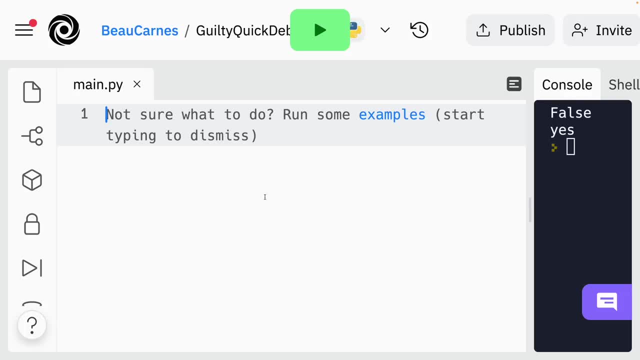 as a sum of a real part and an imaginary part. Imaginary numbers are real multiples of the imaginary unit, which is the square root of negative one, often written I in at mathematics or J in engineering. Python is built in support for complex numbers which 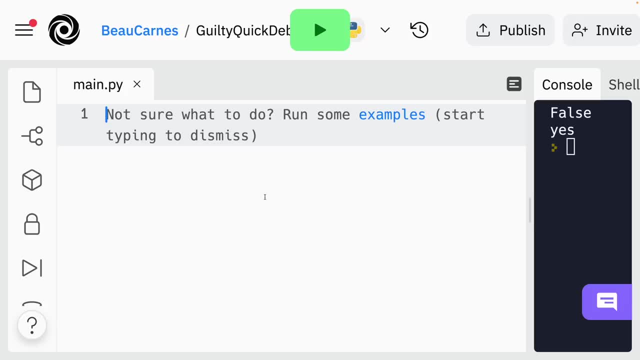 are real and complex And, to be very clear, complex numbers are numeral numbers. So the written with the, the J notation, So the imaginary part is written with a, with a J suffix. So you can combine it, you can use a literal value like complex equals two plus three J. 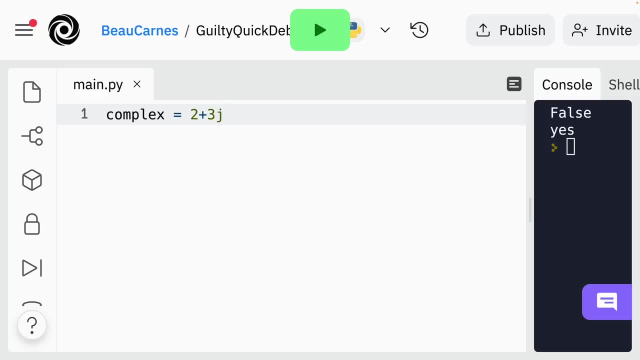 So the J means it's the imaginary part of the number. Or you can use the complex constructor So I can put num equals complex and then I'm going to pass in two comma three. So the three part is the imaginary part, the two is the, the real part, the integer part, And 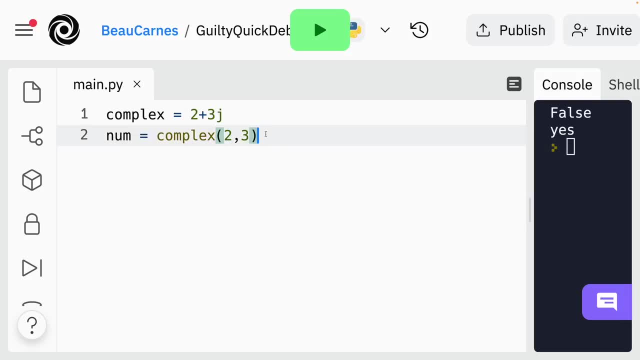 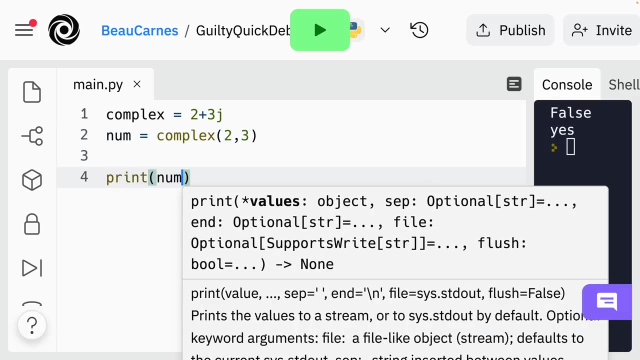 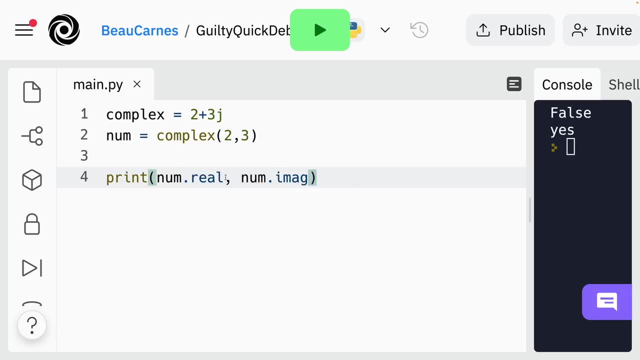 then, once you have a complex number, you can get its real or imaginary part, like this. So I can say: print: num dot real or num dot image. So this is going to be the two, this is going to be the three. So 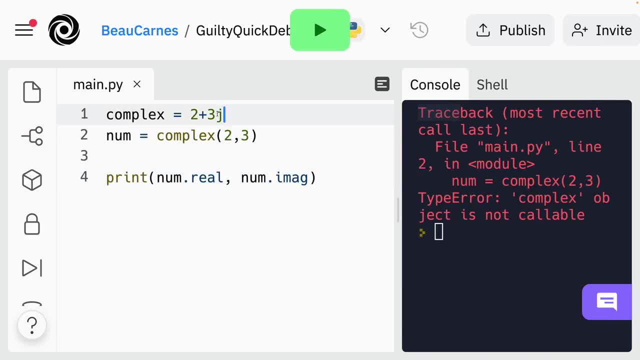 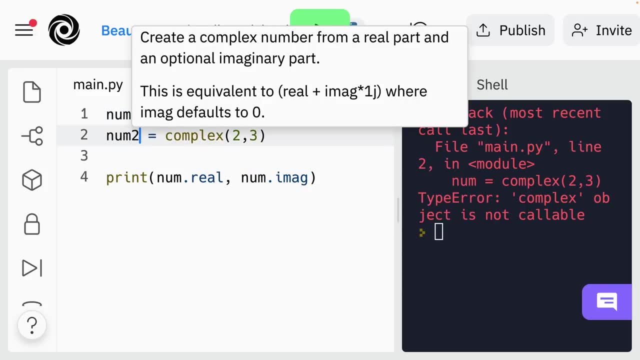 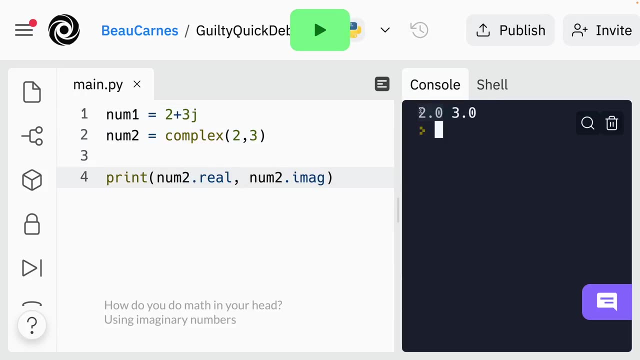 if I just let me. I think the problem was num num one, So I'll do num one and num two, And we're going to do this as num two. Okay, let's check this. So this is the real part, This is the imaginary part, And you can see they're being returned as floats. 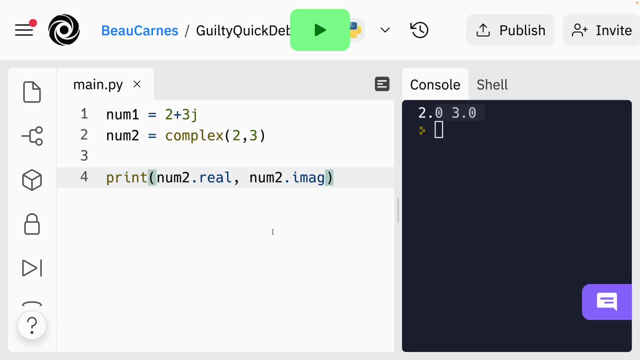 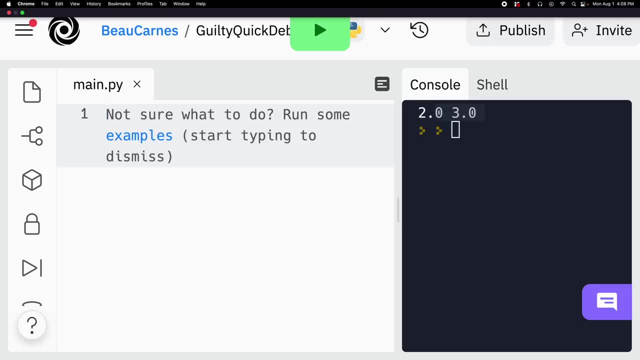 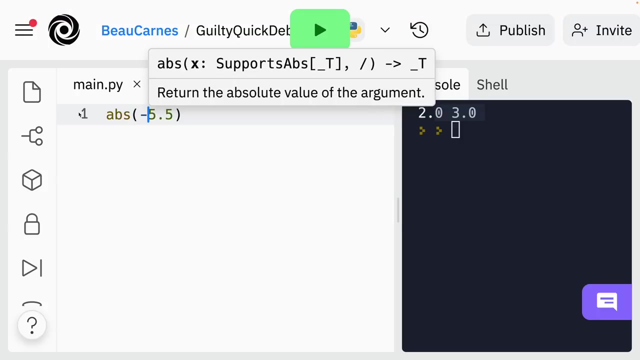 And you can use the type function to check the type. So now let's talk about some built in functions that help with numbers. So one of them is ABS. ABS will return the absolute value of a number. So if I say 5.5, that's just going to be 5.5. But if I put negative 5.5, well it will be. 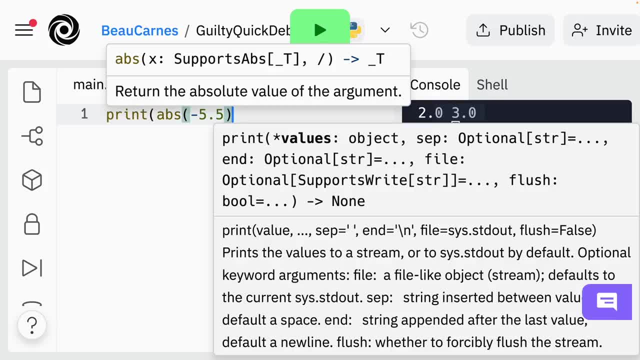 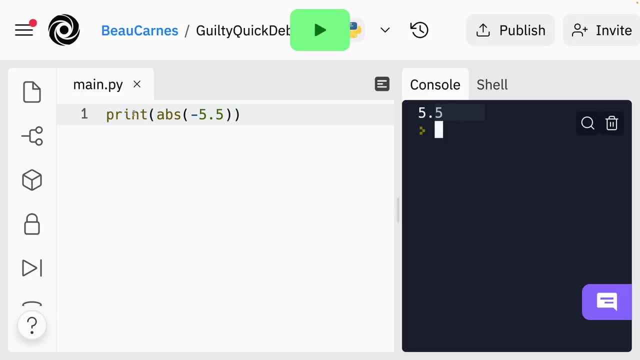 5.5.. So if I print this, the 5.5, basically it just makes it, so it's not negative- then you can also use round. So if we do round, let's make this just 5.5.. Round is going to round to the nearest. 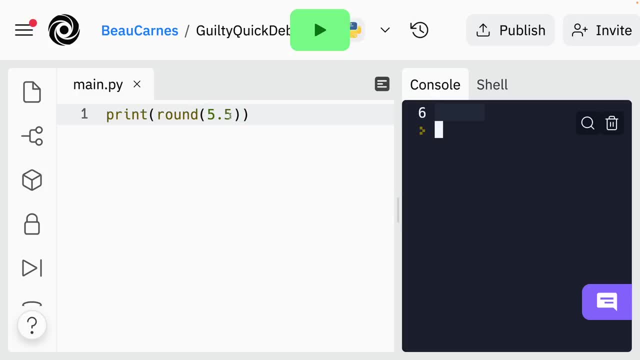 integer. So if I do this, is this going to be six, or point five is gonna round up, But if we did four, nine, it's going to go down to five. you can also specify a second parameter to set the decimal points precision. So I can go to, if I do one here and they round it. 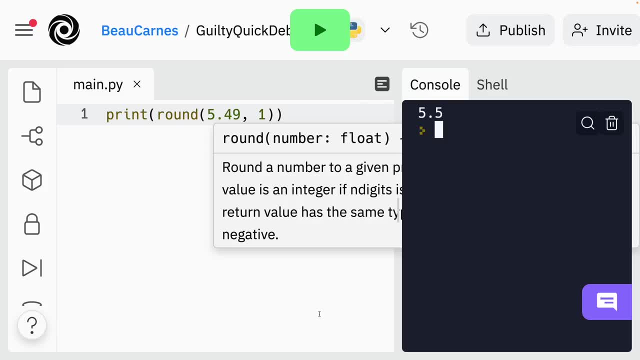 it's going to, instead of rounding to the nearest integer, is now going to round to the nearest 10th place value or one decimal point. There's several other math utility functions and constants that are provided by the math standard library, like there's a math package, a C math package. 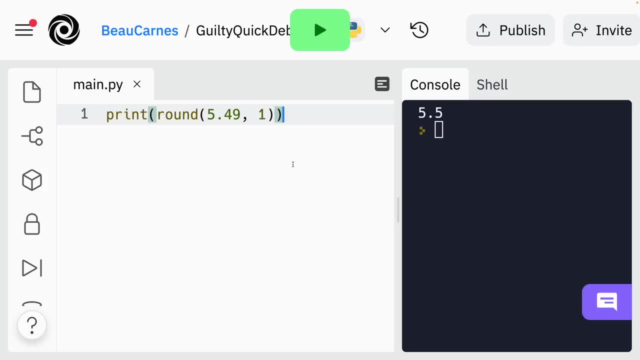 decimal package, frac fraction functions package. that makes it easier to work with different types of numbers. We'll explore some of those more later on. Now let's talk about enums. enums are readable names that are bound to a constant value. So to use enums we're going to have to import enums from the enum standard. 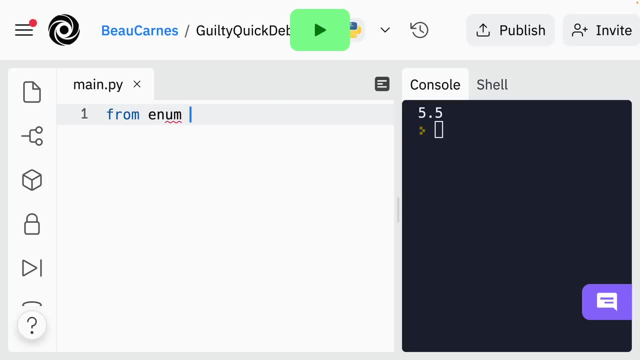 library module like this from enum import enum- And now we'll be talking more about importing stuff from modules later. But once you import it, then we can initialize a new enum in this way, So do class state enum, And so we can have inactive. 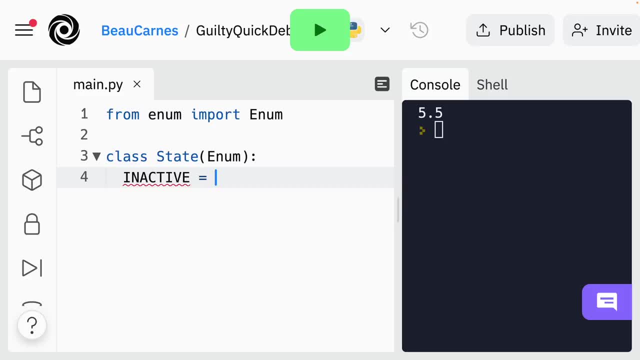 equals zero and active equals one. So basically the word state, this can be anywhere, any word we like. So we're setting a, basically a variable called state dot inactive, which is going to equal zero or state dot active to equal one. So you can reference this how you would reference it. you can do: print state dot. 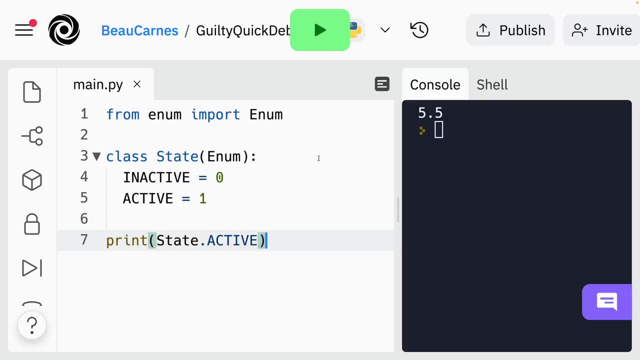 active And then if I just run the program, we'll see. Now you can see it just going to return state to active instead of one, So to actually get the value you use- state to active dot value. And then we run that And then we'll see that it's going to return state to active, And then we'll see that. 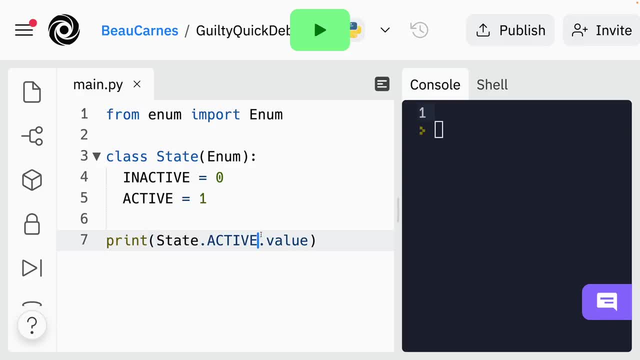 one here. If you we want to just return state dot active, that this, that value can be reached by the number assigned in the enum, So state, we can do one. And if I print that is now going to say state dot active. same for using the square brackets notation. So I could do states, I'll. 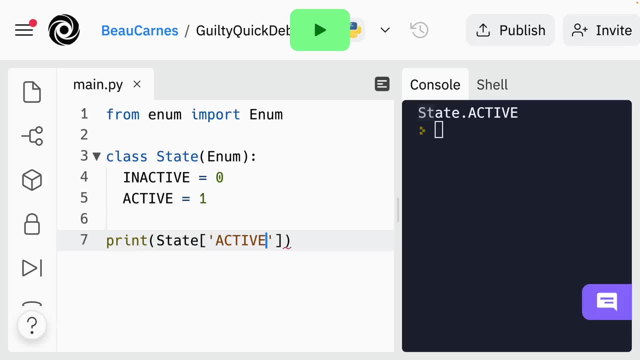 do see square brackets and put active by print that it's going to print. state dot active. So this is basically the only way to create constants in Python. Python has no way to enforce it. a variable should be a constant, So some people use enums to create a constant and then nobody can. 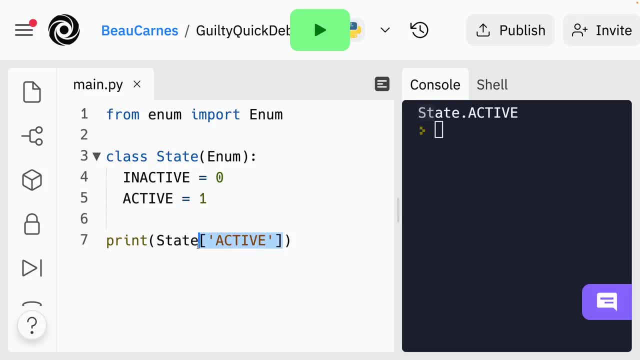 reassign the value. So when we do state or state active dot value, So this is, it's not going to be able to be reassigned. So basically there's two ways to do. we can do this bracket notation or we can go back to the other. 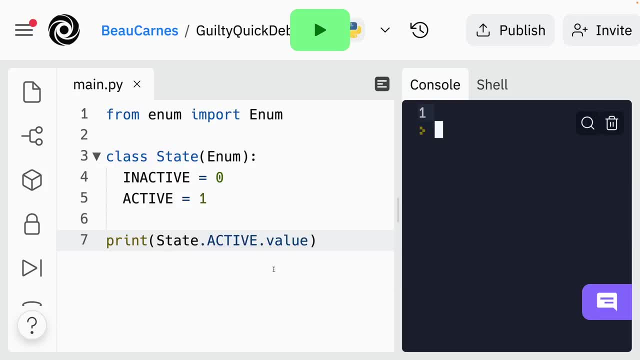 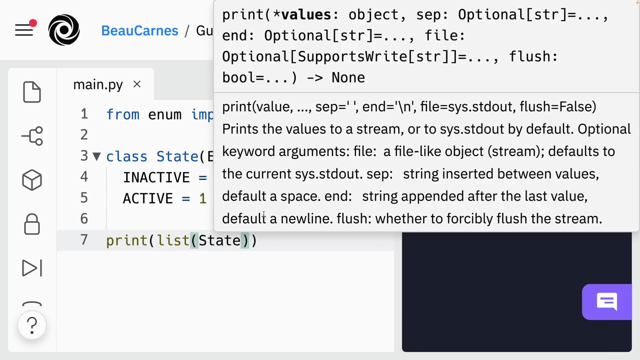 way Active. Now we can also list all the possible values for an enum. So our enum is called state And we can now just print all the values. Oh, I actually did that wrong. It's supposed to be a list. So this is going to list the values of the state And we can see we have an active zero and 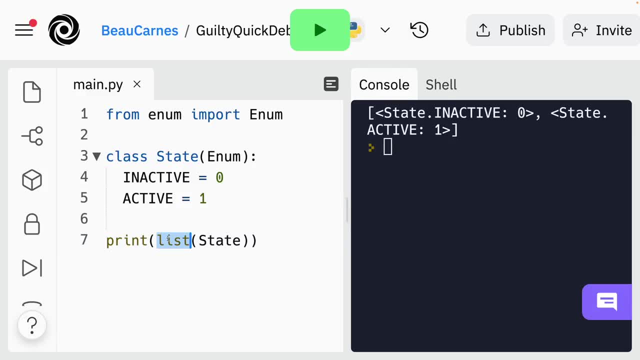 active is one, And we can also count them using the length function. So we're going to print the result of a length state And that's just going to give us two. Okay, let's talk about more about user input. Now we already 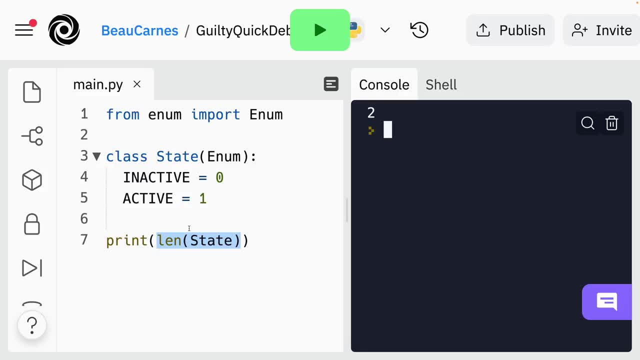 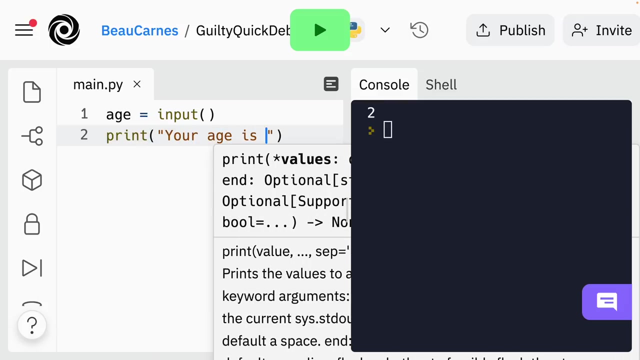 discussed a little bit in our first program. But you can do get user input by using the input function. So let's just get rid of all this And we'll do age equals input And we can say: print your age is, and then we just can concatenate that with the variable age And then also 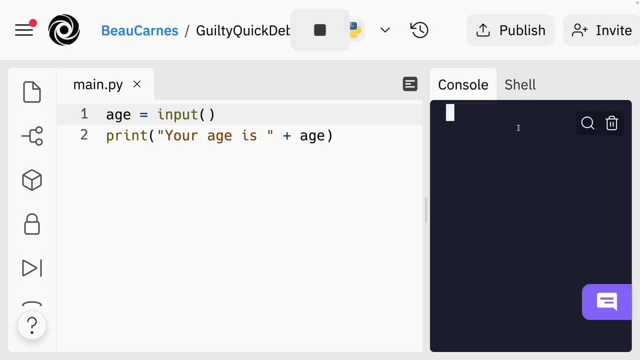 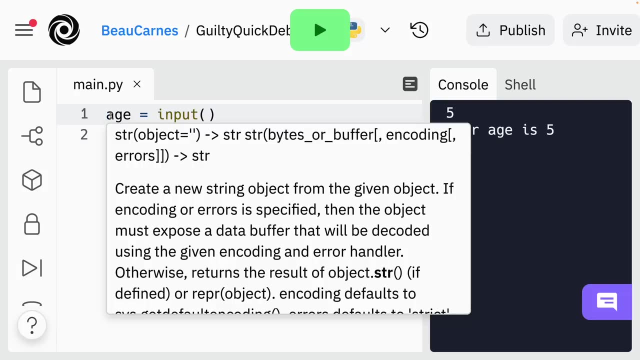 if you want to. so let's just do a quick test And right now it's looking for the age. right now I can put five. your age is five, So there's two ways to make it say what is your age. 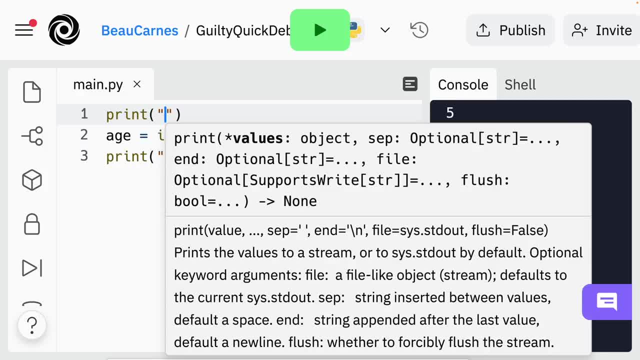 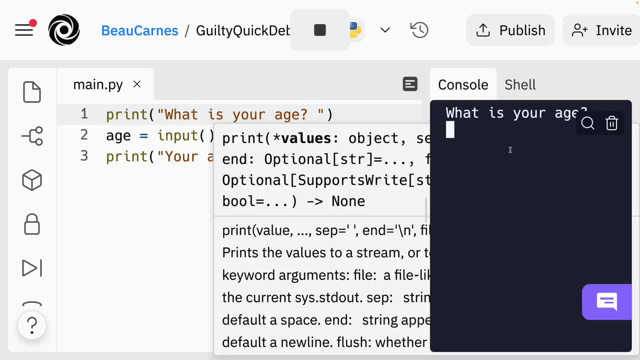 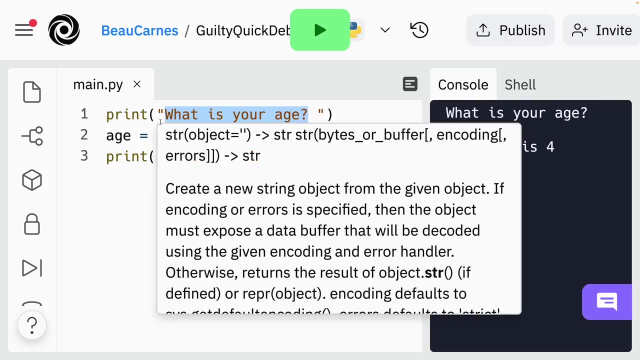 we can do a print statement right before here and do what is your age, And then now we can put four and your age is for now. you can also, instead of putting the print statement right before here, I'm going to copy this- delete that And we can put it right. 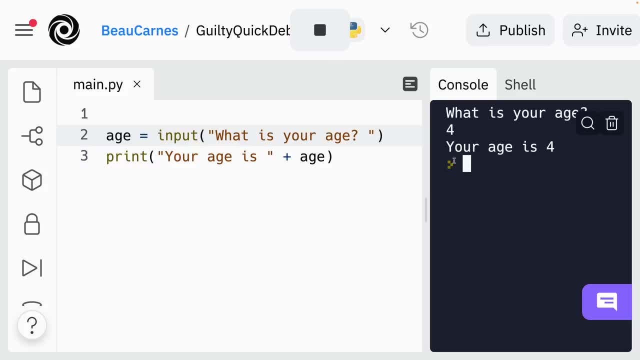 in this input function And then I'll say: I'll still say what is your age, and I can put an age here. So one thing to really realize about this is that it gets the input, you get the input, you get the output, But then it doesn't say that the age, It doesn't really. 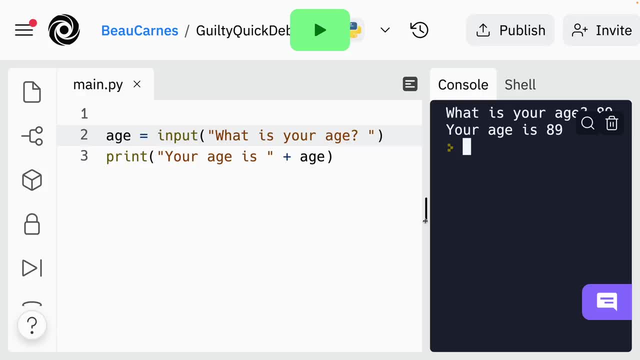 at runtime, meaning the program will stop execution and will wait until the user type something and presses the Enter key. You can also do more complex input processing and accept input at program invocation time And we'll see how to do that later on If you want to get the input when. 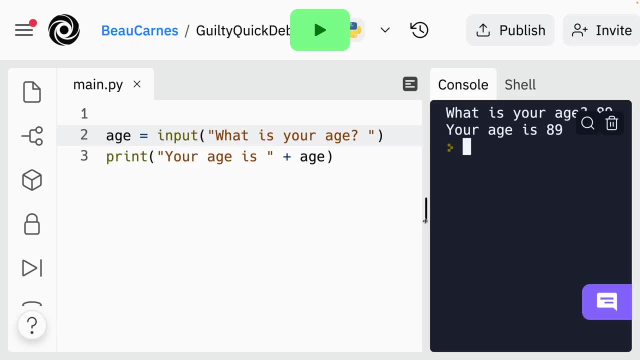 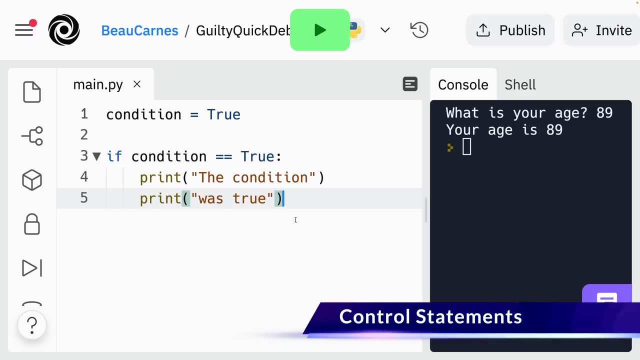 the program is run. that's going to work better for command line applications. Other kinds of applications will need a different way of accepting input. Let's look more at control statements. This is another thing we've already discussed earlier, but we're going to review it and and look at it in. 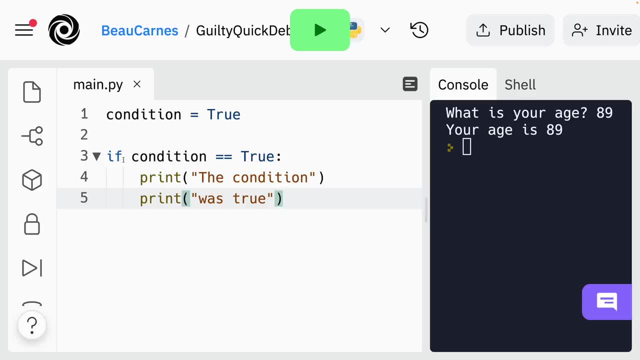 a little more detail. So a control statement is like an if statement. So if condition- this is very over here- equals true, then it's going to run everything in the block. A block is the part that is indented one level. usually it's going to be either four or two spaces. In this case it's four. 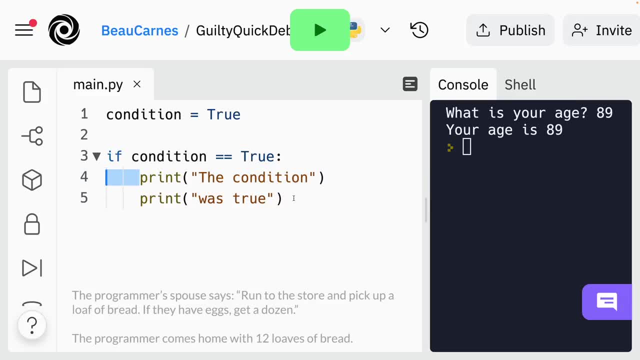 spaces. sometimes it's two spaces, it doesn't matter, it could even be one space, as long as it's the same, as long as every line of code is indented the same amount. So if I just run that the condition was true, the block can be. 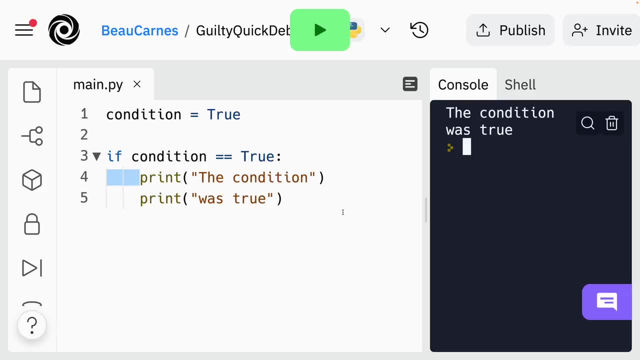 formed by a single line or multiple lines, And it ends whenever you move back to the previous indentation level. So, for instance, if once we are not indented, I can say print outside. if so, then that's always going to prison. it's always going to print this because it's not in. 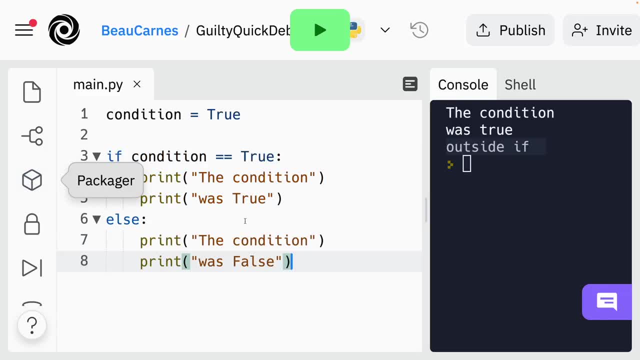 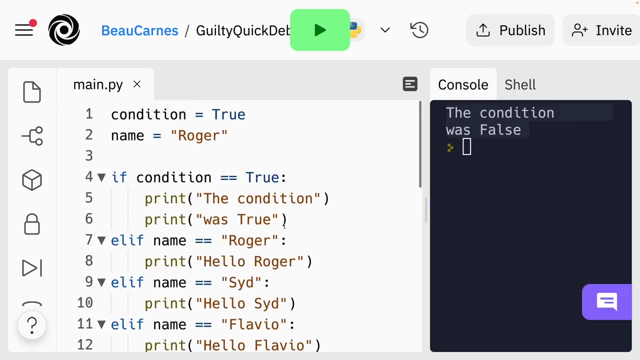 that if statement And then we have the if else statements where the else as if. if this does not true, then it's going to do whatever is in here. So if I just change this to false, then it's going to print whatever the condition was false, And then we can have the. 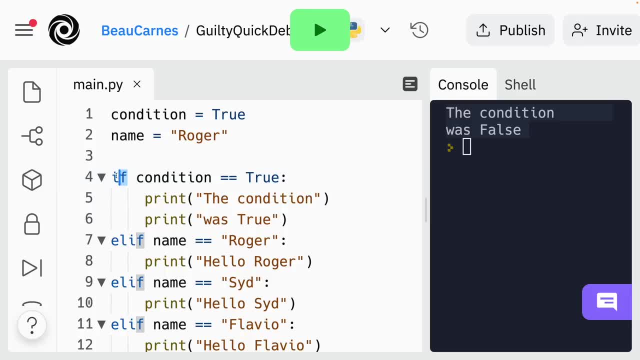 series. this is something that we showed in the program earlier. but if then l if combines else, and if so, if this is not true, then we'll move on to this line. Oh else, if this is true, then we'll do this, else if this is true, and we'll just keep going on And then it will all. 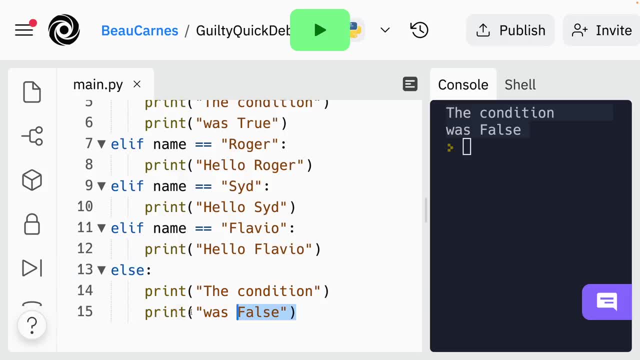 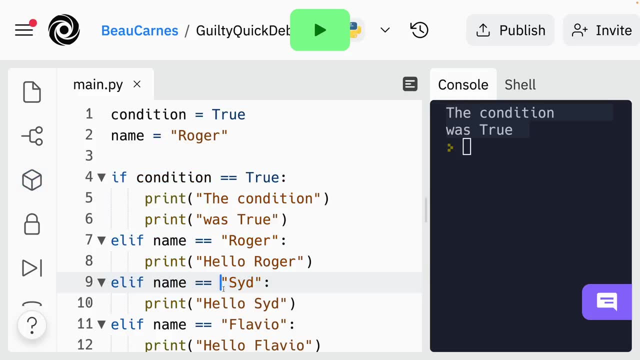 always do that. this is if none of the other ones were true. it's going to do this. So, since it was testing this, it's not even going to evaluate anything later. But if we move this to false and we change this to bow, then it's actually going to skip all the way down, all the way to. 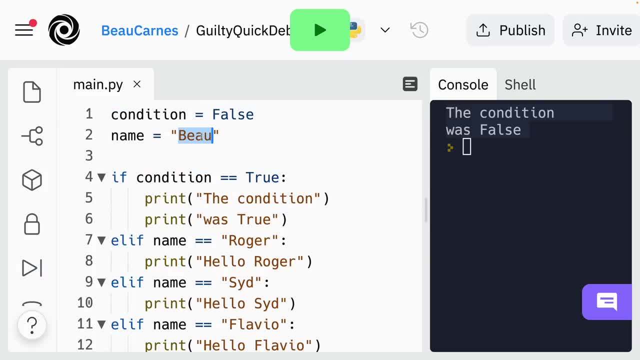 this else here, And if we do Flavio and print that, and then it's going to say: Hello, Flavio, from right here. Okay, that's all we're going to talk about for this for now, since we've already covered it earlier in the course. Now I'm going to go into more detail. 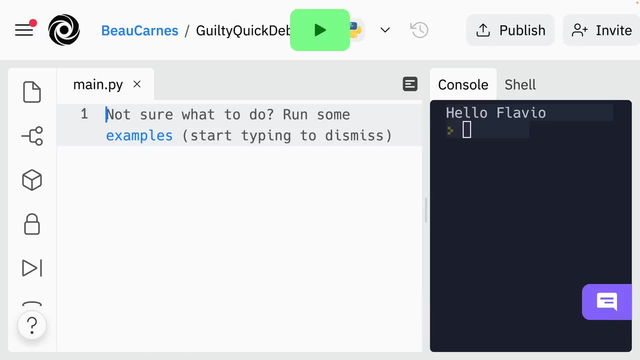 about lists. Lists are an essential Python data structure, And so an example of a list would be: let's create a list called dogs, So we're going to create the dog names. we have Roger, we have Sid, And this allows you to group together multiple values and reference them all with a common name. 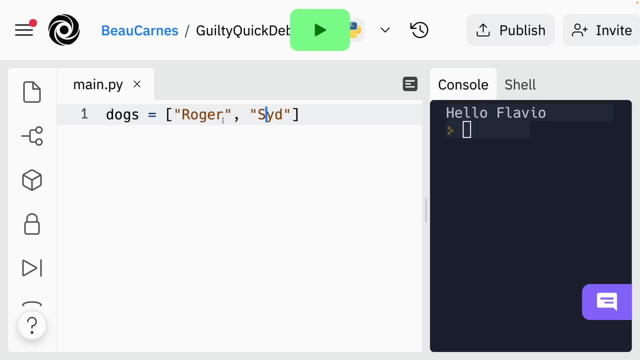 So we have a list of dogs And this is just two strings, So the list always going to have the open and closing brackets and each item in the list is going to be separated with a comma, And a list can hold different types of values. So these are all strings, But we can have a string. 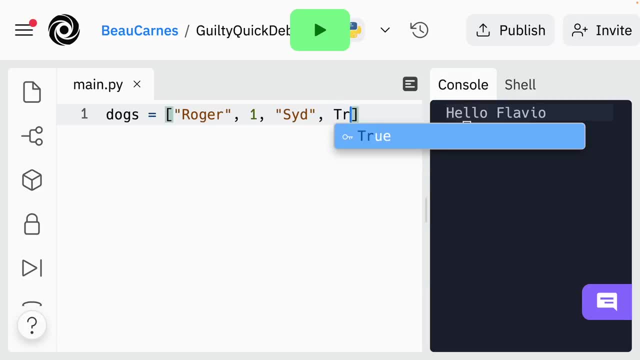 an integer, a string, a boolean, And you can mix different types of data types in a single list, And then you can check if an item is contained in a single list, And then you can check if an item is contained in a single list, And then you can. 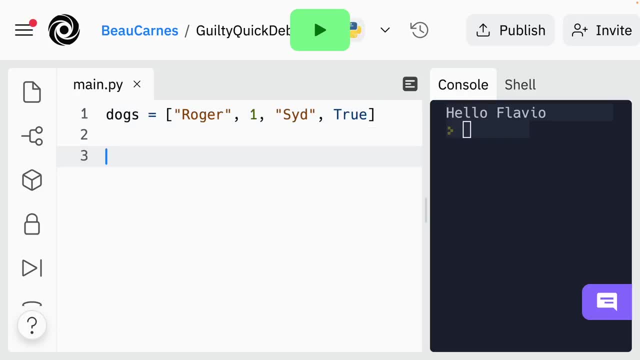 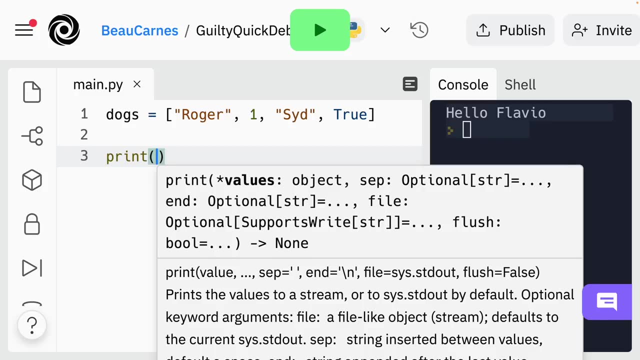 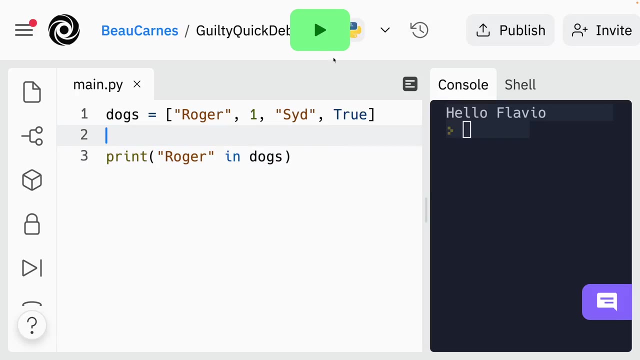 in a list with the in operator. So we talked about the in operator earlier, but let me show you how that works. So we're going to print: here's where we can use the in operator. we're going to check if Roger is in dogs, So let's see. So run that, true, But now let's check if Bo is in. 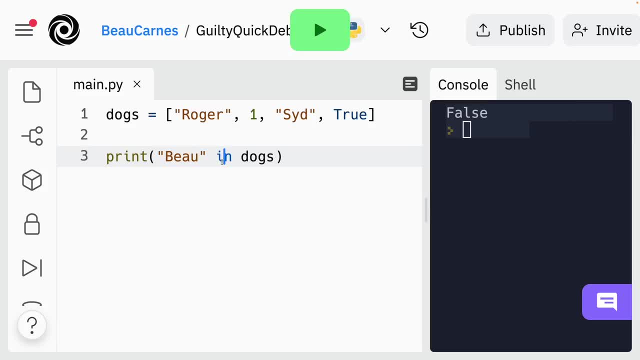 dogs. Well, false, because it's checking. So this is how you can check if an item is in a list. You can also define a list as an empty string, So I could actually just remove all this, And now we just have an empty list, And this is obviously still gonna be false because there's nothing in. 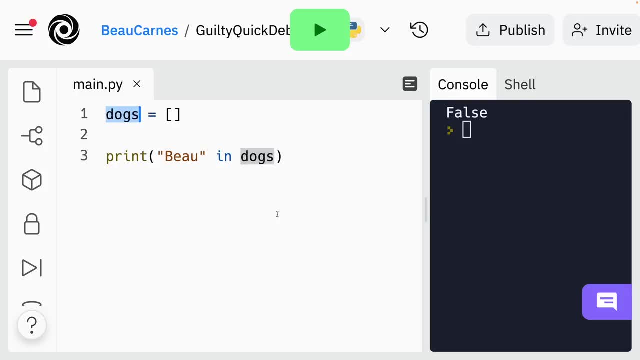 that list. But let's go back to when we had some items in the list And you can reference items in a list by their indexes, starting with zero. So I'm going to do dogs, And then I can use these brackets, So, and I'm going to put that. so this is what I'm going to do, So I'm going to put this in. 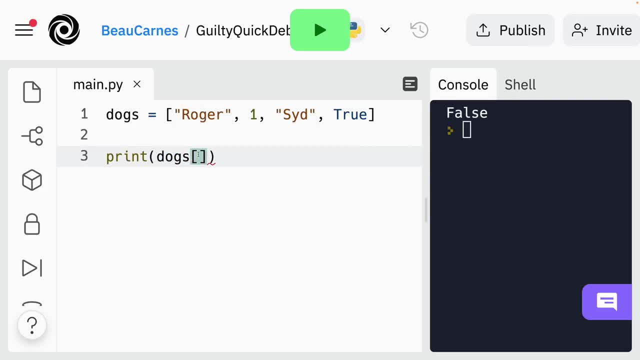 where we're going to reference the thing, an item from the list, and I'm going to type in zero, which will be this item right here, Roger, or I could put two, and it's going to do 012.. And now? 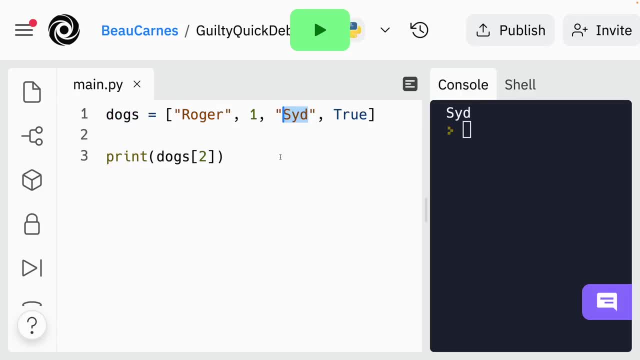 we're going to have said and the same, And you can use this same notation to update an item in a list. So I'm going to add another line of code here and put: dogs two is going to equal bow, And now I'm just going to print the entire list here And now, instead of being Roger. 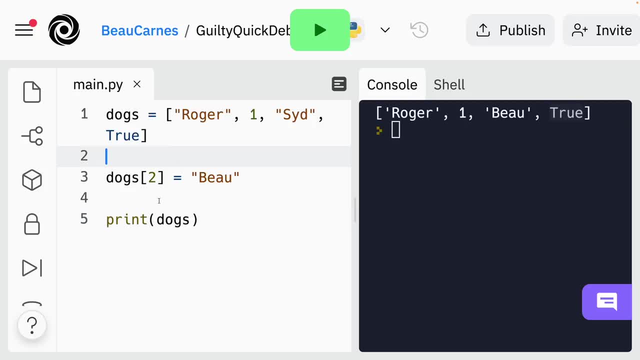 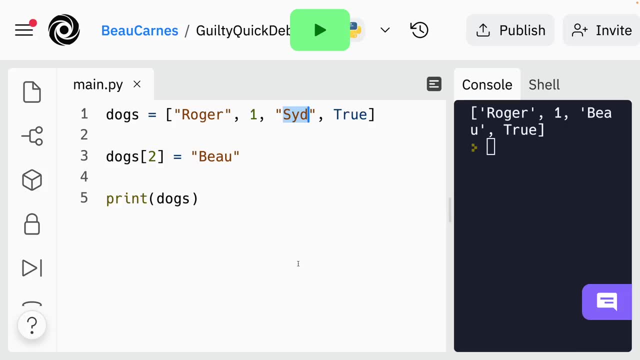 one said true to Roger, one bow. true because we've updated the item at index two to be bow instead of said. Now you can also use the index method. So instead of like: if I want to find the first item on the list, I could do it like this: So you: 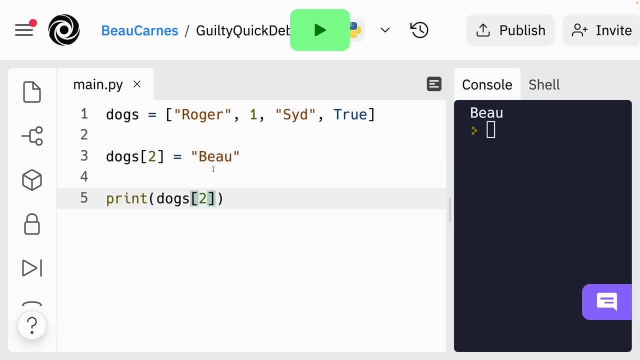 can also use a negative number here, Just how we saw on the string. So negative two is gonna start with one to X. let's do negative one So it should return true here. Okay, true, So it starts with this one. if you put a negative number, you can also extract part of the list. Now, this is very 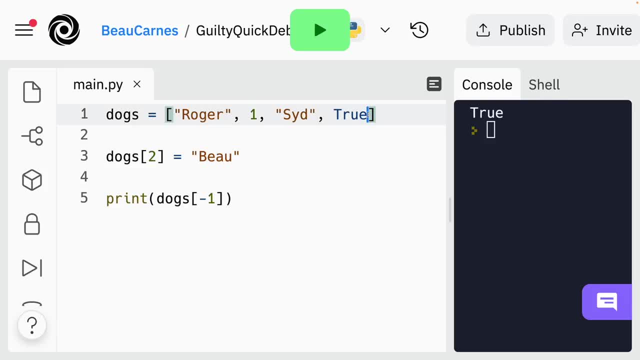 similar to what we showed using with the string. let me just add another item here. Now I am going to use the colon to do part of a list, So I'm going to do two, four, And so this is a slice. So it's going to start at the second, or 012, which is now both we change. 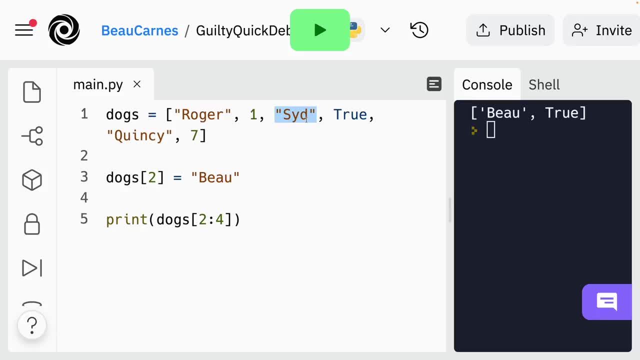 to bow and it's going to go through four. it's going to go through four, but not old Pat, not including four, So it's going to be 23.. And then not four. So just sit and true or bow and true, because we updated to to bow And you can also just leave this blank. So 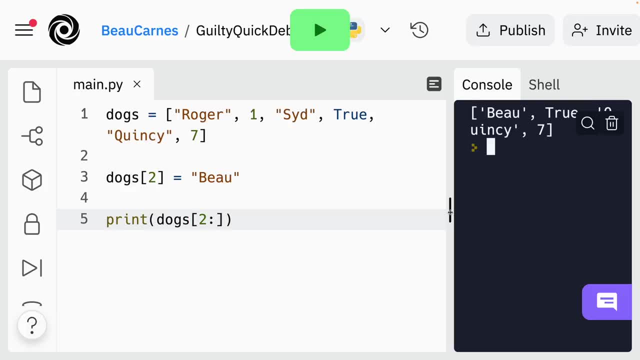 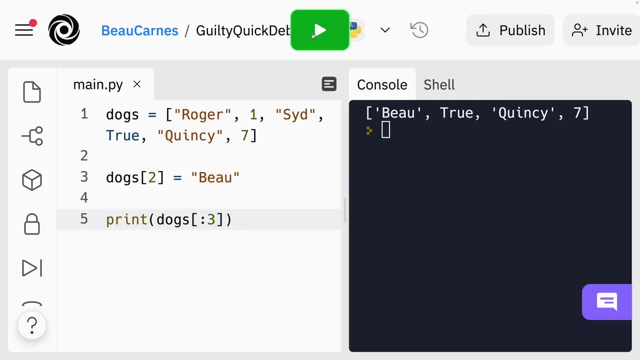 it's going to go through The end of the list. or if you leave the first number blank, it's gonna go. it's gonna start at the beginning of the list And we can go through, for instance, index three And so. 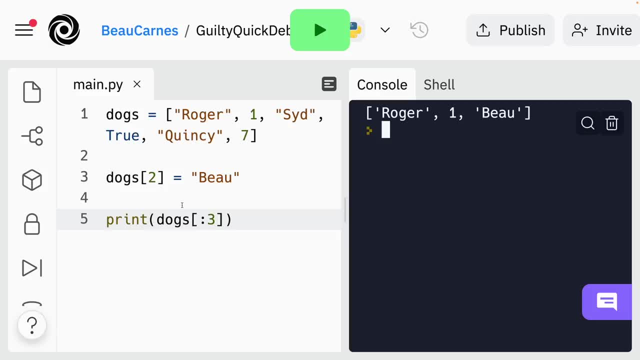 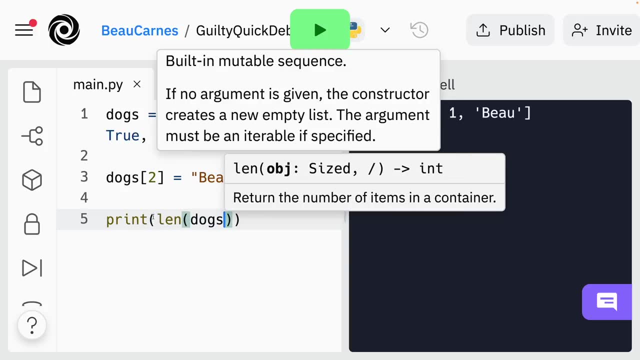 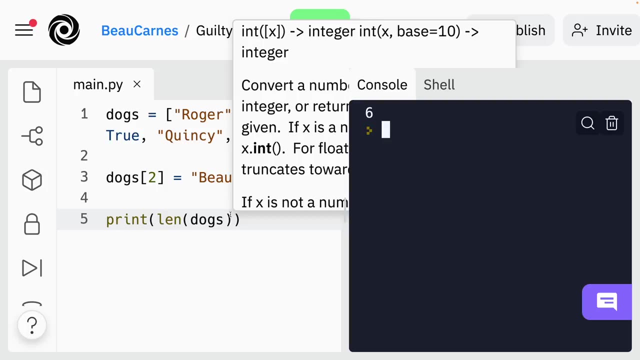 this way to slice the list. you can also use the length function. So let's find out how many items are in the list. I'll use the length. the length of dogs is six or six items in the list. we can also add items to the list. 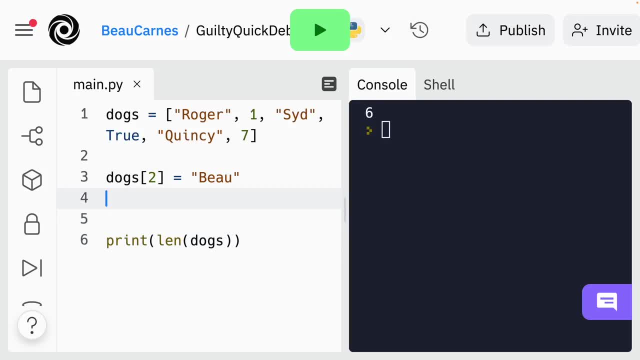 by using the append method. So I'm going to do dogs dot append and then I can add an item so I can say something like Judah, And now if we see the link there's not gonna be seven. And if we just print the full list then we can see that we can see all the items. 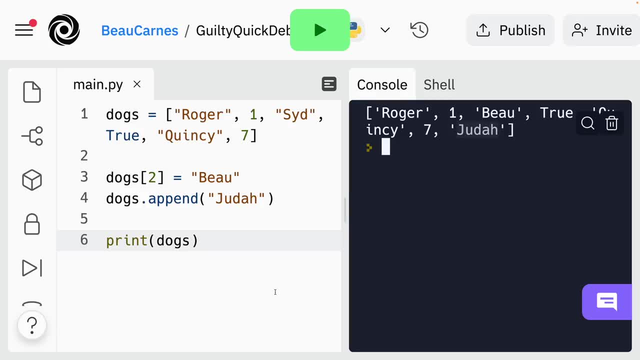 including the one that was just added. we can also use the extend method. the extend, another way to add an item to a list. So if I do, instead of dogs, append, I can do dogs that extend, And then I'm going to pass in. instead of just passing in the string, I'm going to pass in the. 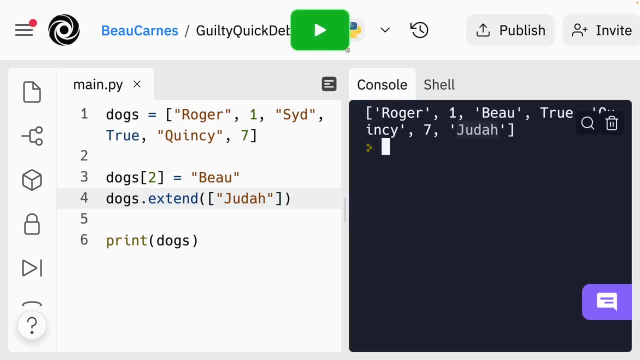 item as a list. So I'm going to, it's going to add it just the same, but now I can actually combine two lists together, So I'm going to put a five. So if I do this, we can see. now we are taking this. 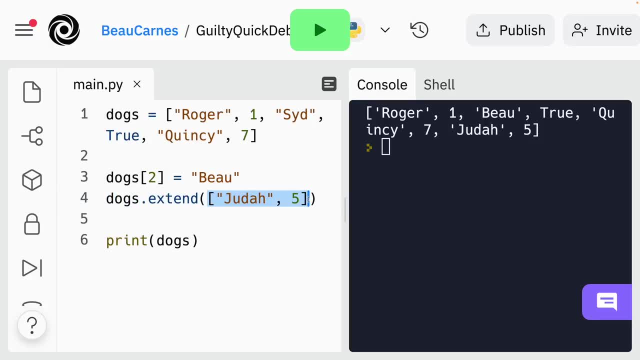 list and extending it by adding this list on the end. this is a two item list. we have that six item list And now we have the eight item list. you can also use the plus equals operator. So to use the plus equals operator, I'm going to do. dogs is the same. it's going to do the same thing. 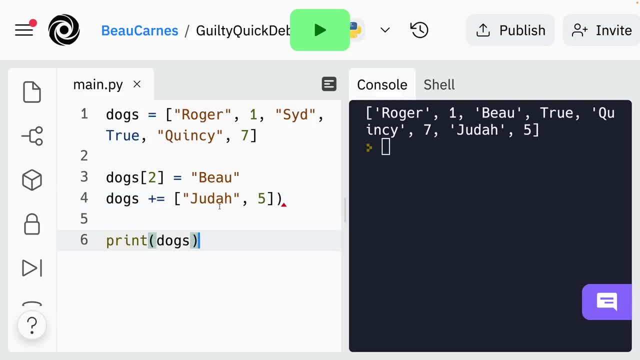 as extend, So plus equals. And then we have this list. take this parentheses off here And it should look exactly the same. See, it's showing up the same thing up here. So the plus equals is going to be the same thing as extend. work. takes the list that's already exists and adds this other list to. 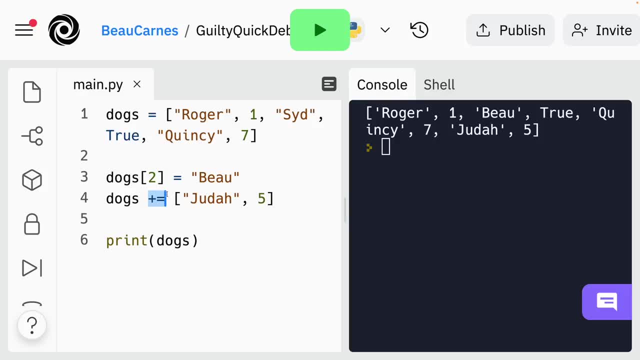 the end, And when you're using the extend or the plus equals, you don't want to forget the square brackets here. So if you, if you forget the square brackets, and let's say, I'm just gonna add this on to the list. 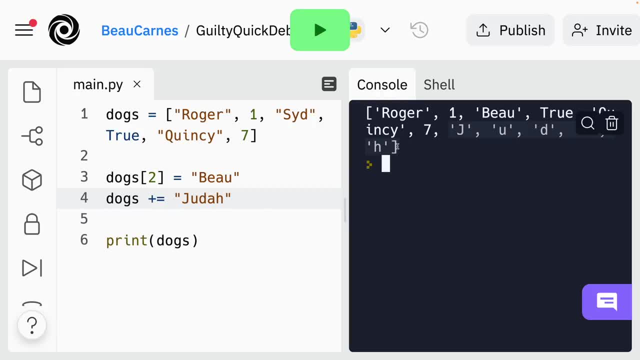 it's now actually going to put each letter individually here. So, if I can see it better, if I move over here, so it so that. so you want to make sure you put the the brackets, And another thing you can do is remove. you can remove an item using the remove method. So I'm going to do dogs dot. 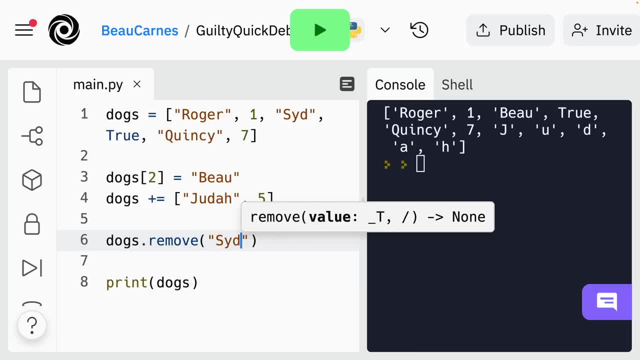 remove Sid. Okay, now I'm going to play it here And it's saying: what did I do wrong here? Oh, obviously, um, I'm moving Sid, but we've already changed the element of Sid to bow. So let's remove Quincy And let's try that. Okay, so now there's no. 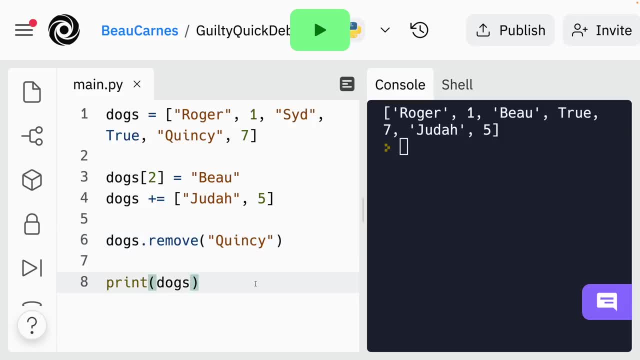 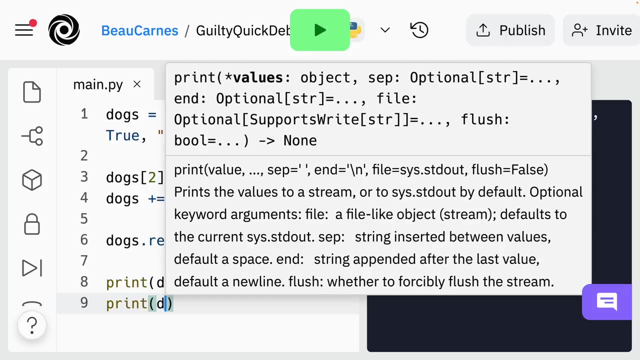 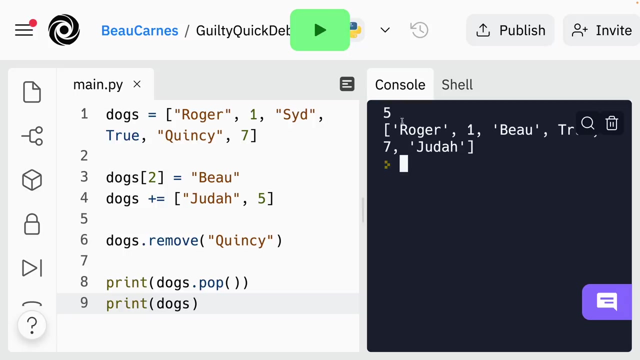 Quincy. So another common thing to do, another common list method, is pop. So if I do dogs dot pop, it's going to remove and return a single item. So first I'm going to do dot print dogs that pop and then I'm going to print dog. so if I so, first it's going to return five. that was the last item that. 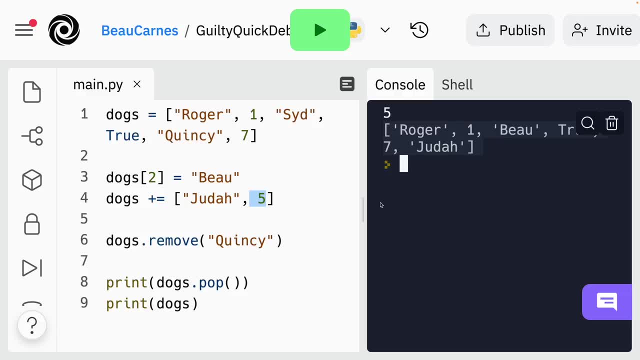 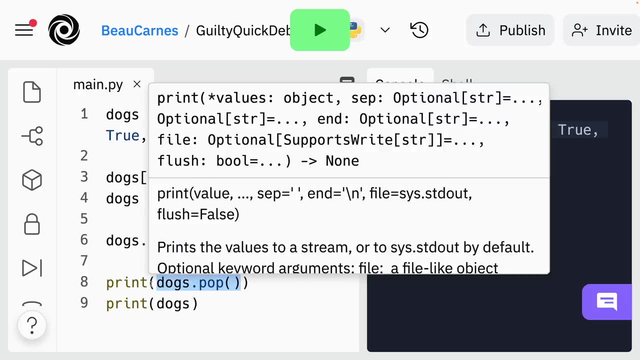 we added on to the list And now when I print the list, that items on the list. so pop is going to remove the last item from the list And it's going to return the last item. it's going to return and remove the last item from. 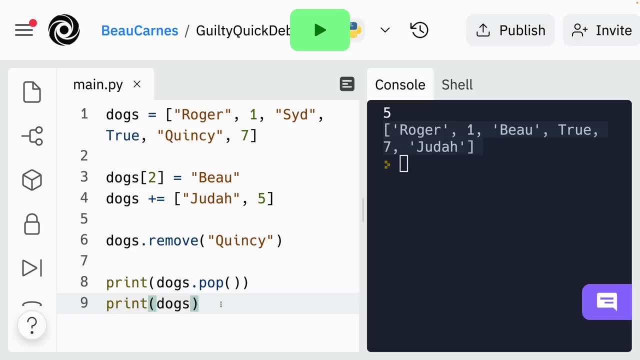 the list and then it's not on the list anymore. Now let's make this, let's let's simplify this. just go back to the initial list And I'm going to change this to items. Now I'm going to show you how to add an item in the middle of a list at a specific index. you can use the insert method. 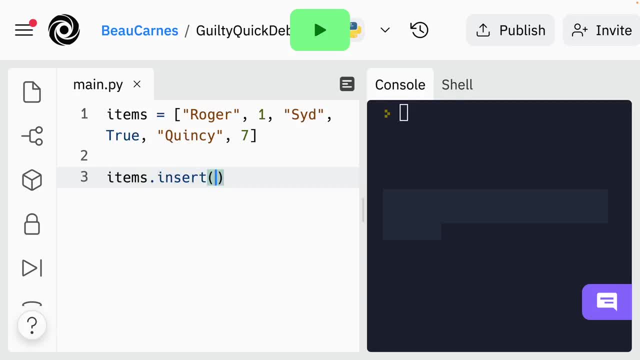 So I'm gonna do items dot insert, I'm going to put the index which is going to we're going to insert at the index number two and the item is going to be test And then I'm just going to print that, print items, And then I'll run that And then we can see index number two. we now see the item. 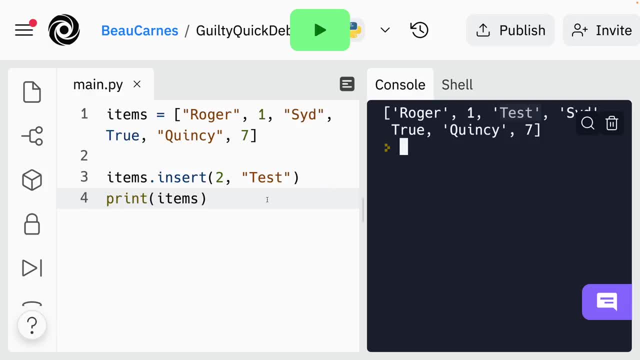 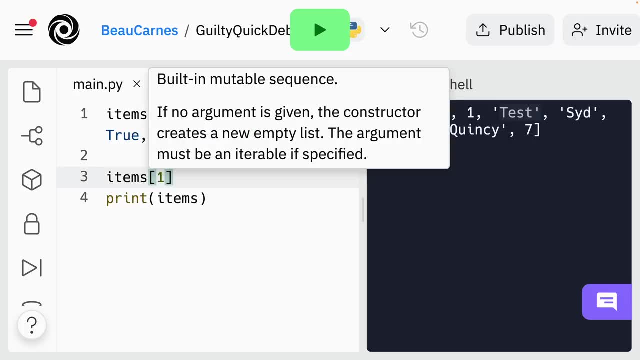 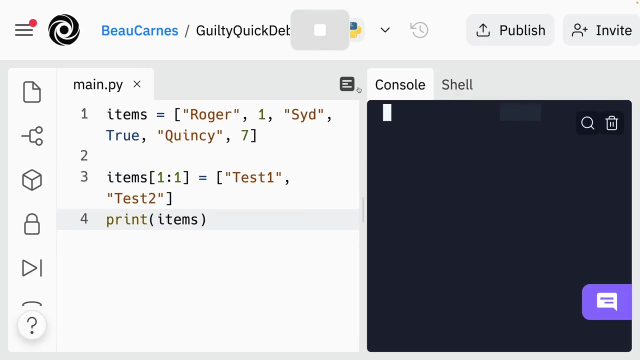 test Now, to add multiple items at a specific index, you need to use slices. So let me show you how you would do that. So we're going to do a slice And then the set that equal to test one test To reprint that. So now you can see we have test one and test two right here. 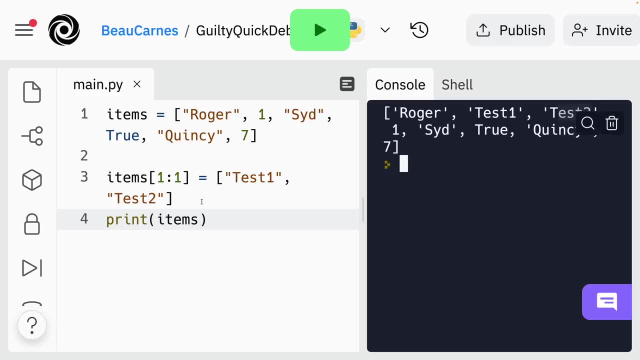 right behind this search thing here And we've entered multiple items And the list starting at index one. Now you can also sort a list. So if I do, here we go items dot sort. it will sort the list, But you have to make sure. Okay, we have an error. it's not supported. 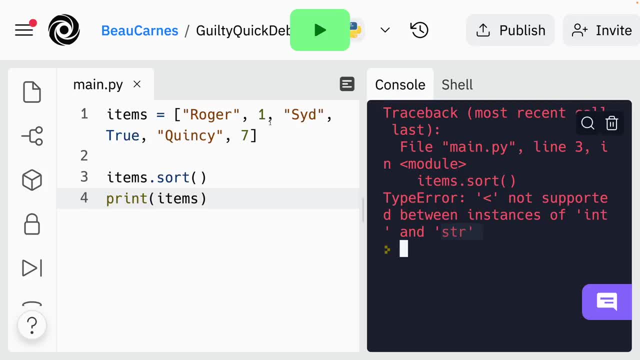 between, and we have a combination of ints and strings, So let's make it so it's all strings in the list, And then it should be able to sort it. Okay. now the strings are in alphabetical order, And if we're using integers or floats and they would just be in numerical order, Now one 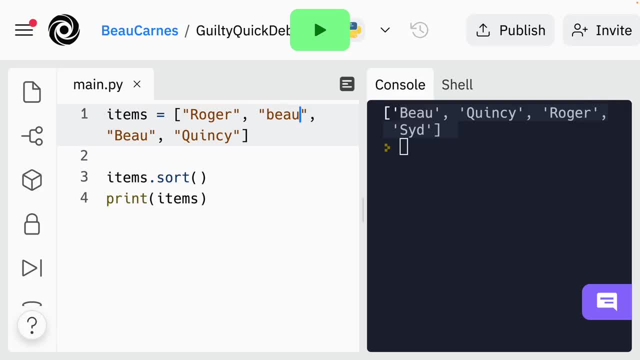 thing that's interesting about that. if I put change this to bow, you'll see now we have this at the beginning and this at the end of the list. So if I put this at the beginning and this at the beginning and this at the end of the list and this at the end of the list and this at the 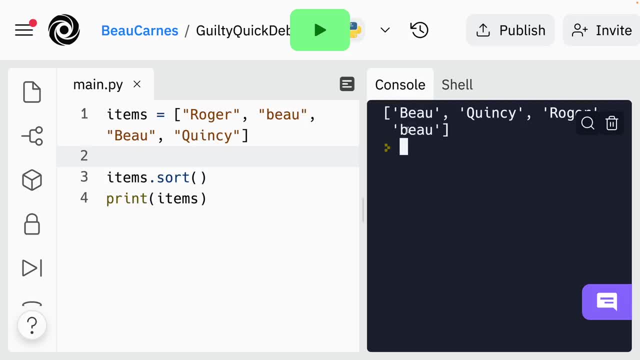 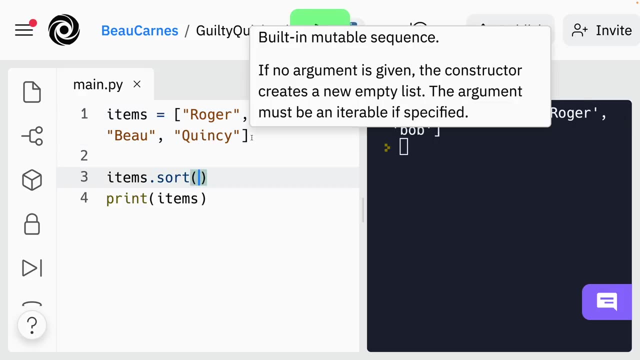 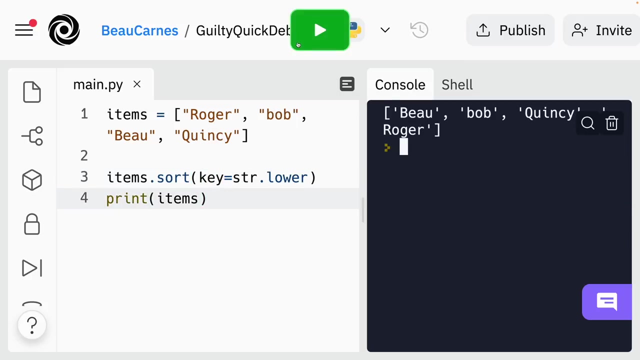 end. So a sort method orders uppercase letters first and then lowercase letters. So to fix that, actually to make it make more sense, we're going to change that to Bob And to fix that within the sort I'm going to, I'm going to put key equals str, dot, lower. And now 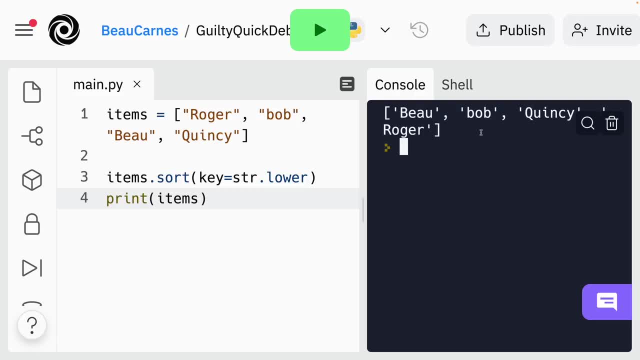 it's going to sort these correctly how you would imagine, not caring about uppercase or lowercase letters. Sorting modifies the original list content, So to avoid that, you can copy the list content using. So let me show you if we do items, items copy equals items and then we make a slice with with nothing at the 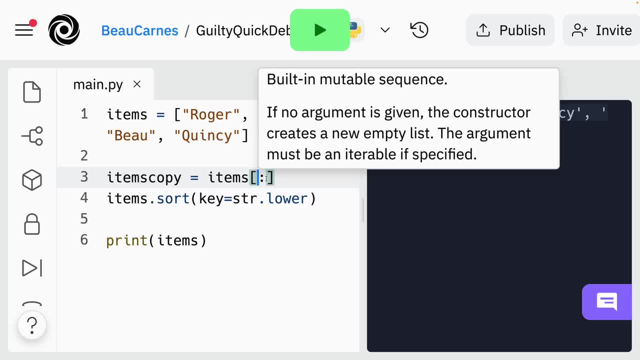 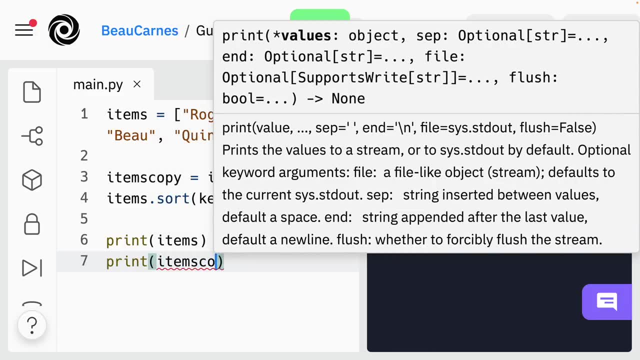 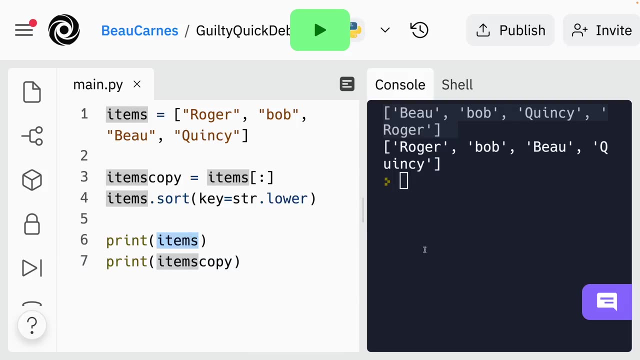 beginning and nothing at the end. So it's gonna start at the beginning of the list to the end of the list And now we can have a copy and I can print items copy So if I print that. so now we see we have the sort of list that we ran the sort on, but we also still have 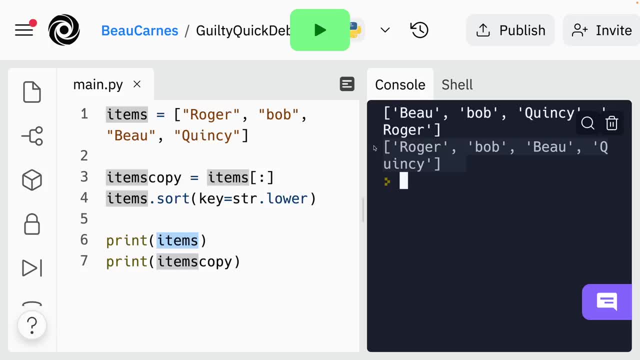 the original list, So with all the words in the original order. And there is also a way to sort a list without returning a new list. There's also a way to sort a list without modifying the original list. So, instead of copying a list, what I'm going to do is items. 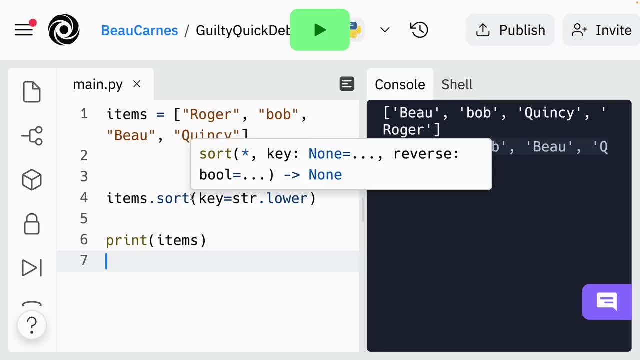 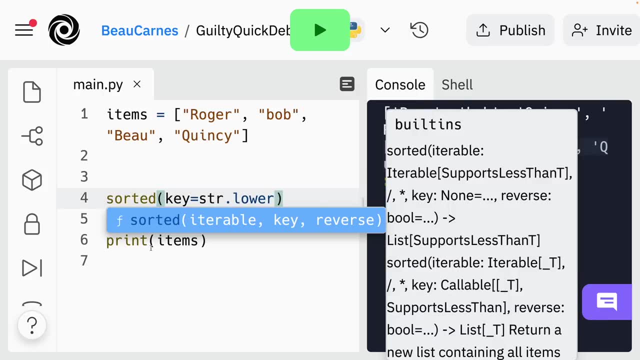 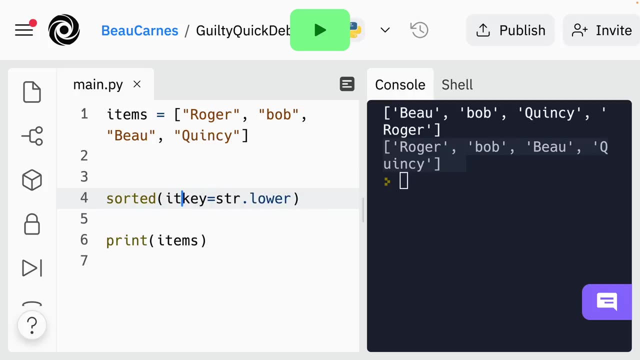 that instead of doing items that sort we are going to do we're going to use a global function called sorted. So in the sorted function we are going to pass in two parameters. So first is the list items And the second is how we're sorting it. So this just makes sure that the key- the case of the 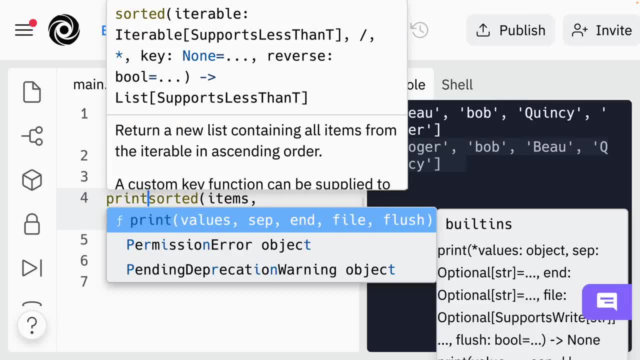 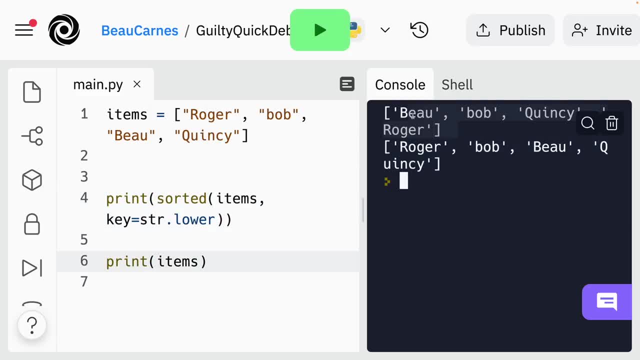 letters don't matter, And then I'm just going to print that. Now, if I run this, you can see we, we print, printed the sorted list And now we're printing the list And it's not. it's no longer sorted, because this create a new. 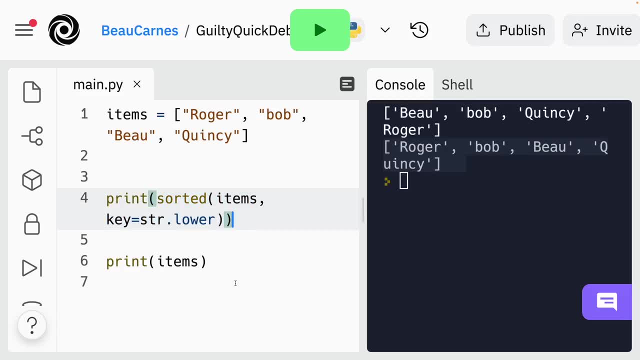 list without modifying the original list. Okay, now let's learn about another data structure called tuples. So this time I'm going to put tuples, So we're using a comment here. So tuples are another fundamental Python data structure. They allow you to create immutable groups of objects. 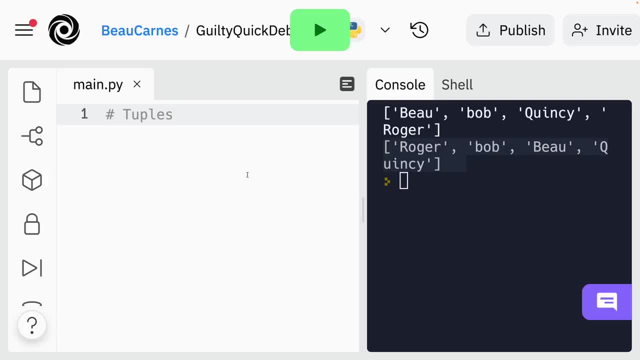 this means that once a tuple is created it cannot be modified. So we already saw that we can modify lists, but tuple you can't even add or remove items. They're created in a way similar to lists, but using parentheses instead of square brackets. So, for instance, I'm gonna do names. 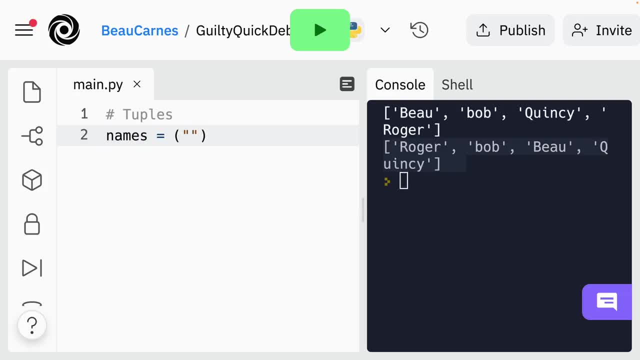 equals. instead of using square brackets, we're gonna do parentheses. Roger and Sid. Okay, so a tuple is ordered like a list So you can get it to values by referencing an index. an index So I could say, for instance, names, And if I do the. 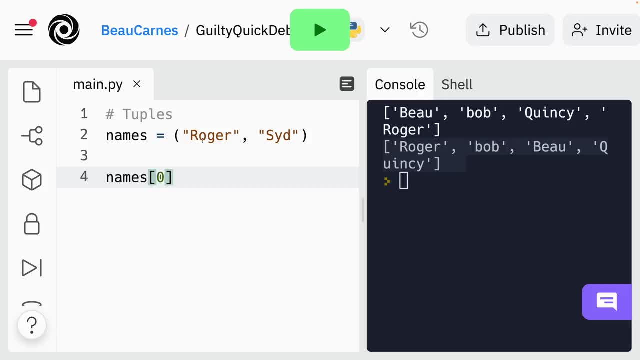 bracket. I could put a zero here to return Roger, And then you can also use index method, for instance names dot index, And then I can pass in something like Roger, and then this is going to return zero Because it's going to get the, the index number of that. So, as with strings and lists, 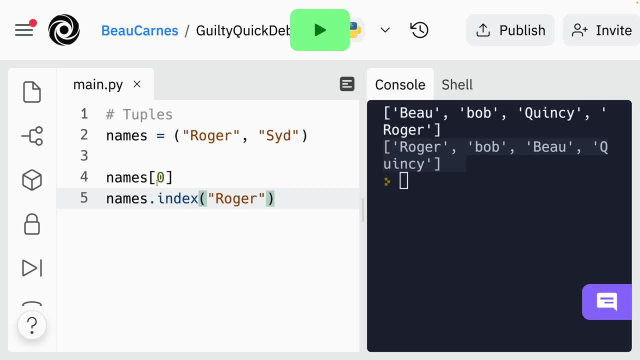 using a negative index, we'll start searching from the end. So I could do that. I can do negative one to start, not negative, zero, negative one to start searching from the end here, And you can count the items in a tuple with the length function. So I could do, if I do, length. 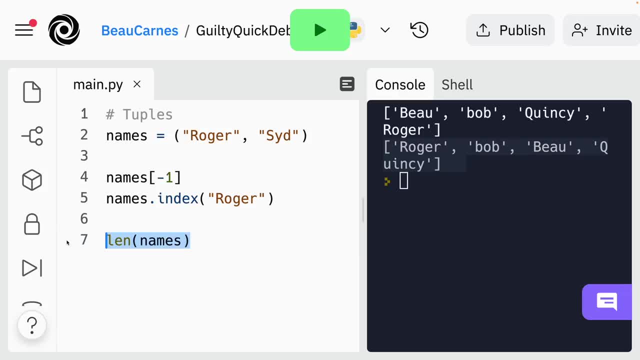 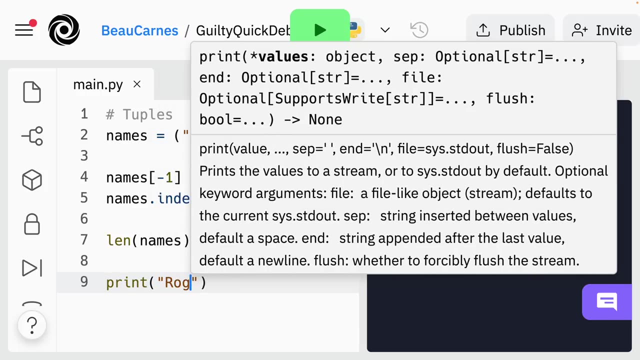 and then do names. it's if I printed that it would just print two, because there are two items in that tuple. Then you can also check if an item is contained in a tuple with the in operators very similar to a list. So I can do this time. I will print it. I'll do print Roger in names. So if 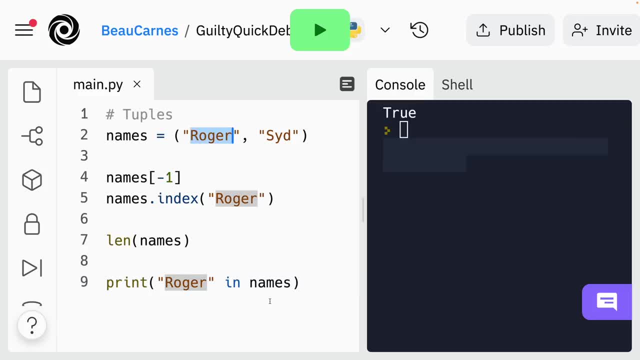 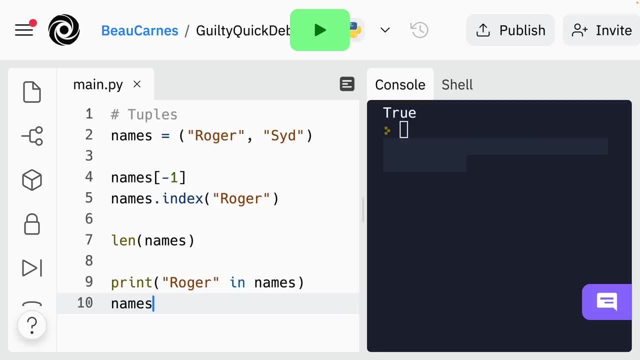 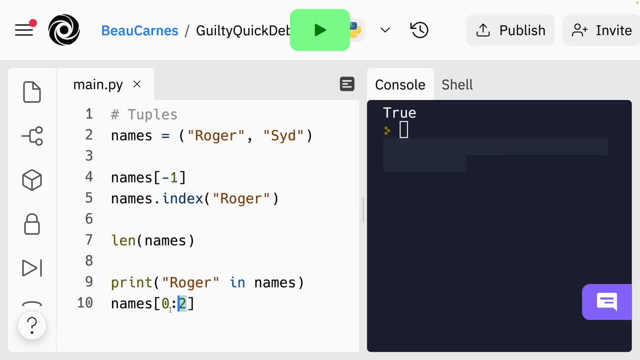 sorted version of the tuple using the sorted global function. So remember, when we were looking at lists, when we use the sorted function, it created a new, a new list, or so when we're creating that using the sorted function for tuples, it creates a new tuple. So 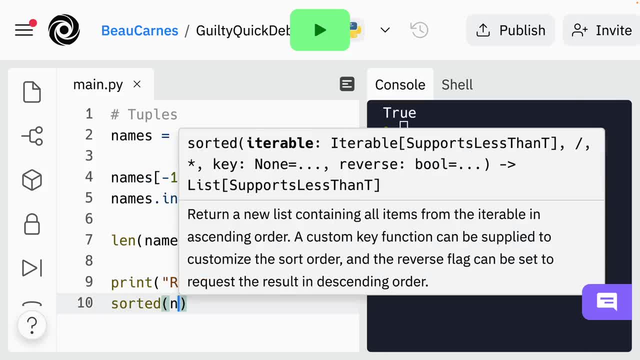 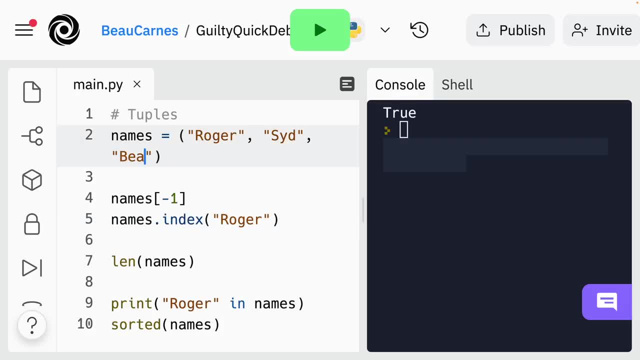 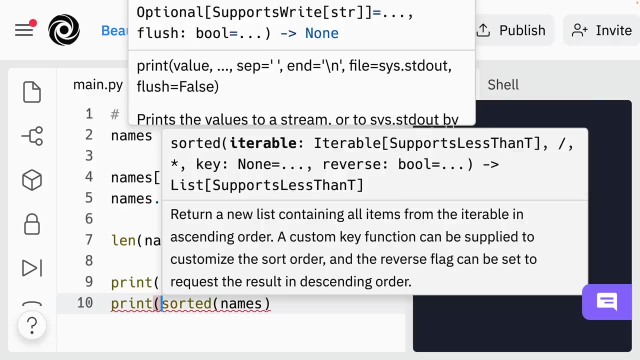 I can say sorted names And this would put them in alphabetical order. they already in our enough book order, but say there was one more word in this list And then I can print this to print the sorted version, but it's not actually going to modify the list, because you cannot modify. 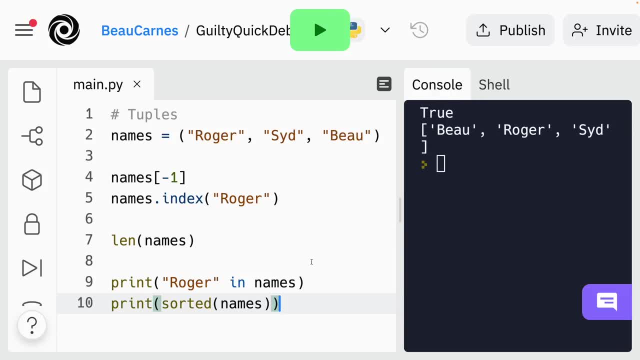 it, But you can modify the list. So you can modify the list. So you can modify the list, So you can modify a couple, And then you can create a new tuple from existing tuples using the plus operator. So I could say something like new tuple equals names, and then I can use the plus operator. 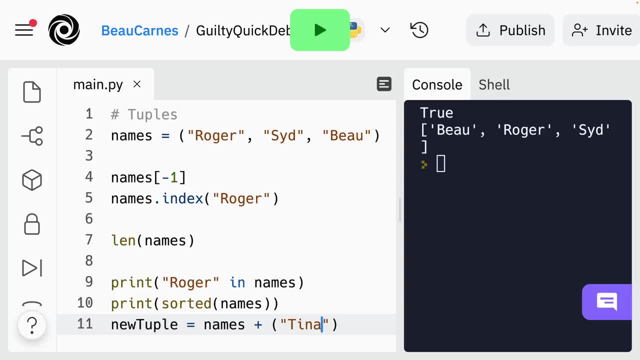 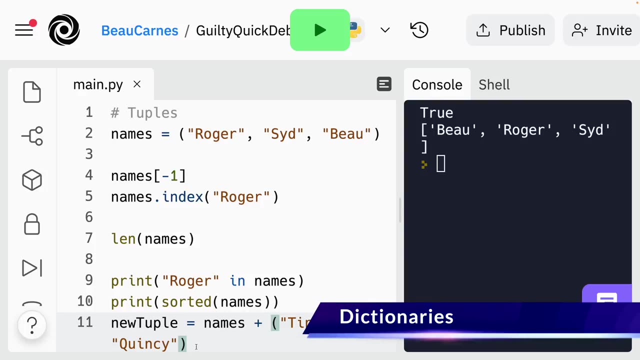 And then I would say I would just say: Tina and Quincy, I could add a few, I could add, so these will combine two tuples into a new tuple, But you can never, like I said, you can't actually modify the original tuple. Now let's learn about dictionaries, Dictionaries. 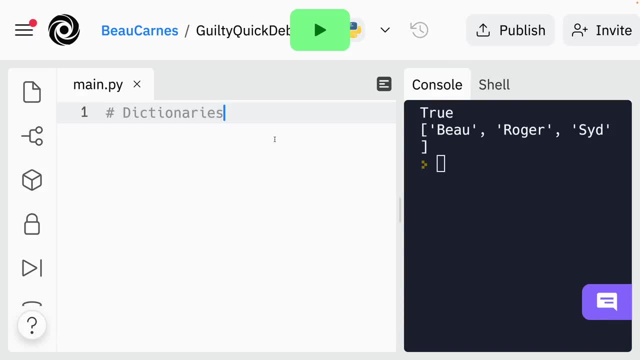 are another very important Python data structure. While lists allow you to create collections of values, dictionaries allow you to create key value pairs. We already discussed dictionaries a little bit, But now we're going to discuss even more about dictionaries, So let me give you an 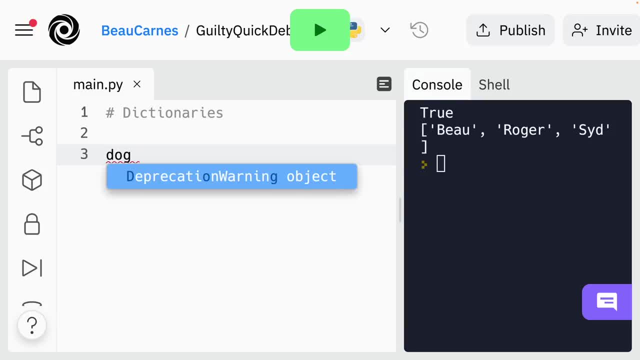 example of a dictionary with just one key value pair, So dog equals. and then you were going to use the curly braces to create the dictionary And I'll put name, And then I will put Roger, And, just like any type of strings, we could make these single quotes or they could be double quotes. 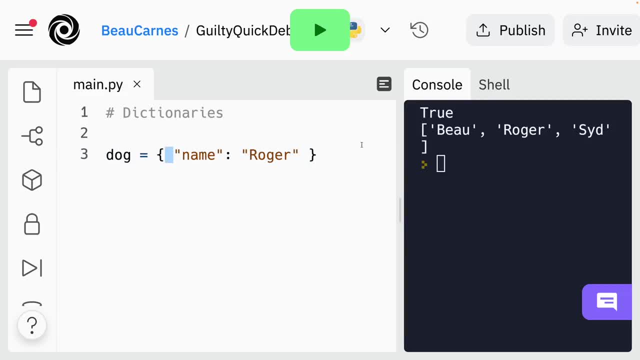 And the spaces here are not very important, But it's common to put spaces in between these things for better readability, And the key can be any immutable value. So this is the key, This is the value, And the key can be any immutable value. 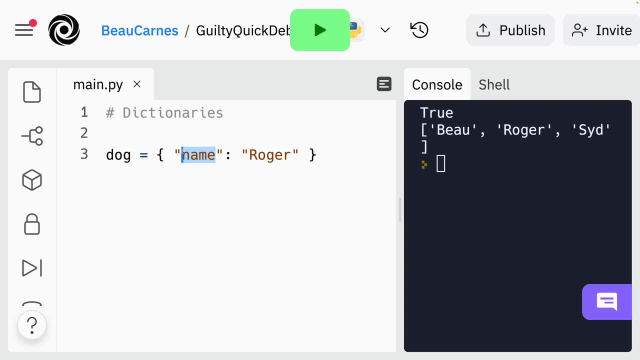 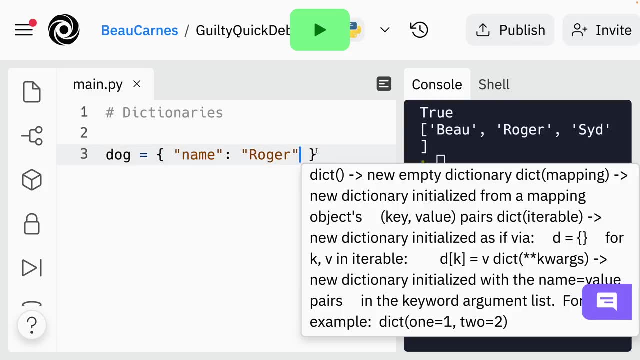 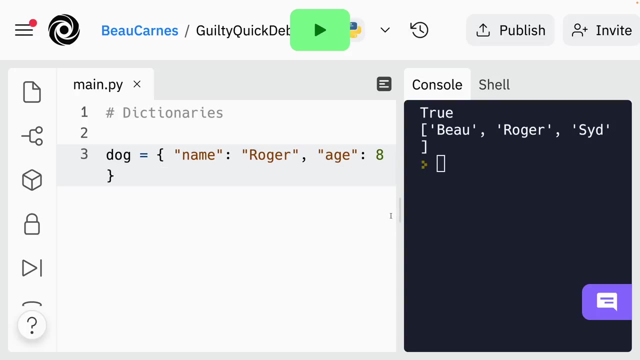 such as a string, a number or a tuple. the value can be anything you want. So a dictionary can contain multiple key value pairs, So like, for instance, we got the name, we can have age, and that's going to be eight, And you can access individual key values using the notation. 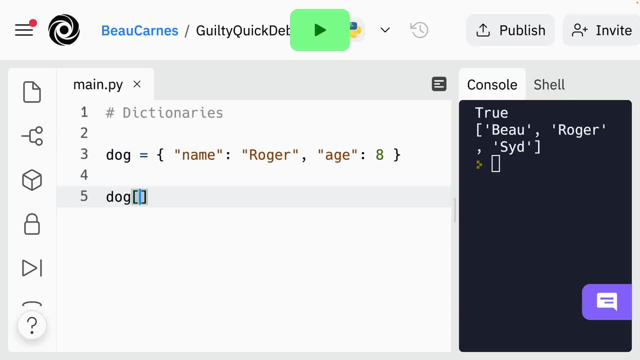 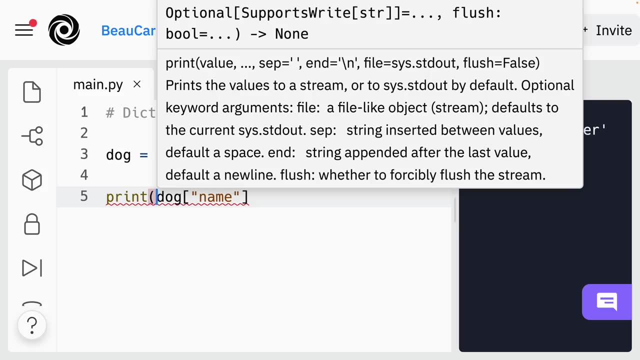 like this, So I can say dog. So I'm using the bracket notation. I can do name, So I print this. it's just going to print Roger, And then again I can use the single quotes too, if I want. 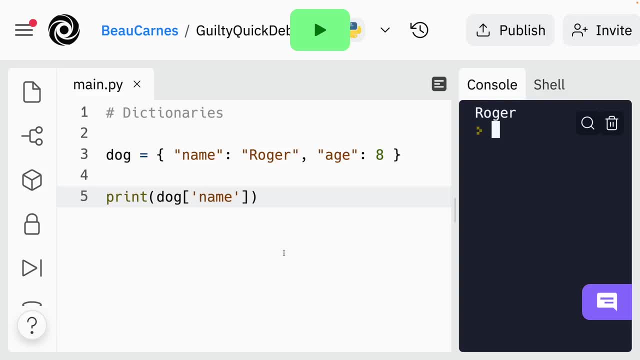 And it still prints Roger, And then you can use the same notation to change the value stored at a specific index. So let's say I want to change the name, So if I do, dog, and I'm going to say that the name is now going to equal Sid. Now, 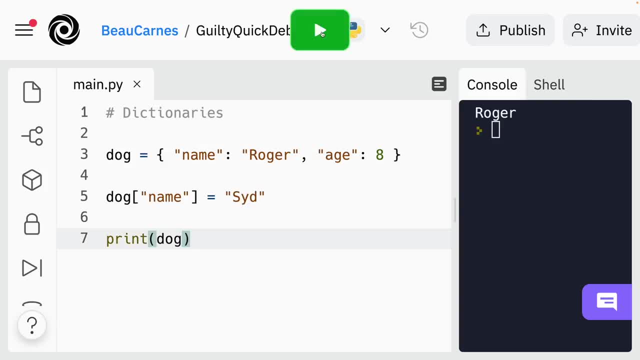 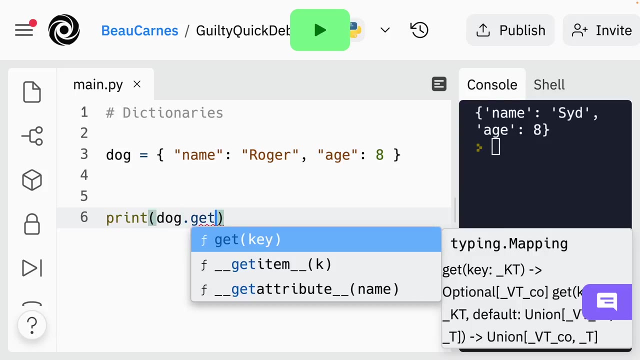 I'm just going to print the whole, the whole thing, And we can see the name is now Sid instead of Roger. So another way to get a specific element is to use the get method. So if I do a dog dot get and then I 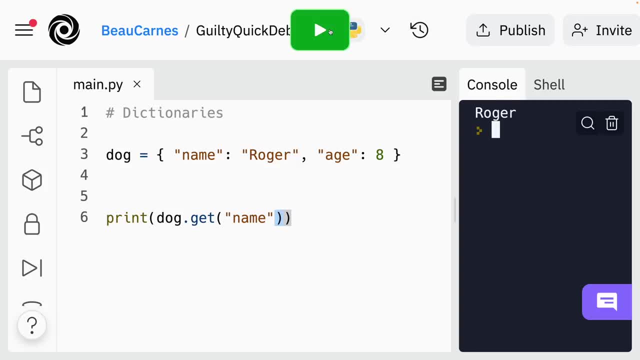 do name, so I'm going to try to get the name here. it's going to return Roger. So one good thing about this is that you can add a default value, Like, let's say I'm going, I'm searching for color And it's saying none. it's giving it none because there is no color. But what if I? 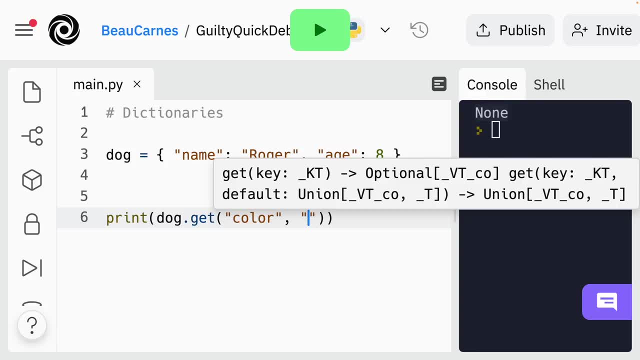 want a default value, so I'm going to put comma and then I'll put brown. So now, if it cannot find the color in the dictionary, it's going to return brown. But if it can find the color, like, let's. 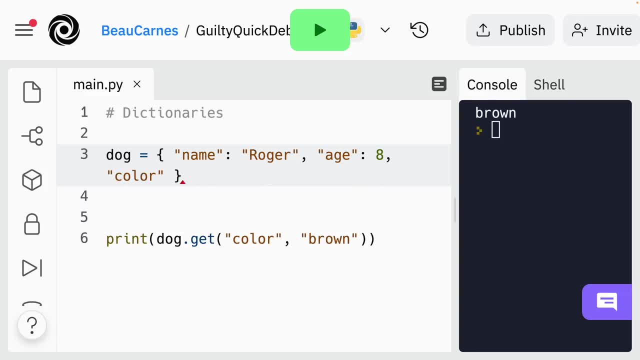 say color and this is a green dog, Okay, we'll return green. So with the bracket notation that was showing you earlier, you cannot have a default value. So that's one good thing about the get method. Now you can also use the pop method to retrieve the value of a key and delete the item. 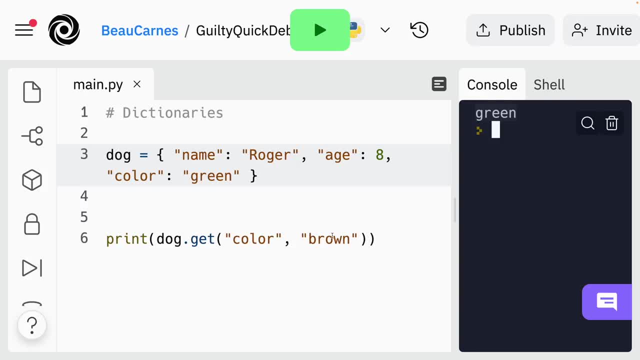 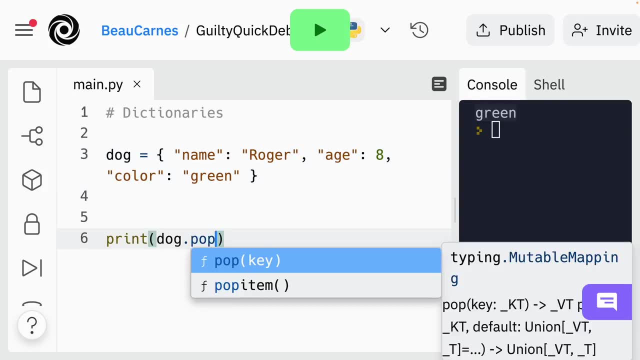 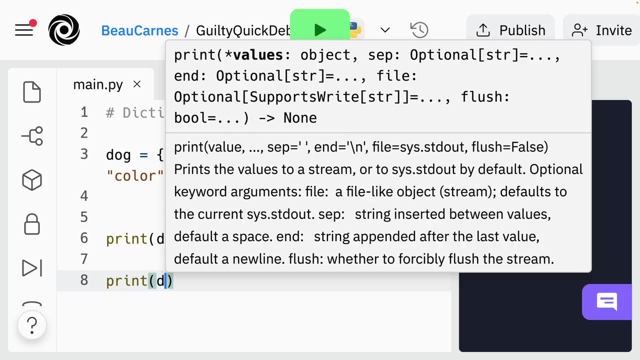 from the dictionary. Well, we also showed the pop method for lists. So for instance, I can say: get dot, pop, and then I will pass in name And then right after that I'm just going to print dog. that the whole dictionary. So first we're going to get Roger And then, when I print the 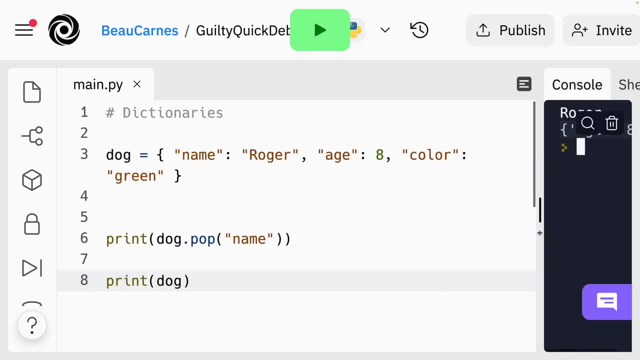 dictionary here. it's not going to show Roger anymore because we deleted it. pop will return the item and delete the item. Now you can also use a function or a method called pop item, the pop item method. well, let me show you that one pop item it's going to retrieve and remove. 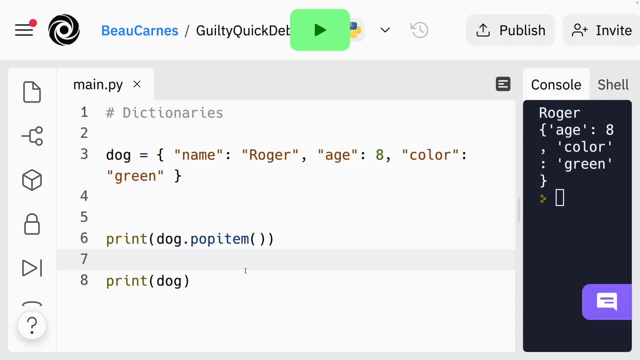 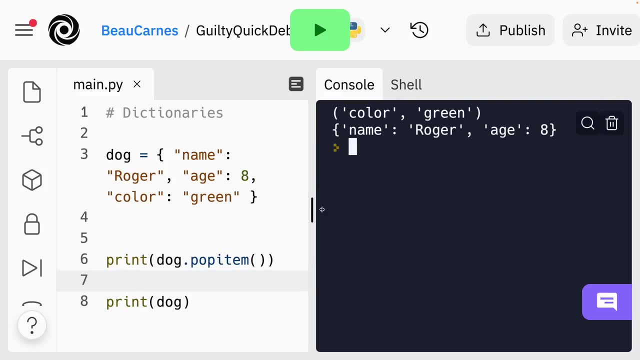 the last key value pair inserted into the dictionary. So in this case it should be color. So if I run this, it's going to return color green. And now when I print out the dictionary it's not going to show the value of the dictionary, But it's going to show the value of the dictionary. 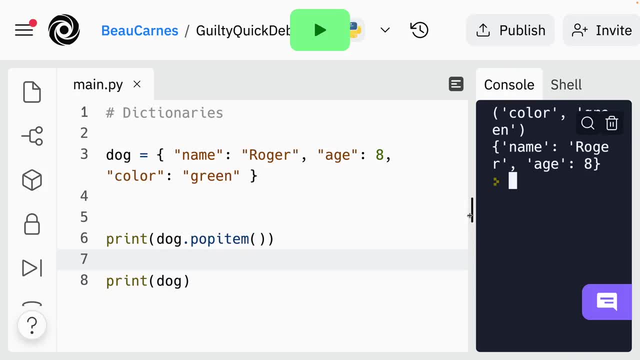 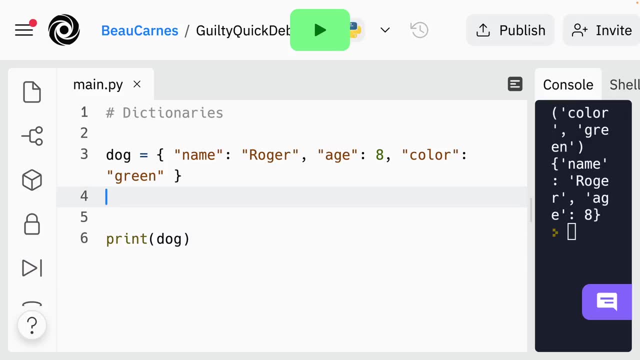 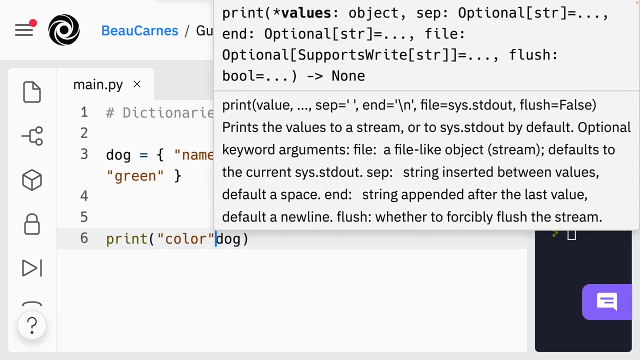 It's not going to show color green because that was already removed. it removed the last item. You can also check if a key is contained in a dictionary by using the in operator. So we're going to say we're going to try to find out if color is in dog, if there's a key called color. 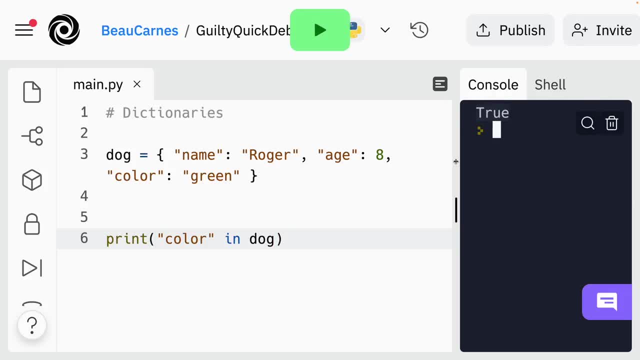 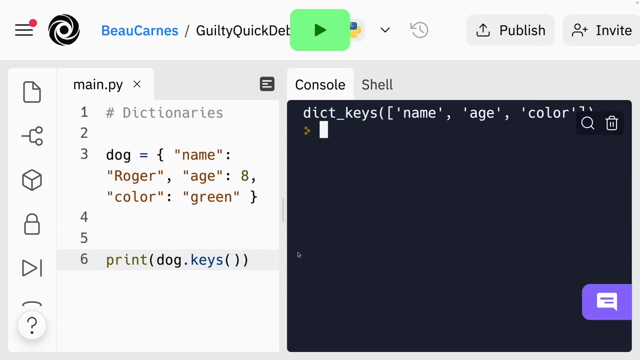 and dog. we run that and it says true. Another thing we can do is get a list with the keys in a dictionary Using the keys method. So if I do dog dot keys and then we'll run that, it's going to show the keys. So the keys are name, age and color. 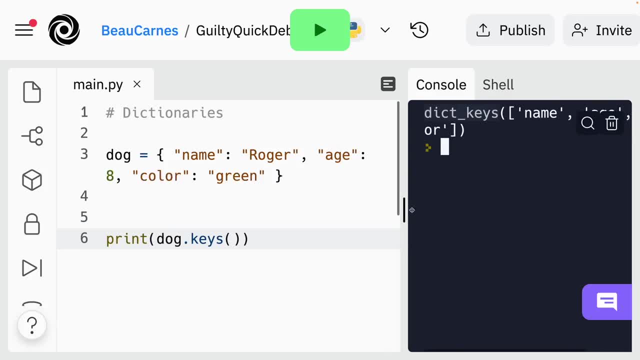 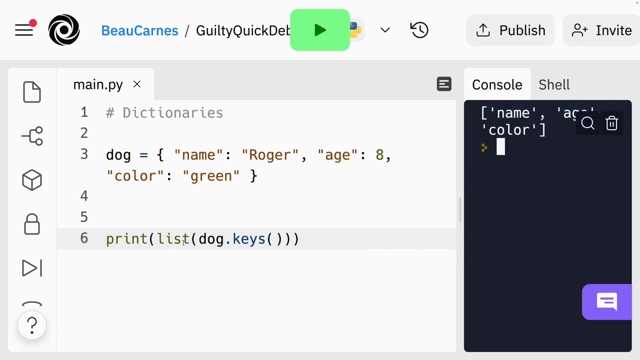 we can see that it's inside the single dick keys. But we can also pass this into list So we return an actual, just the list part. So now we can see it's just an actual list- name, age and color, And then we can do the same thing with values. So instead of dog dot keys let's do print dog dot. 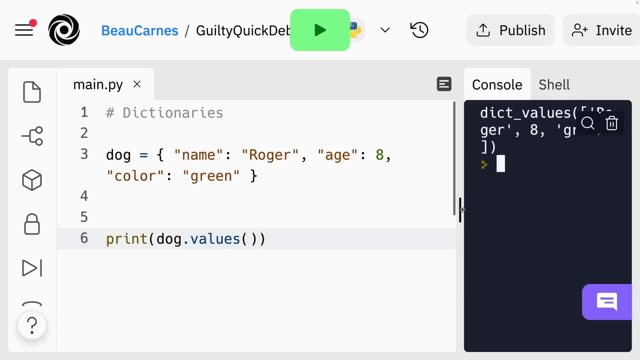 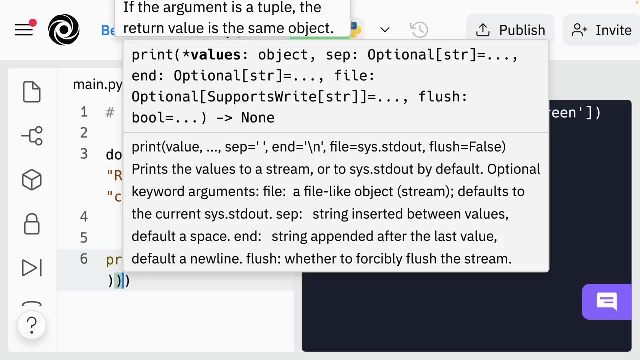 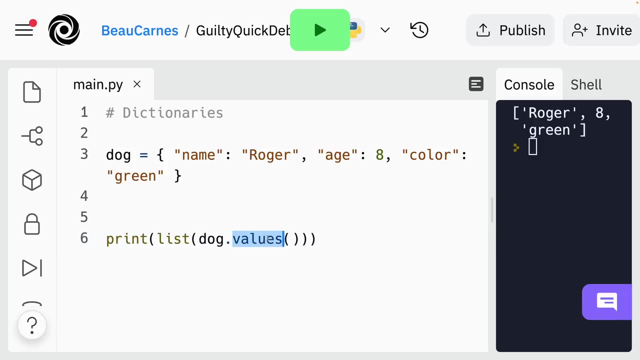 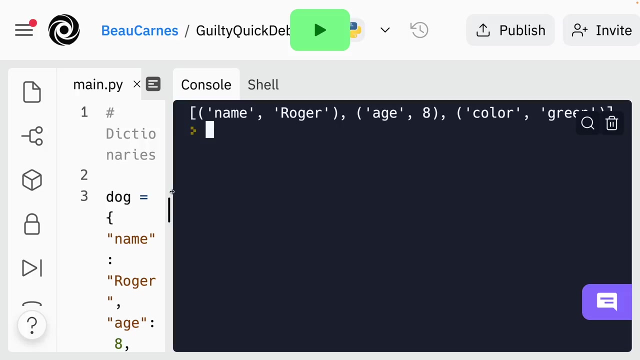 values, Print that And you can see we have Roger eight green. we can pass it into a list to return the, just the list here, Roger eight green. And then finally, if we just do items, it's going to return the items in the list or all the items in the dictionary and convert it into a list. So you 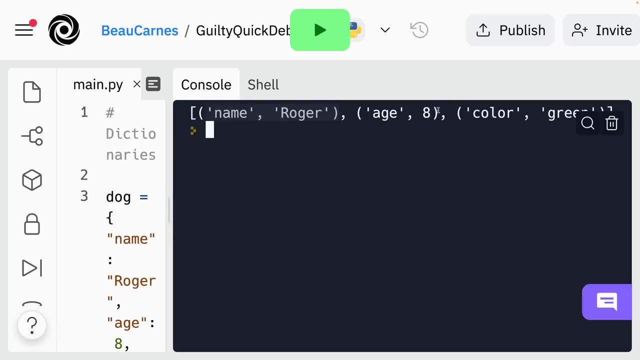 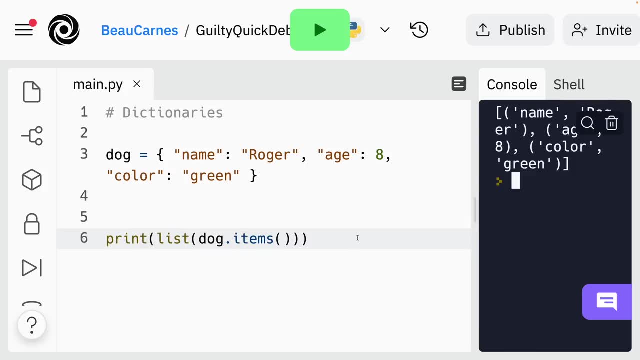 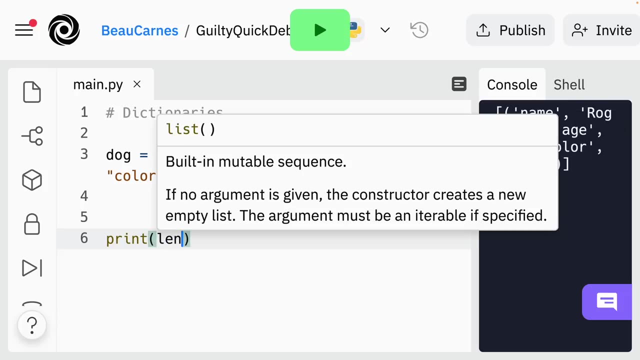 can see. this is the first item in the list, This is the second item, And then we have the third item here, So we can see each item of the list. each item of the dictionary is now in a list And then, like a lot of the other things, we can use the link function And I'll just put dog And we. 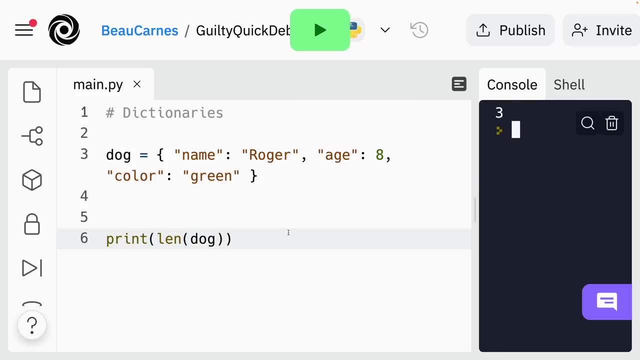 can see that there are three items in dog. Now you can also add a new key value pair to the dictionary. So let's say I want to do dog food, or it doesn't even have to be a single word, I could put favorite food. 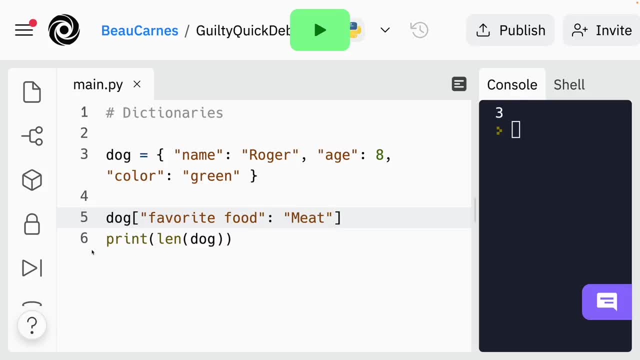 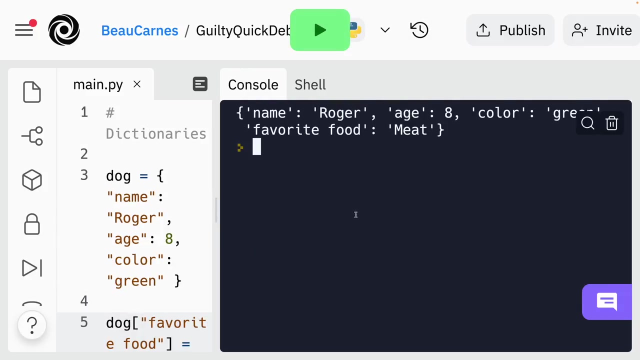 And I'm going to say meat, And now we're going to print that. Let's see what do we? Oh, this was supposed to. I did that a little wrong. There we go. This is actually how you do it. You put: use the bracket notation equals and let's put what equals there. Okay, now you can see. 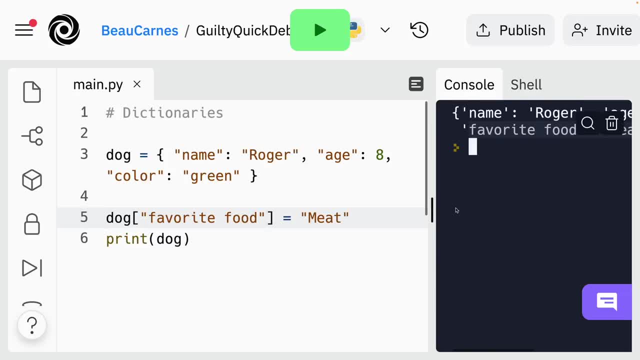 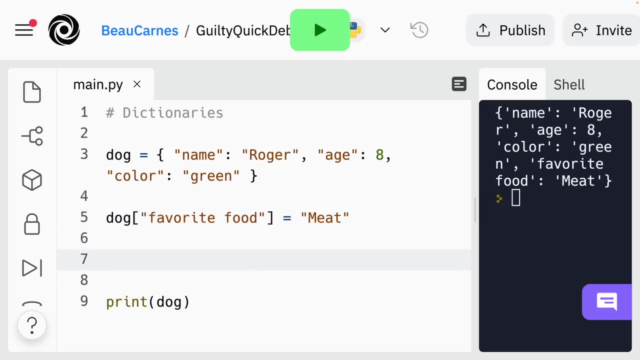 that we now have a new item on the list- favorite food meat. Then you can also delete an item from a list or delete a key value pair. So I'm going to- del means delete dog or dog. there we go, And this time I'm going to delete color And I'm just going to 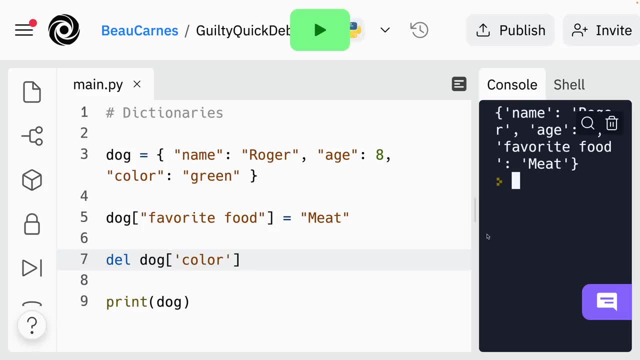 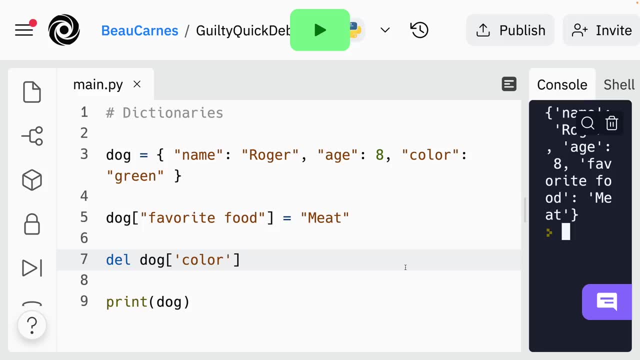 use single quotes instead of double quotes to show you that doesn't really matter the type of quote. And now you can see we don't know what color this dog is. it's no longer a green dog. And then you can also copy a dictionary. So if you want to make two copies of a dictionary, you can. 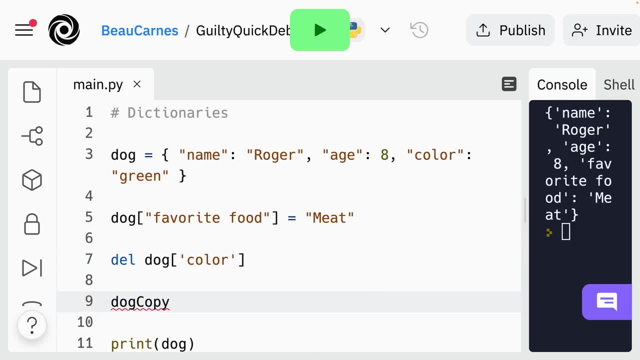 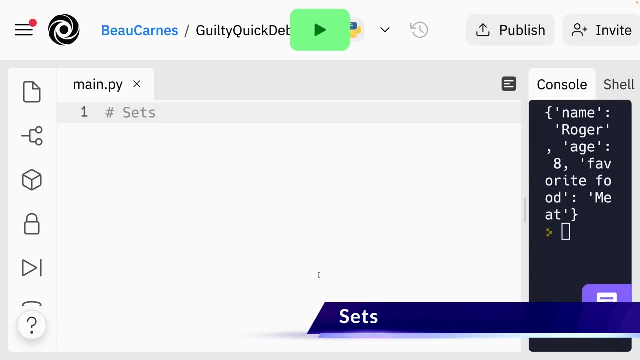 do do, like this, dog copy. That's the name of the new dictionary. I'll do dog dot copy And that would be the new copied version of the dictionary. Okay, now we are going to talk about a new thing called sets. sets are another important Python data structure. sets kind of work like couples. 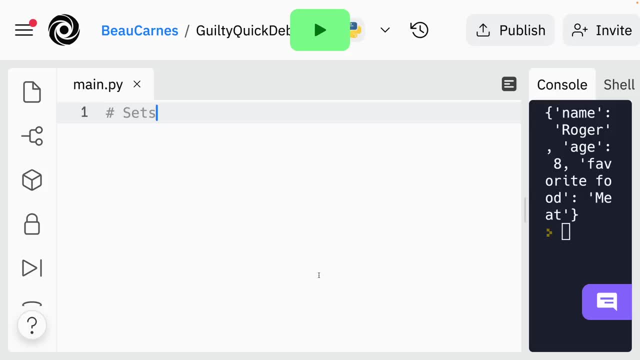 but they're not ordered And they are immutable, So you can change them. You can also say that they can work like dictionaries, but don't have keys. They're all. they have an immutable version of a set called a frozen set. So let me show you how you would create a set. So let's do names, And we're going to use curly. 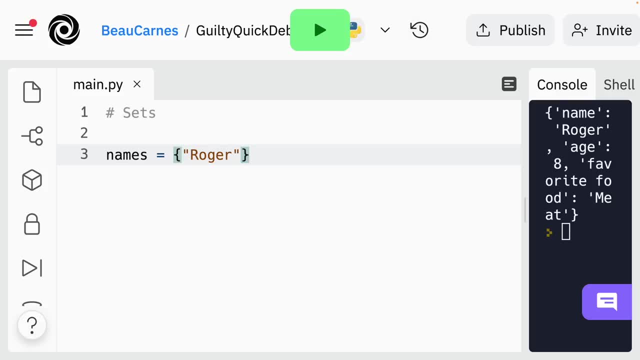 brackets, just like that And just like that. So we have two names. So you can see the differences. the dictionary: you use the curly brackets, but there's gonna be key value pairs, But this doesn't have key value pairs And a list, it's just going to be a item after item, like this, But there's. 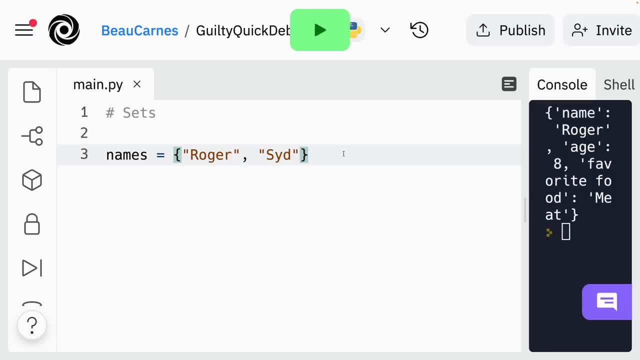 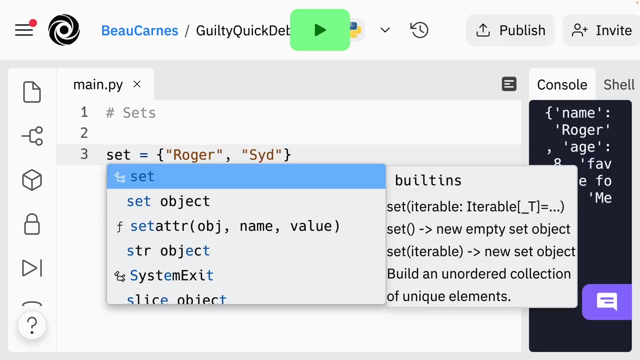 going to be brackets instead of curly braces. So one thing about the set is that they are not ordered. So sets work well when you think about them as mathematical sets. So, for instance, let's have- we're going to create a set, one with Roger and Sid, and we're going to have a set to which is just going to be a set one, And we're going to have a set two, which is just going to be a set one, And we're going to have a set two, which is just going to be a set one, And we're going to 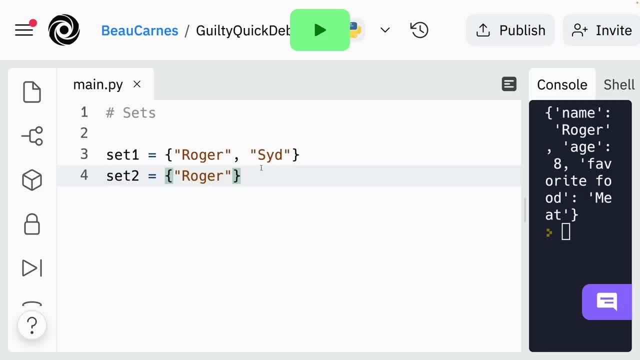 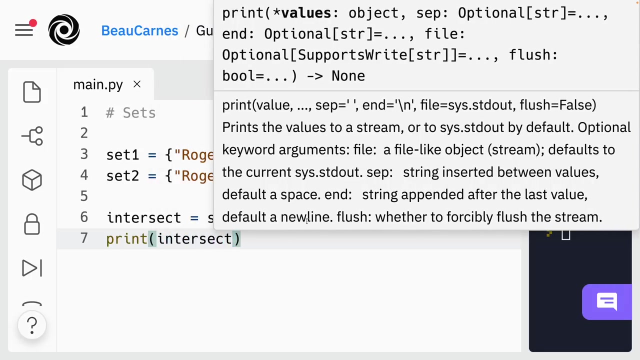 have Roger And so you can intersect two sets. So the inner intersect, the intersection of these two sets will be set one and set two. So if I just print that out, print intersect, and then we can just run that, we're gonna see what. so it's just Roger. So the intersection of these two sets are: 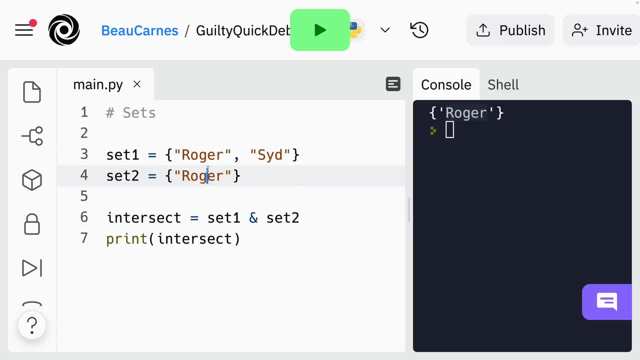 just Roger, And then we can just run that and we're gonna see what. so it's just Roger. So the intersection of these two sets are just Roger, The all the items that they have in common. you can also create a union of two sets, So instead of just calling this union, I'll put 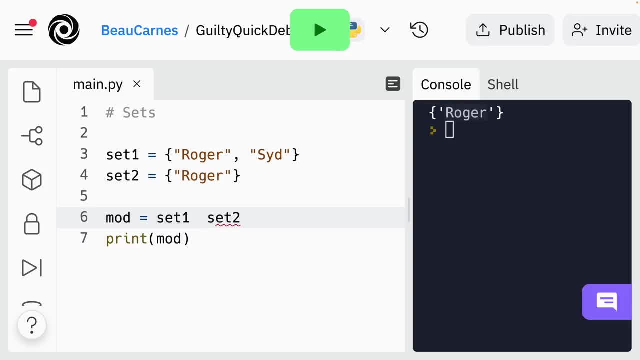 mod for modification And so I can show a few different things with the same variable name. And the union symbol is just the straight line, like this And I. it's just the straight line. It's on the same key as a as the. was it the forward slash, backslash, one of the slashes? 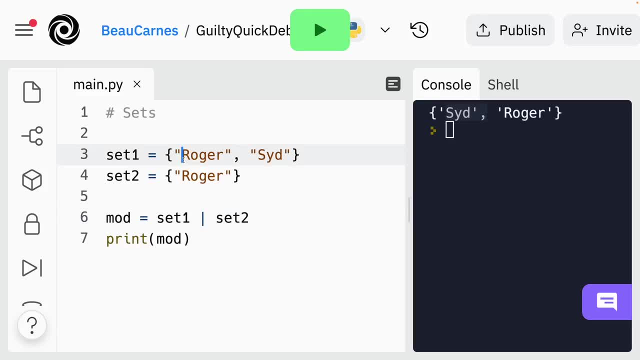 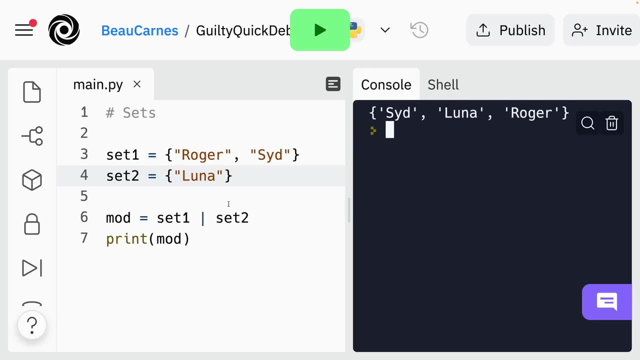 Now we're going to get every single item in both sets, which happens to be, in this case, just happened to be the same as set one. But if we change this one to the word Luna, just a different name, And now we're going to get each item in both sets. or said Luna, Roger for the intersection. 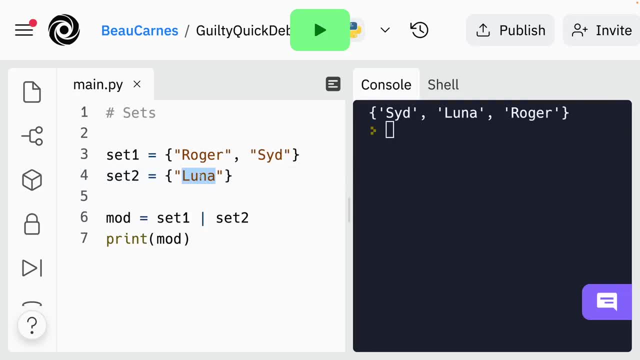 And then we can also get the differences, the difference between two sets. So let me change this to back to Roger, And for the difference between two sets I'll use a, the minus, and the difference is just going to be said. that's the only thing that's different between the two sets. 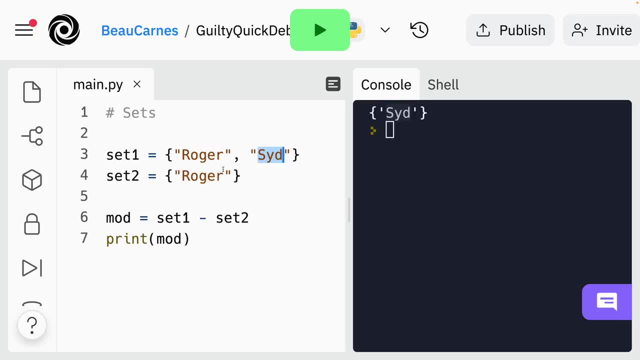 You can also check if a set is a superset of another and if a set is a subset of another. So how you would do that is. So we're just saying like: is this greater than that, which means it has everything of the other set? True, Now, if we put the other direction, is: does this set have? 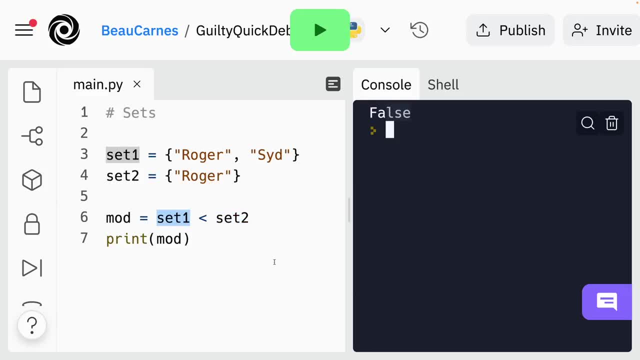 everything in this one? No, it doesn't. You can also count items in a set with the length function. that's pretty self explanatory. I won't even show it to you. We've seen the length function so many times. You can also get. you can also get a list from the items in a set by passing. 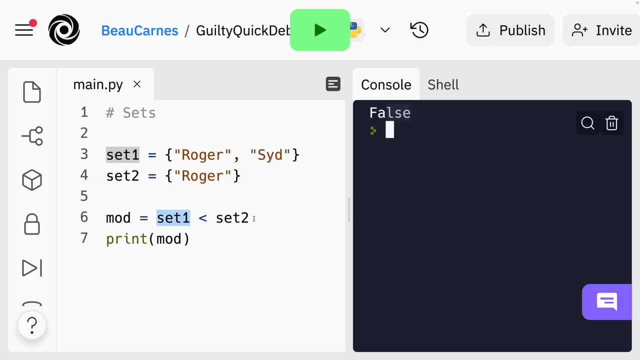 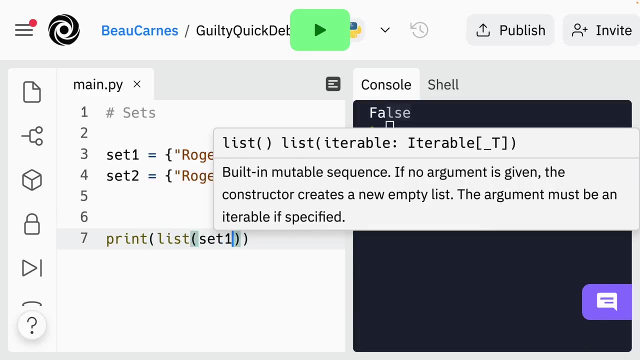 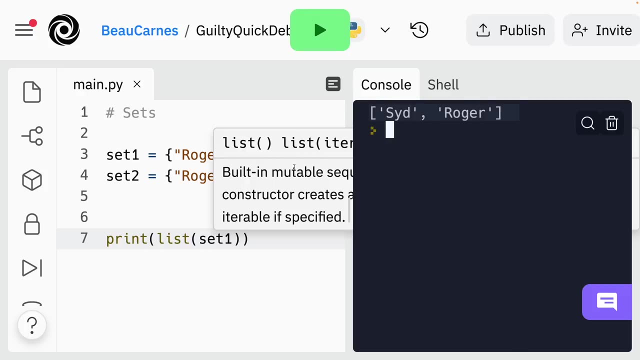 the set to the list constructor. So I'm just going to remove this And we will do list Set one. Okay, so now we have a list of the set And then you can check if an item is contained in a set with the in operator, just like the. 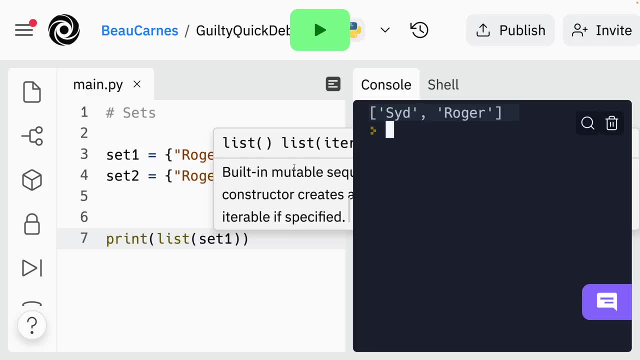 list and the other way we, the other places, we use the in operator. And then one more final thing about a set. a set cannot have two of the same item. So that's another thing that's useful about sets. So if I type in Rogers, now we have Roger said Roger. if I play this, we'll see it's only 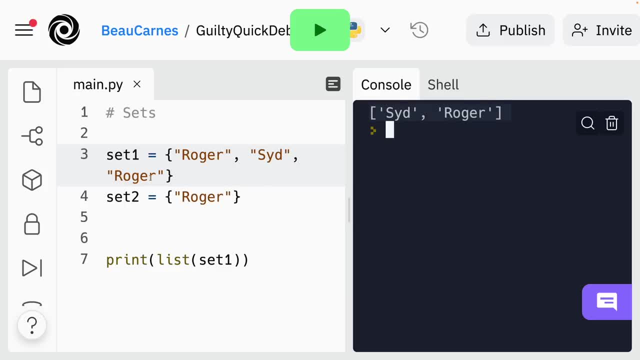 going to print Sid Roger. it's not going to add the Roger twice to the set, So that's. another useful thing about sets is that make sure there's only one of each item in the the set. So if you have a list that has multiple items, you can. 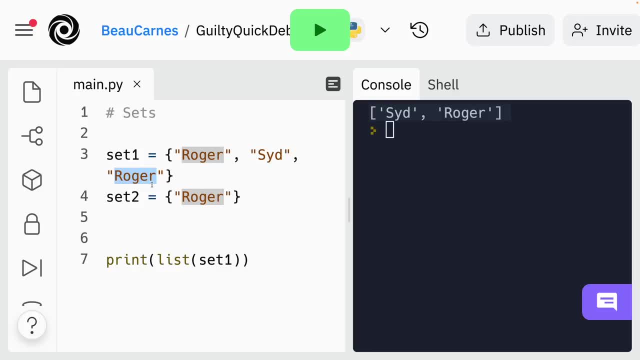 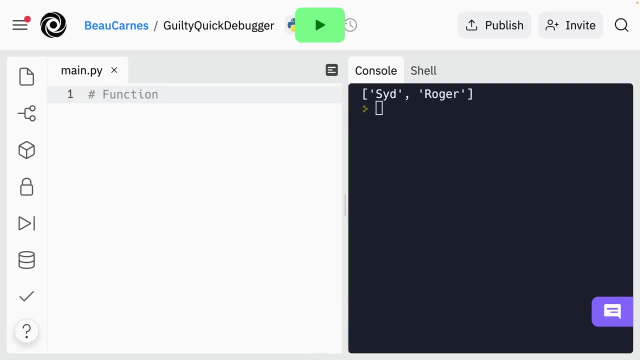 convert it to a set And then I'll just make sure there's only one of each thing in that set. Now let's talk more about functions. We already talked about functions in the last section, but we're going to do a review and then go into even more detail about functions. So a function. 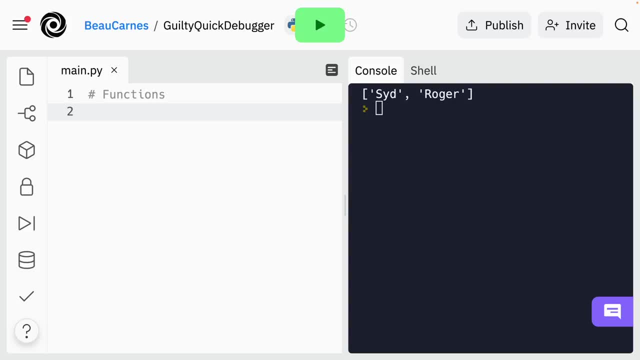 lets us create a set of instructions that we can run when needed, And I'm just going to paste in a function. And again, the indentation. it can be either four spaces, two spaces, as long as it's indented the exact same amount. So functions are essential in Python and in many 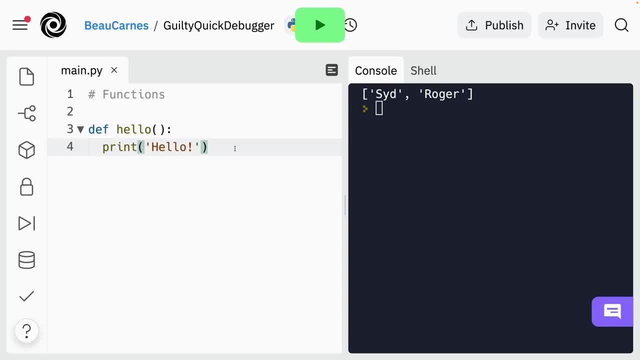 other programming languages. They help us create meaningful programs because they allow us to decompose a program into manageable parts And they promote readability and code reuse. So this one is a function called Hello that just prints Hello. this is the function definition. So there's a name called Hello. this is the name here and then the body. 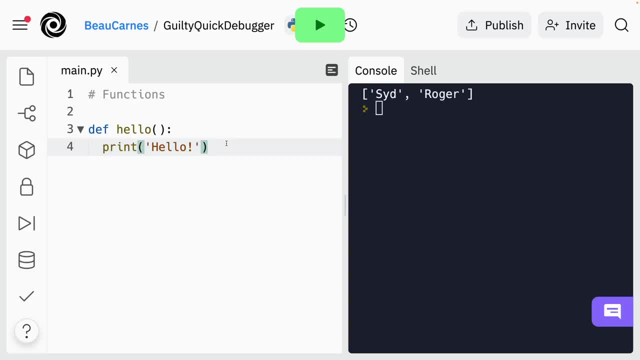 of the function, which is the set of instructions, And the body of the function is everything that's after the colon and everything that's indented one level on the right. So to run this function we must call it, so I can just type in, Hello, Hello, And then this is the syntax to call the: 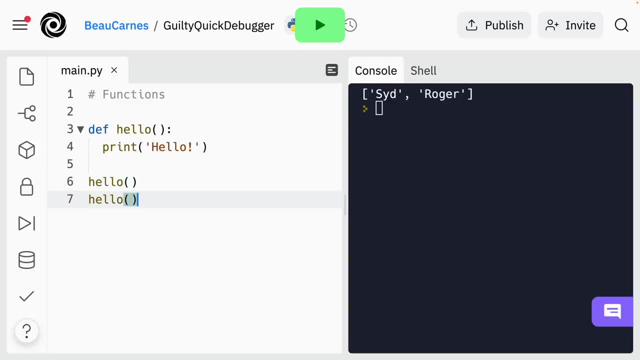 function And I can call it multiple times. So I can just copy this and paste it. And now if I just run this program, it's going to print Hello three times. the name of the function is very important. So the name of the function is Hello. it should be function. name should be descriptive. 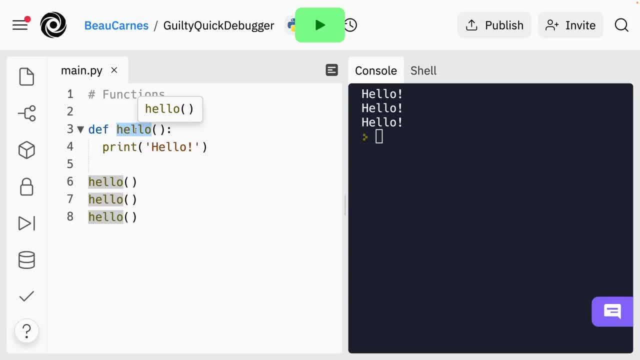 So anyone calling it can imagine what the function does. A function can accept one or more parameters. This is something else that we saw before, But I can type in a parameter right here And this becomes a variable that we can use in the function. So I can change this. instead of printing Hello, it's going to print Hello. 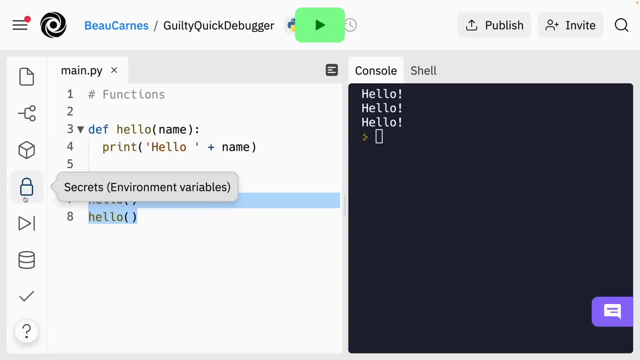 And then we'll just put name, And now I can call the function with the name And I can actually call it with different names. So we'll do bow and we'll do Quincy And then, if I just play that, we see Hello bow, Hello Quincy. 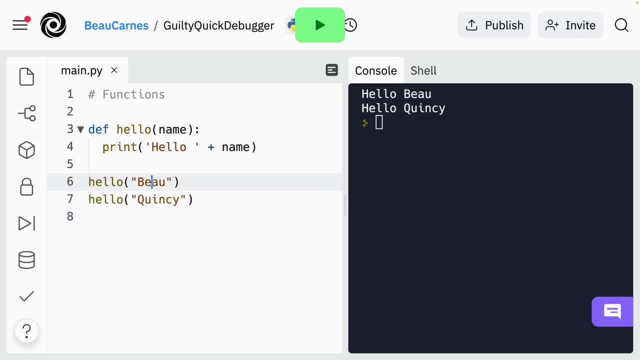 So, as you can see, we call the function by passing the argument, And again, you can use single quotes or double quotes. here It's better to be consistent: just always use single quotes or always use double quotes. But for teaching I like to switch it up to just to emphasize that. 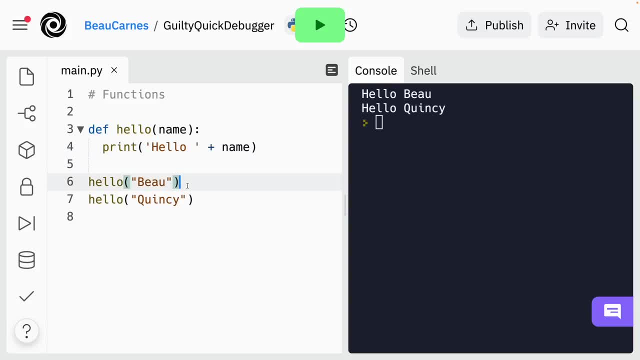 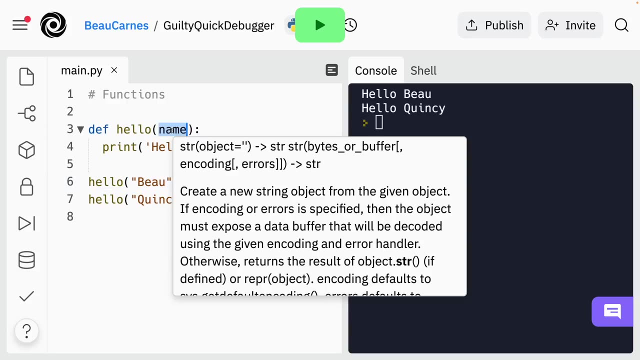 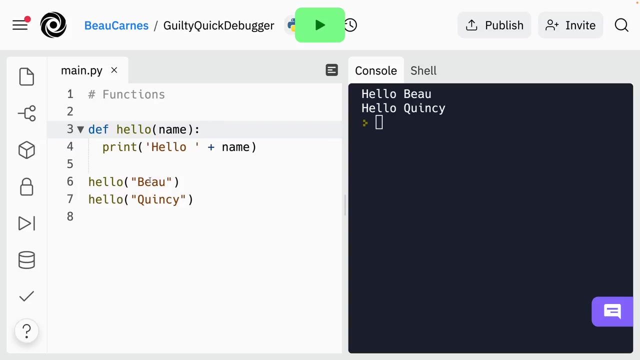 you can use either. So let me tell you about the difference between parameters And arguments. These two words, parameters and arguments, are sometimes used interchangeably And it's common to get confused about the distinction. we call parameters the values accepted by the function inside the function definition, And arguments are the values. 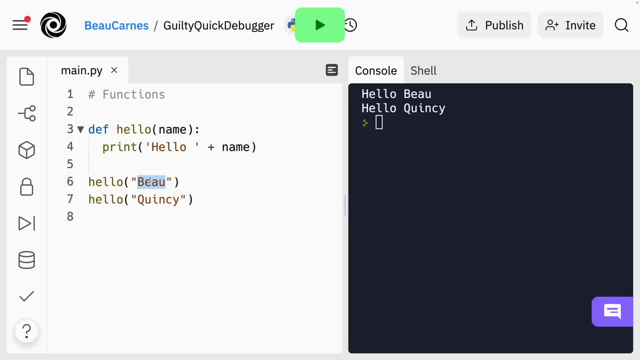 we pass to the function when we call it. Also, an argument can have a default value that's applied if the argument is not specified. So let me show you how I would do that. So we have a name. So right now always needs to be get a name. Well, first let me show you what would happen if I 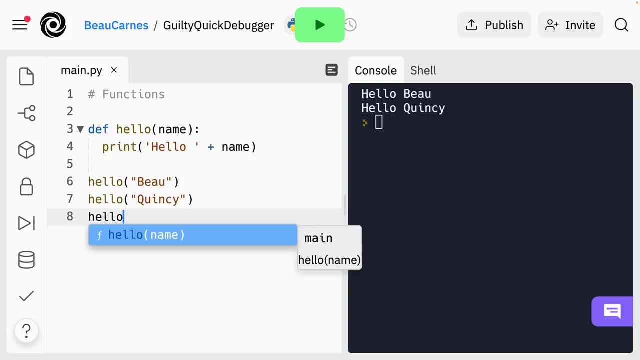 call the function without passing the name. I'm just going to run that And we can see we're going to get an error. Hello, missing one required positional argument name. But we can make it so you can call this function without passing a name where it's optional. you can, if you want. 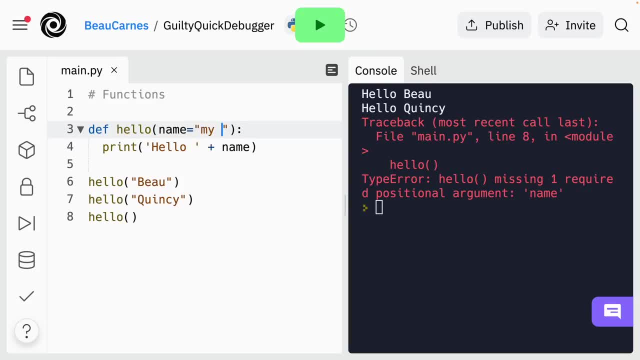 I'm going to put an equal sign and then I'm going to type in my friend And just to make consistent, make this consistent, I'm going to make this all double quotes. Okay, so this is now an optional argument, So it's, it's, you can pass in the name, But if 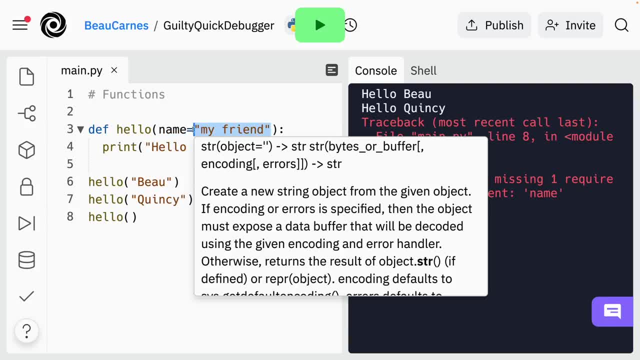 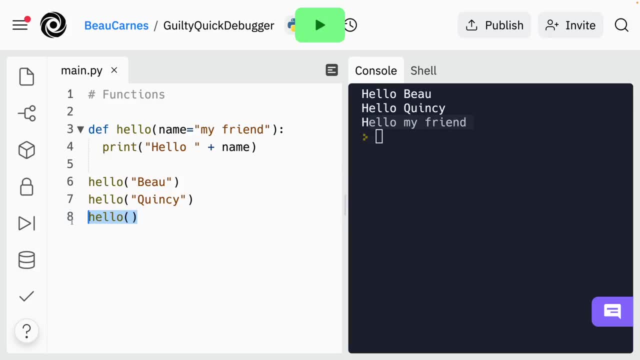 you don't pass a name, it's going to default to my friend. So I'll just run this again with that default value. And now it's Hello Bo, Hello Quincy, Hello my friend, Because we called this and we didn't specify any argument or parameter, And then we can also. 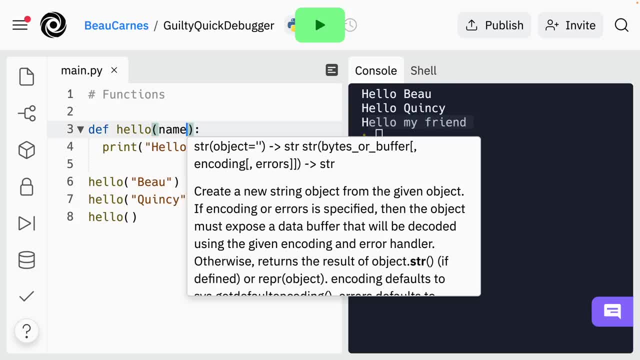 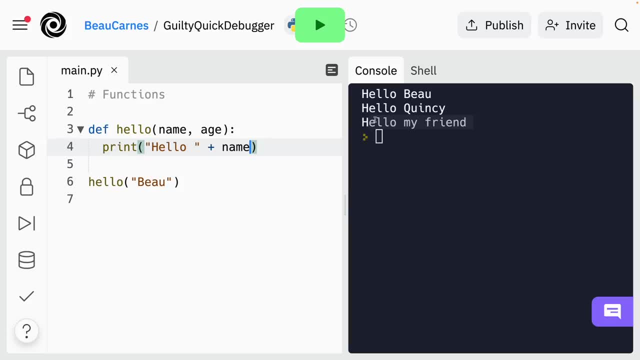 accept multiple parameters. So I'm just going to get rid of this default value And I'll put age. now we're accepting a name and an age, So we can now use both parameters in our function. So I can do plus: Hello, name, You are. 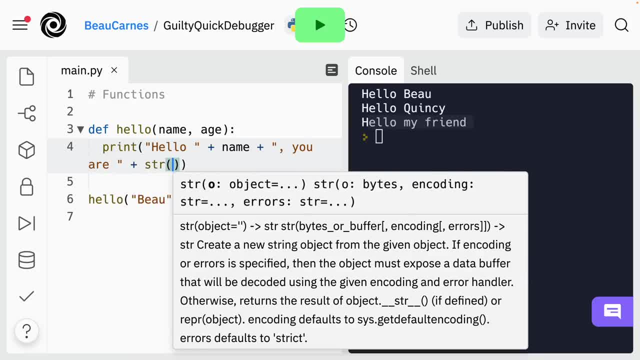 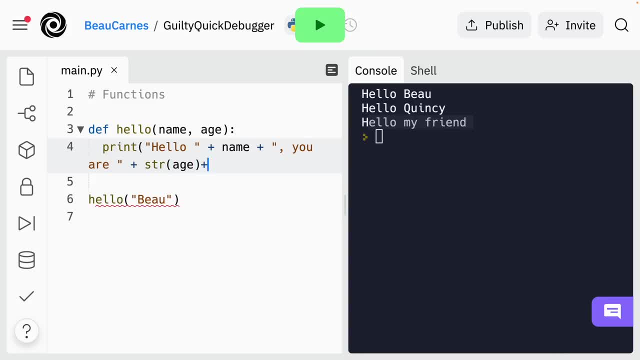 and we're going to add the age, And now it's going to be passed in as a number, but we're going to convert it to a string, So you are years old, And then we have to make sure, we have to make sure to add a space in here, So there'll. 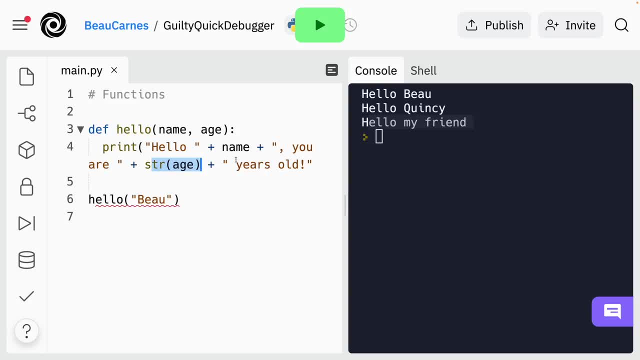 be a space, space after this word, then the number and a space and then years old. So I'm going to now have to pass in the number And now I can run this function Now showing the red squiggly lines. I sometimes the red squiggly lines will appear when it's actually correct. 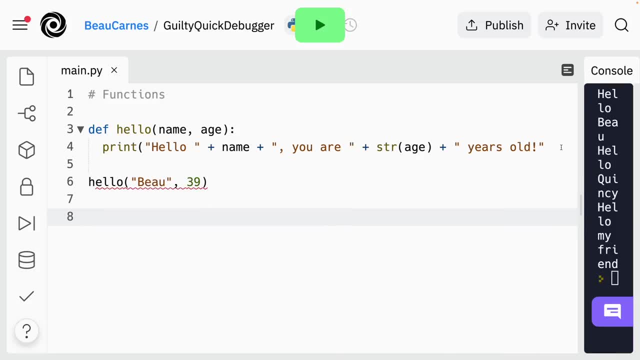 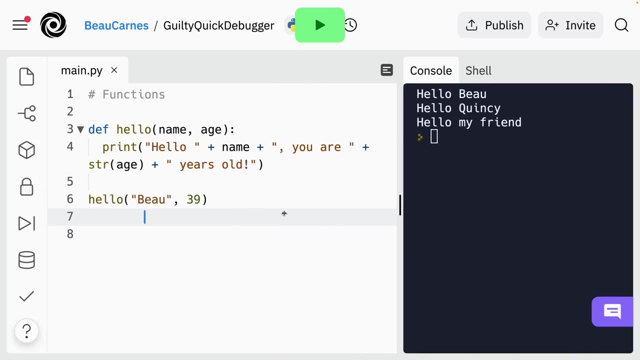 So let me, what am I? am I doing something wrong here? Oh, I need to put the parentheses. If the red squiggly lines appears when it's actually correct, it will go away, usually within a few seconds, or if you hit Enter. So that actually was a. 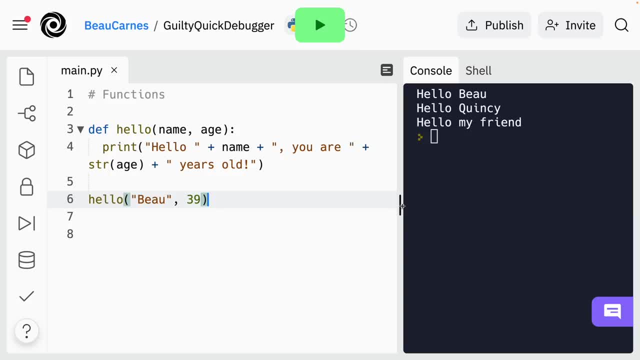 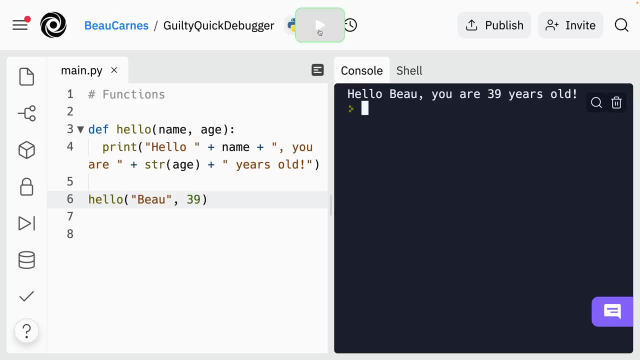 problem. I forgot the parentheses at the end. So you can see. this is what the whole function looks like If it's all on one line, but I'm just going to move that over. So, hello Bo, you are 39 years. 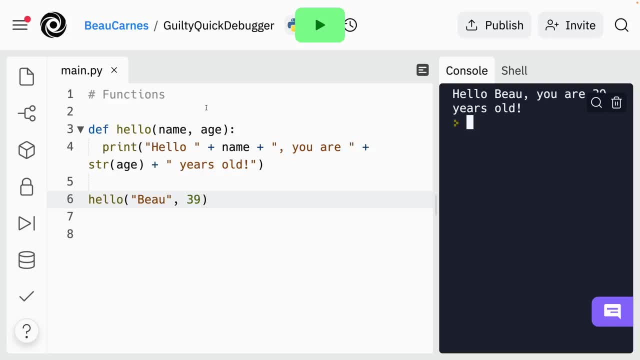 old, So we've used the name and the age. So parameters are passed by reference all types of Python or objects, but some of them are immutable, including integers, Booleans, float strings and tuples. This means that if you pass them as parameters and you modify their value inside the 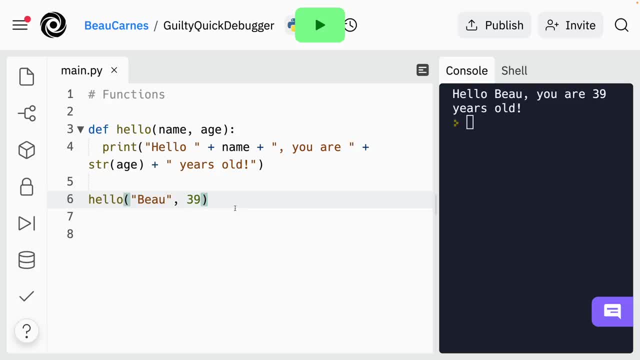 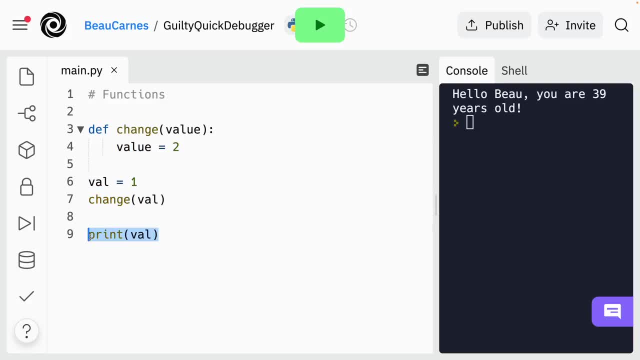 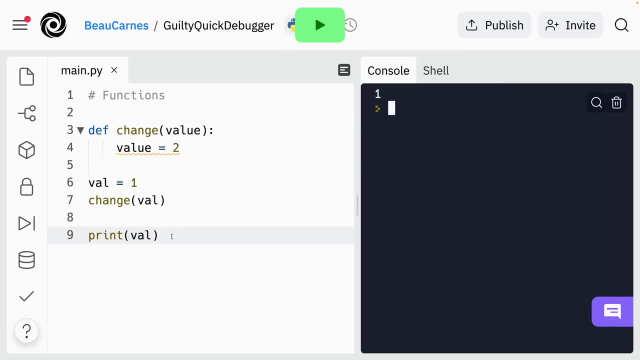 set value to two. well then we're going to print the value and see what happens. And you can see it's now just one here. So So it didn't change the value, the value. So what we change inside the function doesn't affect anything from outside the function. And then you can see we have these orange. 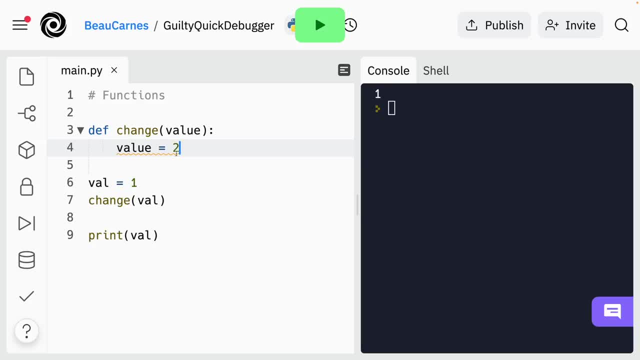 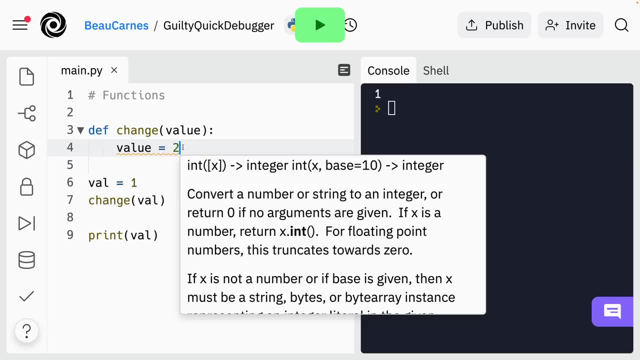 squiggly lines here. local variable value is assigned but never use. It's just showing that actually this isn't really doing anything once it's inside the function And when we change it doesn't change anything outside the function. So if you pass an object that's not immutable, you do change one of its. 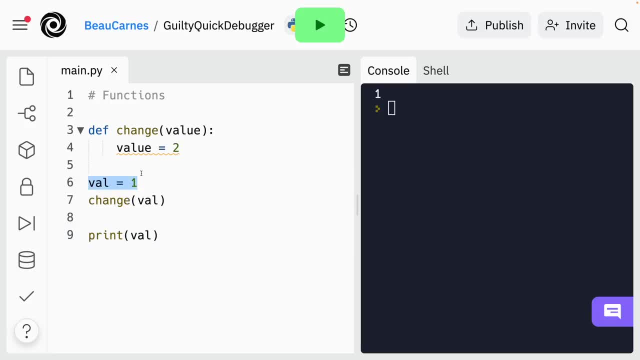 properties and the change will be reflected outside. So this was mutable, this is immutable. an object that would be mutable would be like a dictionary. So if I change this to a dictionary and I put name and I said to bow, but then inside the change I do. 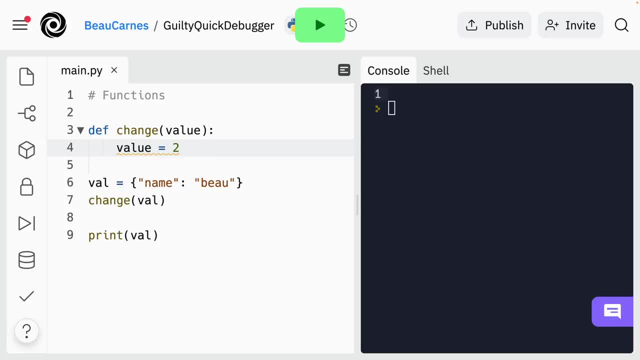 each value dot name or not. output the brackets value name. So the key of this dictionary- and I said that to Sid and I run this, we'll see. now the name has changed to sin, So we changed. we use the change function to change name to Sid And now it actually is changed. 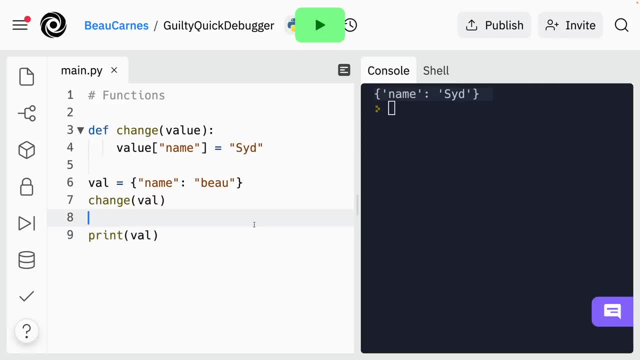 because a dictionary is mutable, So a function can also return a value using the return statement. So I'm going to update this whole thing and talk about return statements. a function can return a value using the return statement, So it's going to return this. 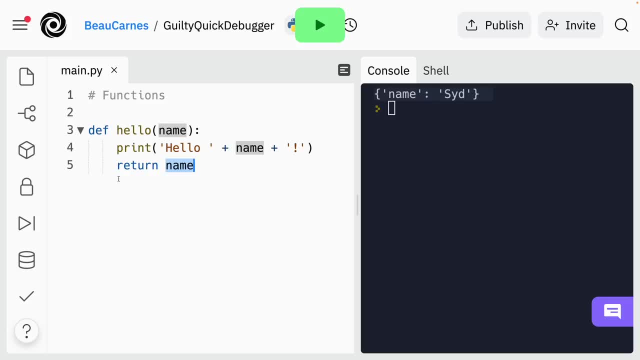 name that we then can continue to use in our, in our program, And it doesn't have to return name. it can return anything that happens inside the function And the when the function meets the return statement, the function in. so you can have a return statement, have code after it, but it will. 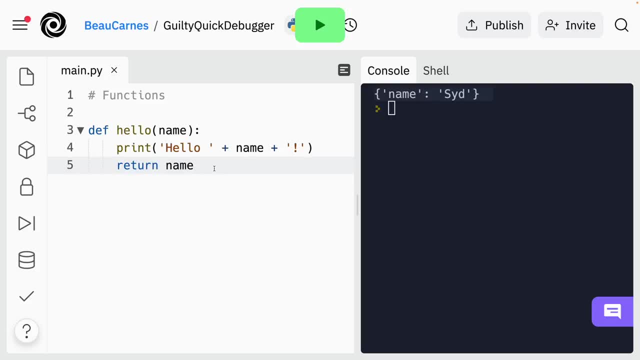 just end, Like, for instance, if you have the return statement in a conditional, like in an if statement, we can also omit the return, the return value. So it's just going to end the function and not return anything. So I had mentioned having the return statement in a conditional, So that's. 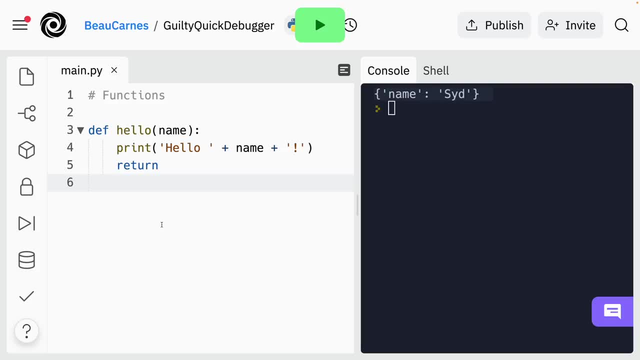 a common way to end a function if the starting condition is not met, Like, for instance, if we update the function to this. so if not, name return this. so if I mean if not name return, or else if you don't even need an else because this will. 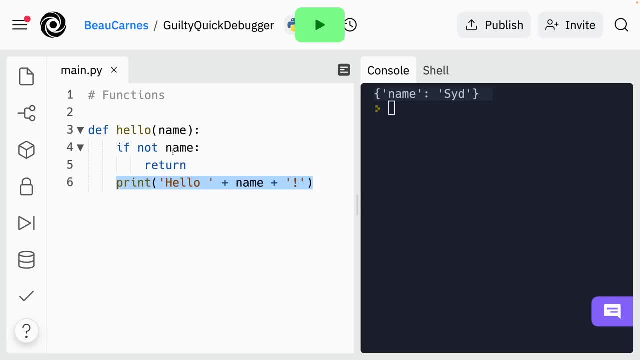 just in the function and you don't even need an else. this will happen if there is a name. Now we just said that you have to pass in something if you don't have a default value. So the way to get to that would just be to call the function with false. 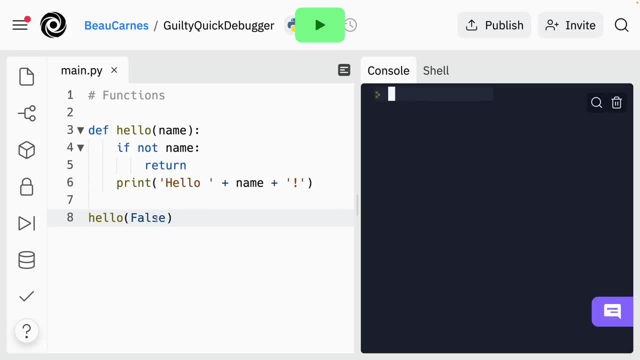 So if we call with false, then it's just going to return, it doesn't do anything. But if we call it with bow, then let's see: Hello bow. So you can also return multiple values by using comma separated values. So, for instance, I can- I'm just going to take this part off here. 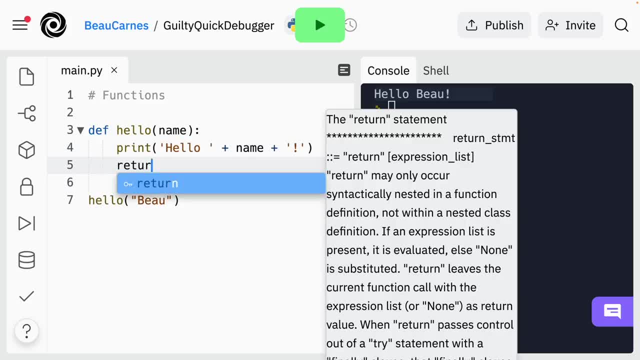 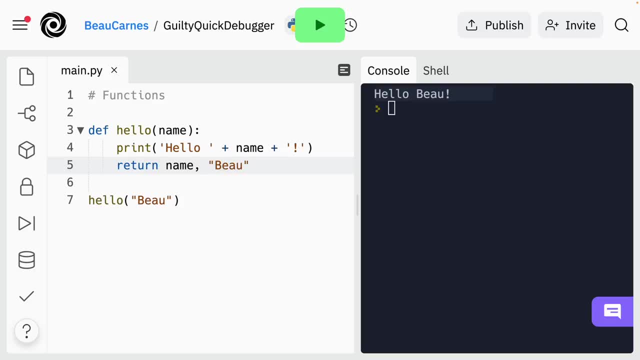 and then add a return statement, return- and then I can return the name. I can return bow. in case that's not the name, I can return eight, and then I can call this- and I'm just going to call this with Sid And we can see what happens Now, Oh, 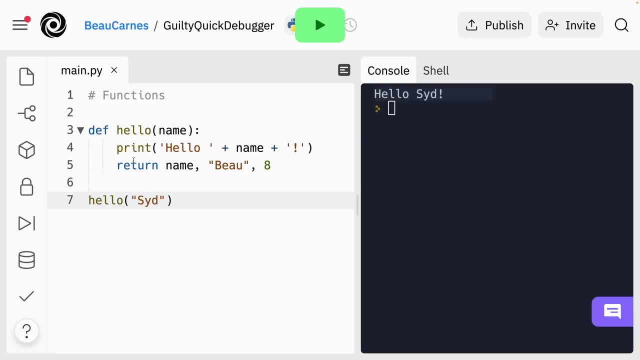 it doesn't. it's not, it doesn't actually print what's been returned. But if I print this, here we go, then we can really see what happens. So in this function is going to print this, but now we're also going to print what's returned. So let's see what that looks like. So 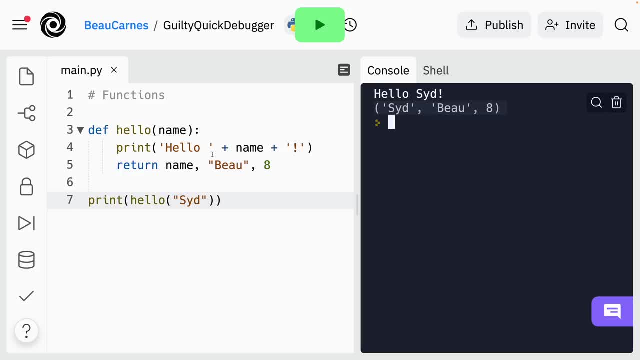 this is what it. when we print what was returned, it looks like this: So it's Sid bow eight. So one thing related to functions and also related to other parts of Python is variable scope. So let's look at this. we've declared a variable up here, And when you declare a variable, 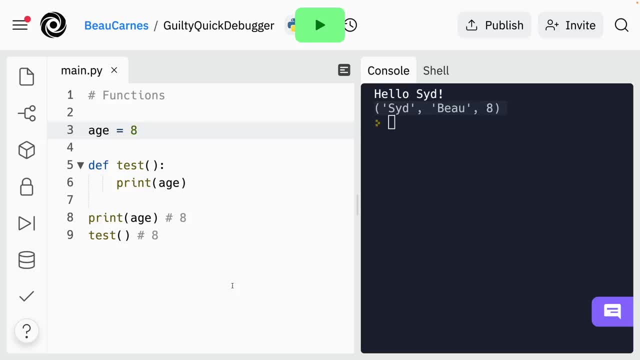 that variable is visible in parts of your program depending on where you declare it. So if you declare a variable outside of a function, the variable is visible to any code running after the declare, after the declaration, including the variable. outside of the function, the variable is. 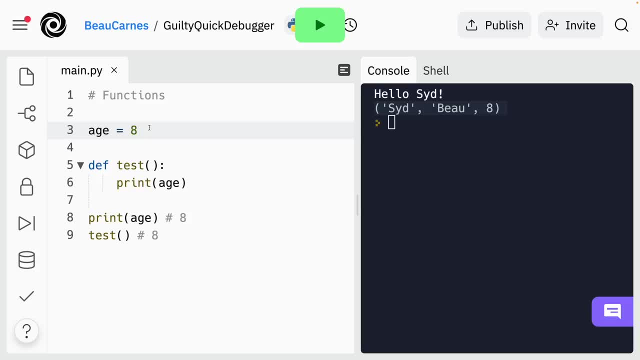 visible to any code running after the declaration, including functions. So we call this a global variable. So we've declared this before the function, So we can now access it inside a function and also outside the function. So, if I so, we can see eight and eight and it shows right. 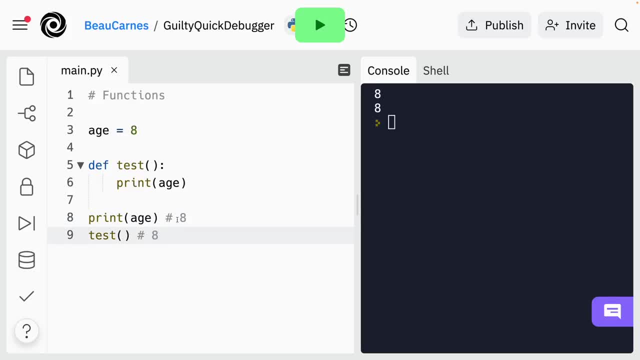 here what's going to show in the console here. But if we declare a variable inside a function, let me give you an example. If we declare this variable inside the function- I'm just going to move it down to here. Now it's a local variable And it's only visible inside the function. So let me just delete this. 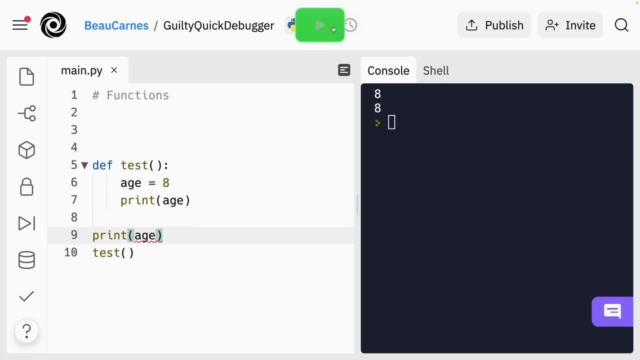 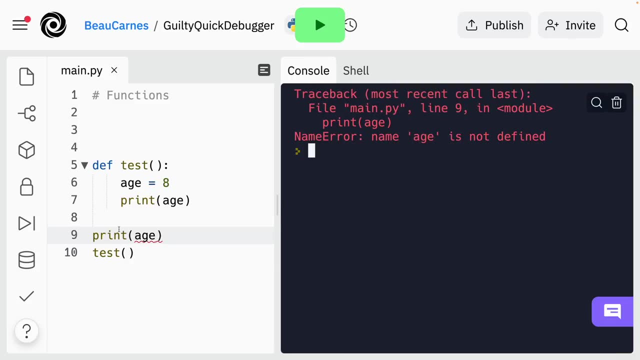 because it's not actually going to be doing that. So if I run this, we're going to see there's there's an error. Name age is not defined. we're trying to print the age here But since the age was declared inside the function, it's not available outside the function. it's only available inside. 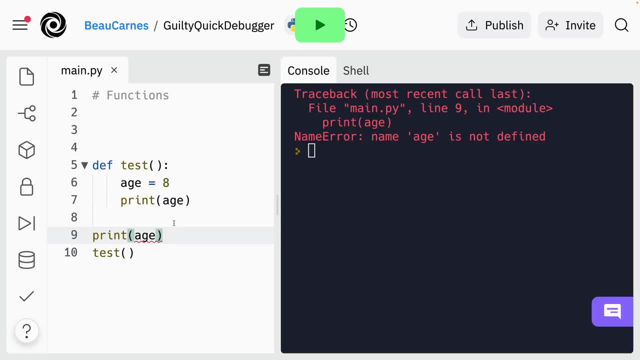 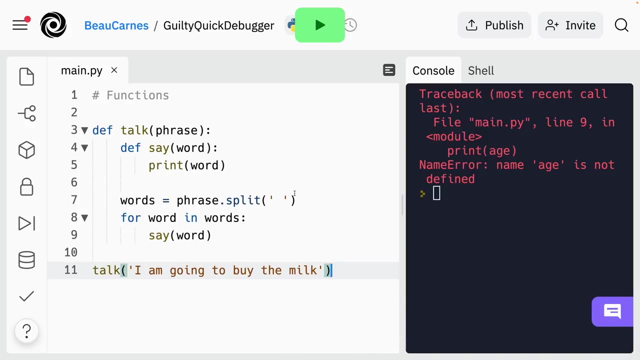 the function. So you just have to be aware sometimes there's local variables that only play inside the function And there's global variables that can apply inside a function and outside a function. Okay, now let's look at something else with functions, And this is nested functions. functions in Python can be nested. 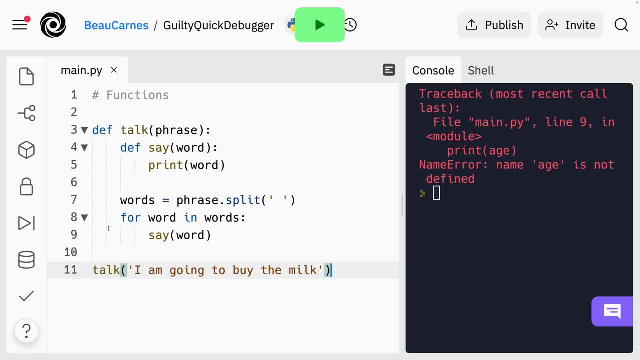 inside other functions. A function defined inside a function is visible only inside that function. This is useful to create utilities that are useful to a function but not useful outside of it. So you might ask, why should I be hiding this function if it does no harm? Well one because 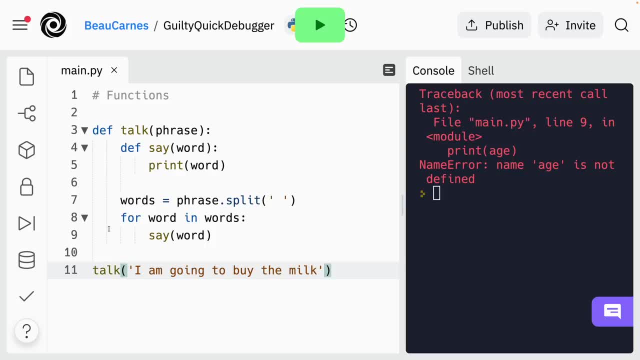 it's always best to hide functionality that's local to a function if it's not useful elsewhere, also because we can make use of closures, which we'll talk more about later. So So look at this example. So we have this function, talk, And inside the function, 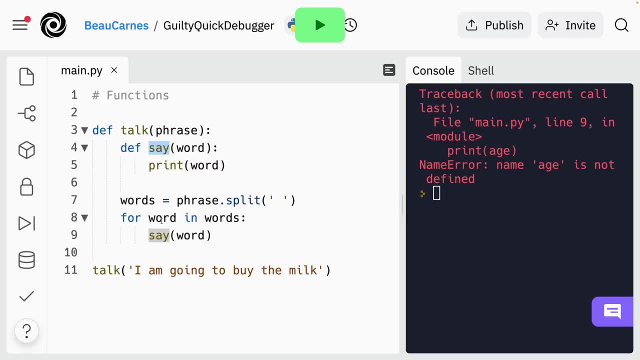 we defined another function called say, and then, with what we, what we do is that we can call that save function inside the function, And so the way this works is we pass in the phrase, so here's the phrase, and the phrase I'm going to buy the milk, And here we do, we, we split it. So 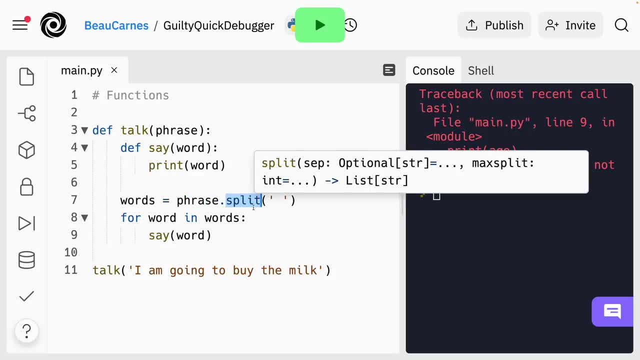 split is a way to create a list of out of this string. So we have the string but it's going to split it on every space. So it's going to create a list of each word individually And then we're going to run this loop- more on loops later- And we're going to for every word in the words list. 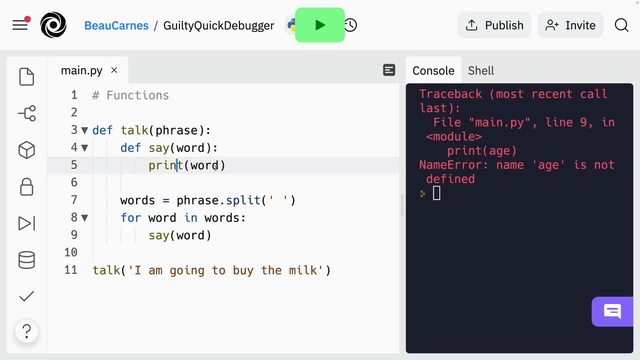 we're going to say the word. we're going to say the words, just going to print the word. So if I just run that I am going to buy the milk, And every time it prints it, it prints it on a new line. So this would just be an example, because we're never going to want to use this save. 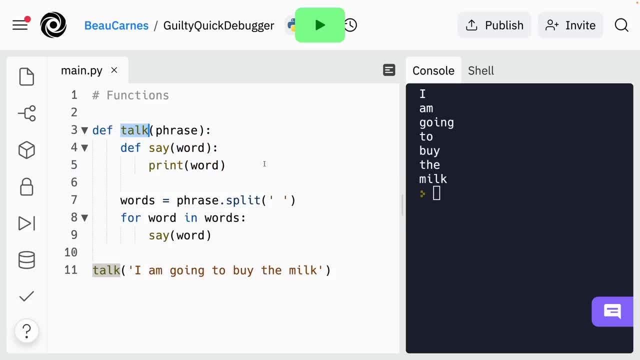 function outside of the talk function. So it's better just to put it inside the talk function And then I'll just paste in another example here. If you want to access a variable defined in the outer function from the inner function, you first need to declare it as non local. So we're using non local here at non. 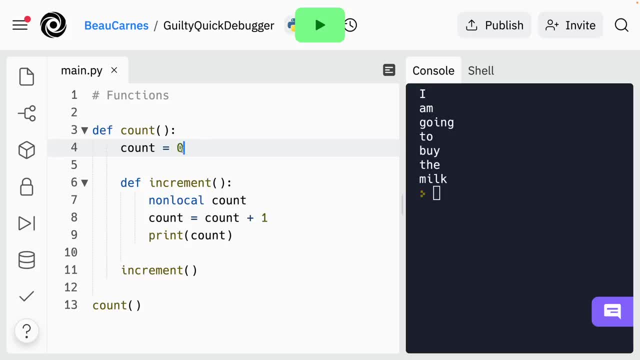 local count And this allows us to access this variable that was declared inside the out. So this is the outer function, count, And we have this variable called count And to be able to access that variable in the inner function, we have to call it non local, or we already talked about variable scope And if we didn't call, call this. 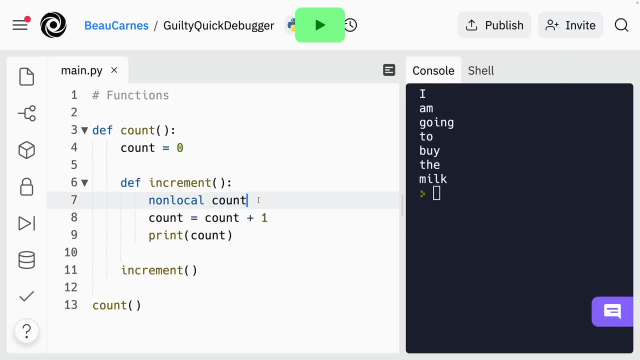 non local, then we could not access the count variable from inside the function. So like, for instance: I'm going to run this, it's going to print the count, which is just count plus one. it's just adding one to this number. that's all the function does. But if I take off this word, 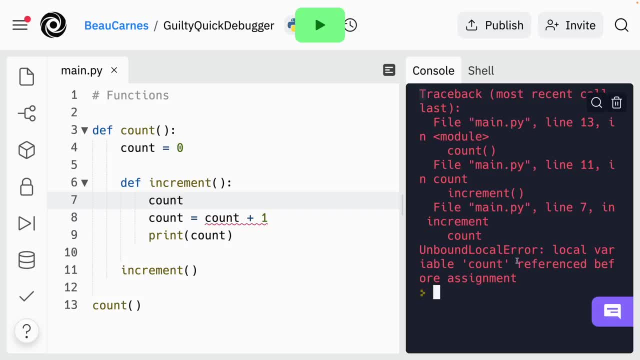 non local here and I run this, we're going to get an error because it doesn't know what count is. it doesn't know that we're going to get an error, So we're going to get an error, So we're. 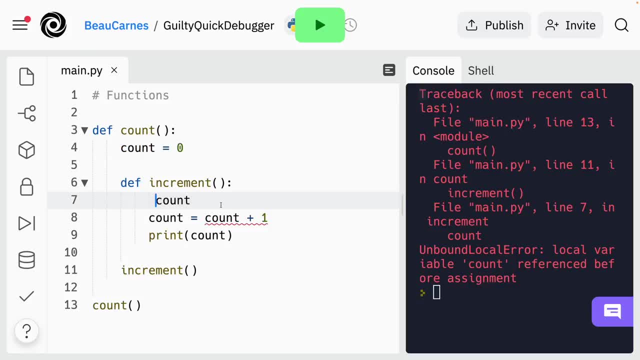 referring to this count in the inner function. So we'll just put that back on there And then it should work again. This is especially useful with closures, which we're just about to talk about. So closure is a special way of doing a function in Python. If you return a nested function from a 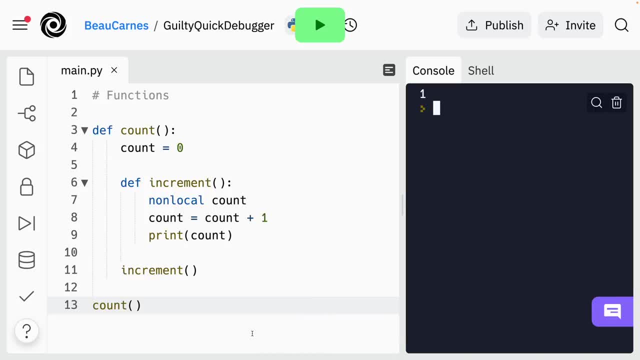 function. that nest function has access to the variables defined in that function, even if that function is not active anymore. So let me show you an example. I'm going to paste in code. there'll be very similar to this, but I'm going to paste in code that's not active anymore. So let me show you. 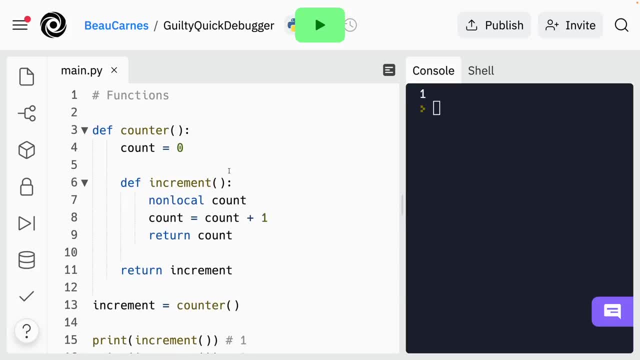 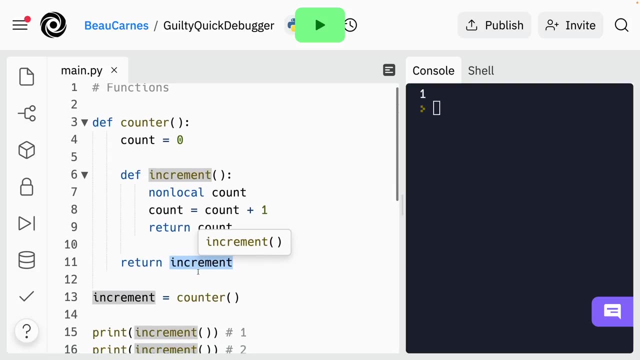 this code, but just a little different, and then I'll explain it. So now, instead of count, it's a counter. So we're returning count from this nested function And from the outer function. we're returning the nested function, we're returning the increment function, And then 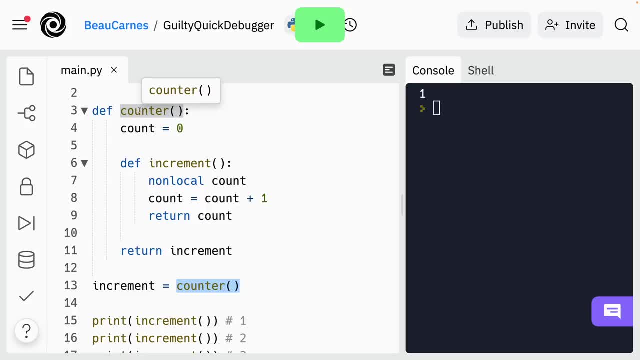 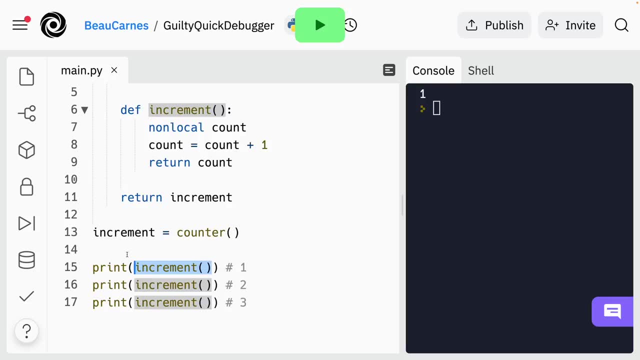 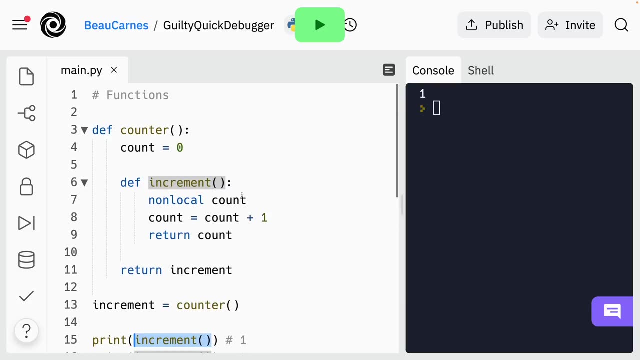 here, instead of just calling the function directly the outer function, we're assigning it to this variable. And now we're going to print, we're just going to call, we're going to call this variable, which is the returned inner function. So we're basically calling the inner function And 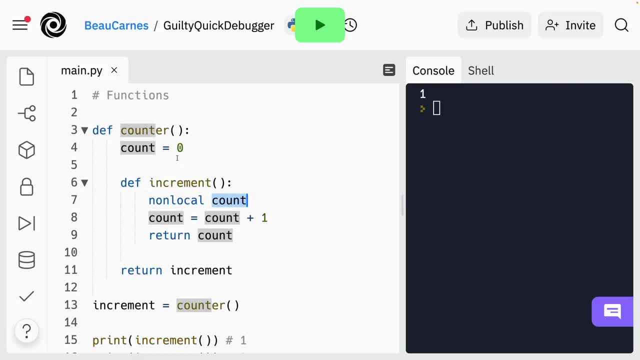 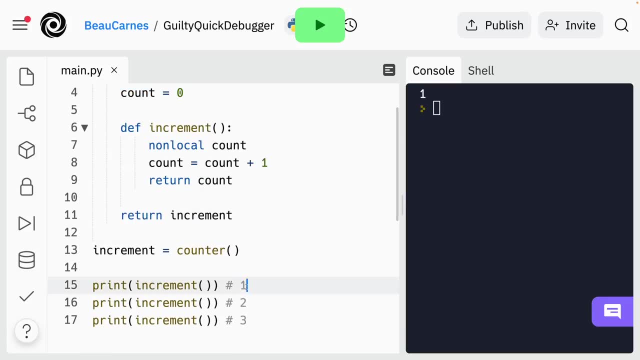 it's still going, it's because we're calling the inner function. it's not going to reset the count to zero every time And it can keep track of that value. And we have this using a common what it's going to return. But we can also run the program And we can see 123, just like that. So we return. 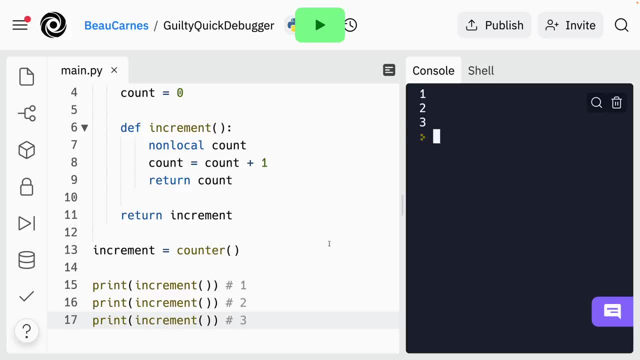 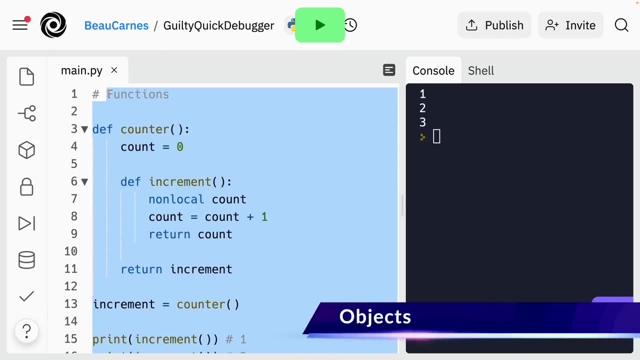 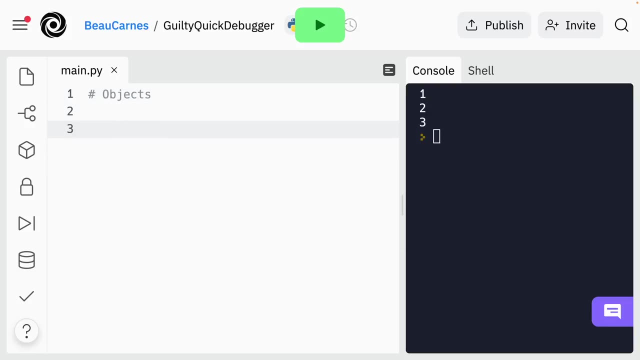 the increment inner function and that still has any function. And then we're going to call this access to the state of the count variable, even though the counter function has ended. So let's move on to objects. Everything in Python is an object, even values of basic prim of types. 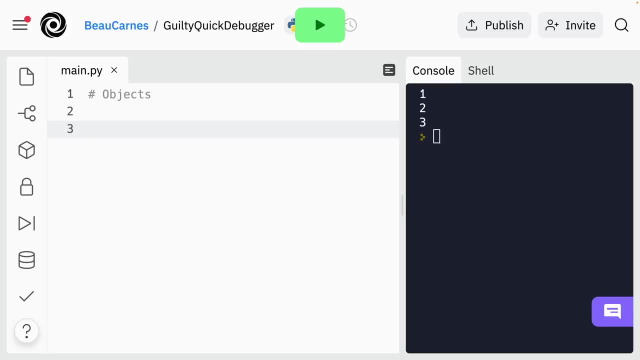 like integer strings, floats our objects, lists our objects, as well as Tuples, dictionaries and pretty much everything. So objects have attributes and methods that can be accessed using the dot method vertically, which are either large traded attack methods or expres and. 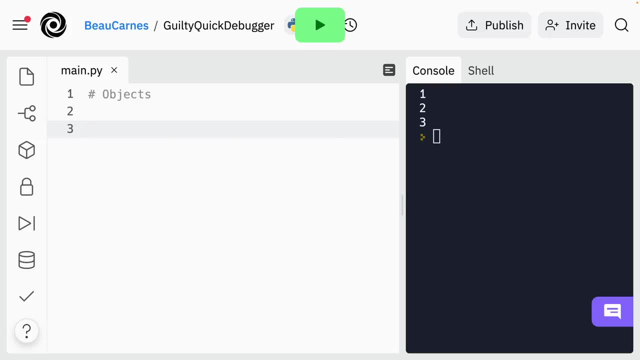 variable typeraisers, Double article types, dh r letters, stumes or etcetera, and타 l syntax. For example, let's define a new variable of type int. So I'm gonna do: age equals eight. 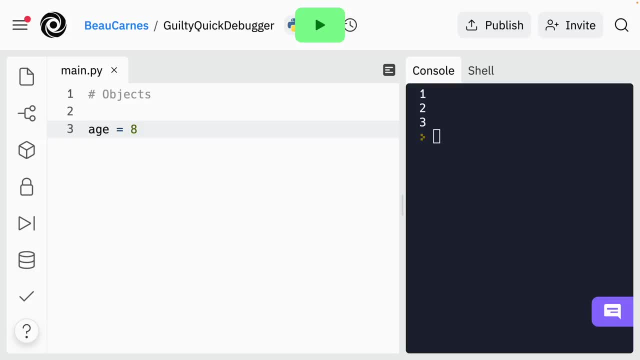 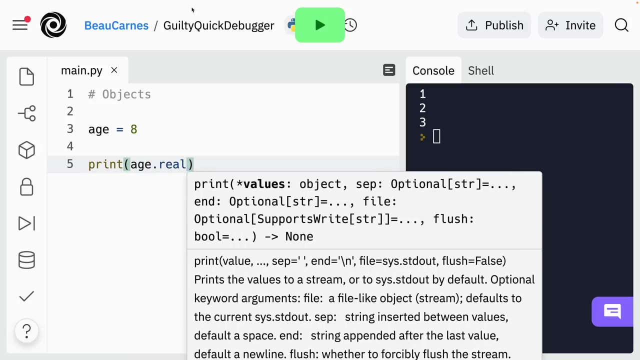 age now has access to the properties and methods defined for all int objects. This includes, for example, access to the real and imaginary part of that number. So I can do print age dot real And then if I just run that the real part is eight, I can also print the imaginary part of. 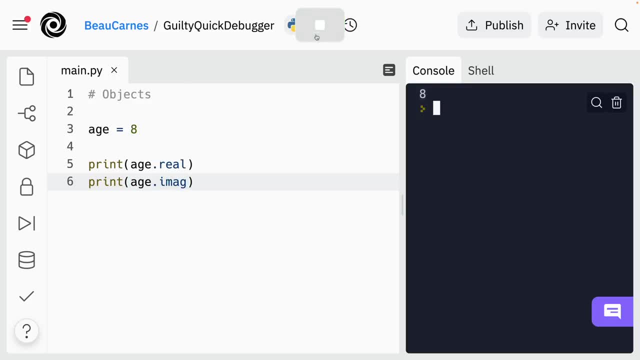 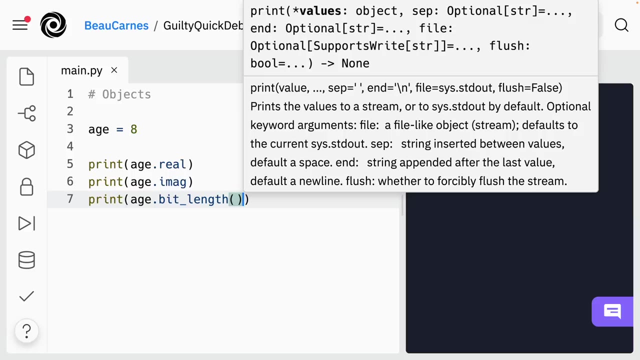 the number image And there is no imaginary part of the number, So it just does zero. I can also get the the bit length- age, dot, bit length- And if I run that we can see the bit length is zero. And then if I run that we can see the bit length is zero. And then if I run that, 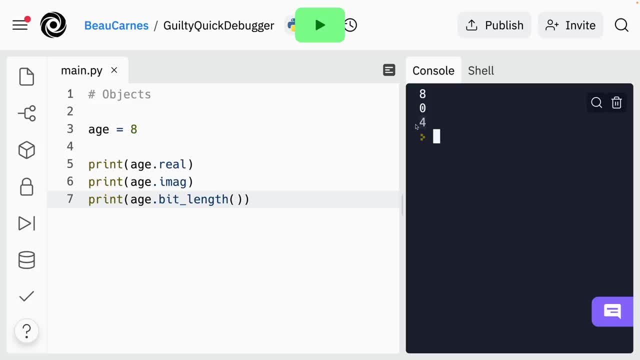 is four. So the bit length method returns the number of bits necessary to represent this number in binary notation. So there's just a lot of things that you can use for all int objects, And these are just a few of them. So a variable holding a list value has access to a different set. 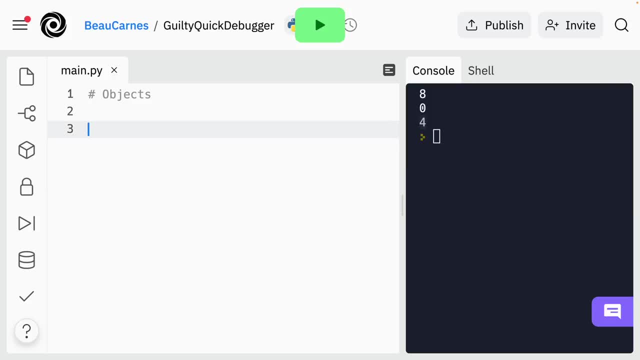 of methods. So I'm going to update this again. we're going to do items equals and we're going to create a list: one, two, So I can do items dot append. I can append a. three. append another item. I can do items dot pop. 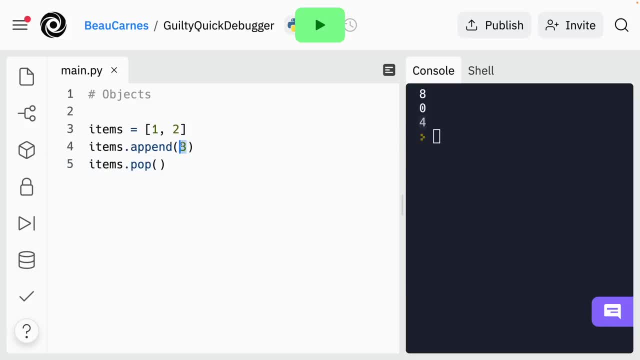 which is going to remove and return the last item, which is the three And the methods. so So these are the methods of pin and pop, And the methods available to an object depend on the type of value. The ID global function provided by Python lets you inspect the location and memory for a particular object. So, for instance, 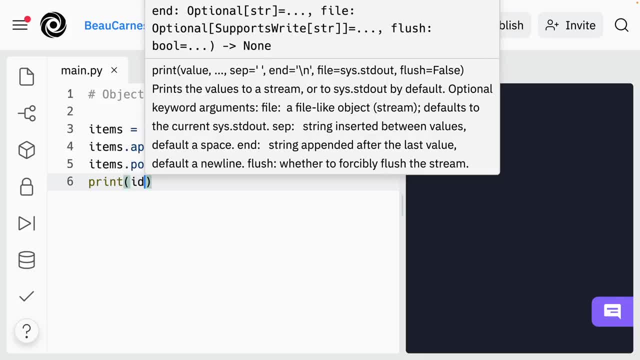 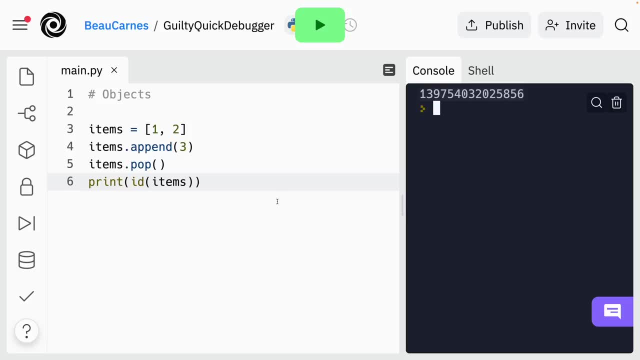 I could do print and I'm going to do ID. what's the ID of the items, object And we can see? this is the location in memory. So some value, some objects are immutable, while others are immutable. this is something that we already talked about a little bit. That depends on the object itself. If 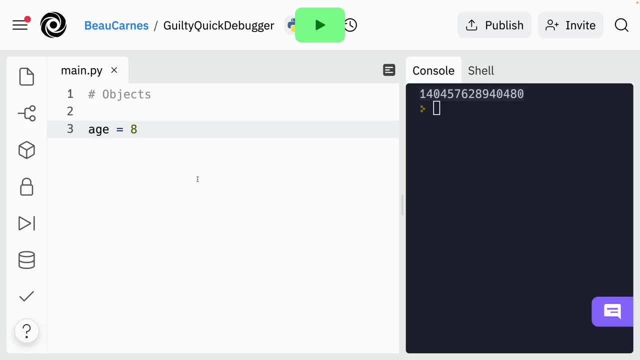 the object provides methods to change its content, then it's mutable. Otherwise it's immutable. Most, most types defined by Python are immutable. For example, an int is immutable. there are no methods to change this value. So if you increment the value like with age equals age plus one. 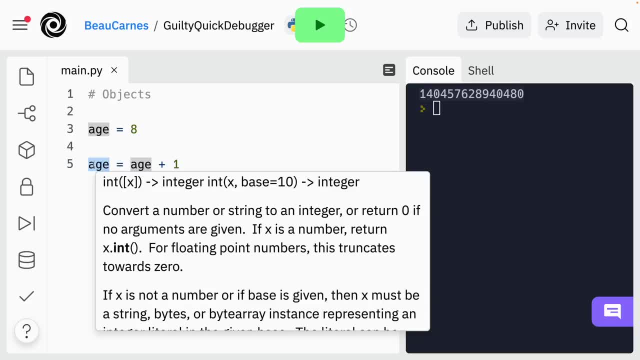 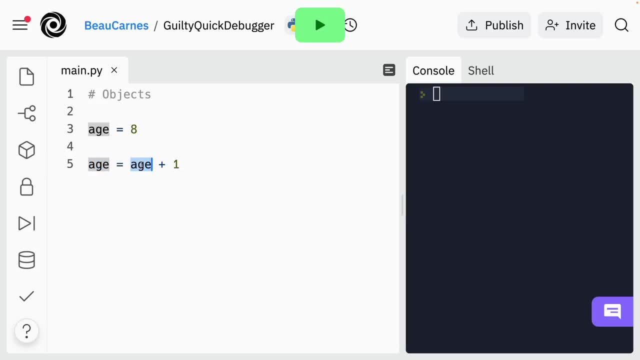 it's actually going to create an entirely new value. So it's not going to even be the same object at all Because age you have to create a whole new one to reassign it, but something like in an ad dictionary: it would actually be the same object, but you could just change different parts of it. Now, 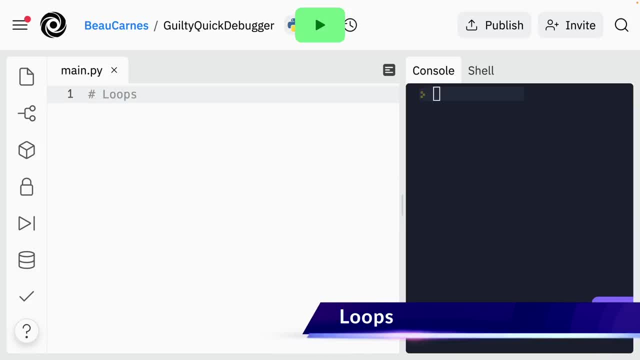 let's talk more about loops. So this song we already discussed a little bit in the previous section. But loops are one essential part of programming And in Python we have two kinds of loops: while loops and for loops. So before I show, I'm going to paste in this code, But I just want to show something really quick. See how. 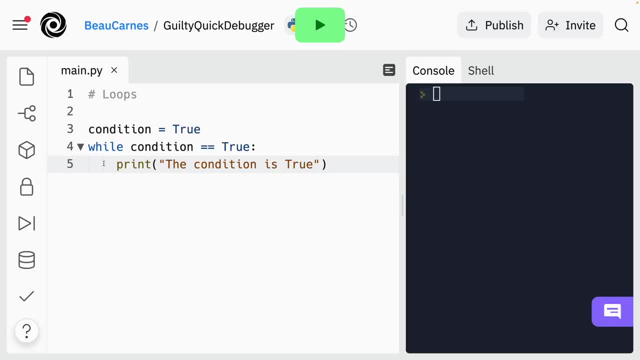 there's a line like dotted line here and a dotted line here. This is showing the default indentation which we can change. So I'm actually going to go and change that really quick. Wait, I think I'm going to have to. Yeah, I'm going to zoom out so I can get to this And I'm going to change the. 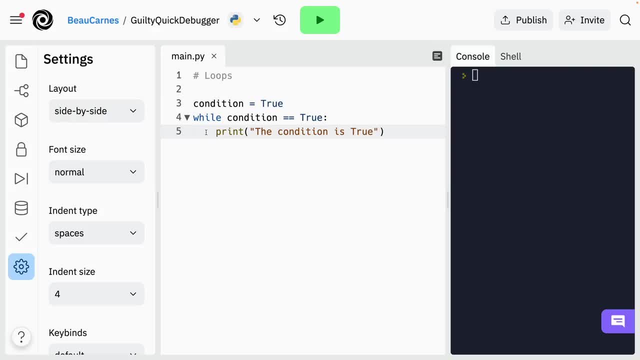 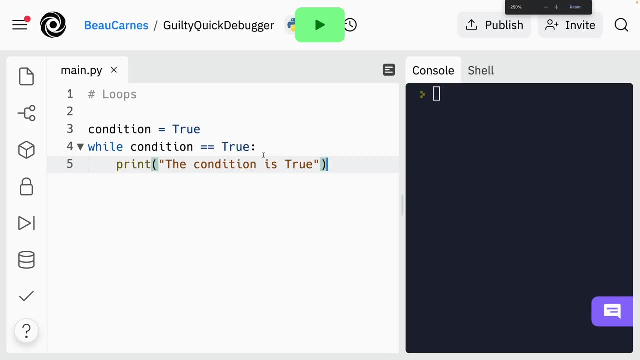 indent to four, And now it's not going to have a little line right in there. So now I'm going to go back up here And let's zoom in again. Okay, so let's talk about while loops. while loops are defined using the. 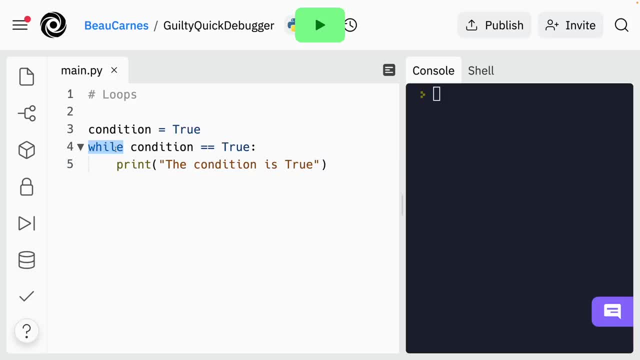 while keyword and they repeat their block until the the condition is evaluated as false. So while condition equals true, So this particular example is an infinite loop. it never ends because this condition is always the same. So this condition is always the same. So this condition is always. 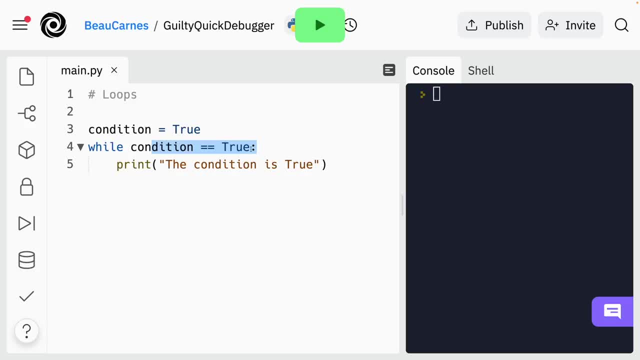 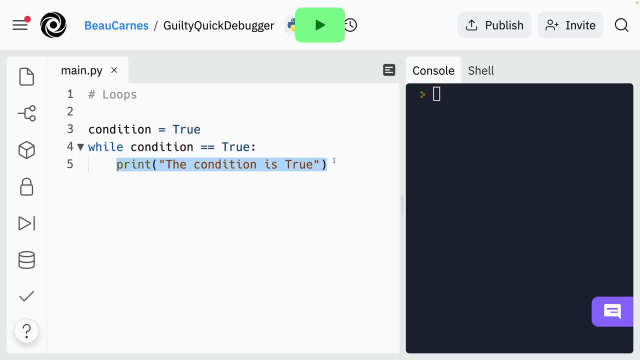 this condition is true. keep running the code inside the loop, all the lines of code that are indented the same amount. So let's halt the loop right after the first iteration. I can do: condition equals false. So now, if I run it, 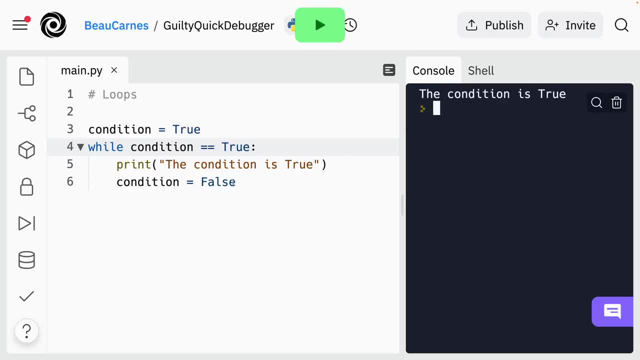 it just runs the loop one time. So in this case the first iteration is run as the condition is evaluated true, And then at the second iteration the condition test evaluates to false. So the control goes to the next instruction after the loop, which in this case there is no one's. next, 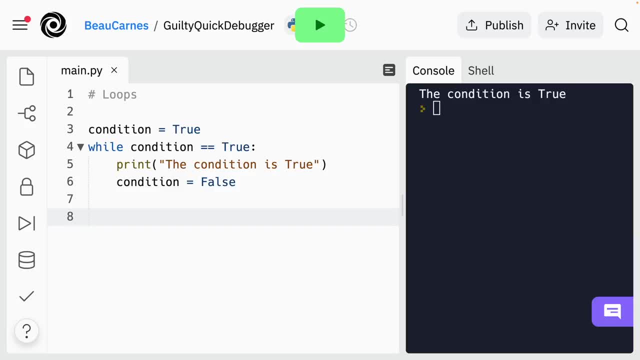 instruction after the loop. it's common to have a counter to stop the iteration after some number of cycles. So here's a while loop And it just runs the loop one time. So in this case the first iteration is running the loop with a counter. So you start the counter at zero And then while count is less. 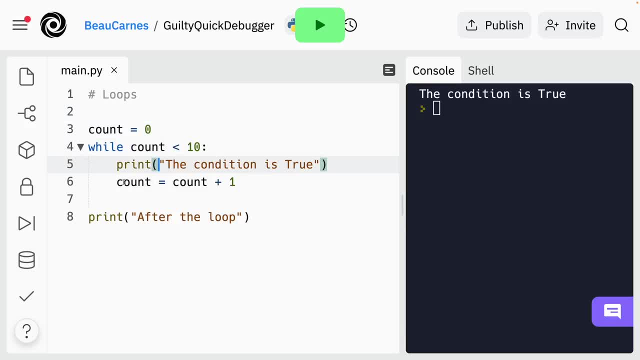 than 10.. We're going to print this: count equals count plus one. So it's going to increment the counter every time until we get to the end. So it's going to see it's going to print this until eventually the count is greater than 10.. So, or 10 or 10 or greater, while count is less than 10.. So 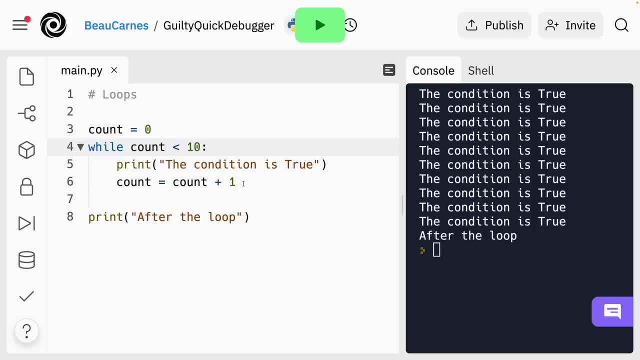 once it gets to 10,, though, the loop will stop Again. another way out to doing to do this, we could have just done plus equals plus equals one, So if I run that, it's going to do the exact same thing And other type. 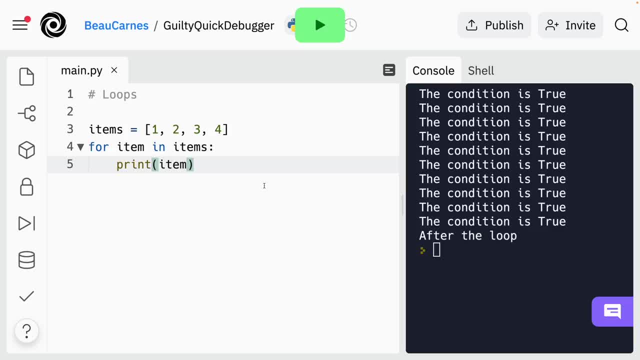 is the for loop. So, using for loops, we can tell Python to execute a block for a predetermined amount of times, upfront and without the need of a separate variable and conditional to check its value. It's commonly used to iterate the items in a list. 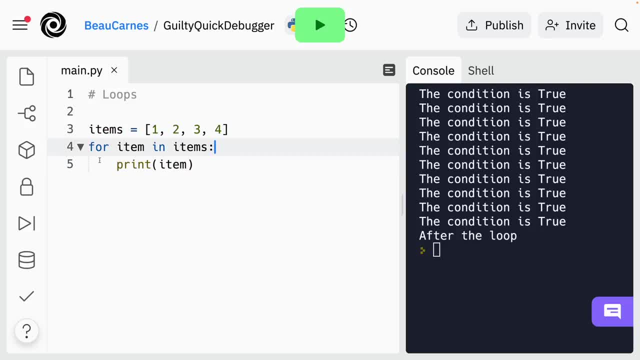 So we have this list. there's obviously four items here and then four item in items. So items is this list And then for each item the list. we're going to print the item- pretty straightforward And it prints each item in the list, Or you can iterate a specific amount of times using 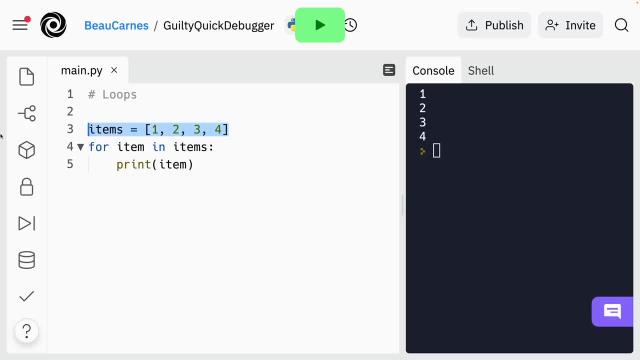 the range function. So let's say we don't have, we're not going to define this here, we're just going to do for item N, and then here I'm going to type in range And then I'm just going to type in a number- how about 15.? So I'm using the range function. that 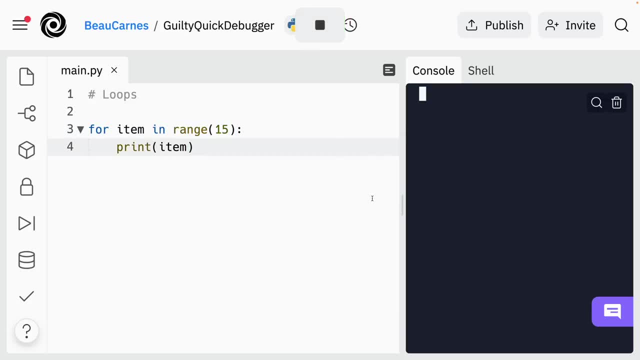 basically just returns a list And then, if I do that, we can see it's going from zero to 14.. So the range function is going to return a a list that goes from zero to 14.. So there's 15 items. 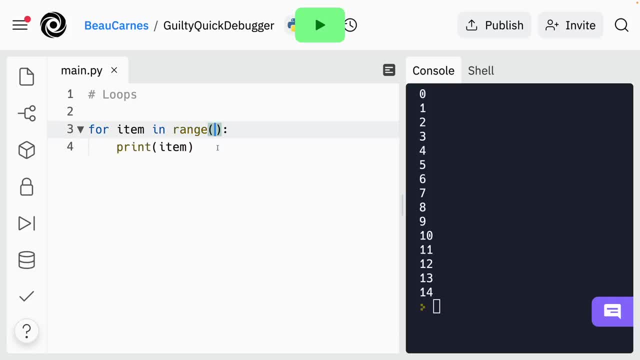 it's going to print the items. Now, if we just go back a few steps to when we had the list here we can. I can show you how to get the index. So right now it's just printing the items: 1234.. But 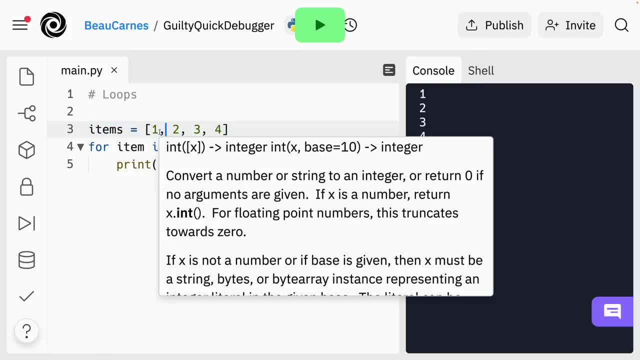 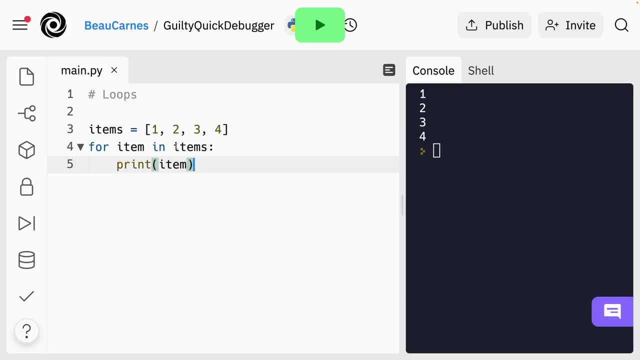 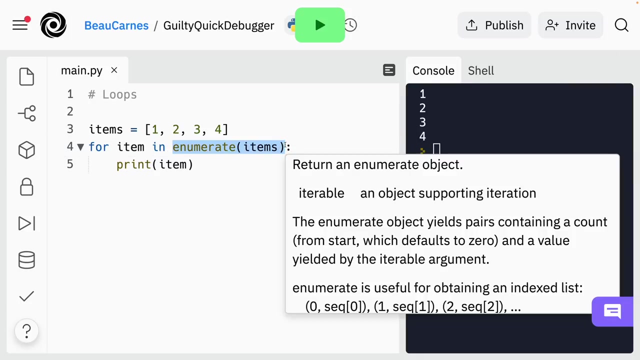 what if we want the index of the list? we can do that by using the, by wrapping the sequence in the enumerate function. So for items in, and then I'm going to do enumerate, I'm going to pass in the. So this is going to return each item and the index of the item. And since there's gonna be an item in, 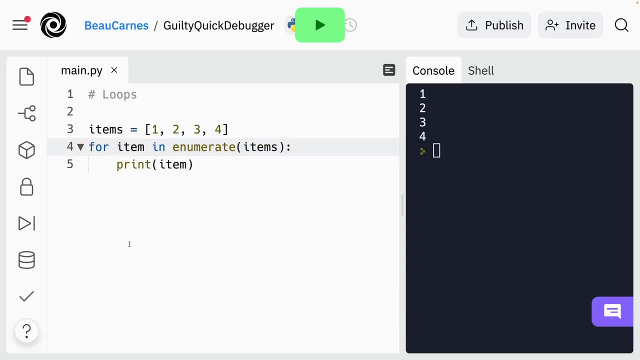 an index, but it's actually the index and then the item. I'm going to type in: index, comma, item. So this enumerate is going to get the index and the item. So now I can print the index and the item here And if I run that, so index zero item one, index one item two, index two, item three and 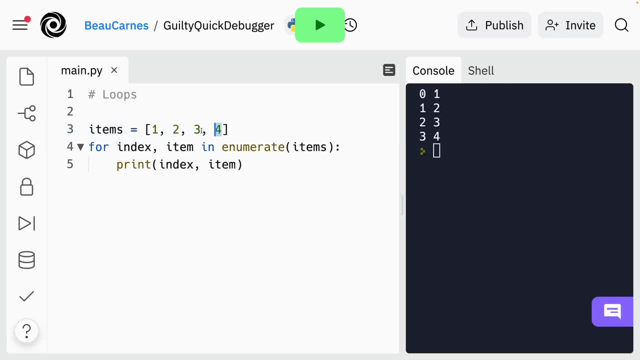 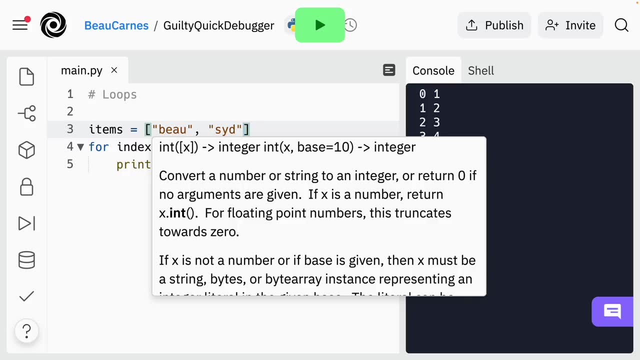 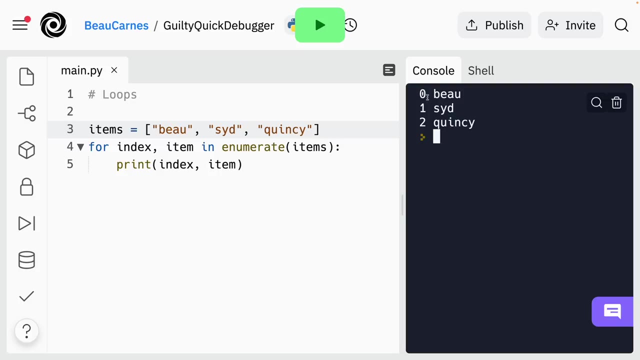 so on, And it doesn't even have to be numbers, we can do names, And if I just run that, what's not that one, And then we can see the, the index and the item, Then let me put in some more code here. 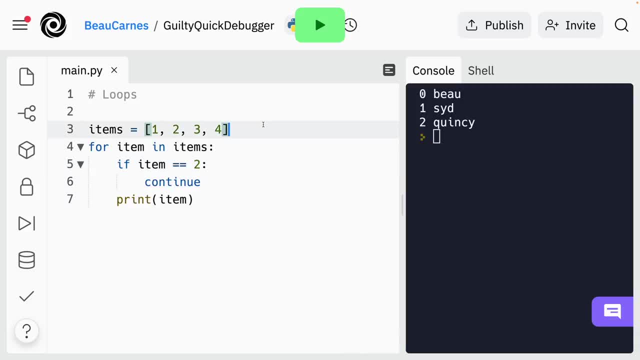 So I can talk about break and continue. Both while and for loops can be interrupted inside the block Using either break or continue. Continue stops the current iteration and tells Python to execute the next one, And break stops the loop altogether and goes on with the next instruction after the. 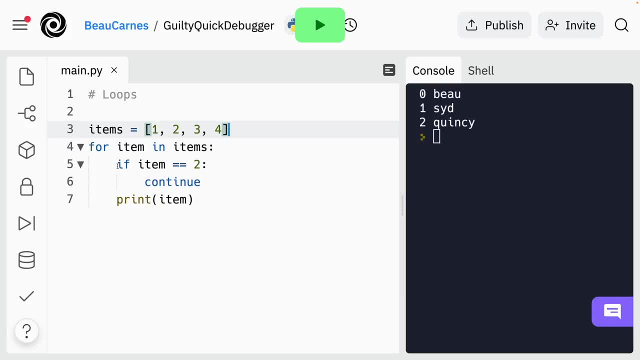 loop ends. So I'm going to just play this. So here we're saying: if item equals two continues, that means it's going to skip that iteration. So if I play this 134, so it's not going to, it's not going to get to the print item because it's actually skip that iteration. it just 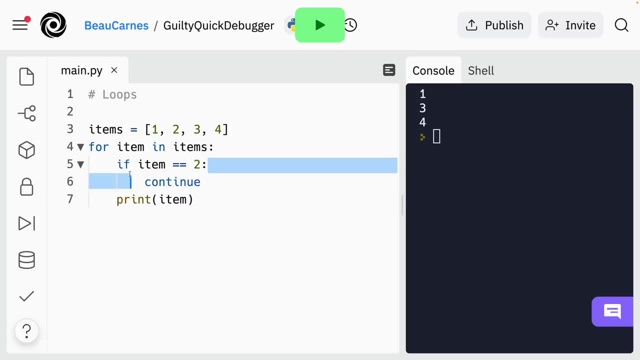 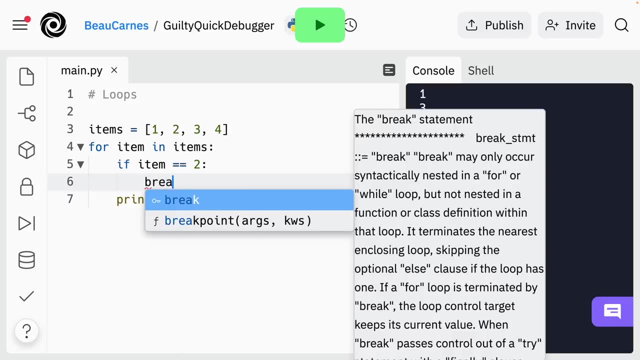 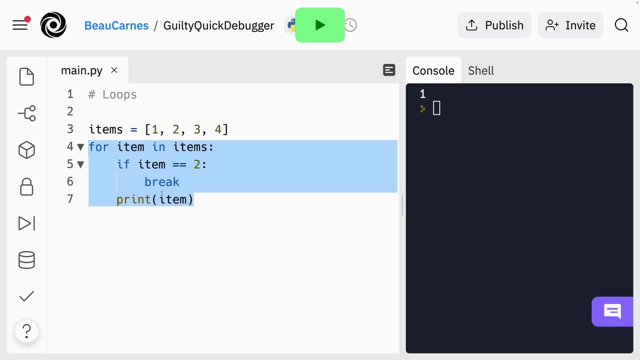 doesn't run any code after the continue, if this is true, And so it doesn't print two. So if we change this to break, it will be very it'll be a little different here. This time it's going to just print one, because now it's breaking out of the loop entirely And it's not going to run any. 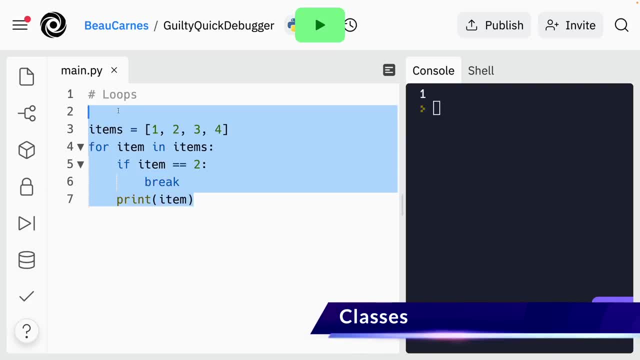 more iteration of the loop. Okay, let's talk about another thing: classes- classes in Python. So, in addition to using the Python provided types, we can declare our own classes And from the classes we can instantiate objects. An object is an instance of a class. a class is the type of. 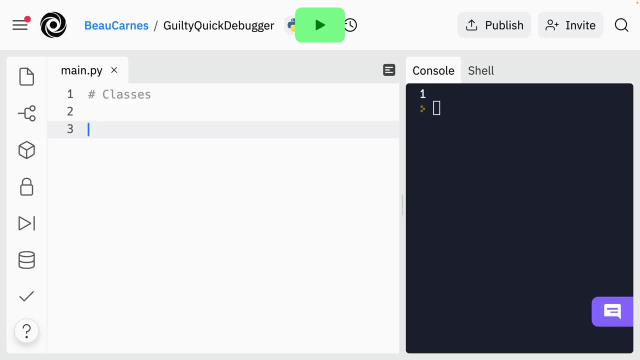 an object. So here's an example: I'm going to create a class called dog. So to create a class, you just put the word class and then put the class name, And now next I can, I can add a method for the class. So to define a method, I'll just do: define bark. 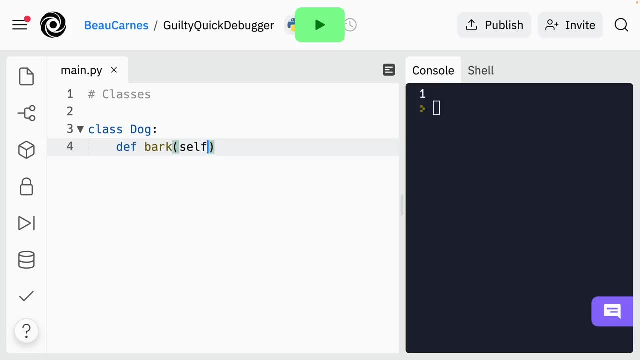 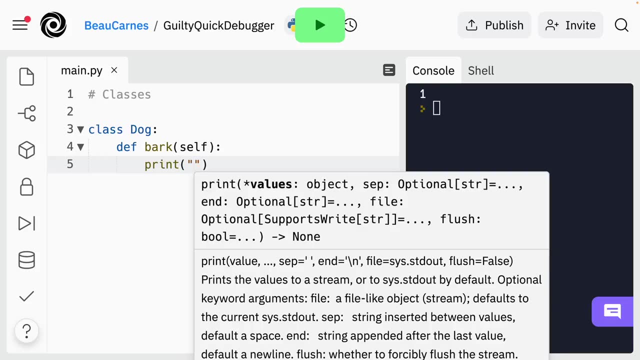 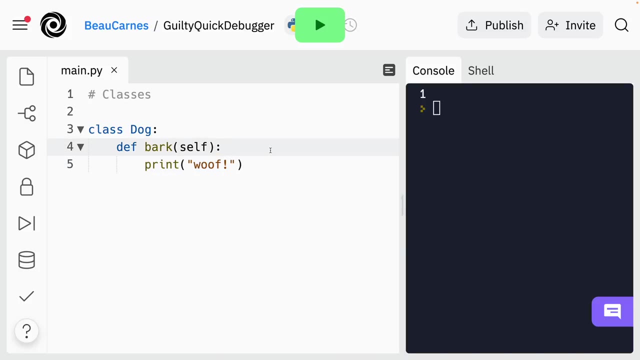 And I'm going to put the word self here, And inside this I'll print woof, Okay. so self as an argument of the method will point to the current object instance and must be specified when defining a method. So when you're creating a method inside a class. 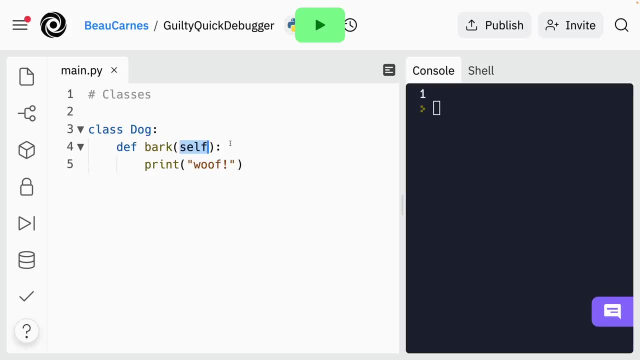 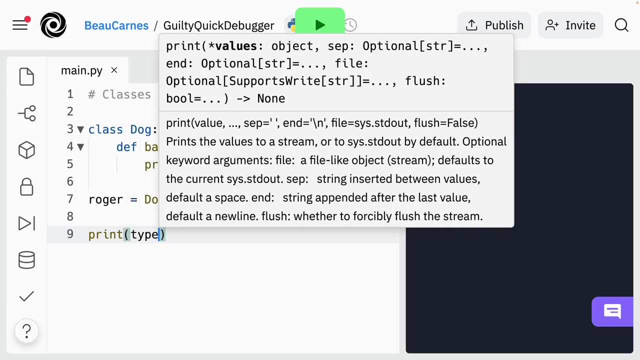 you're always going to start with self. So we create an instance of a class which is an object, like this. So I'm just going to put Roger equals dog, Okay, so I've created a dog. Okay, just like this. And then I can print type Roger. So let's see what the type of this Roger is. 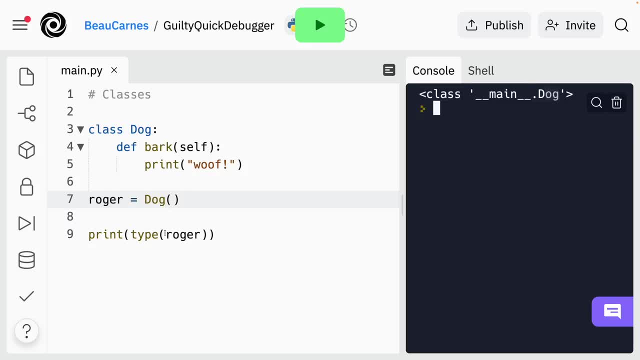 we can see, it's the class, the dog class. Roger is a dog, A special type of method called in. there's a special type of method called init, which is a constructor. So let me show you how to create a constructor. 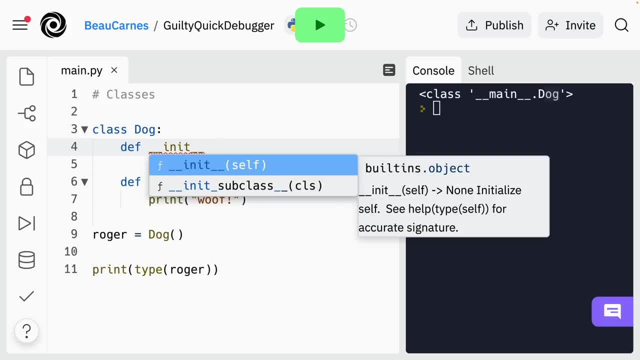 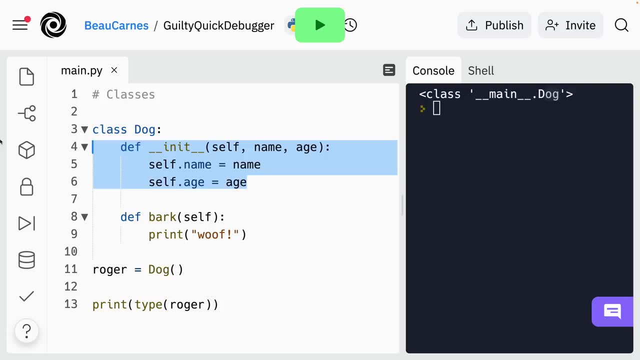 def. So we can use this constructor like this to initialize one more properties when we create a new object from that class. So you can see, we always have to add self. But now these are the two variables we can pass in when we create a dog And that will associate, be associated with that. 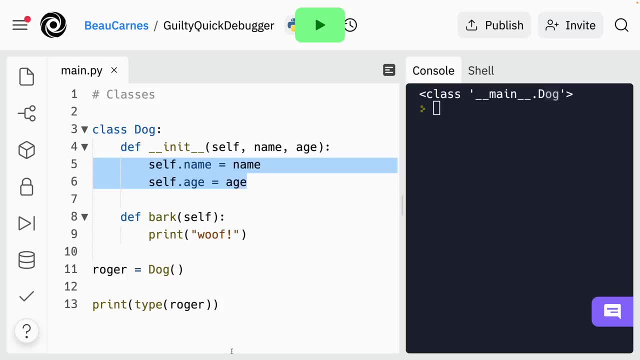 that object. So down here I can call, I can call dog, but I can pass in Roger for the name and the age. And now when we create this dog, it's going to assign the name to self dot name and it's going. 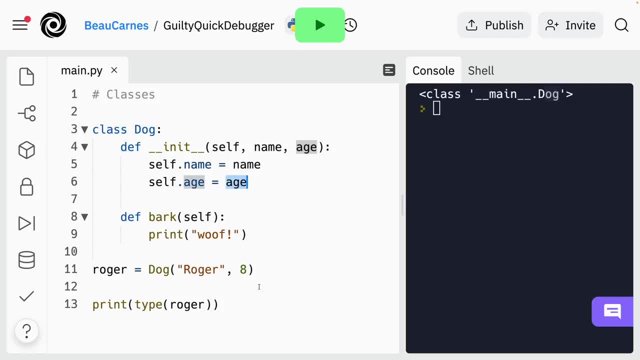 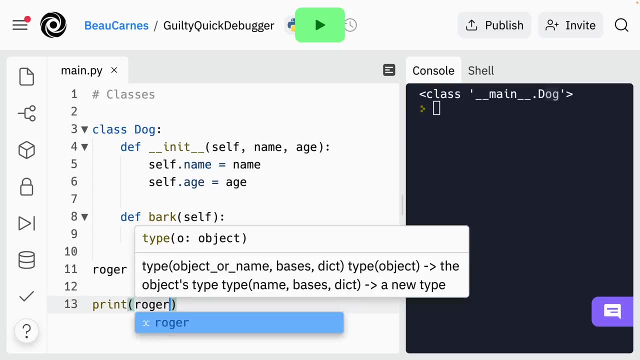 to assign the age to self dot age And let me show you how you can access that information. So I'm going to print, instead of printing the type I'm going to do Roger dot name. And now it's going to: when I do Roger dot name, that's self dot name. So self is Roger and we do self dot name, it's going. 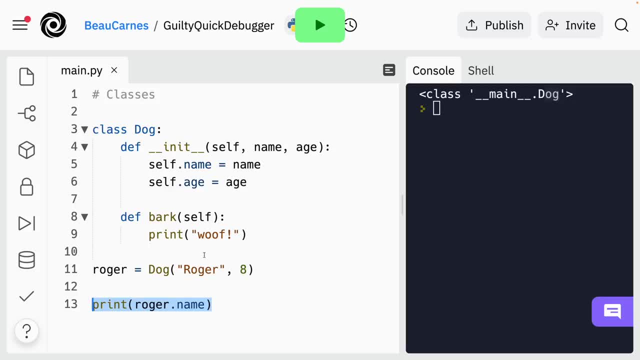 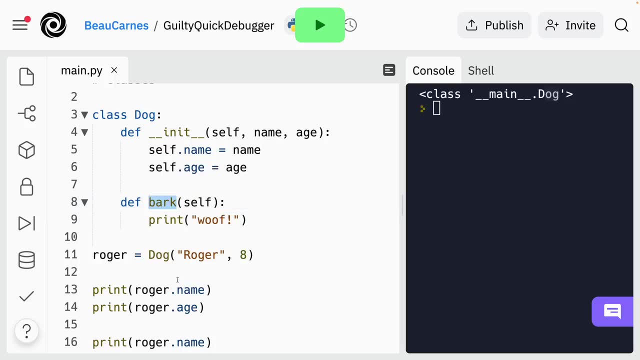 to be the name that was passed in, And then we can also do the age, And then we can finally call the bark method. So we have bark here and then we can see what that does. So I'm just going to run that. 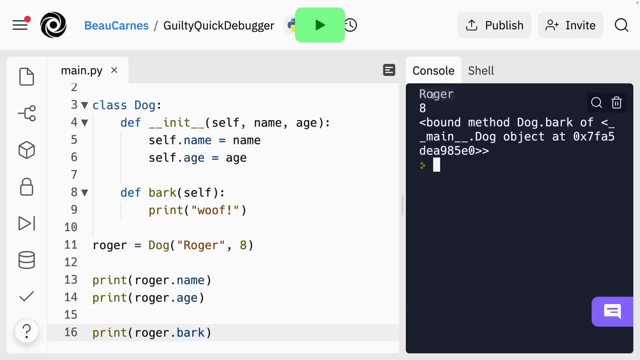 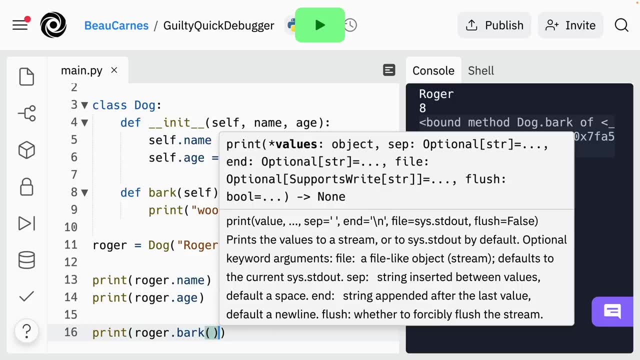 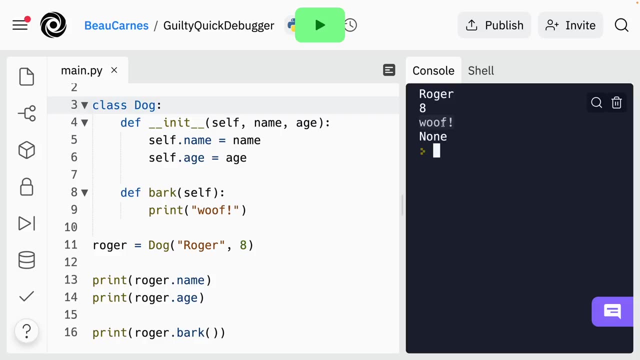 And we have Roger, we have eight. And then- this is because I should have put parentheses here, So let me put parentheses after bark. And so we have wolf here. So Roger, eight wolf. And the reason why it says none here is because I didn't have to put the print, So I put pranks. I was in this. 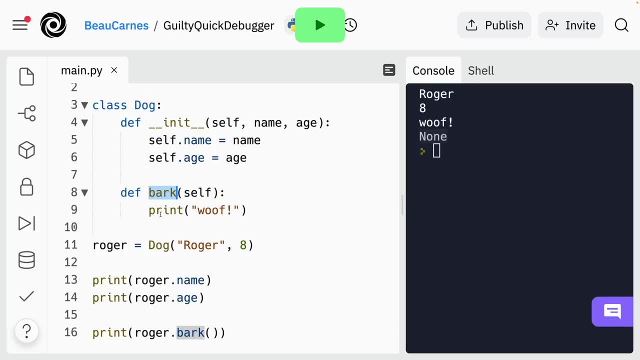 groove. you're putting print on everything, but calling bark already prints wolf. So when I do, it's when it's when it's printing. it's printing because since Roger dot bark doesn't return anything, there's no return statement. That's why it printed none. So there'd 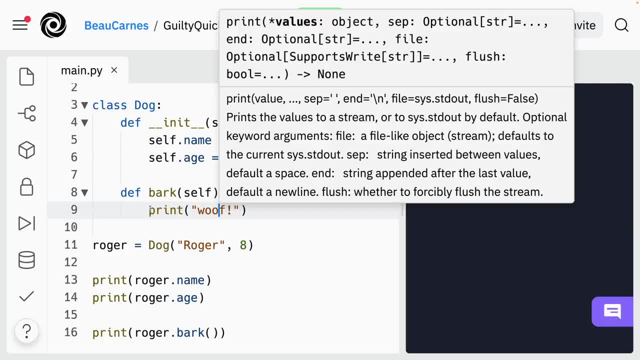 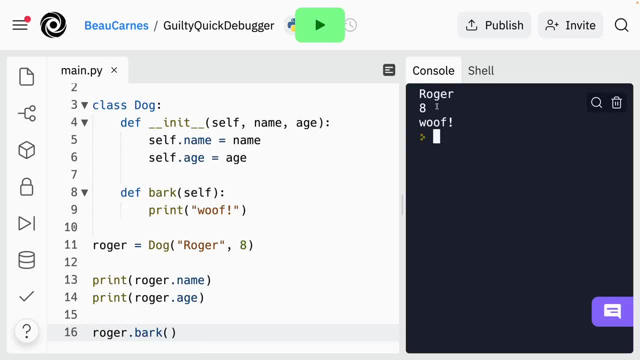 be two ways to fix that. either instead of printing wolf, I could return wolf, or I could just not do the print here, So let me just take that off. Okay, Roger, eight wolf. So one important feature of class is inheritance. Let me show you an example. 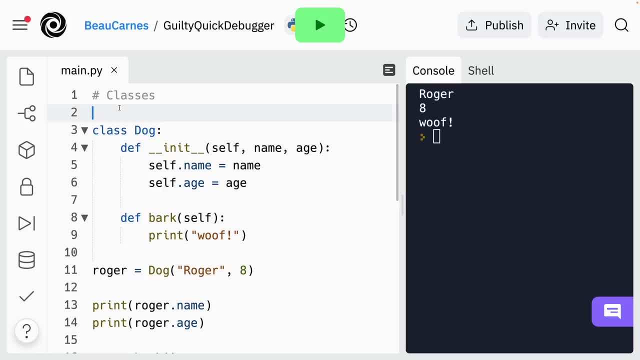 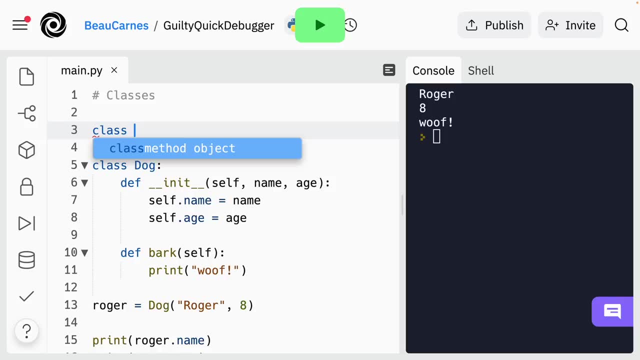 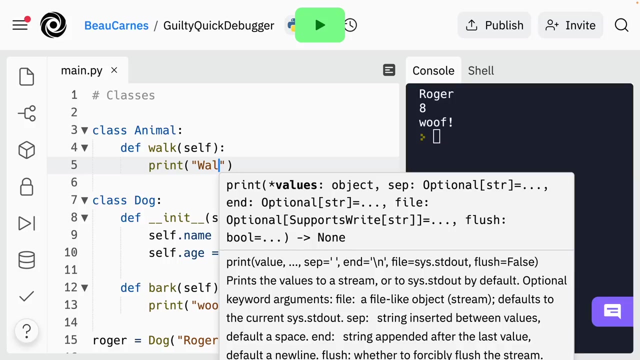 of inheritance. I'm going to create a new class before the dog class And this is going to be a class called animal And the animal class. I'm going to put a function called walk And I'm going to pay you always pass in self And this is going to print walking And then we can make the dog. 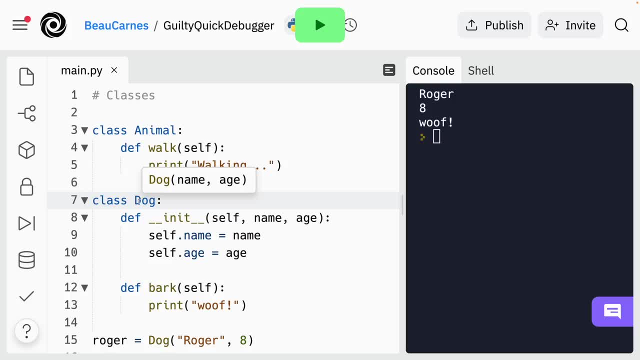 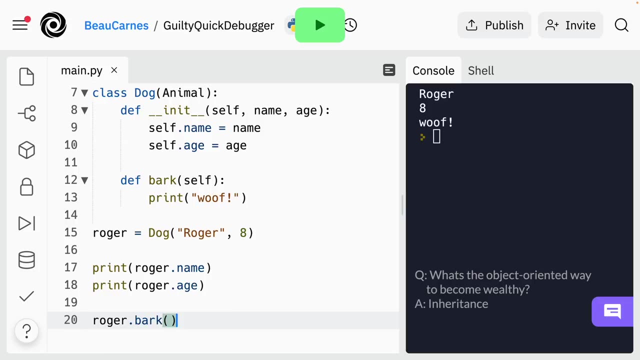 class inherent inherit from the animal class. So we have class dog But if I put parentheses here then I can type in animal And now the dog class is going to inherit from the animal class. And now I can go down here And after Roger bark I can do Roger dot walk And if I run that, okay, so Roger. 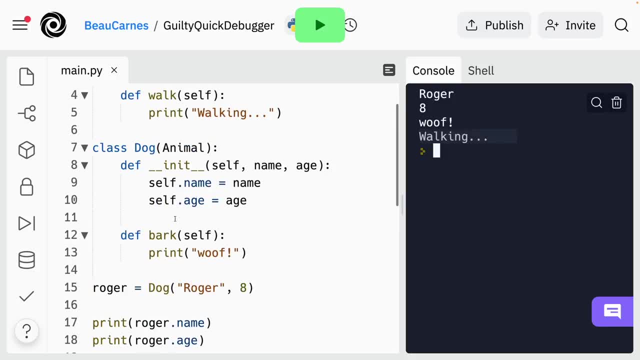 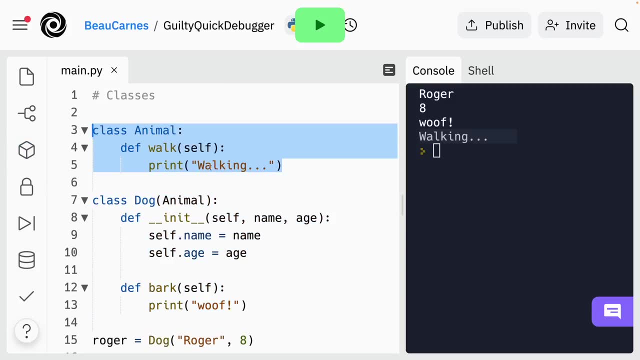 eight wolf, but now it's going to be able to do walking And you can see, the dog class doesn't actually have a walk method, but it's getting it from the animal classes inheriting this method. And in that way you're able to- I could create a class cat, class frog, a class bird, and each of them could inherit. 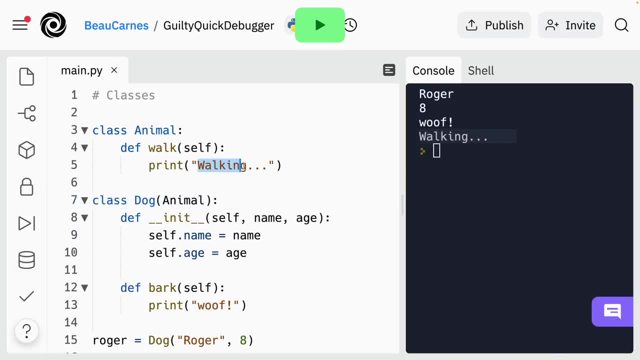 the walk method and then it would have walking And we'll be doing a little more with classes in the final project in this course, because we'll be going a little more over object oriented programming. But right now let's talk about something new. I'm 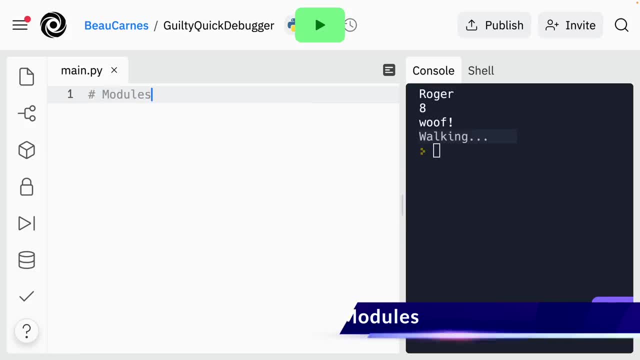 going to just delete all this And we're going to be talking about modules. So every Python file is a module. you can import a module from other files And that's the base of any program of moderate complexity, as it promotes a sensible organization and code reuse. So it's basically 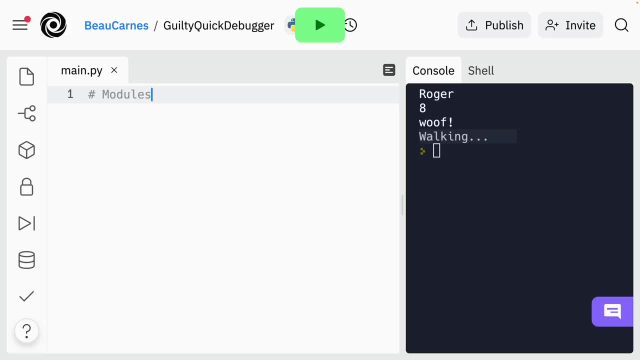 how you can create a software that has multiple Python programs in the same piece of software. So in the typical Python program, one file acts as the entry point And the other files are modules and expose functions that we can call from other files. So let me just show you an example. I am 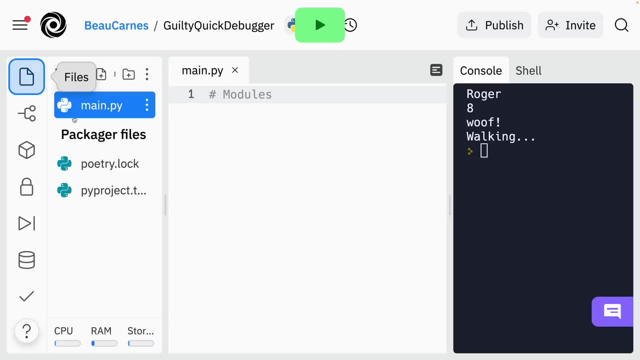 going to open up this files tab and I'm going to create a new file And this is going to be called dog dot pi. And now I have dog dot pi open. I no longer have the main dot pi open And I'm going 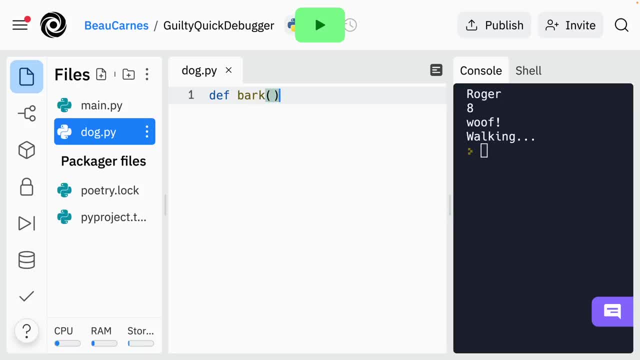 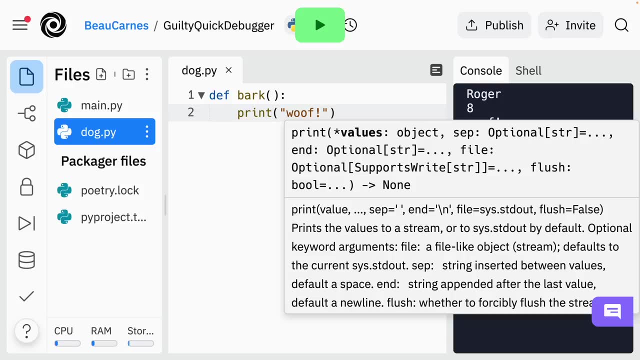 to define bar, And this is going to be called dog dot pi, And this is going to be called dog dot pi, And what bark is going to do is just print woof. Okay, now I'm going to. it's just going to. 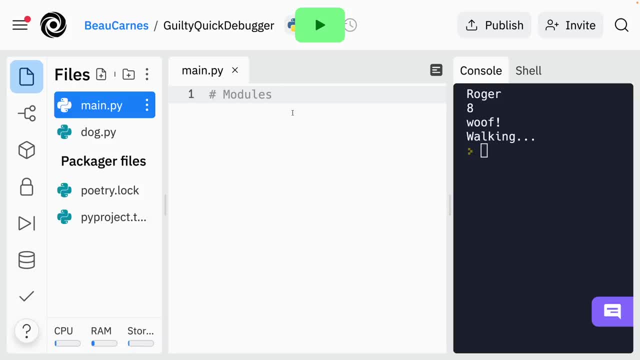 automatically save for me. I'm gonna go back to the Python file And now I'm going to import dog And let's see, oh, just saying it's unused. I thought maybe this thing wrong. But that just means I import dog and I haven't used it, which I'm about to do right now. So dog. 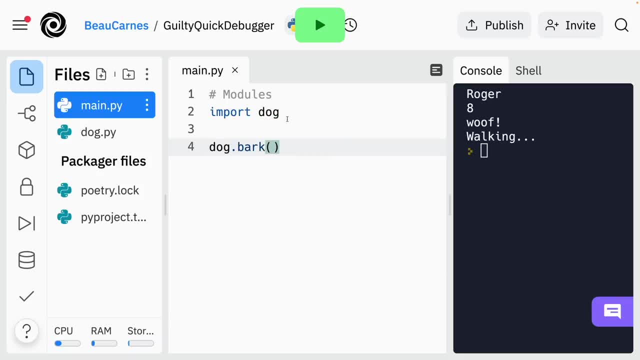 dog, And now I'm going to import dog, And now I'm going to import dog, And now I'm going to import dog And bark. So now, if I run this program, it's going to say wolf, but that's not from this file. 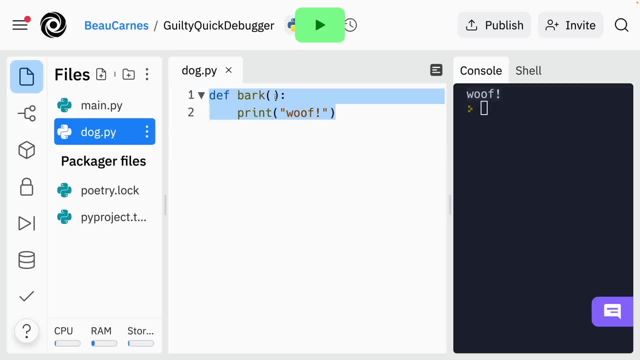 it's actually importing this function from from the dog file. So that's a way you can break up your code into multiple files. We can also use the from import syntax and call the function directly. Let me show you what I mean. So instead of import dog, I'm going to say: 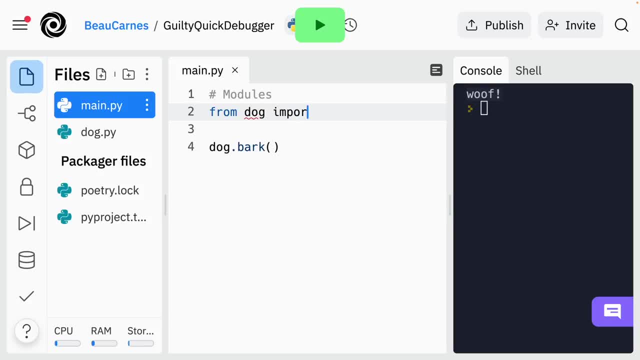 from dog import bark And then instead of calling a dog dot bark, I can just call bark, because we're only importing bark. well, we've imported bark directly instead of the whole dog, So I can run that And it says wolf. So that the first strategy allows us to load everything. 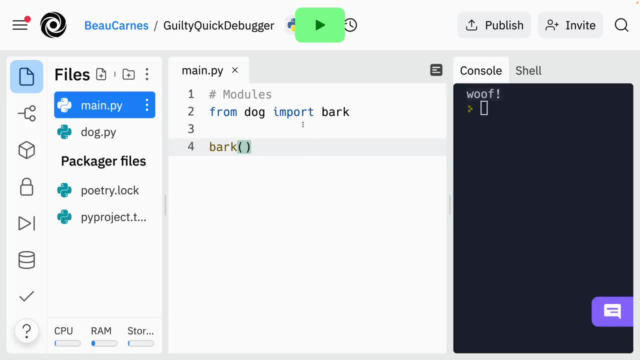 together And that's what we're going to do here. So we're going to import dog And then we're going to find in a file. when I just said import dog, that allows everything to find in a file. So I could have a bunch of function like bark or walk name, or there could be a bunch of functions If 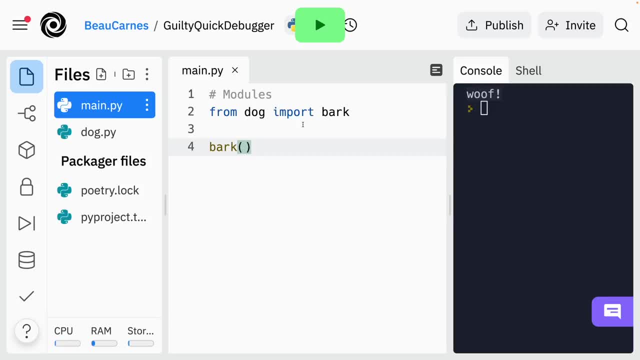 I just say import dog imports all of them. But the second strategy, from dog import bark allows us to just pick the things we need. So we're only going to import the specific functions that we need. Those modules are specific to your program And importing depends on the location of the file in the file system. So suppose you put dogpy in a. 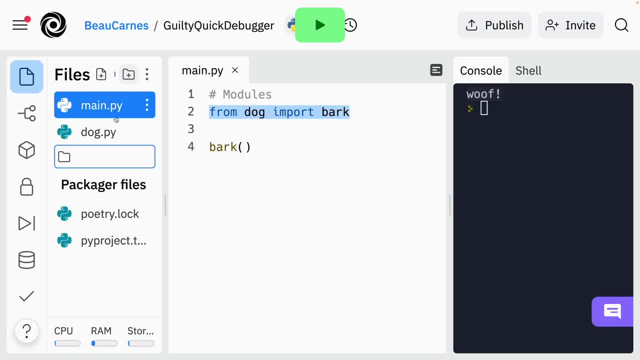 sub folder. For instance, let's say I create a folder and I call it live for library. And let's say I put dogpy in this sub folder like this: Now in this folder, to make this work, I'm going. 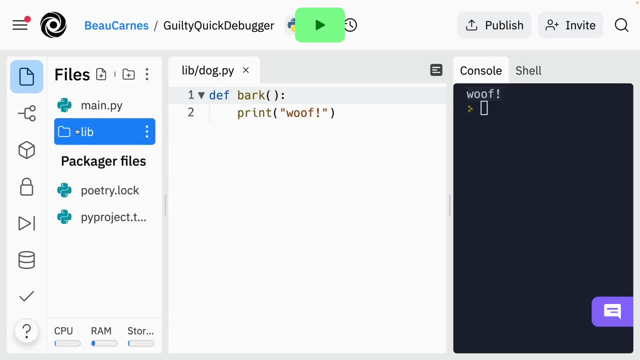 to have to create an empty file named init, dot, pi. So I'm going to add file and I'll do init dot or under underscore- underscore init, underscore, underscore dot, pi, And this tells Python that the folder contains modules. Now I'm going to go back to my main file And I 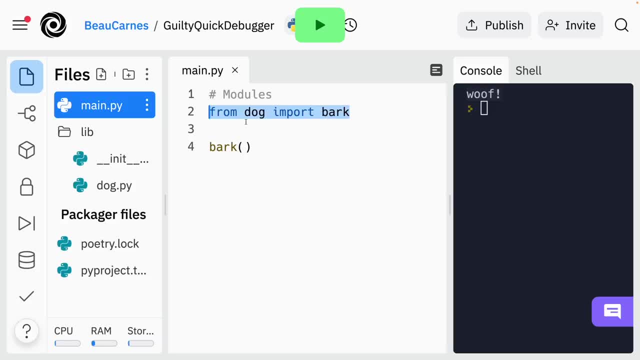 can. I can import dog from lib. So I'm going to say from lib, that's that sub folder, import dog, And then I can do dogbark. So let's run that to make sure there's no errors. it worked correctly So I was able to. 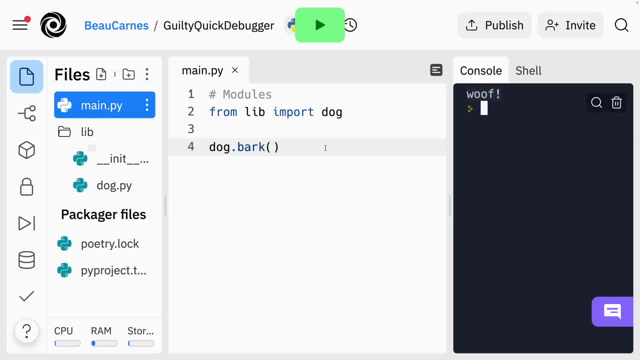 import this file from the sub folder Or you can reference the dog module specific function by importing from lib dot dog. So I can do: from lib dot dog, import bark. And now instead of calling dog that bark, I can just call bark And it says: 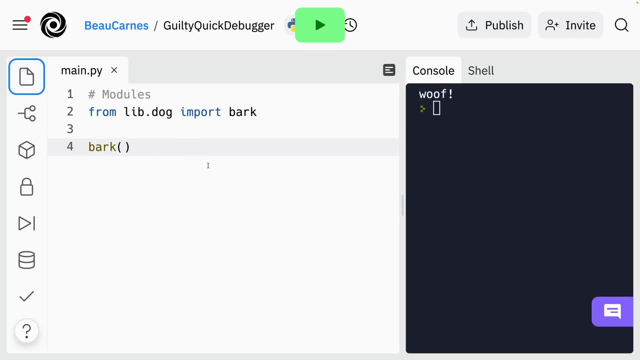 wolf. So I'm going to close this here And now let's talk about the Python standard library. So basically, there's all these pre built modules you can. you can load a lot of code from the standard library. Python exposes a lot of built in functionality through its standard library, The 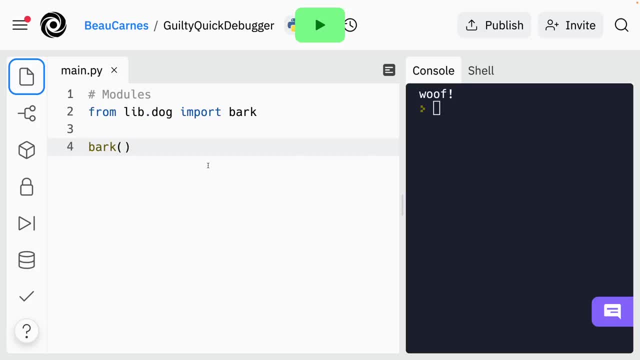 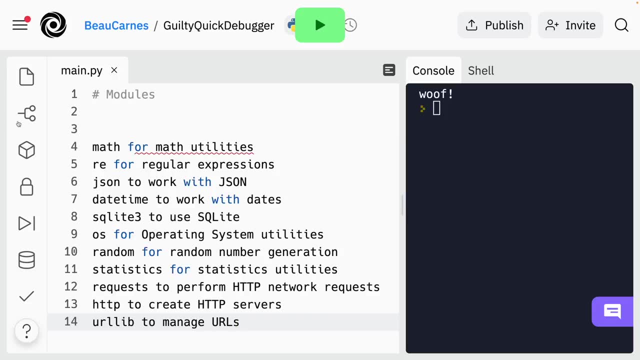 standard library is a huge collection of all sorts of utilities, ranging from math utilities to debugging, to creating graphical user interfaces. So there's a bunch of them, But here's some of the more common ones. We have math for math utilities, reef, regular expressions, JSON to work with JSON, datetime, SQLite- three OS for operating. 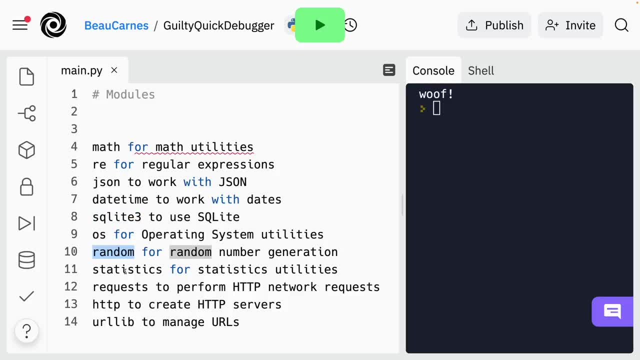 system utilities: random for random number generation. So statistics: requests for HTTP requests: HTTP to create servers, URL lib to manage URLs. So you can import these modules that allow you to get extra functionality. So we already looked at a little bit at the math one. we already looked a little bit at random in 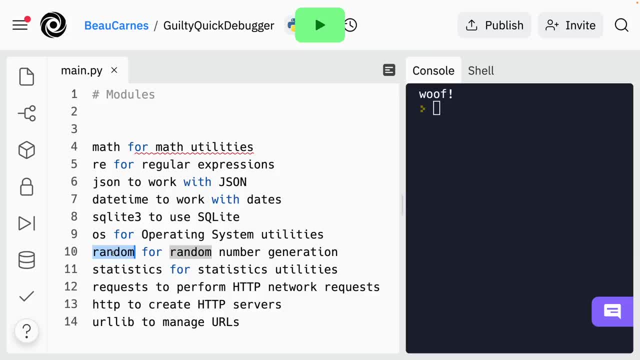 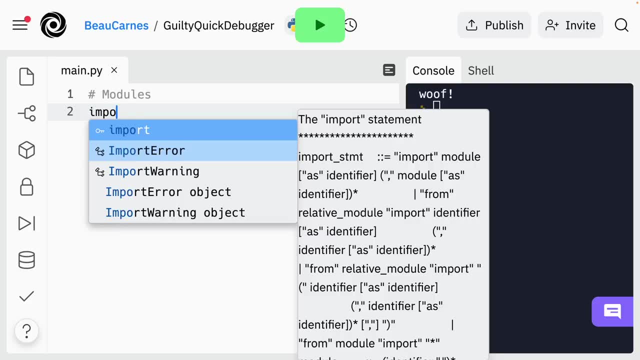 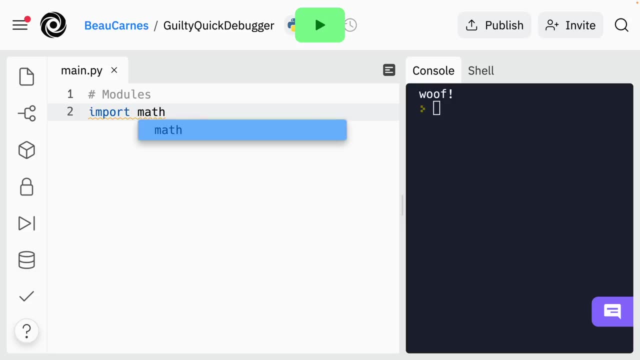 the first project that we did, But let's just kind of look at a little more how you would do this. So now we are going to use the math one, we're going to import math, And so this is how you would introduce: you would use a module of the standard library. So we already saw how to import modules. 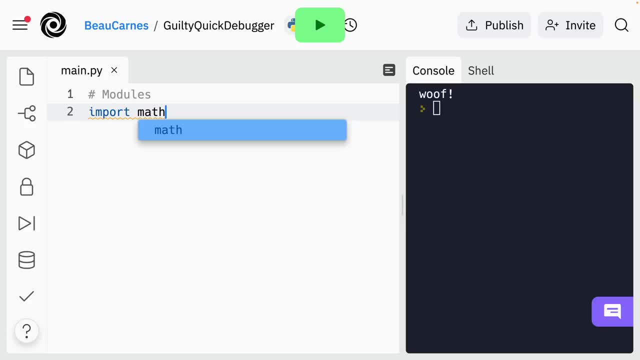 that we created. It's very easy. So we're going to import the modules that we created And then we see it's very similar with the standard library. So now that I've imported math, I can now use functions and methods from from the math module. So I can do math, dot, square root and I can pass. 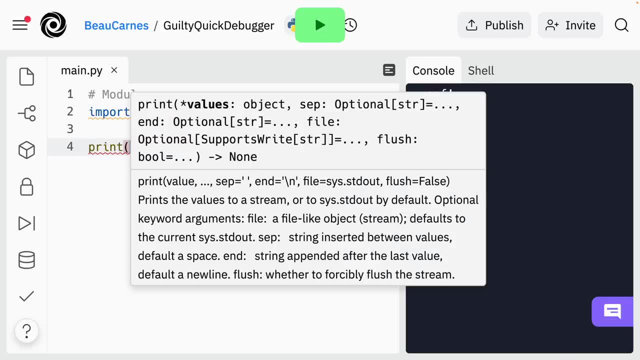 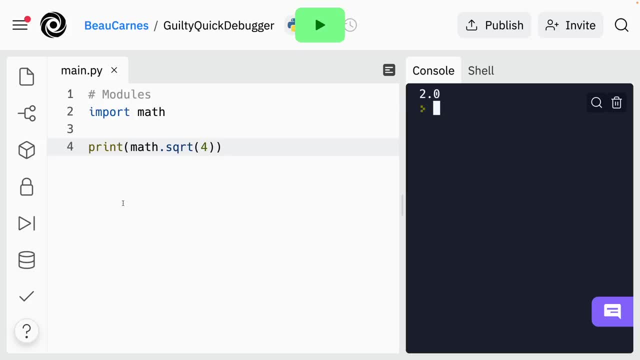 in four And then I can just print that so we can see what the result is. Okay, 2.0.. Or we can just like we shall. we saw before, instead of importing math, I can say from math, import square root, And then, instead of just doing math, dot square root. 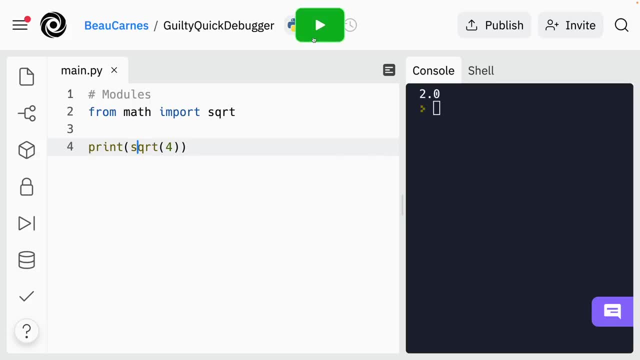 I can just call this square root method here, And it's going to do the same thing. So that's basically how it works for all the modules in the standard library. Okay, now we're going to start going over a few kind of miscellaneous, slightly more advanced topics in Python, So we're going to 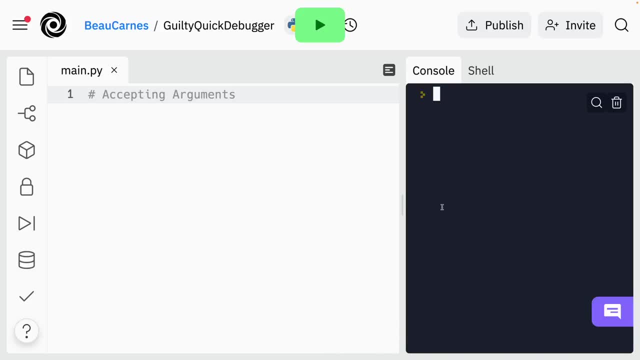 talk about how to access the standard library, And then we're going to talk about how to access the standard library, And then we're going to talk about how to access the standard library And arguments from the command line in Python. Well, first of all, let's see how to run a program from. 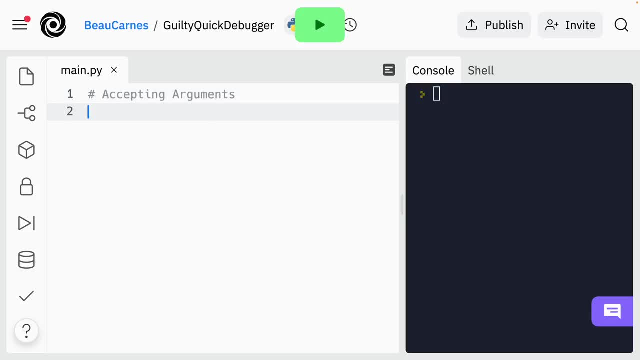 the command line in Replit. So let's say we have a program. it just says print Hello, Okay, so we've been running it by just clicking this play button. But there's another way to run a program in Replit. 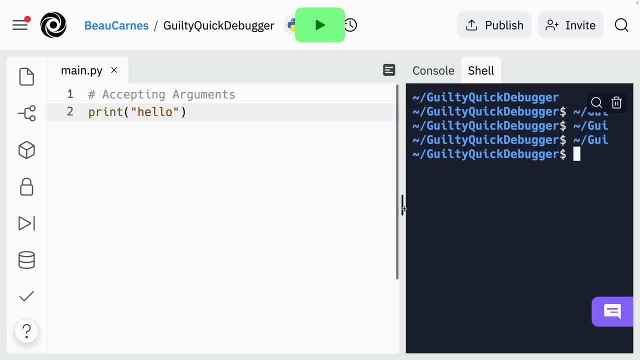 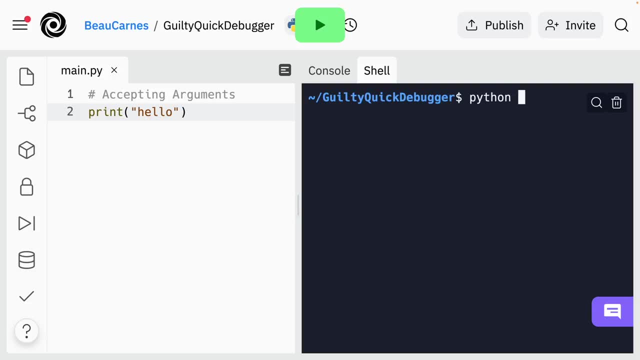 And I go over to the shell. So this is the command line in Replit. we can clear this, And now I'm just going to type in Python: main dot pi. Okay, so we call Python to run the Python program, And then 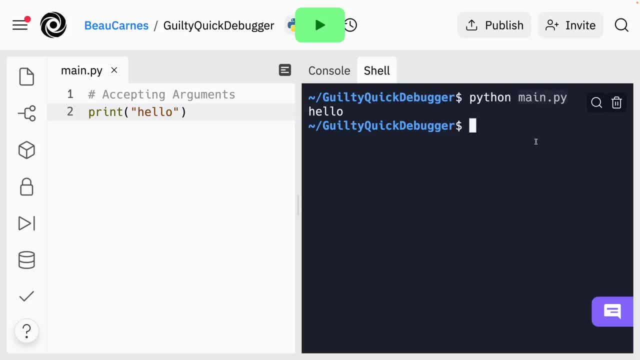 we just put the name of our file with main dot pi. So whether you're in Replit or if you're running things locally, you should be able to run a program in the same way, Depending on how you install the program locally. instead of typing Python, you may type in Python three sometimes. 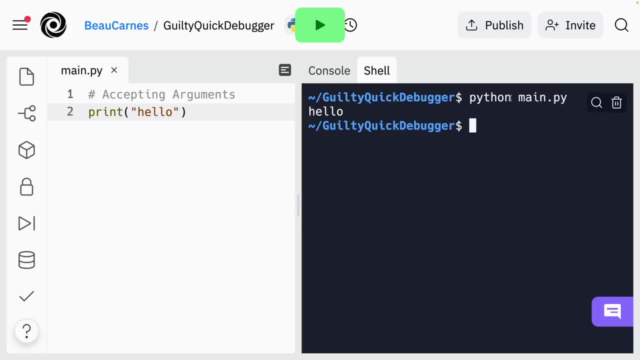 the way people install Python. it will be Python three, because we're using version three of Python. So now let's see how you can call a Python program on the command line and pass in some arguments right when we run the program from the command line. So a basic way to handle arguments is: 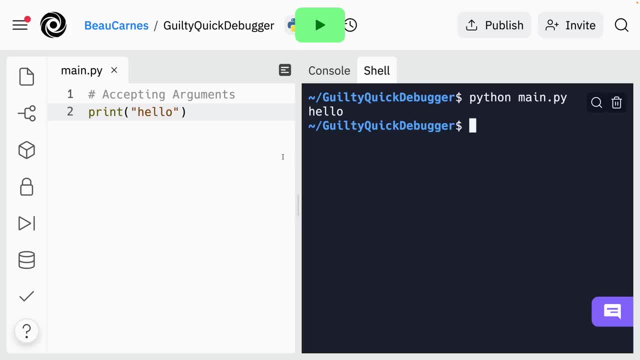 to use the sys module from the standard library. So let me give you an example. So let's say we're going to import sys Now, just so you know, usually you're always going to have import statements on the first line. I'm just putting this comment on the first line to remind us what. 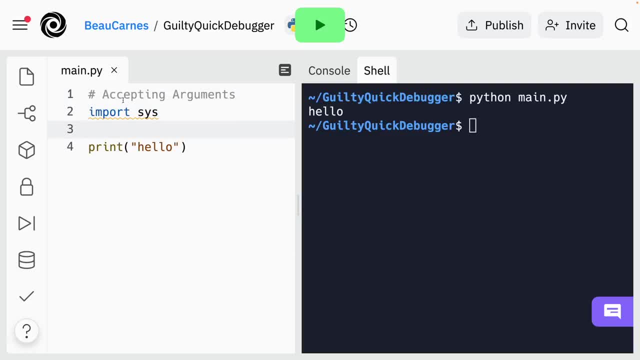 we're working on right now. So now I'm going to, we're going to import the sys library. Now I'm going to print And I'm going to. first I'm going to, Oh, we're going to print the argument sysorg. 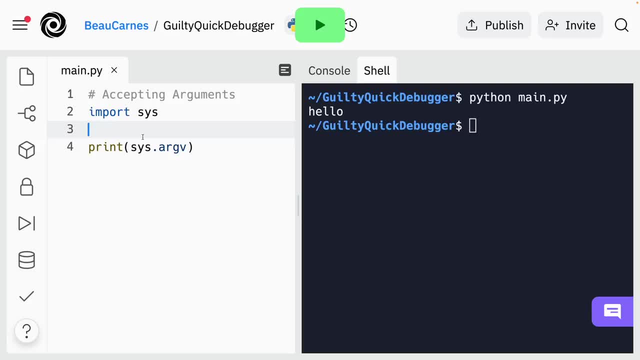 the. so this is how we can print all the arguments that were passed in what when we call the program. So. so I'm going to see we have Python, main, dot, pi, And now I'm going to put bow 39.. Okay, so you can. 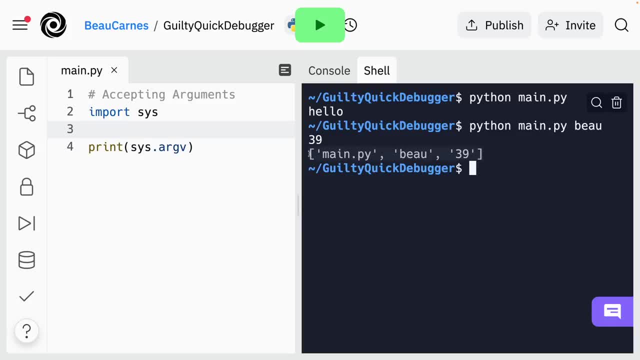 see it's printing the list of arguments. So this is basically just a list. The first item is the name of the file, then we have the first word and then the second one, And you can see they're both strings. even though this is a number, it's coming in as a string. So 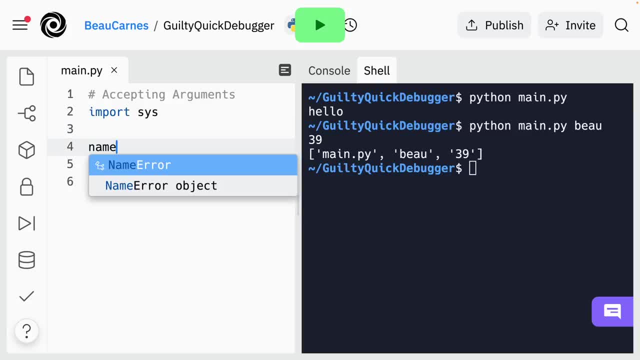 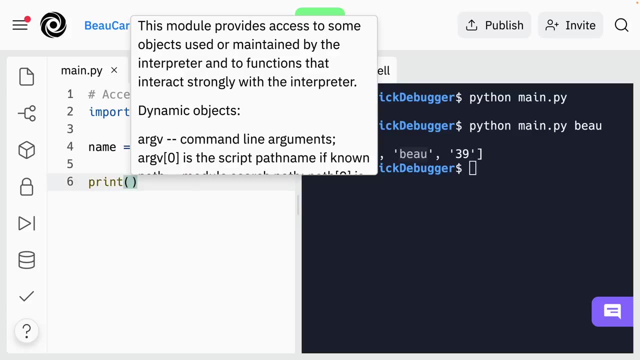 then we could do something like this: we could say: name equals sysorg v, And then I would get the element at index one, which is the name here, And I could print Hello. And then we're going to do a name, And then we're going to print hello, And then we're going to do a name, And then we're. 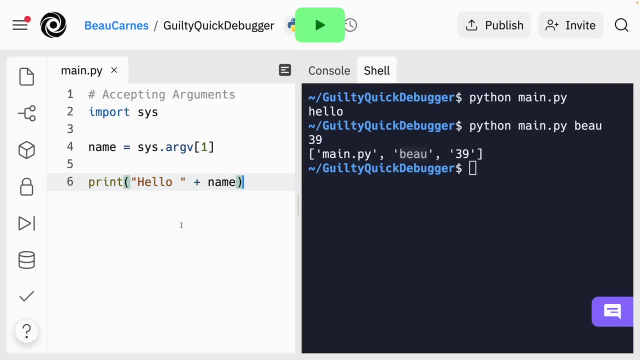 going to print hello, hello and the name. So let's call this again And instead of- I'm not going to do 39, is this going to be Python main dot pi bow, Hello bow. So we've now been able to use the argument that was passed in. Now, this is a simple way to do it, But you really would. 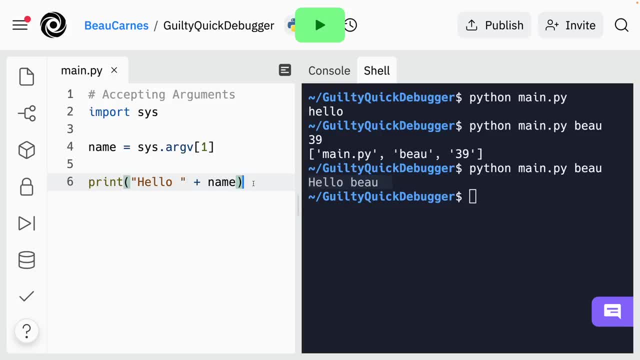 have to do a lot of work using this method, Because you really should validate the arguments, make sure their type is correct and need to print feedback to the user if they're not using the program. So we're going to print the argument And then we're going to print the argument And 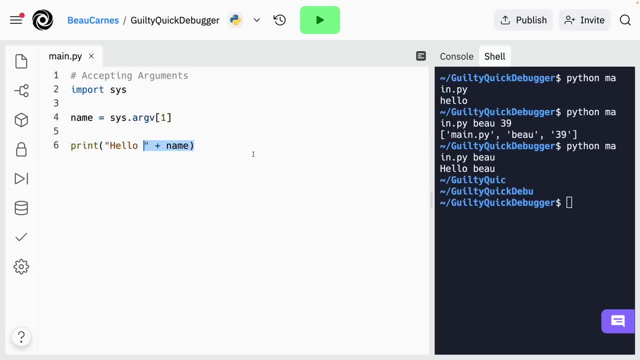 then we're going to submit feedback to the user if they're not using the program correctly. zoomed out a little bit And I'm going to show you this other method. So Python provides another package in the standard library to help you, called arg parse. So first you would insert import our 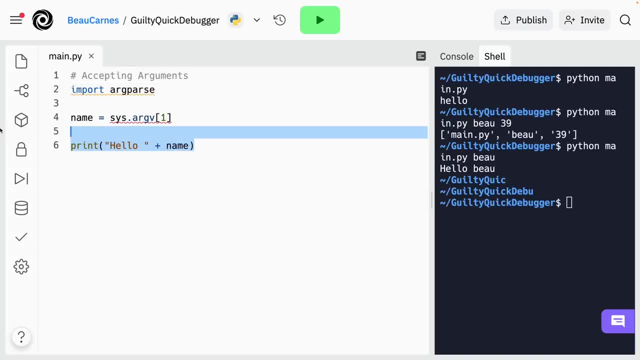 parse And then let me show you how you would use it. So you call our parse dot argument parser and then pass in the description of the program. So the description of the program is: this program prints the name of my dogs. then you proceed to add arguments you want to accept. So for this. 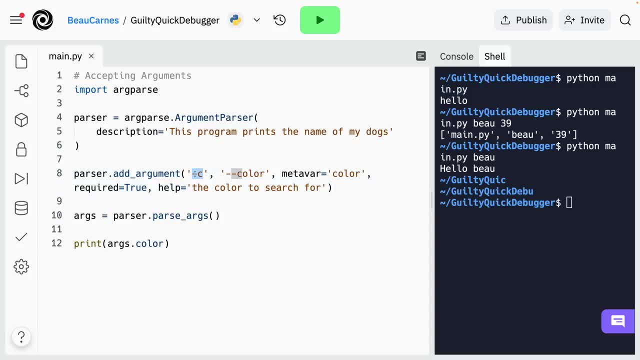 example program. we are going to accept the C option or it can be slash, slash dash C or dash dash color And we are going to be calling it color and then later we can we do parser dot dot, parse args And then we can add access args dot color to get the color that was passed in. 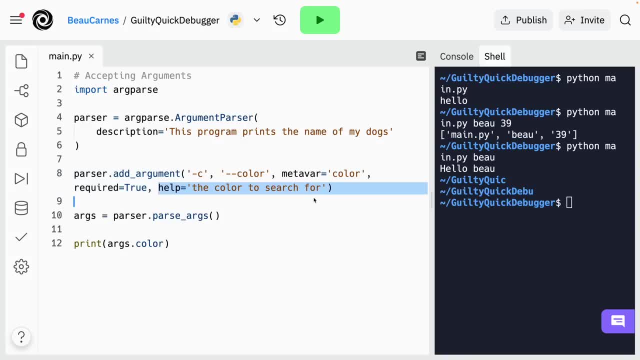 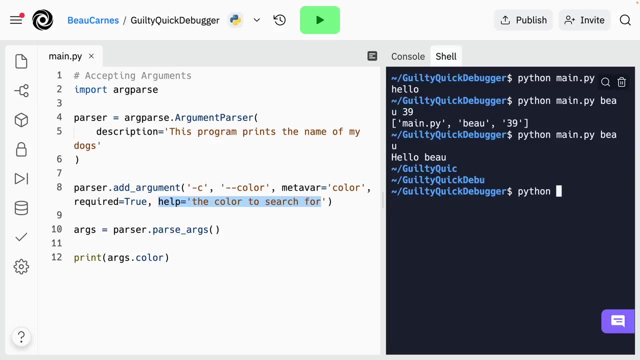 And then you can specify whether it's required and what help is going to go along with that. So let me show you how you would do that. We're going to do Python, main dot pi, I'm gonna put dash C and then I'm just going to put red. Okay, so you can see if I go out a little more. you can see. 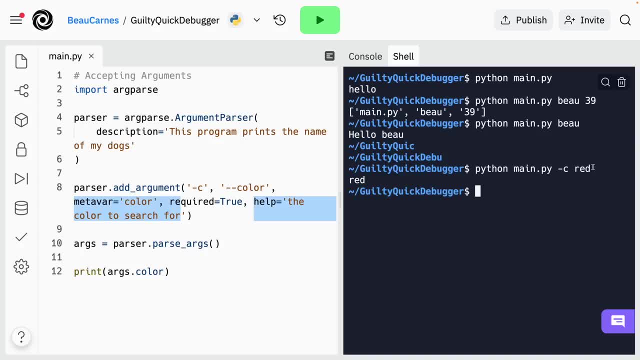 this is the command I call, this is the command I run, I pass in red and then it just printed red. So we have right here. And so let me show you what would happen if we, if we don't specify the argument, So if I just run it without the red. so it's now giving me some information usage. well, 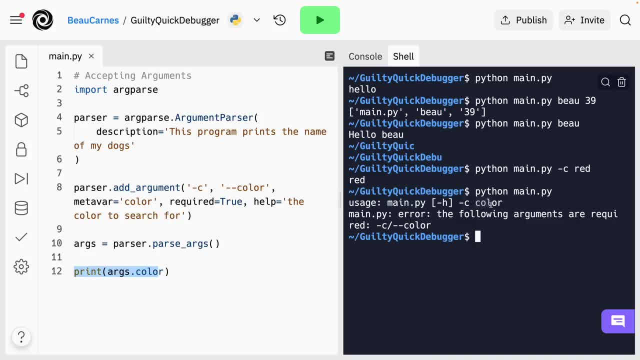 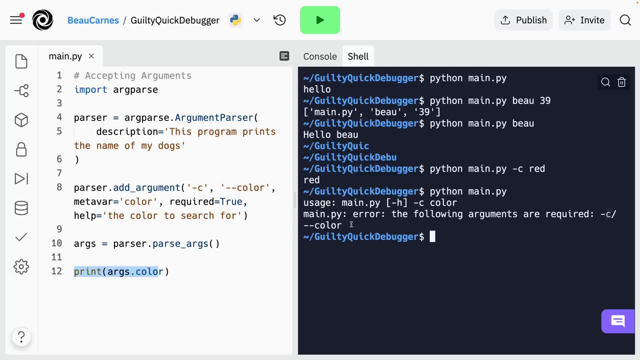 main dot pi. we need to put dash C and then we have to put a color, And then it says the following arguments are required: this dash C or dash SC. So it's, it's showing us that we need to if we've 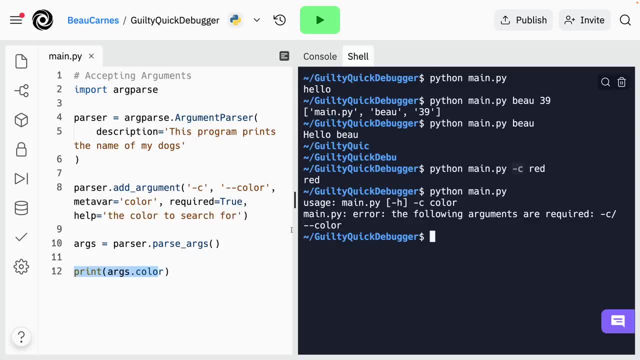 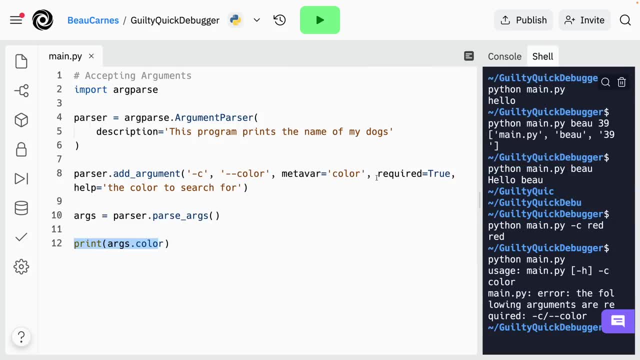 called the program wrong and we're going to need to call it with a dash C. you can also set this option. we can set an option to have a specific set of values using choices. So, after required, true, after this comma, I'm going to type in choices And I'm going to set this to equal. 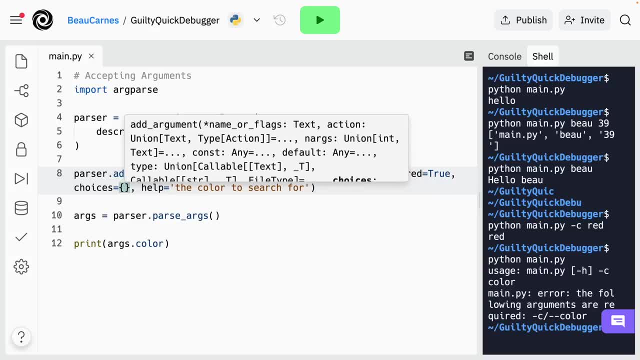 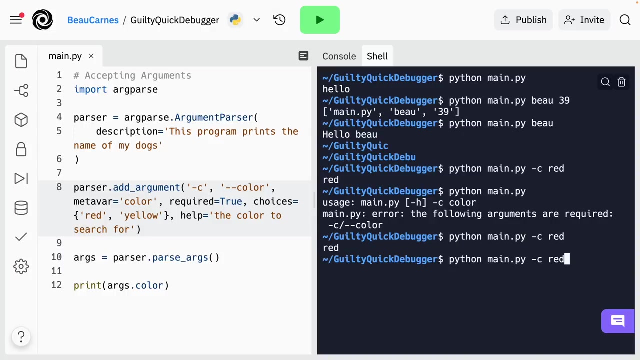 Sadie, this empty dictionary- but I'm just going to learn how dictionary- but because there's not going to be a key value pairs when you do red and yellow. So now it's, it can only accept two options. So I can call it here with red, But if I call it with blue it will say invalid choice. 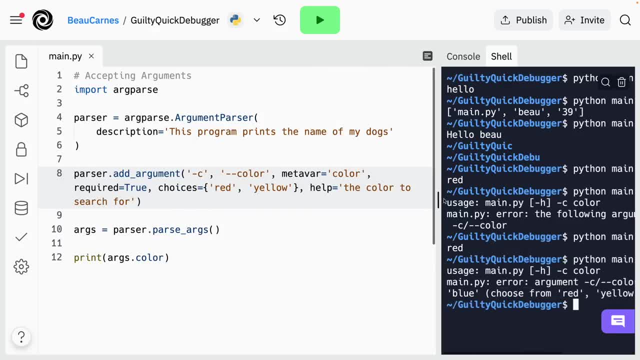 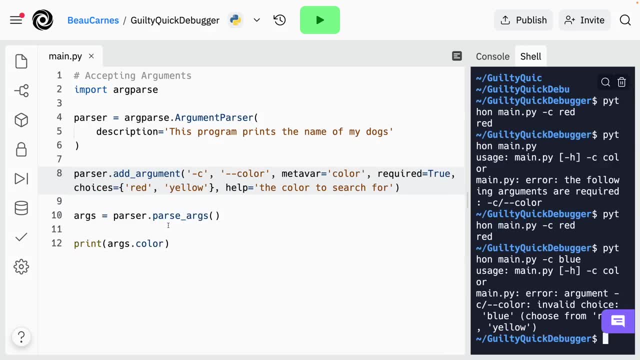 blue. I need to choose from red or yellow. So using this arg parse makes it easier to deal with arguments And also it makes it easier to communicate information back to the user about what we're trying to get. So there are more options with this, But those are. those are the basics Now. 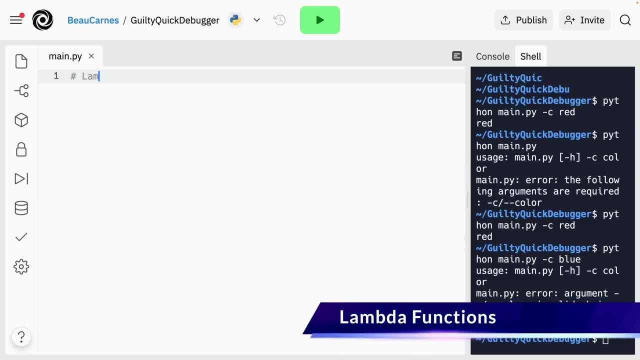 let's talk about something completely different: Lambda, lambda functions. So let me just give you a quick example: Lambda num- num times two. So lambda functions, also called anonymous functions, are tiny functions that have no name and only have one expression as their body. So they're. 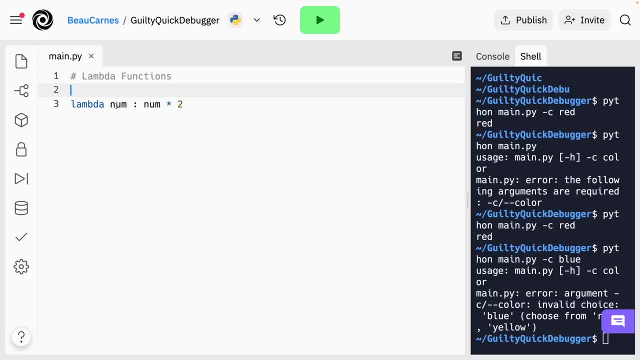 defined using the lambda keyword, And so this is going to be the argument And this is going to be the expression. The body must be a single expression And it has to be an expression, not a statement. So this difference is important. and expression returns a value. a statement does not, So it has to return. 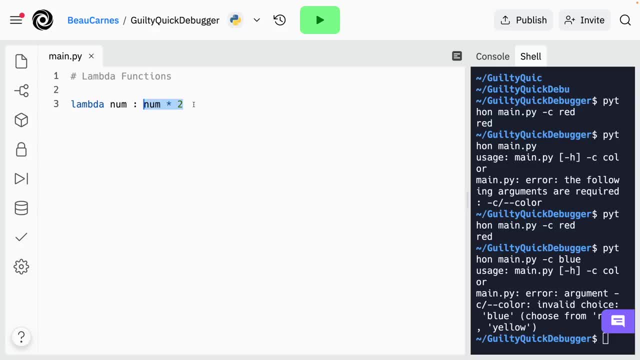 a value. So the value is being returned is the number times two. the number that was passed in is going to multiply it by two in this example. So this is basically the simplest example of a lambda function. it just doubles the value of a number, And lambda functions can accept more arguments. So 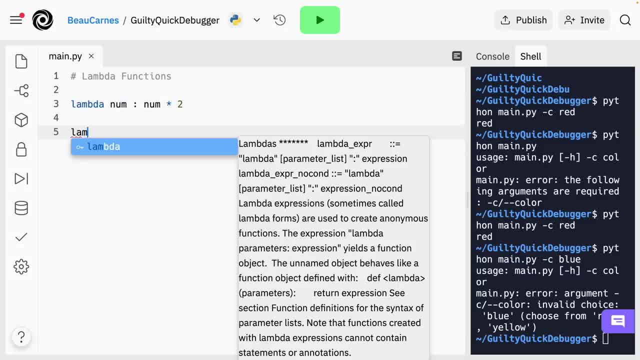 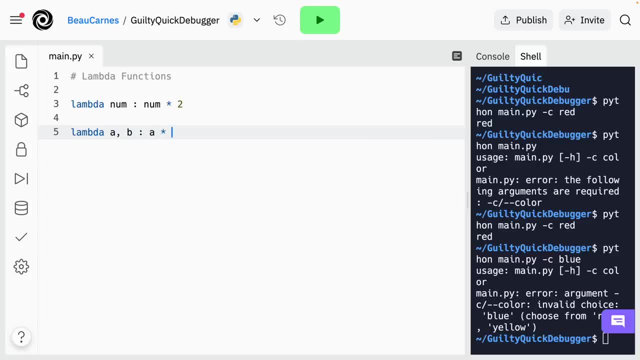 so, for instance, I could do lambda a, comma B, and then we can multiply A times B. Lambda functions cannot be invoked directly, but you can assign them to variables. So for instance, I can assign this to the variable called multiply. So multiply is going to. this function is going to be assigned. 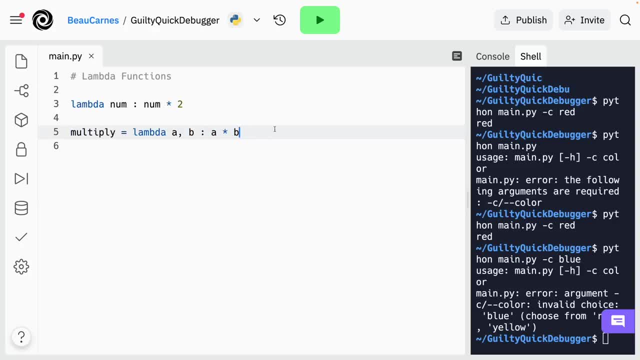 to this variable here. So for instance, I could do lambda a, comma B and then we can multiply a times B, So for instance: So then the way that I use that I could print now I'll print the result of calling multiply. 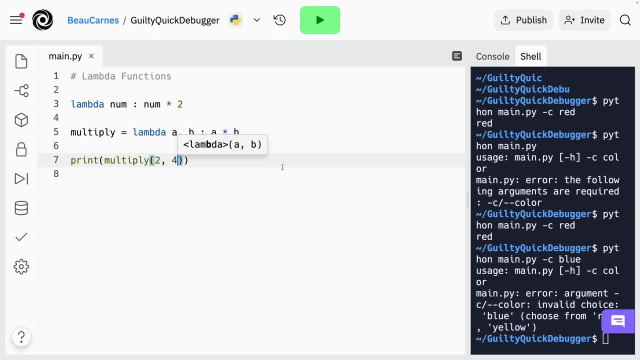 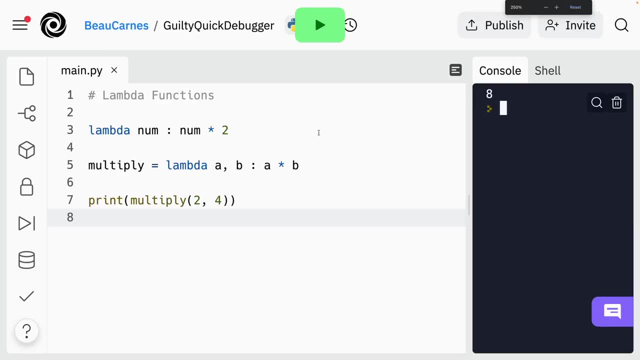 And then I pass in two and four. So if I just run that, okay, two times four is eight. we can see right in the console here, And I'm going to just zoom in just a little bit. So the utility of lambda functions comes when combined with other Python functionality. 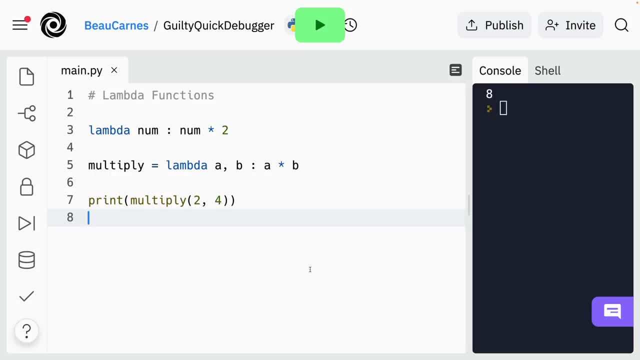 for example, in combination with map filter and reduce. So, speaking of map filter and reduce, that's what we're going to talk about now: map filter, reduce. So Python provides three useful global functions we that we can use to work with collections. So this is map. 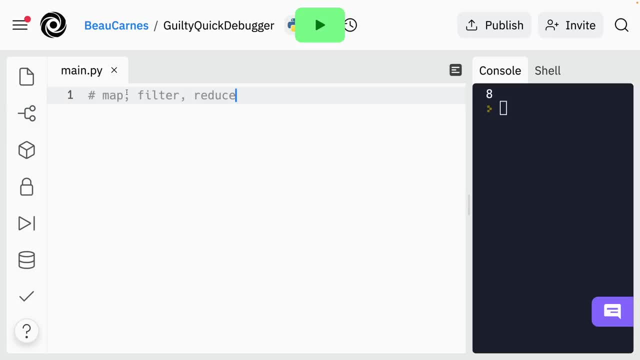 filter and reduce. So first let's talk about map And since they're functions, are going to have the parentheses at the end. So map is used to run a function upon each item in an integral item like a list, and create a new list with the same. 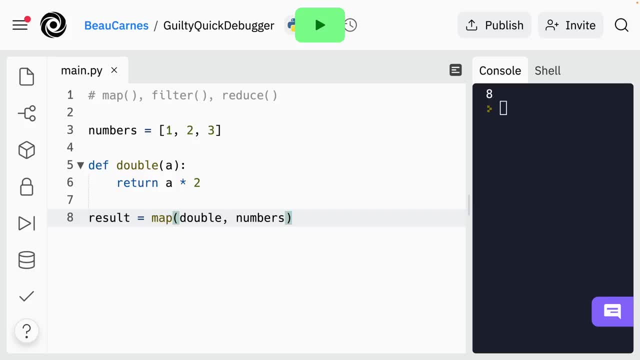 number of items, but the values of each item can be changed. So here's an example: we have this list, And then here's the function, And then we are going to map through each item in the list, And so here's the function we're going to run. we're going to run this function. 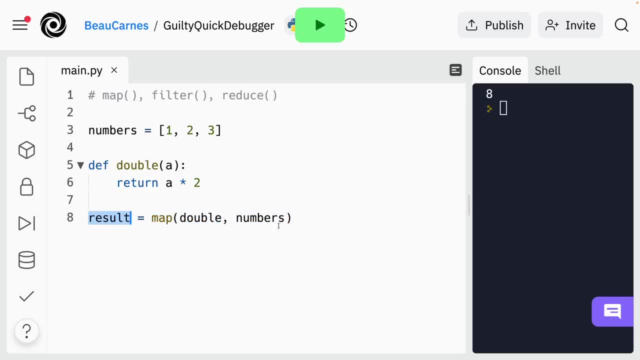 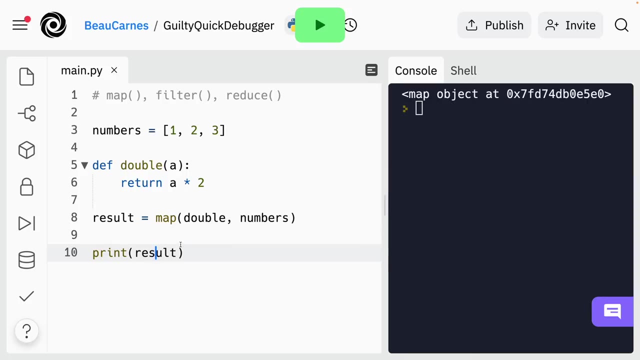 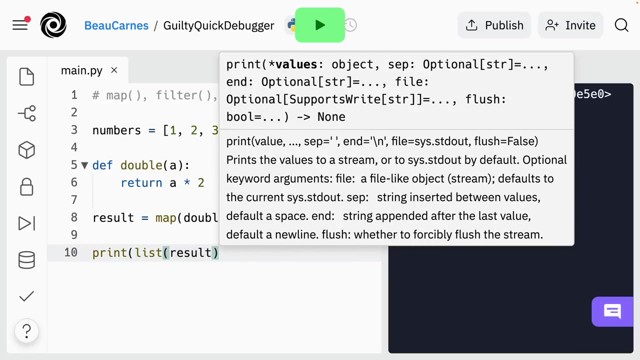 on each item in the list. And now we're going to get a new list So I can do a print result. Now, if we print that, I'll just run that function And we can see. okay, we get a map object. So then we can always just pass it into the list function And then 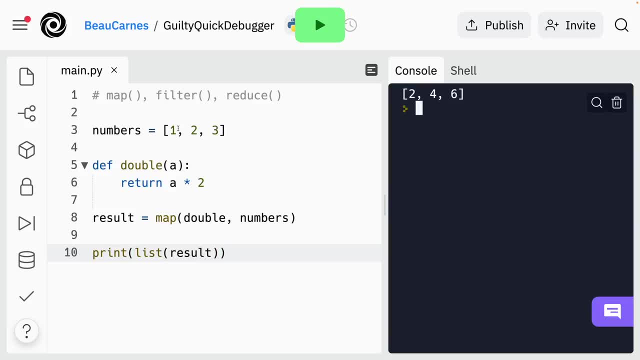 we can run the program again two for six. So 123 became two for six. So yeah, whenever you want to do run a function on each item in a list, you can use map, And when the function is a one liner, it's common to use a lambda function. So remember. 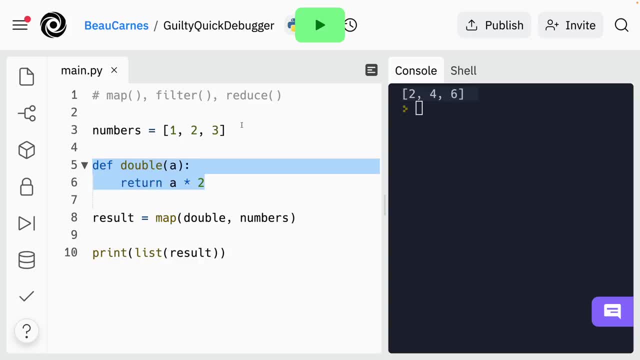 we just talked about lambda functions, So now let me show you how you would do this as a lambda function. So double is going, this is going to be a variable and we're going to assign it to a lambda function, And I'm going to. so now this lambda function takes: 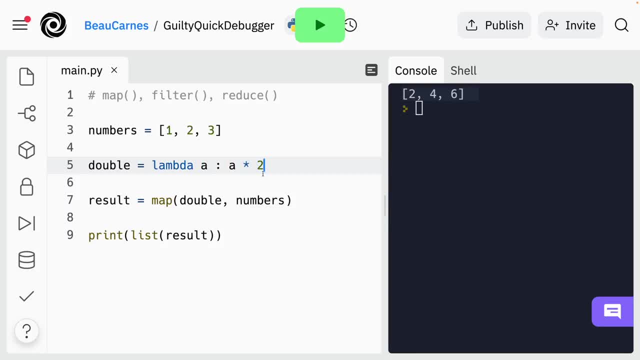 the number a and then does a times two. So and this we just keep the same, because now we're using a lambda function here And we're taking each number and passing it through the function where we have the the. this is each number in the list and we multiply it. So if I run this program it should look exactly. 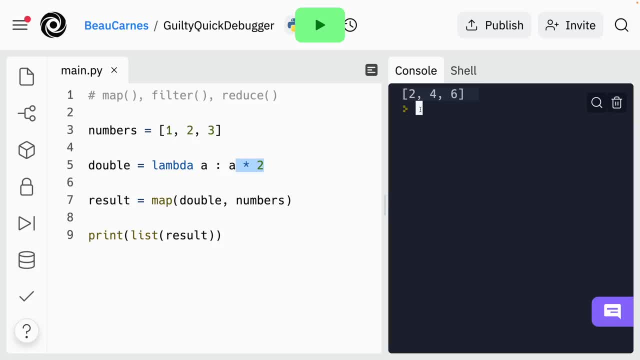 the same, And we can even simplify it even more. So this is where lambda functions really shine. Instead of assign it, assigning it to double, first, I can copy the whole function, I can delete this completely, And now I can just put it right in here. So now we're mapping over this function And we don't even have 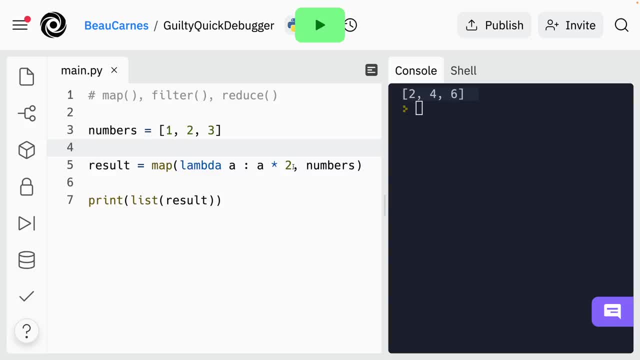 to create the function in a different line and assign it to a variable. First we can put the lambda function right in the same line, right within the map. And now I run this and it's going to give us the same result. So remember we started with. when I first showed you this example, we had a much longer. 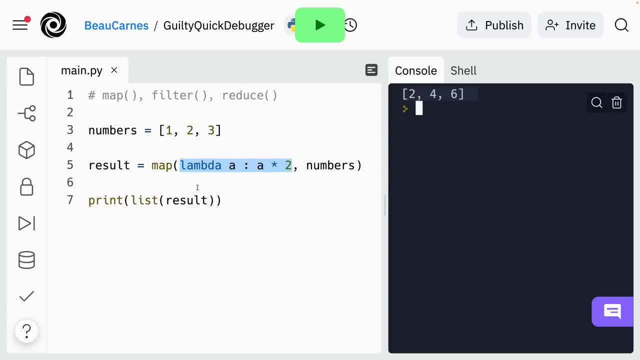 piece of code. Now we've simplified it with the lamb lambda function, So the original list- the original list- is left untouched And the new list with the updated values is returned by map. the result is a map object which is an iterable, So that's why we needed to cast it to list, to. 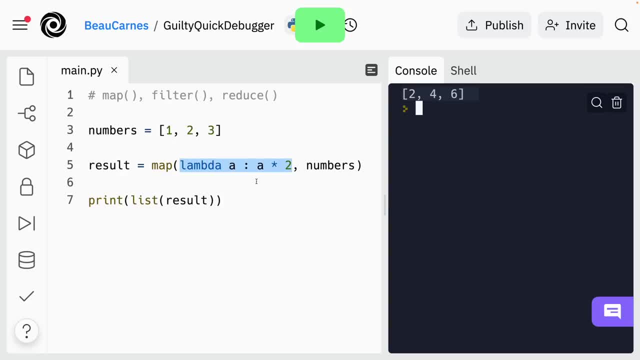 print its content. Okay, now let's talk about filter. Let me put in, let me just update the code here. It's kind of similar, But now we're using filter. filter takes an iterable and returns a filter object, which is another iterable, but without some of the original items. So you can. 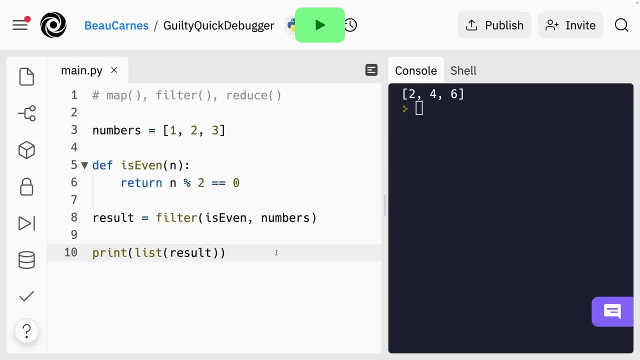 do so by returning true or false from the filtering, the filtering function. So here's the filtering function. we are going to check if the item passed in is even so. So here's the list here. So you can see. we're calling filter, we pass in the function, the filtering function. 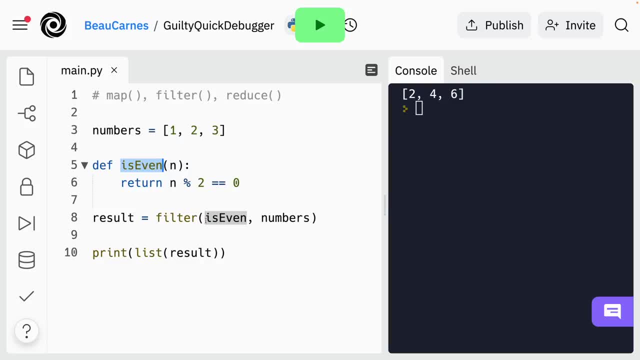 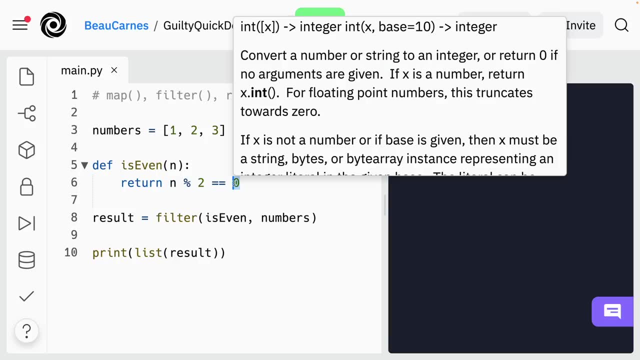 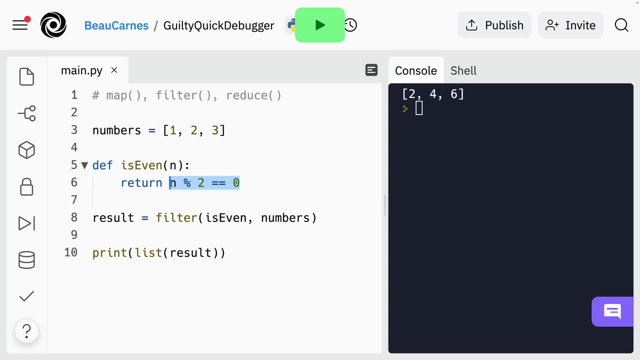 and then the list, And we're going to return true or false from the function. So, if it can be, if it's divisible by, if, when you divide it by two, we have zero remainder, then it's even So. that would return true. So this line would return true. And then, if not, 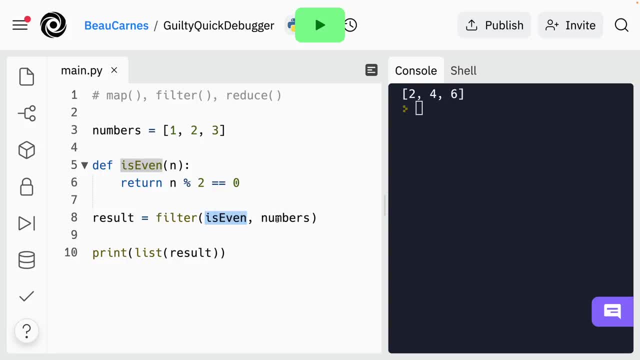 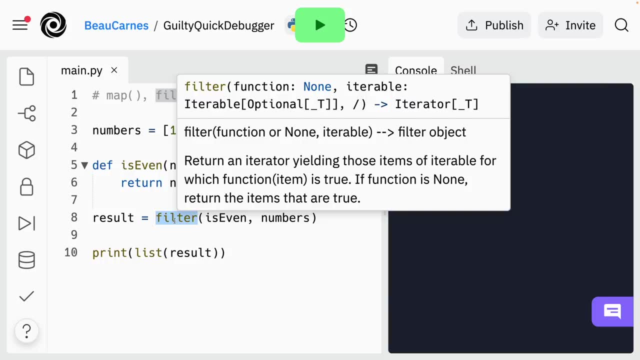 it would return false if it's odd. So now any even number is going to be added to the result, And any odd number is not going to be added to the result. So basically, we're filtering the list based on this function, And then here we just. 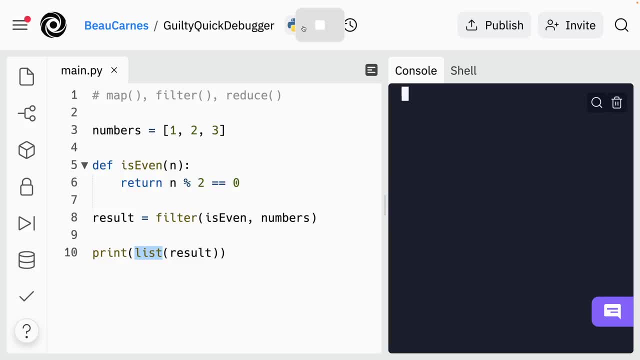 print, we convert that result to a list And if we run that it's two. And obviously, if we can just put in more numbers here and run that again, we have 246.. And then we can just like before. 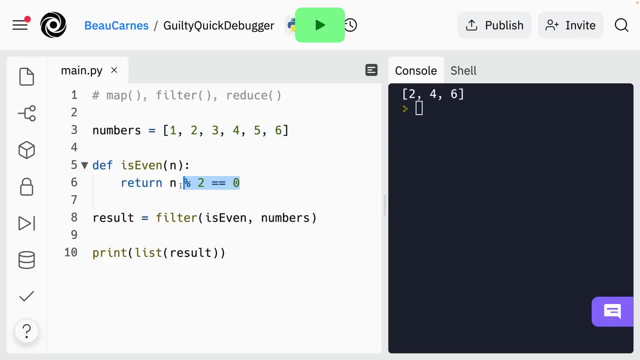 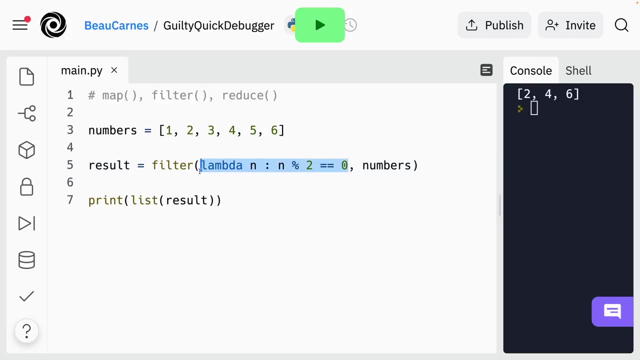 we can use a lambda function. So I'm just going to copy this here. we can just delete this whole thing And we are going to put a lambda function here. So lamb duh. So now you can see, we're just putting the lambda function in the in line here And we are checking. 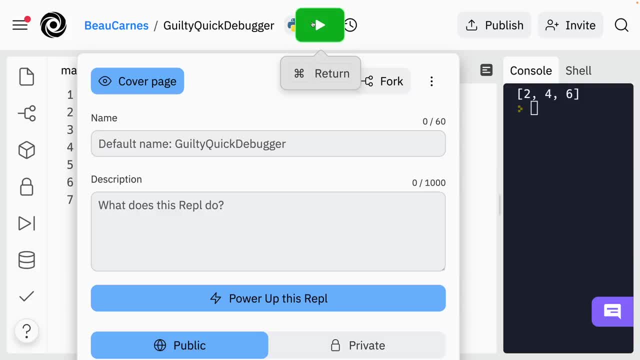 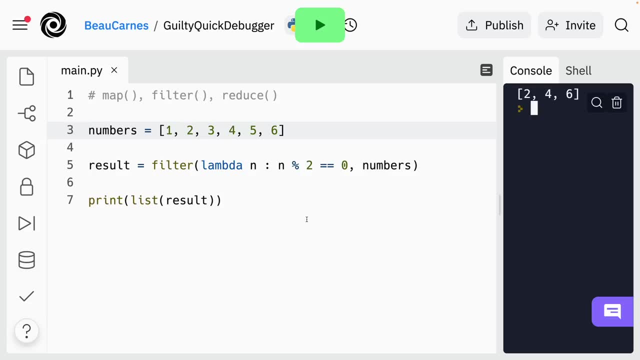 to see if this is going to turn true or false, whether it's even or not, And so I run the program and it's going to give me the exact same result here. Okay, the final thing we're going to talk about is reduce. reduce is used to calculate a value out of a sequence like a list, So for 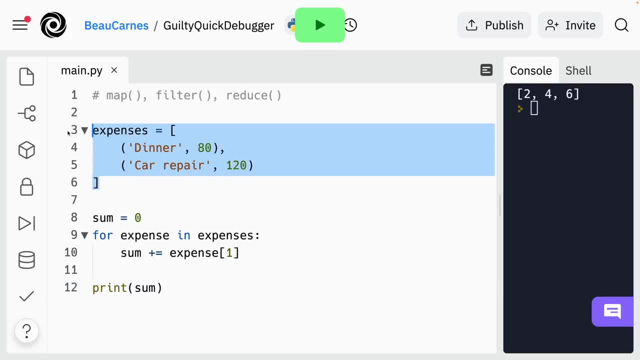 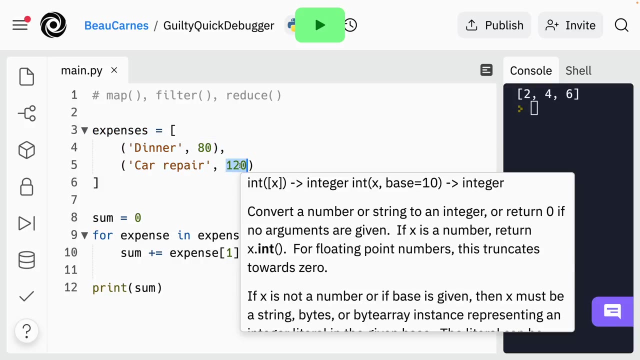 example, suppose we have this list of expenses stored as tuples, And so so we have dinner at 80, car repair 180, or 120. And we want to calculate the sum of this property in each tuple, in this case the cost of the expense. 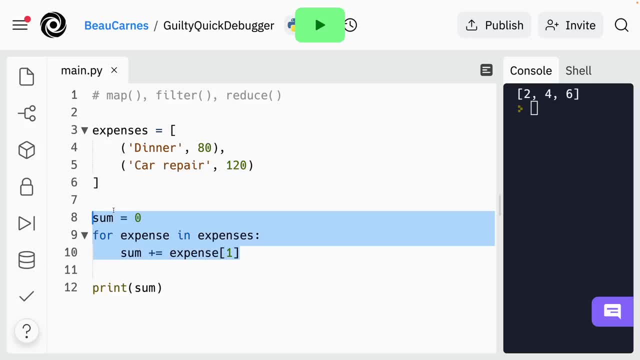 So here's kind of the long way of doing it without using reduce. we basically take every expense and expenses And then we add to the sum here and we add expense one that's going to be the, the item at index one, and then we get the sum and we can print the sum. So that's kind of like. 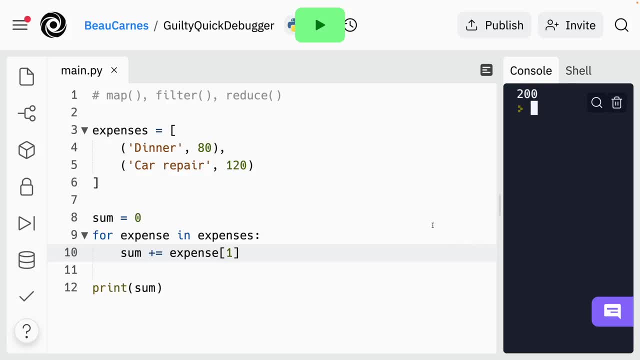 the long way of doing it without reduce, But there's a quicker way. So to use reduce. reduce is a little different from map and filter. where it's not available, It's not. it's not available automatically. we have to import it from the standard library func tools. So I'll do from func. 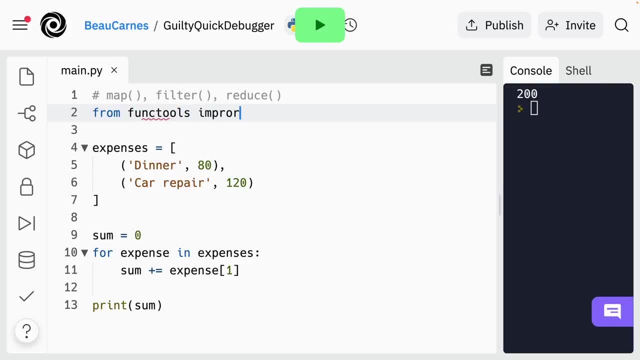 tools or function tools: import, reduce, And now I'm going to create a new. I'm going to create a new variable called sum And we're going to set it to reduce. we're going to use reduce And now I'm just going to. 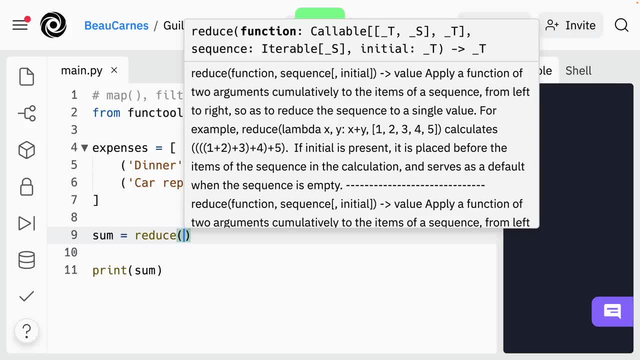 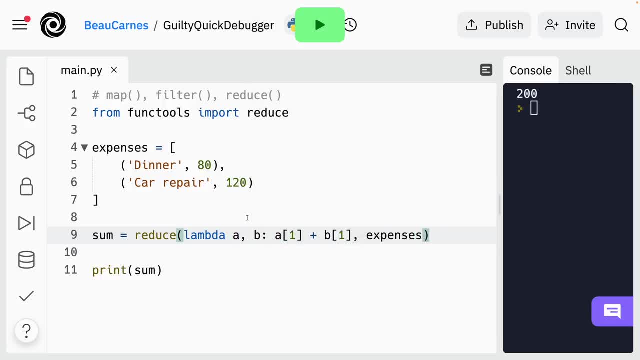 pass in. I'm gonna go directly to the lambda function. So, lambda, let me just kind of explain this for a little bit. So reduce, the first is going to take a function, the reduction function, and then the interval here, and the function has to take two. 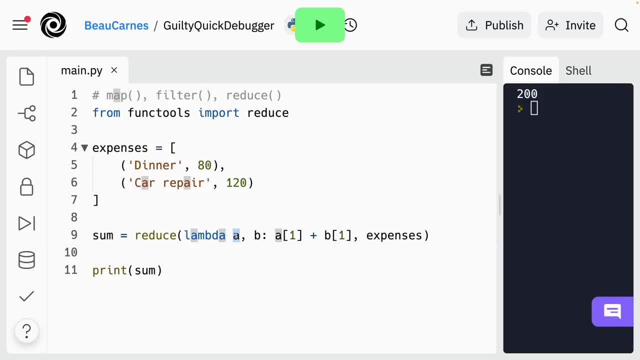 arguments. So this: the first argument is the accumulated value And then the right argument is the updated, the update value from the interval. So we're going to continue adding these two items. we're going to basically add every item together and reduce the item, the numbers at the first. 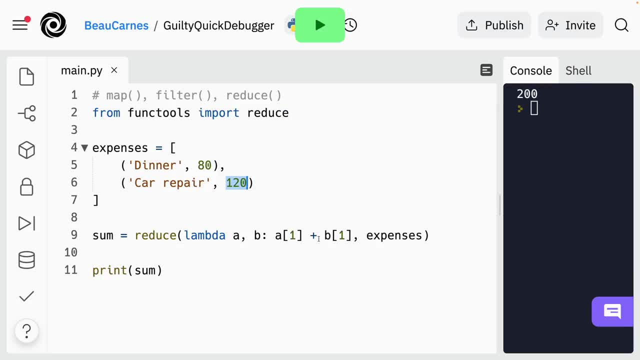 index all into down to one value by adding them all together. So just pray here, play here, and then we get the same number, 200.. And you can see it's a lot. it's a lot quicker just to use the reduce function compared to the other code we have previously. Okay, next up we're going to talk. 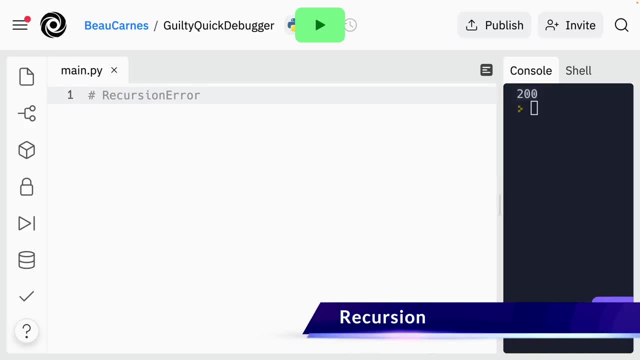 about recursion in Python, not recursion error, just recursion, And a function in Python can call itself. that's what recursion is, And it can be pretty useful in many scenarios. A common way to explain recursion is by using the factorial calculation, So let me show you how you would. 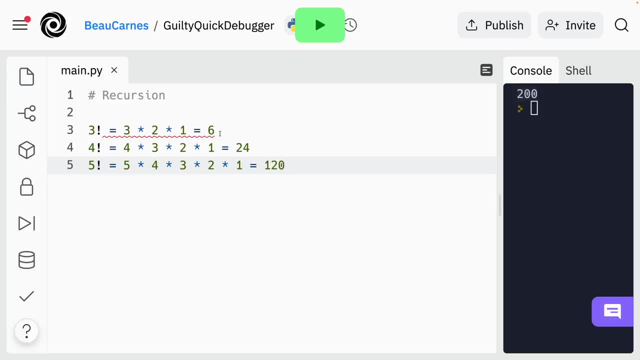 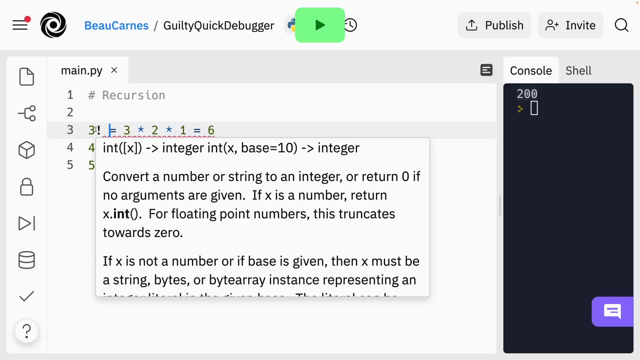 calculate factorial. This isn't Python code, this is just an example here. So a fact: when you do three factorial, that means you do three. you multiply it by two, you multiply it by three, every number between three, between this number and one together. So three times two times one. 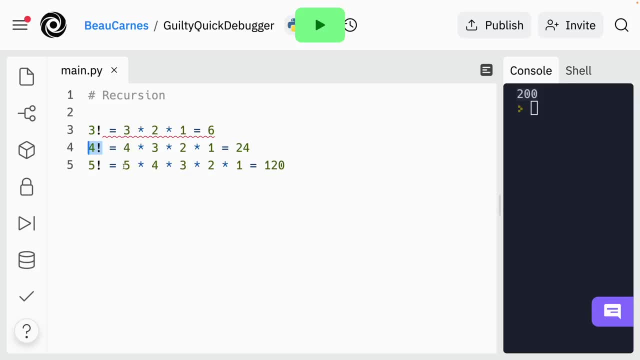 equals six. four factorial is four times three times two times one, five factorial, and you know, five through one and so on, And every number, you multiply, every whole number down to one. So using recursion, we can write a function that calculates the factorial of any number. So let me show you. 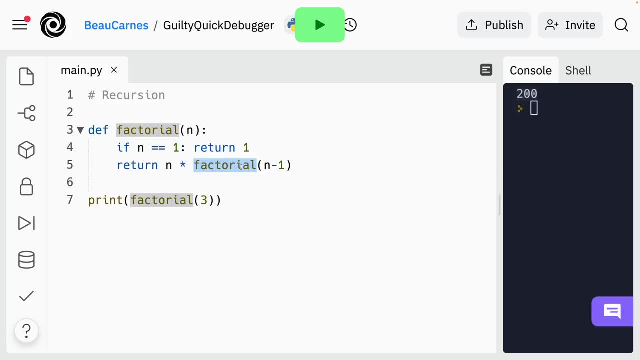 So here's the function. you can see inside the function. it's calling the same function, So a cursive function. it's always going to have a base case, that's this and recursive case. So the base case is when we're going to leave the recursive function. So if n is equal to one, 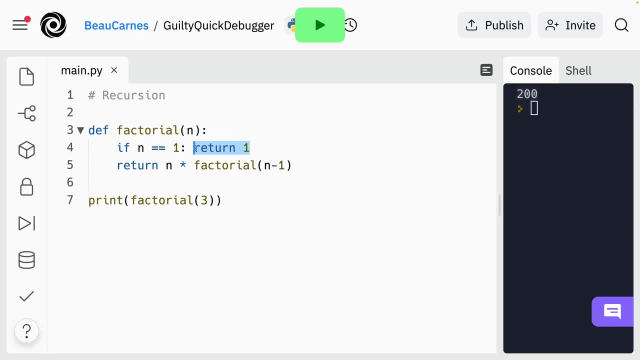 we're going to return one and that's basically going to get out of the recursive function. But if it's not going to equal one, then we have the recursive, the recursive case where we're going to call the function. So you always need to have at least 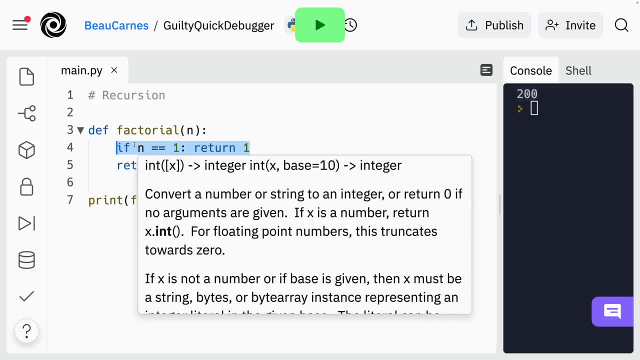 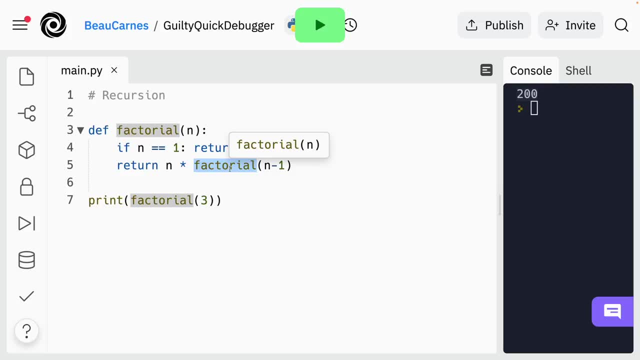 you always have need to have a base case So eventually the recursion can stop. If the recursion doesn't ever stop, then you're going to get a recursion error. It basically Python by default will halt recursions at 1000 calls. that's when you get the recursion error. So this: 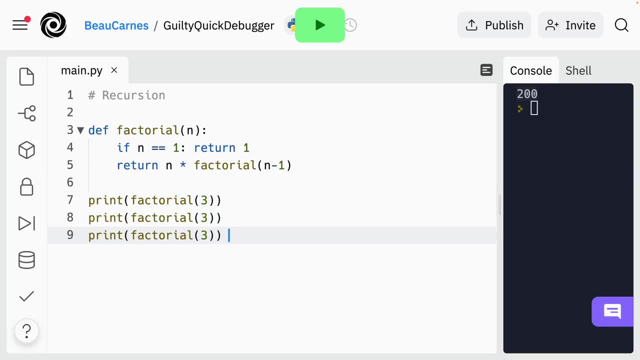 is going to get the factorial three, but let's just do this a few more times So you can see the difference. So three, four, five and now we'll test this out- 624 120.. Okay, now let's talk about decorators. So decorators in Python are a way to change. 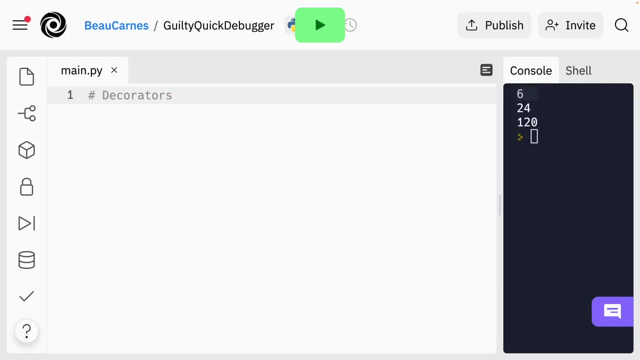 enhance or alter in any way how a function works. decorators are defined with the at symbol followed by the decorator name just before the function definition. So, for instance, let's say we have a function hello And it's just going to be the simplest function, we're just going to print. 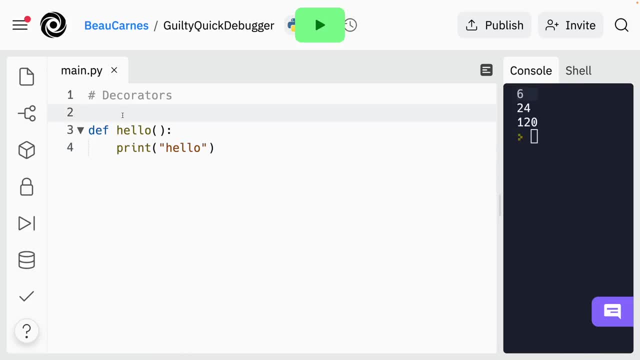 hello. So to make that to add a decorator, I'm going to put like this: an at sign and then the decorator name. In this case we're going to type in log time, So the function has the log time decorator assigned. So whenever we call the Hello function, the decorator is going to be called a. 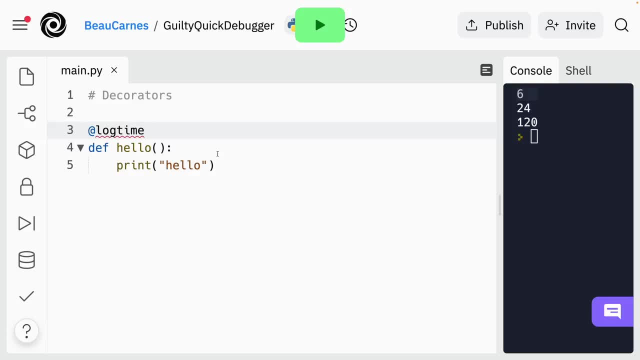 decorator is a function that takes a function as a parameter, wraps the function in an inner function that performs the job it has to do and returns that inner function. So, for instance, I'm gonna create another function here that's going to be the log time function, And now we can do something. 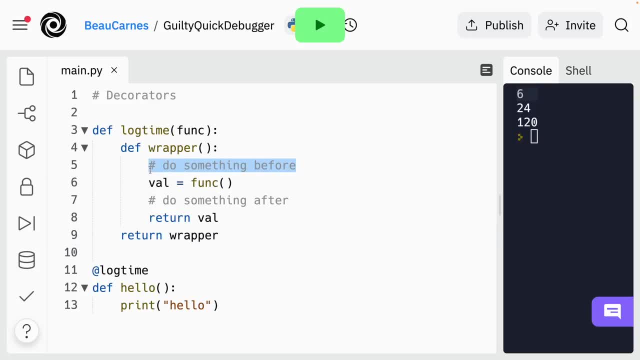 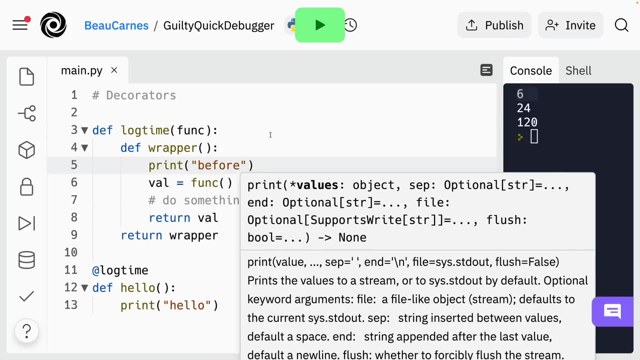 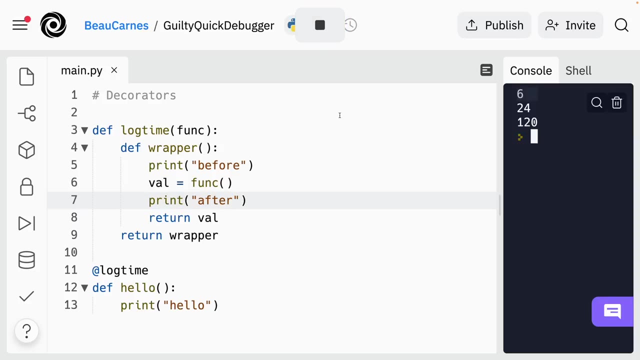 before and after the function. like, for instance, we can say print before and then after. we are going to print after. Now, if I run this, oh, and we have to call the function. that's always important. Now, if I run. 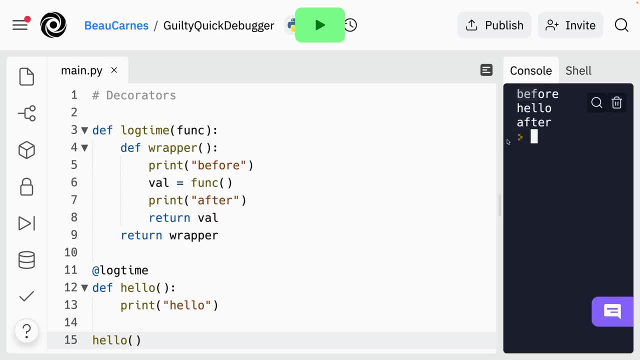 this before, hello after. so you're going to often use decorator functions when you want to change the behavior of a function without modifying the function itself. So a few good examples are when you want to add logging, test performance, perform caching, verify permissions and so on. 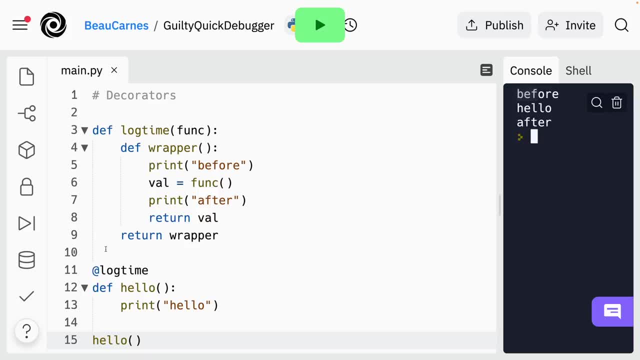 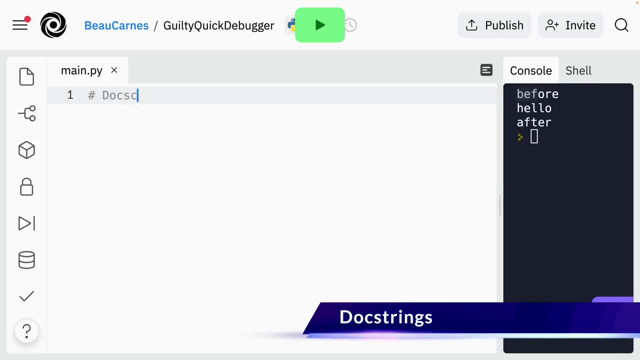 You can also use one of these functions called the decorator function, And you can also use one of them when you need to run the same code on multiple functions. Okay, now let's talk about doc strings. So doc strings- documentation is hugely important, not just to communicate to other people. 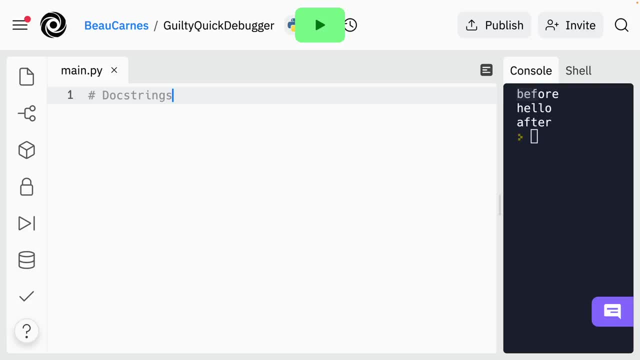 what the goal of a function or class or method or module is. But it's also. it also communicates to yourself When you come back to your code. like many months from now, you might not remember all the knowledge you're holding in your head when you wrote the code. So at that point, 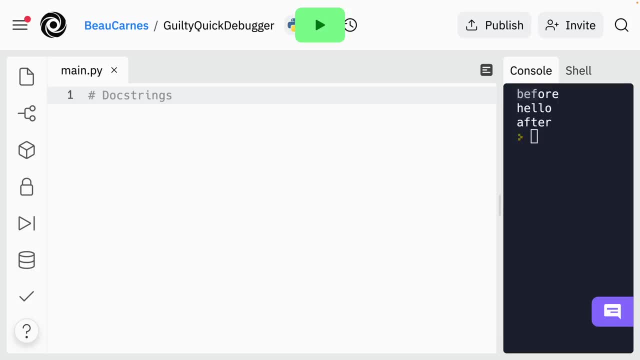 reading your code and understanding what it's supposed to do, So that at that point reading your code and understanding what it's supposed to do will be a lot more difficult. So a lot. That's one of the reasons why people add comments. So another way is to use a doc string. 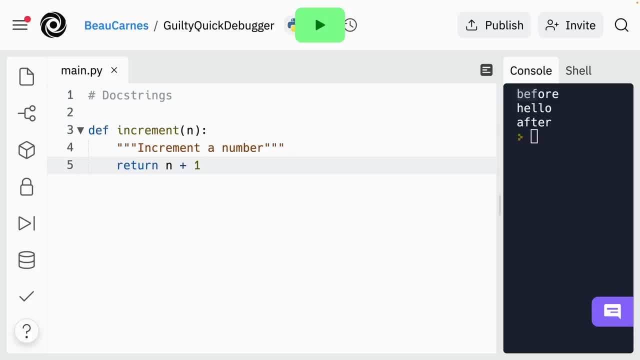 So let me show you what a doc string looks like. The utility of a doc strings is that they follow conventions, so they can be processed automatically. So this is how you would define a doc string for a function. Basically, you're putting the three quotation marks here. three quotation marks. 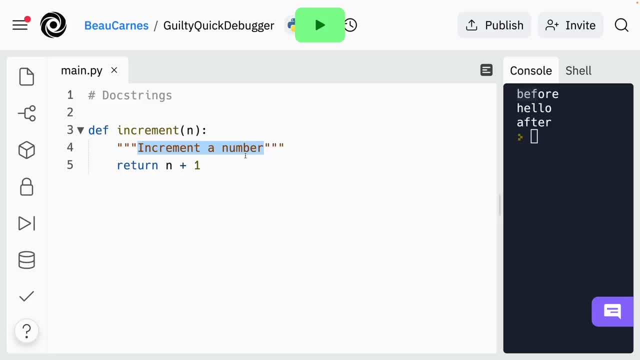 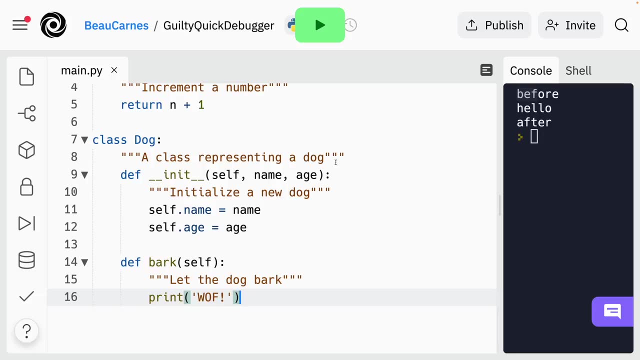 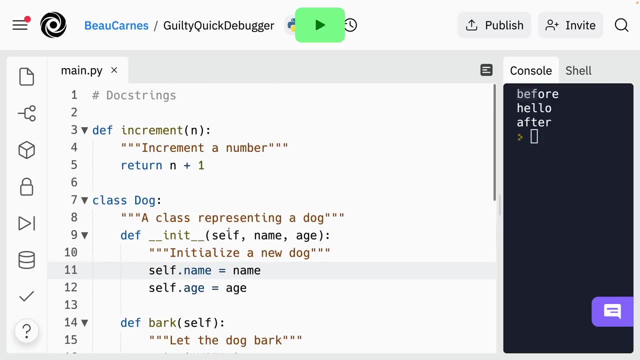 there. And then this is a description of what the function is. This is how you would define a doc string for a class and a method. So get the class this what the class is, this is what the method does. And then it's also common to add docs. place a doc string at the top of the file. So if you put 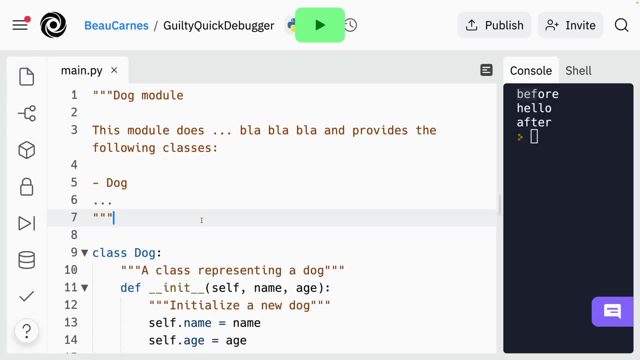 a doc string at the top of the file. you're going to get a class and a method And then you're going to get a doc string at the top of the file. it's gonna look like this And it's going to explain. 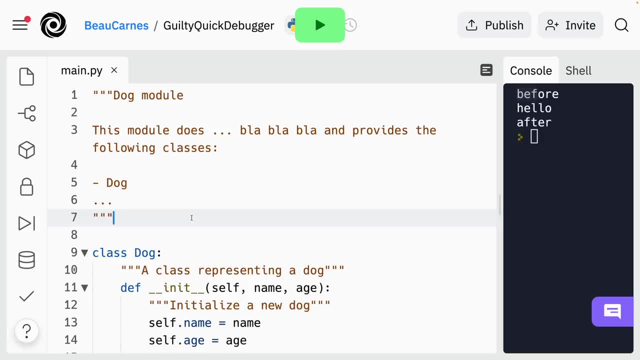 what the file is all about And Doc script stock strings can also span multiple lines, just like this is a multiple line doc string, as long as it has a three quotes- three quotes at the top, three quotes at the bottom- And then Python will process the doc strings And you can use the Help. 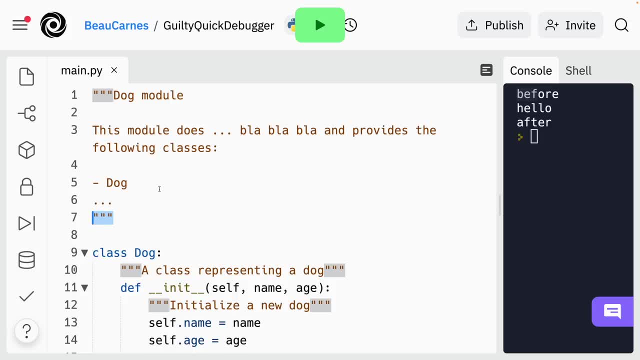 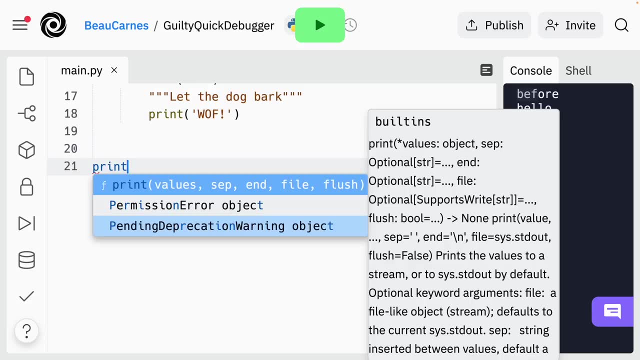 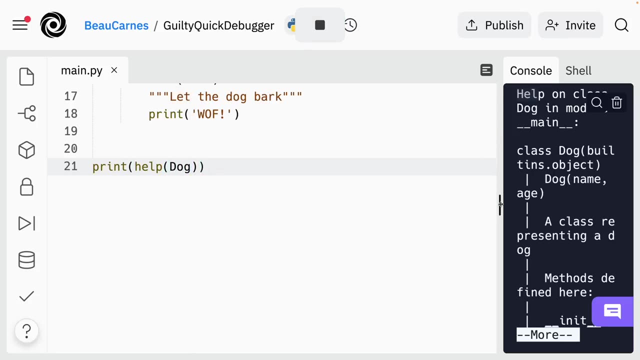 global function to get the documentation for a class method of function or a module, For example. I'm gonna go to the bottom of this and I'm gonna say print help. And then I'm just going to type in: dog, Now I'll run this And let me just run it. 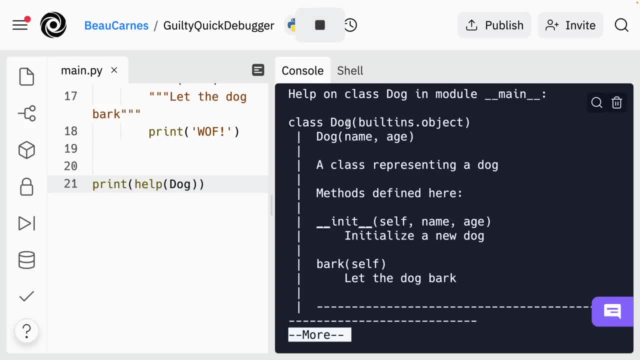 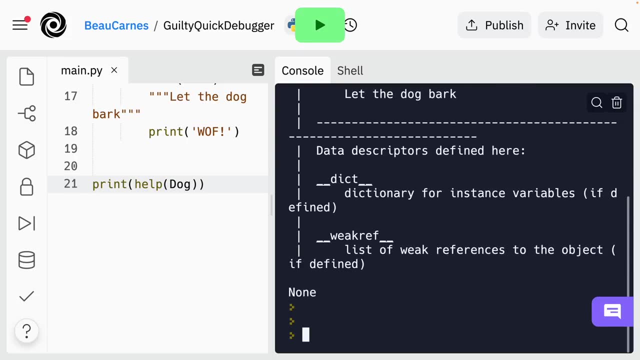 again. So now you're going to get information about the dog. we know that dog has a name and age, it's a class representing a dog and has these specific methods, And then it says more. we can get more information, data descriptors defined. here we have, and this is just gonna. 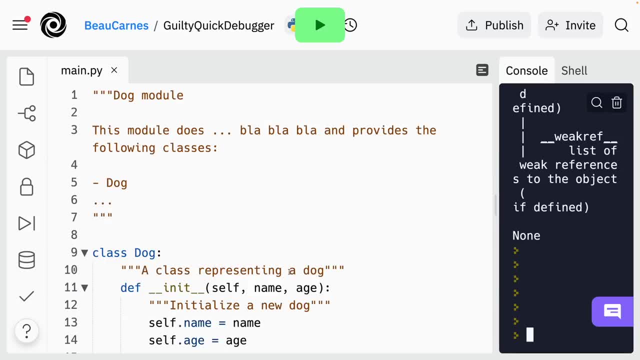 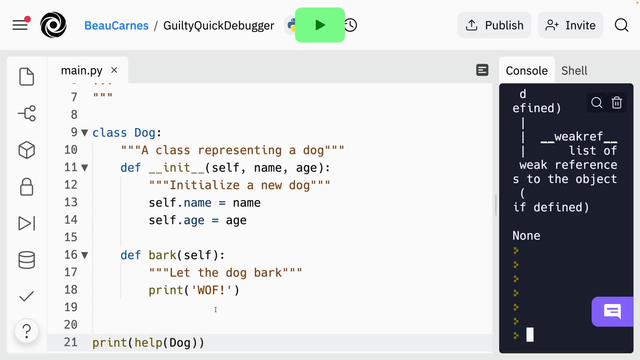 give us all this information about the dog And we, and so that's why it's good to use doc strings, because there are specific standards And it makes it easier to get information using different helper methods And standards allow, and standards allow us to have tools to extract doc strings and automatically. 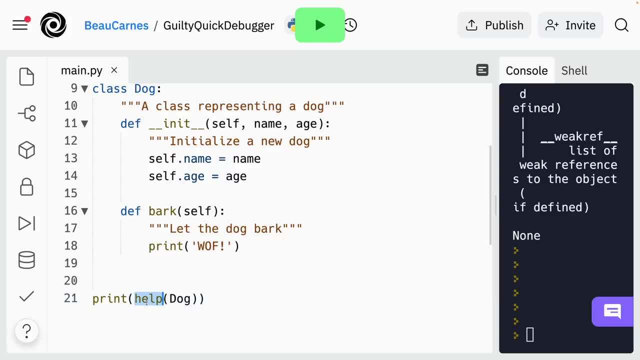 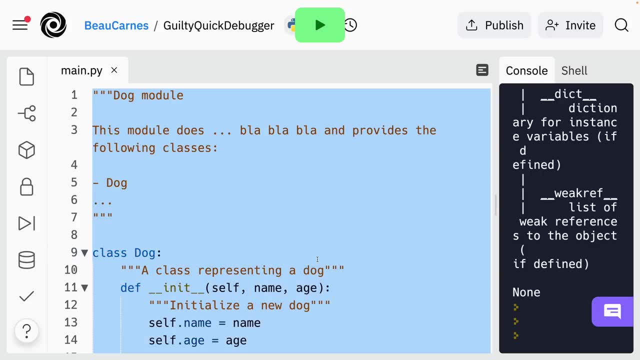 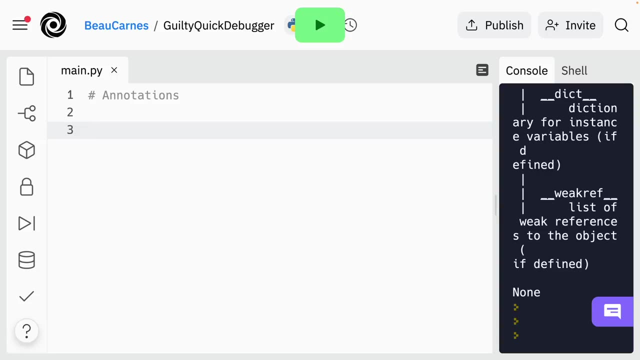 generate documentation for your code. So besides just this help functions, there's a lot of other methods to pull out these doc strings and get information about your code. And next we will learn about annotations. Python is dynamically typed, So we do not have to specify the type of 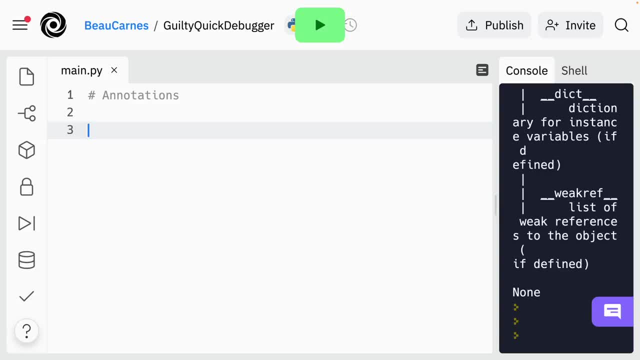 a variable or function parameter Or a function return value. annotations allow us to optionally do that. So if we want to actually show what type we're expecting for different values, So here's a function without annotations. And then here's how we would make it have annotations. So we want to make this function. 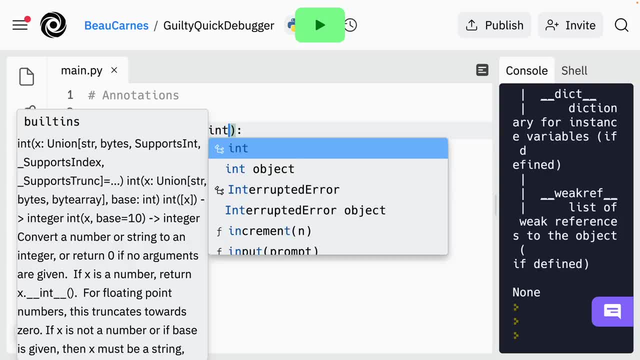 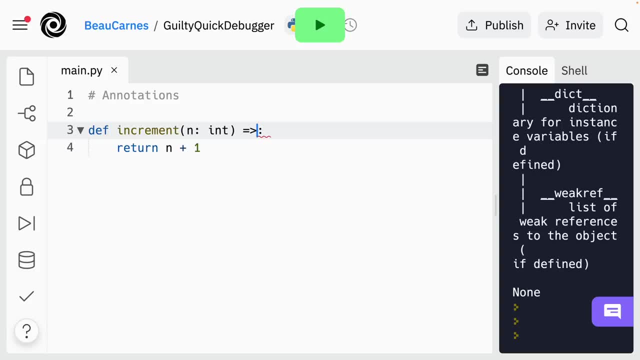 only accept an int. So I'm going to put colon int And then after here I'm going to put, actually before the colon, here I'm going to put a little arrow here, And then I'm going to put in int. So now we're. 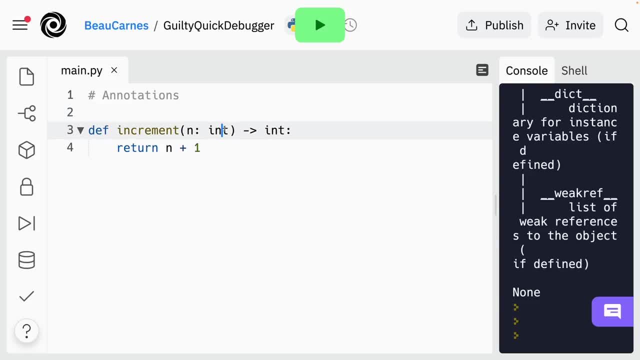 specifying that this function receives an int And then it's also going to return an int. And you can do the same thing with variables. So if we have a variable, if I had a variable called count and was equal to zero, I can add an annotation to make it be an int like that. So now we're specifying: 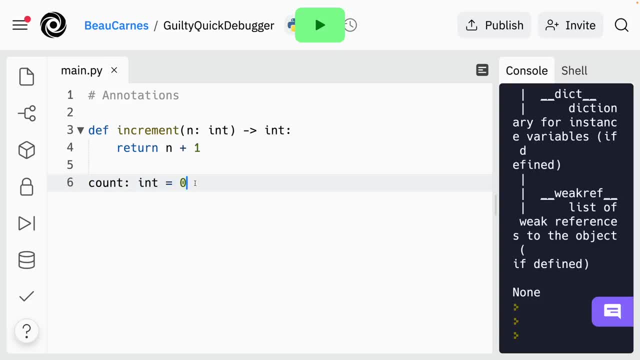 that this variable is going to be an integer. Python will actually ignore these annotations. a separate tool called my pi can be run standalone or integrated by ID ease to automatically check for type errors statically while you're coding. It will also help you catch type mismatch bugs. 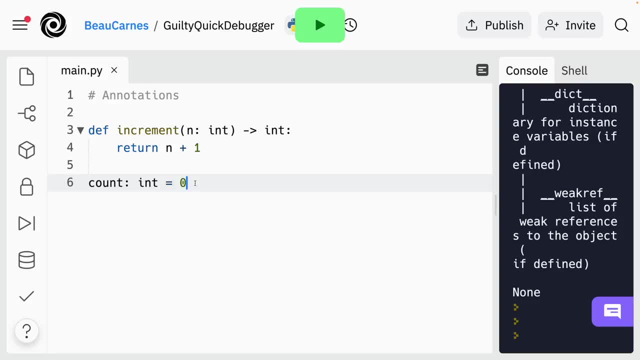 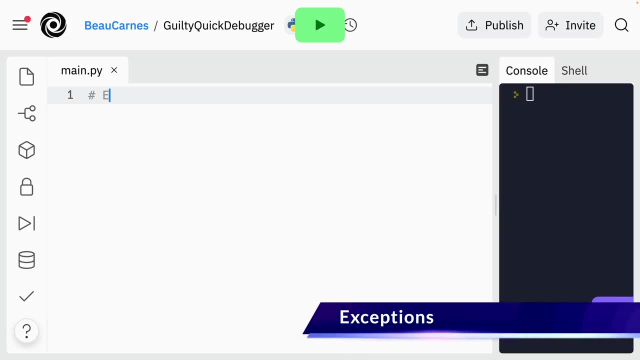 before even running the code. A great help, especially when your software becomes large and you need to refactor your code. Okay, now we'll talk about exceptions. It's important to have a way to handle errors, And Python gives us exception handling to do so. So 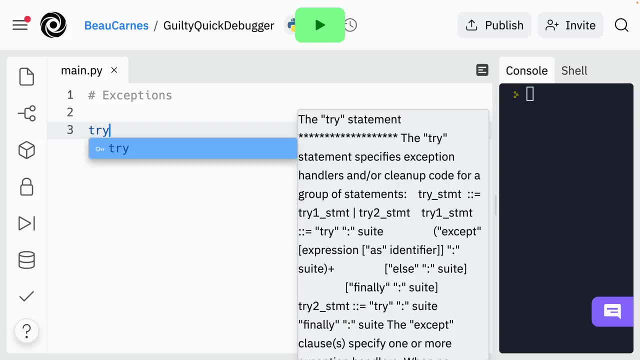 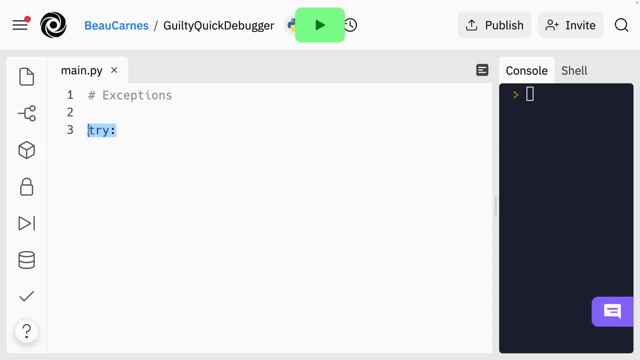 for exception handling, you would wrap lines of code in a try block And then inside this block you'll put the lines of code And then, if an error occurs, Python will alert you and you can determine which kind of error occurred using an except block. So we're trying some lines of code. 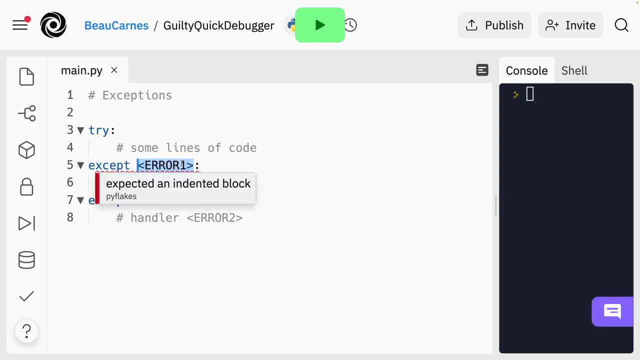 here and then we're checking for a specific error And then if that error happens, we would handle that error, But if a different error happens, then we will handle the different error. You can also catch all exceptions using an, except without an error type. So at the very end, 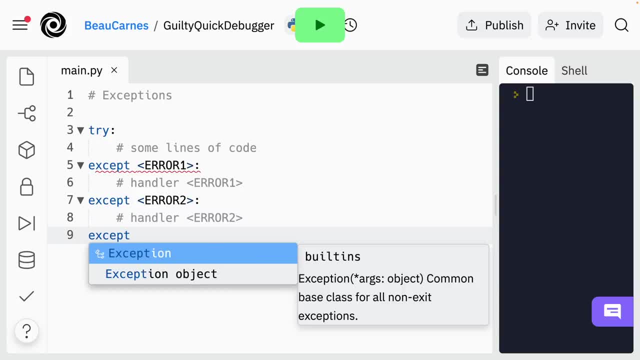 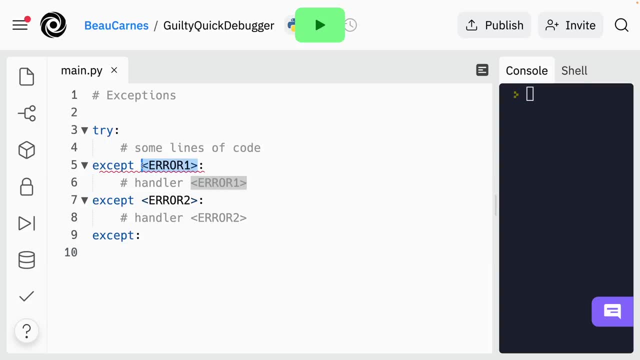 you could just do except. And then if you don't have an error type, then it's going to handle the rest of the exceptions. And just to make this clear, this just an example. where it says air one, you have to put a specific air in that spot. You can also. 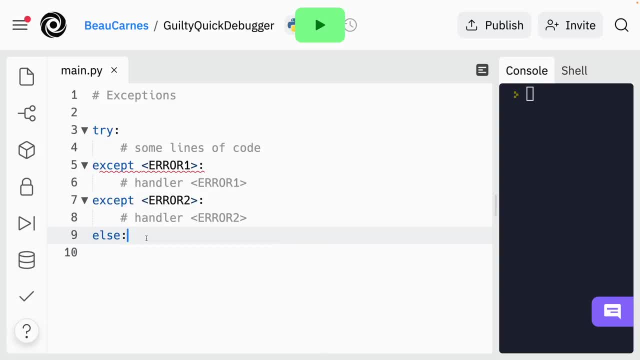 put an else block at the end to handle that. that will run if the no exceptions are found. So if there are no errors in this code that's read up here, we can have an else and then run specific code at the bottom that that runs if there's no errors And then we can have a finally block. So 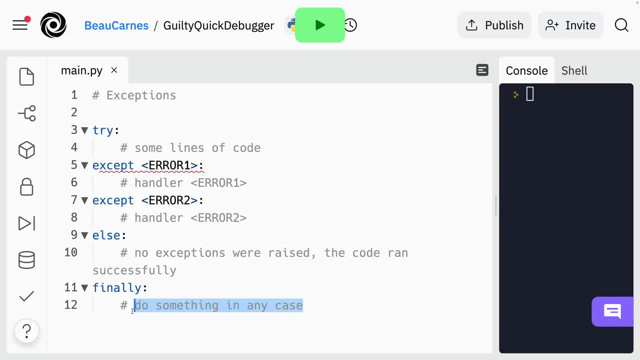 anything in a finally block is going to just always run at the end. whether or not there were exceptions or no exceptions, the code in the finally block is always going to run. the specific error that's going to occur depends on the operation you're performing. For example, 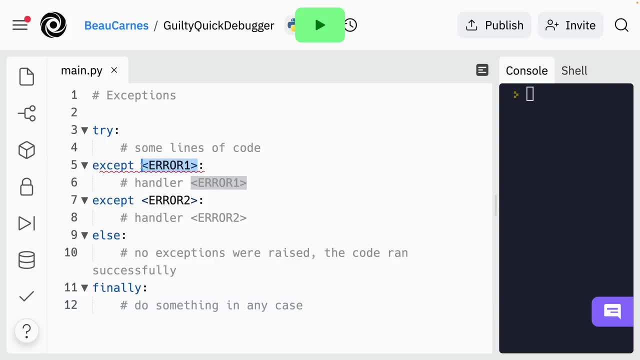 if you're reading a file, you might get an EF error. would just look like this: EO F error, which means end of file. If you divide a number by zero, you'll get a zero division error. If you have a type conversion issue, you might get a type error. So let's try. 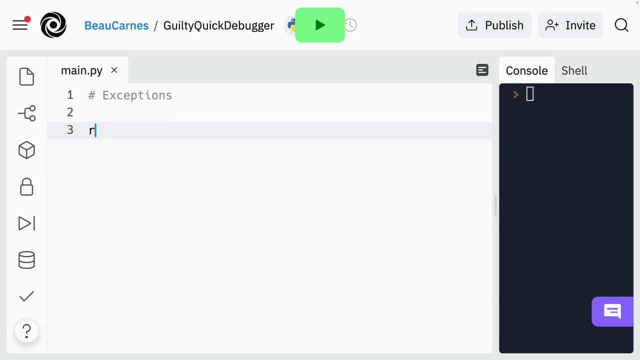 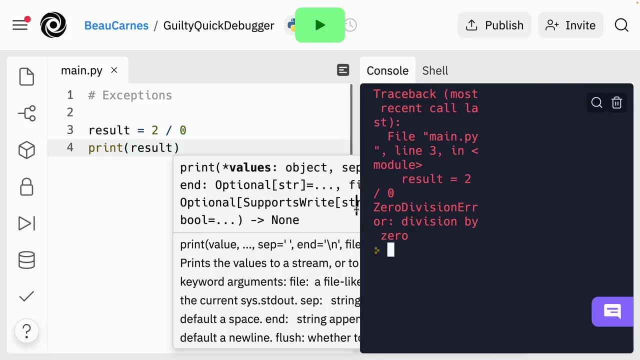 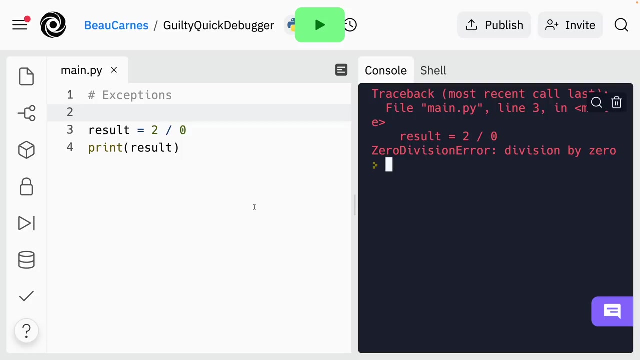 this code. So I'm going to just delete all this And we'll do: result equals two divided by zero, which you cannot do. So just print the result And if I run that, we'll see this error over here: Zero Division error- division by zero. So it's gonna get an error when we run the code And 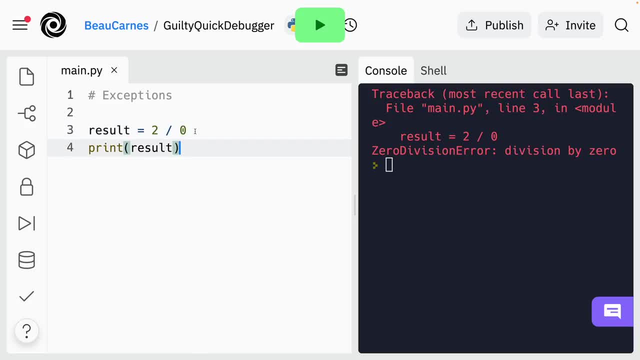 then whenever there's an error, anything after the error occurs will not happen. So we're not going to print out the result, because the resist, because the this, this line resulted an error, So we're not going to run the following line of code. So now let's try adding that. 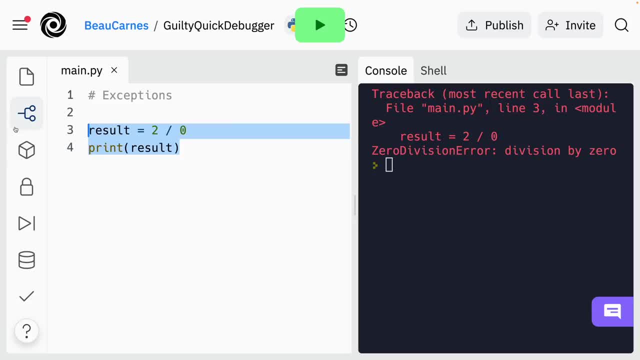 operation in a tree block, So I'm just going to paste all in here, And so we're putting the etta in a try block And then we're expecting a zero division error where we'll print: cannot divide by zero. Finally, we will set the result to one and then print the results. So let me just run. 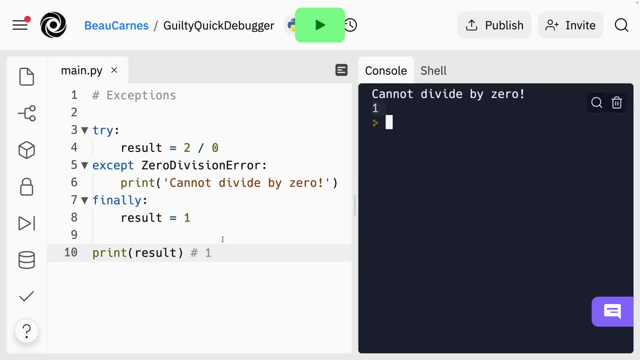 that code See cannot divide by zero. and then we print one. what we we? because we set it in the finally block here. So this try block lets us recover gracefully, and move on with the program. you can raise exceptions in your own code to using the raise statement, So I could type in: raise. 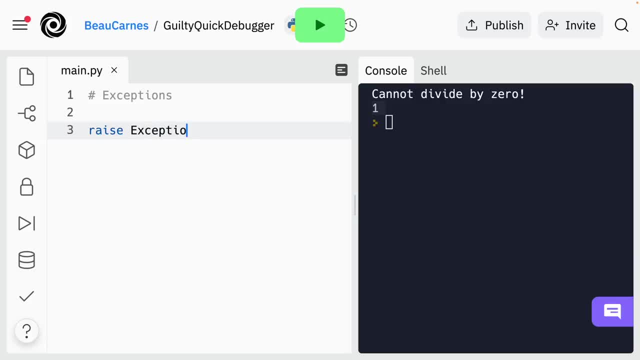 and then we can raise an exception: intentionally And error. So if I just run this, it will say: and error, because that's what we typed in. So you can make it say anything you want for your error, And this raises a general exception And you can, and you can intercept it. 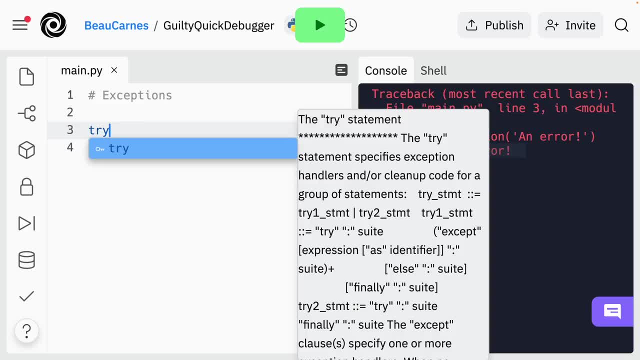 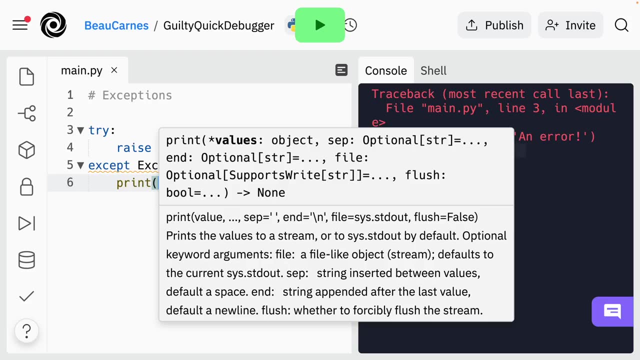 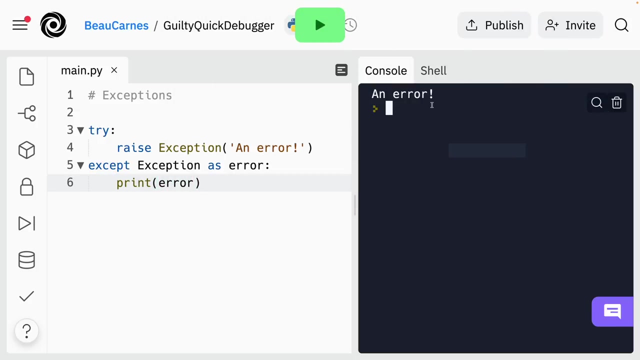 just like this. So I could say try And then we raise that exception And then we can do accept exception as error, And then we can print the error. Okay, if I run that. so now, instead of we don't, we don't see all that red anymore because it's not stopping our program because of the air. 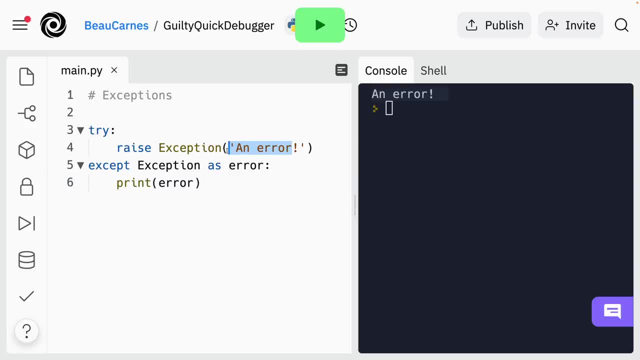 but it's now printing the error And then we can do accept exception as error And then we can print the error message right here. just like that, You can also define your own exception class extending from exception. So I could do class dog not found exception And then I will extend from exception. 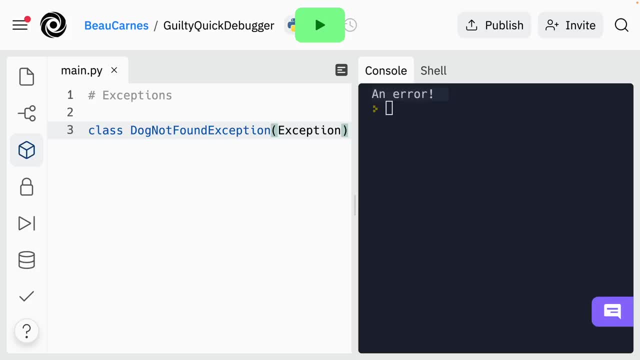 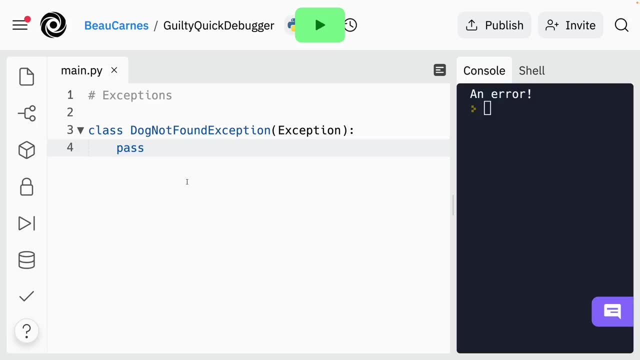 And then I can just put pass for this one here. let me just that. So pass here just means nothing, And we must use it when we define a class without methods or a function without code. So if you're not going to put anything, this is just an example. 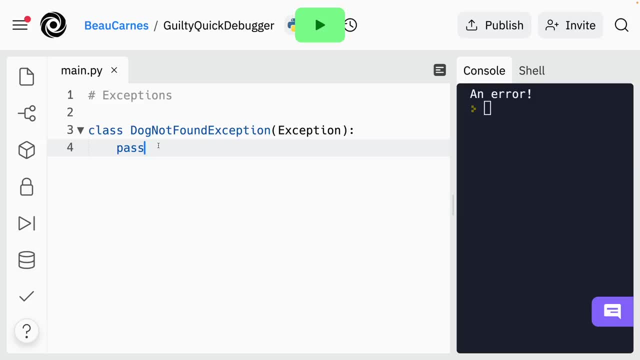 So I can just put pass to mean that we're not going to have any code in this. So now we can try it out. So let's paste that. So we're going to raise dog not found exception And then, if we're going to candle this exception, we're going to do a pass here And then we're going to paste that. So 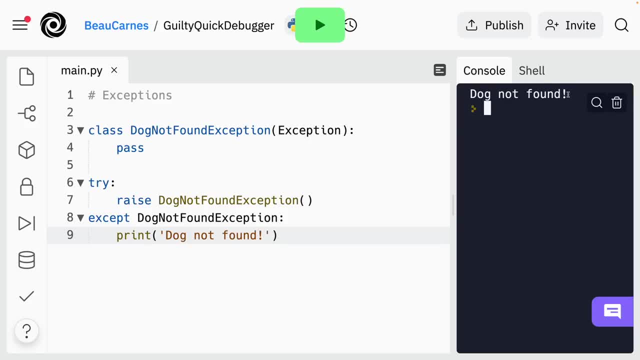 we're going to do a pass, And then we're going to do a pass, And then we're going to do a pass And just print: dog not found. So let's try that Yep: Dog not found because it raised this exception. 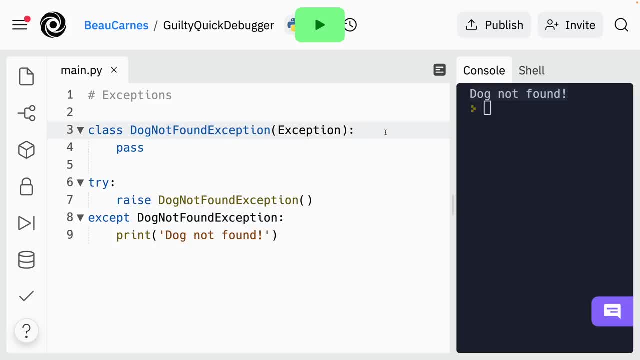 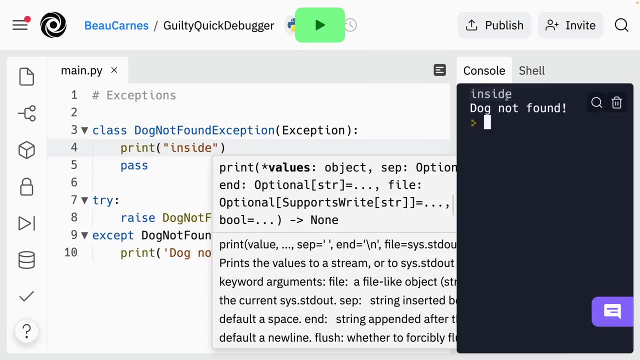 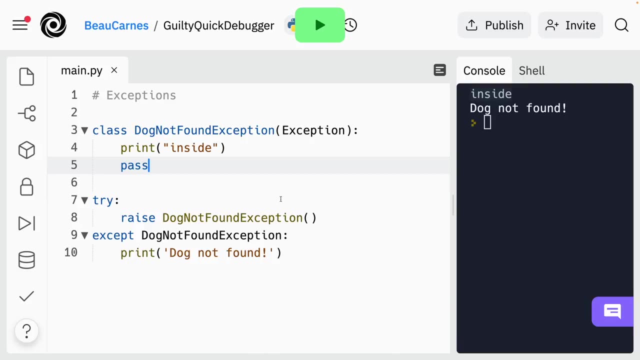 here We can also actually do something in the exception print. So if I can say, print inside and then I'm going to run that and they'll do inside and dog not found. The width statement is very helpful to simplify working with exception handling, For example when working with files. 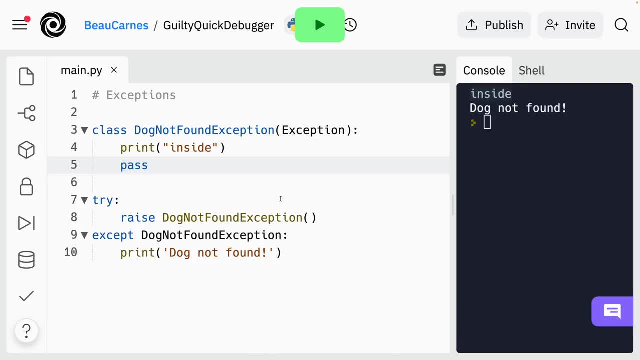 each time we open a file, we must remember to close it with makes the process more transparent. So let me show you some example code without the width statement. So we're not going to go into a lot of details about working with files here, But I just want to kind. 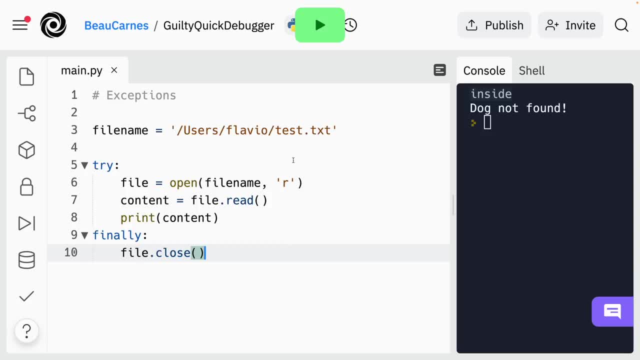 of just give this one quick example. So if we're going to be working with files in Python so we can open the file and then we can read the file, we can print the content from the file, And we're going to try that because there could be an exception- And then, finally, we're going to 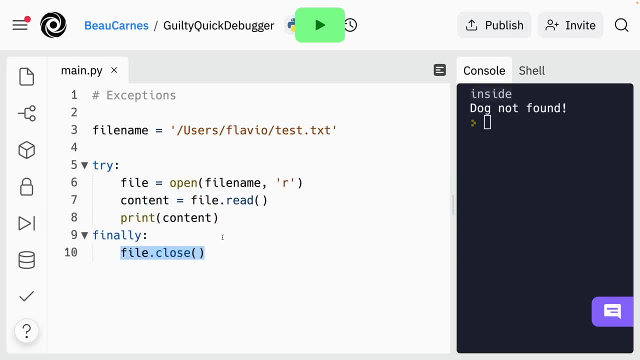 make sure to close the file, But an alternate way to do it would be like this: So with we're going to open the file as file and then content file dot read and then print the content And with using width, it's going to make sure to automatically close the file at the end. In other 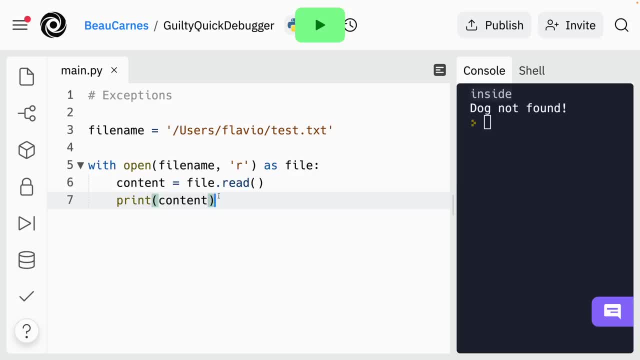 words, we have built in implicit exception handling, as close will be called automatically for us And with can do a lot more stuff as well. This example is just meant to introduce its capabilities. Now let's talk about third party packages, And we're going to talk about pip, So let's learn how to install third 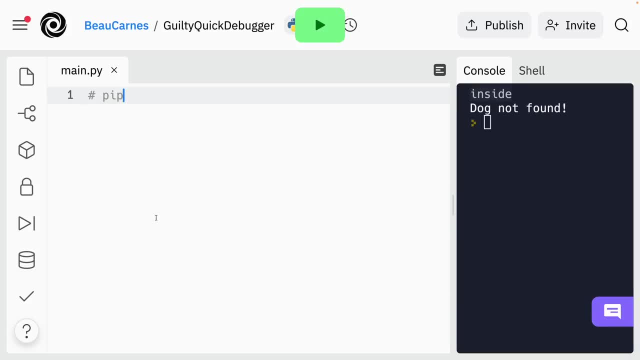 party packages in Python Using pip. the Python standard library contains a huge number of utilities that simplify our Python development needs, but nothing can satisfy everything. That's why individuals and companies create packages and make them available as open source software for the entire community. 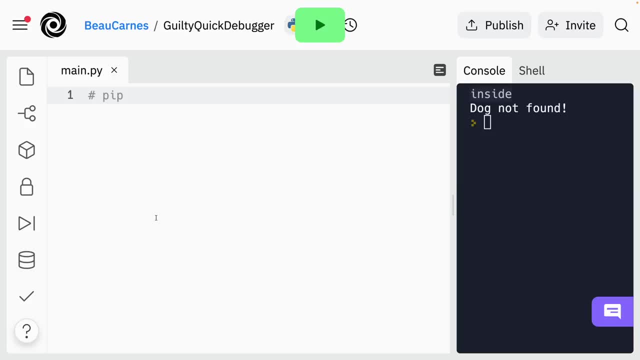 So the modules are all collected in a single place called the Python package index, which is available, available at pi piorg. That's pi piorg And they can be installed on the system using pip. there's over 270,000 packages freely available. Most computers are. 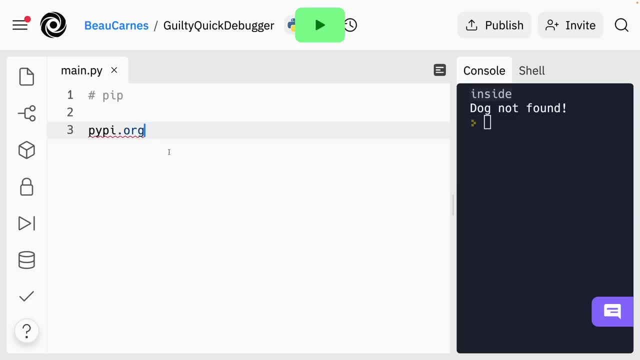 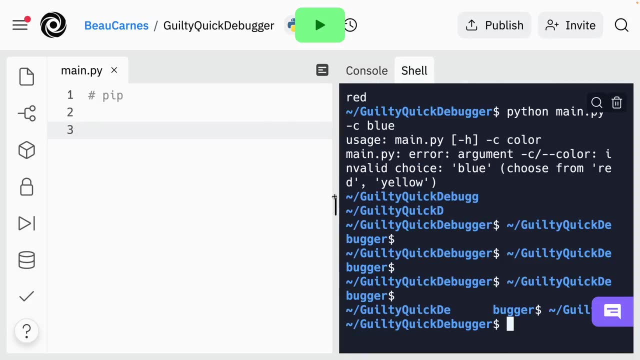 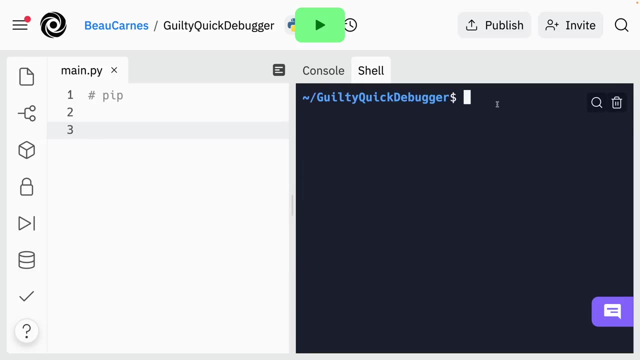 already going to have pip installed and replica already has pip installed. So let me show you how you would install a package. we'd have to go over to the shell here. If you're not on Replit, you can just do in your terminal, And I'm going to clear this here. And I'm just going to do pip install And 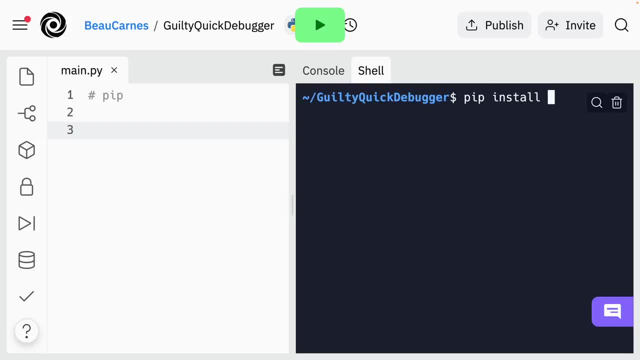 then you can put the name of a package, For instance, a. one popular package is called the request package. It's an HTTP library, So I can do requests And let me, just so you can see, I have to make sure I spelled that right. 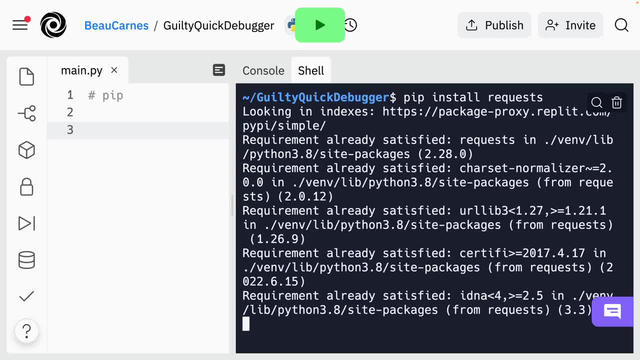 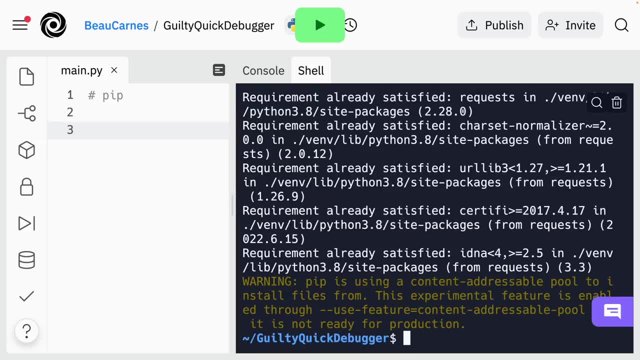 And it's going to install that package right now. So once we install this package, it's going to be available for all our Python scripts, because packages are installed globally And the exact location depends on the operating system. You can also upgrade a package to its latest version by: 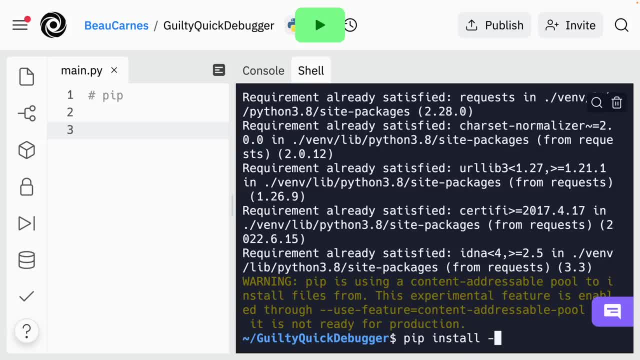 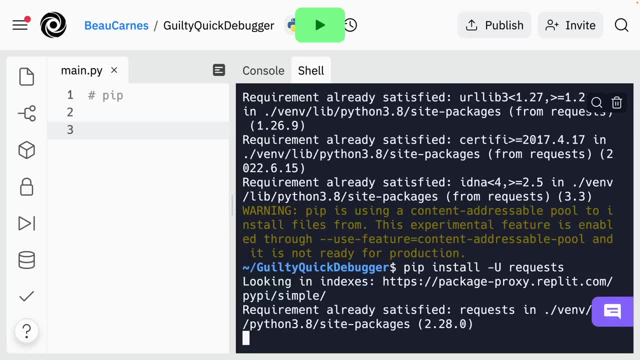 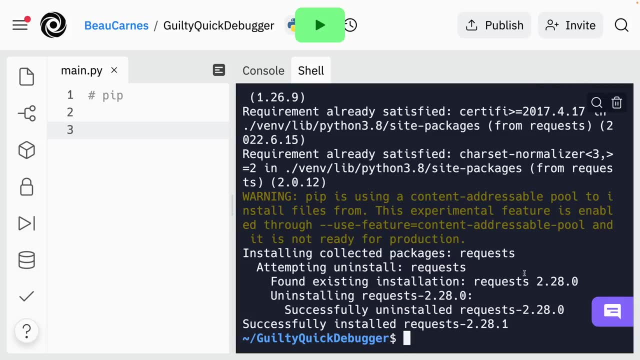 doing pip, install dash u, And then I will just put the package name. So in this case we'll just do request again And then it's going to just update it to its latest version. In this case it updated from 2.2- 8.0 to 2.2- 8.1.. You can also specify a specific version when you're installing, And then 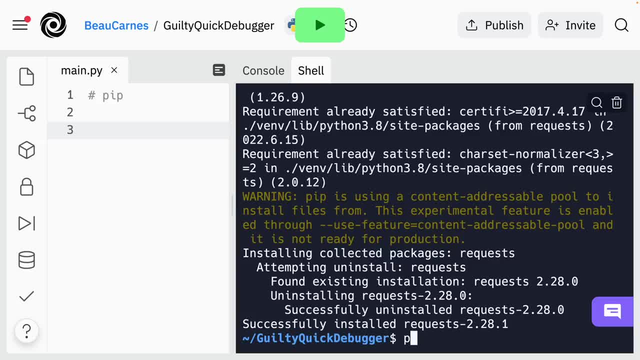 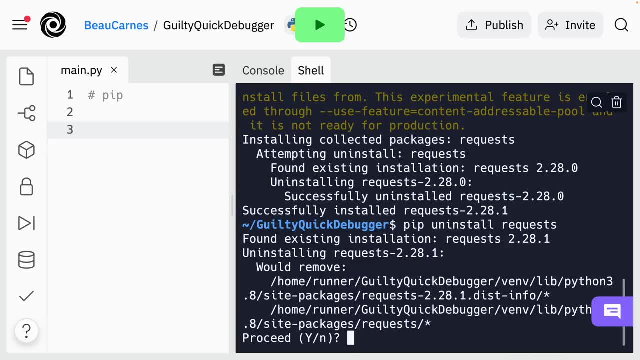 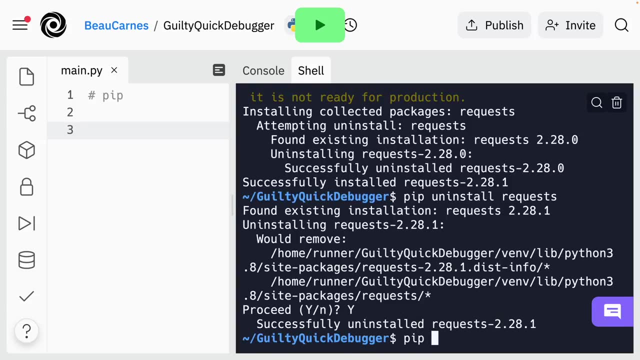 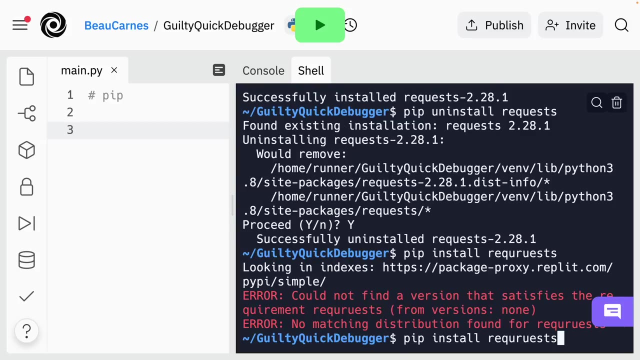 you can also uninstall a package. So I'll do pip uninstall And then I can say that yes, I do want to uninstall that. And then when, when you have a package installed, I'm just going to install request again. And then you always have to make sure you spell it. 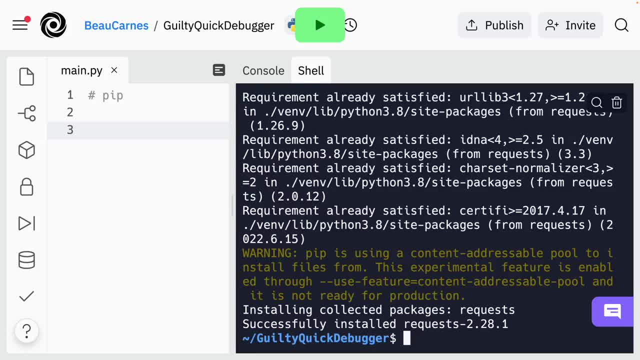 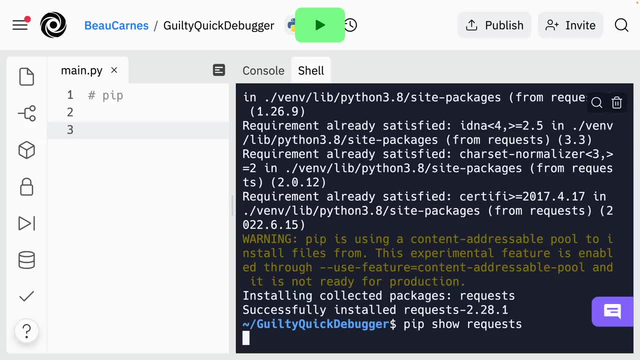 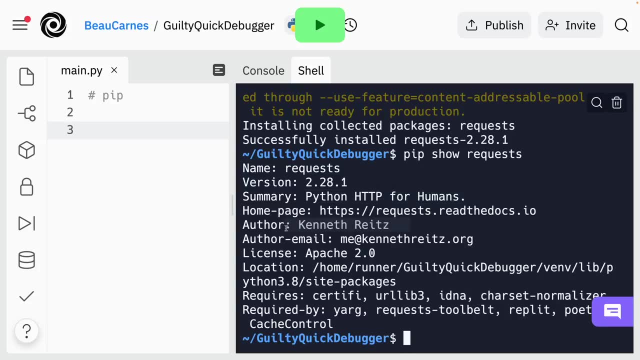 right. So once you have installed you can do pip, show requests, And then it's going to show some information about the package. So see, we can see the name, the version, the summary and then a bunch of the author and a bunch. 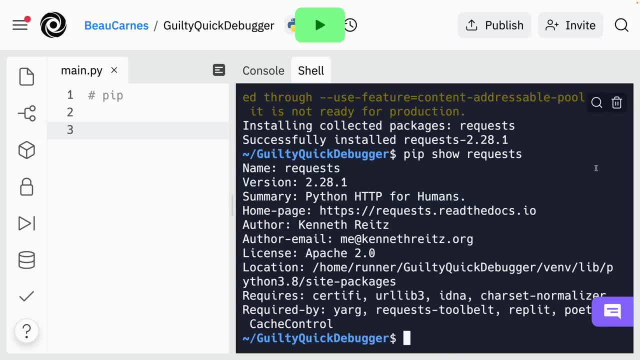 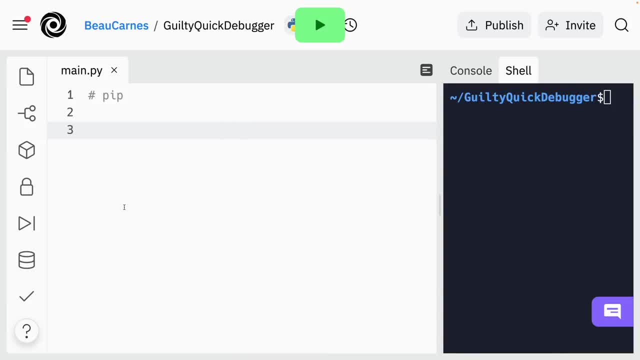 of other information about the package. Okay, I'll just clear this. Now we're actually gonna backtrack a little bit. We already talked about lists, But I'm going to talk about a more advanced way of using lists, called List compression. lists compressions- So list compressions- are a way to 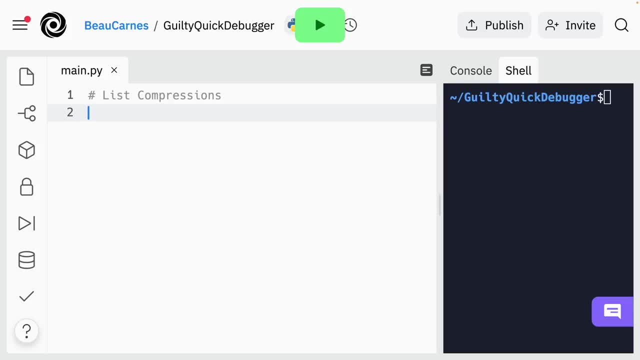 create lists in a very concise way. So let's see now: So we've created a list And this is for our list. So let's say I've created a list And I have a list here and I want to say I don't want this. 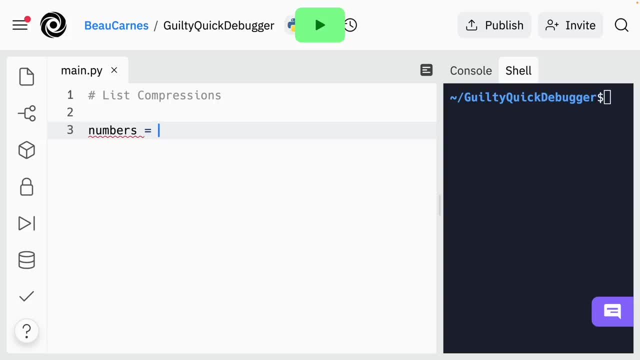 suppose you have this list like this: it's a list of numbers And we'll just do 12345.. So we can create a new list using a list compression composed by the numbers list elements to the power of two. Let me show you what I mean. So let's get make a new list: numbers Power. 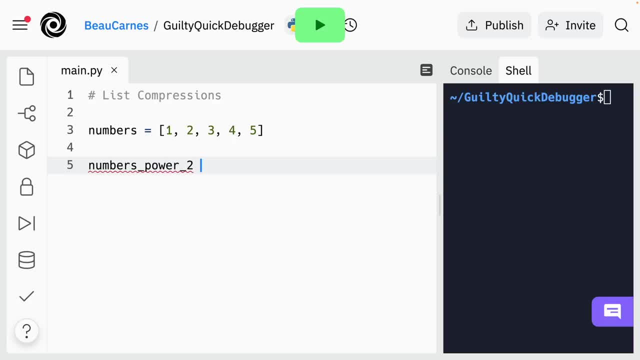 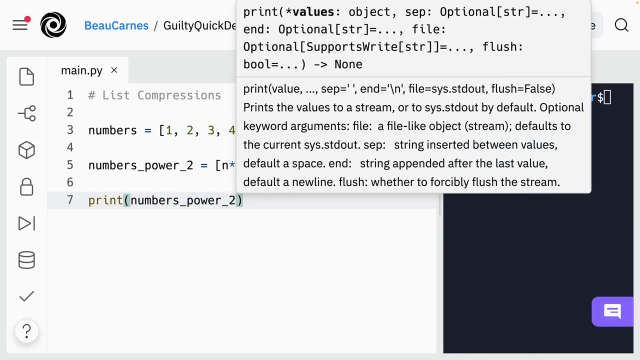 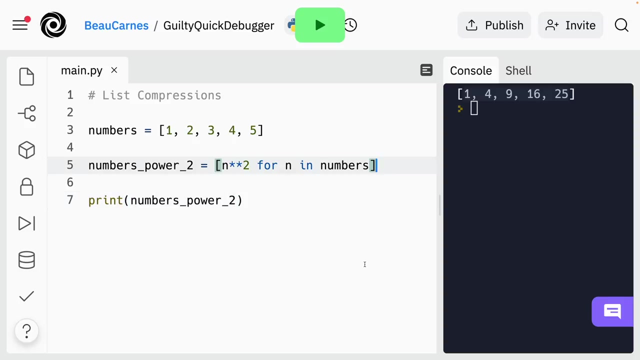 two equals And let me just show you how you do this: list compression. So this is the list compression syntax And if I print this, we can see that now we have every element in the list to the power of two. list compressions are a syntax that sometimes preferred over loops. 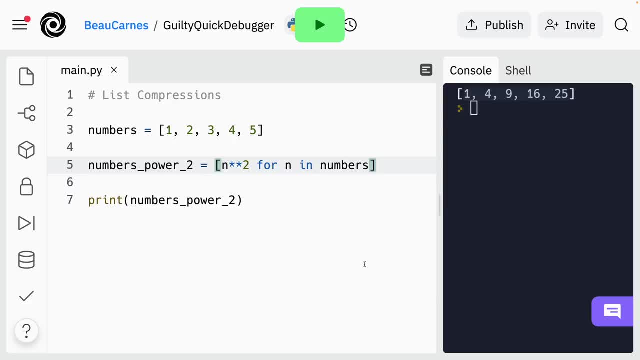 as it's more readable when the operation can be written on a sentence. So let's go ahead and do that. So let's go ahead and do that, So let's go ahead, and single line. So, for instance, this is how you would do it with a loop. So what we do in a single 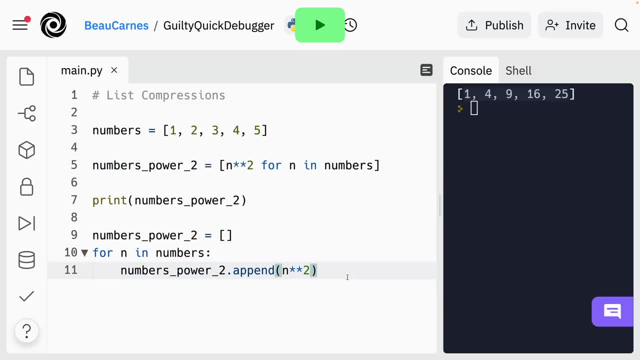 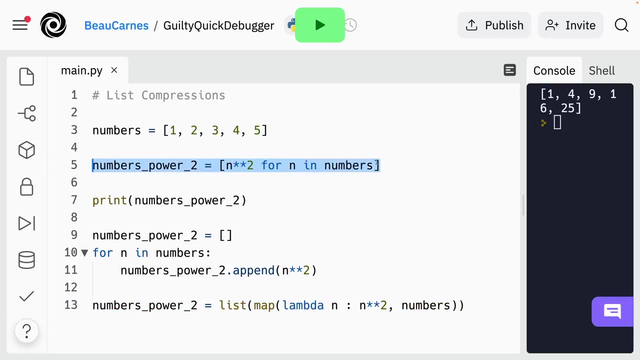 line up here we take a few lines to do in the method with a loop. So list compression just makes it simpler, And then you can do the same thing with math as well, But again it's just a little more complex. It's sometimes. it's just simpler to use a list compression using the. 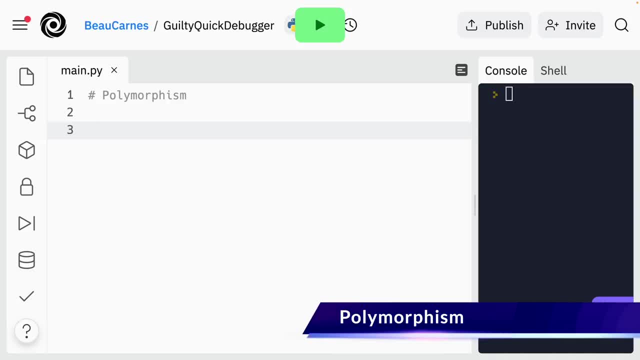 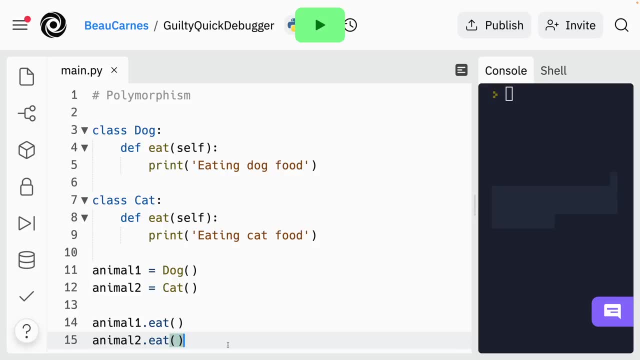 syntax here. Now let's talk about a few more advanced topics in regards to functions Polymorphism. Polymorphism generalizes a functionality so it can work on different types. It's an important concept in object oriented programming, So see in here. 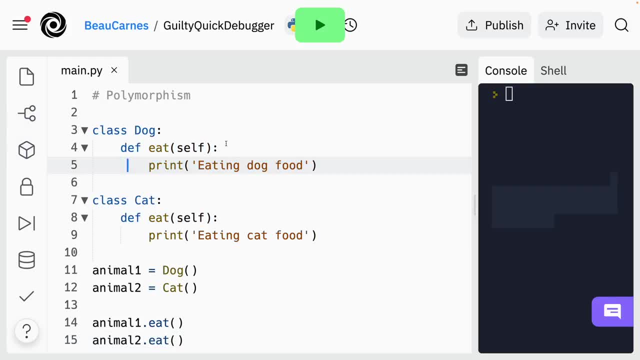 we've defined the same method on different classes. So the dog has eat and the cat also has an eat method. then we can generate objects and we can call the eat method, regardless of the class the object belongs to, and we'll get different results. So we create the two objects. 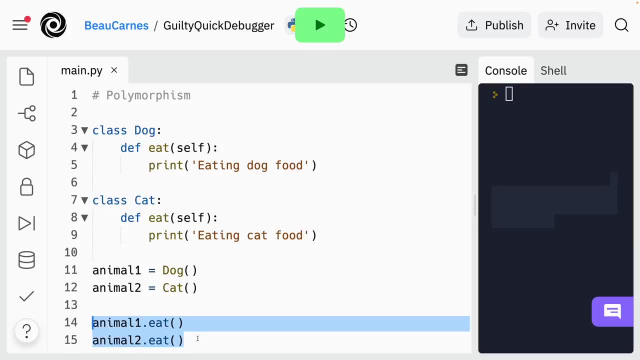 the dog and the cat here And we're calling the eat method on both objects And if we run this, you can see what we're getting eating: cat, dog food eating cat food. And so you could do a lot of things with this, like maybe you have a list of different animals And then you can loop through. 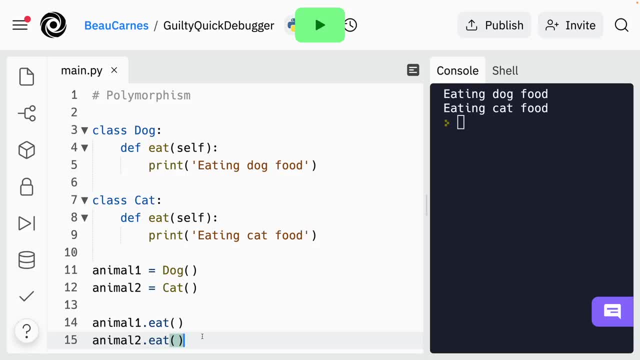 that list and call the eat function or the eat method on each animal in that list, And they don't have to be the exact same class to be able to still run the eat method. So we build a generalized interface And now we do not need to know that an animal is a cat or dog. 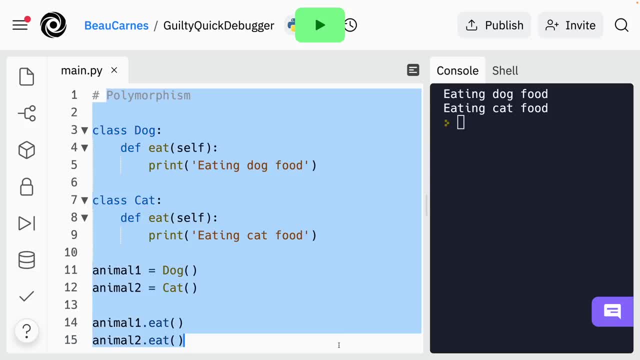 we just need to know that we can call eat on it. Now let's talk about operator overloading. Operator overloading is an advanced technique we can use to make classes comparable and to make them work with Python operators. So let's take this class dog. So here's a dog class And you. 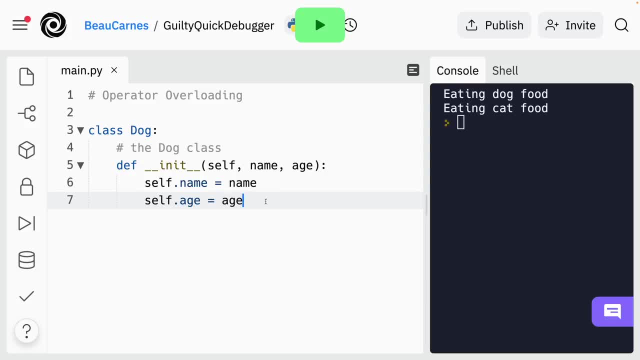 can create a dog with a name And you can create a dog with a name And you can create a dog with a name and age. then we'll create two dog objects. we'll do Roger equals dog And we can pass the name. 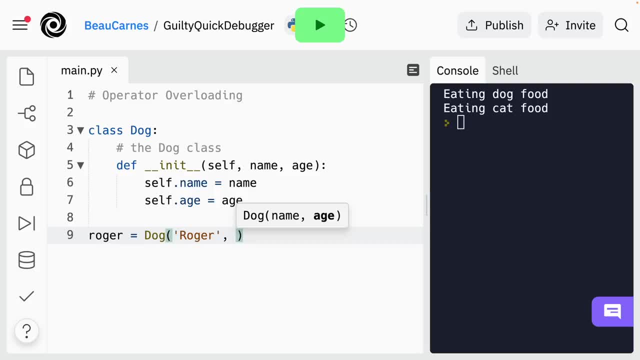 and age, And then I'll make another one. We can use operator overloading to add a custom way to compare these two objects based on the age property. So like: how could you compare this dog and this dog? Well, we can make it possible with operator. 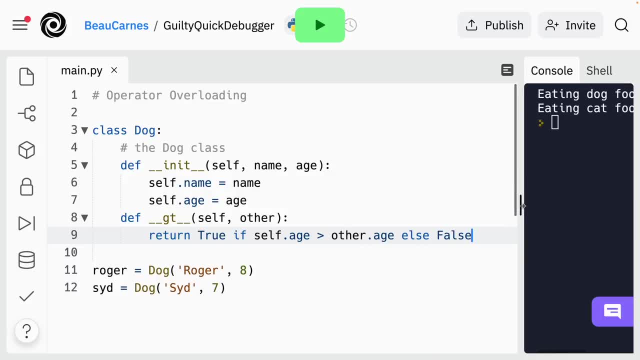 overloading. So let me just show you this example here. So this function here, GT, is going to compare things as to figure out what is greater than you can now will be able to compare to dog objects to see which one is greater than the other. And this is how we're going to figure out which is greater. 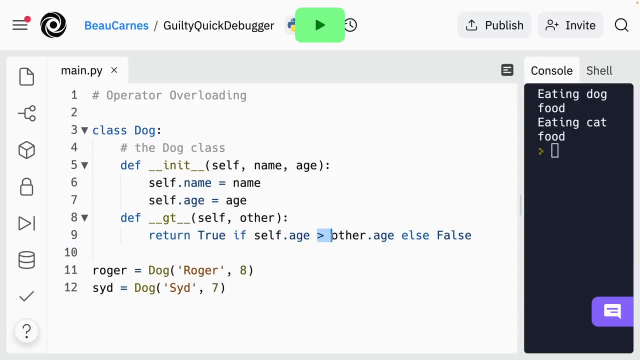 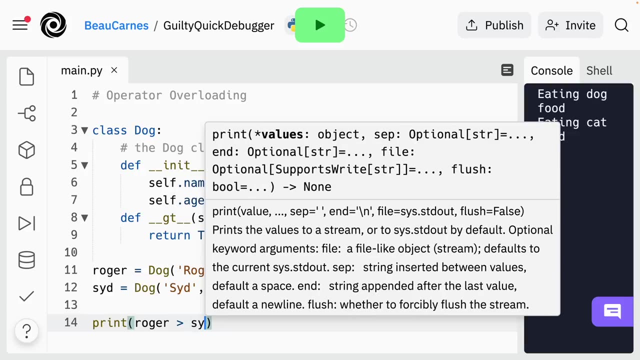 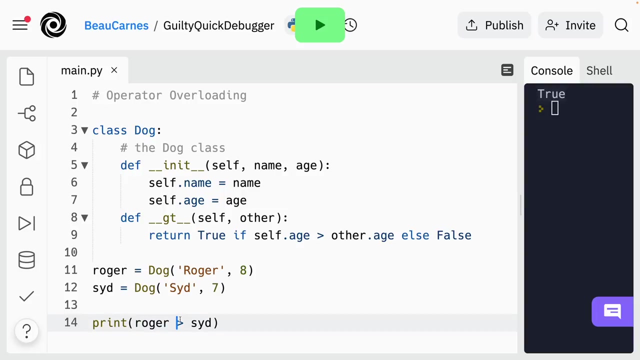 than return. true if self age is greater than other than age, which is the other one you're comparing it to, else false. Now we can do print: Roger is greater than Sid. So we're trying to figure out this is true or false. If I run this, it's going to say true, Roger is greater than Sid because eight. 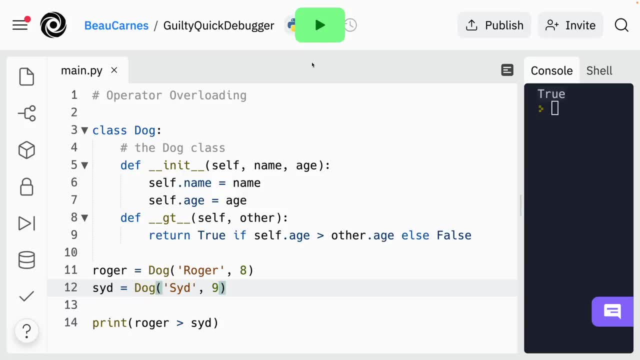 is bigger than seven, But if we like put nine here, run that. Now it's gonna be false. So in the same way we define this underscore, underscore, GT, underscore, which means greater than, we can also define methods for like less than lower, or equal to greater, equal to or not equal. And then 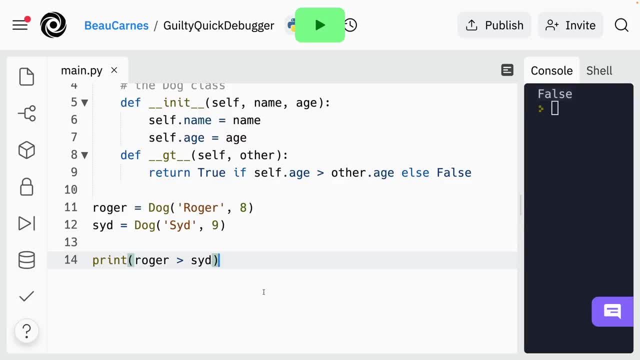 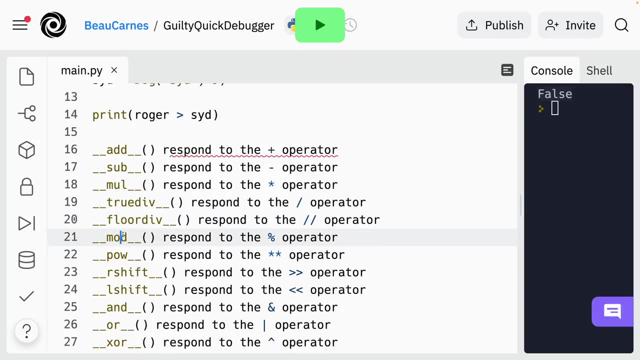 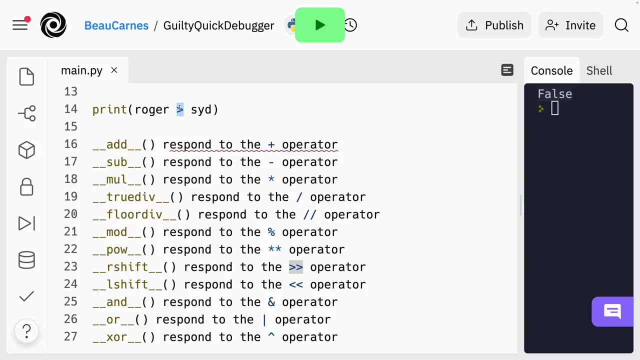 you can also create methods to go with different arithmetic operators. So we can do add, subtract, multiply, division, floor, division, mod power, So you can see all these different ones. you can make it respond to the different operators. So the example was just a greater than operator, But we can make. 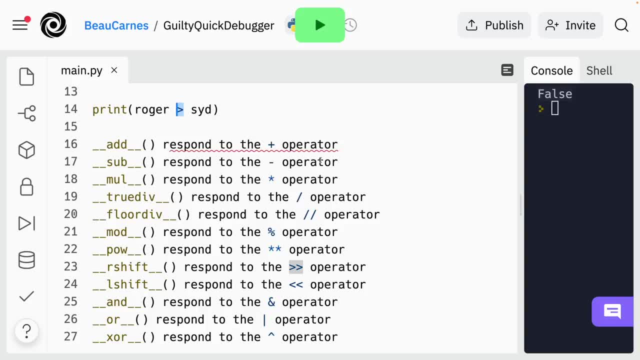 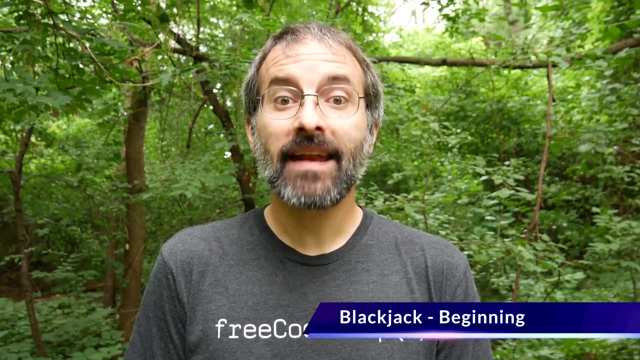 functions to show how it's gonna respond to all these different operators. There's even a few more methods to work with other operators, but you get the idea. We've learned a lot about Python And now we're going to bring a lot of what we've learned together to code a blackjack card game. 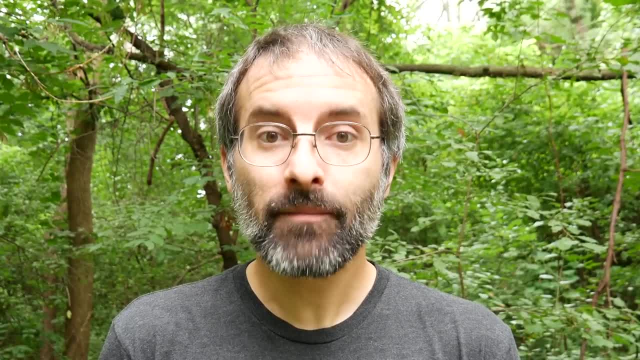 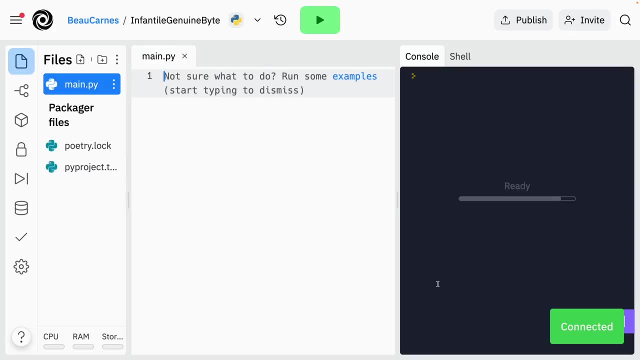 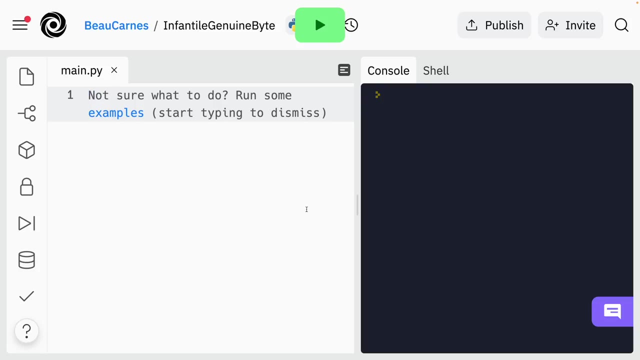 And in the process we'll learn about object oriented programming in Python. So we'll start by creating a new Python project on replit- And I'm just going to close this tab here And I'll zoom in just a bit And just like our first. 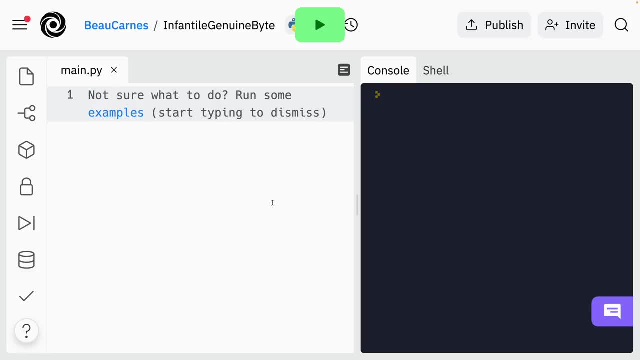 project. I'm going to say what I'm about to do And I want you to see if you can do it on your own before I show you how to do it. And with all you've learned so far, you're probably going to be able to figure it out on your own as I give you the instructions. 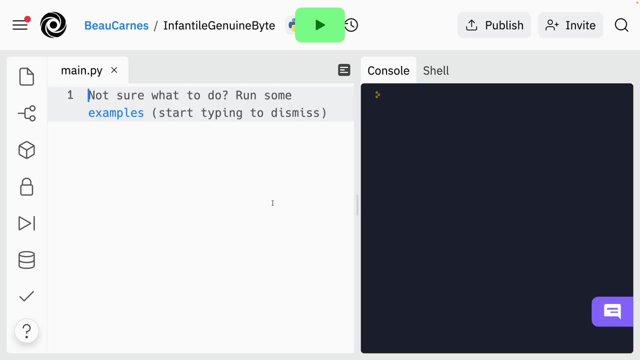 without even seeing how I how I do it. But then you can come back to the video and see how I do it, Or I guess you can just watch, not even try to do it yourself. But you're going to learn a lot more if you try to code this by yourself, along with me as I do it. but right before I do the different, 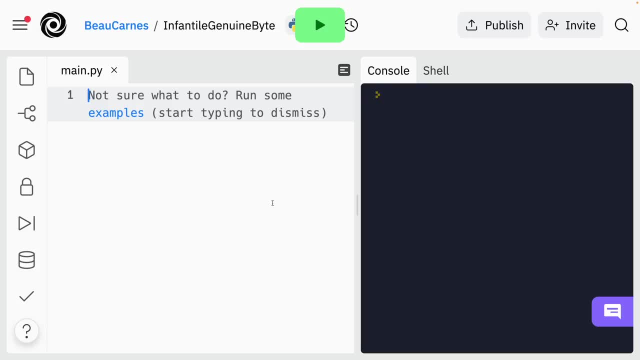 steps. So the first thing we're going to do is create a variable called the suit and set it to equal to hearts, and then a variable called rank and set it to equal k for King, and then a variable called value and set to equal 10.. Okay, simple, two variables equal to strings and one 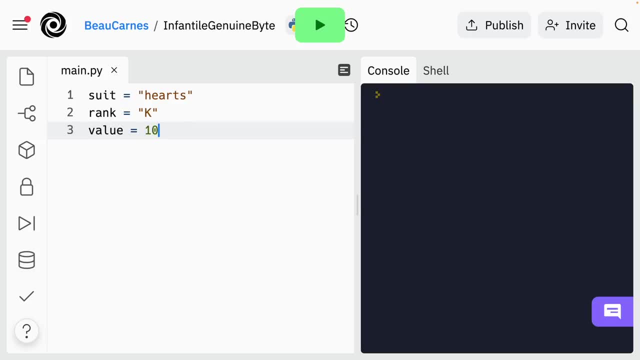 variable equal to an int. So now we are going to add a print statement and print the phrase your card is with a colon at the end, And then we'll add another print statement and print the rank. So now we're just printing the variable here And we're going to be doing a lot of refactoring as we create this program. Let's 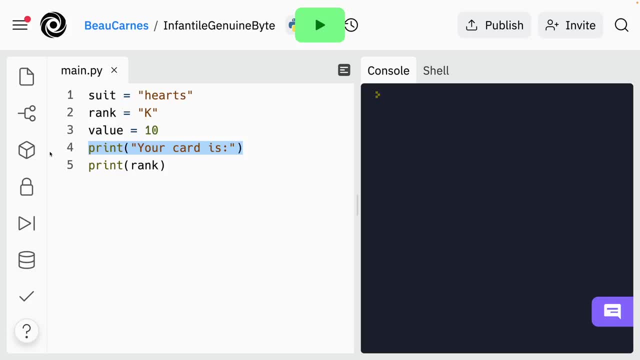 refactor this So it's just one print statement that's going to print your card is colon space and then the rank. So we are going to be doing string concatenation, Just like that, So you can concatenate as many strings and variables as you want. So let's update the 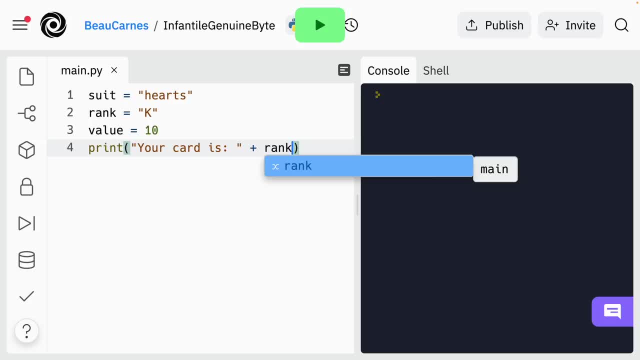 code so that the print function print prints your card is K of hearts. So we need to add of and we have to make sure we put spaces on each side of the word of and then suit, And let me just adjust this here. Okay, as you know, you can use a list and. 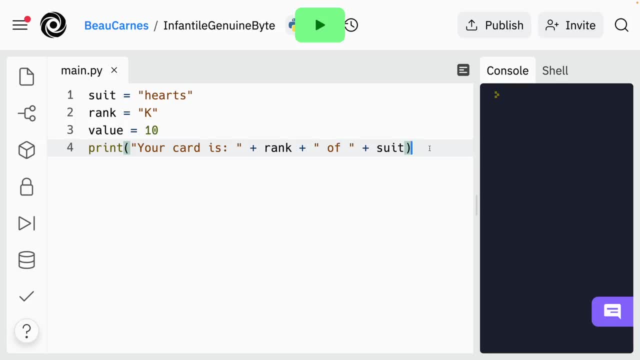 Python to store multiple values or items at a time. So, above the suit variable, create a suits variable and assign it to a list of suits, In this case, spades, clubs, hearts, diamonds. We learned about how you can use the bracket operator. 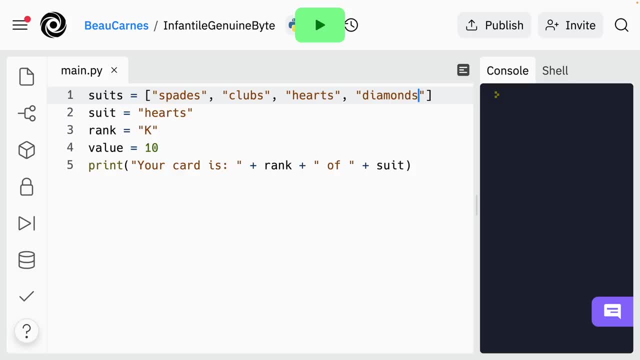 to access a specific element in a list. The number inside the bracket specifies the index of the list to access. remember the indexes start at zero. So you update the suit variable so that the value of hearts come from comes from the suits list. Now we'll practice a for loop. 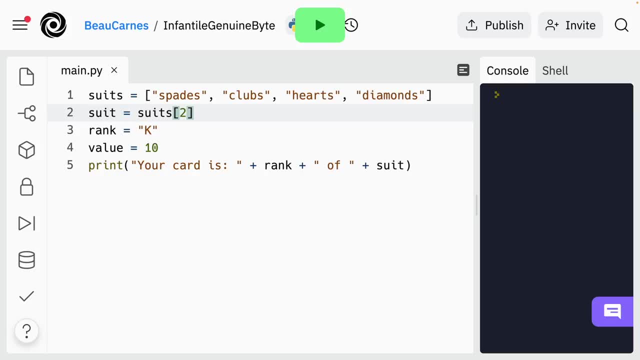 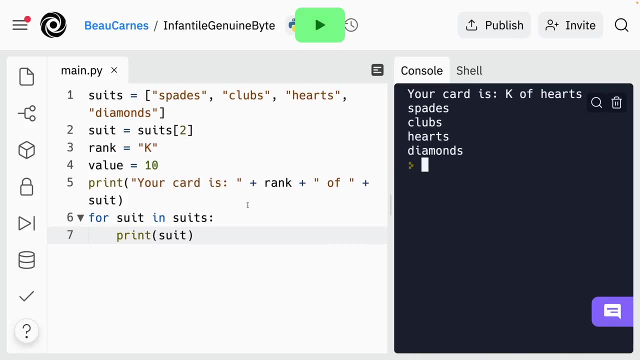 So add a for loop to the end of the code that prints each suit, And then we'll just test this out. I really hope you actually are following along and trying it out right before I show it to you. That's how you're going to learn the best here. So spades, clubs, hearts, diamonds. 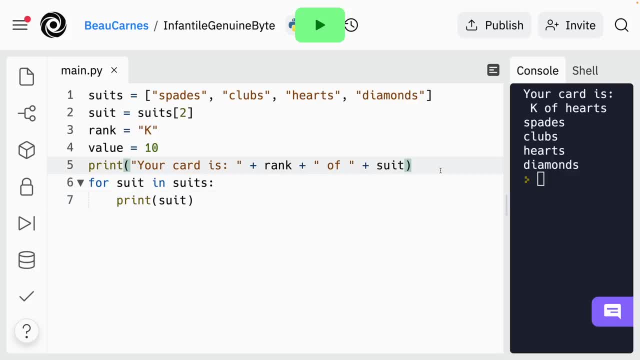 Now this next thing is is just to see if we can do it. So it's not gonna be part of our final code, But right before the loop we just added: see if you can add another item to the suits list. That's the string snakes. 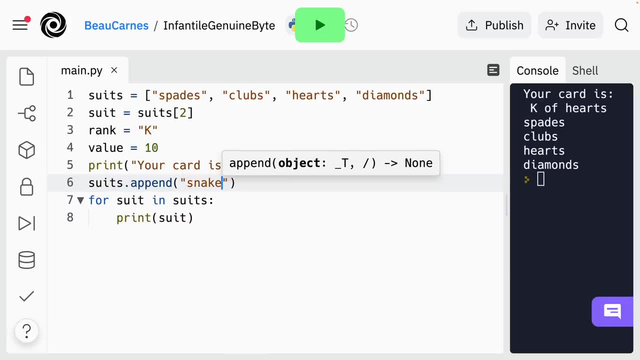 There's a few different ways to do it, But we will use a pin- snakes. So this is just going to up in the word snakes at the end of the list. So if I run this, we can now see snakes at the bottom. 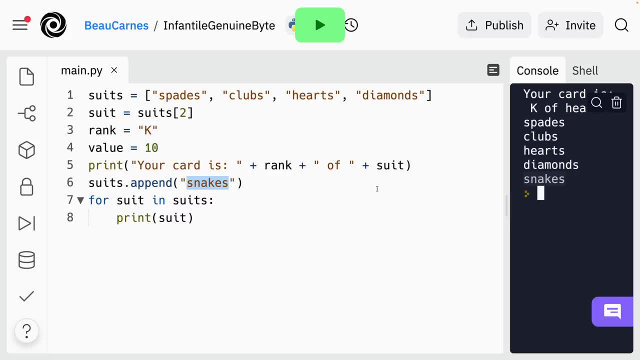 Okay, now we're gonna start the process of representing a full deck of cards, cards with Python code. So we're going to actually get rid of a lot of this. we're gonna get rid of all this, we're just gonna have the suits, And then we're going to have this for loop at the 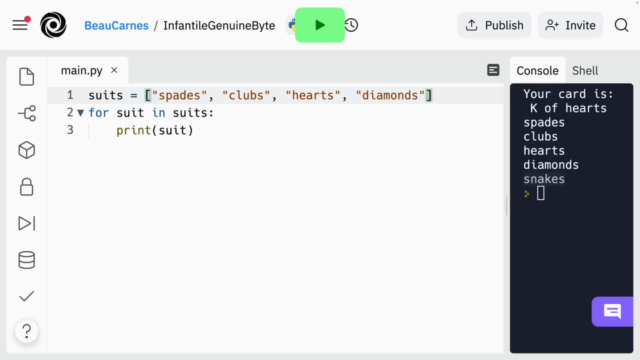 bottom. we're gonna do a lot of refactoring as we go, mainly for educational purposes, but also so we can get the really good blackjack game. So we have a list of suits. After that we're going to create a list of ranks, That's a: two, three, four, five, six, seven, eight, nine. 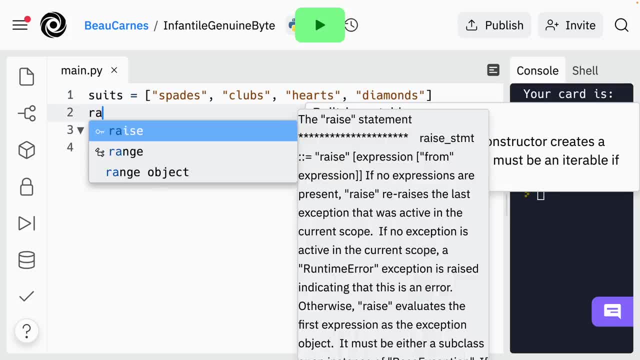 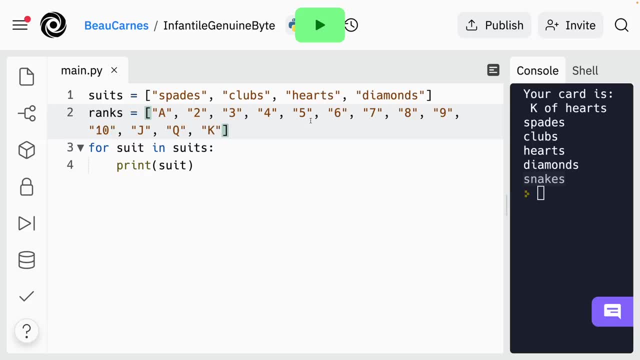 10,, j, q, k. Now, before the suits list, create a new variable called cards and assign an empty list to the variable You can. an empty list is just two brackets with nothing inside. Now in the cards list there should be an item for each of these lists, And then we're going to create a list of 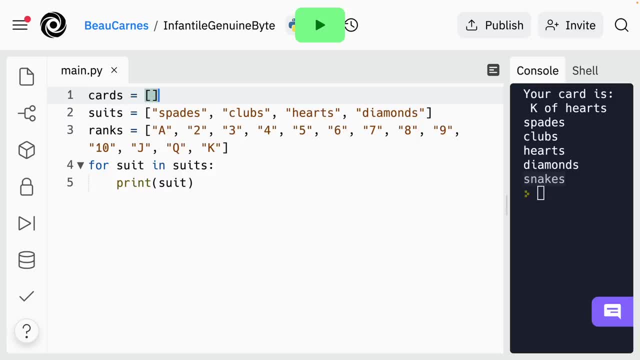 each card in the deck, Each item in the suits list should be combined with each item in the ranks list for a total of 52 items or cards. Let's work our way up to that. So first we'll update the print statement in the for loop so that it prints a list with two elements. The first element, 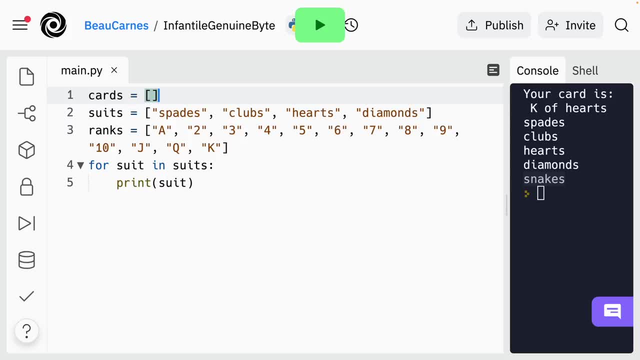 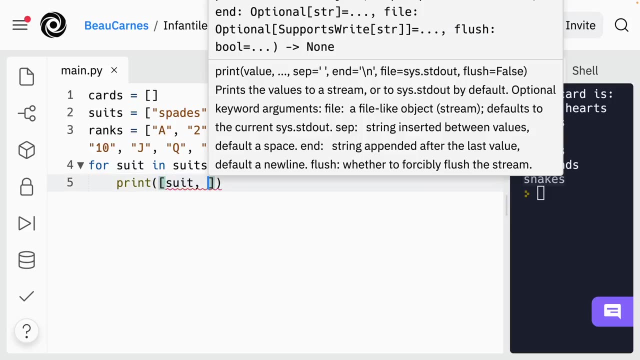 should be suit and the second should be the first element of the ranks lists. So this should print an ace in every suit. So I'm going to go ahead and create a list of suits And then I'm going to update this. So it's going to be a list with suit and ranks. The first item is going to be at index. 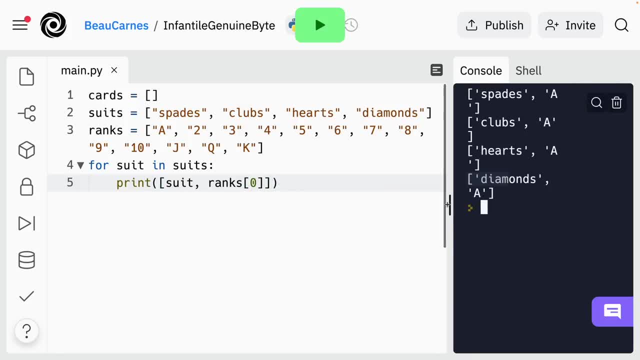 zero. Now let's print that out. So we got these four right here. Now, instead of just printing an ace in every suit, let's print every rank in every suit. This can be done easily with a for loop nested within another another for loop, So inside the for loop. 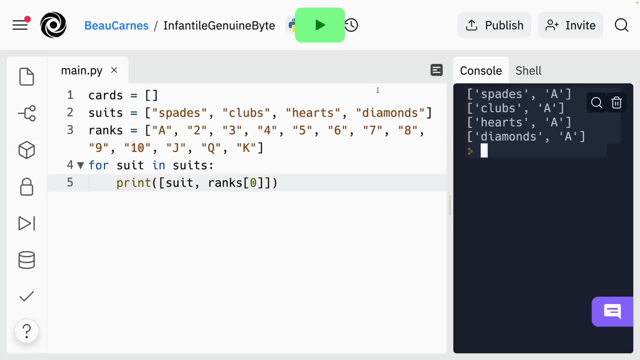 add another for loop that loops through the ranks, then update the print statement so that it's not just printing the first element in the ranks list but it's printing the rank from the four other for loop. So let me show you what I mean We're going to do for for rank and ranks. And then we have to. 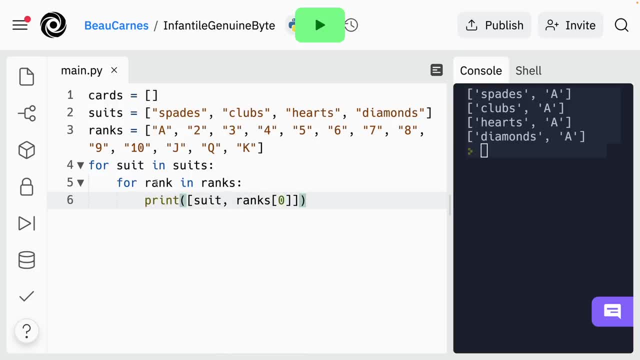 make sure to indent this print statement So it's inside the for loop, And then we're going to add this for loop And this is now just going to be rank, So it's going to print the suit and rank And I'll just run that And now we have, with this nested for loop, we have every card, every rank. 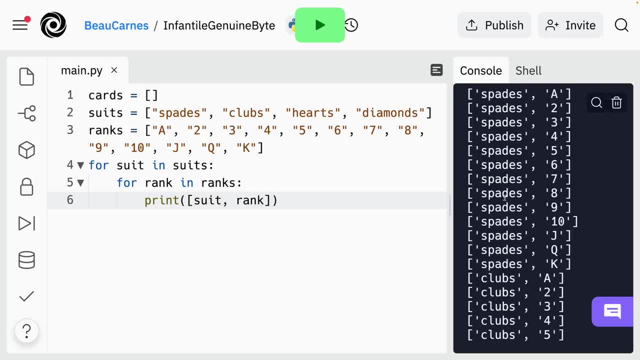 in every suit. all 52 cards are printed as two item lists. An element in a list can be another list. So instead of printing 52, two item lists, let's append those 52 cards to the cards list. So we already have the cards list here. it's empty, but I'm going to do cards dot, append And 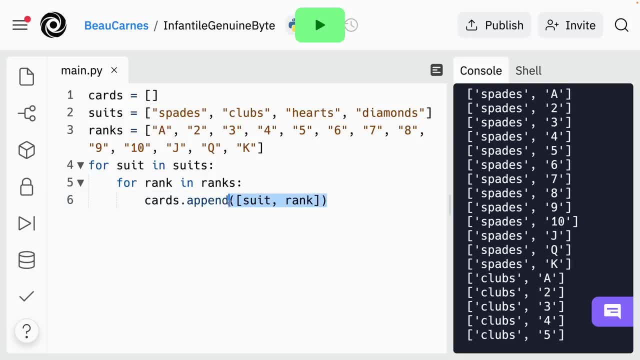 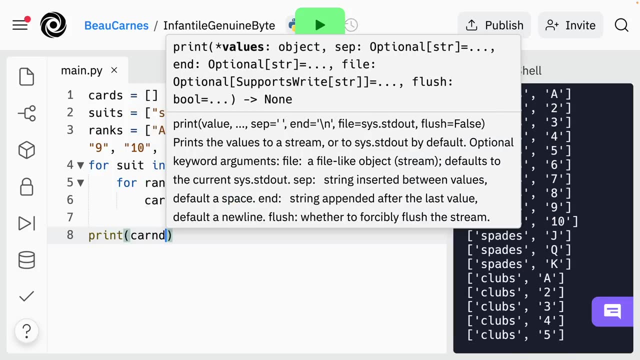 so we're appending this item, that all these items, to the cards list. So let's check what the cards list looks like by printing out. printing it out at the bottom- Remember, make sure this is not indented at all- And we'll do print cards And I'll run that. 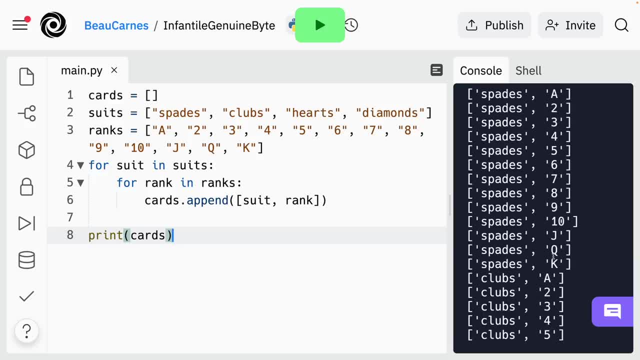 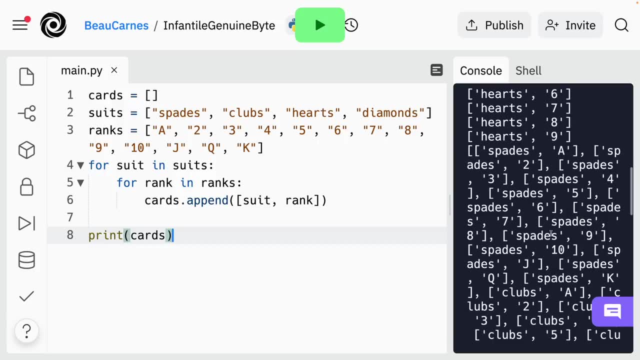 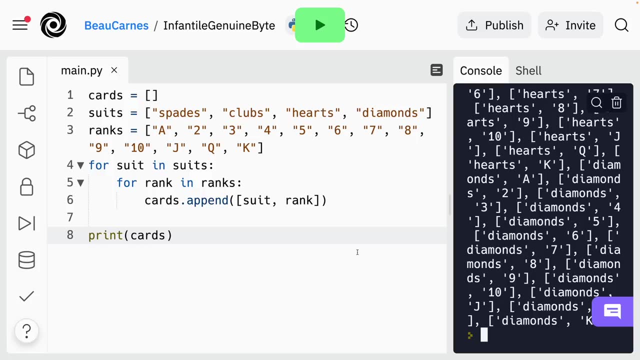 And then here it is here. So this is the list. It's not what. there's just a comma between each item in the list. here You may notice that all the cards are in order in the cards list. For a game like this, though, the cards must be shuffled. So to help with this, import the random module at the 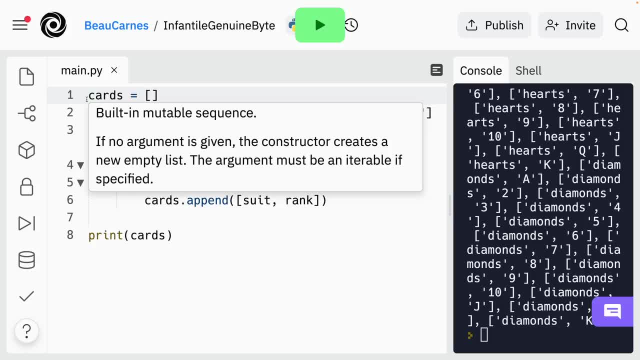 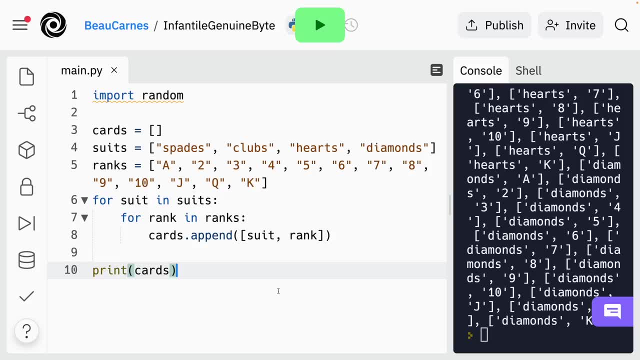 top of your code. So that's just. we just do import random. Now we'll be able to use the, the random module. So this is going to import the random module, which contains a variety of things related to random number generation And, as you. 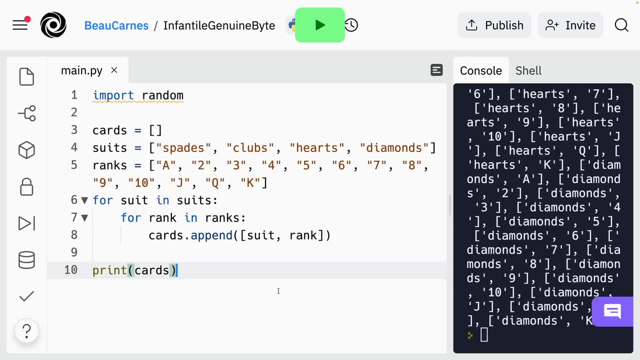 probably remember, when you import a Python module, it allows you to use additional commands in your code. Specifically, we're going to be using the random dot shuffle function. So right before at the end, which says print cards, we're going to call random dot shuffle and pass in. 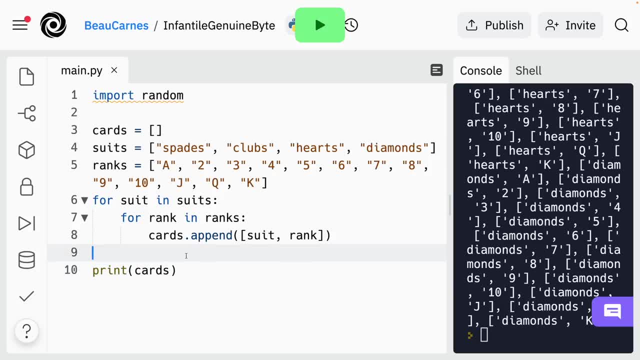 random dot shuffle. So right before at the end, which says print cards, we're going to call random dot shuffle. So right before at the end, which says print cards, we're going to pass in the cards list to that function And then, if I play this here or run the program, we can see that these are not in. 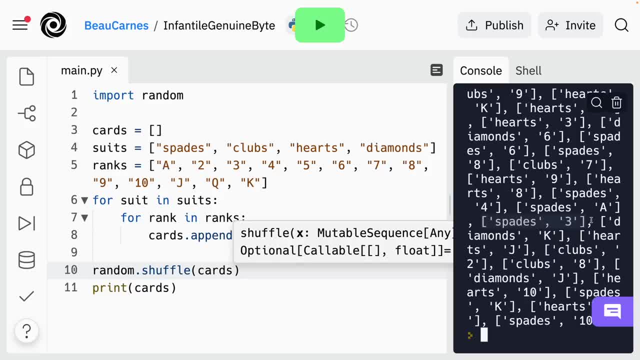 order anymore, See ace of spades, three of spades, king of diamonds, jack of hearts. So these are no longer in order because they've been shuffled. Now let's remove a single element from the cards list. This is similar to dealing a card from a deck, And this can be done with the pop method. So after the 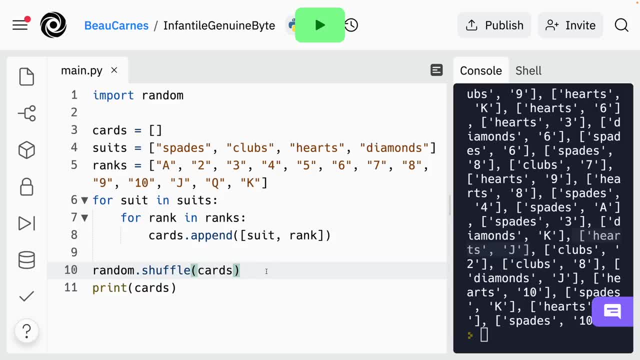 cards are shuffled. let's create another card variable and just pop off a card from the cards list and put it into that variable called card and just print that card. So I'll do card equals cards, dot pop And then, instead of printing all the cards, I'm just going. 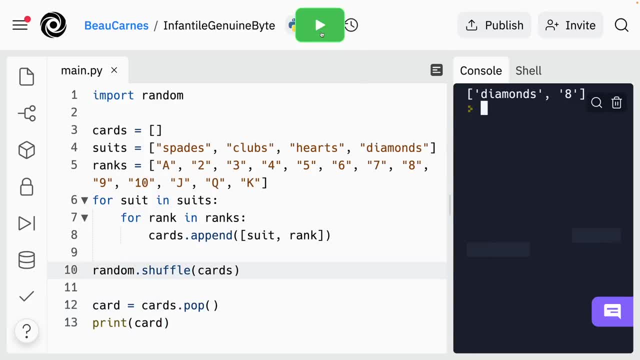 to print a single card. I'll run the program. See, every time I run the program, you can see we're getting a different card. we're dealing a different card because it's been shuffled. So we've already learned all about functions And now we're going to create a function. 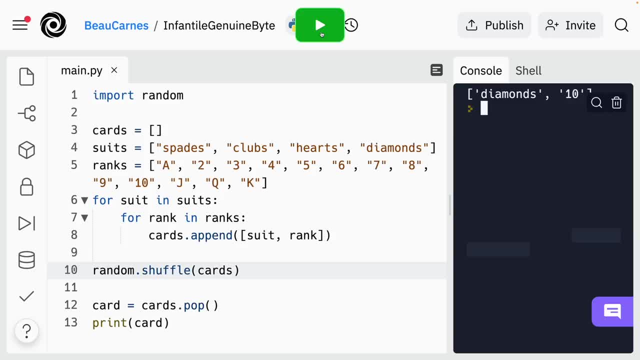 So create a function called shuffle that just has the single line that shuffles the cards, So it's a step shuffle, And then I just have to make sure this is indented. So now when we call the shuffle function, it will shuffle the cards. So right before the print statement. 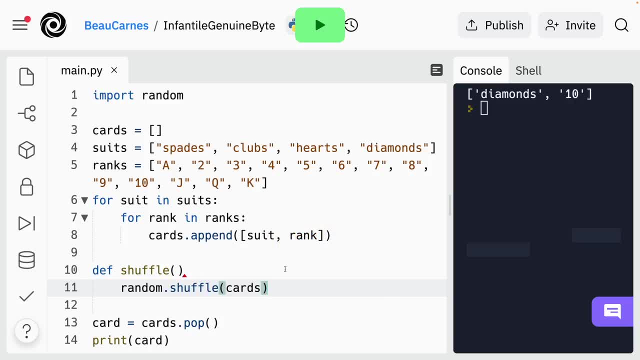 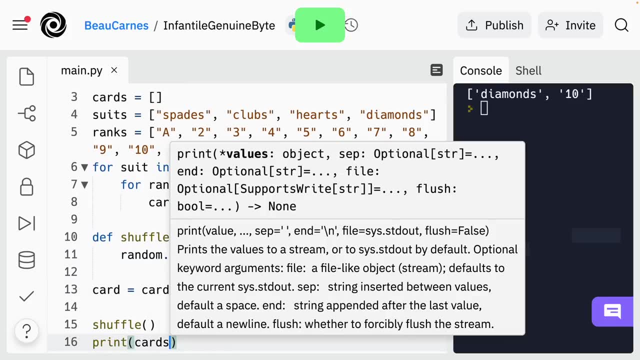 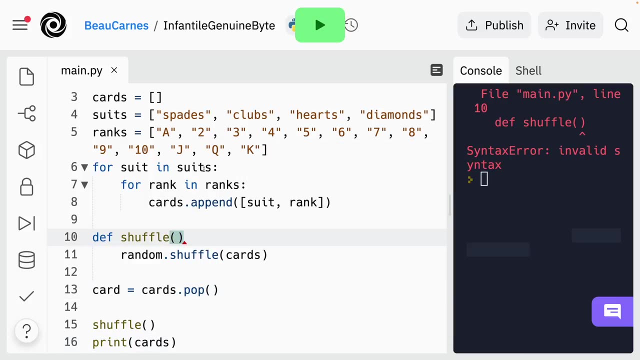 call the shuffle function And instead of just printing the single card, print the cards. So do shuffle, And then I will print all the cards. And let's just try out the program And we can see there was a problem. It's because we didn't put the colon here. 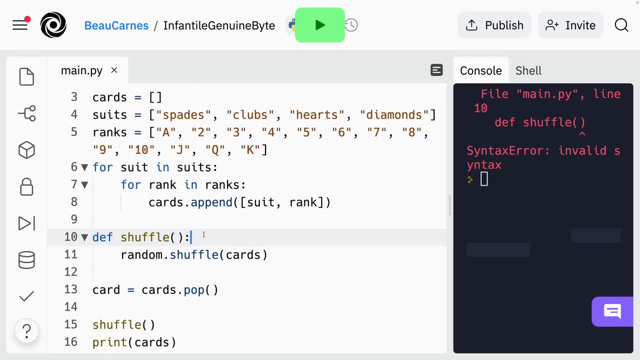 So that's an important part of creating a function is putting the colon there. Now we'll create another function called deal And we'll put this line inside the the deal function. So we're going to define deal And I'll put the colon this time. 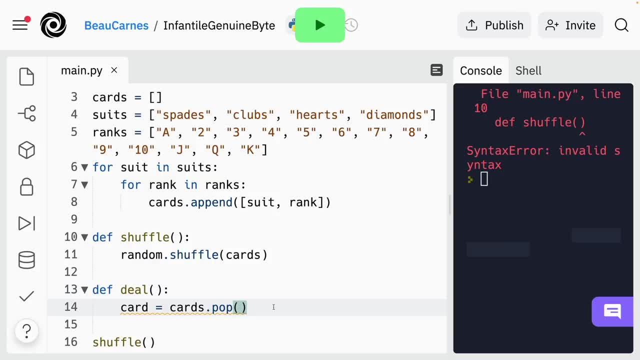 and make sure to indent that, And we can see this has a orange squiggly line underneath it, because variables can only be accessed in the context that they were created, So the card variable will not be available outside of the deal function. you can get a value out of a function by 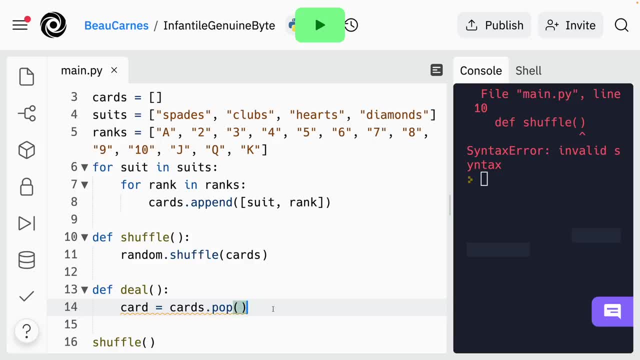 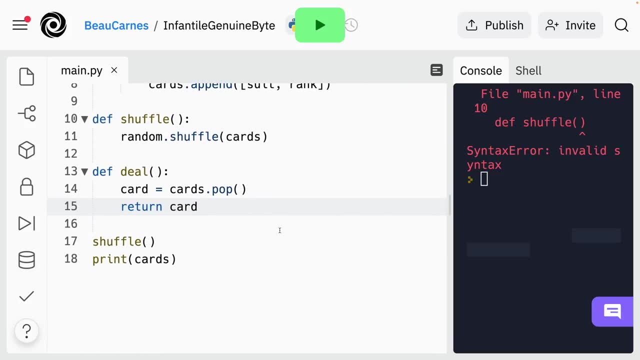 returning a result using the return statement. So at the end we're going to return the card. Okay, now we've taken care of that squiggly line there. So after the shuffle function is called, we'll call the deal function and assign the return value to a variable named card. Then 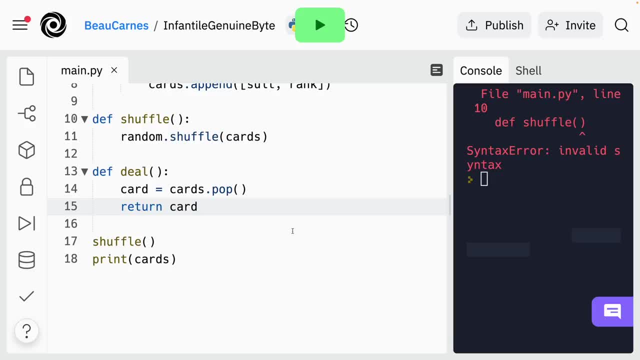 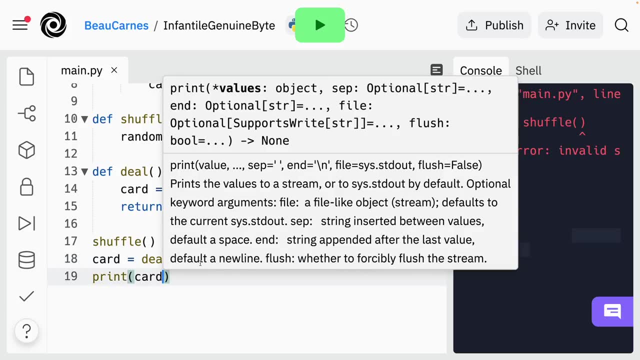 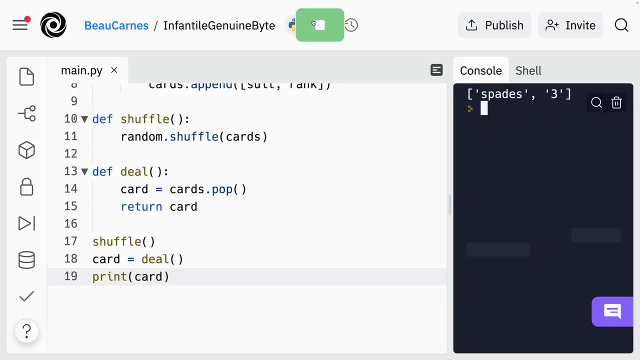 we'll update the print function to print card instead of cards. So card equals deal, And then we'll just print the card And again we see a different card every time we run the program. What if you want the deal function to deal more than one card? Well, let's refactor the deal function to an accept to accept an. 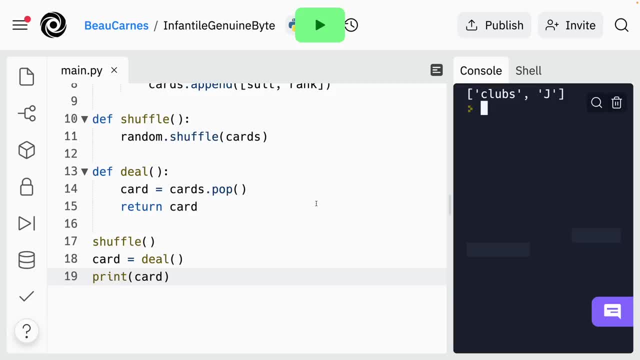 argument, So any number of arguments can appear inside the parentheses when a function is created, separated by commas. Inside the function, the arguments are assigned to variables called parameters. So start by making it so. we'll start by making it so the deal function takes an. 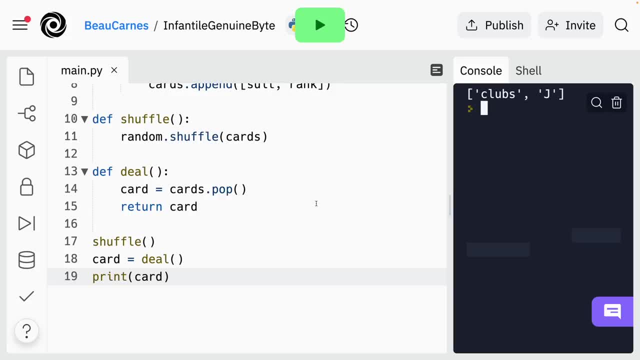 argument named number, then we'll make sure, when we call the function, we'll make sure that the deal function is assigned to the argument named number, And then we'll make sure, when we call the function, we use the new parameter by making it. so we're going to deal two. 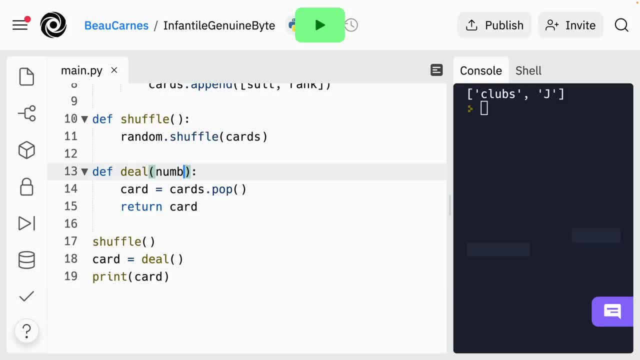 So I'm just going to put number: here is going to deal a number of cards and we're going to deal two, And I just didn't say this before. But now instead this is not one card anymore. So we're going to update this to be cards dealt. But there's a special shortcut you can either. it's: 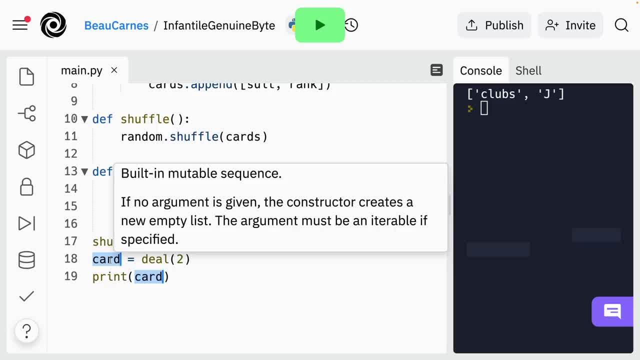 going to be come command or Ctrl D, And now I'm actually selecting the card two different times. See, I now have multiple cursors here. So basically, I selected the word, I double click to select the word, then did command or Ctrl D. Now it's selecting two words And now I can type in: 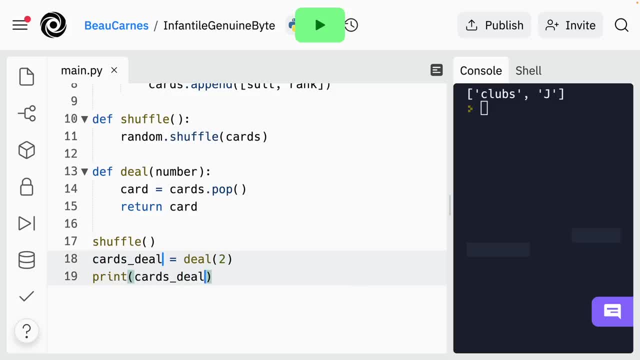 cards dealt. So now I can type in two places at one time. So that's a cool thing that you can do in replete And you can do it in many other code editors And I'll run the program. but it should still only deal one card, because even though we're passing this parameter into here, we're not doing. 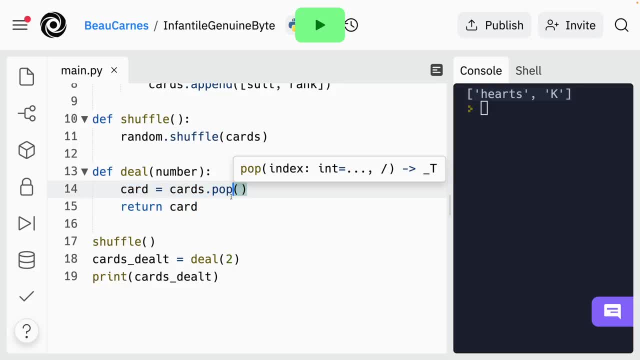 anything with it. So I'm just going to do that, And then I'm going to do that, And then I'm going with it yet here. So we want to update the deal function. So it's going to return a list of cards. 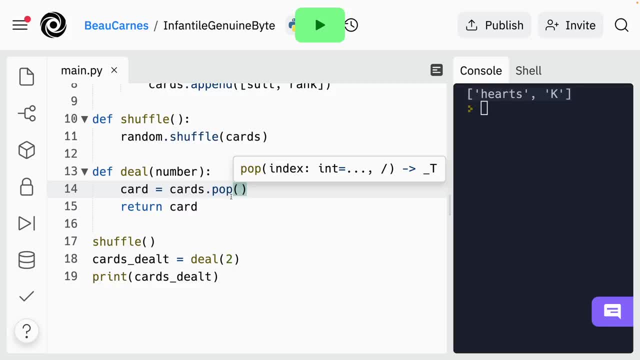 instead of a single card In the first line of the function, create an empty list named cards dealt. then update the last line of the function to return cards dealt instead of return card. So let's do that really quick. We're going to do: cards dealt is going to equal an empty list And 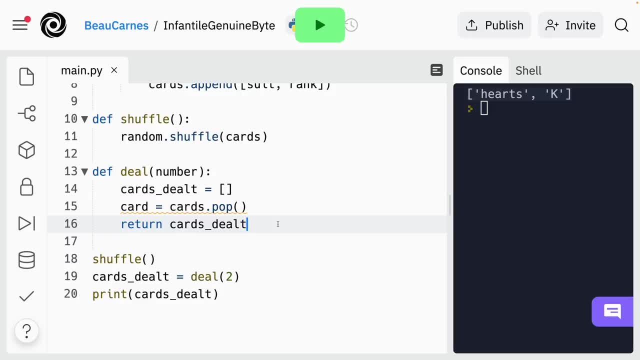 I'll just copy that and paste it right here And then I'm going to do a new function And I'm going to change this to do is I'm going to use the add a card from the deck for each card dealt. So we can do that by creating a for loop for X in range. number. Now this is a common thing you're going to be doing in Python, creating a for loop for X in range number. Just remember that the formula is essentially the wahoo argument. right, Let's go toków des говорamhet ish. could Х user nal jogam OutKard sio and. 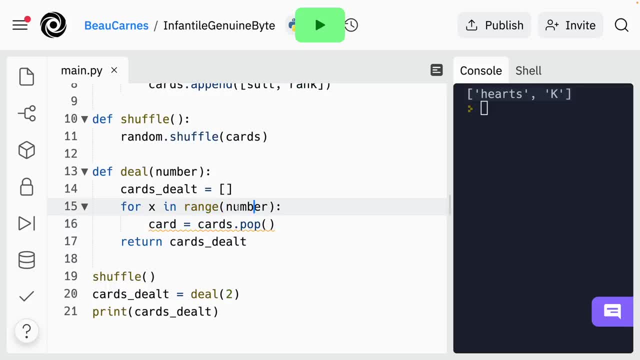 enter like a interrupt Jones is equal to P zero, yal, Let's give it a little��안 ale And loop that's going to be in range number, because now it's going to loop this many times. it's going to loop this many times, which is the number we pass in here, And we're going to do a few things. 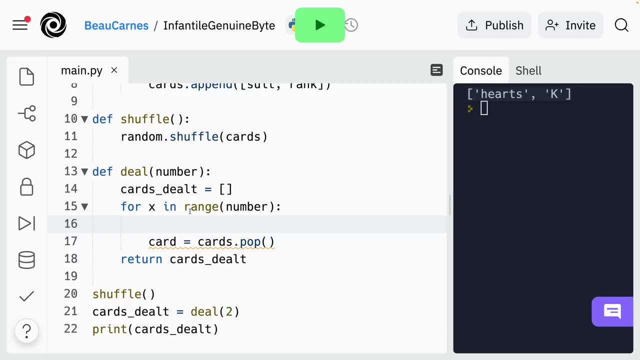 in this for loop. First we are going to actually do this, what we already have- card equal, cards, dot pop- And then we'll do cards dealt- dot append card. So now we're just this card that we popped off the deck, we are appending it to the cards dealt And then we're returning the card dealt. 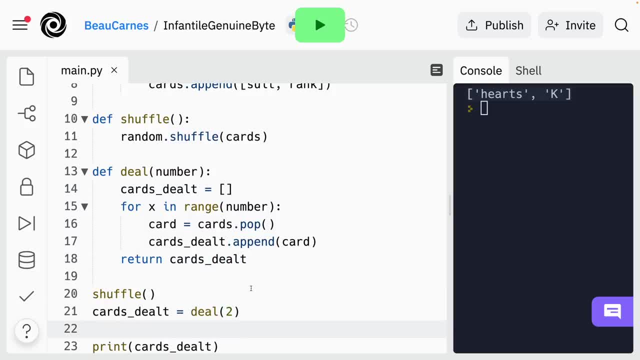 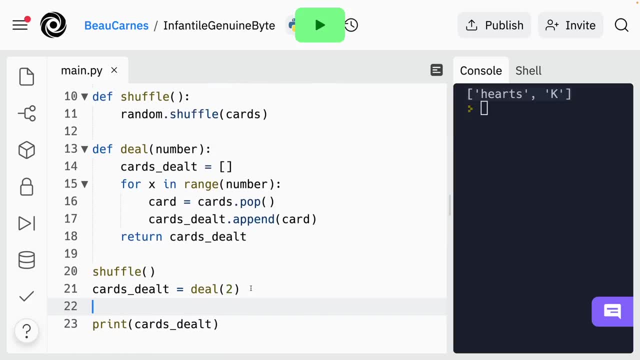 here. So down here in the code let's separate out a single card from the two cards dealt. So let's create a variable called card and set it equal to the first item in the cards dealt list And then we'll just print that card instead of cards dealt. So we are. 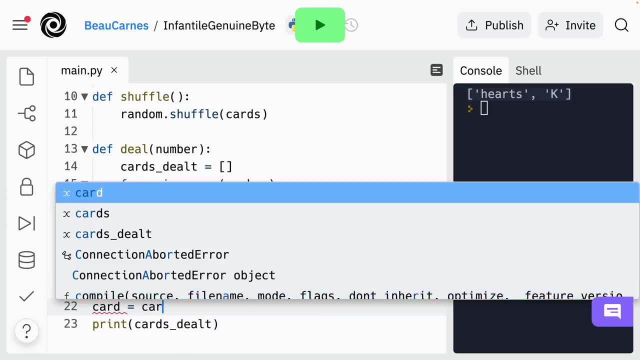 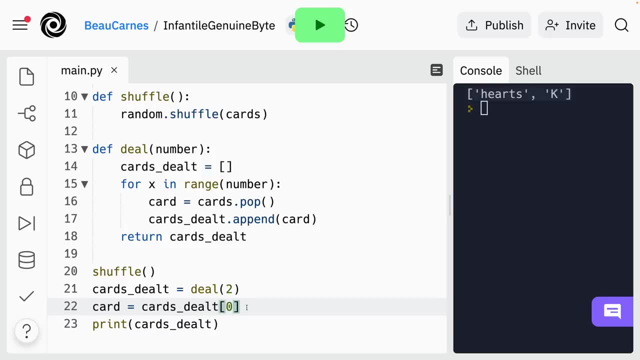 going to do card equals, cards dealt, And then we just use the brackets and put zero to get the first item in that list And then we'll just print a card. Now I'm just going to test out the program, or still just seeing a single card here, But it's doing a lot more behind the scenes. 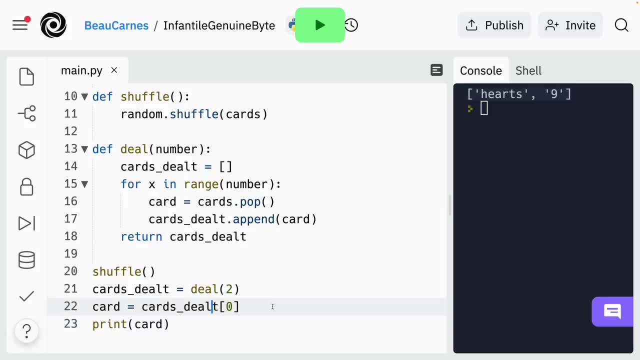 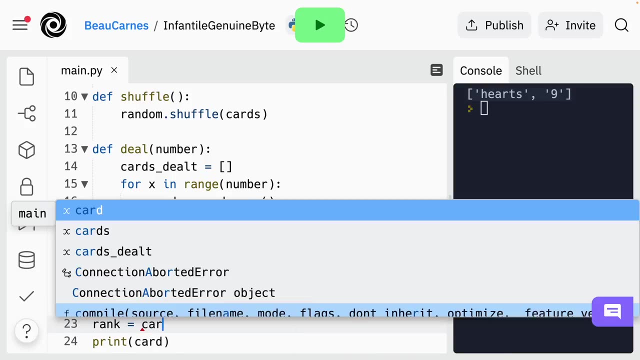 Now. So now let's separate out the rank part of a single card. So after we create the card there, let's create a variable named rank and assign it the rank from the card. So we'll do rank equals card. And then I have to get index one because the rank is this. that's the nine here. 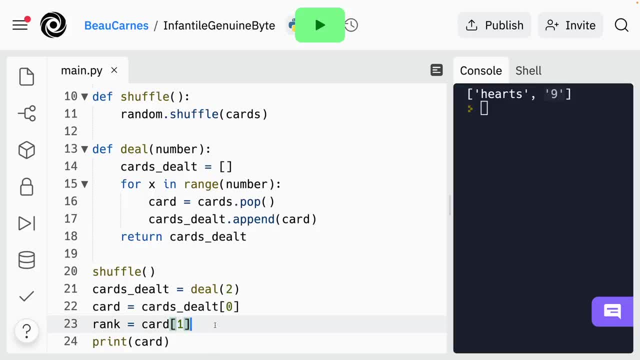 the second item in this card is the rank. So each rank has a different value And blackjack. the value of an ace or an A in this, in this program, is 11.. Or sometimes it can actually be one. it's gonna be 11, or one, but we'll get to the one part later. So Jack J Q. 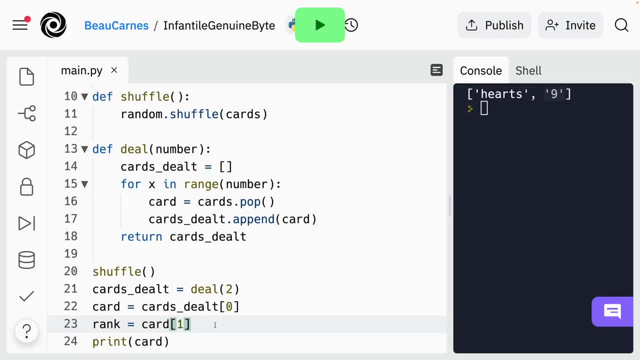 and K, which is Jack, Queen and King, have the value of 10.. And then the numbers have the value of the number. So we need to check what the rank is and set the value depending on the rank. So this is the perfect time for a conditional statement. Specifically, 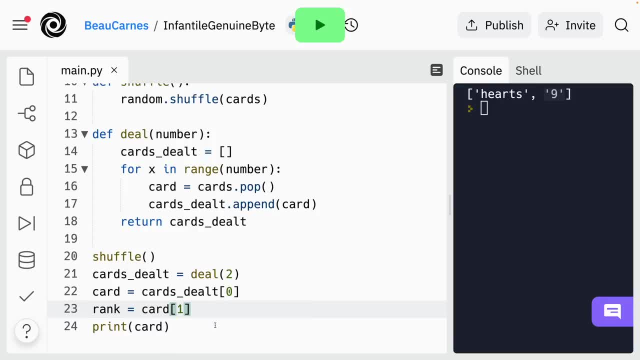 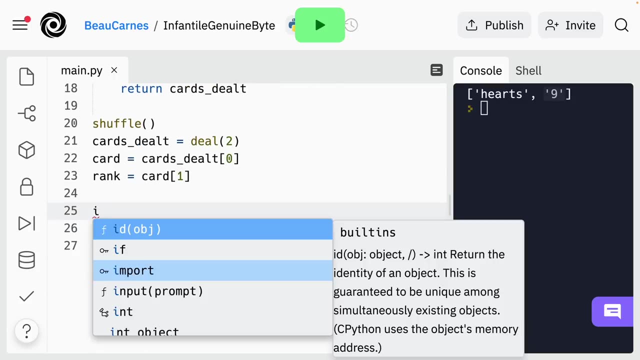 an if statement. Before the final print statement or program, we're going to add an if statement to check if the rank equals a and if so, we'll assign 11 to a variable named value. So we'll do if rank and I hope you remember, if you're following along, I hope you remember to use 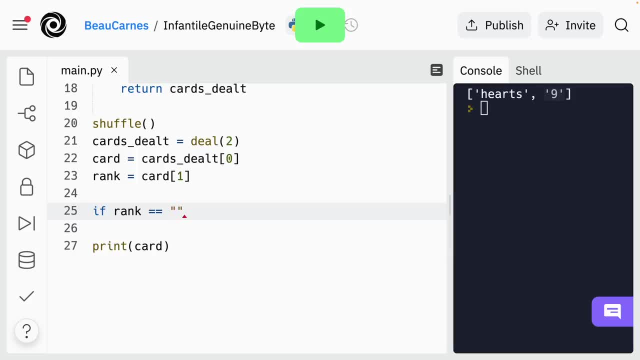 two equal signs instead of one equal sign here. So if rank equals a, then value is going to equal, with a single equal sign is going to equal 11.. Now, if rank does not equal a, we'll want to check if equals j, q or k. That can be done with an LF statement. For now we'll just create an LF. 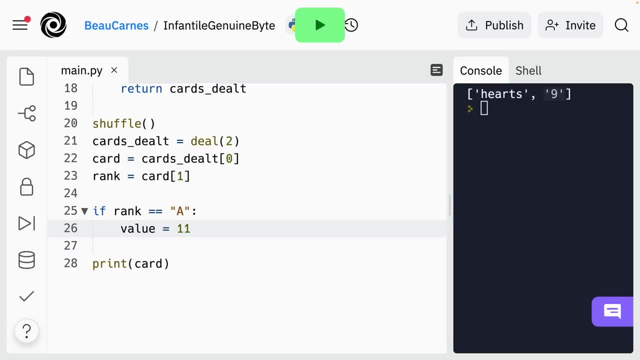 statement to check if the rank equals J And then, if so, we will set the value to 10.. So we talked about the three logical operators, and or and not. you can use these three operators In conditional statements to check multiple conditions at once. So we want to check if rank. 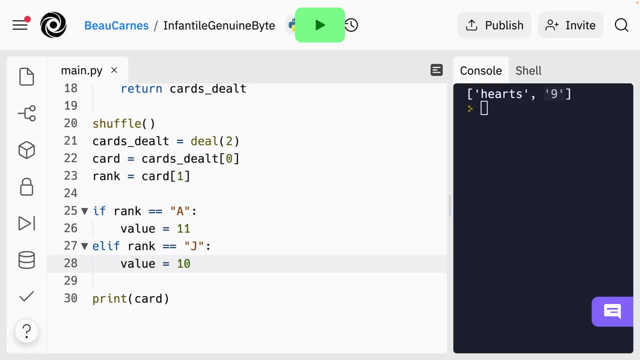 is J or rank is q or rank is k. So update the code with the ant with the oars. Now there can be any number of LF statements after an if statement, But at the end there can only be a single L. 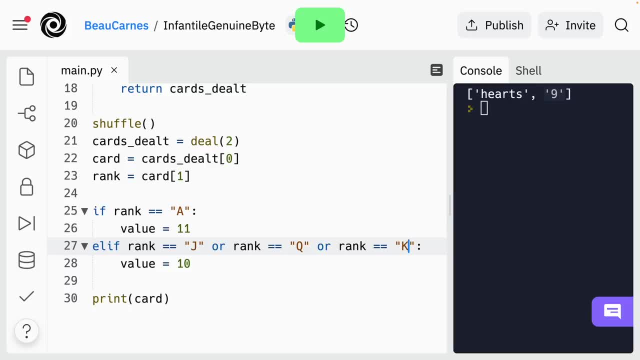 statement And, like we discussed, else is just going to be if none of the other ones are true. So let's add an L statement And inside we'll just assign rank to value, because we've already gotten all the letters out of the way. The rest are numbers and we can assign it directly to the value. 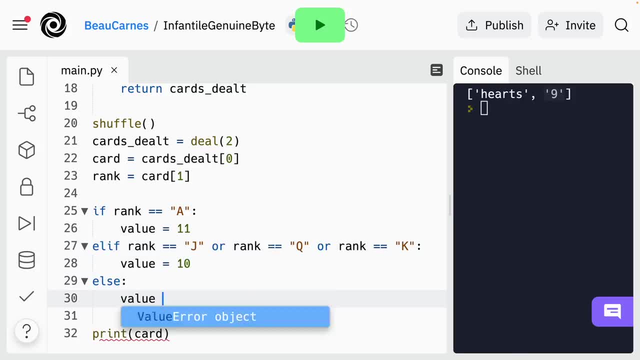 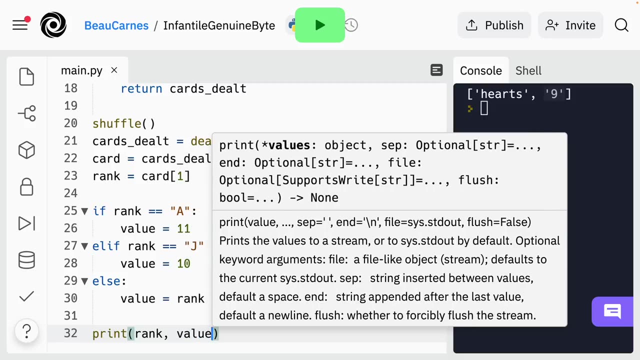 Now we'll, instead of printing the card at the end, let's print the rank and the value. So I can just type in rank, comma, value And when that multiple values in a print statement are listed with a comma separating them, both values are printed with a space. 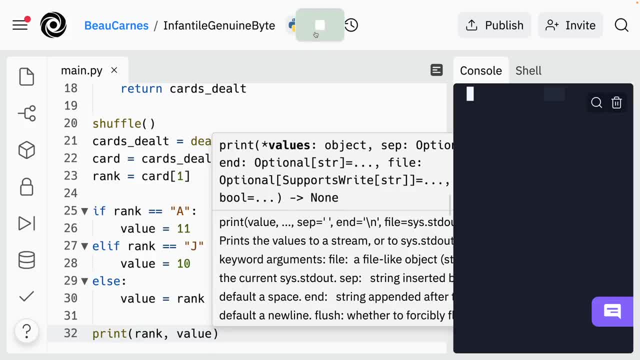 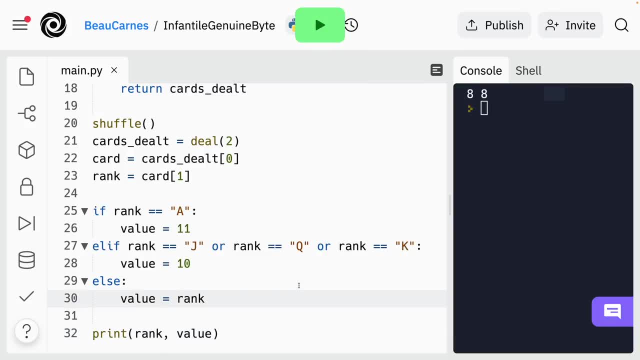 In between. so let's test this out a few times: q 105566.. So we can see every time we press it. it's going to be a random rank and value. Now we already talked about dictionaries. in Python it's like a list, But more general. you can think of a dictionary as a mapping between a set of. 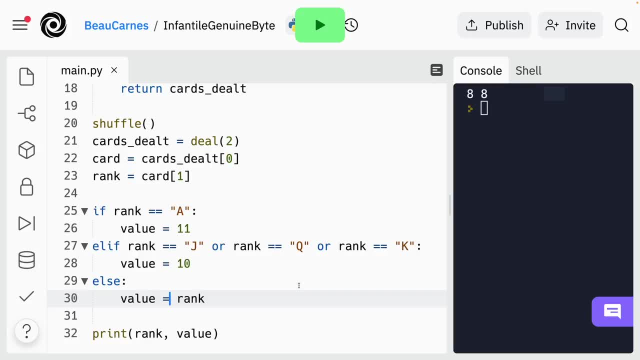 indices, which are called keys and values, So key value pairs. each key maps to a value. So, above the print statement, let's create a variable called rank. underscore di CT for dictionary, and create a dictionary with two items: a key value pair for the rank and a key value pair for 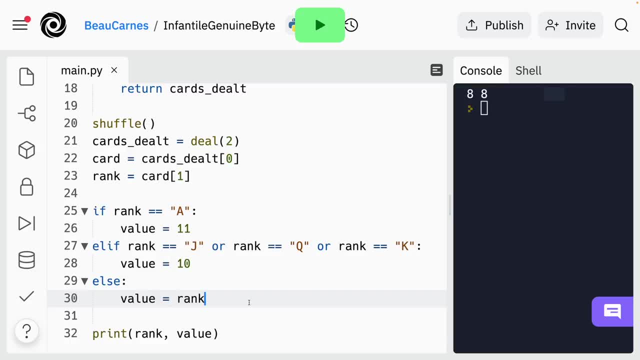 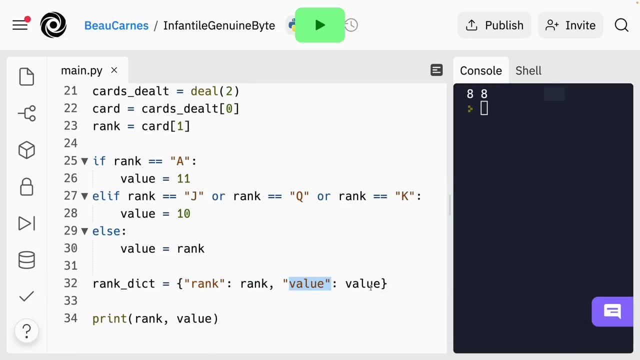 the value. So we have the string rank here and then the actual rank variable, string value and the actual value variable before we are printing the rank variable and the value variable. but let's update this code So we're actually getting the rank and value from the 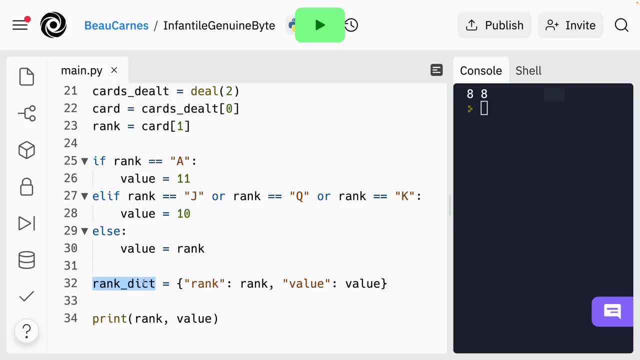 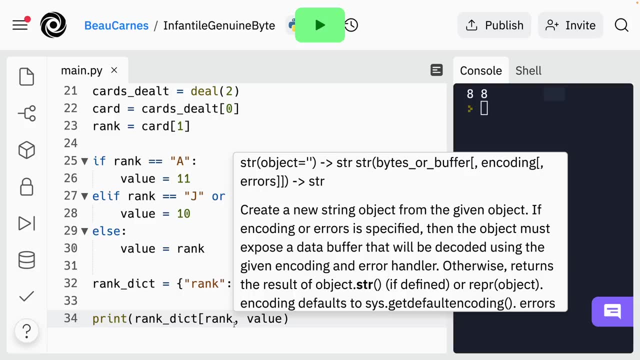 rank syntax. And now let's break this code down and now we can use built general n elements by dictionary, right here. So I'm going to copy that And then I just pasted that. But now I'm going to use bracket notation And so I'll put two brackets, but then I also have to surround this in quotation. 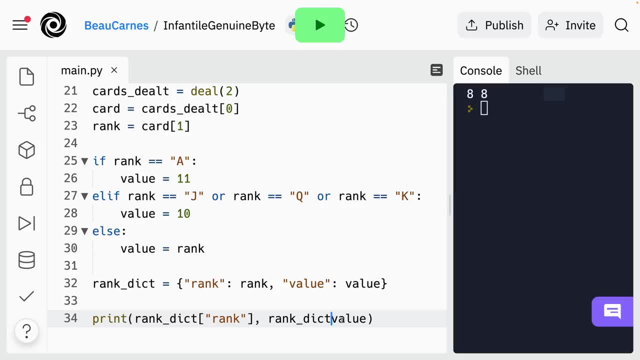 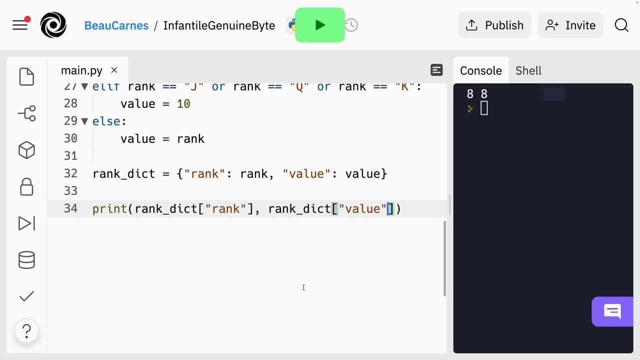 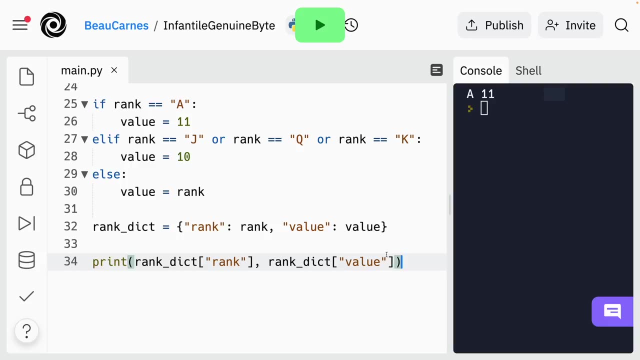 marks, And then I'm going to put the rank dictionary, the brackets and then the quotation marks, because we're accessing that key there, And then I can just run the program And it's still doing the same thing as before, just a lot more complicated as far as the code goes, But it's. 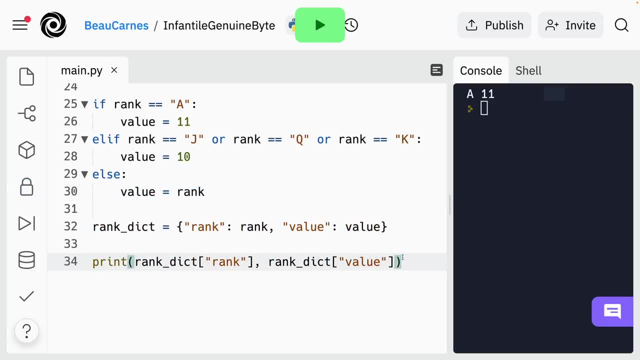 going to be good to have more complicated code, as our program is going to become more complicated as we go. So when writing a program, there are many ways to do almost everything. Now we're going to refactor the code to get the value of each rank without using an if statement Instead. 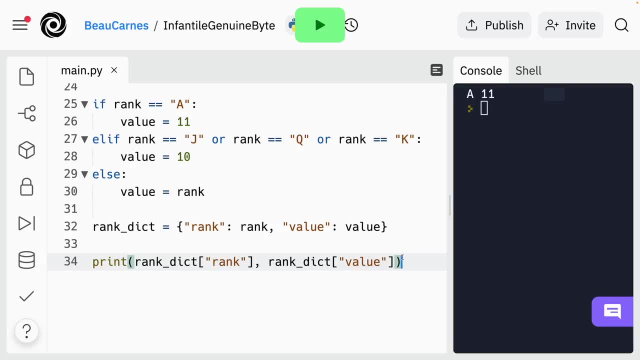 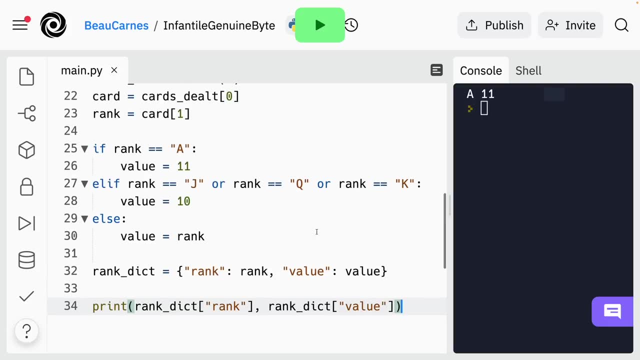 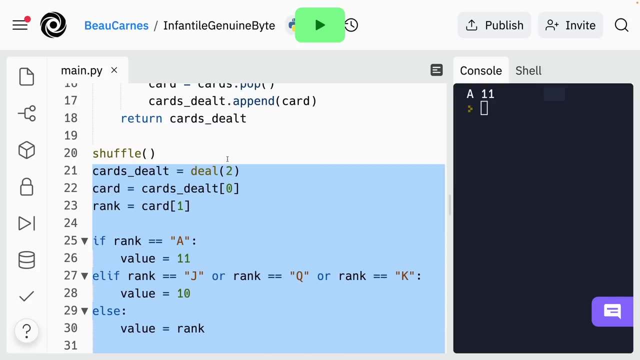 we'll store both the rank name and value in the ranks list using dictionary. So let's delete all the code lines of code after where it says shuffle. So here I know we typed in a lot of stuff there, But it was just kind of practice And now we're. 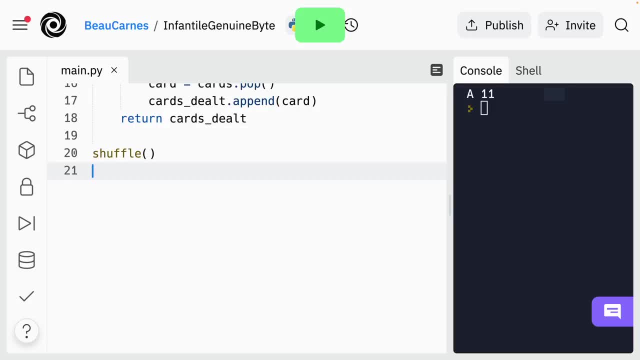 going to practice a different method of doing this. So now let's create a new card variable, new variable called card at the end, And let's assign to the card variable a single card that will deal from the deck, but we'll make sure that card is not in a list. So 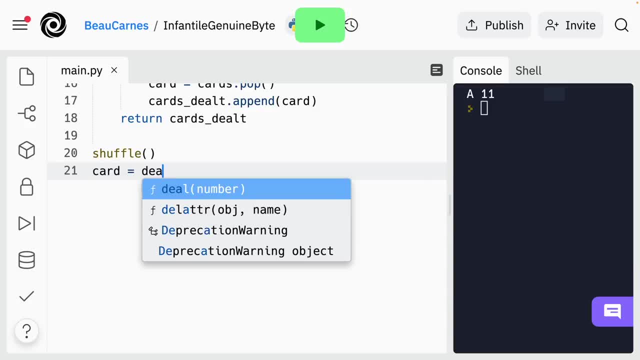 this is a little tricky. I'm going to do deal and I'll deal one card, But now I have to get the first item. So this is going to deal one card, but the one card is going to deal is going to be. 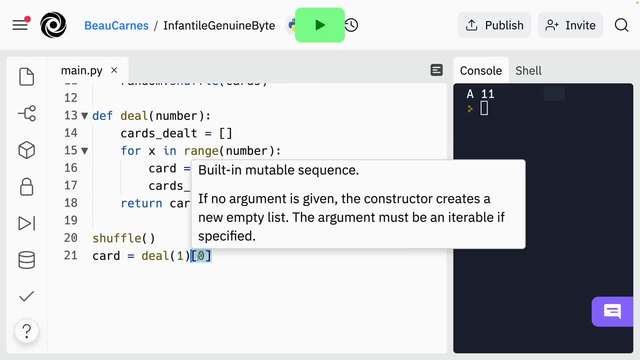 in a list. So I want to get the first item in the list, which is going to be the only item in the list. So I have to put this zero in brackets here to get that card out of a list before it goes into the card variable. Now we're going to update the 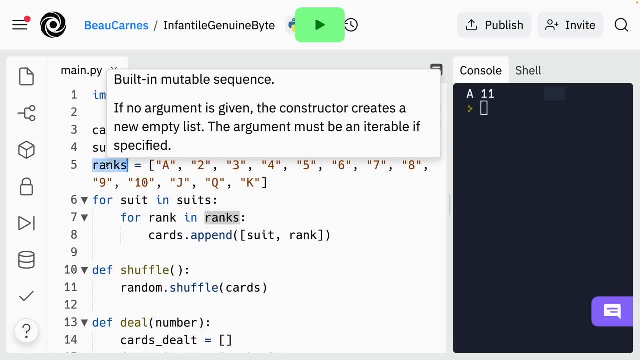 ranks list. So here's the ranks list: each element. the list should now be a dictionary. When lists or list elements are long, it's common to put each element on its own line. So we're going to put each element on its own line And each element is going to have the rank and the 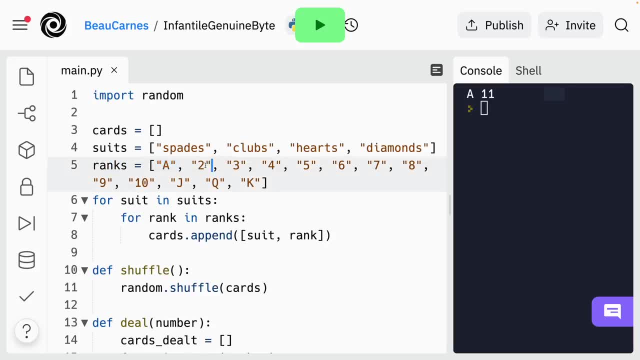 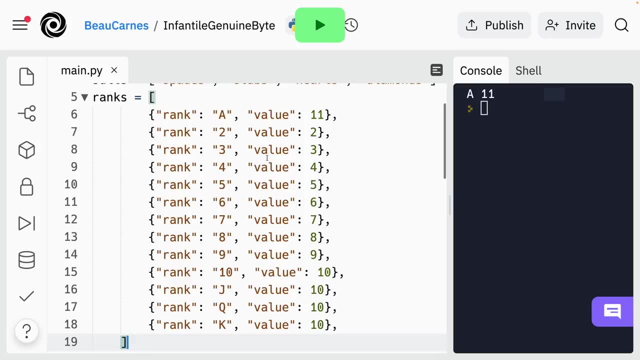 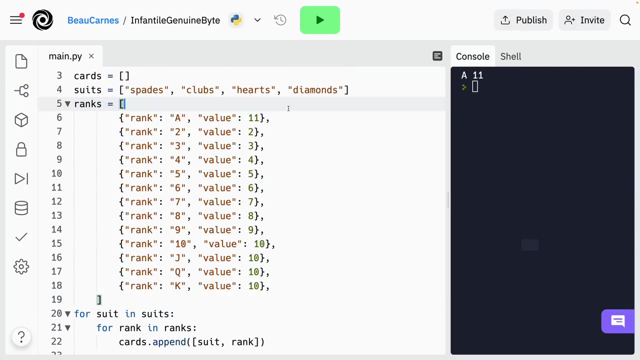 value. So, for instance, it will be a rank, a value 11, rank two, value two. So it's going to look like this- And now I'm actually going to zoom out just a little bit- And we have all these. there are all these ranks, and each one in this list is a dictionary. 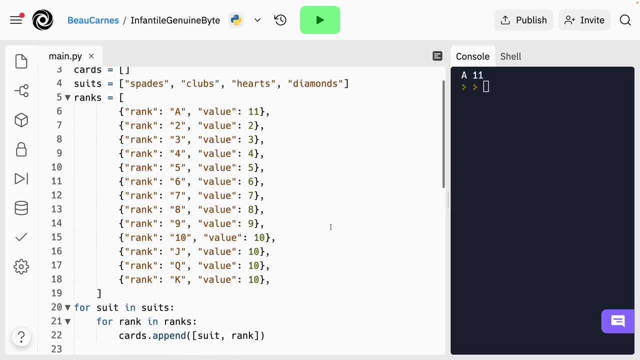 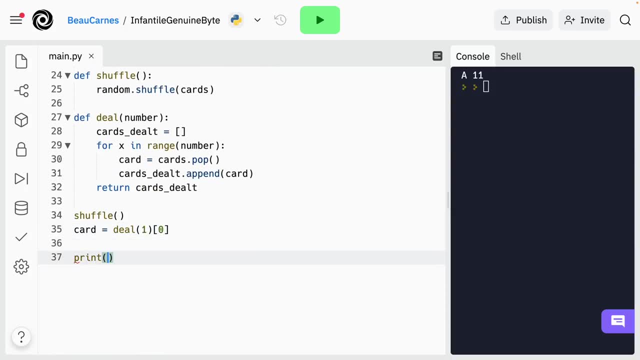 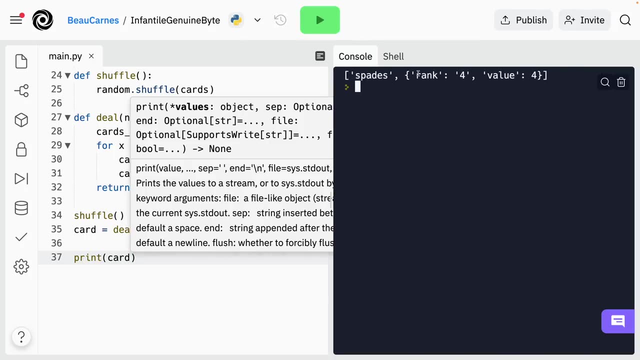 each element in the list is a dictionary. Okay, now that this is updated, let's go down and just print a card So we can see now that we've updated that ranks list. So print card. Okay, so this is what it's going to look like coming from our list. So we got the suit And then we have the rank. 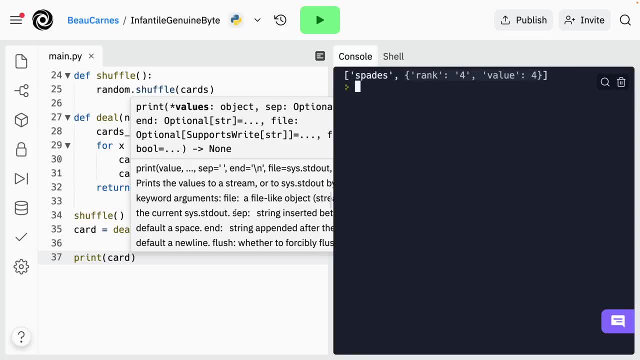 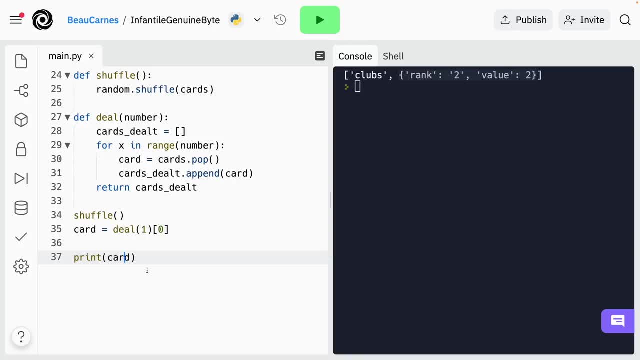 that's also going to have the rank. And then we have the rank. that's also going to have the value Here, the rank and the value We can see every time I click it. we get a random item. Now let's update the code. So instead of printing the whole card, we just print the value. So in this example, 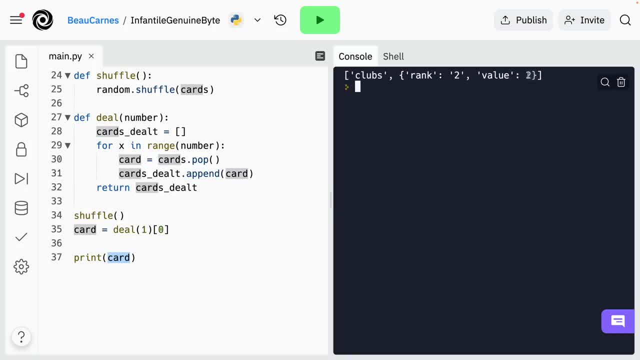 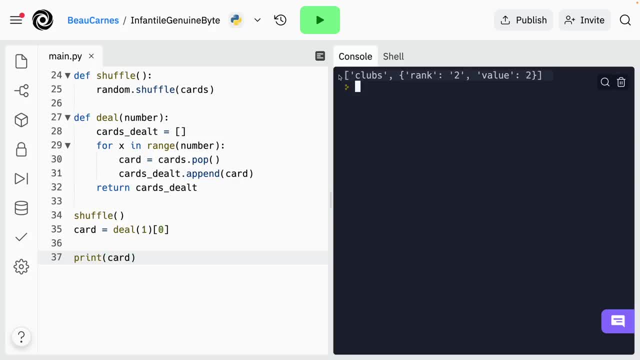 there. So first of all we have to see that we're in a list And we need so. this is the first element of the list, This is the second element. So we have to start by getting the second element of the list, which is index one, And then we have an object here, or a dictionary, I mean. 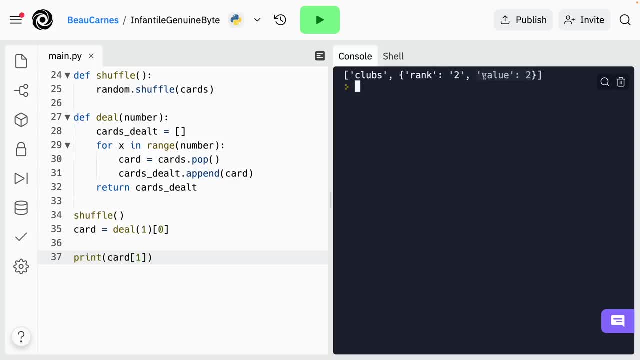 and we need to get this. So here we have this key value pair. So we need the value at that key. So to get the value of that key, we are going to put more brackets and I'm going to put value the key. 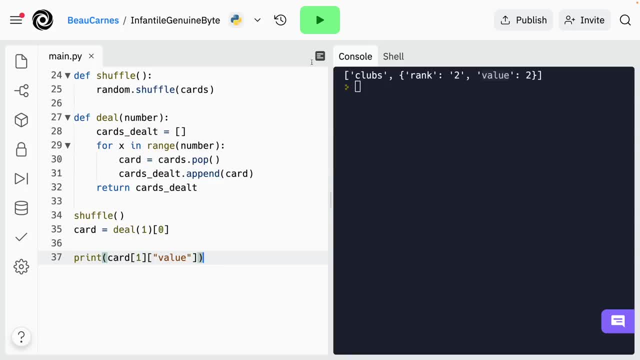 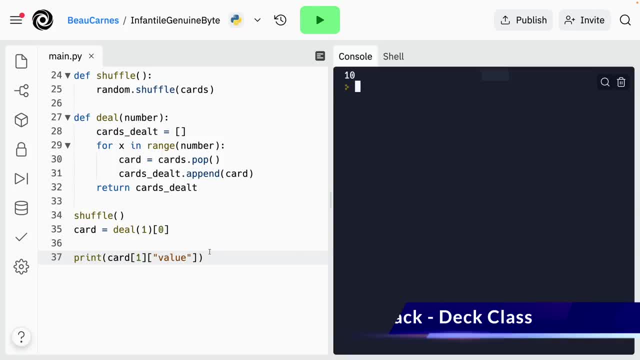 just give us the value of the card. Now we'll start defining classes that will be used in order to separate out different aspects of the game. So classes, you may remember, provide a way of bundling data and functionality together. creating a new class creates a new type of object. 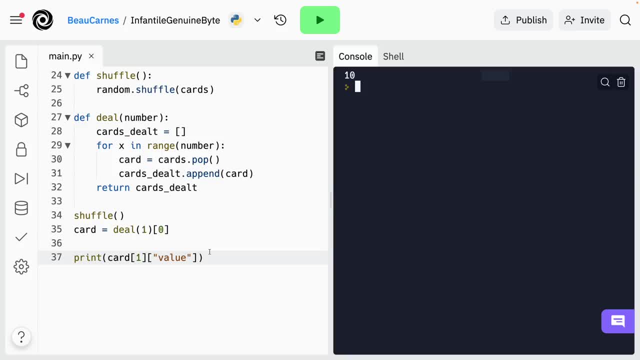 allowing new instances of that type to be made. An object can contain a number of functions, which we call methods, as well as data that is used by those functions, called attributes. So we're going to use classes to model three parts of the game: a card, a deck and a hand. So far, 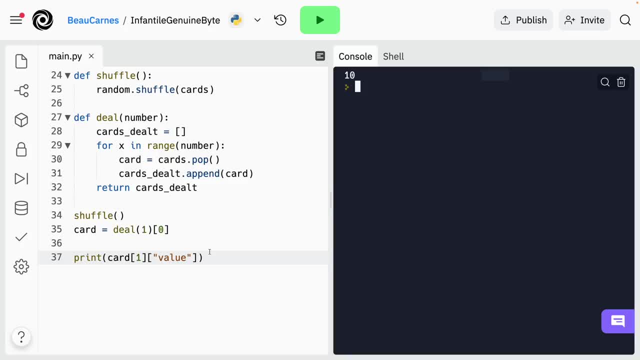 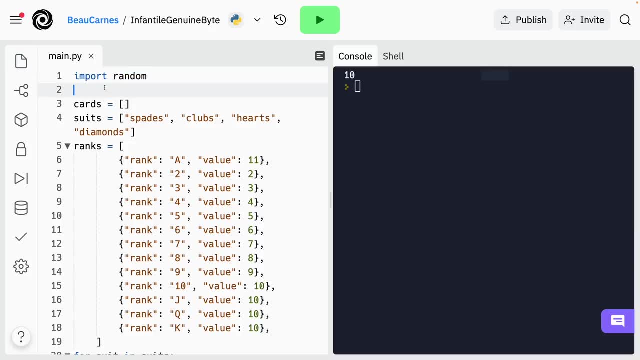 we've mainly worked on the elements of the deck class. So right after this import statement at the top, we're going to make a class, a class called deck, And we're going to put everything that we've written so far in that class. So we're going to put a class called deck and we're going 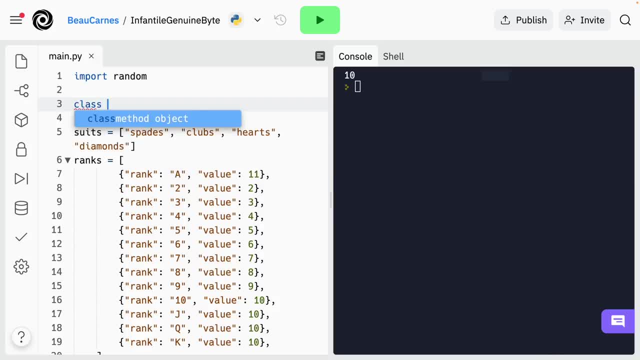 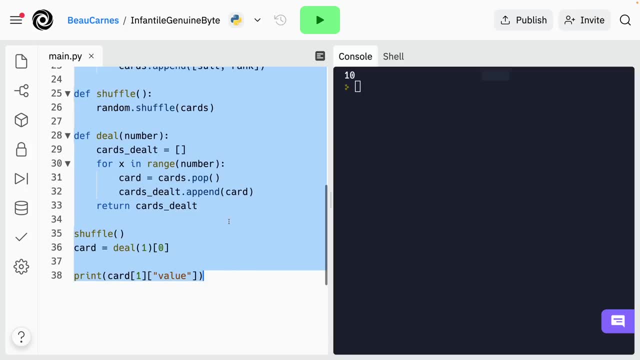 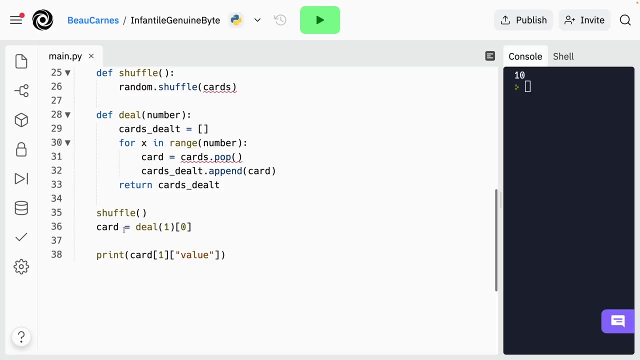 to put a class called class. So we're just gonna do class deck colon. Okay, now we just highlight everything here And then I'm going to press tab to put everything in the class of deck, because everything's indented a little bit, And then these last few lines of code we don't need, So I'll just 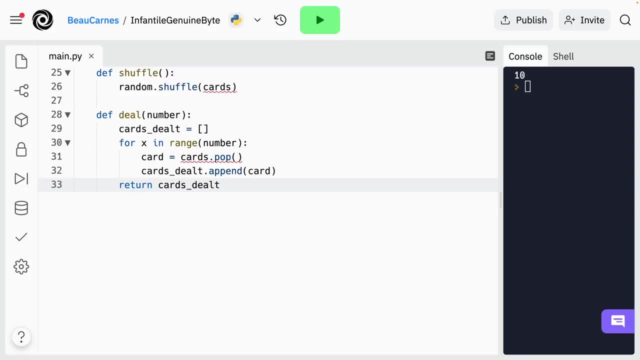 delete those. Those are just for testing out. A class is like a template. you can use that class to create an instance of the class called an object. Then you can use the instance. each instance keeps track of its own state So you can update. 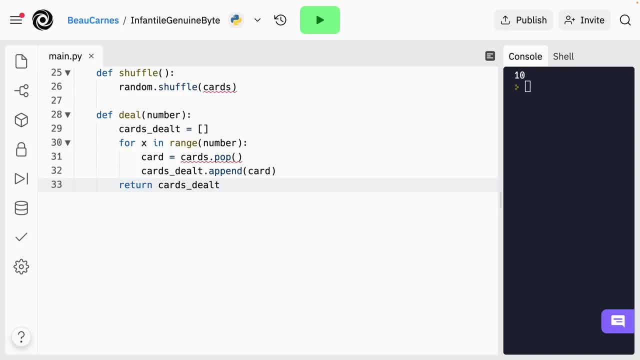 an instance created from a class and it won't impact other objects created from the same class. Soon you'll see an example of all this to make it easier to understand. But first let's prepare a class to create an instance from it. When you create an instance of a class, Python automatically. 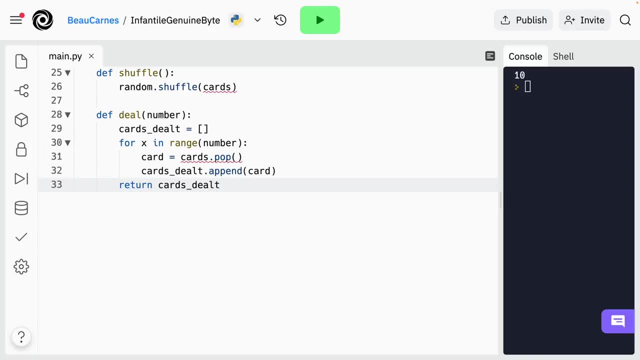 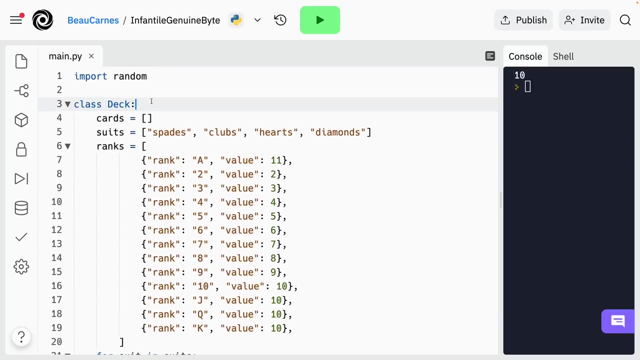 calls a function also called a method in the class, named init. We already discussed this earlier in the course. So the contents of this init method should be code that is run one time to initialize the instance. So at the beginning of our class let's create this init function. So we'll do def underscore. 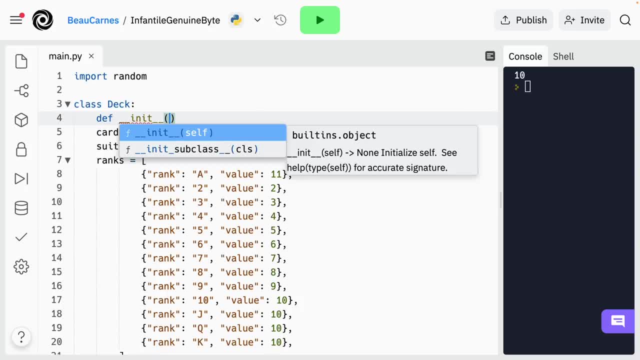 underscore, init, underscore, underscore. And if you remember from before, we always have to pass in self to all of these functions in a class, because then it gets. a self is referring to the instance of the class that we've developed. Now we're going to indent all the code. that's not. 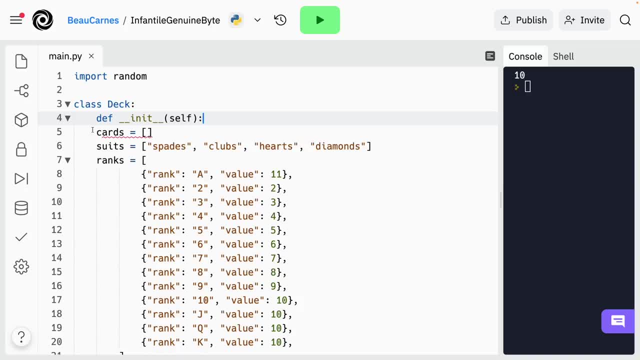 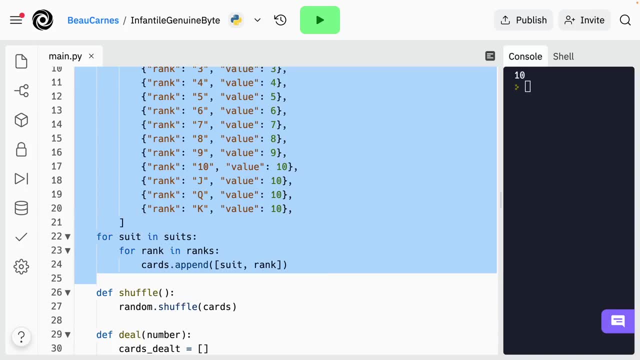 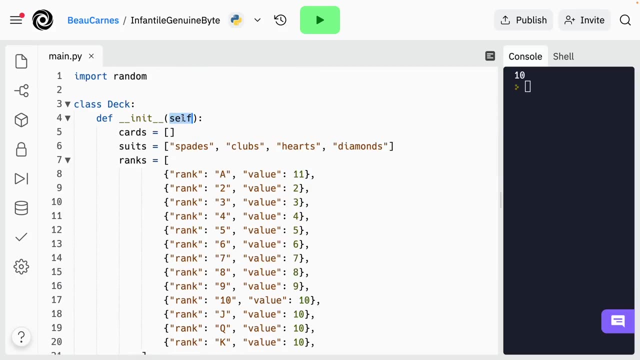 part of the shuffle or deal function, So the code will be part of this new function. So I'm just going to highlight all of this here, including the suits here, and then just press Tab. So, like I said, we just added self in here, you should always all the methods in a class or all the 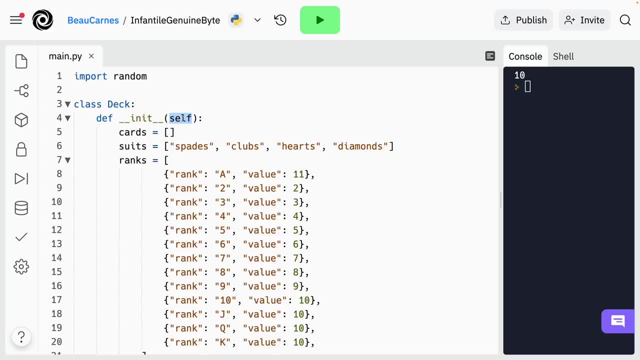 functions should have self, anything inside the parentheses, remember it's called an argument. there are variables here. there are variables here. there are variables here. there are variables past them, from the color to the functions. As I said, all functions in a class should receive. 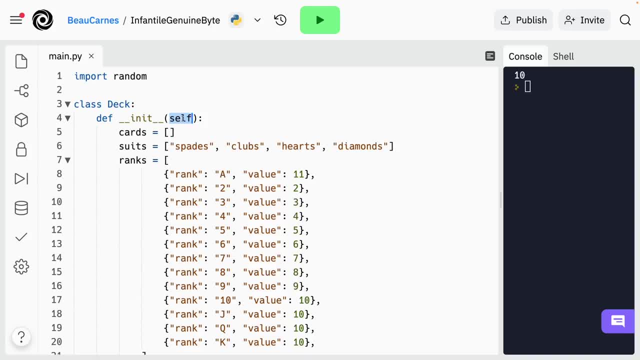 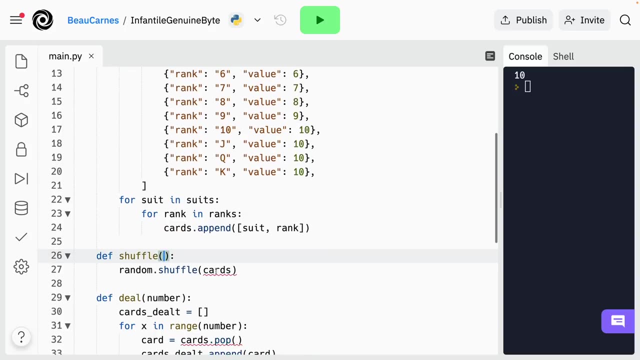 self as an argument And self represents the instance of the class. By using the self keyword, the function can access the attributes and methods of the class. So let's make sure to add self as the first item in the parentheses of the other functions. So we are going to add self here And 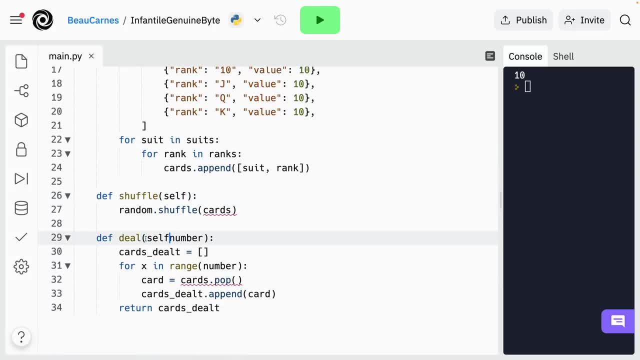 then see how we already have number here, but we're going to add self at the beginning, And then we're going to add self here And then see how we already have number here, but we're gonna add self at the beginning And we, so we can still call this function with just a single number. 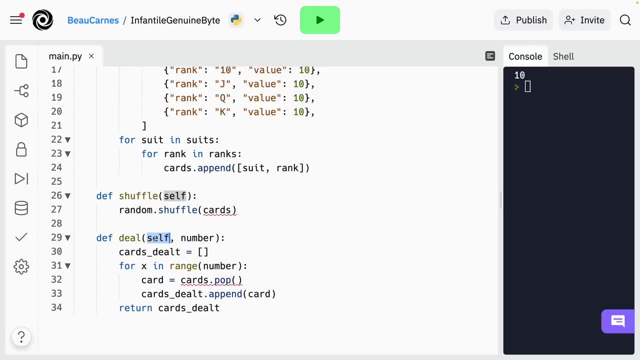 but it's going to also get a reference to the instance here. Now I want you to notice that the cards here is underlined in red. So before it wasn't- when we were before we made this into a class- we could just access this cards variable, but now we cannot, So let's fix that Inside a 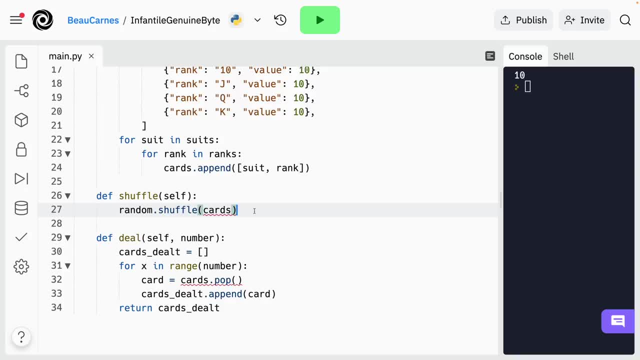 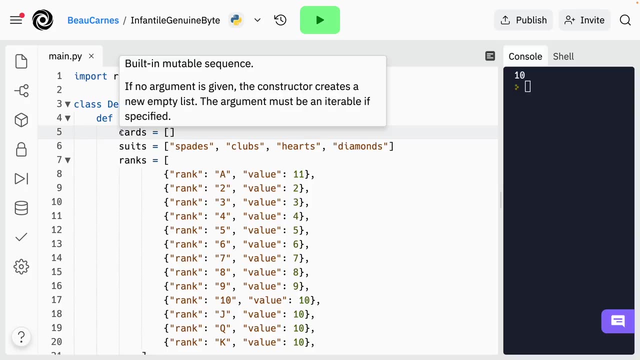 class. in order to access a variable in multiple functions, also called methods, the variable has to start with self dot. So we're going to change all instances of cards in every function to self dot cards, starting with this. So self dot cards Now. 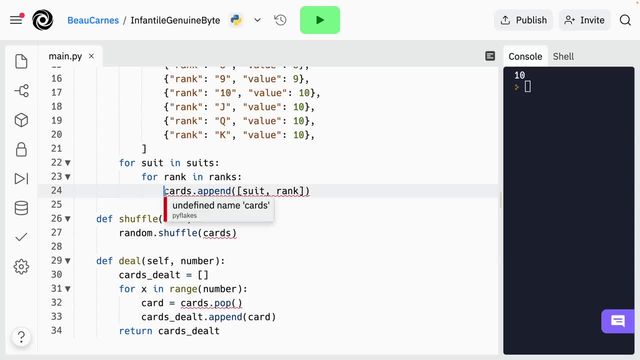 this is going to make it so we can access it in other places, And then we'll change this to self dot cards, And then this is self وت Cards, and then selfdigit dot dot Cards, And then self dot default without actors, dotletmil. This variable again has to start with And. 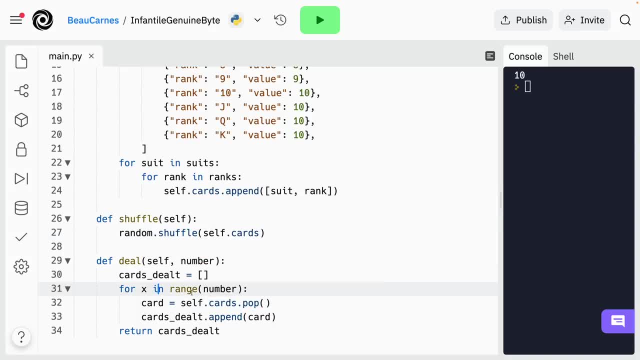 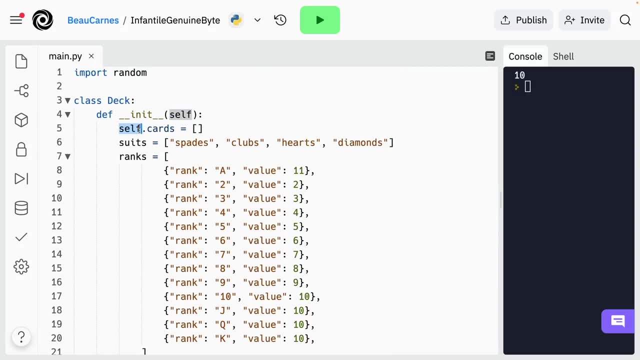 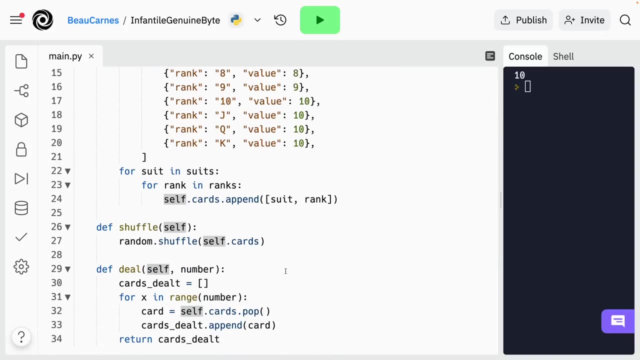 cards. So now this will be a variable that specifically associated with the instance of the deck that's created, And then we can access it in all of these other methods. Okay, we can now create an instance also called an object of the deck class. So at the very 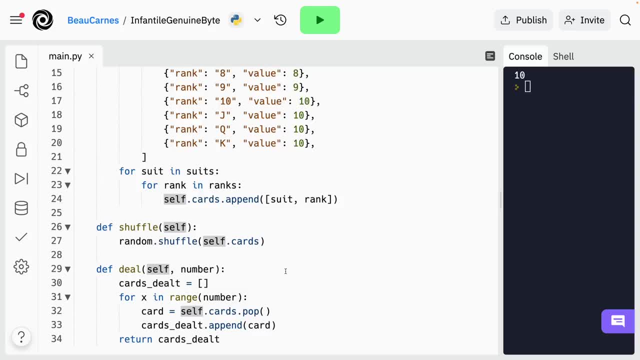 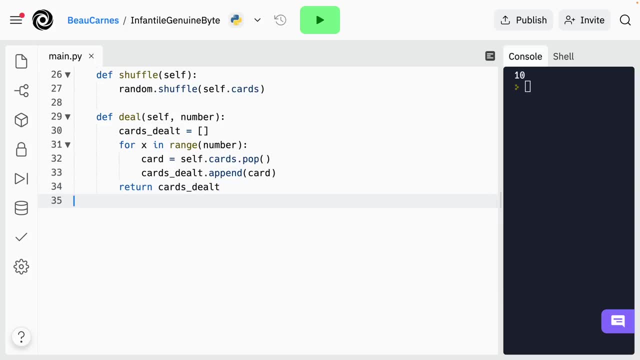 end of the code. let's create a variable called deck one and make it an instance of the deck class. So to make sure I'm not indented at all and I'll do, deck one equals deck. There we go Now. 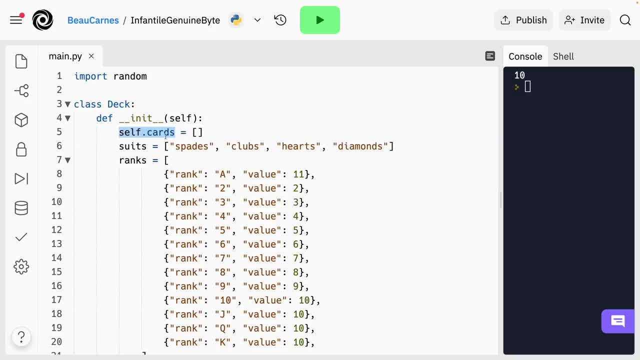 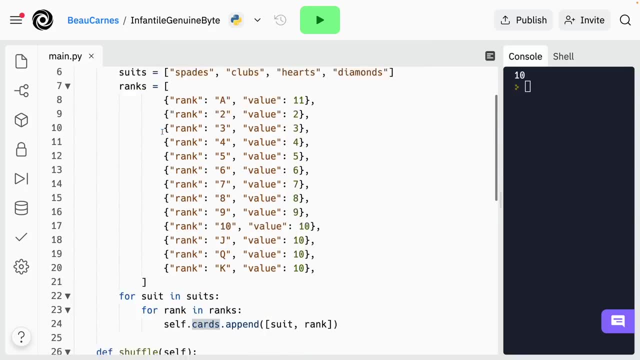 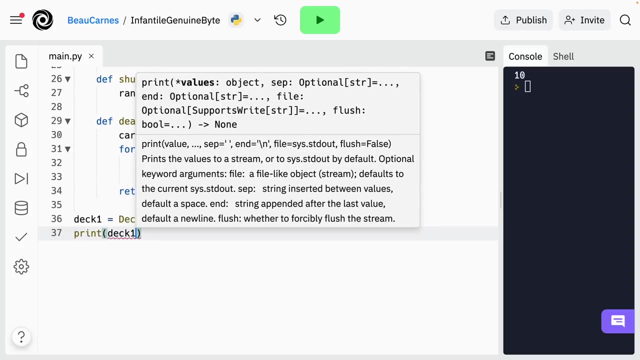 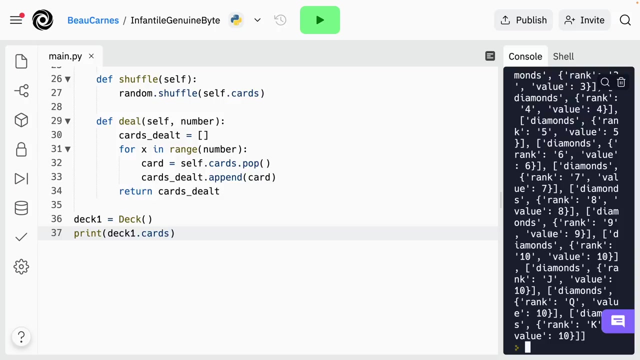 since we create a card with self dot cards, we can access that. we can access cards from the instance of the class. So let's just print out the cards from our deck one. So do print deck one dot cards And we can try that out. Now you can see the the list of all of these. 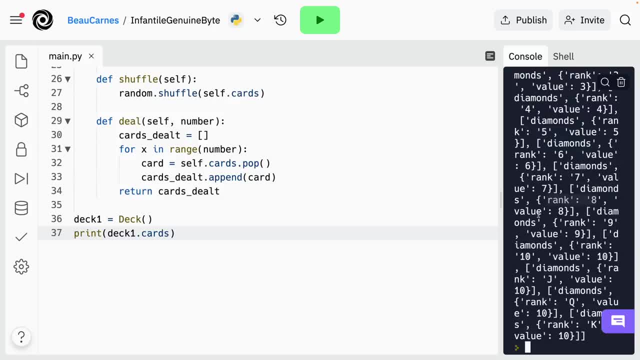 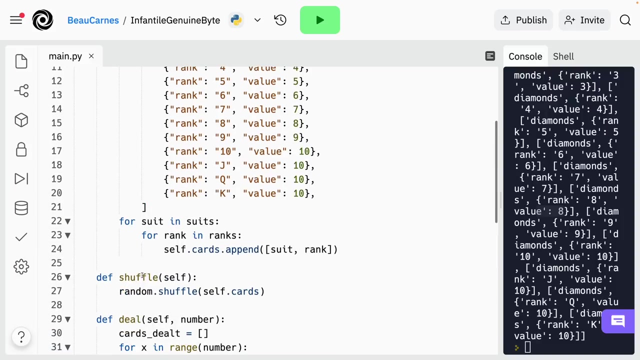 cards has the suit and the rank and the value for each card. So underneath where we created deck one, let's create deck two. we'll create another instance of another deck. So so now we can call methods on these instances. And you see some of the methods we have. we have shuffle. 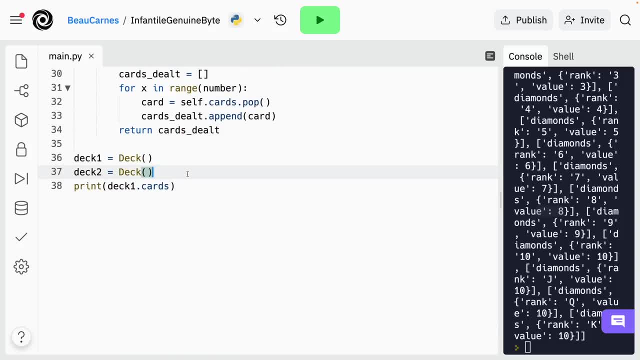 and deal. So on deck two: right after we create the deck two, let's shuffle the deck. So deck two dot shuffle. And then I have to make sure to put the parentheses at the end here. Right, we print deck one, let's print deck two or the cards of deck two. So I'm going to copy that And 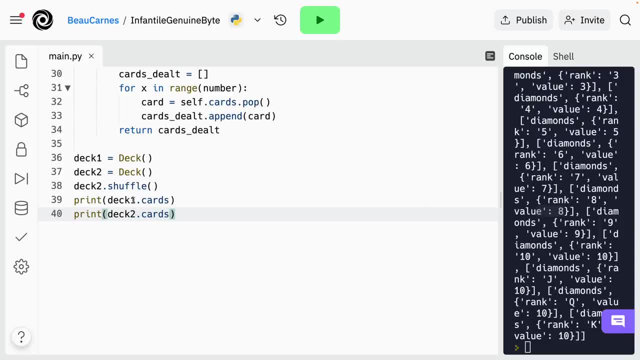 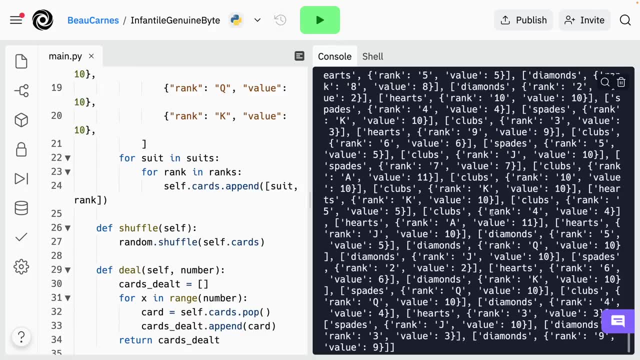 then we'll print deck two cards. So now we should see the deck two cards. So now we should see the deck one cards are not shuffled and the deck two cards are shuffled. So let me move this over here. I'm going to run the program And let's see if we can see that where deck one. So here's where. 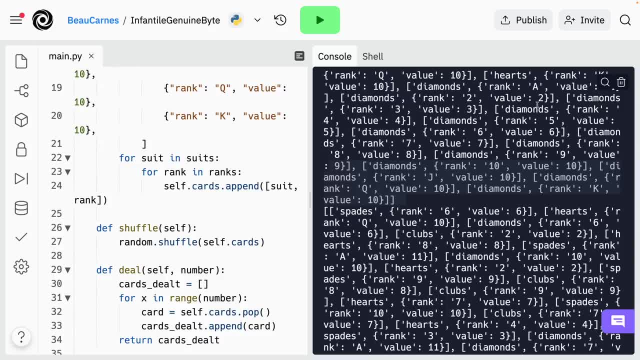 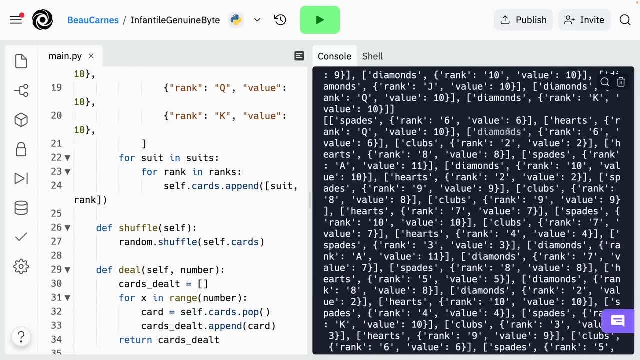 here's deck one And we can see how it's all: diamonds, diamonds, diamonds, diamonds, diamonds. all the diamonds are in a row because unshuffled. But then if we go into deck two we can see we have diamonds, clubs, spades, diamonds, hearts, So these are shuffled in deck two. they are shuffled. 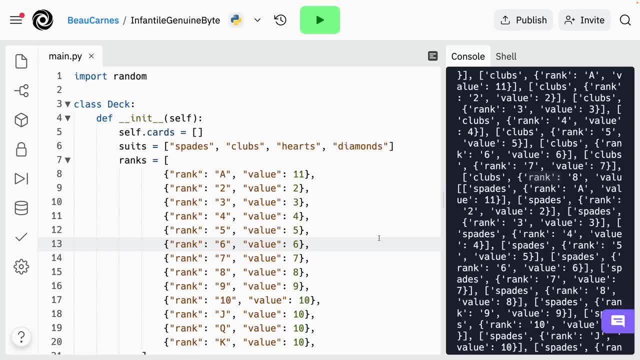 Okay, the deck works. Now let's add safeguards to prevent errors. Every time the deal function is called, a card is removed from the cards list. You can only remove a card if there are cards to remove. So before the program tries to pop a card off, self dot cards is to check if the length of 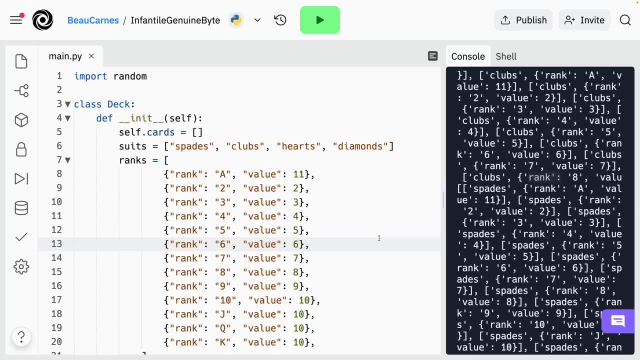 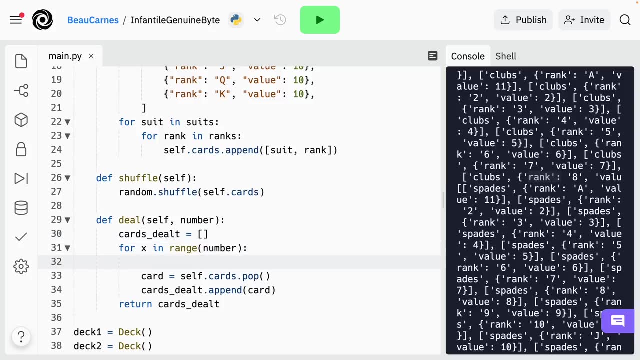 self dot cards is greater than zero. Remember, you can get the number of items in a list with length. So see if you can figure that out on your own. And then I'm about to show you how it's done. So when it's going to deal here, right, as we're dealing, we're going to add an if statement here. 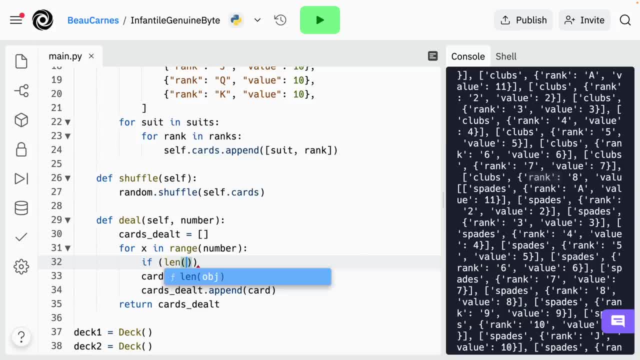 So if the length of self dot cards is greater than zero- and we do, we don't need this parentheses here. So if the length of self dot cards is greater than zero, then we'll do this. we'll pop up a card and add it to the cards dealt. If not, we just won't do anything. 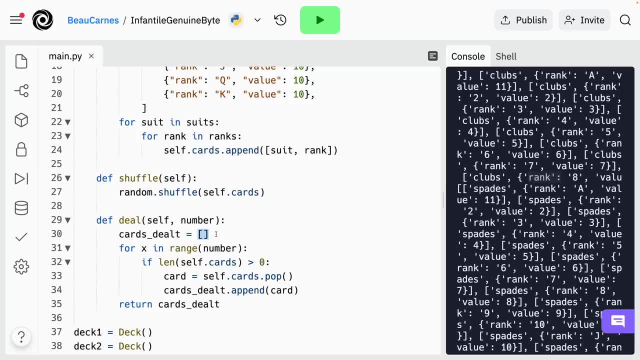 And then we'll return cards dealt, which could be an empty array if there were no cards on the deck. And now let's add something to the shuffle function. A deck with only one card does not need to be shuffled, So let's add the appropriate if statement to the shuffle function. 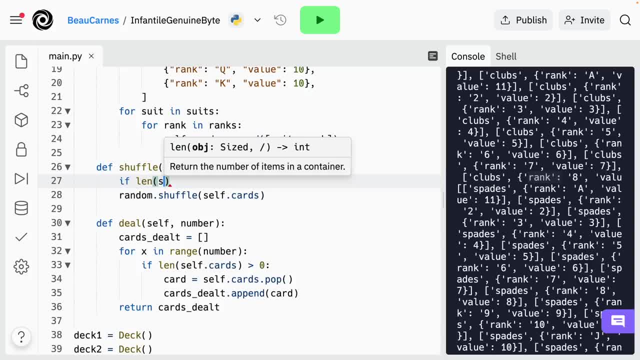 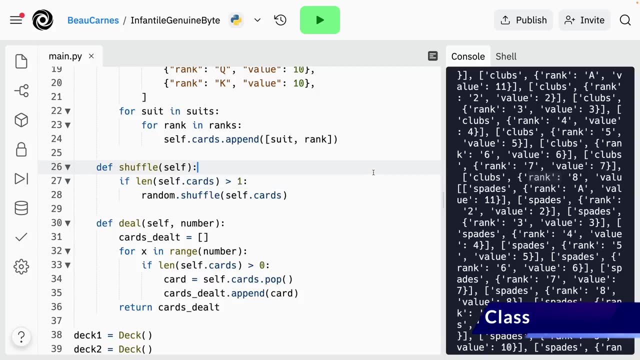 So do if the length of self dot cards is greater than zero and accordingly, if the length of self self dot cards is greater than one, then we will shuffle and then make sure. I'll make sure to put the colon there, Okay, Since a card is a separate concept than a deck. Next, 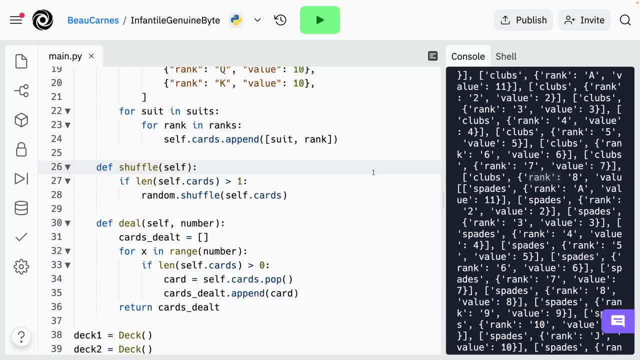 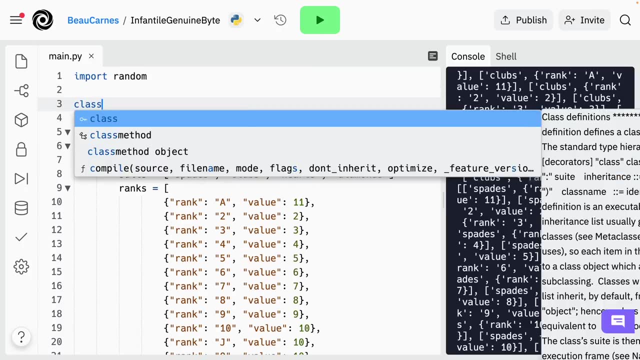 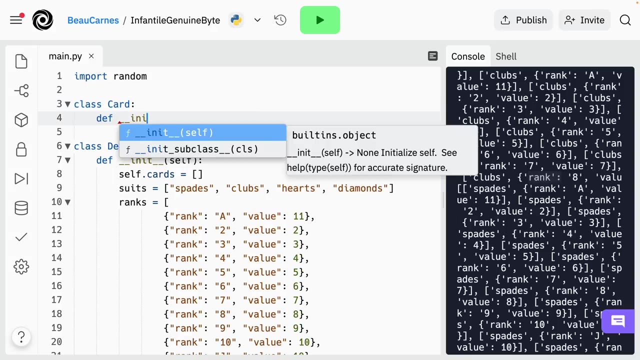 we'll make a card class. So let's create a card class with an init function And in that init function we'll set self dot suit to equals hearts. So hopefully you already tried this- I'm going to do class card And then I will do def net And then, after the suit will lose self dot. 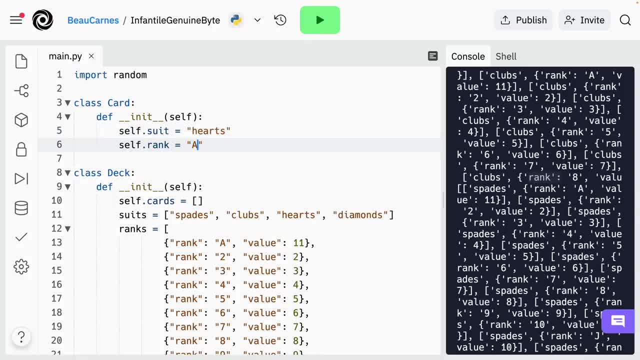 rank instead of a. So currently, anytime a card is created, it will be an ace of hearts. Let's refactor that For the code so the suit and rank are specified when a card object is constructed, So the init method can take additional parameters beside self that are passed into it as objects is. 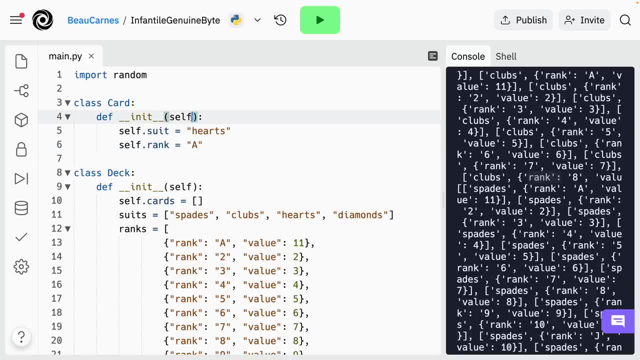 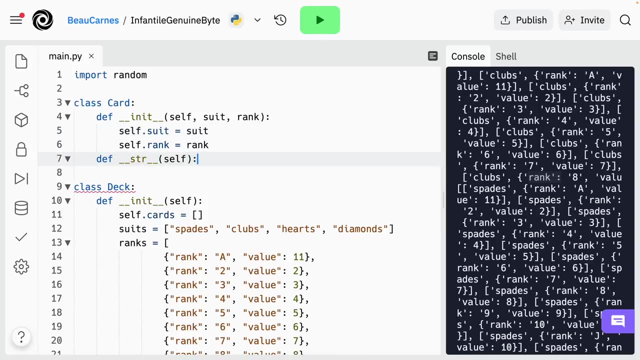 constructed, So update it to take suit and rank. Now we'll create a special method That's underscore, underscore, st r, underscore, underscore. When a class has this specific method, that's going to take its character ID and the object. Let's say that this is the image of my 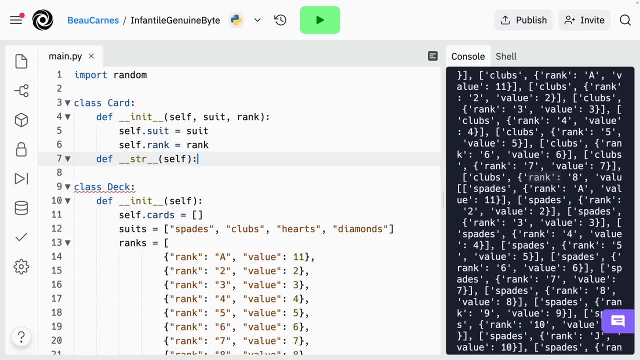 it's called when print is invoked on an object from the class. So we want to make it so. when we print an object from the card class, it will print something like 10 of hearts or three of clubs or something like that. So we don't do print here, we do return is going to return this. 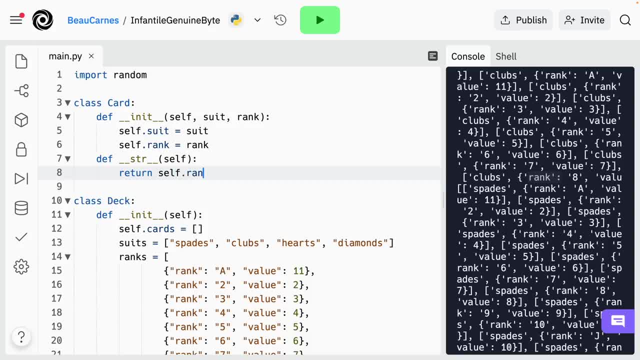 to the print statement to return self dot rank. And then we have to get the rank And we do plus and then of it to put a string there: plus self dot suit. So now it's going to return the rank, which is like two or a of, and then the suit which is one of these. So let's 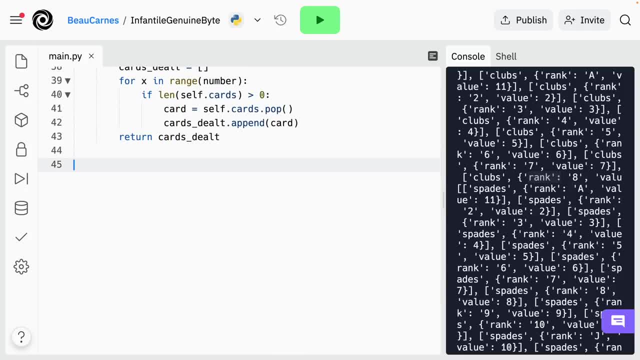 just try it out really quick And we go to the bottom. we don't need any of these two tasks because we're testing something completely different now. So to card one equals card. I'm gonna create a card I have to pass in right, right after first pass in the suit. 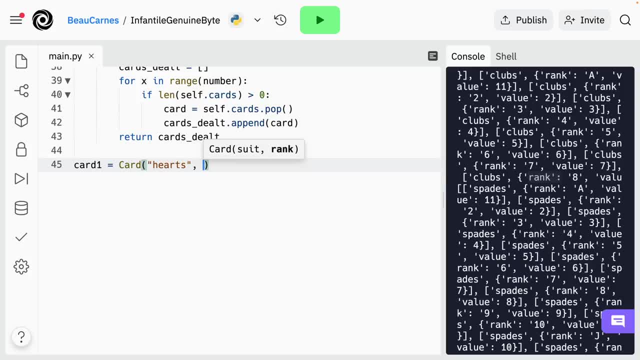 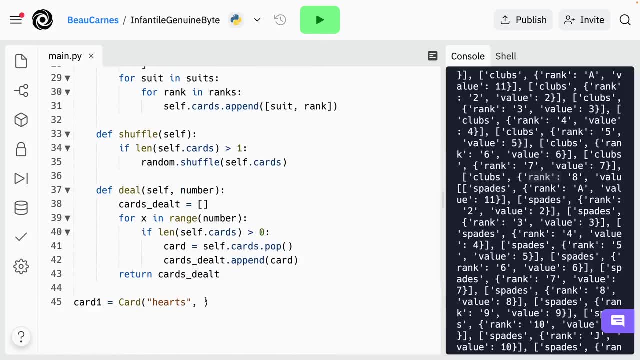 so how about hearts? and then I have to pass in the rank, but we want to make it look like these ranks, So I'm just gonna copy one of these here And then, after we create the card, it's going to be print Later. let's just paste that. However, once again, this will come impact. 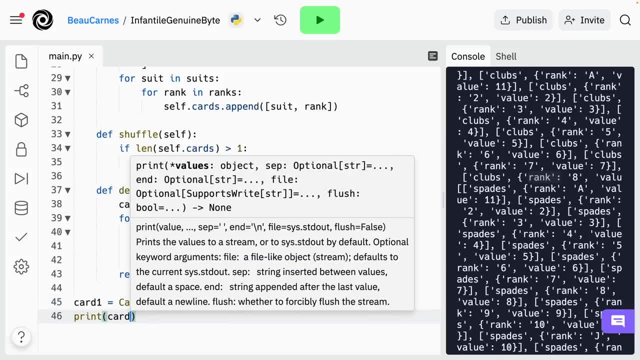 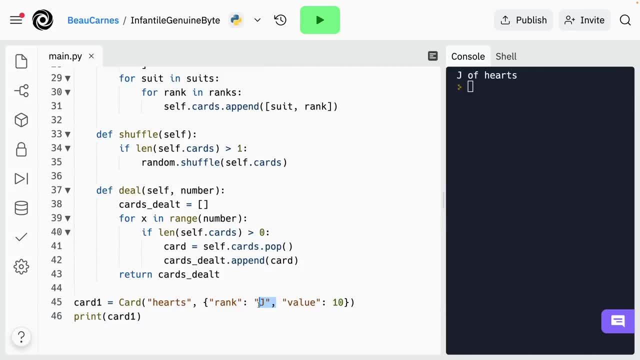 just like alles, fireworks are random, which is all, So in my case it's five plusik This card. I can just print card one. Let me clear this, and then I'll just run that J of hearts- I see it got the J of hearts- And feel free to add a few more cards like this and test. 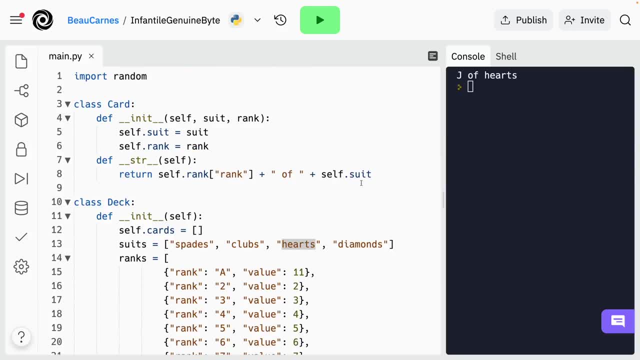 out a few more if you want. Okay, now we're going to refactor this slightly. You remember, way toward the beginning of this course we talked about f strings. So f strings allow us to put variables right within a string. Do you remember how to do that? Let's see. 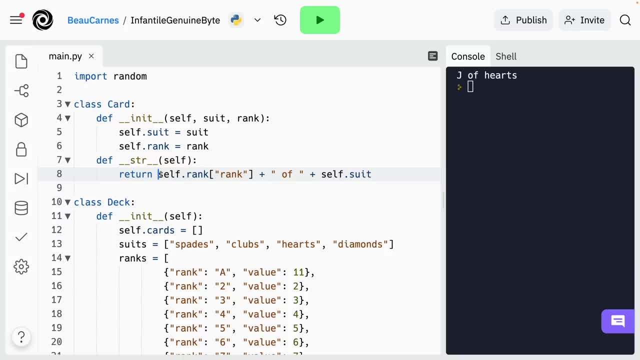 if you can update this to use an F string. So first we're going to create a new string, but we're gonna start with the letter F, And then inside this string we put curly braces around the Python code And we don't need these other strings here. So now we put another. 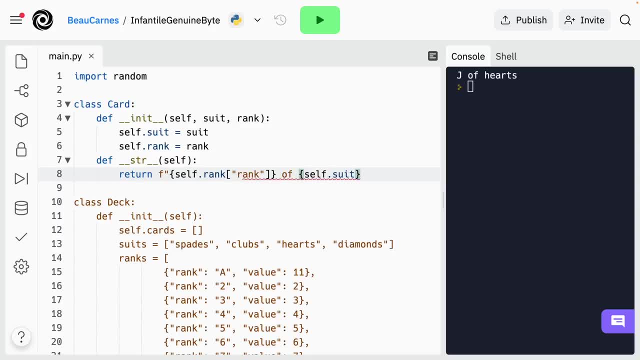 curly brace And then it binding string here. Okay, it's still showing these red squiggly lines, because if I have a double quote around the strings and anytime other quotes are in the middle, I have to put a different type of quote. So we're going to use single quotes. Okay, so now we can. 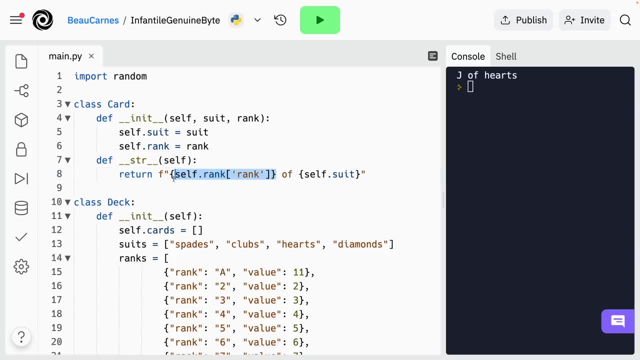 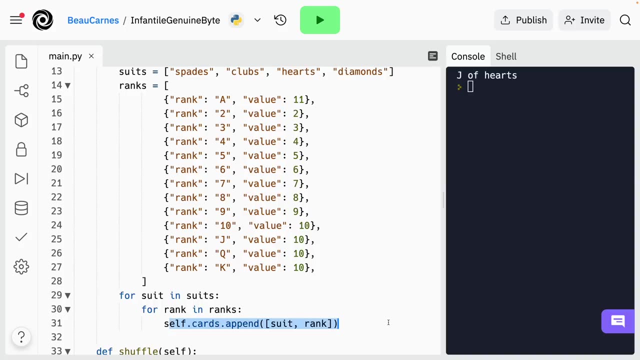 make this a whole string, but we use the brackets to put the variables right within the string. So now we've updated that to use an F string. So currently in the deck class we're going to use the last line of this. init method appends a list as an item to the cards list Instead. 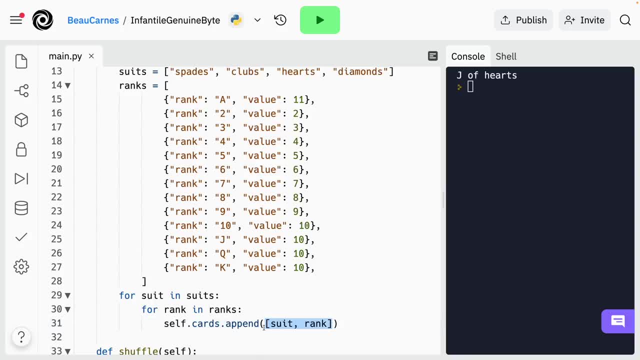 of appending suit comma rank. we'll create an append, an instance of the card class. Then afterwards when a deck is created it's filled with cards. So it's just like this: we're just going to delete that, I'll put card And then I'll pass in a suit and they rank. 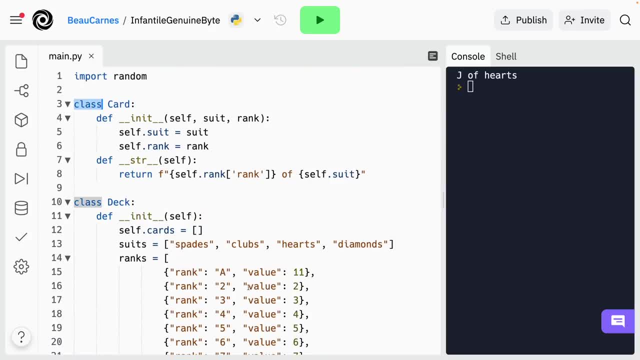 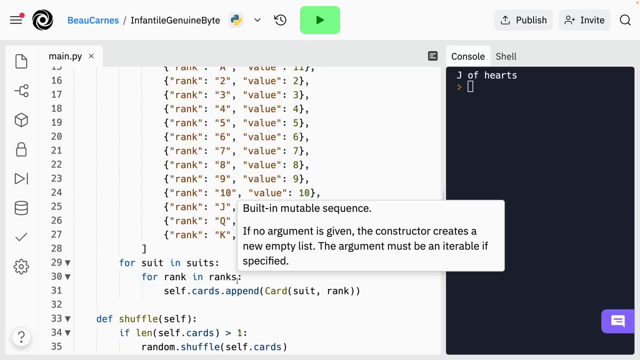 rank. So now we're passing in card instances. So we're done with the deck and card classes, And we created them in such a way that they could basically be used for any card game. Now let's make a hand class. This will represent a hand in the game of blackjack, So create 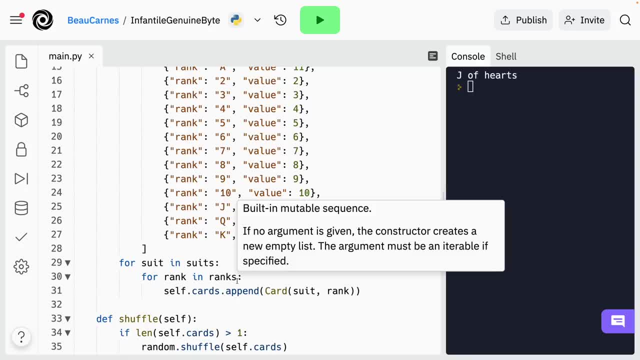 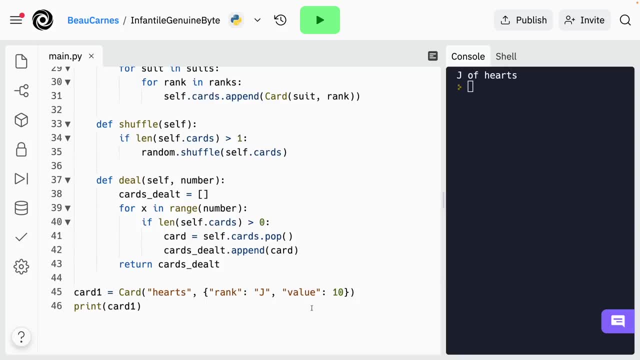 a hand class and add an init method and initialize a variable called self dot cards that is set to an empty list. So let's go down here And we can also get rid of all this test code here. So the new class is called a hand And we'll. 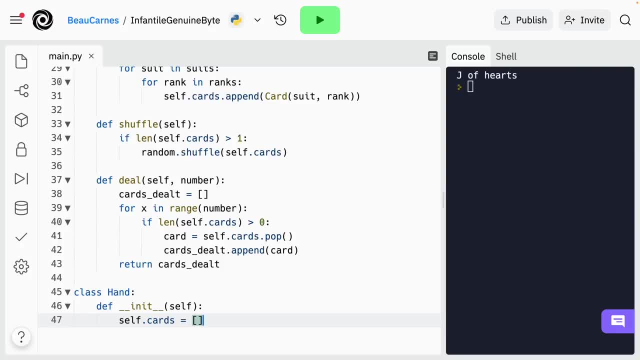 also make the hand keep track of the value of the hands, of self dot value. we'll start it at zero. In this blackjack game there will be a human control player and a program controlled dealer. So let's add a dealer parameter in the init constructor method of the hand. 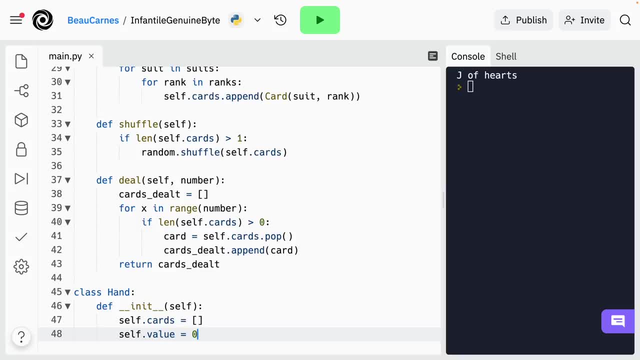 class And then when the hand class is created, dealer should be set to true or false. So to keep track of what type of hand it is, So I'll pass in the parameter dealer And then we just have to create a variable and called dealer and set it to dealer, So self. 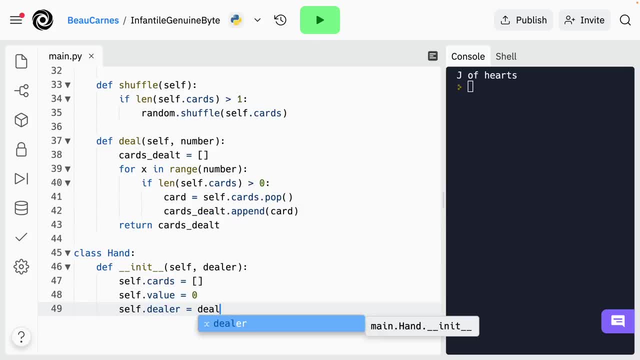 dot. dealer equals dealer. If you remember from before, function parameters can have default values. So we want to make it so that default value of dealer is false. So then if we create a hand and we don't set the dealer value, it will automatically be false. So that's. 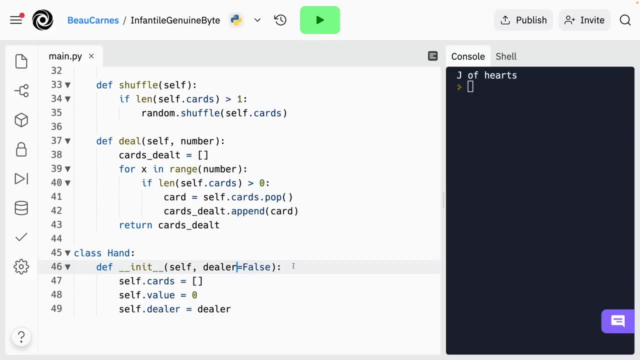 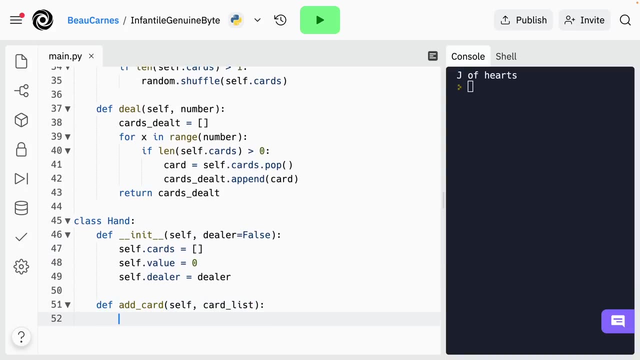 it false And I'm just going to take up these spaces here to make it smaller here. So now a hand can be created. Let's give us some functionality. we'll add an add card method, And the method should take a card list as a parameter, And then we need to add that. 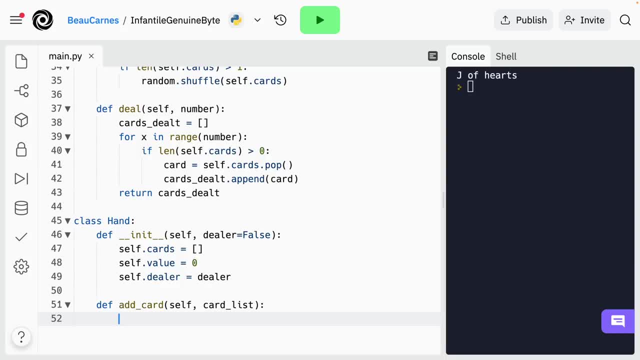 card list to the cards. So we can use the extend function, the extend method, to append each item in card lists on to the cards list. So it's just gonna look like this self: that cards dot append, no extend, I mean dot extend, And then we pass in card list. Now let's just 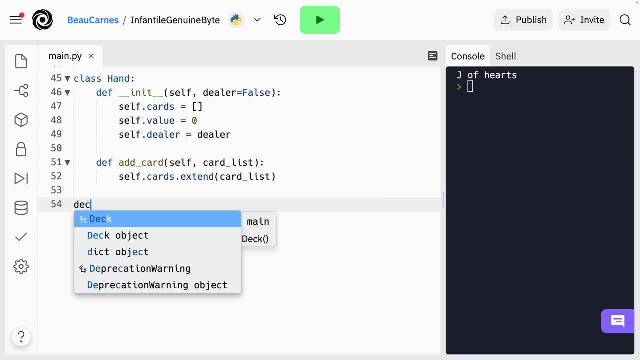 add some code to test that what we have so far. So let's create a deck And then we will shuffle the deck. deck dot shuffle. Now we'll create a hand. So Now we can add cards to the hand. So hand dot, add card And we will deck dot deal will deal two. 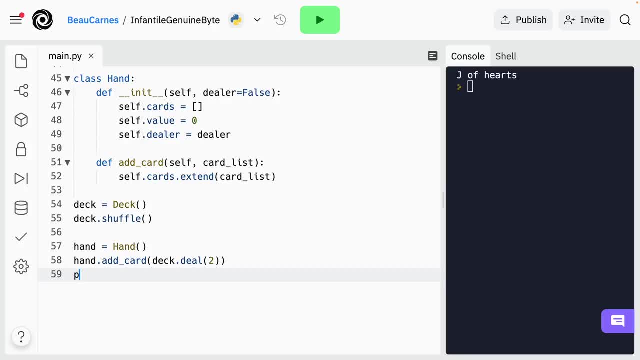 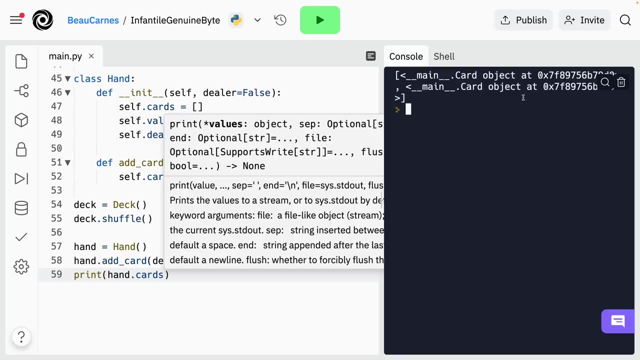 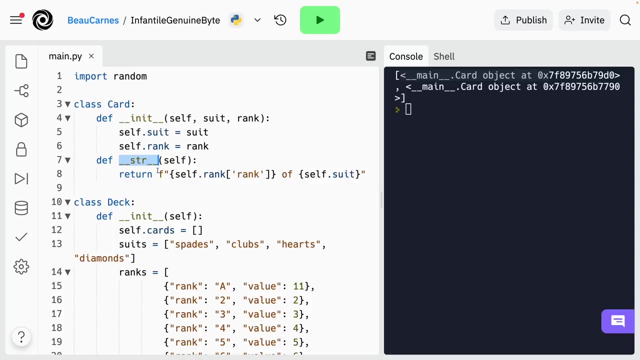 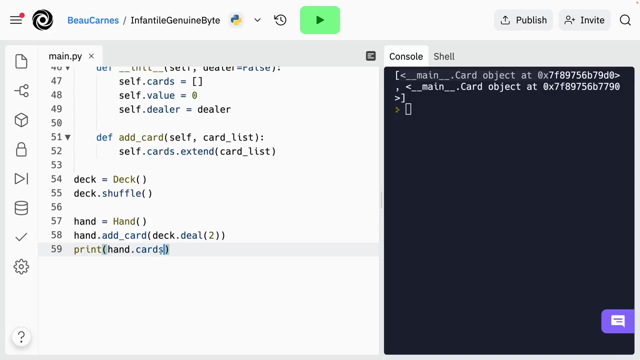 cards into the hand And then we'll just print hand dot cards. Okay, so this is how it printed out. I was expecting this to look a little different Because of this function- it print. it should print like that, But I think the reason is because this is a list, So it's printing a list. 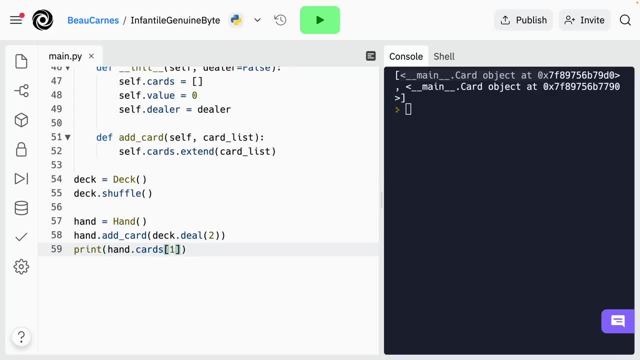 on an individual card. So let's change this to print an individual card. I'll print the first card, So put zero in there. I'll try it again. nine of diamonds, And then we can also print the next card. Three of hearts, And then we can also print the next card. three of hearts, And then 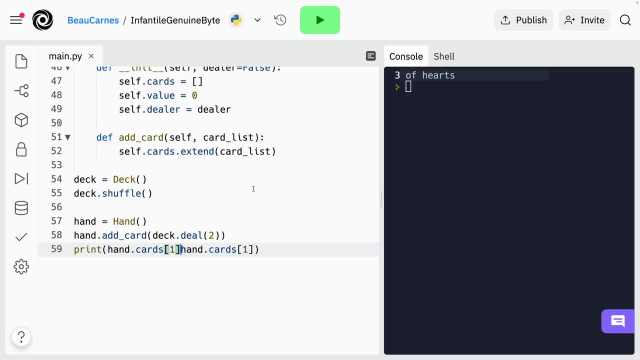 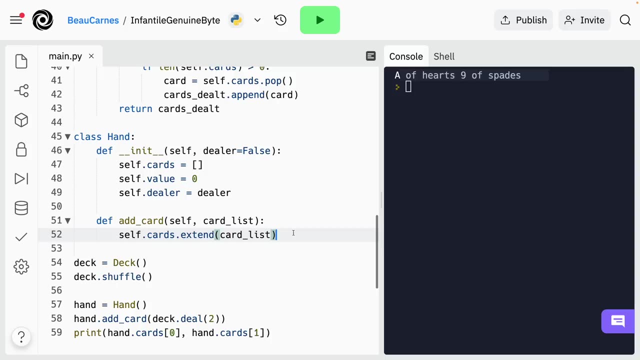 we can also print both cards if we just copy that and do hand that cards. zero, hand that cards: one, Okay, eight- of hearts and nine of spades. So those are the two cards that were dealt to the hand. Now we'll go back to the hand class And we'll add the ability to calculate the value of a hand. So let's. 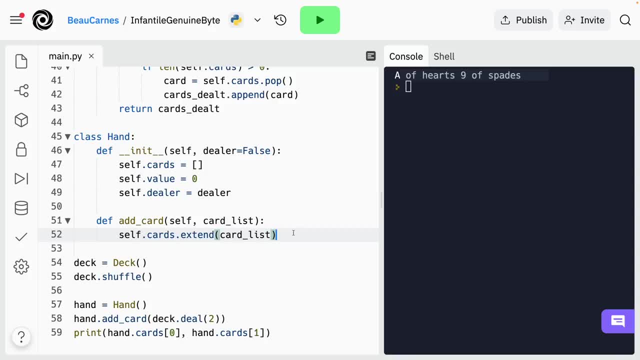 add a method called calculate value And inside the method we'll set self dot value to zero. Okay, now we'll take this one step at a time. First, let's let's make a for loop that's going to go through every single card, And inside the for loop we'll just set the value of the card to a. 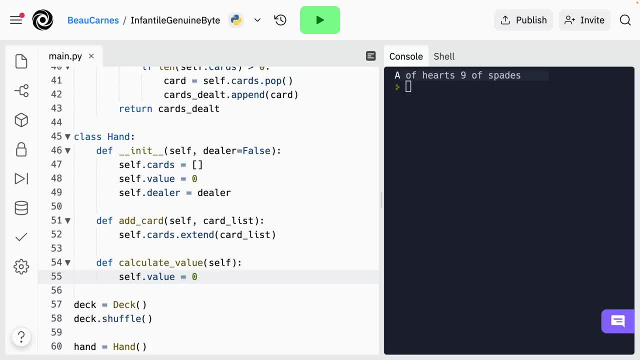 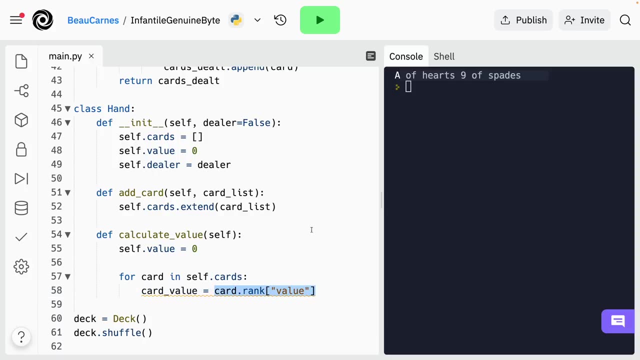 variable called card underscore value. So I'll do for card and self dot cards. Okay, so we're not doing anything with that yet, But we're going to in a second here Now we want to make sure that this is an integer, So let's convert that to an integer. If you remember, you just use int And 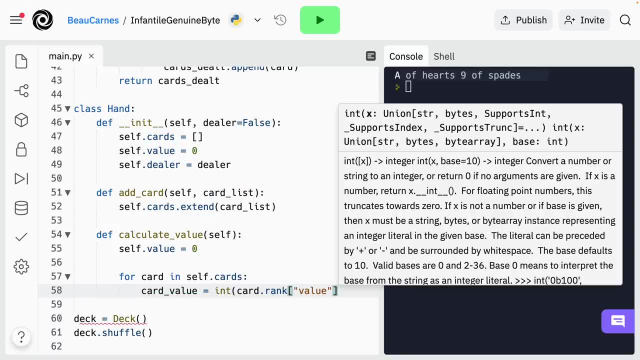 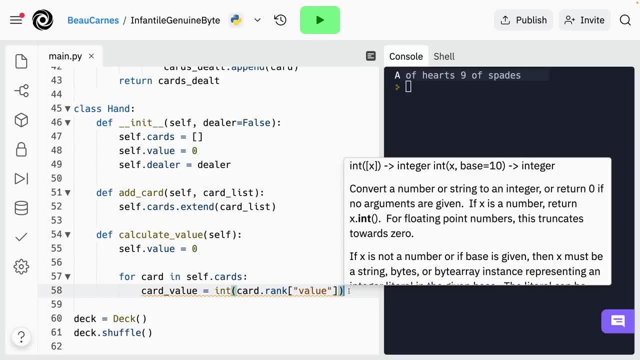 then put it in print int, And then inside the parentheses we put this value. Now, just getting the card value for each card is not enough. something must be done with the variable. So let's add that value to self dot value. So we'll do self dot value. So we'll do self dot value. So. 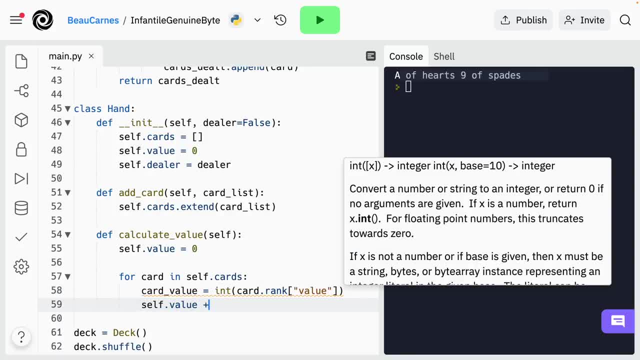 we'll do self dot value And then, if you remember from before, we can use the plus equals to add that to the current value. they'll still do card value. So, as you may know, in blackjack an ace can have the value of either 11 or one, depending on what is better for the player. So there's a few. 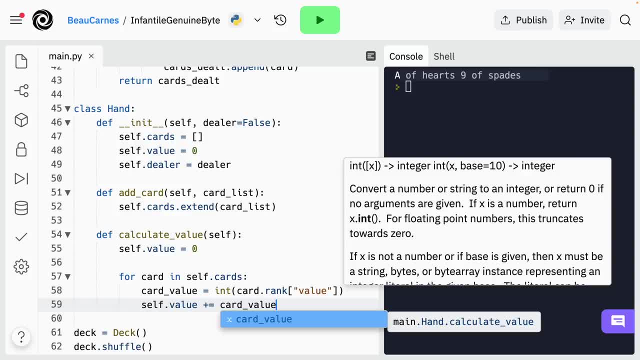 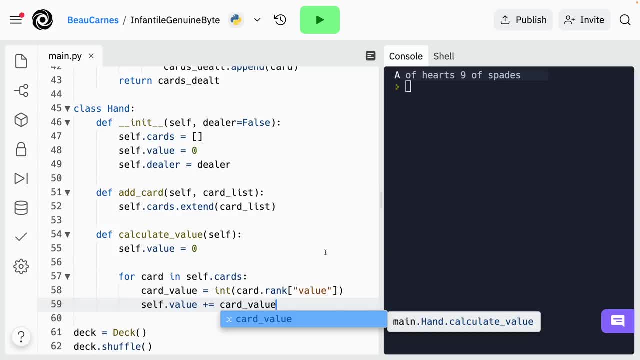 ways to implement that in code. So we're going to do one way. that's relatively simple. First we'll check if the hand has an ace. So let's first create a variable that will store whether the hand has an ace. will just be called: hand has underscore ace. 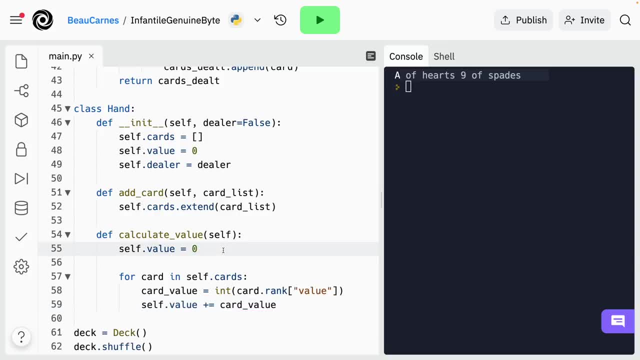 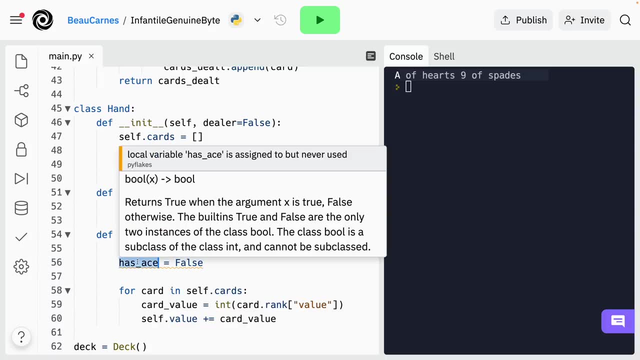 we'll set to false And we'll put it right under here. So do has ace and we'll set to false. And since we're only going to be using has ace within this method, we don't need to use self dot has ace. 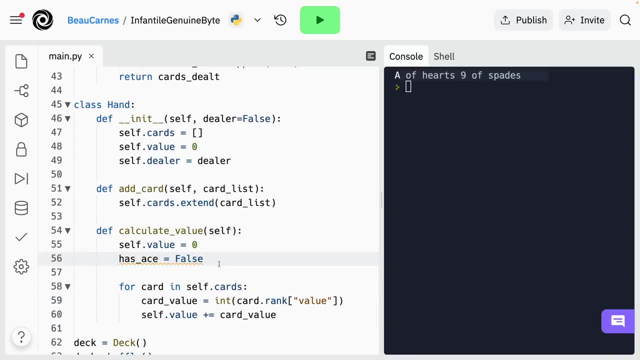 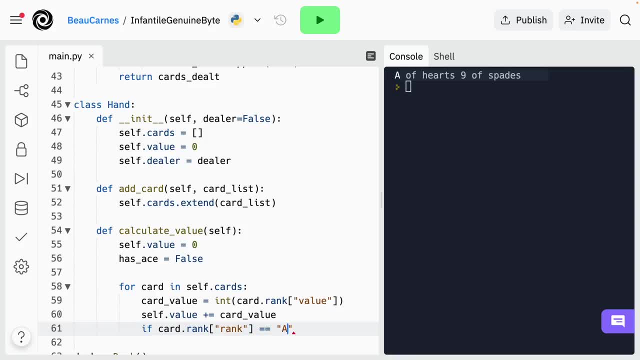 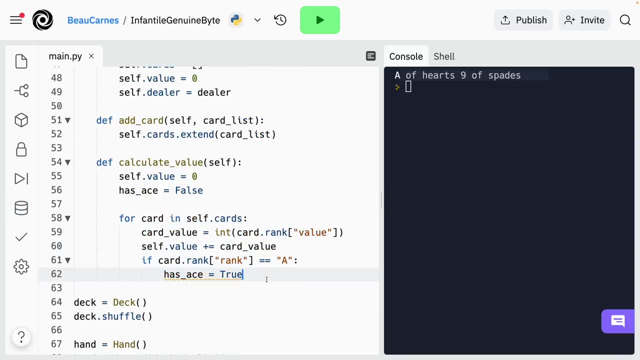 is going to be equal, double equal sign if it equals ace. After this entire for loop, we're going to check if the card has an ace And if the value is over 21.. If so, then we'll just subtract 10 from. 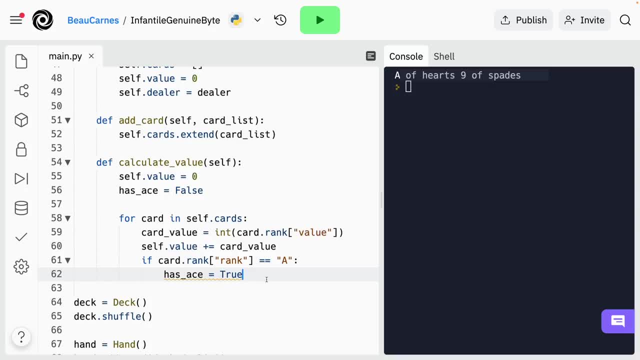 the value, because that will be the same as setting the ace to equal one instead of 11.. So we'll just do if has ace and self dot value is greater than 21.. The self dot value minus equals 10.. Okay, and look at. 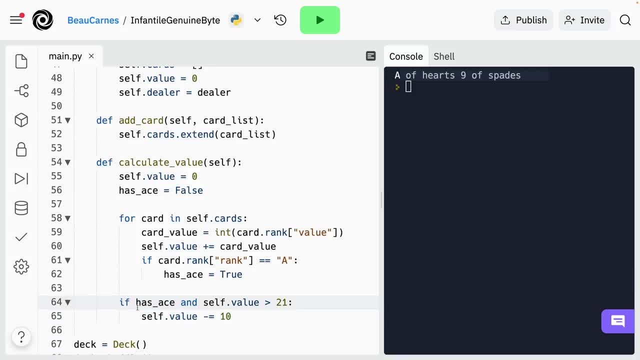 this. this is something I don't think I've discussed yet. You could say if has a equals true and self dot value is greater than 21.. But you can also- it's like a shorthand- you don't have to say if has a equals true, if has a, because has a is just going to equal true or false. 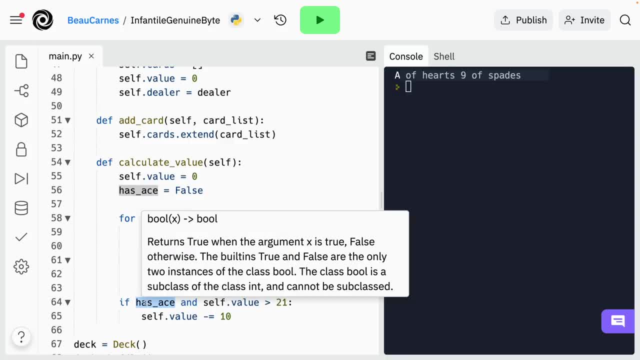 you can just say if has ace. So that's just the same as saying if true or if false. And so we're seeing, if both of these evaluate the true, then we will subtract 10 from the value. Okay, now we'll just add another method to get the value of a hand. 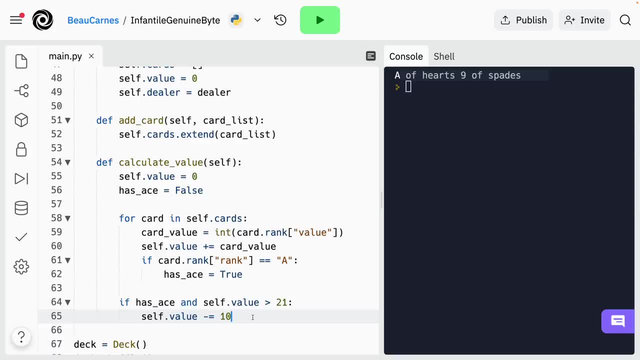 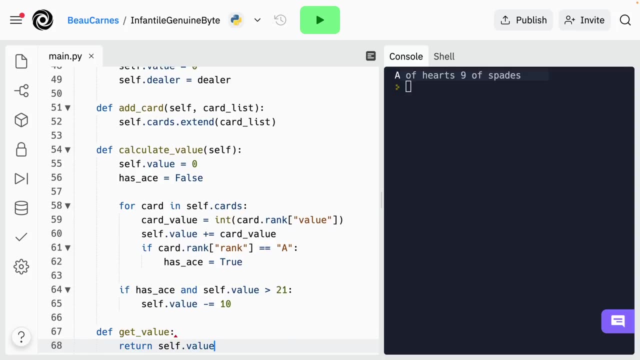 called get value and the function will just return self dot value. So we're going to make sure that we're not we're indented correctly and do def get value return self dot value. And then I have to make sure I put the parentheses here. 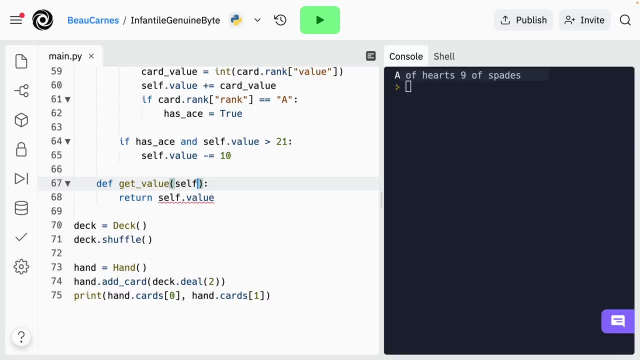 Okay, and then I remember to put self, since this is a self dot value we could call down here, like we could call hand value to get the value. But it's generally better to make a function to return the value, So I can do get value That way. there may be some extra code you want to. 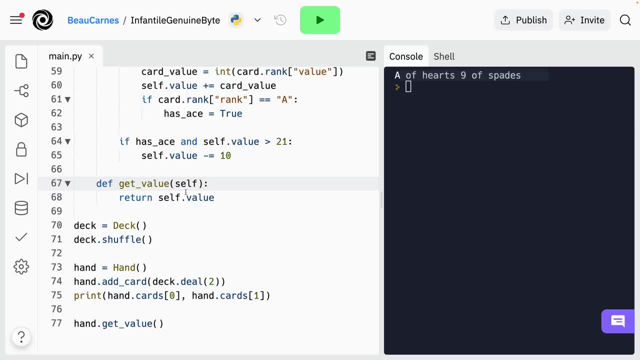 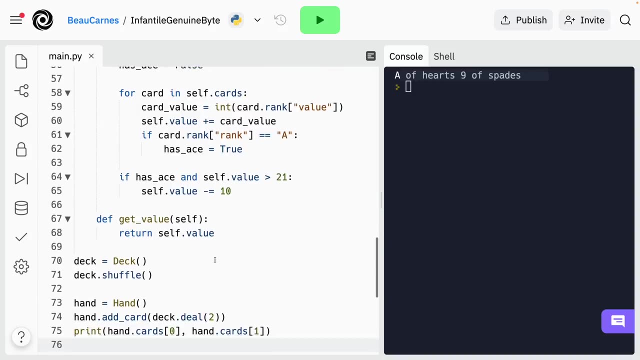 run in there like. depending on different conditions, you may want to modify the value before you return it, So it's best practice to create a method that will get a value like this for you. So currently, this value that's returned could be: 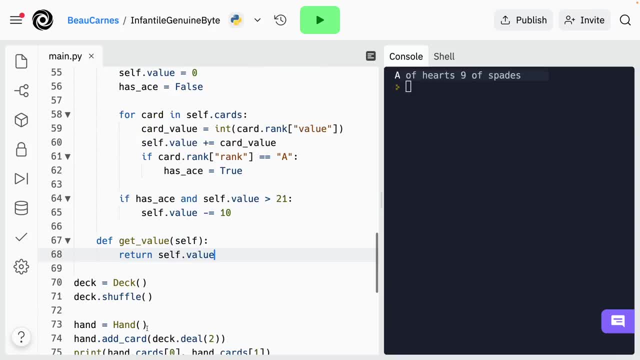 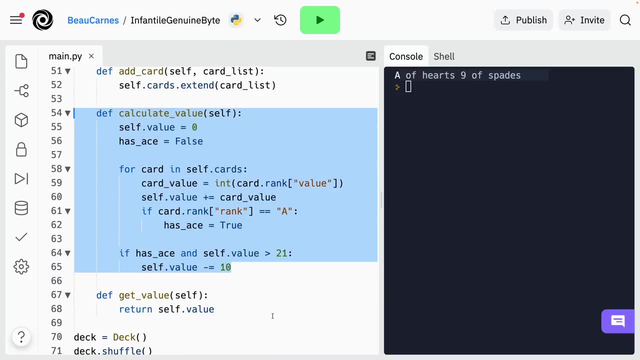 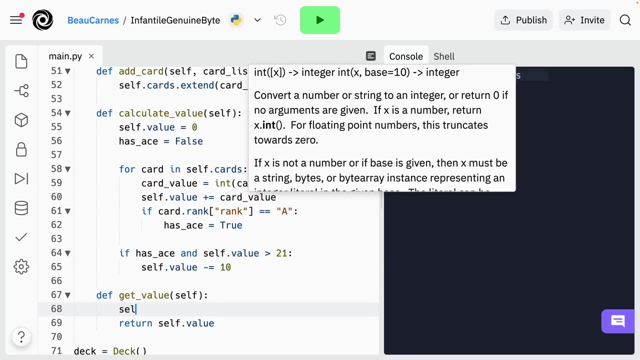 incorrect, Because if someone's going to get the value, the value has to be calculated correctly first, and like checking for aces and and other things. So let's call, let's calculate the value before we return the value. So I'm going to do self dot: calculate value. 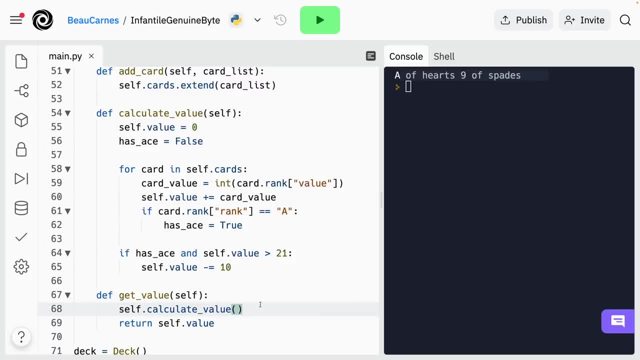 So this is something that I think is new- where to call calculate value from within this we're going to have to call self dot calculate value, And self will refer to the instance that we're working with. So we're calling the calculate value on the instance, That's. 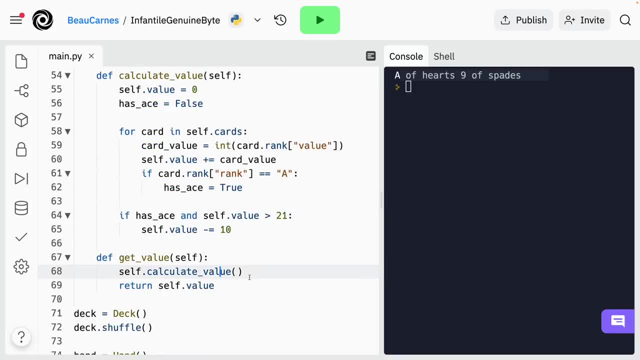 that is the hand instance, and we're getting the value and then we're returning the value. Okay, let's create another method, called is blackjack, And it will return true if there's a blackjack and false otherwise. So it's a blackjack if the value is 21.. So I'm going to do. 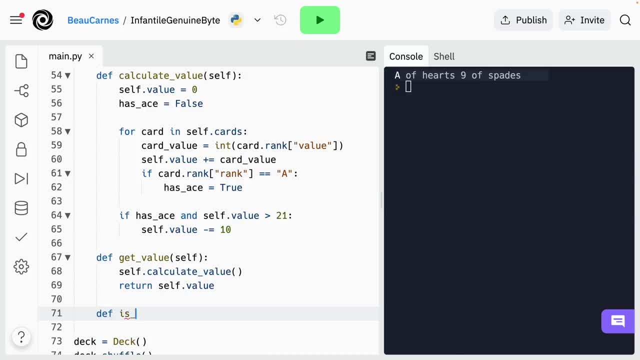 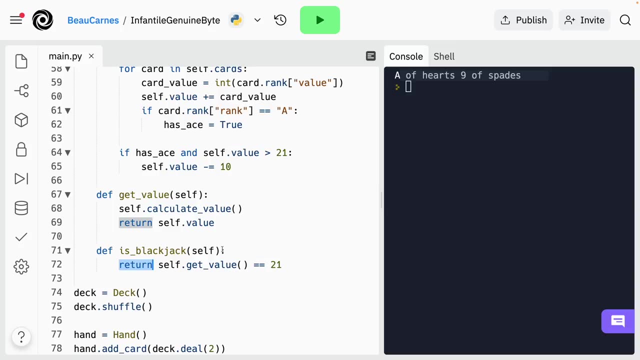 def: get or is. Oh, and put self here. Okay, so this is going to evaluate you to either true or false and return true or false depending on whether there's a blackjack. Now we'll create the final method in the hand class that will display information about the hand. So let's create. 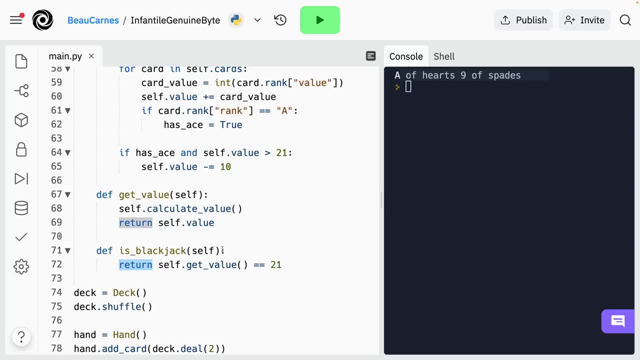 a method called calculate value, And we're going to create a method called calculate value And display, though, though, to start with, we'll just print your hand. Okay, now let's do a quick refactor: Instead of saying your hand, it should either say dealer's hand or your hand, depending. 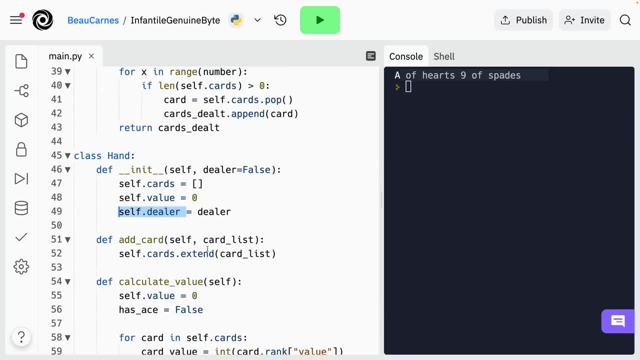 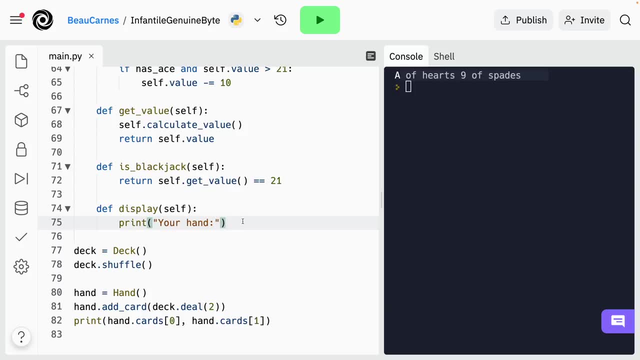 on whether self dot dealer is true or not. So we're going to use to do this all in one line. we're going to use a few things that we learned about earlier, including ternary operators, F strings and going between double quotes and single quotes. 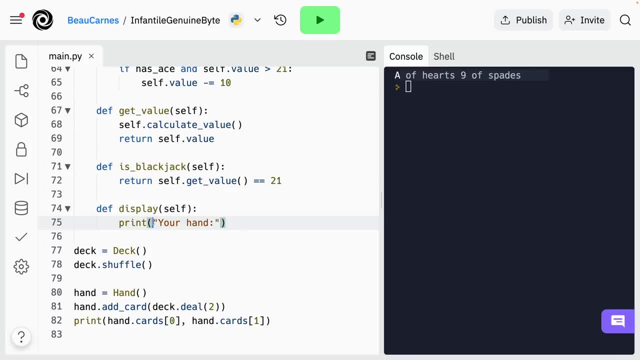 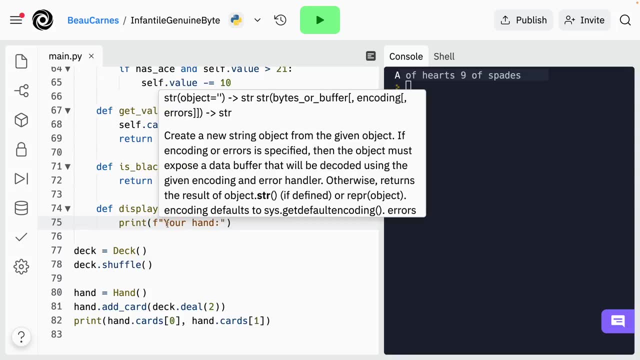 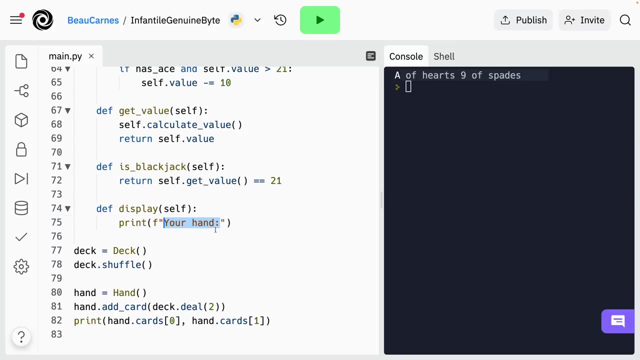 And then one other new thing: we are going to make this into an F string And then we are going to be using actually single quotes and double quotes within this F string. So if you want to use single quotes and double quotes within a string, then you're going to want to use double quotes And 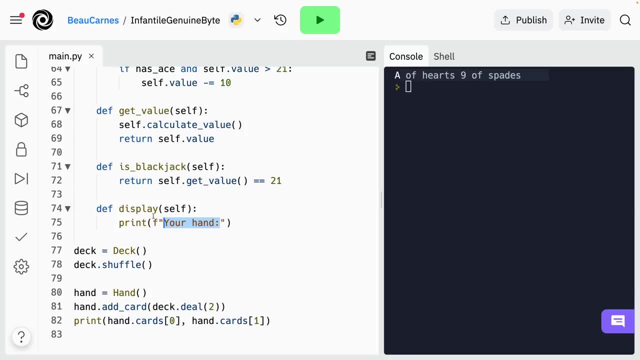 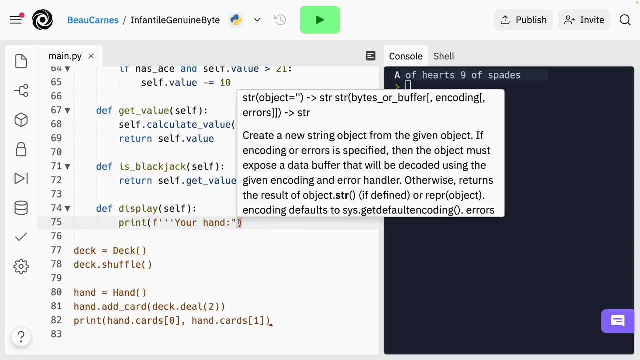 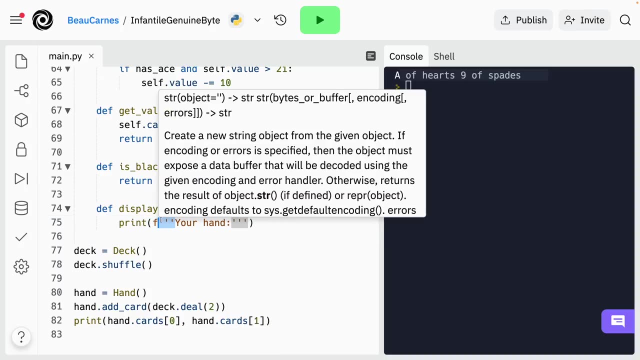 then you can surround it with a triple single quote. So I'm going to delete this quote, just do three single quotes. and then delete this quote and do three single quotes, And so we get the double quote. single quote and now this is a triple quote. So now we can use the double quote. 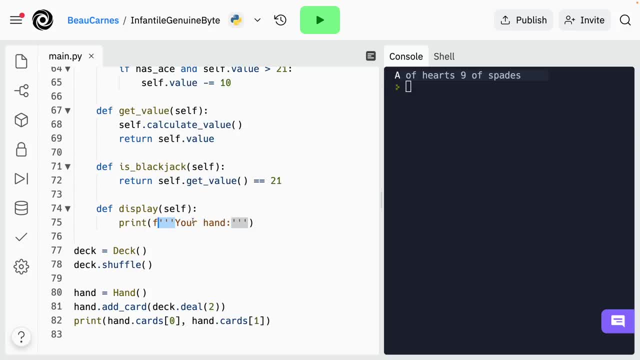 and single quotes within this string. So I'm going to- I'm just going to delete your right here And we are going to put a ternary operator to see if it's going to say dealers or yours, either dealers hand or your hand. So to do some code, I'm gonna have to put these curly braces here And then to 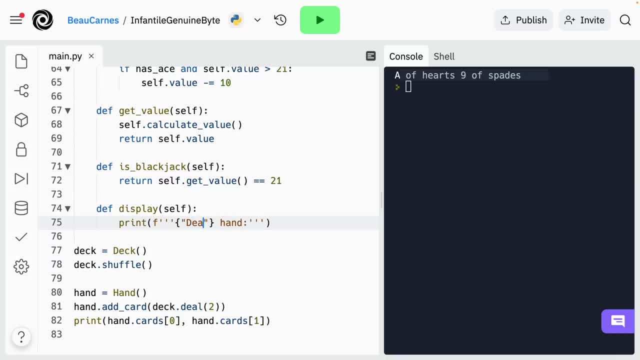 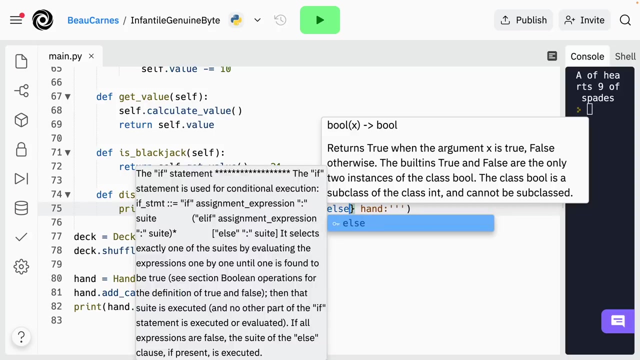 do this ternary operator. we're going to put dealer And now here. so here's the double quote and here's the single quote. So, dealers, it will return dealers if self dot dealer. so basically, if self dot dealer equals true. So return dealers if self dot dealer, else will. 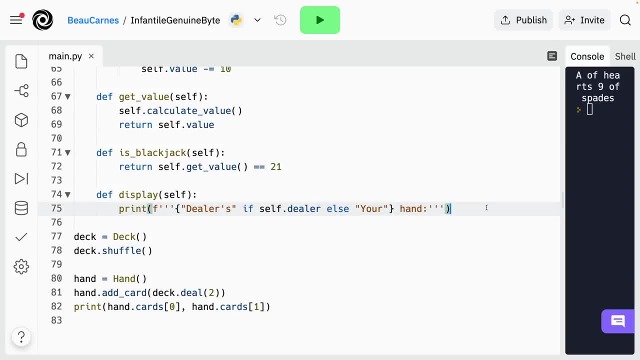 return your. Okay, that's the line. So it's going to be a dealer's hand or your hand, And next we will add a for loop that will print out each of the cards. So for card and self dot cards print. 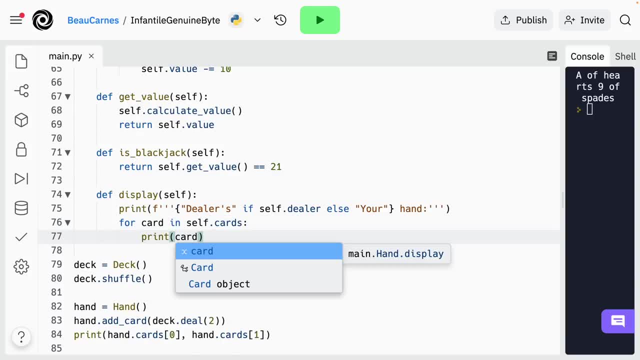 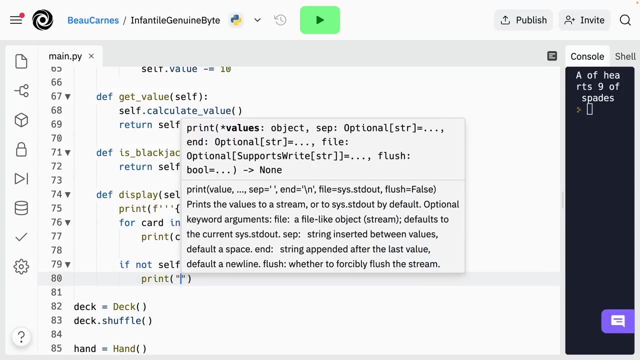 card. And then, finally, if the player is not the dealer, it should print value and then a colon and then print the value of the cards. So do this, we can actually use the not operator. So if not self dot dealer, then we will print, and we'll print value, value, And then I can just put: 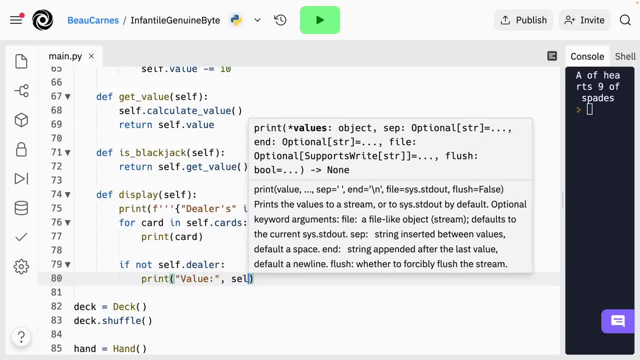 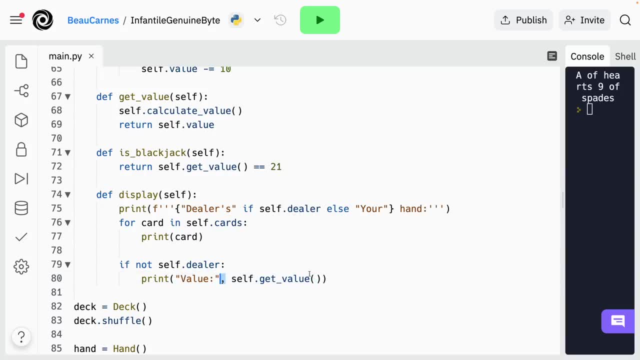 a comma to print two different items. So the string and we'll print self dot get value And it's gonna. when you put a comma and two different things, it's gonna put a space in between And then finally, we'll just add an empty, a print statement that will print a blank line. Okay. 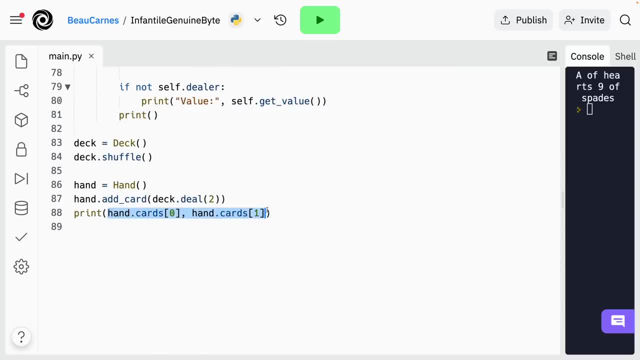 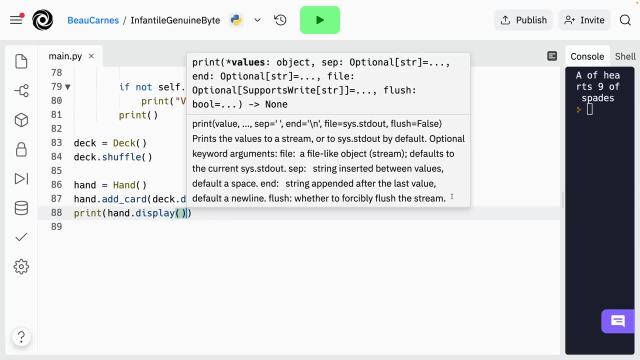 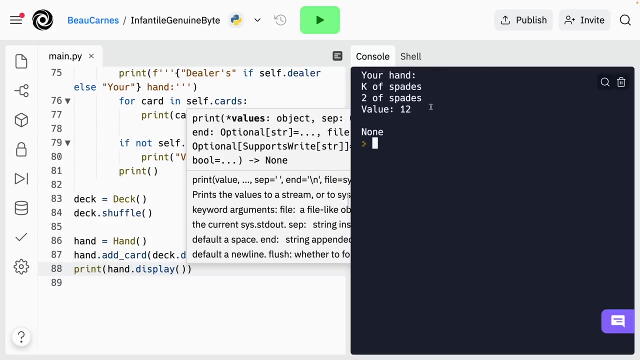 let's test this out by, instead of printing this, we are going to print hand dot display. See if this all works How we thought it was going to work. So your hand k of spades, two of spades, value is 12.. So 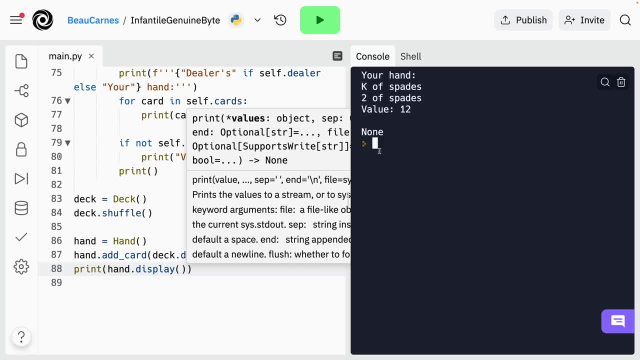 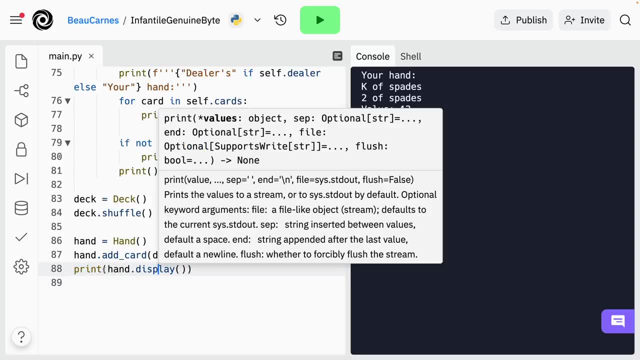 it's actually calculating that correctly, because that's 10 plus two is 12.. And then it's going to print none, which indicates that we did something wrong, which is that we did not need to print this because hand display display already prints. So now just call hand dot display, Okay. 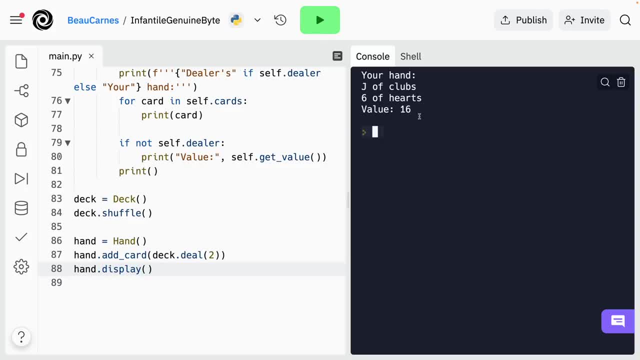 so now it doesn't put none or doesn't? Yeah, it doesn't put none at the end, So that looks right. Okay, when you're playing blackjack, you don't get to see everyone else's cards, So we're going to update this. So, when the dealer's cards are printed during the game, only the second one. 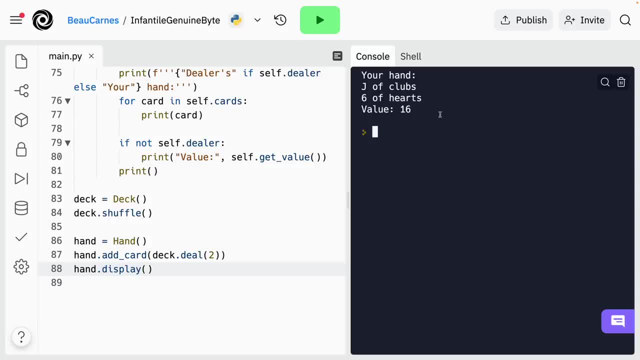 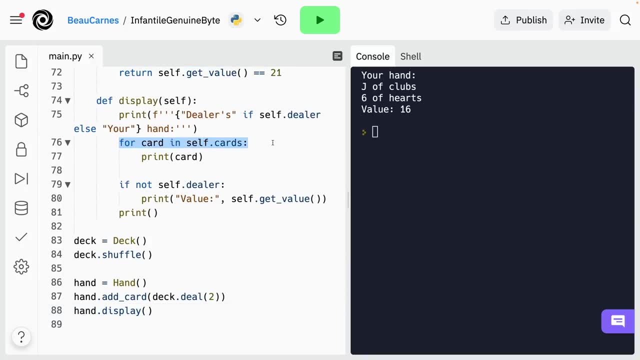 should display. the first card should display as hidden. So in this for loop, when we're displaying the cards, we're going to need to get access to the card index, since that will determine which to display, since we're only going to display the second card. So let's start by updating this. 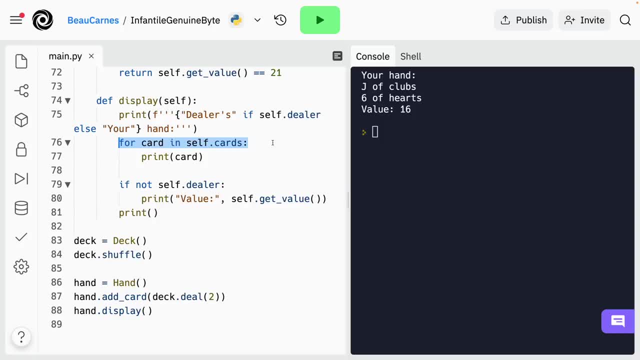 for loop So we can get access to both the card and the card index. We briefly touched on this earlier in the course. we're going to be using the enumerate function. So when I see for card in and I'm going to type in enumerate and I'm going to pass in self dot cards And this is going to 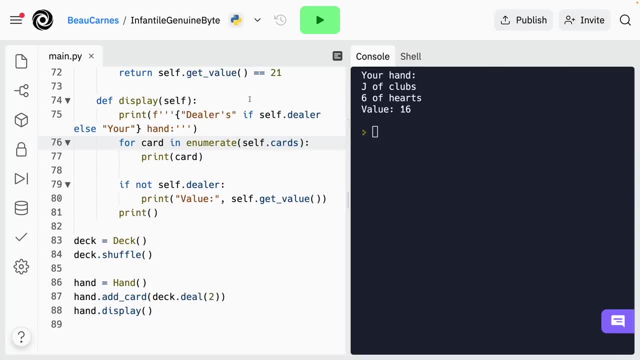 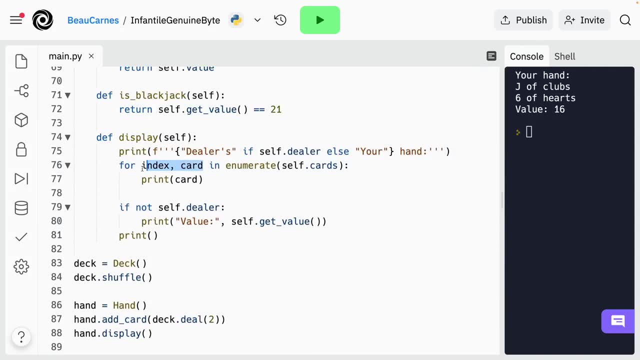 return the index and the card index, And this is going to return the index and the card index. So I'm going to type in index comma And so in we're getting the index and the card for all the items and self dot cards, And so now we just have to update what's in the for loop to print hidden. 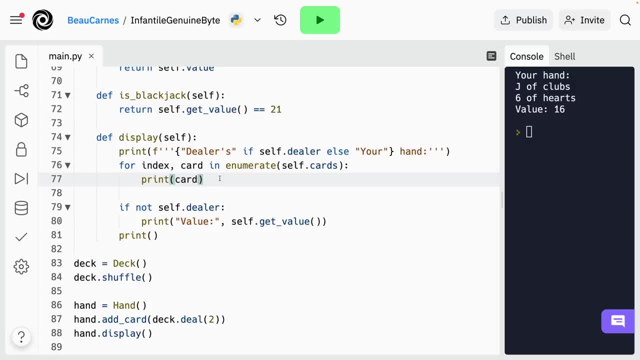 if it's the first card and it's a dealer, So we'll do. if index equals zero and self dot dealer, then we will print hidden And then we can use an else. And the other time- And let's make sure this lines up correctly- And the other time we will print the card. So what we did wrong. 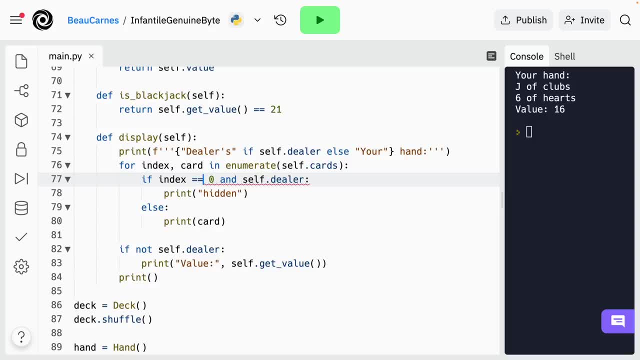 here is: this should be double equal sign. I did, almost did the. the main mistake you always have to watch out: never use a single equal sign when you're checking equality, because that's the single equal sign is the assignment operator. So if index equals zero and self and we, it is the dealer, then we'll print hidden. So 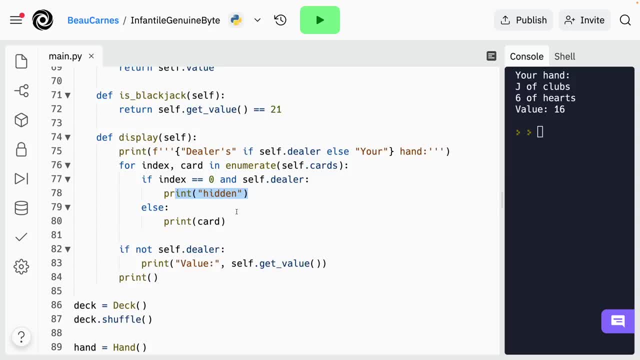 in our version of the game, at the end of the game that all the dealers cards will be shown, so you can see what the dealer had So to do that, we're going to create a new parameter in this display method And it's going to be called: show all dealer cards And. 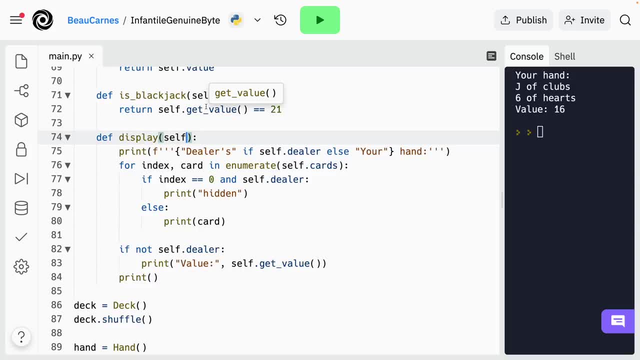 with underscores for spaces and we're going to set the default value to false- show all dealer cards- and when the default value is going to be false Now, we'll add it to this if statement. So we'll add another and not show all dealer cards. So 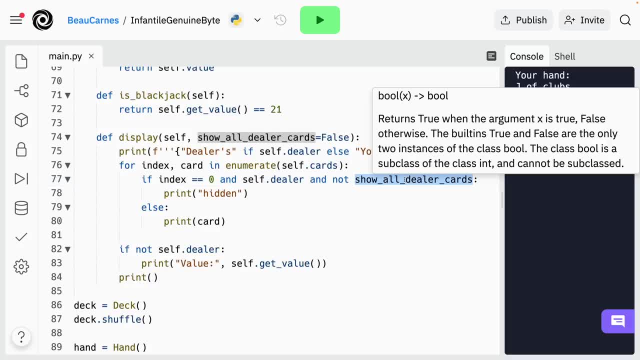 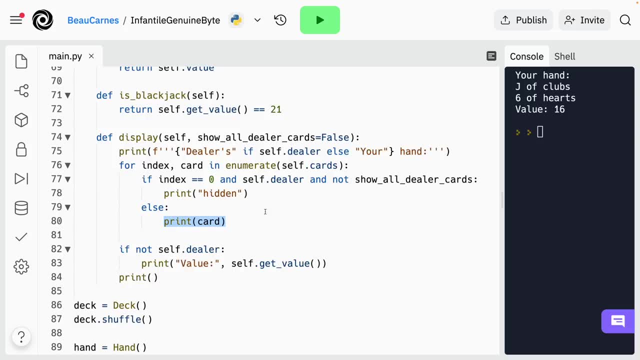 it's going to be hidden if we're not showing all the dealer cards. But if we are showing all the dealer cards and then this whole if statement will be false. so we'll just print the card. And there's going to be one other scenario where we're not going to print hidden if there's a blackjack. 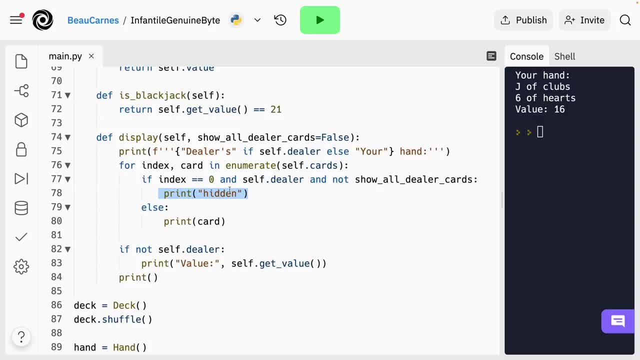 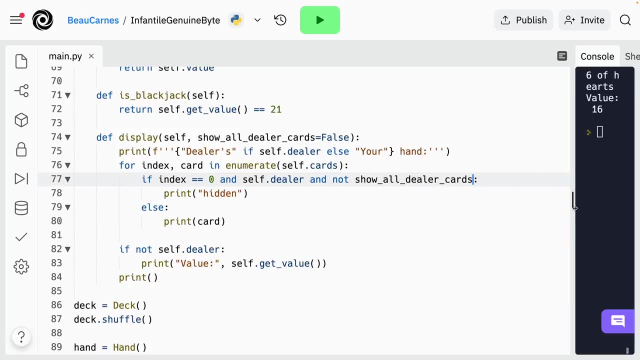 then the game is over. the person with the blackjack is just going to win, And then we'll just print all the cards. So we're going to add that to this long if statement here. So we'll say: and not is blackjack- And it should be self dot- is blackjack to be able to call this. 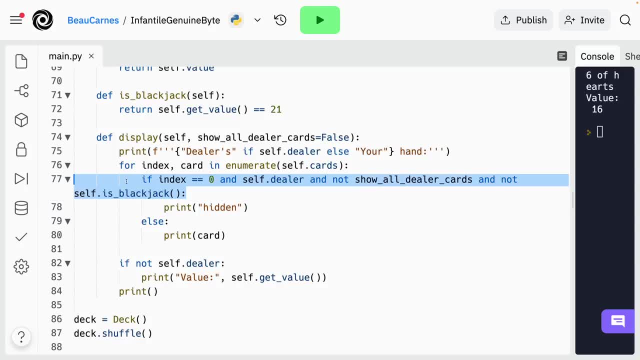 method here And since this is such a long line, is always going to go to this next line. we can do this special thing: We can add a slash here And then just go to the next line. So this slash or it's a backslash, I mean this backslash. 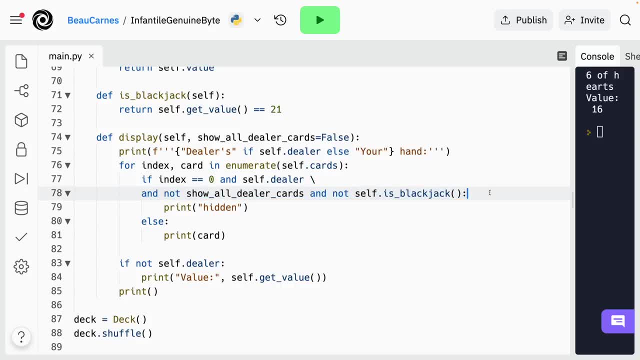 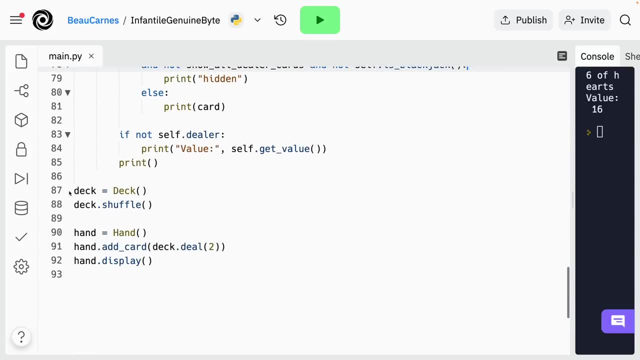 will indicate that the line continues on the following line: Okay, we're done creating the hand class, So we'll delete everything that we were using for testing before. Okay, it's time to code the final and longest class that runs the game. So what I want you to do is create a class. 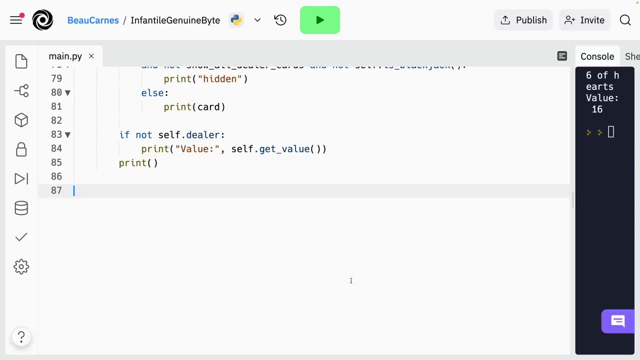 called game And inside the class create a method called play And inside the method create a variable called game number, with the underscore and then the class name And then inside the code for the space and set that to zero. So class game And then we'll create another variable. 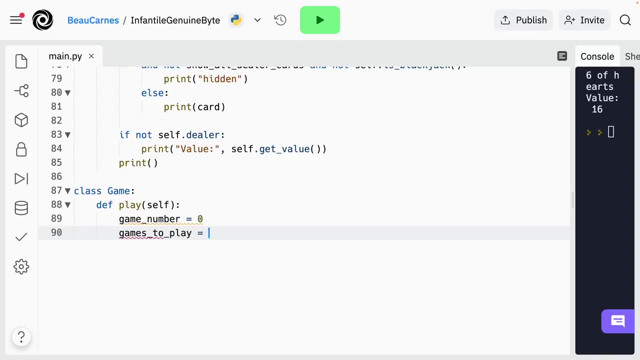 games to play and set that to zero. Now we're going to set games to play to be whatever the user inputs after they're asked how many games do you want to play. So you may remember how to do input from before. So we just do input Now we want to make sure. 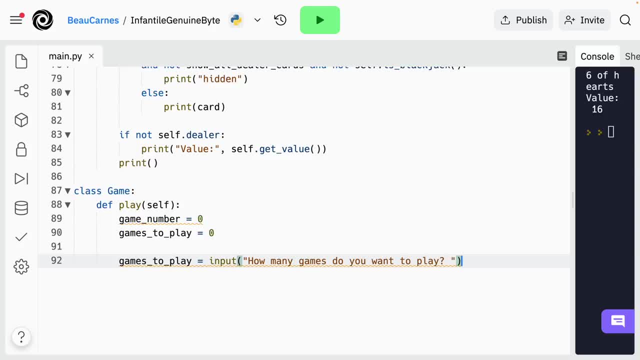 the games to play as an end. So you seem to convert this to an end. Okay, now let's test things so far. So at the end I will put G equals game. I'm going to create a new game and then G. 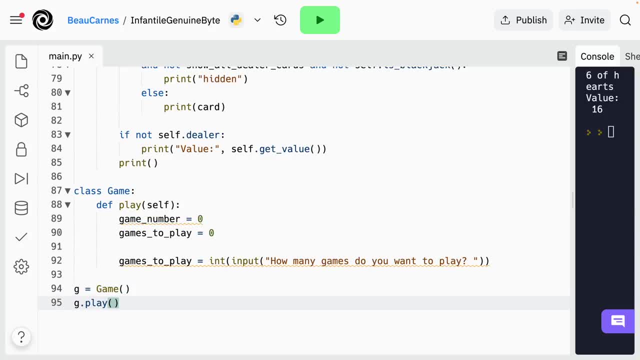 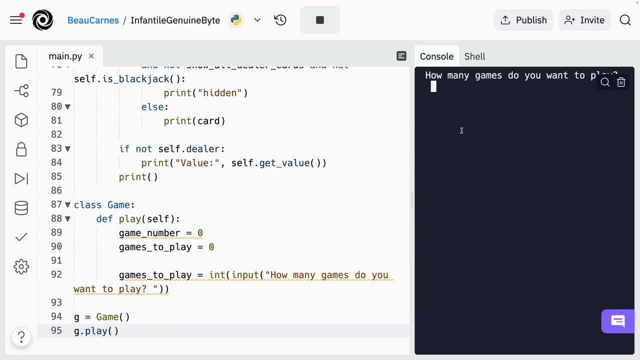 dot play. Okay, let's test this. How many games you want to play? Five, Okay, well, it's not gonna play the games that we still have to create that. So there is a potential for an error here If I do this again and I just put how many games I put you or some letter. 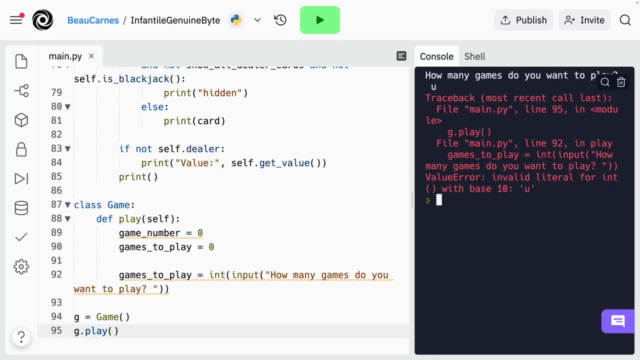 we're going to get an error. So basically, anytime someone puts something that's not a number is going to be an error. So let's create a try except block to handle the exception And if they put something that's not a number will print. you must enter a number. So let me arrange this. 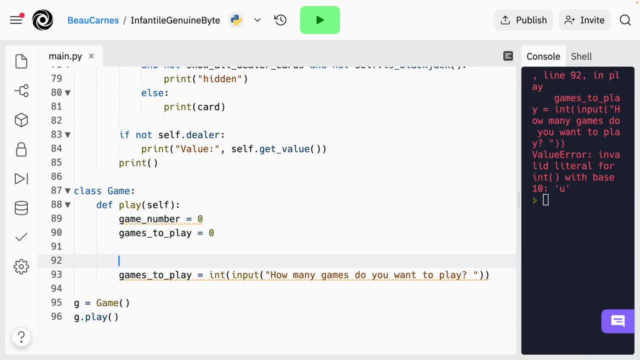 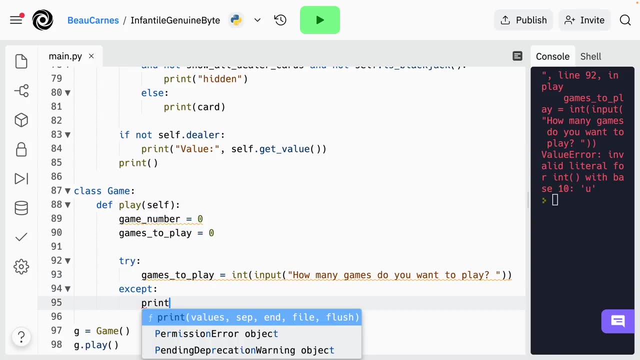 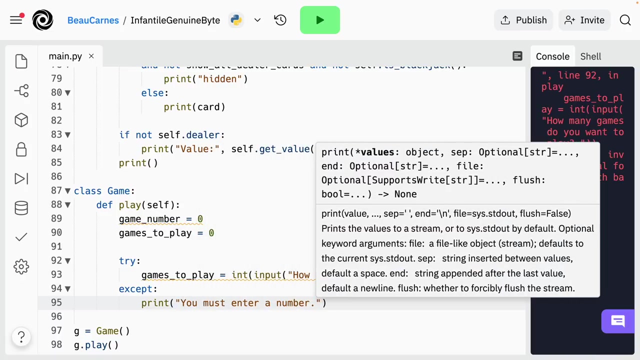 And we've already learned a little bit about try except blocks. I'm going to put try And it's going to try this, And then, if that doesn't work, if there's an exception, it will print. you must enter a number. So currently the user gets only one chance to input a correct value. Let's make 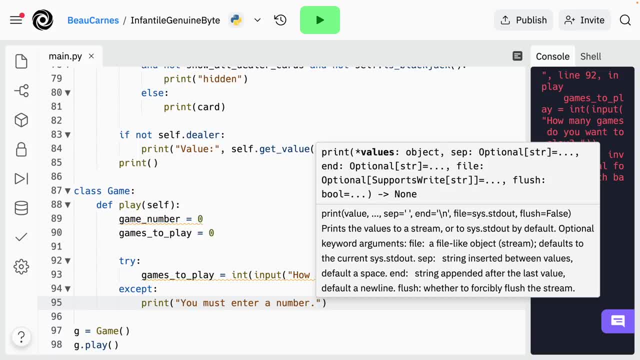 the program keep asking the user for a value until the user enters a number. This can be done with a while loop. The while loop just keeps looping while something is true, So keep looping until the user enters a number, by putting the entire try catch block into a while loop that keeps looping. 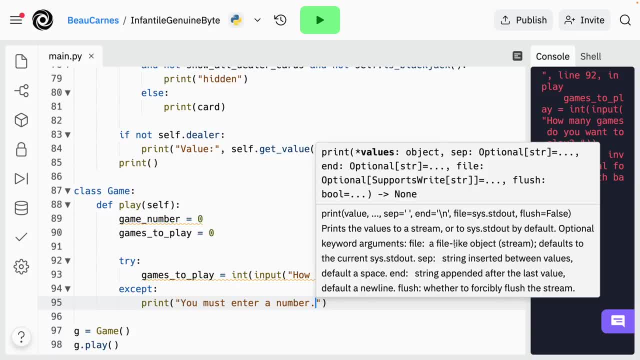 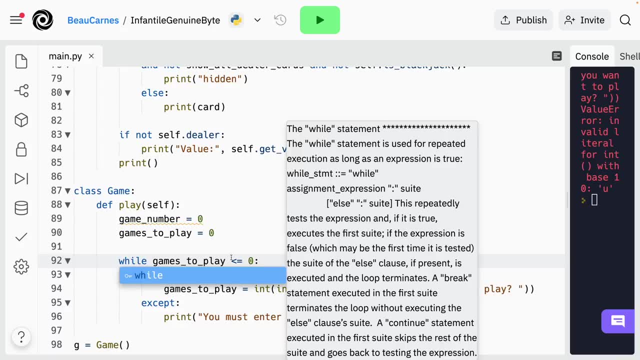 while the game's a play is less than or equal to zero. Oh, and I have to make sure I spell while correctly. Okay, now let's go back to the program. Let's go back to the program. Let's go back to. 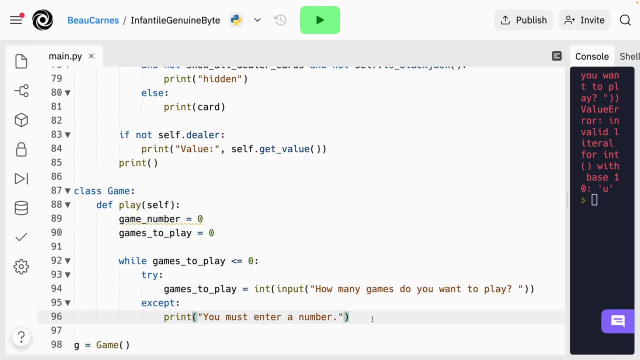 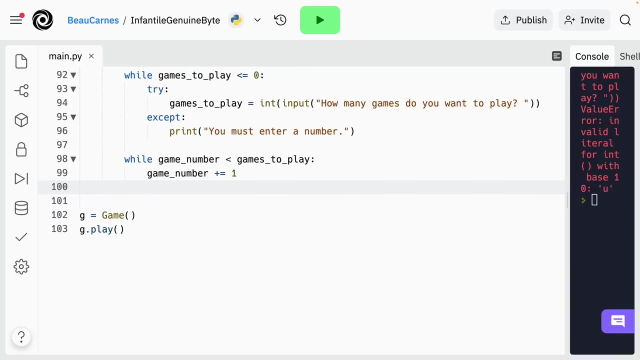 create the main game loop. This is a new loop that will loop one time per game played. It should loop while game number is less than games to play And the first line of loop should increment the game number by one. Inside the loop we'll create a deck object in a deck variable and shuffle the. 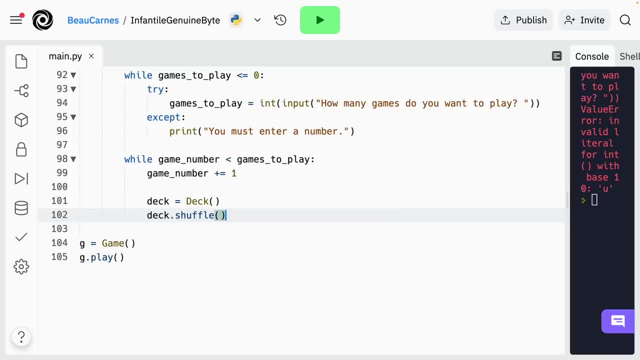 deck. Now we'll create a variable called player hand and set it to a hand object. And then we'll create a variable called player hand and set it to a hand object. And then we'll create a variable called dealer hand and set it to a hand object. But this time we'll make sure to specify. 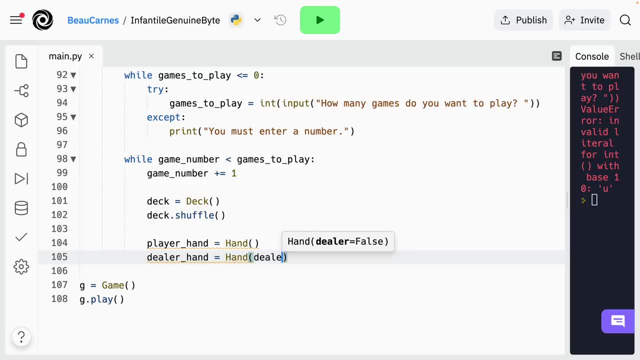 that dealer equals, true? Okay, this next part will be a little more complicated. we'll create a for loop that loops two times, And each iteration should add a card to the player's hand that is dealt from the deck and add a card to the dealer's hand that is also dealt from the deck. Okay, 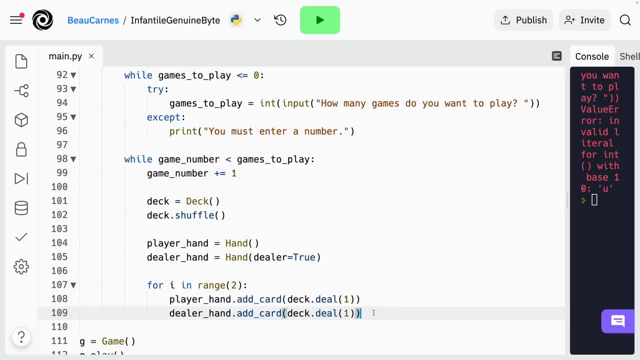 we've just dealt two cards And now we're going to create a loop that loops two times, And then we'll create a card to each player. Now, information is going to be printed to the console for each game, So let's start by printing an empty line. Now we'll print an asterisk 30 times to make a divider. 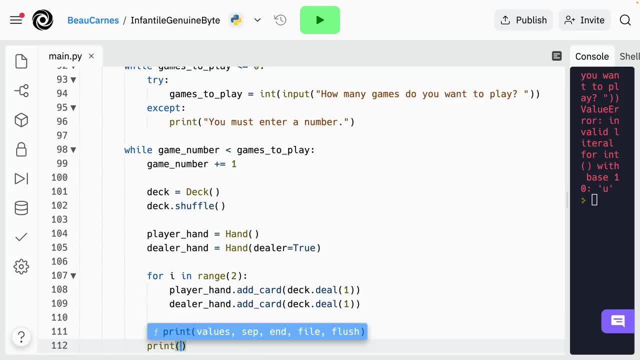 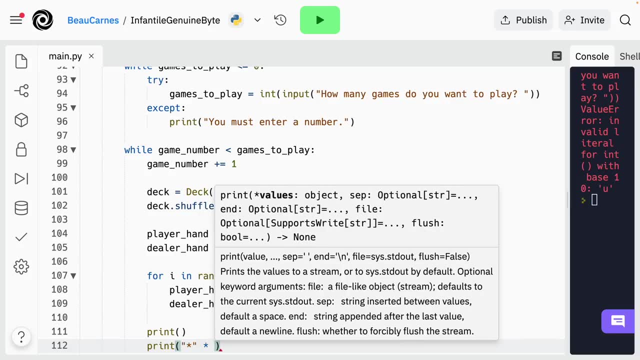 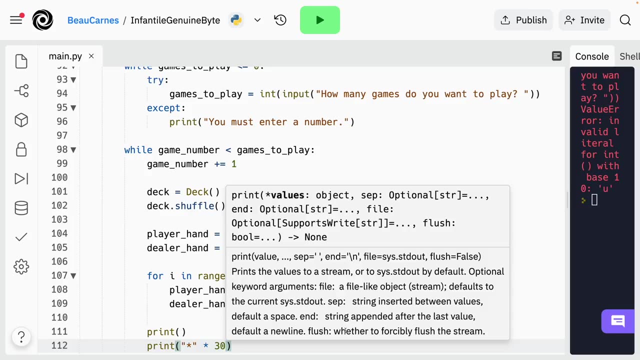 There's a trick to printing something a lot of times, So I can put an asterisk in in quotation marks and then just do times 30. So it's going to print it 30 times. Now we'll print the current game number out of the total number of games And then we're going to print the current number out. 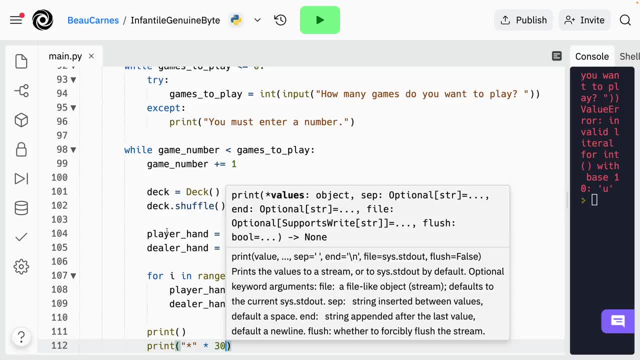 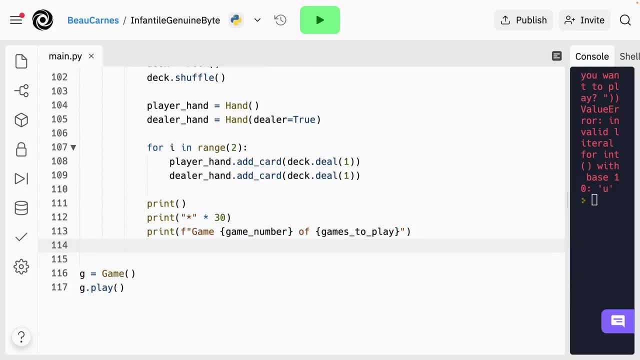 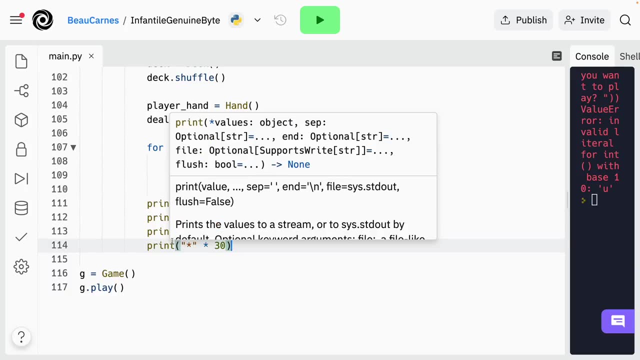 of the total number of games. So it will be something like game four of 10.. And we'll use an F string And then we'll just print 30 more asterisks. Now we'll display the player's hand And then the. 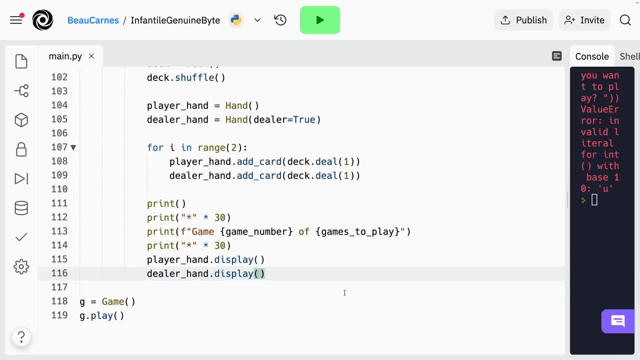 dealer's hand. At this point in the game someone could already have won if they got a blackjack. the code should check if there's a winner. Let's put the code to check if there's a winner And a separate method of the game class. So create a method called check winner, For now the method. 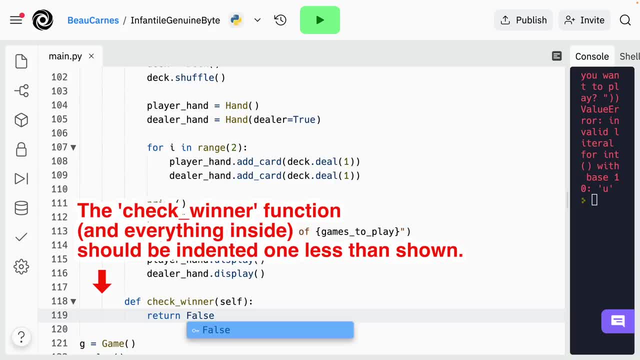 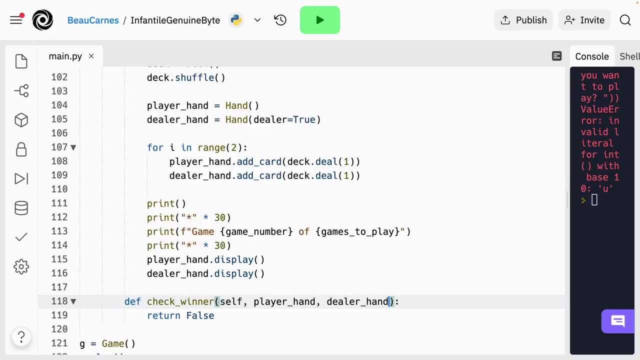 should just return false And just make sure everything's indented correctly. this should be less indented than the previous line here. The check winner function should take the player hand and dealer hand as arguments. Now, before this return statement, we're going to check if player. 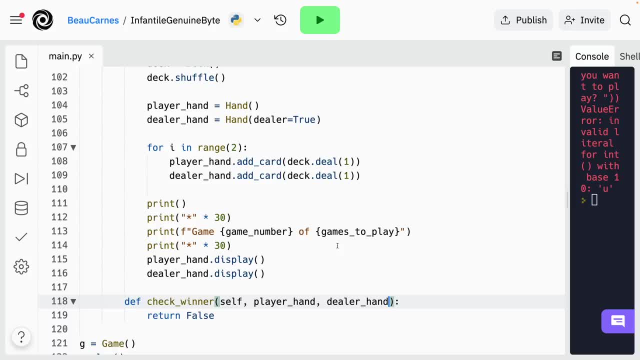 hand dot get value is greater than 21. And then we'll print the return statement And then we'll return true. If so, we'll print you busted dealer wins and then return true. And remember, once the program gets to a return statement, none of the following statements in the block are run. 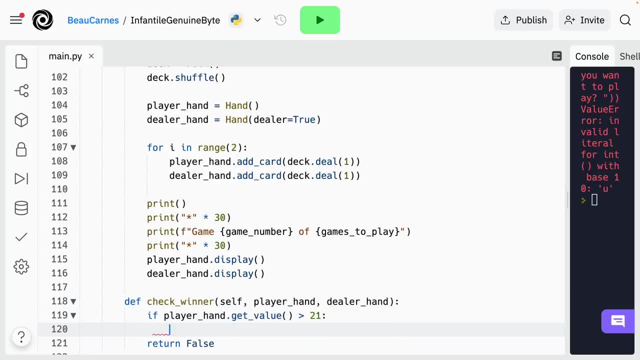 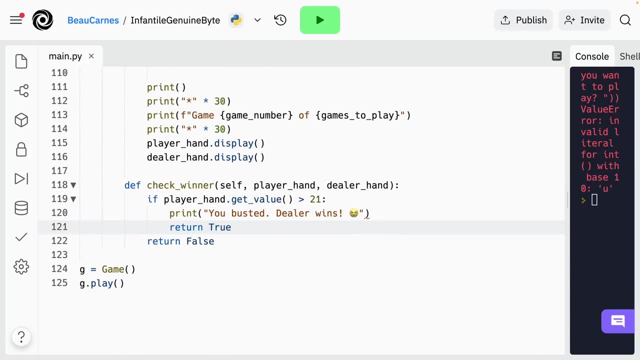 Now we'll use a few LF statements to check for various other conditions. So we'll add an LF statement to see if the dealer got over 21.. And then we'll print: dealer busted you win and then return true. And then we'll print: dealer busted you win and then return true. 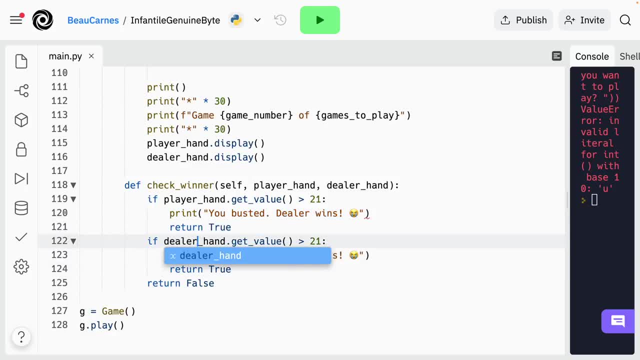 Oh, and I just copy all this. but this should be an LF, not if. And then we'll add an LF statement to check if both players have a blackjack. And then we'll print both players have a blackjack tie and then return true, And then we'll add an LF statement to check if player hand is a blackjack. 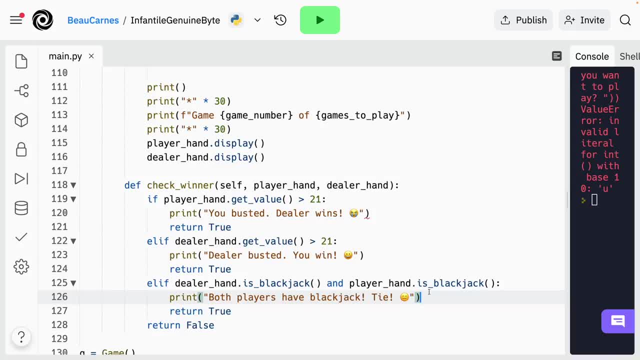 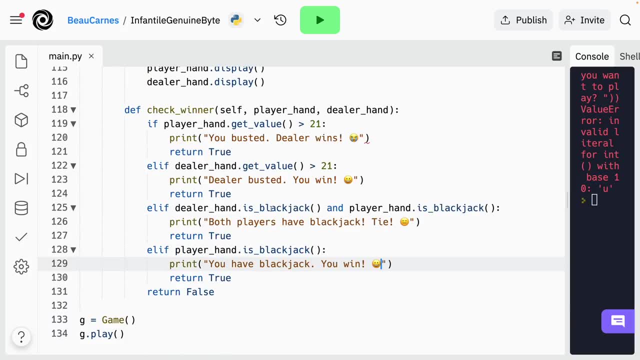 And then we'll print: you have blackjack, you win, then return true. And then we'll check if the dealer hand has a blackjack and then say: dealer has blackjack, dealer wins and return true. Okay, we're done with all the hand when conditions. 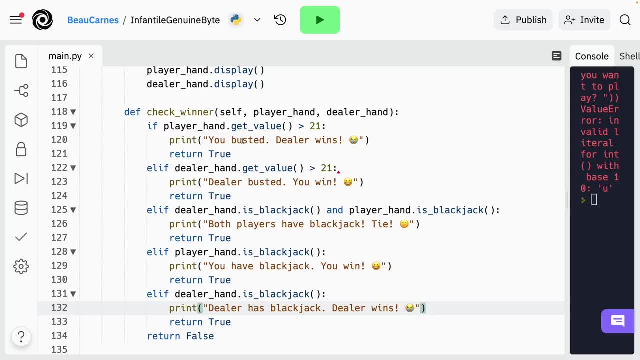 but the game can also end if both players choose not to get more cards. So we're going to add a new argument to the check winner method. with a default value it's gonna be game over equals false, So we'll add game over equals false. If it's true, that means both players have chosen. 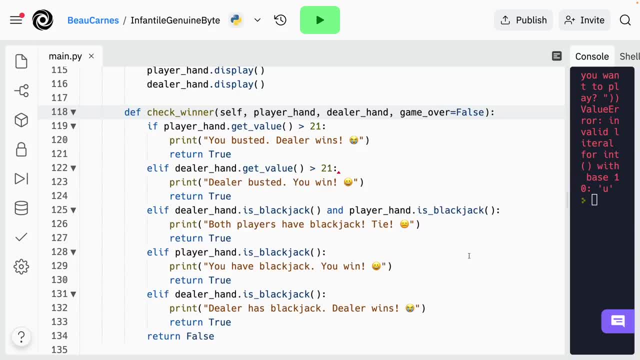 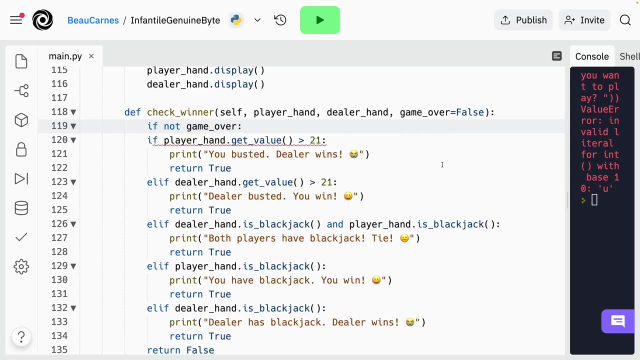 not to get more cards. Now we'll use the new argument: the string of if and lf statements should only be run if it's not a game over, And we'll make sure the line return false is not in the if statement. So here we'll say if not game over, and then I'll just select all these and put them in here. So if 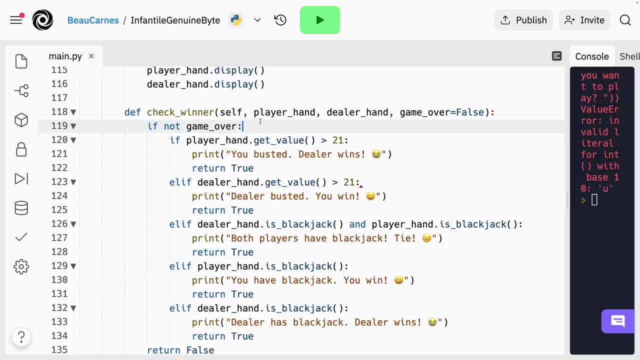 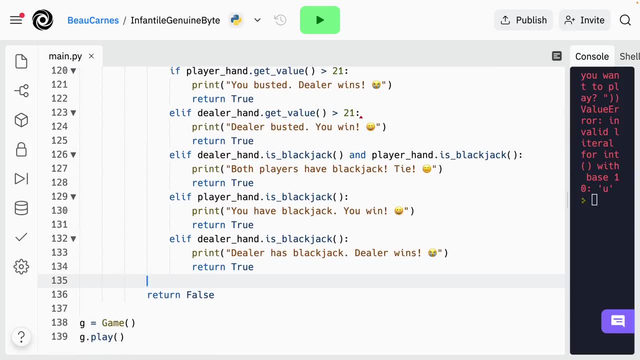 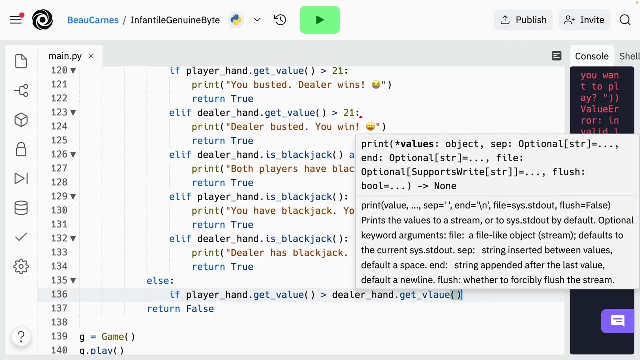 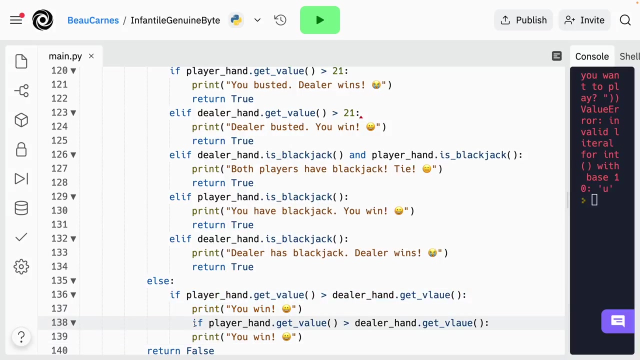 game over is true, we'll check if the player hands value is more than the dealer hands value And if so we'll print you win. So we can do this with an else here Else If player, And then we'll do an lf, for if it's a tie, So this is an lf And we'll say if these are equal to. 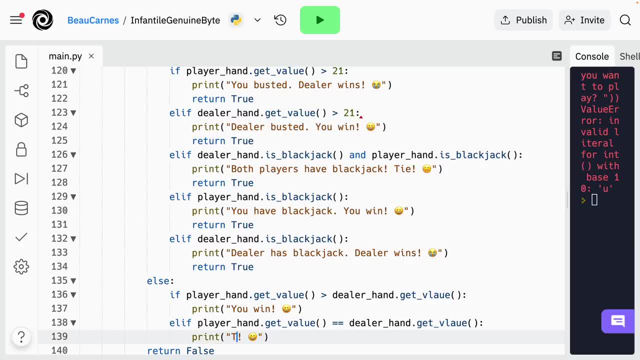 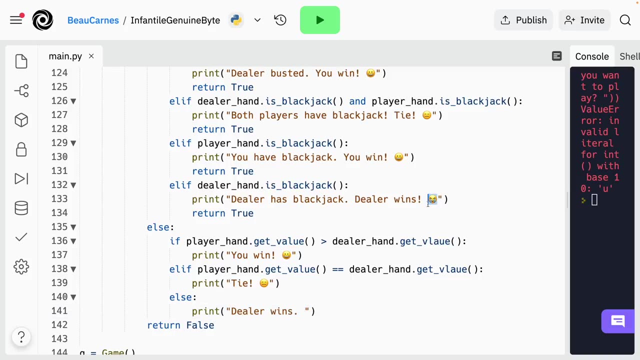 each other and we'll print tie. Then make sure we have the correct emoji for a tie And then else the dealer is one, So we'll just do else And then, at the exact same level of indentation as the else we just added, we'll add return: true. 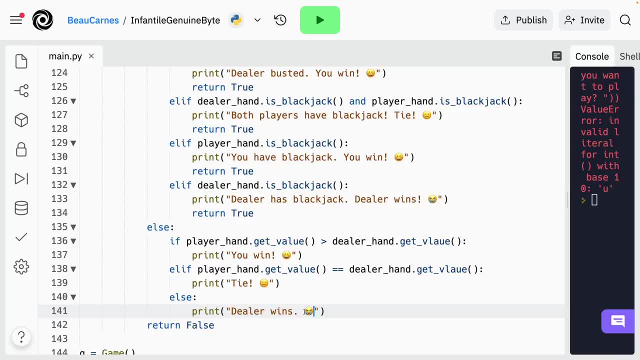 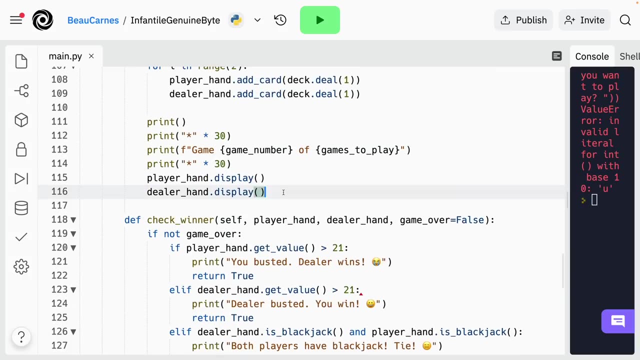 this will make the method return true if game over equals true. Now let's go back to the play method inside the while loop And then we'll do an if statement And we'll do if and then we'll call the check. winner function with the player hand and the dealer hand. So let's go back up here. If self check. 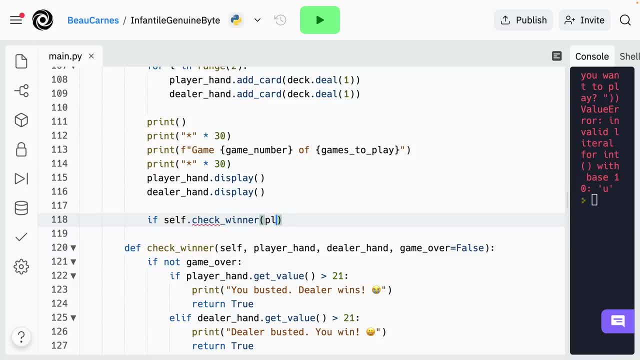 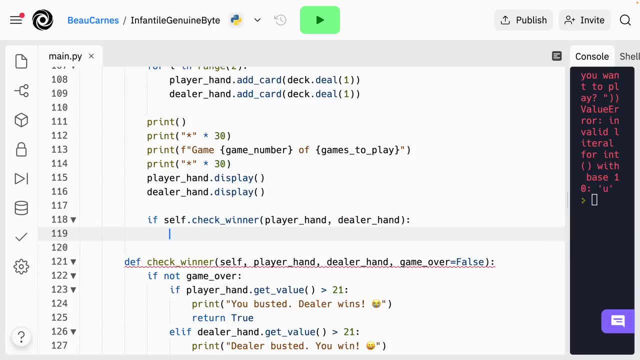 winner and then we'll enter the player hand and the dealer hand. So if this is true, that means we should go on to the next game To do that. we do continue. So continue is going to just go to the next iteration of the loop, And the loop we're on is this loop. So when we go to the next iteration, 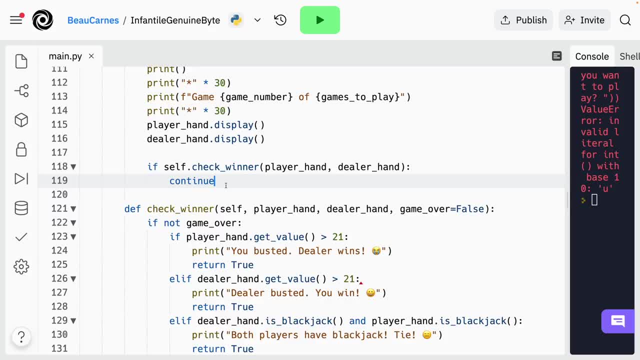 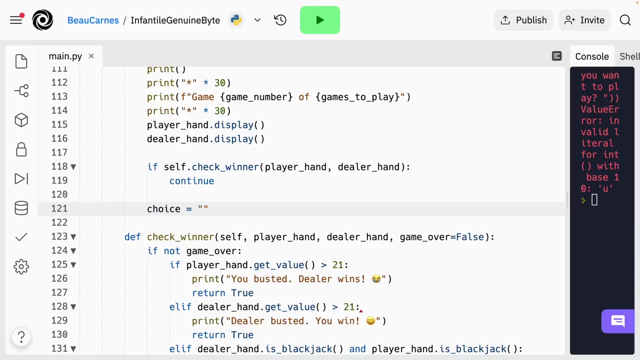 we start a new game. At this point in the game the player will be able to choose hit or stand. So inside the while loop, but not inside the if statement we just added, we'll create a variable called choice and set it to be an empty string. The player should be able. 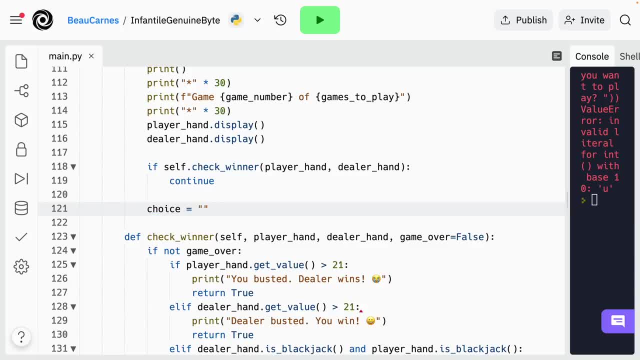 to keep choosing until the value of their hand is over 21.. So right under the choice variable we'll add a while loop that loops while player hands value is less than 21. And inside the loop we'll add a line to get the choice That's either going to be hit or stand. 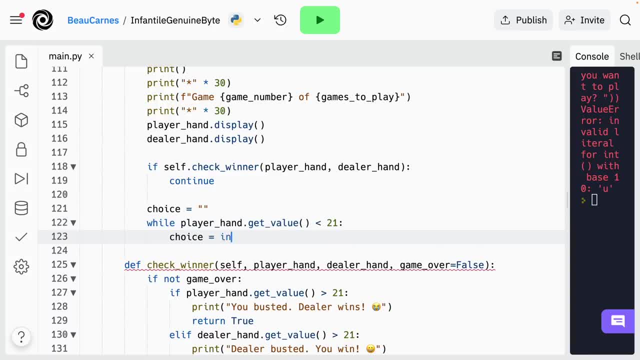 And then we'll just add this to convert. whatever the answer is. whatever the user put in, we are going to convert it to lowercase. The while loop we just added should also stop if the user's choice is stand or or s, So we'll update the line that starts the while loop to 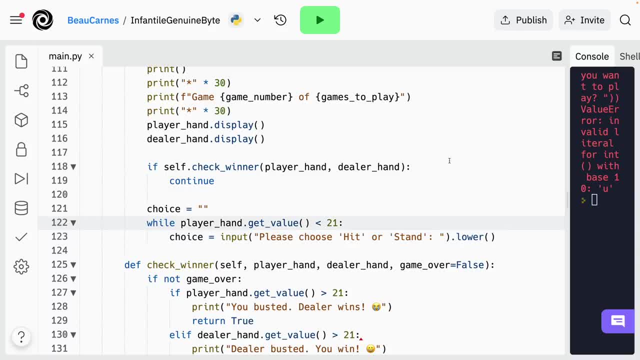 also stop. if the choice isn't s or stand, So just do and choice, Not in. And this is there's a few ways to do it, But this is kind of a new way that I'm just showing you here. So we are checking if choice is not in this list And inside the list we have two. 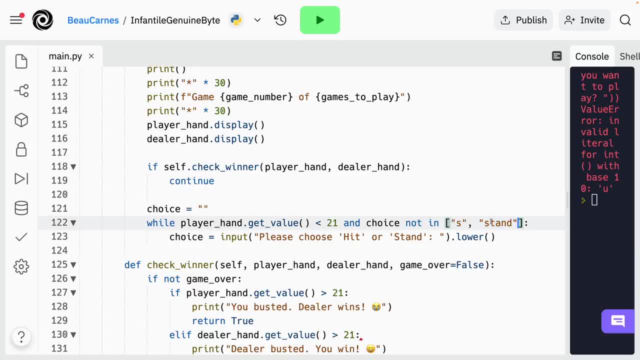 elements s or stand. So if choice is not in that, if the choice is not s or stand, then we'll continue the loop And then after the input, will print an empty line. Also, we want the program to keep asking the user for choice until the user enters a valid choice. The 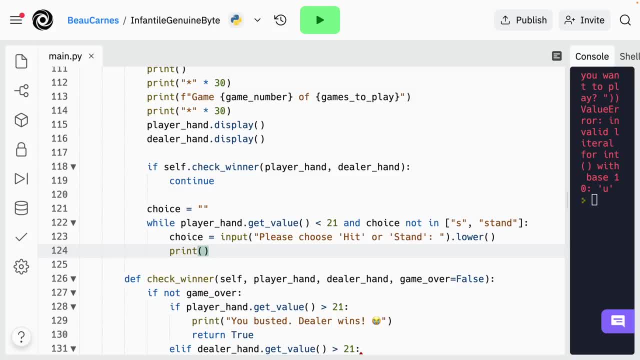 valid choices are h, s, hit and stand. So right after the last print statement, at the same indentation, we'll add a while loop that will keep looping until the user enters a valid choice And inside that while loop we'll ask for input again. but we'll specify it can be h or s as well. 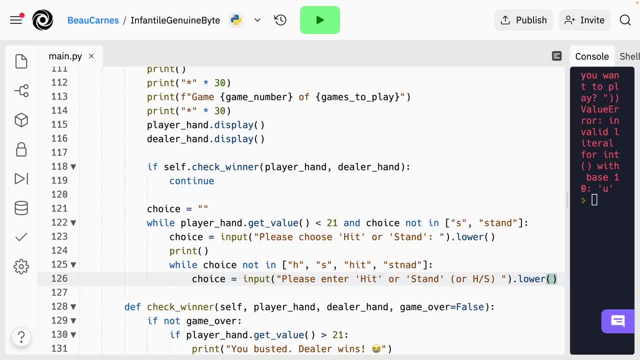 So this is going to look very similar to this line, but it's going to kind of clarify things just a little bit And then we'll print another empty line, The last while loop. we checked if choice was not in a list outside of the recently added a while loop, But inside the loop we just 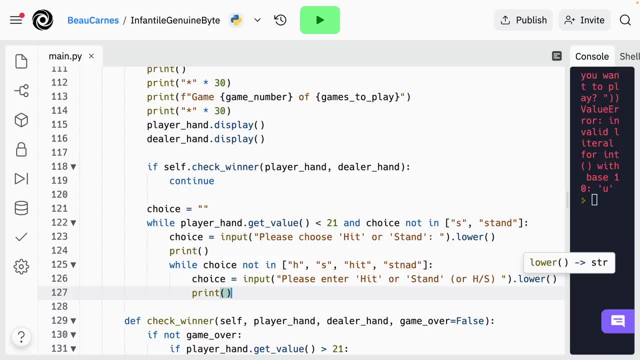 added before that one. we'll add an if statement to check if choice is in the list hit or H, And if so we'll add a card to the player's hand. And then we'll add a card to the player's hand And. 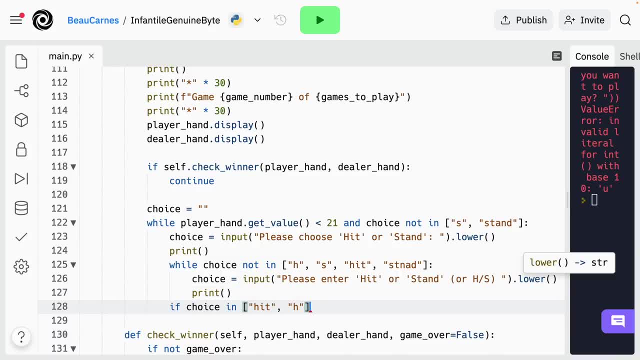 that is dealt from the deck And then right below that will display the player's hand Outside. all the while loops about the player making a choice. we'll check for a winner. we'll use the same if statement continue, statement that we use last time. we checked for a winner, So I'll just copy this. 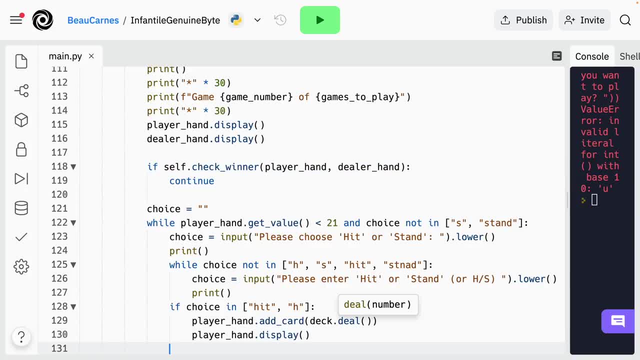 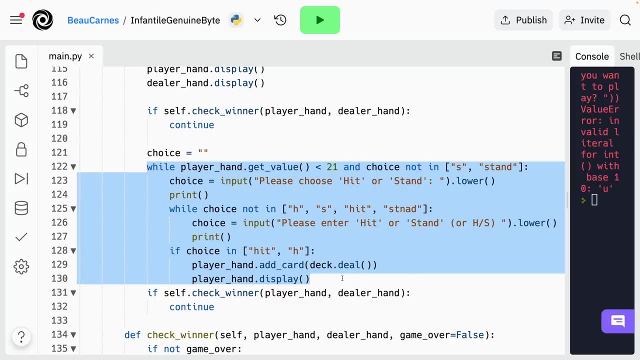 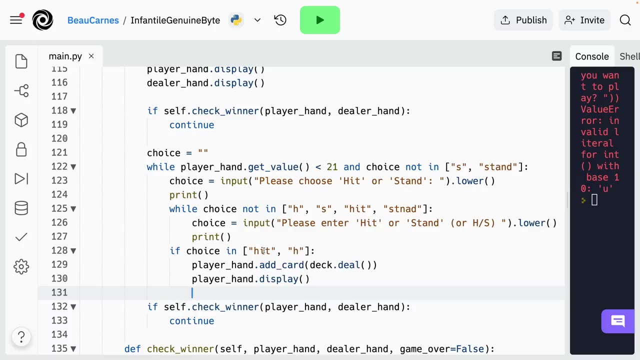 And then we have to make sure it's lined up correctly. Okay, so this is outside of this while loop. So after this all is all done, we check for a winner. let's just add an empty line there to make it more clear that the while loop is over. Now we'll store the value of the player's hand in a variable named. 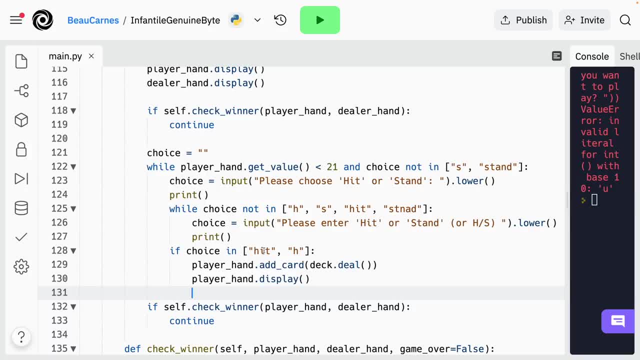 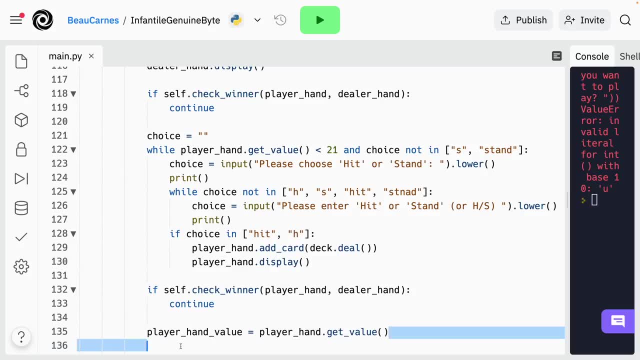 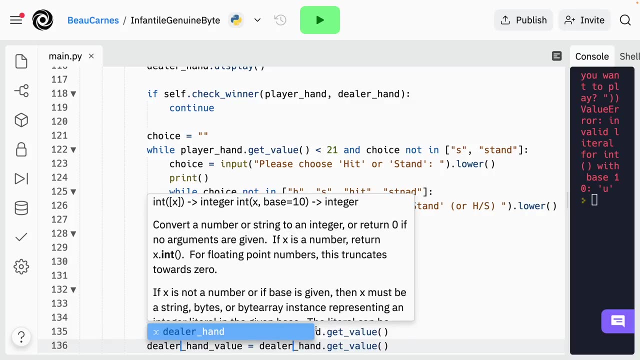 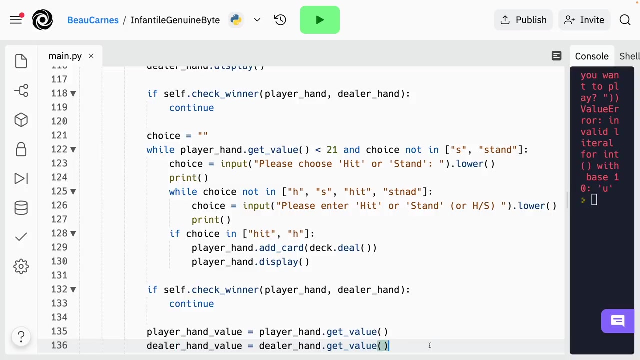 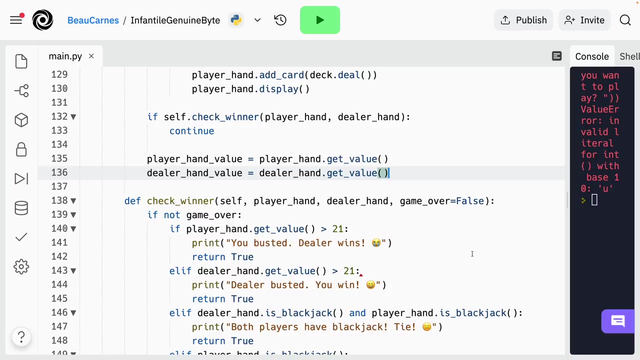 player hand value with underscores for spaces, And we'll do the same thing with the dealer's hand. Remember, I could use the command D or Ctrl D to select two words at once and change them both at the same time. Okay, the dealer should keep drawing cards until dealer hand value is more than 17.. So we'll make this happen. 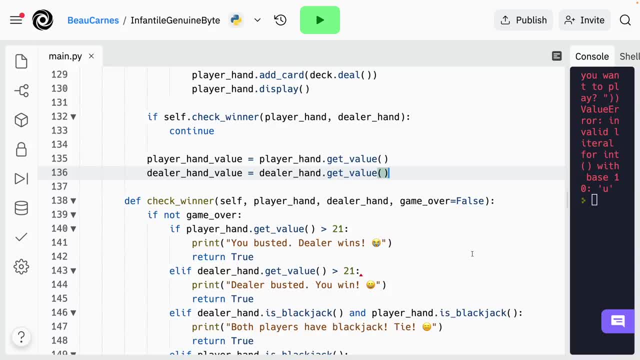 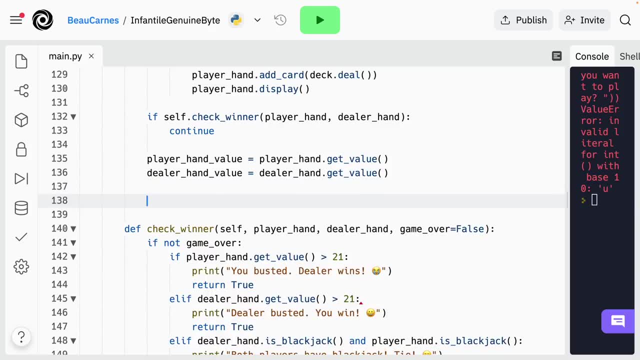 with a while loop And inside the loop we'll make sure the dealer is Delta card from the deck and that dealer hand value is updated. So you can try that yourself. but I'm gonna show you right now while dealer hand value d. 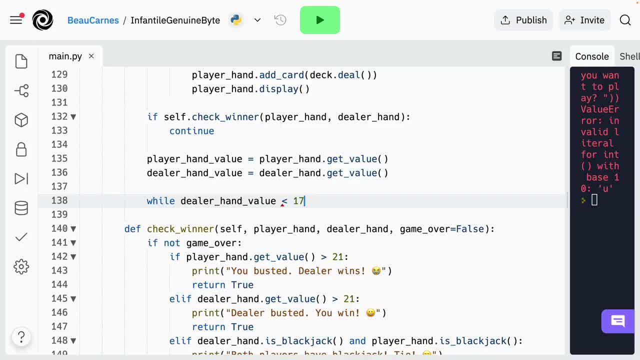 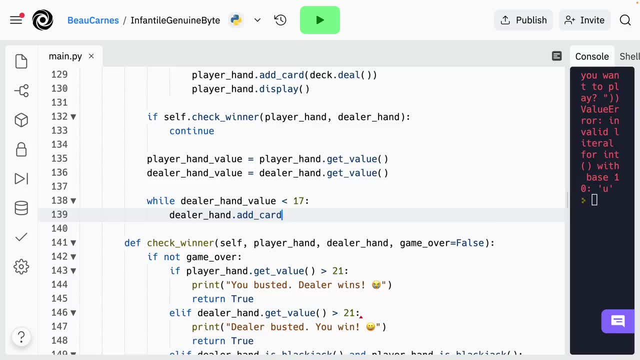 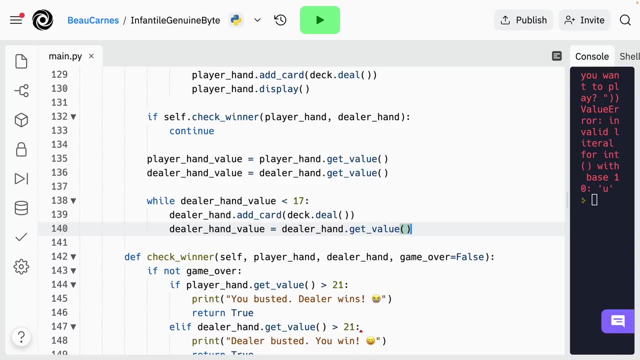 value is less than 17.. Then we will do dealer hand dot, add card Okay, and after this while loop we'll display the dealer's hand And when we call the display method we'll make sure to set show all dealer cards to true. And since it's the end of the game, that's why we're just showing. 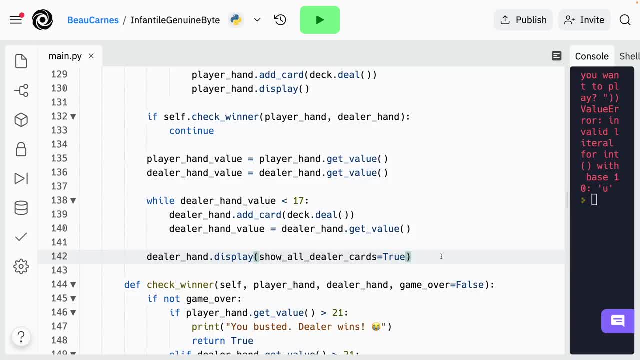 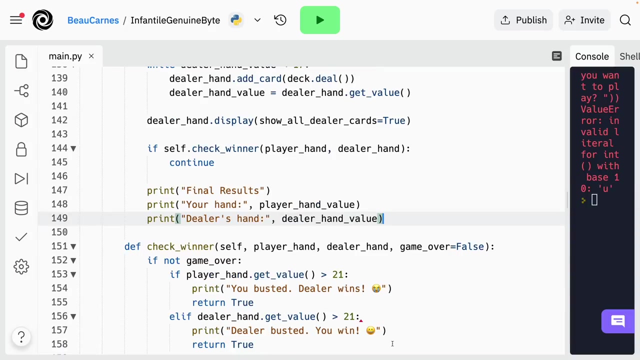 all the cards. Now we'll check for a winner just like before. Then we'll print final results. Then we'll print your hand colon and then the player hand value And then the dealer's hand. Now we'll call the check winner function one final time, But this time it should not be in. 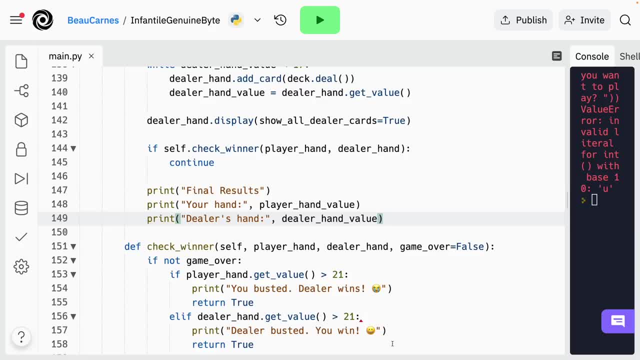 an if statement And we'll pass in the hands like before, But this time we'll add a third argument of true to indicate that the game is over And at this point in the code the game is over. So outside the outer while loop and in the play method we'll add the final line of seven. 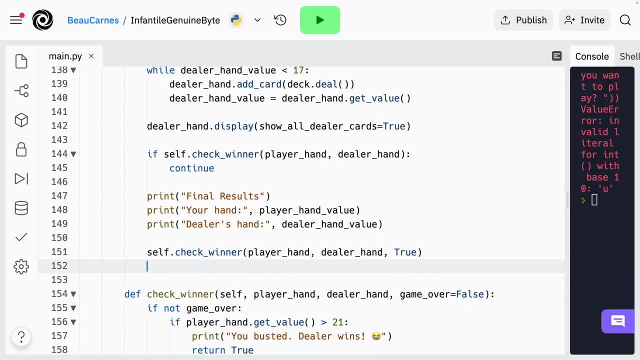 saying Thanks for playing. So it's going to be outside that while loop and we'll put print And just to demonstrate it I use an escape character to add a new line. So this slash in is going to add a new line and then do things for playing. And when I line this up for with 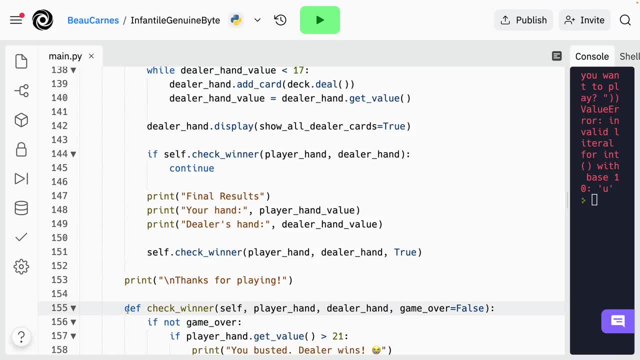 the while loop, I realized that this entire function should not be lying lined up with the while loop. Sometimes it gets tricky with figuring out the exact right indentation, So if I kind of go up straight up here I should say: see that this should be lined. 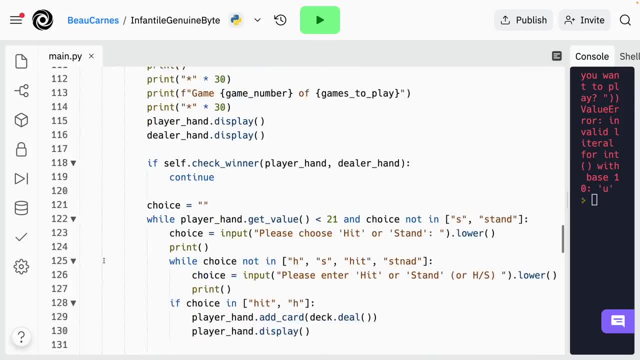 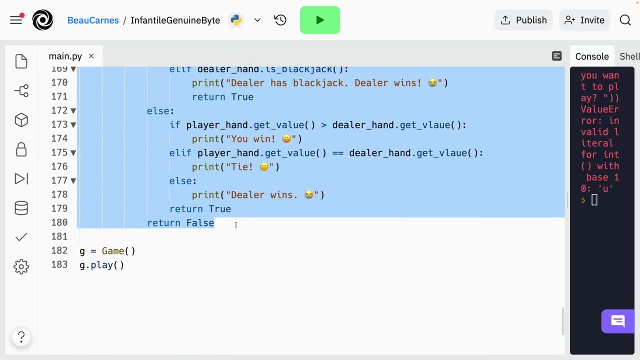 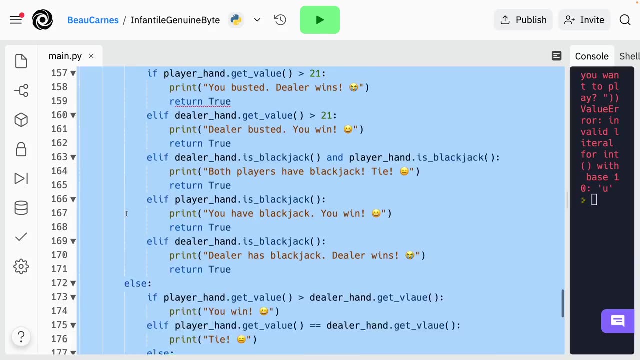 up with this play function. So I'm going to come back down to this function, I'm going to copy this all And I'm just going to do shift tab to indent it all one less. This happens to be the same as sometimes when writing Python code. sometimes the indentation can get all mixed up, But that 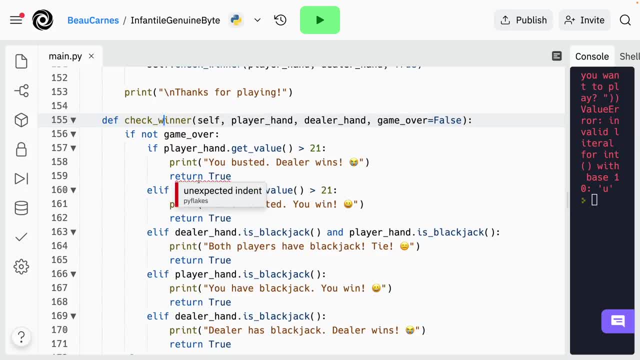 should be correct now And I think the red squiggly lines here on the return true are not a mistake in the code but a mistake in the error checking because it comes after that emoji and it doesn't know how to handle the emoji. But it's perfectly fine for code. 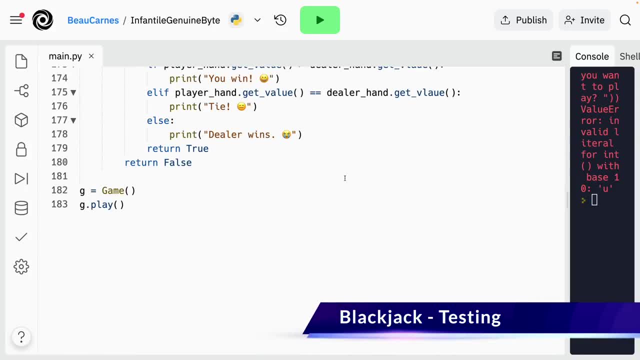 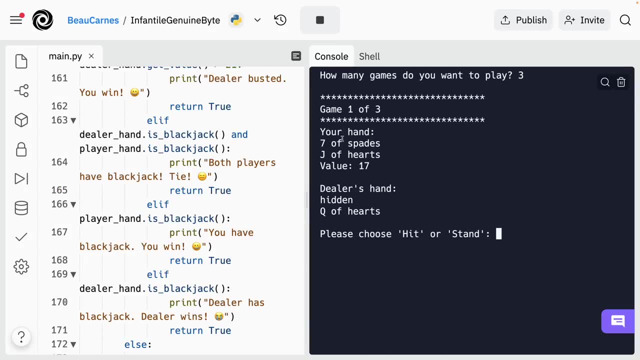 to have emojis. Okay, let's run the program and try it out. So press play. How many games want to play? I'll do three, So game of one of three, So I can see I have 17.. I don't know what the dealer has. 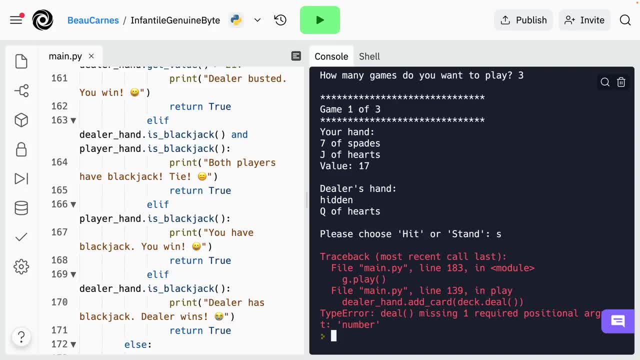 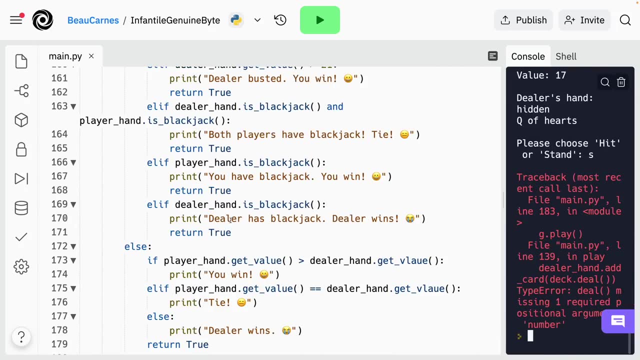 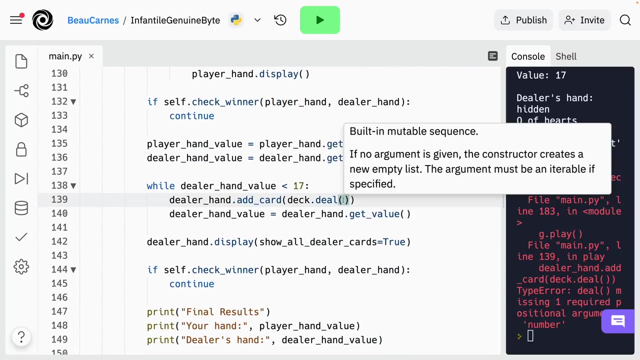 but I'm going to s for stand. Okay, it's always good to test. So it says: deal is missing one required positional argument. So let's go up to. it says line 139.. So this can kind of help us know where to go. So let's go up to 139. And yeah, I want to deal a single. 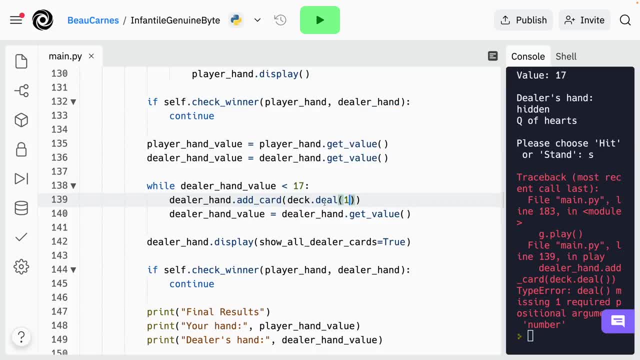 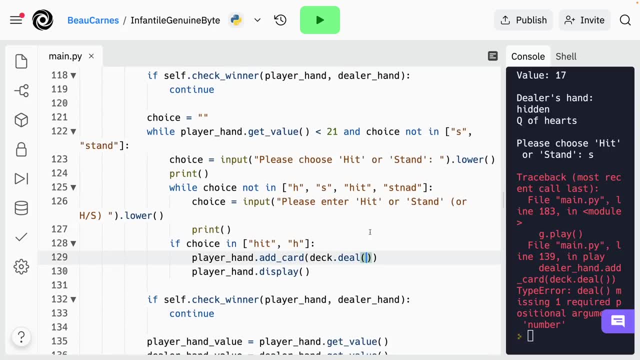 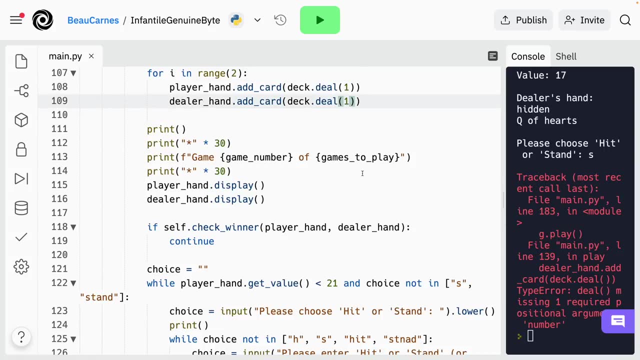 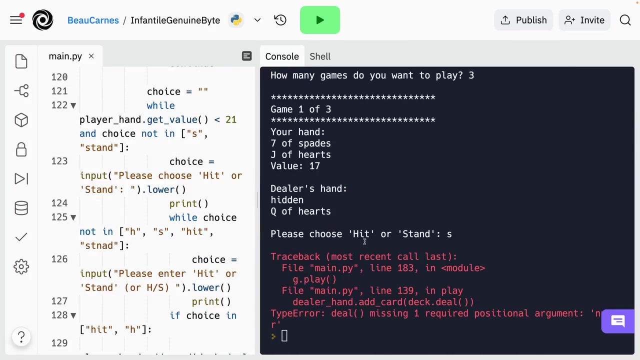 card. So I'm gonna deal one card here And were there any other times I did use deal. I went to deal one card here And I got the deal one up here, So I just think I just forgot the deal one in those places. So, thanks to these error messages, whenever you have a 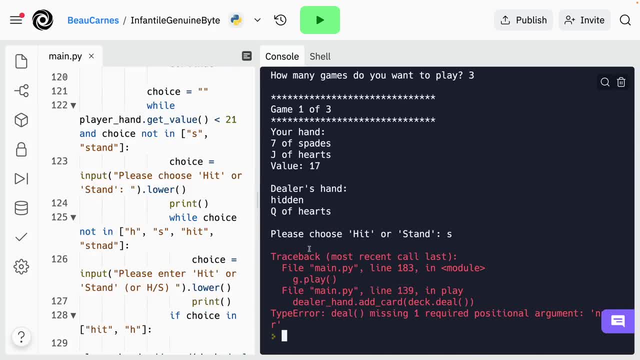 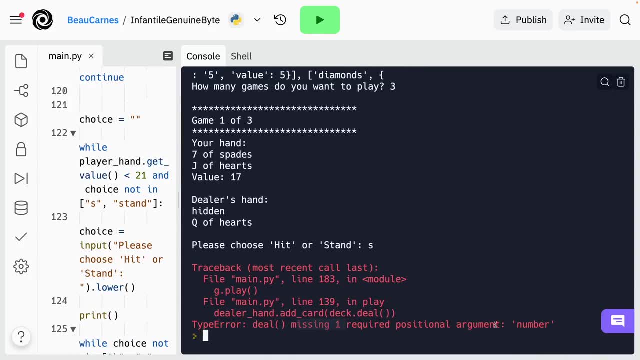 problem. make sure to read the error messages And it can often give you a a very good idea of what you need to do wrong because even says deal is missing one required positional argument: the number. So that can really help figure out what's wrong with your. 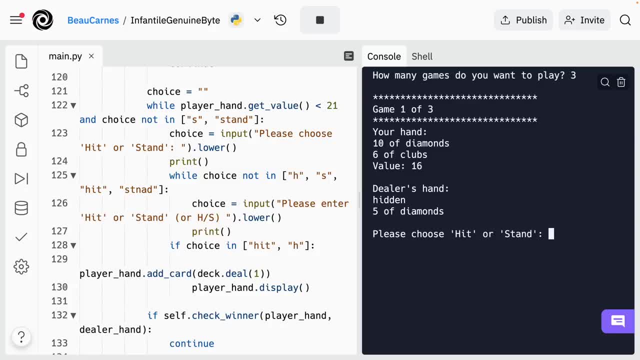 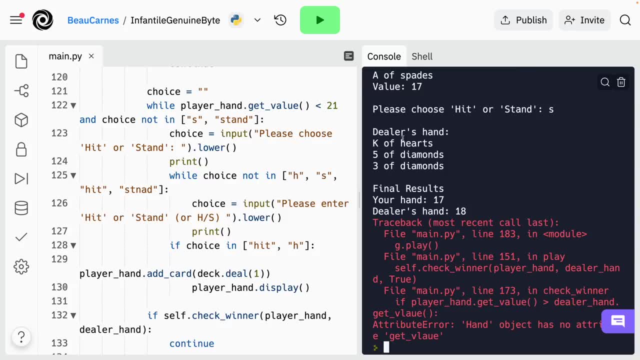 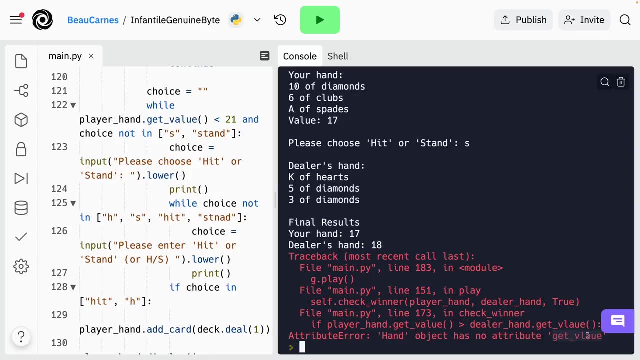 code. So let's try that again. We'll do three games And then this time I will hit and I'm going to stand. Okay, so now we have another error. So it says 173.. And oh, I can already see this is spelled wrong. So let's go to.